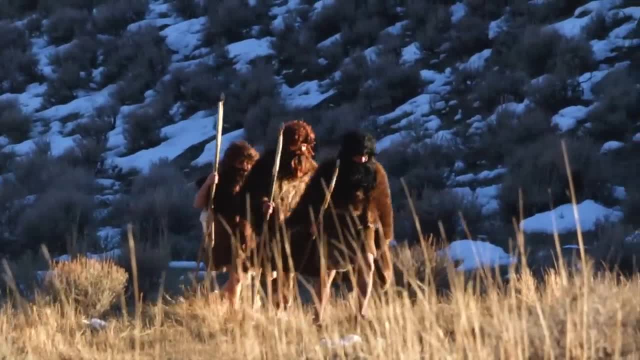 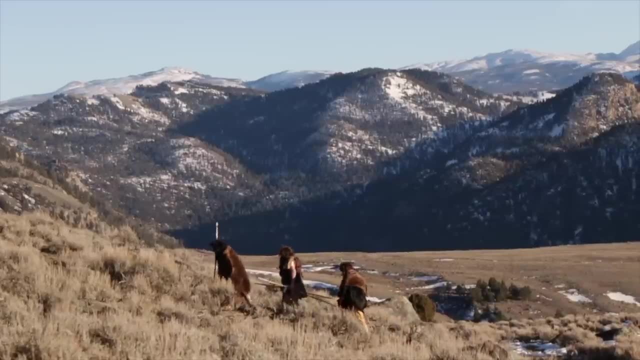 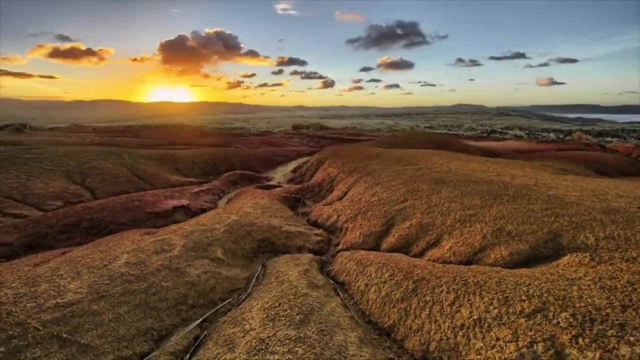 Neanderthals, our closest extinct relatives. They have long fascinated us with their enigmatic presence in our evolutionary history. They roamed from the frozen tundra of Northern Europe to the arid deserts of the Middle East. for hundreds of thousands of years They left behind extensive 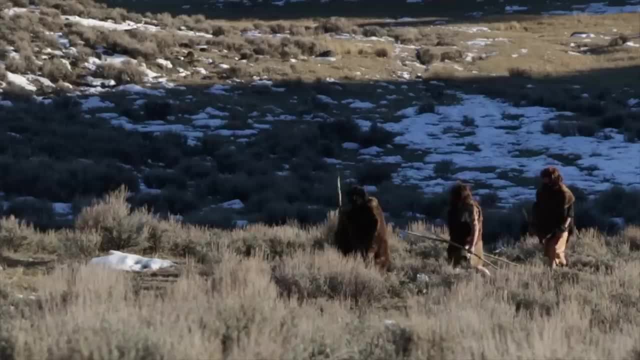 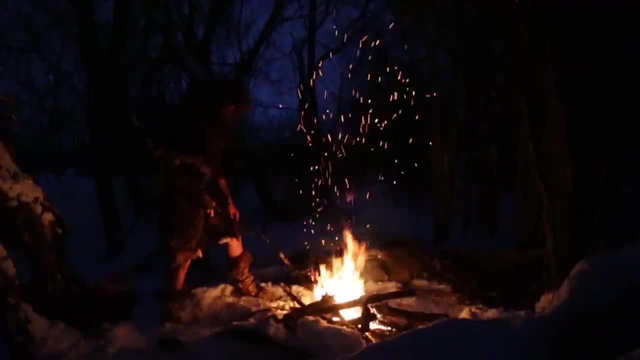 records of their complex tools and way of life. Then, in a relatively short amount of time, they vanished from the fossil record. In this documentary, we delve deeper into the world of Neanderthals, exploring the latest scientific discoveries and theories about their biology. 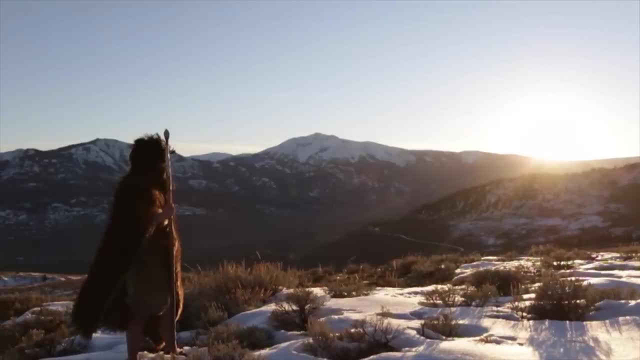 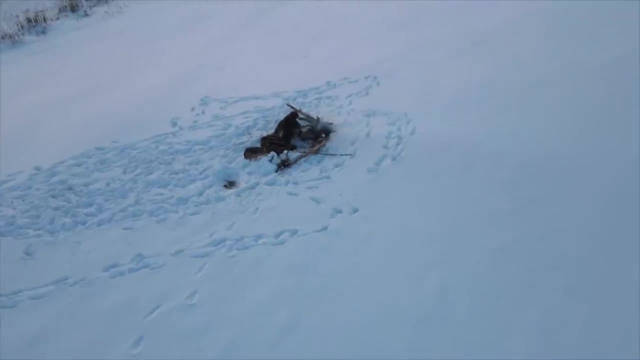 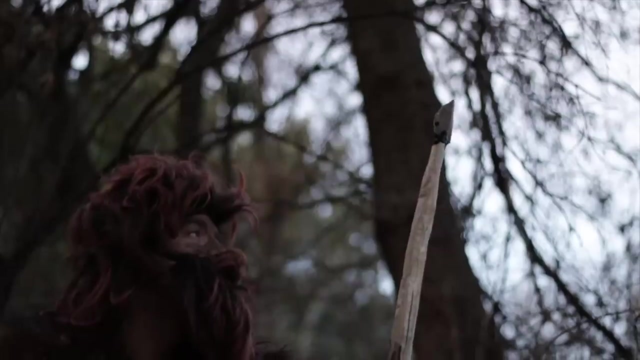 behavior and interactions with modern humans. With the help of scientific literature and a paleoanthropologist, we will seek to answer some of the most intriguing questions about our distant cousins. Who were the Neanderthals? What kind of world did they inhabit? What made 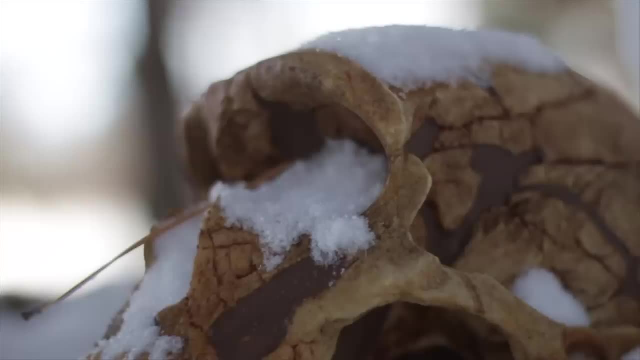 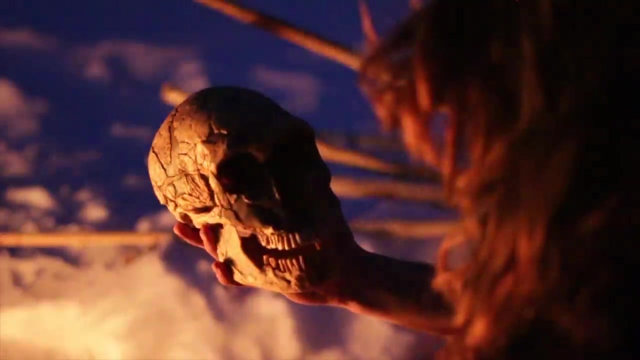 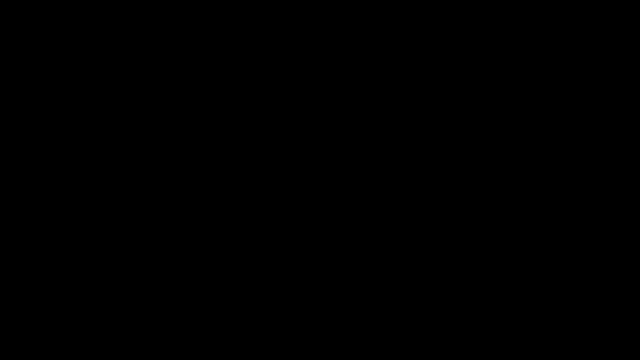 them different from us? What did we have in common And, ultimately, what led to their extinction? Join us as we unravel the mysteries of the Neanderthals and discover what their story can teach us about our own origins and place in the world. The story of the Neanderthals is inseparable with the larger 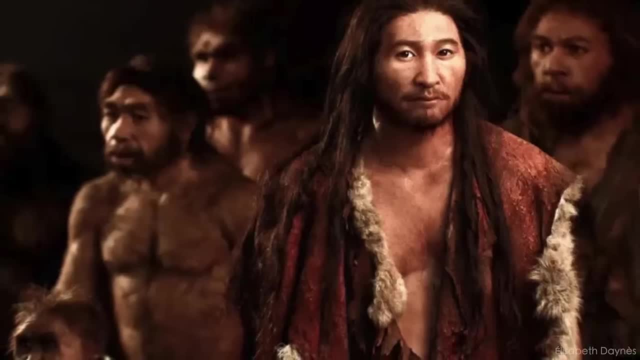 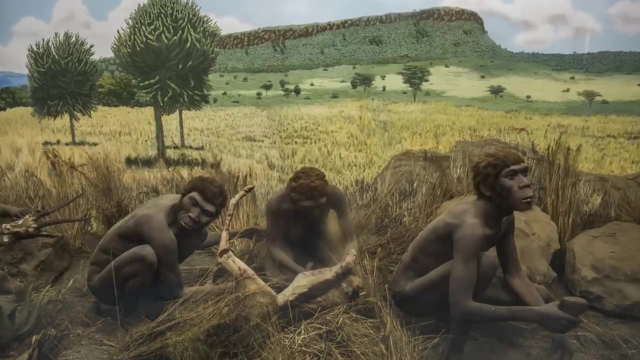 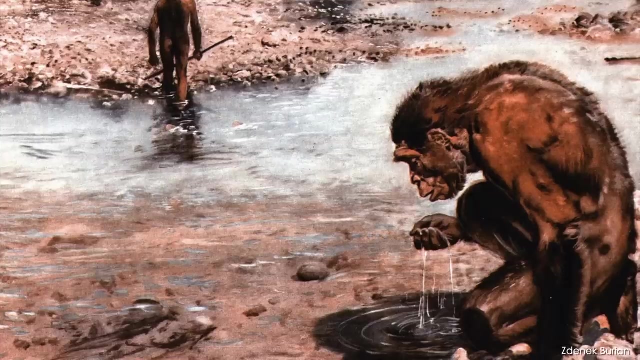 picture of human evolution. Neanderthals, modern humans and another dozen species make up our genus. Homo First appeared in Africa nearly 3 million years ago. These distant hominins descend from Australopithecines. Australopithecines were a quite successful genus of bipedal ape that lived. 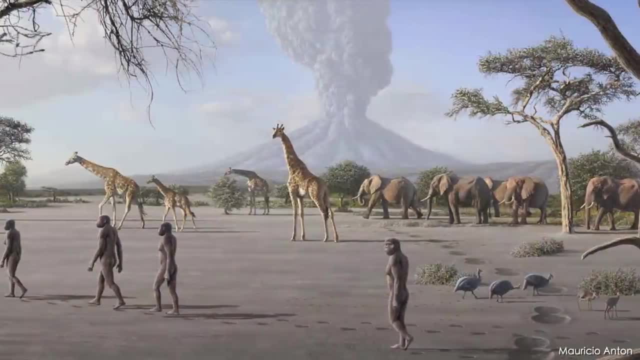 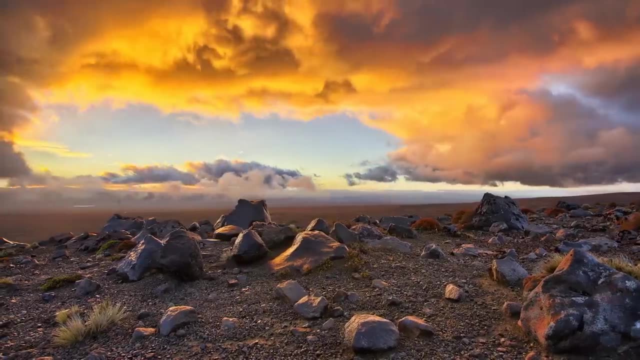 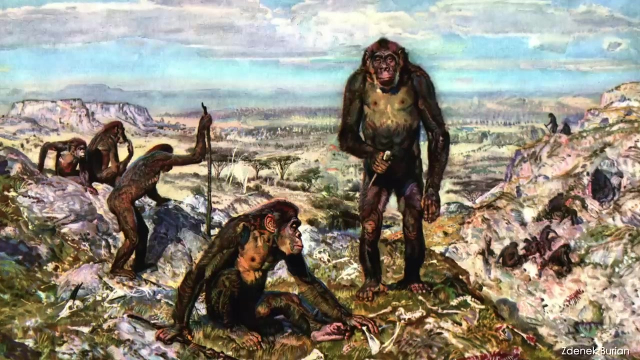 in eastern and southern Africa. They were entirely bipedal, with an upright posture, and made the first stone tools ever found on this planet. 3.3 million years ago, Australopithecines were creating modified stone tools at the site of Lomaquith III. This is a much more complex and 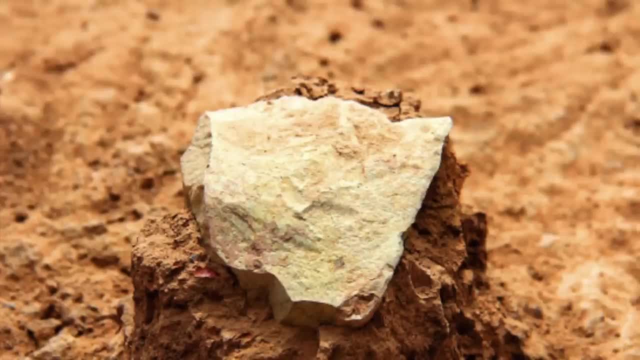 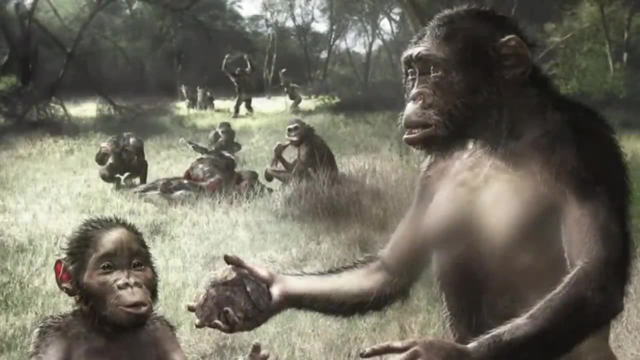 complex behavior than simply using a rock. They had to select stone capable of fracturing conchoidally and they had to hit it in just the right way to create a sharp edge. These tools were likely used for butchering scavenged carcasses, but other uses, such as shaping 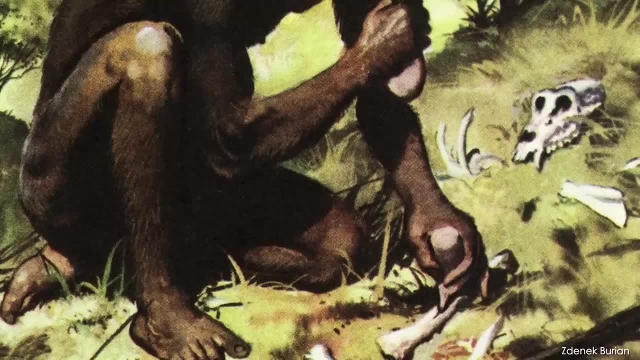 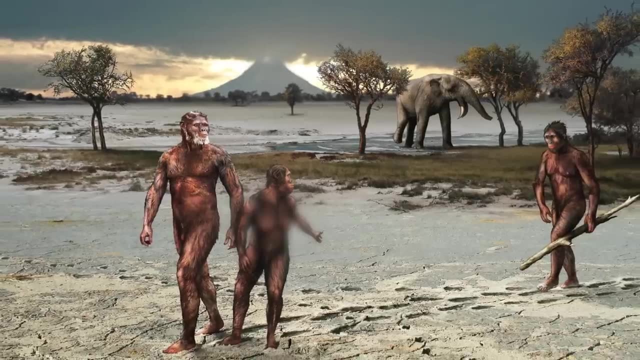 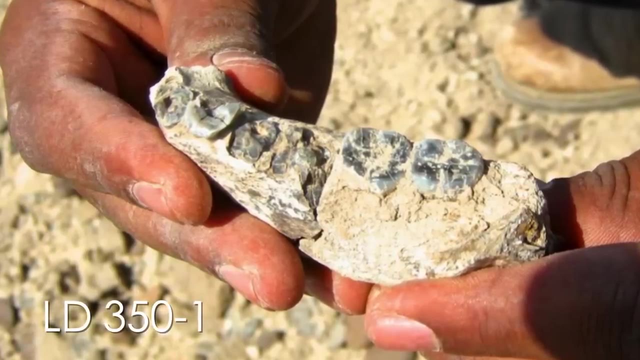 wood or defense must also be considered. Though some Australopithecines did use stone tools, many of them did not. Our genus almost certainly descends from the ones that did. The oldest evidence of our genus comes from a 2.8 million year old specimen. 2.6 million years ago, the first oldowan tools 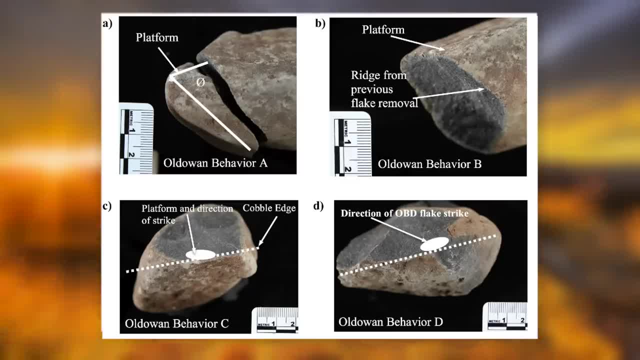 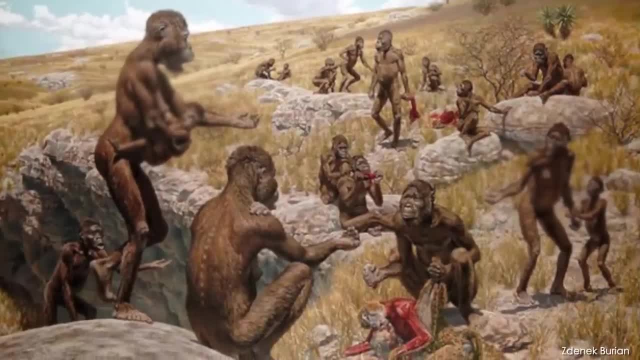 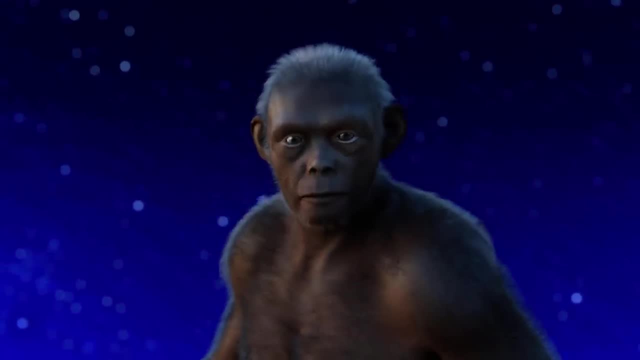 were being made. Oldowan tools consist of stones with a few flakes taken off to create a sharp and robust edge. Our genus was certainly around during the inception of these tools and it is very likely that they were the creators, Homo habilis. one of the earliest members of our genus appeared 2.3. 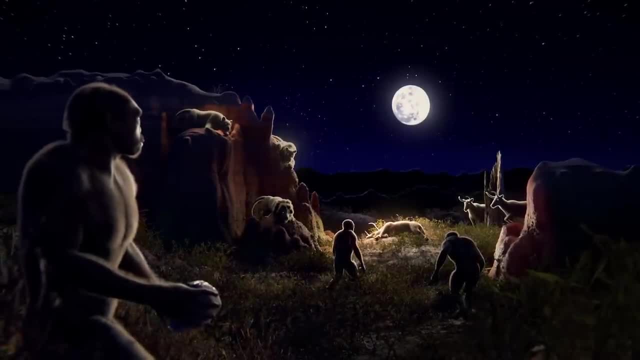 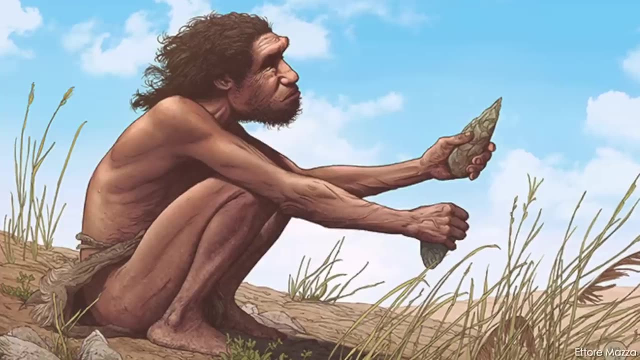 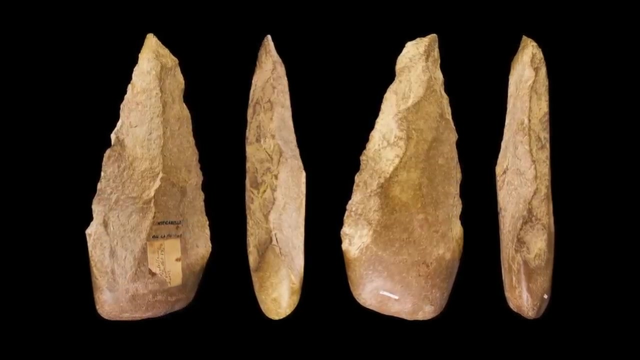 million years ago and was using oldowan tools. Homo erectus, often considered the first human, would evolve 2 million years ago and would eventually pioneer a new stone technology called the Acheulean. These hand axes were made by taking much more flakes off of both sides of a core to produce a much longer cutting edge. They are often 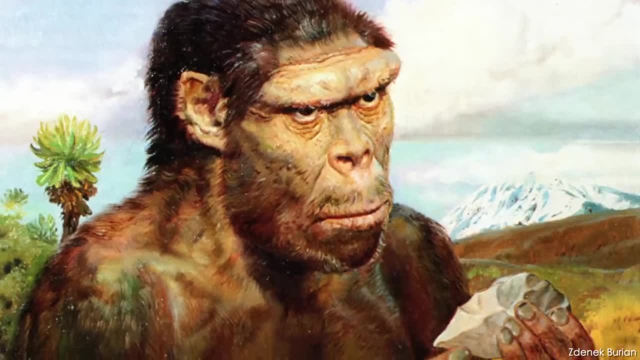 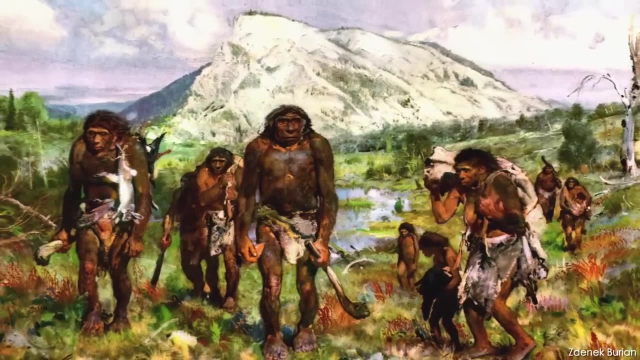 considered the pocket knives of their day, capable of butchering, game shaping wood, digging holes and even for defense or hunting. This technology would spread out of Africa with a wide variety of tools, and they would be used to create a sharp and robust edge. This would 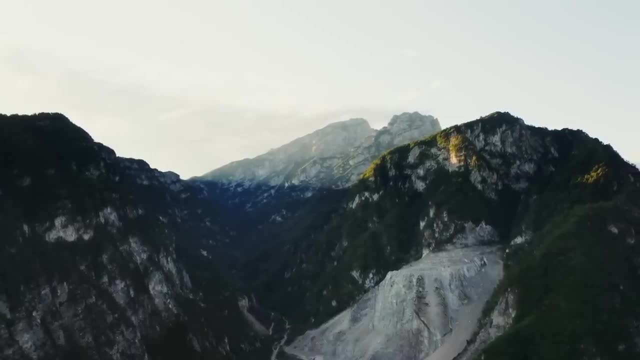 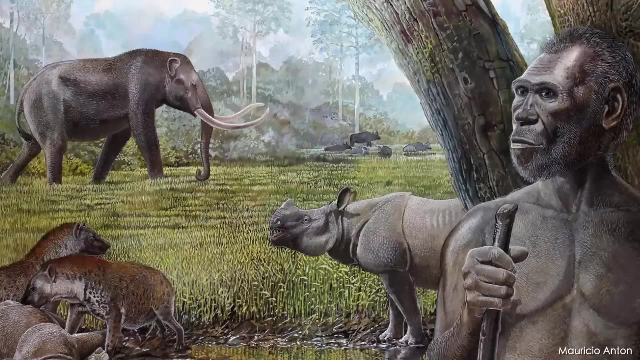 be used to create a sharp and robust edge. This technology would be used to create a sharp and robust edge, Homo erectus, to many parts of Eurasia, including Northern Europe, the Middle East and Southeast Asia. These populations would adapt to their new environments and would either evolve into distinct 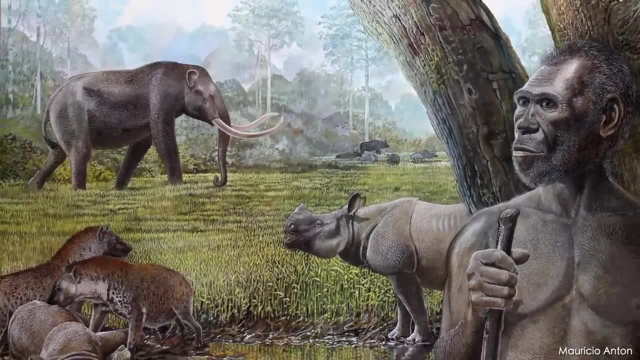 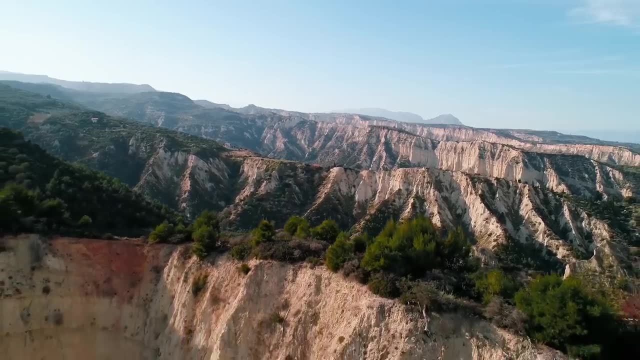 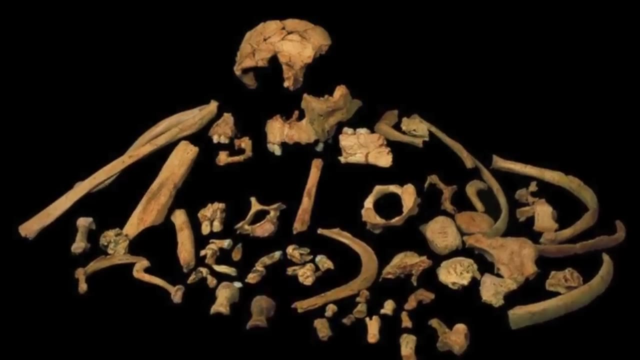 species or more derived forms of Homo erectus. One of these descendants was Antecessor. They lived in Western Europe 1.2 million years ago. This makes them the oldest known hominins to call Western Europe home. They were thought to have been an offshoot of erectus, Their tools. 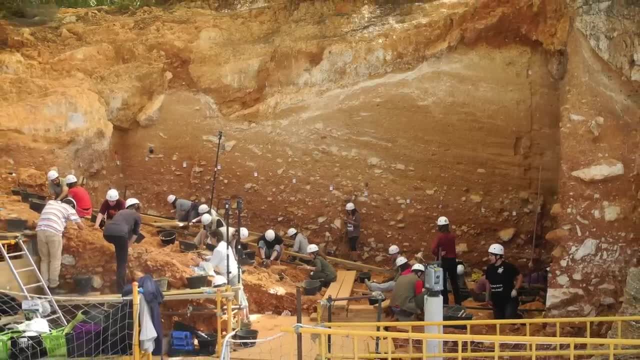 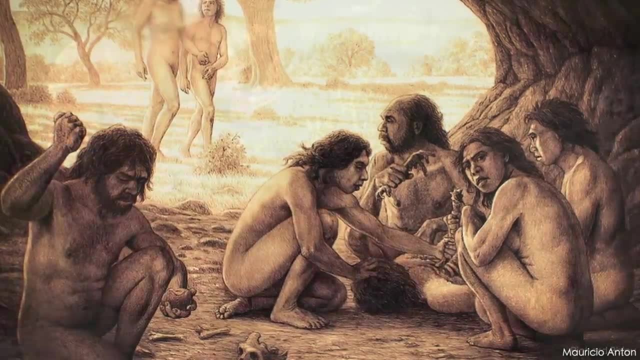 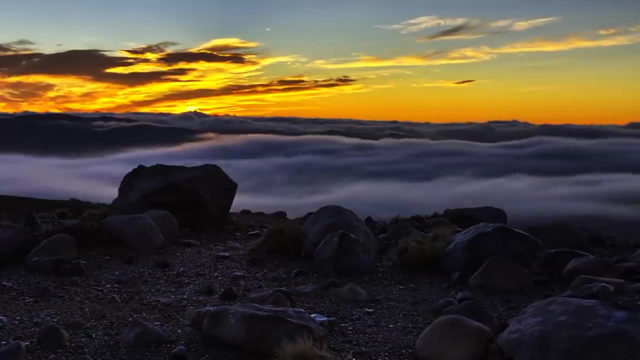 were quite simple and they would eventually go extinct. around 800,000 years ago. It is thought that they did not contribute to the genetics of future species living in Europe. Another wave of erectus, or perhaps a more derived form, would replace them By the middle Pleistocene 780,000. 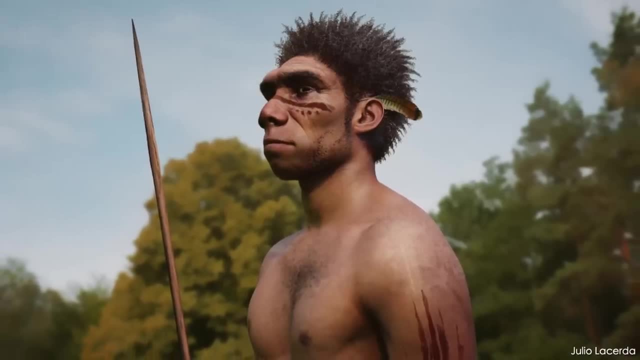 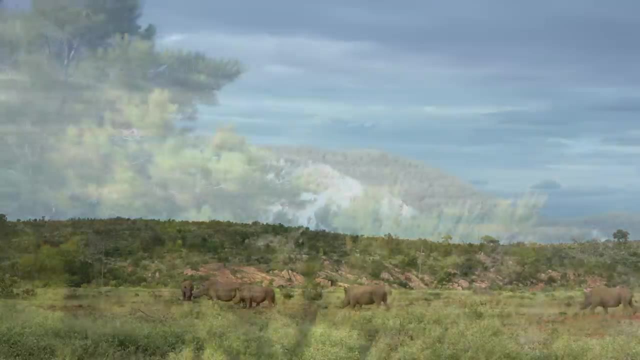 years ago, the descendants of erectus had evolved into more modern forms with larger brains and more complex technology. The hominins living throughout Africa, Europe and Western Asia during the middle Pleistocene are collectively classified as Homo heidelbergensis. 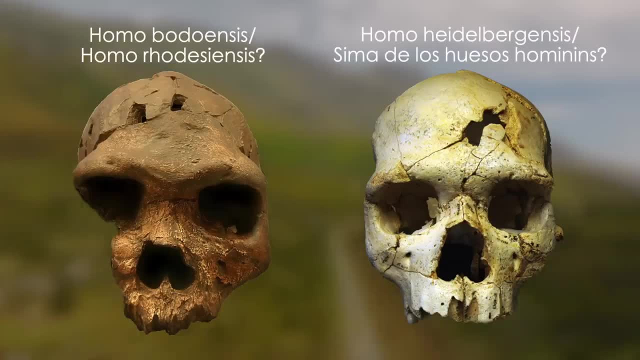 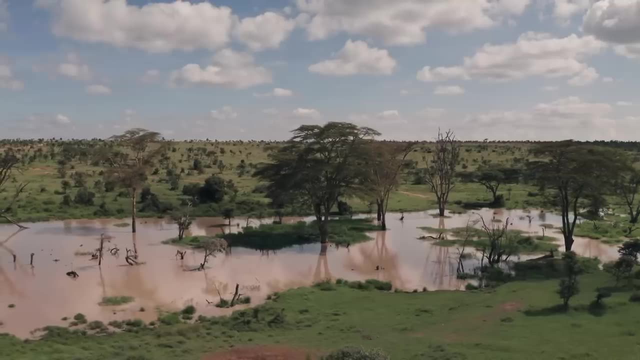 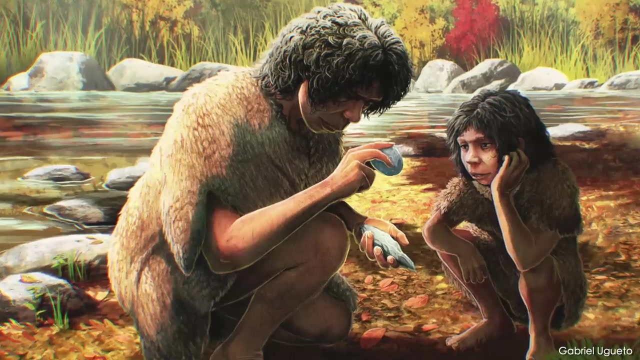 There has been debate regarding whether to consider African populations as a different species than Europe or Asian populations, because they are quite different. Genetics suggest that possibly as early as 700,000 years ago these populations would separate. The differences between these populations would continue to. 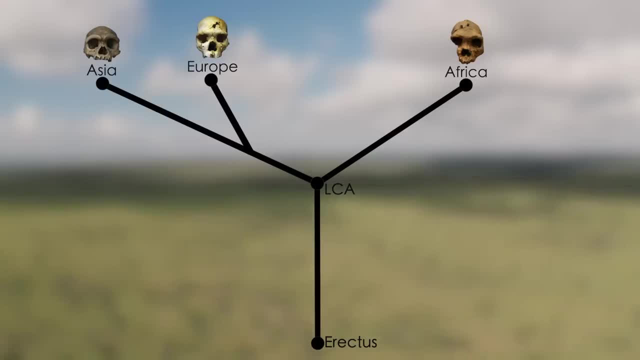 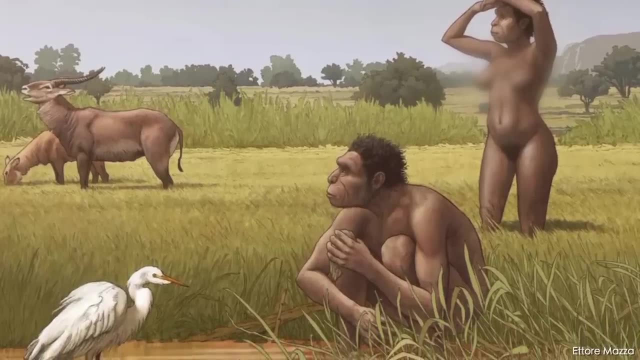 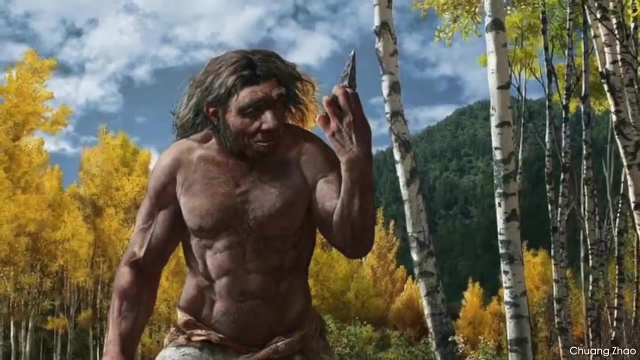 accumulate and by about 300,000 to 400,000 years ago would be enough to identify them as different species. In Africa and some parts of the Middle East lived our own ancestors, while in Europe and parts of Asia lived the Neanderthals and in East Asia lived the 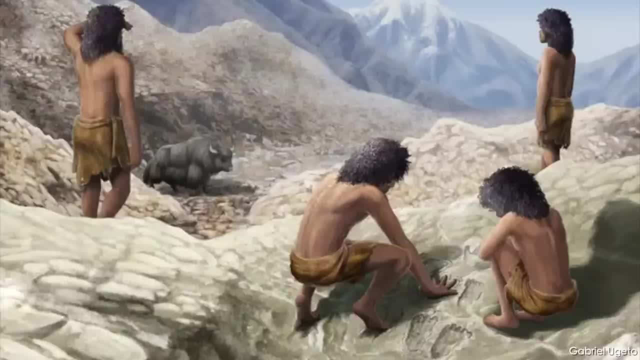 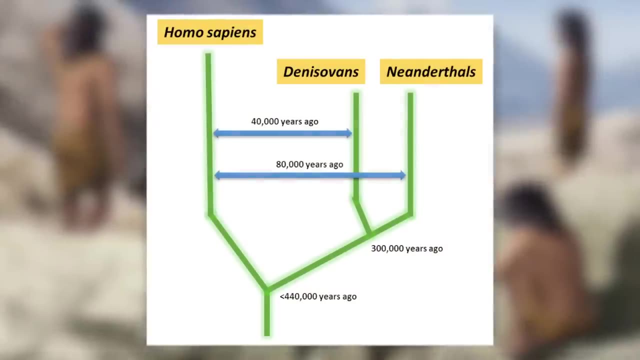 Denisovans and other hominins. Denisovans are another hominin very important to the story of the Neanderthals. This is because they are more closely related to Neanderthals than we are. Based on NDNA, Neanderthals and Denisovans share a more recent 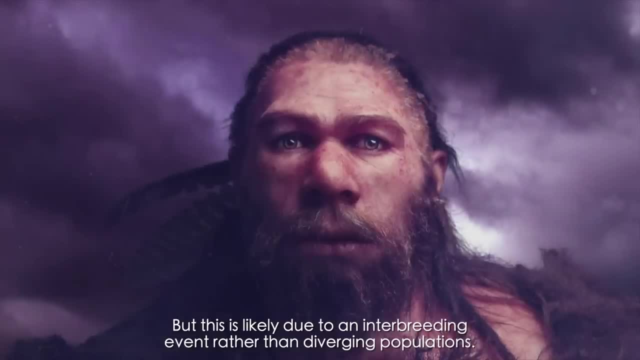 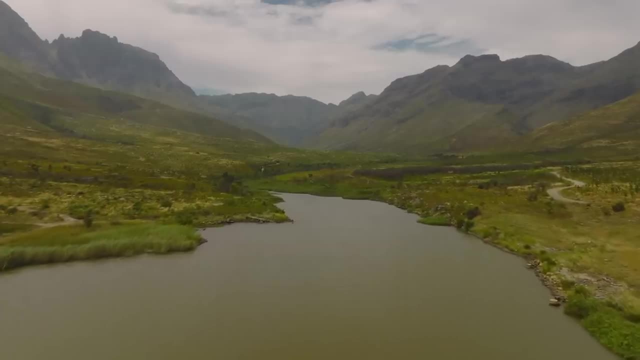 common ancestor with each other than with Homo sapiens. This common ancestor population, nicknamed Neanderthsovans, is thought to have spread from Africa to Eurasia, replacing and interbreeding with the other Archaic hominins in these areas. 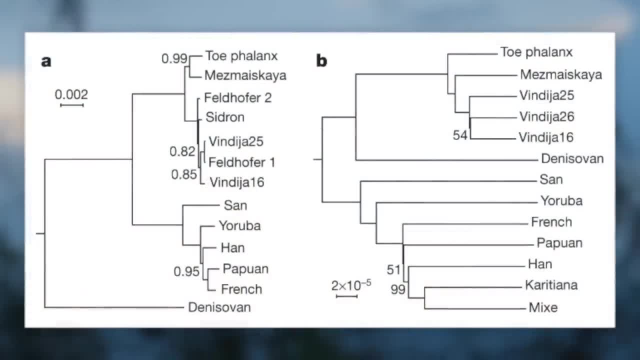 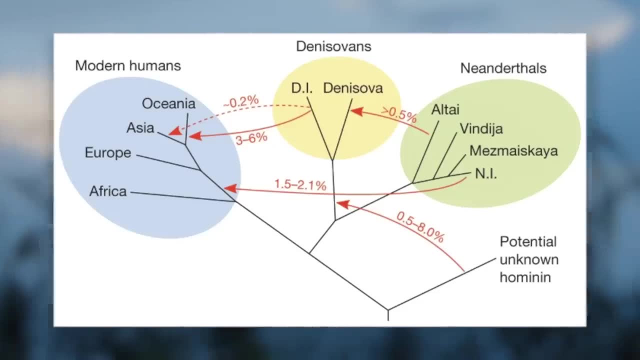 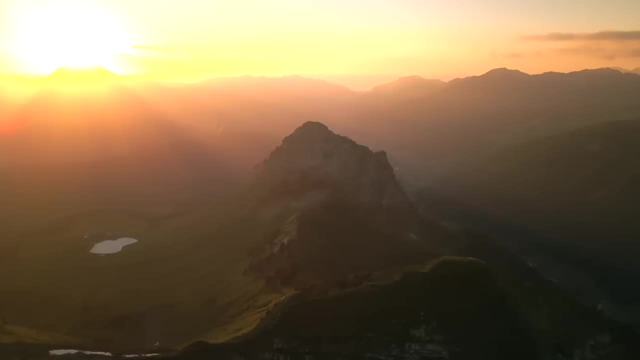 Based on mutation rates, this population would diverge into Neanderthals and Denisovans between 470,000 and 380,000 years ago. This correlates with the appearance of early Neanderthals during this time. 450,000 year old remains from France. 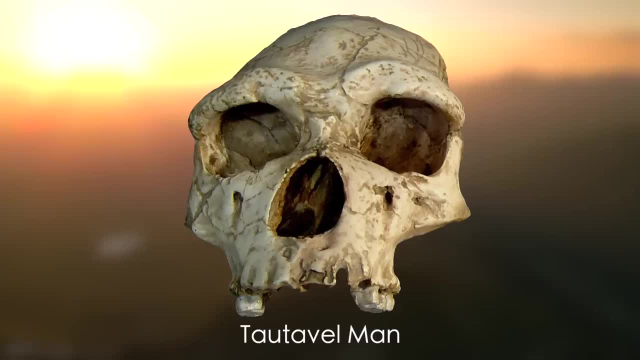 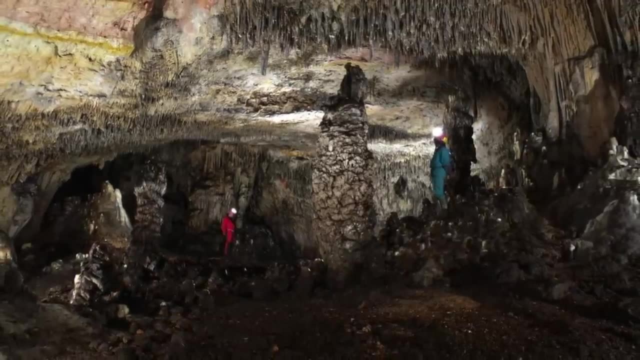 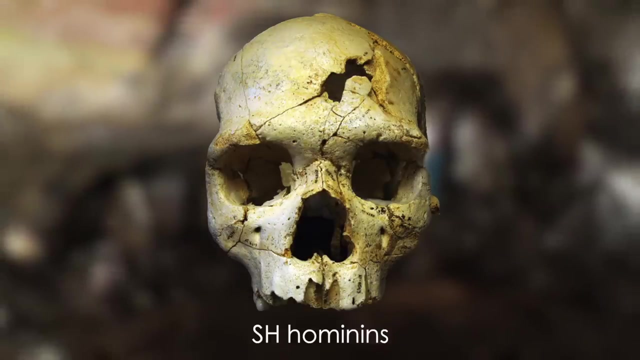 which are generally classified as Heidelbergensis, show the first appearance of Neanderthal features. 430,000 year old remains from Sima de los Huesos from northern Spain have much more similarities with Neanderthals and are widely considered to be ancestral to later classic Neanderthals. 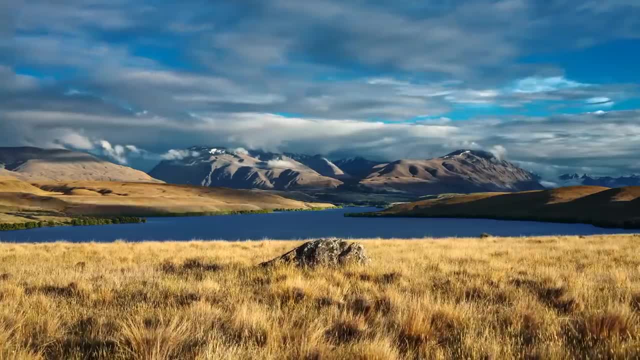 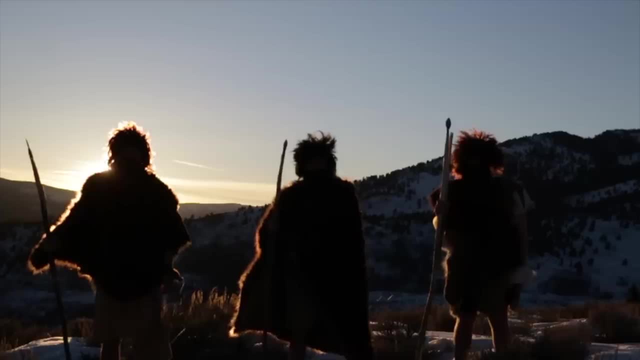 Neanderthal features would continue to evolve. Around 130,000 years ago, classic Neanderthals would appear which have an array of distinguishing skeletal features from early Neanderthals. These populations are much better understood due to the quality of the fossil. 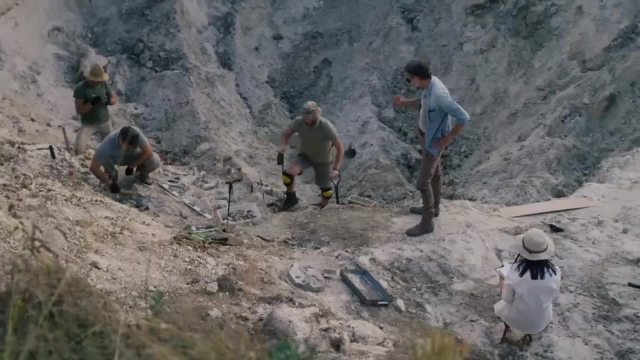 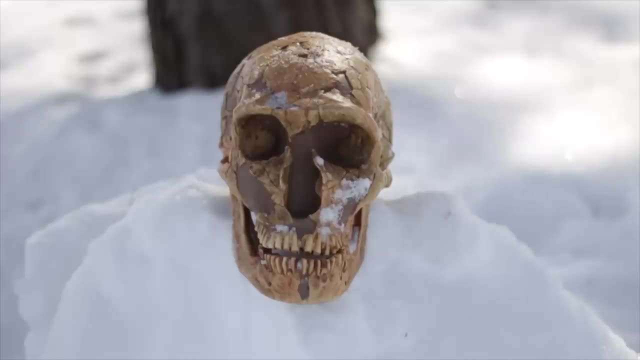 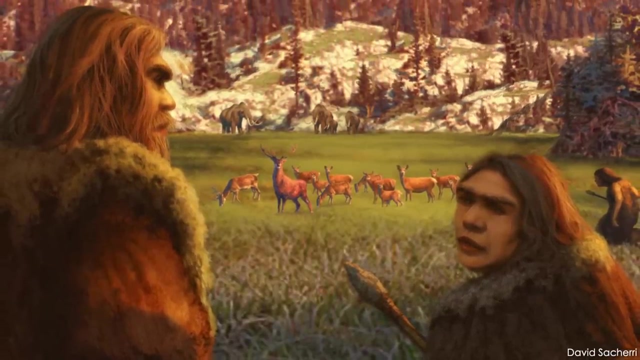 record increasing as time gets closer to us. Before talking about the anatomy of these people, there is one question left to answer: Were Neanderthals really a distinct species? The question may seem fairly simple at first glance, but it is extremely nuanced. 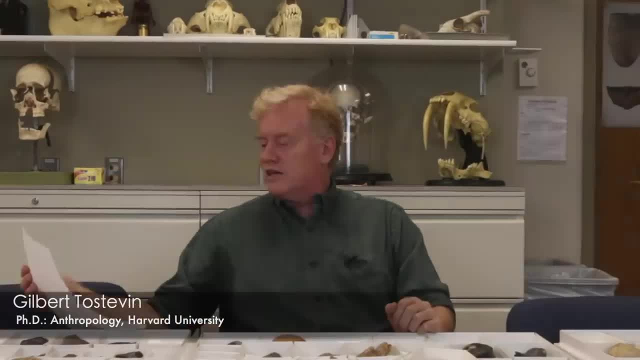 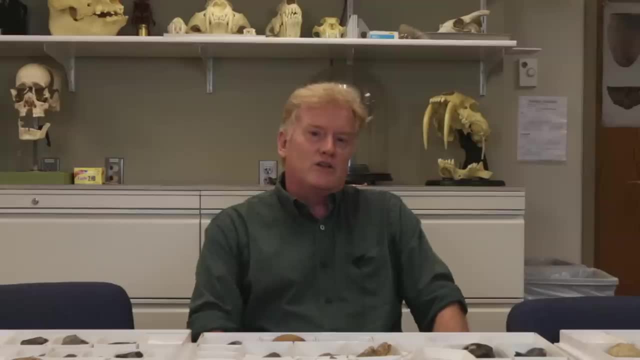 To gain a better understanding, I asked paleoanthropologist Gilbert Tastaven from the University of Minnesota. I do think it's a really good question to ask about what defines a species and how does one consider Neanderthals in terms of species relative to modern humans? 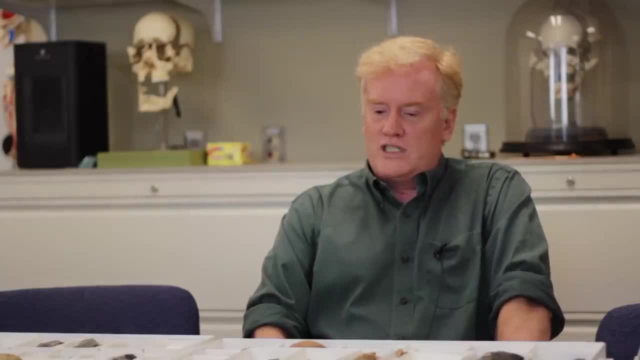 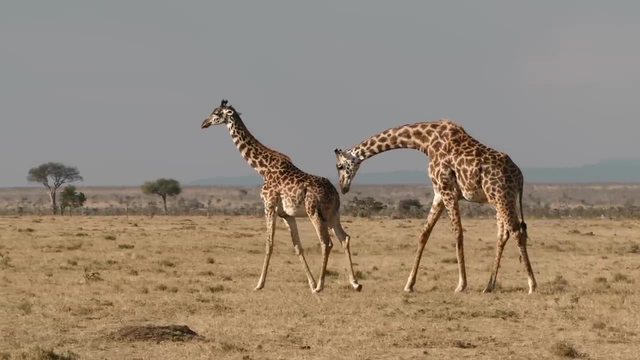 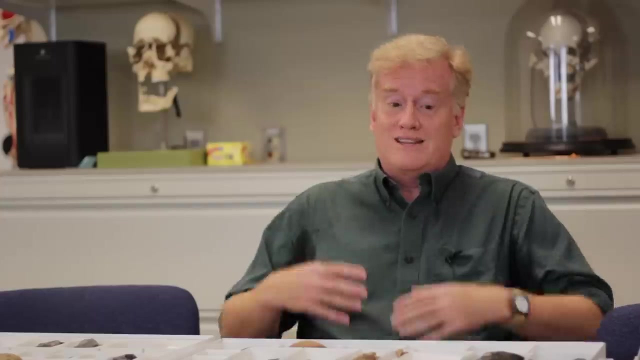 In terms of the most standard, extreme version of the definition of a species concept, which would be the biological species concept of Ernst Mayr, which states that you, that you know, individuals of a species can reproduce together and produce viable offspring that they themselves can reproduce. So when we look at the context of, let's say, 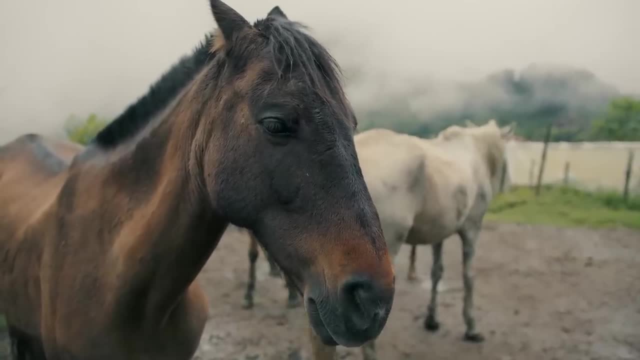 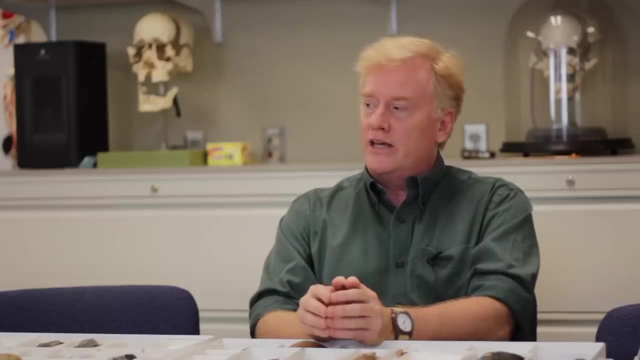 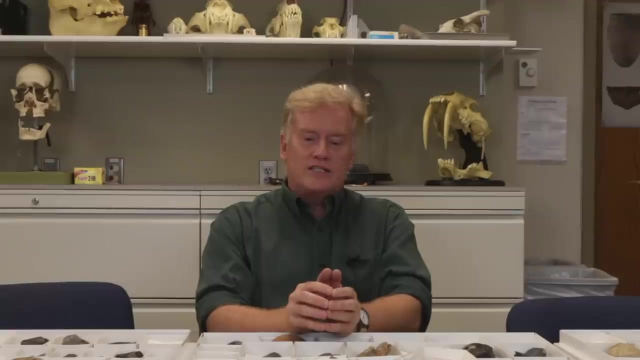 a horse and a jackass. they can mate and produce a mule, but the mule will not be fertile. There's a chromosomal difference such that they they don't produce fertile offspring. the mules do not, and so in that case they aren't that mule that that horses and jackasses are not. 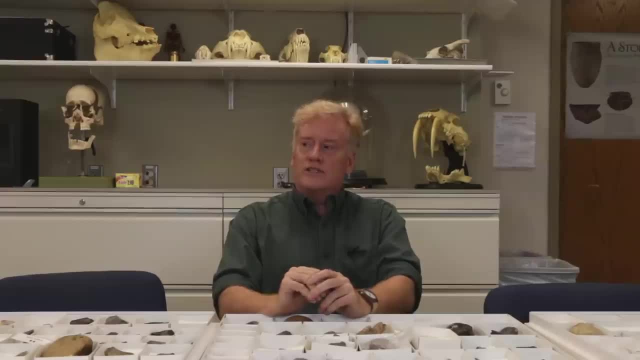 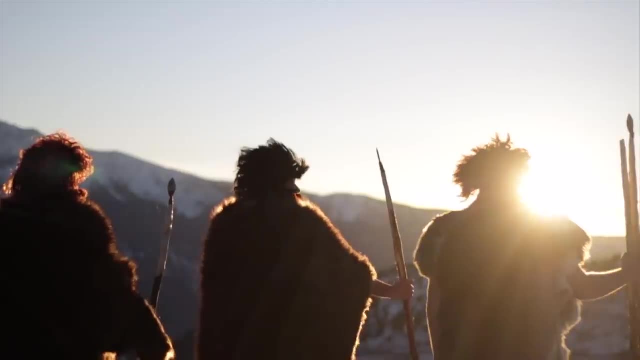 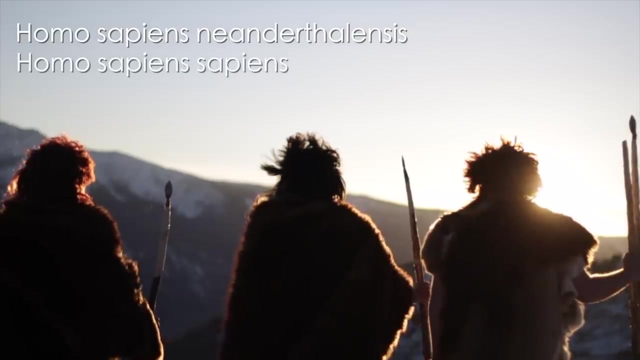 the same species In terms of the definition for a species. in that sense, Neanderthals were part of our species, So you could say: let's say that it was Homo sapiens Neanderthalensis, so a subspecies of humans versus modern humans being Homo sapiens sapiens. 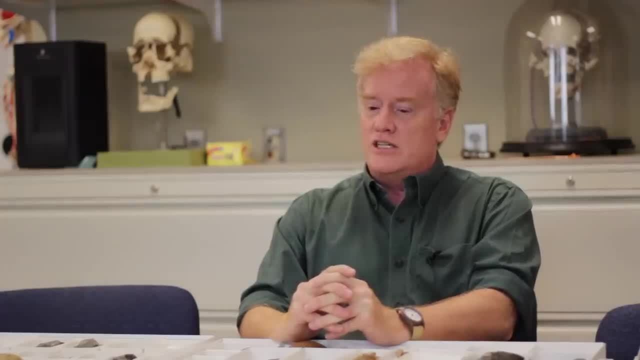 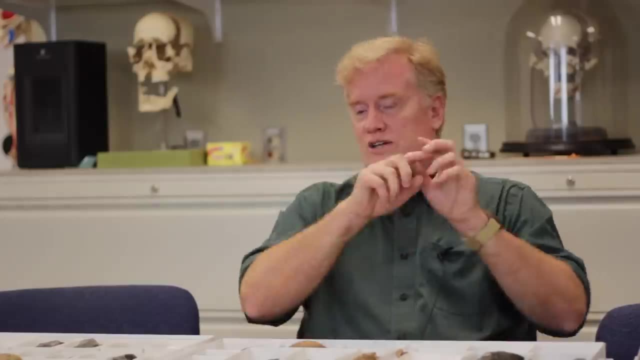 On the other side of it, we have to recognize that speciation is not an event, it's a process. But in fact all the different concepts of speciation are part of a continuum. So you start off with a separation of two lineages, usually geographically, If you have a geographical barrier. let's say one population expands into an area that has a geographical barrier. eventually you might get two populations on either side of the barrier, diverging by random chance, which we call genetic drift. If their adaptations in the population are different, then you have a separation of two lineages. In those locations start, by natural selection, start fitting to those different locations. they might develop unique traits that allow them to survive and reproduce in that particular environment. that might make them different enough that when the populations come back together, let's say on the other side of the geographical barrier or through time that they might one not be able to reproduce, but also might not, that selection might fade, And then you have to favor them not to reproduce being. this is where you get what's called the species mate recognition point in speciation, where you have two populations that won't. 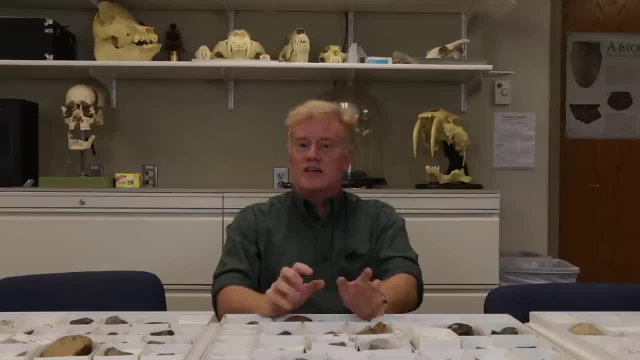 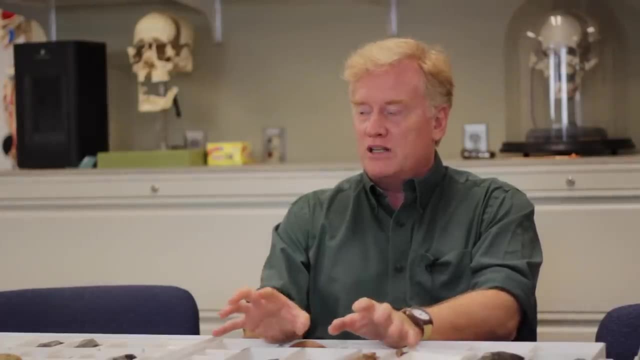 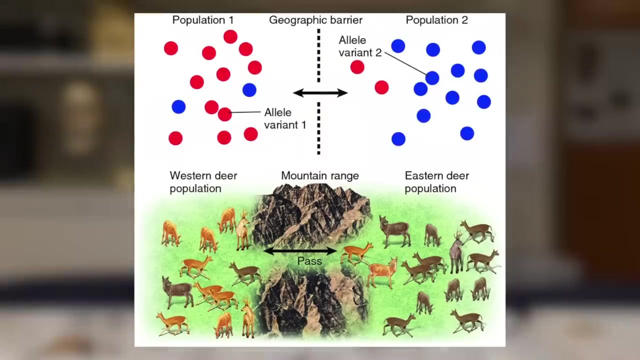 recognize each other as mates. This is one of the ways that evolution gradually separates the genetics, such that the populations in different places, which with different selective pressures, will actually be adapted for those locations, even when they're on the edges of those distributions. They might come back together and potentially mate. Looking at species issues a lot of times I want to call Neanderthals just like modern humans. in terms of modern human species they are late homo sapiens, but evolutionarily they have some. 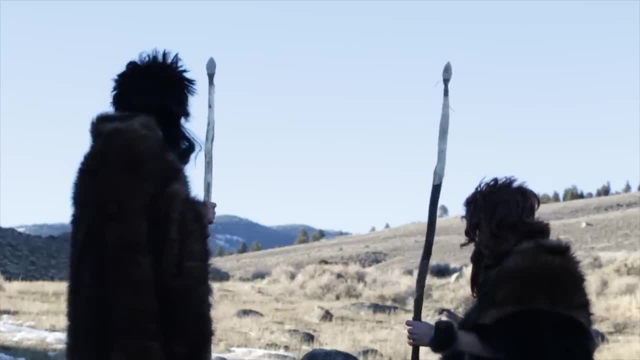 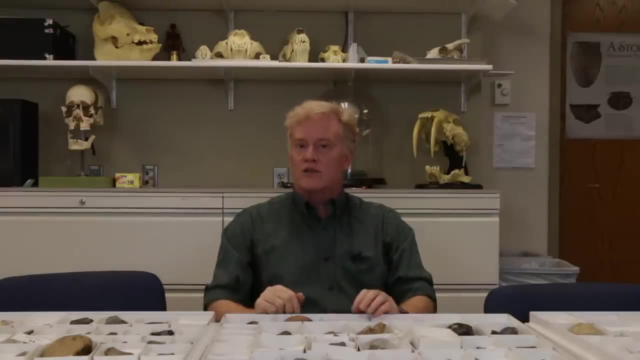 uniquely derived traits that no modern human has today and that modern humans who were alive at the time that Neanderthals were also did not have. So like, for instance, I mentioned, you know, parts of the hand anatomy, some aspects of the shoulder and the pelvis. they are different And this shouldn't really. 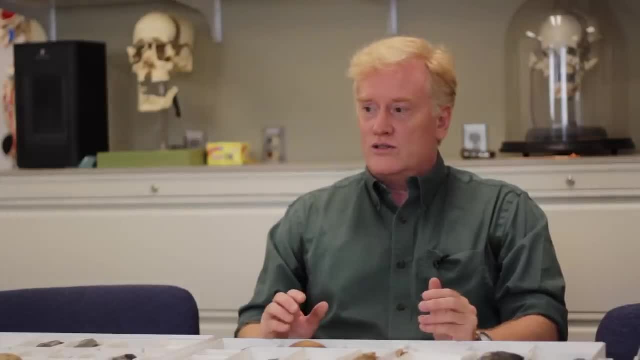 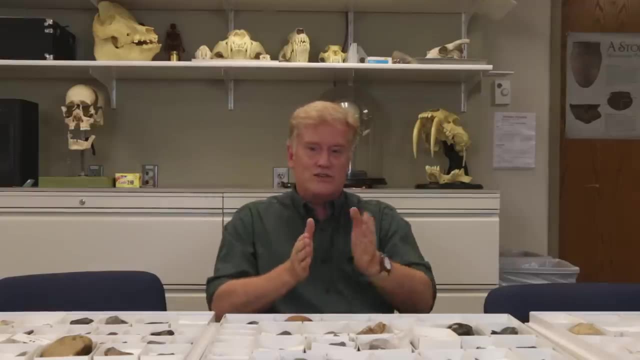 surprise us, because if evolution actually works, then species concepts cannot actually be hard. They can't be hard-lined. You can't actually have a really strong. this will always be on this side or this side, because evolution wouldn't happen if you can't have a gradual process of speciation. 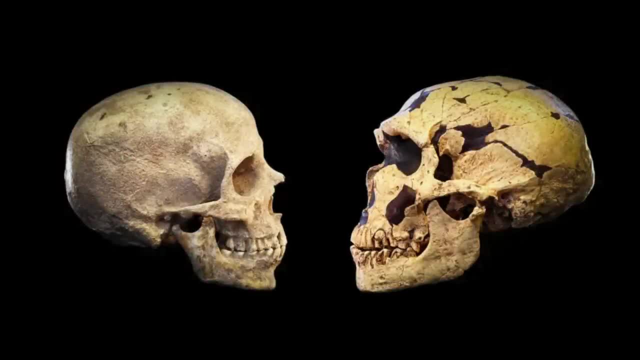 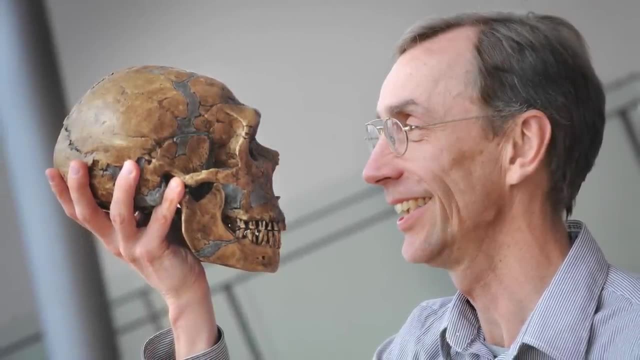 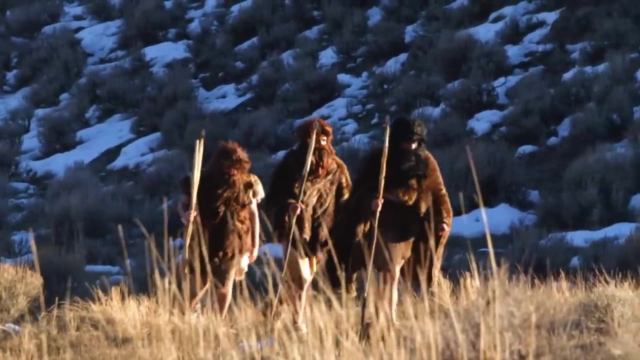 Neanderthals were indeed far different than any modern human alive today. This statement stands when considering that all modern humans actually have Neanderthal DNA. Considering Neanderthals to be another species or considering them to be in our own species is undeniably subjective. Many paleoanthropologists would consider them to be a different species. 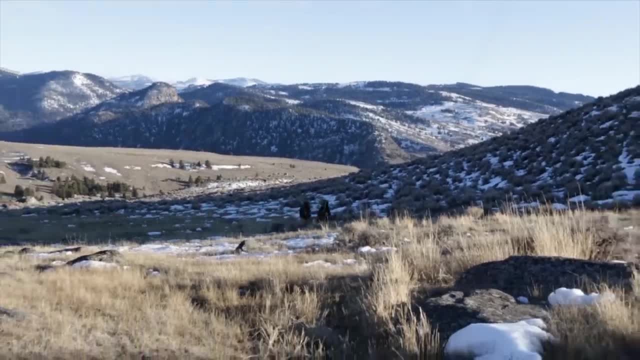 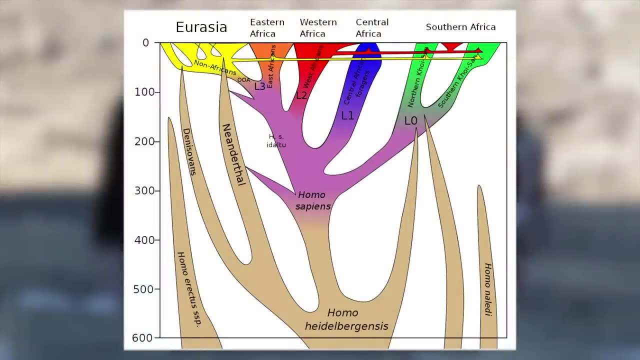 For understanding the place of Neanderthals in human evolution, it is useful to consider them a different species, because they were separated from our ancestors for hundreds of thousands of years. What you should learn from all this is that the designation of species really is a scientific. 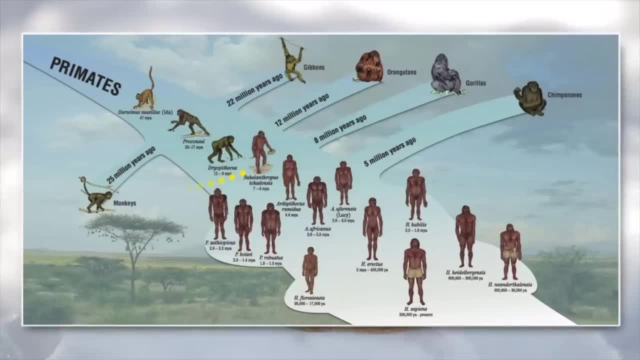 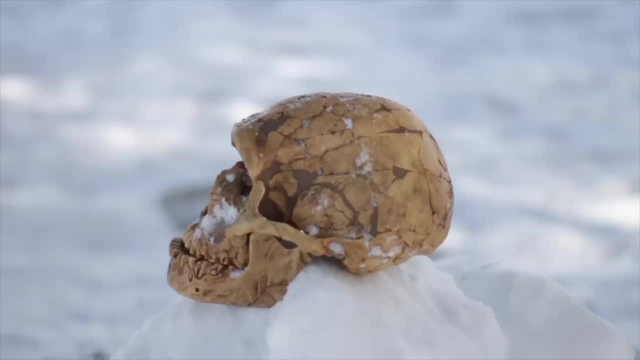 construct that doesn't necessarily apply to the reality of biology, as rigidly as the word may suggest. you should know more about Han지는 Ai over the years in this series by liking the video above. But this creates another question: Should we consider them human? 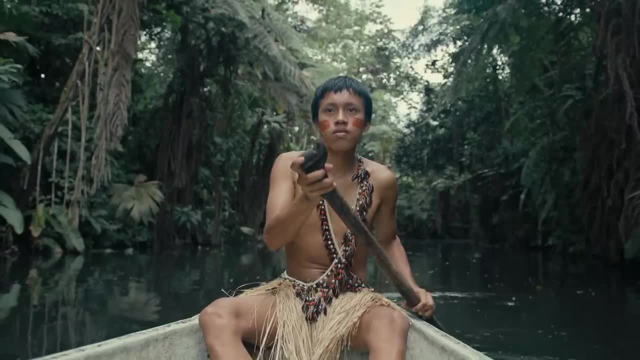 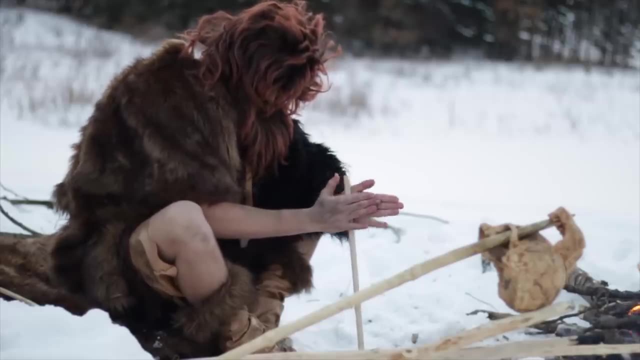 Well, human does not simply mean homo sapien. Human is not a taxonomic word and therefore is subjective. Since Neanderthals seem to have behaved in very similar ways to modern humans, most anthropologists would say that they satisfy with a human antelope. But that is not enough. most anthropologists would say that they satisfy with a human antelope, But that is not enough. most anthropologists would say that they satisfy with a human antelope. most anthropologists would say that they satisfy with a human antelope, But that is not enough. 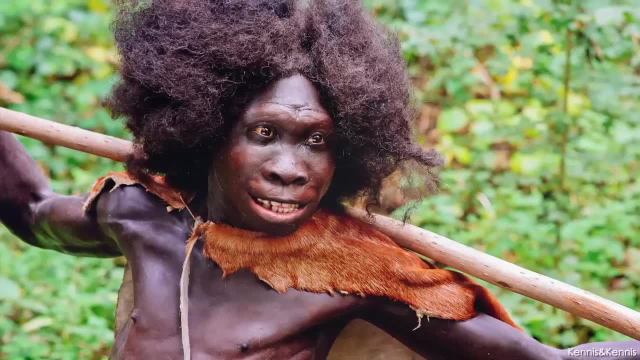 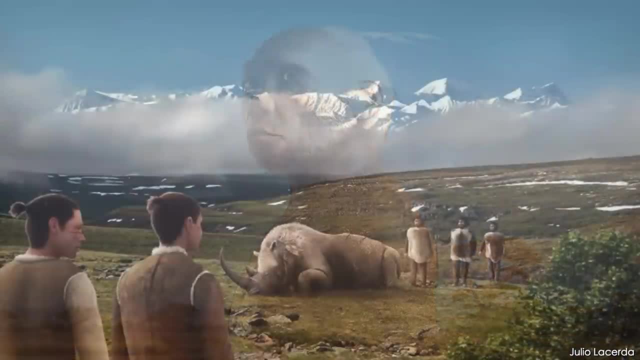 that they satisfy the requirements of being human. Many would even say that other species as far back as Erectus or even Habilis should be considered human. From a distance, you would likely recognize them as a member of our species. Neanderthals had a build and appearance relatively 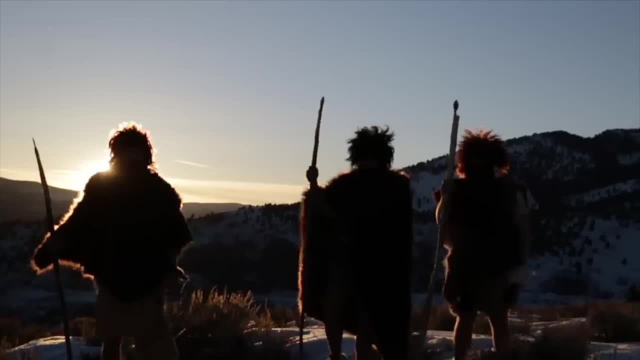 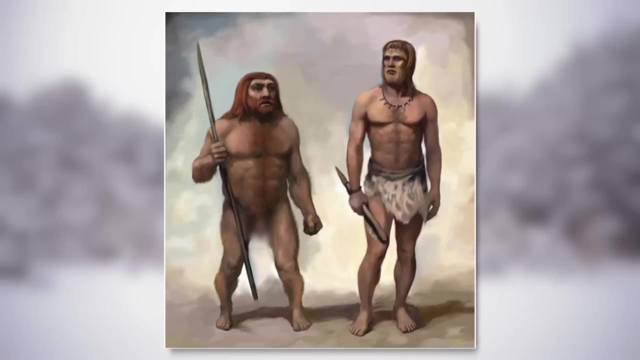 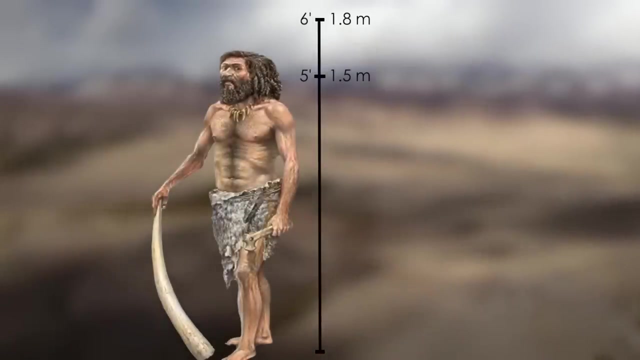 similar to modern humans. One of their main differences was their shorter and squatter bodies. Their limbs were shorter, their chests were wider and their muscles were larger. Based on 45 Neanderthal long bones, the average height was 165 cm, or 5 feet 5 inches for males, and 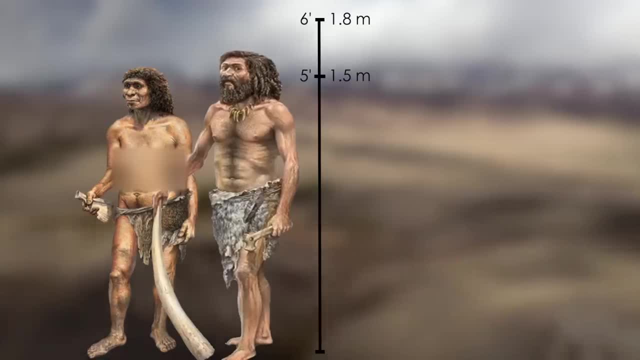 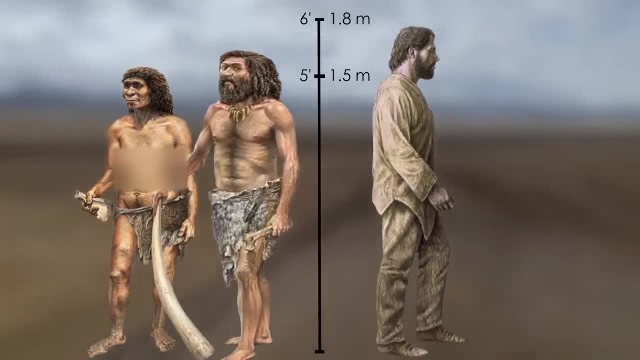 152 cm, or 5 feet tall for females. For comparison, the average height of Upper Paleolithic European humans is 176 cm, or 5 foot 9 inches tall for males, and 163 cm, or 5 foot 4 inches for females. 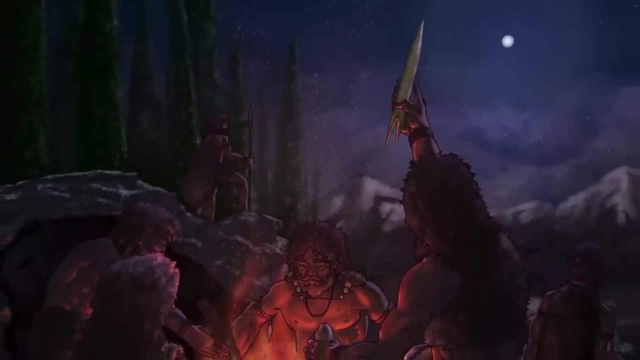 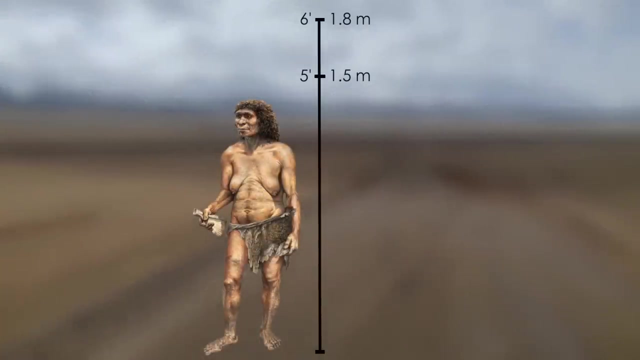 On average, the modern humans that would later dominate Europe would be about the same height as Neanderthals. The fossil record shows that adult Neanderthals varied from about 147.5 to 177 cm, or 4 foot 10 inches tall, to 5 foot 10 inches tall. 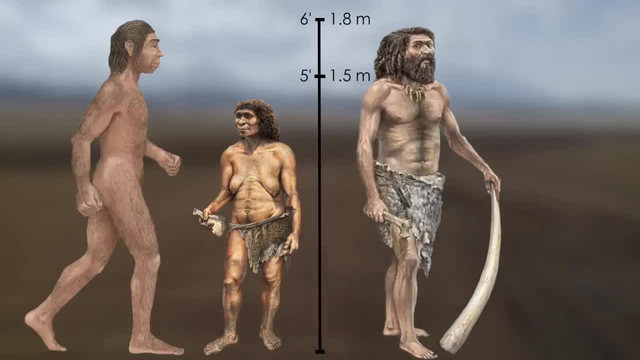 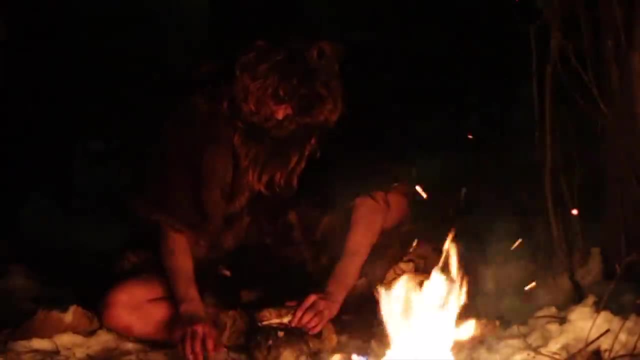 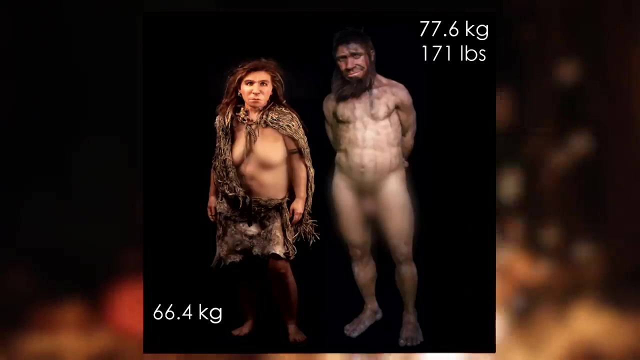 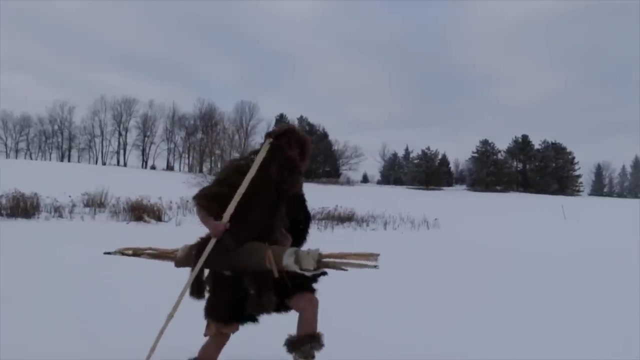 Some certainly grew larger and a height of 182 cm or 6 feet was likely attainable For Neanderthal. weight samples of 26 specimens found an average of 77.6 kg or 171 lbs for males. The body mass index for Neanderthal males was calculated to be 26.9-28.2,. 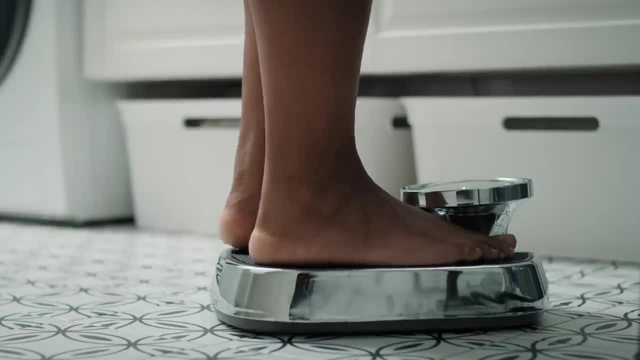 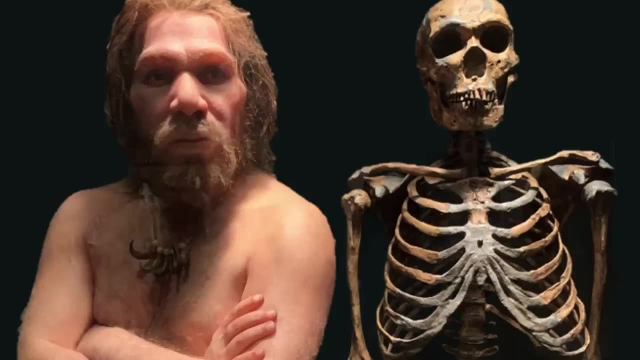 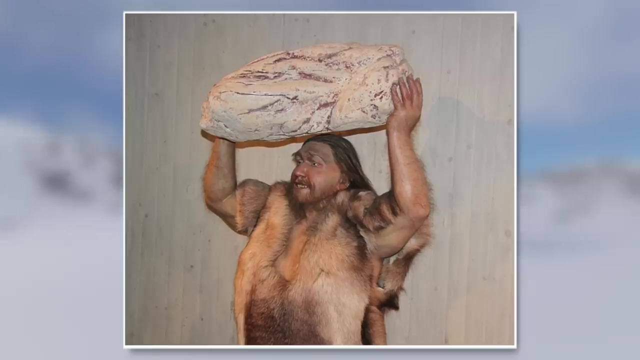 which, in modern humans, correlates to being overweight. Though Neanderthals were literally big boned, their bones were thicker and denser than modern humans. These bones likely result from a combination of naturally thick bones and a very active lifestyle. Neanderthals also had more muscle mass than the average modern human. 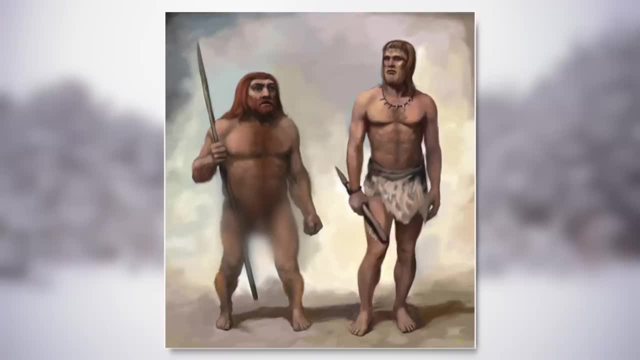 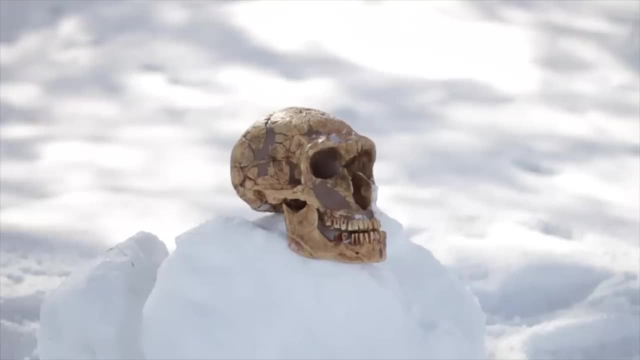 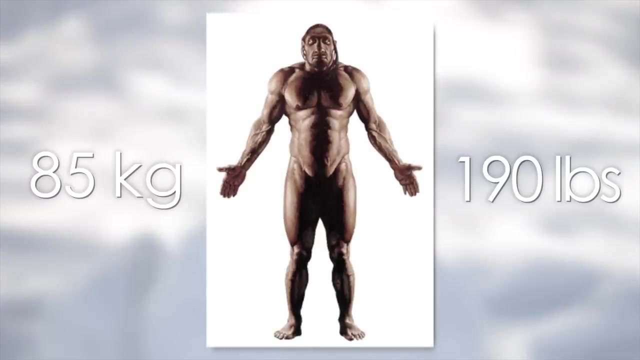 Overall, they were about 15% heavier than the average modern human, despite the fact that they were shorter. One of the most famous Neanderthal individuals, Laferrazi I, was only 1.6 meters or 5 foot 2 inches tall, but he weighed an estimated 85 kilograms or 190 pounds. 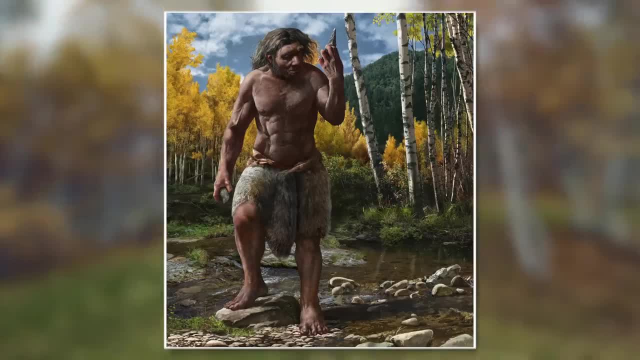 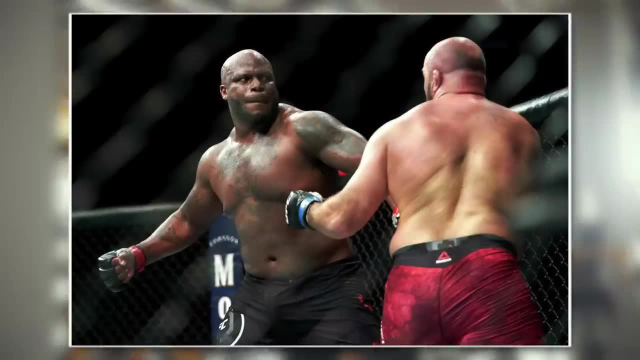 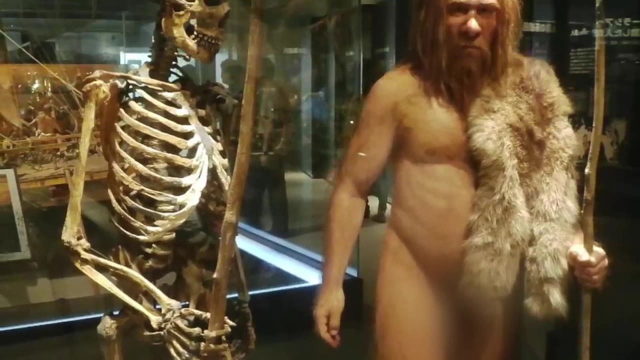 This individual was undoubtedly very strong in his lifetime, Though people tend to over-exaggerate their strength. Modern athletes and powerlifters who regularly exercise reach similar, if not higher, levels of strength. Their morphology has caused many different hypotheses regarding its function. The most common explanation has been that they were adapted to glacial conditions. 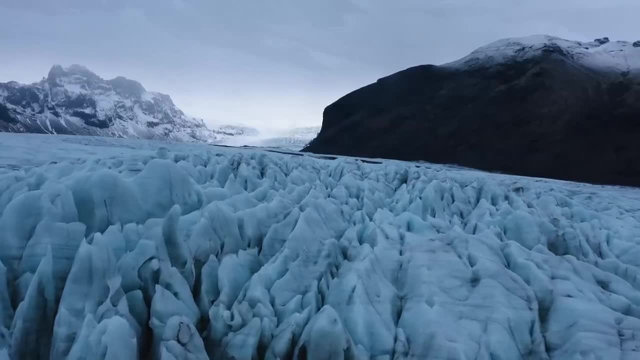 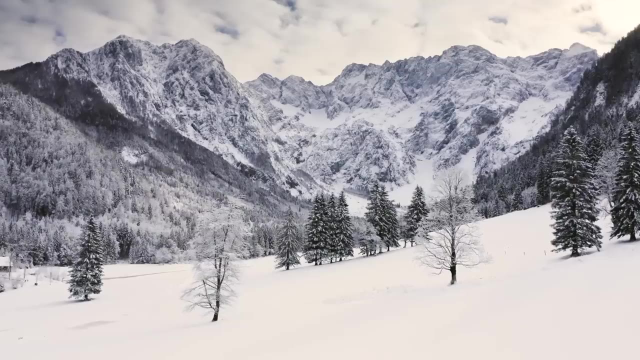 Neanderthals experienced at least four separate glacial periods. These periods would have been very hard to survive in Central Europe. Europe is already globalized. It would have been very cold in the modern day, but it would have been much colder during these periods. 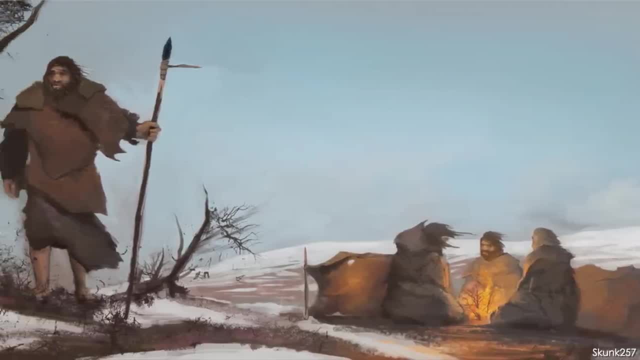 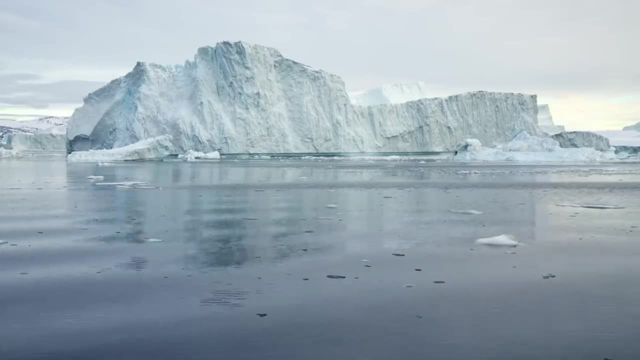 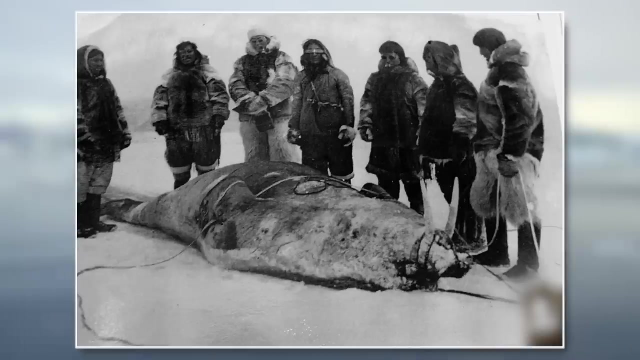 The idea is that Neanderthal morphology evolved to be shorter and squatter to survive these freezing conditions. It comes down to simple physics: Less surface area means less heat lost. This correlates with populations of modern humans living in arctic conditions. They have also evolved shorter limbs and squatter bodies. 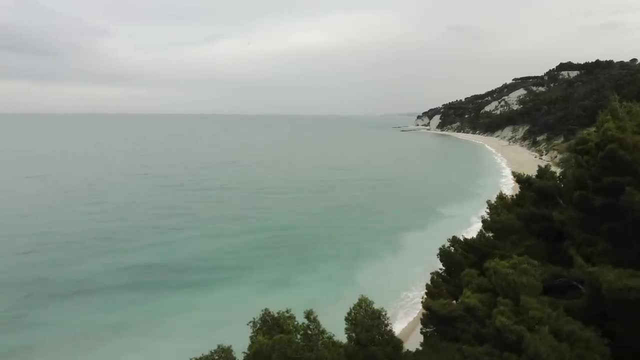 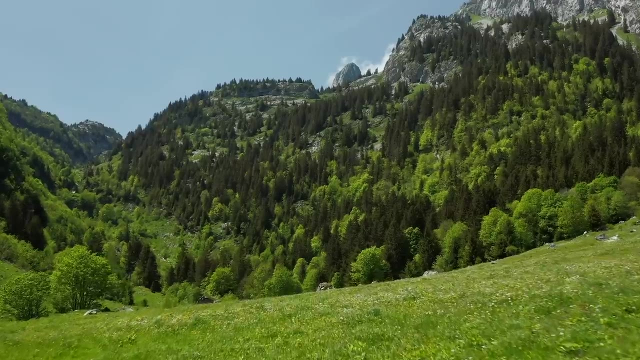 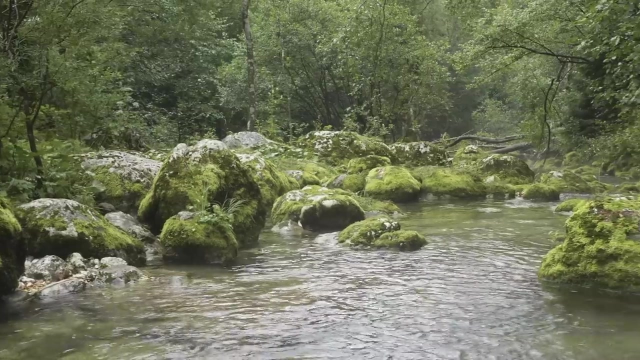 The problem with this thought process is that Neanderthals living in warmer conditions in the Mediterranean and the Middle East also retained this squat morphology. And to add to this, during interglacial periods Europe would have been quite warm. Alternate hypotheses have also been proposed. 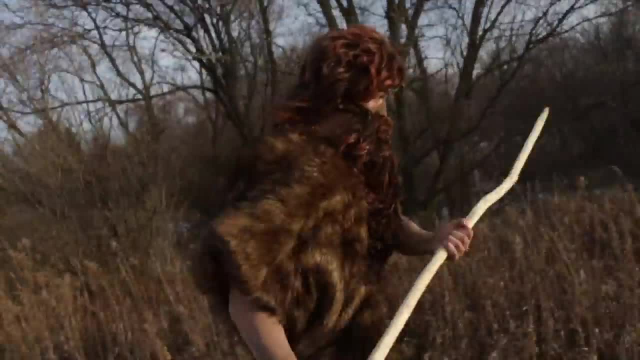 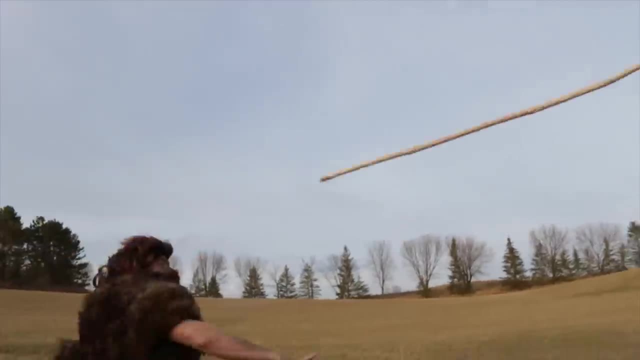 In 2019, English anthropologist John Stewart suggested that Neanderthals were adapted for sprinting. Their robust bodies may have allowed them to quickly run after prey. DNA analysis also indicates a higher proportion of Neanderthals living in warmer conditions. 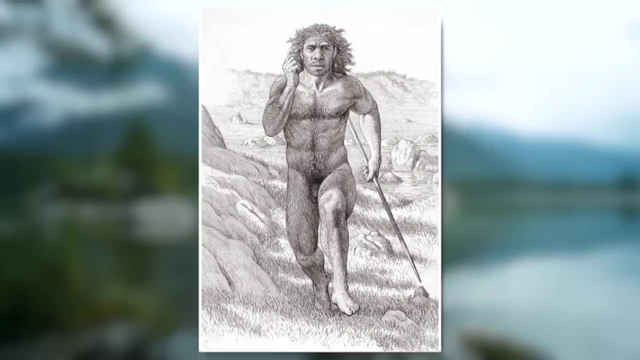 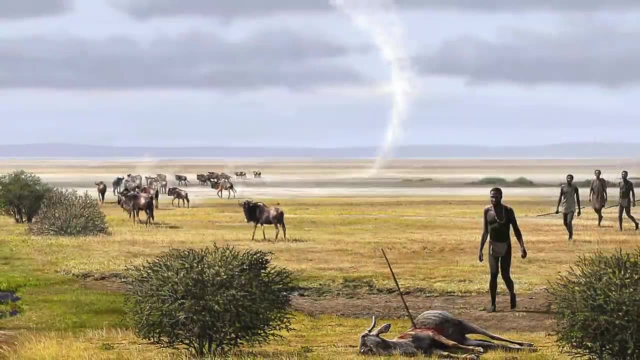 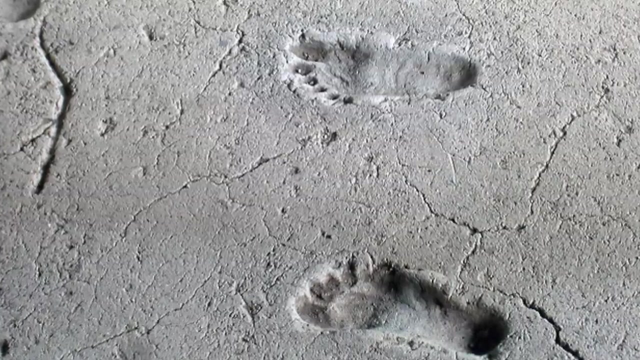 They had a higher proportion of fast twitch muscle fibers in Neanderthals than modern humans. He explained their body proportions and greater muscle mass as adaptations to sprinting, as opposed to the endurance-oriented modern human physique. They had longer heel bones than modern humans, which means they also had a longer Achilles tendon. 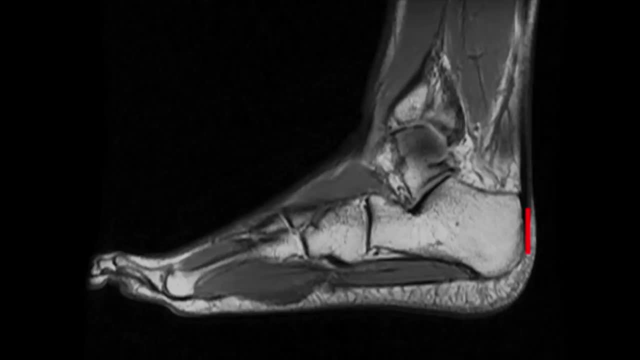 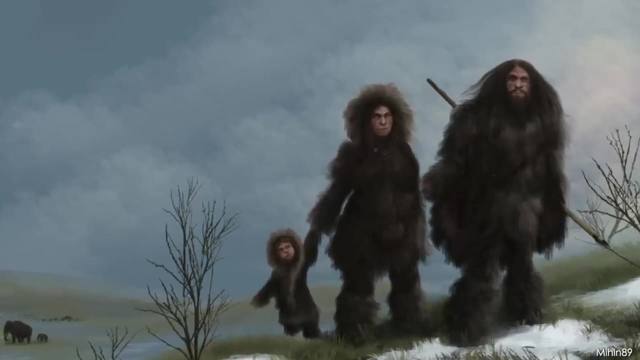 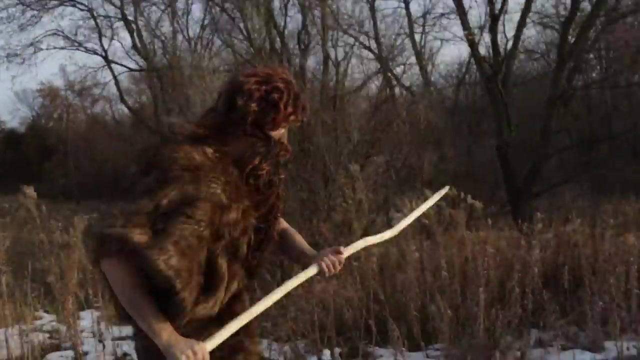 A longer Achilles tendon would have been less efficient at storing energy for long-distance running and more suited towards sprinting. Their shorter limbs were certainly not useful for hiking, But they were for staying warm and for sprinting. Both the hyperarctic hypothesis and the sprinting hypothesis are likely true in their own ways. 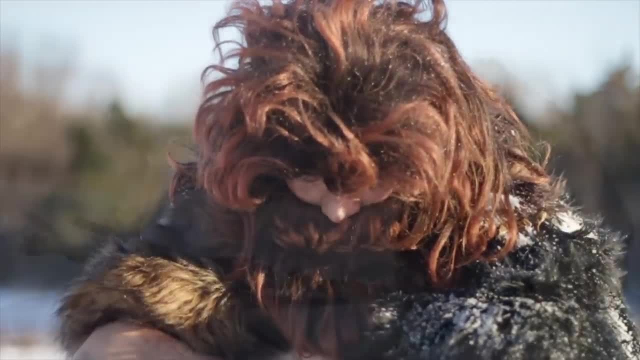 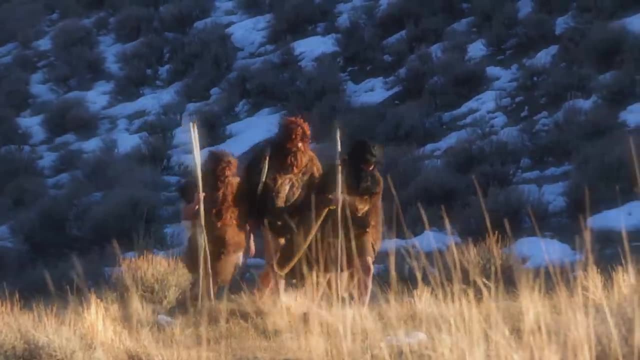 It is undeniable that Neanderthals lived through some very cold conditions, and their morphology couldn't help but be affected by this. For example, the Neanderthal LEPR gene, concerned with storing fat and body heat production, is similar to that of the woolly mammoth. 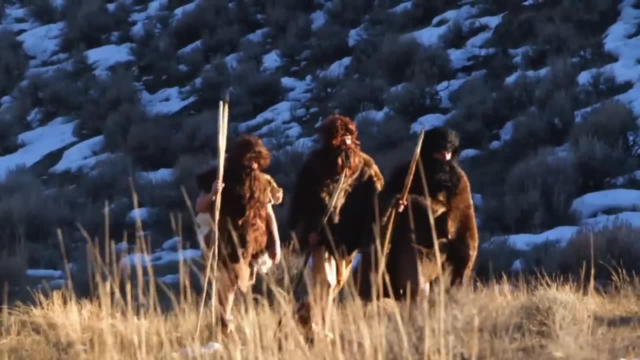 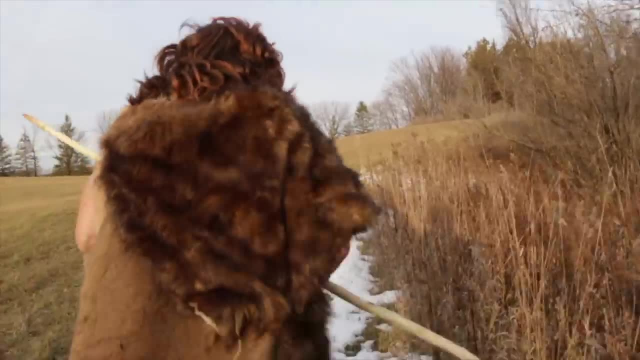 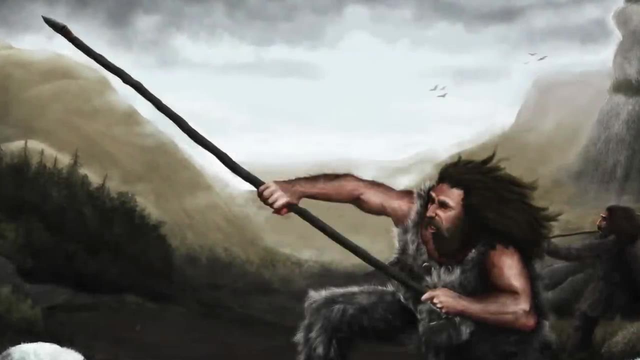 It was almost certainly an adaptation for a cold climate. Other aspects of their morphology, such as their heel length and fast twitch muscle proportions, suggest that sprinting was a part of how they were shaped. Another aspect about Neanderthal morphology that has long been debated is whether their humeri allowed them to throw efficiently. 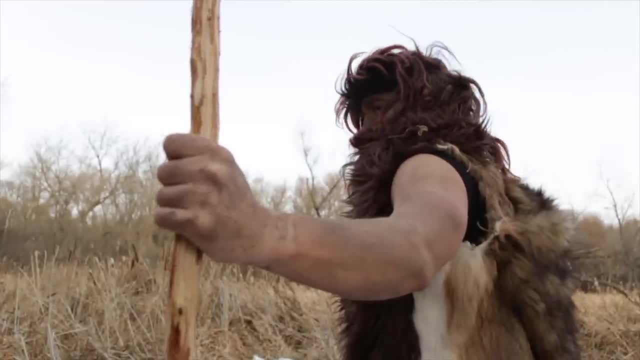 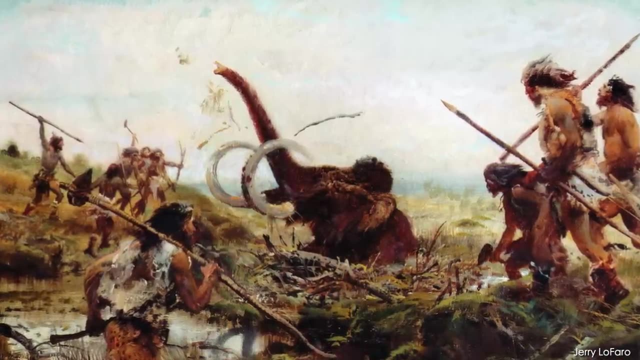 Original evidence seemed to indicate that their shoulders could not over arm throw well, Though additional studies and physical evidence now highly suggest that they could throw. Berthalm et al 2014 found that Neanderthal humeri were both efficient at thrusting and throwing. 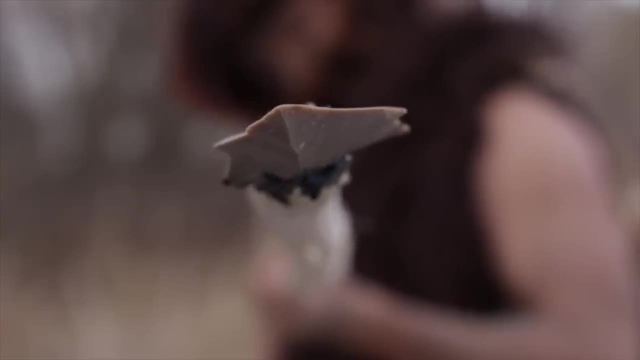 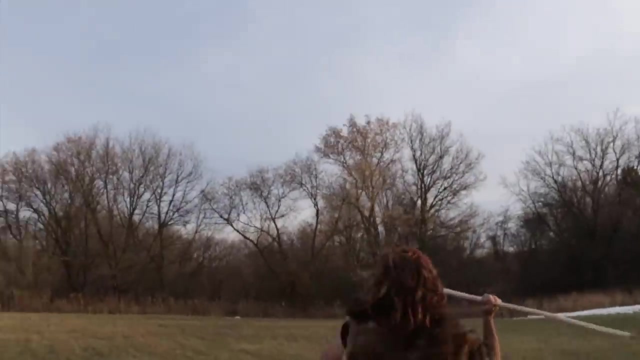 There was no evidence that thrusting was more prominent. It also found that sapien and Neanderthal humeri, although different, showed similarities in resisting throwing and thrusting stresses. At a site in northern France, Neanderthal arm bones have micro-experiments. 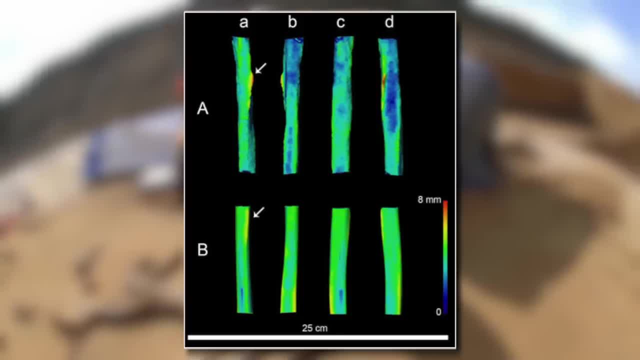 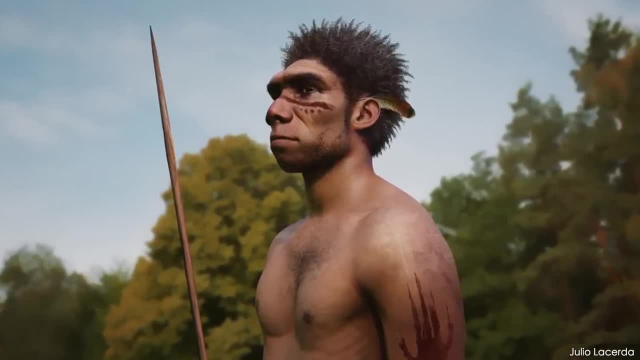 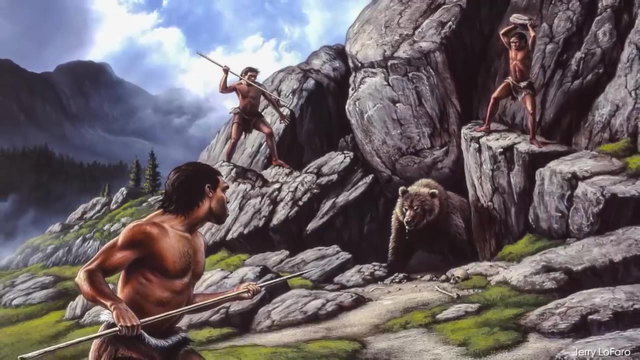 There are also macro traumas associated with habitual spear throwing. The discovery of the Schoeniggen spears also provided physical evidence that spears may have been being thrown in Europe even by the ancestors of classic Neanderthals. They were certainly able to throw, and evidence suggests that they did, though their shoulder mechanics are not the best for over arm throwing. 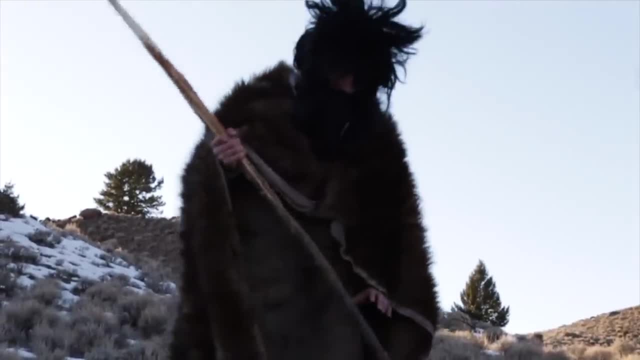 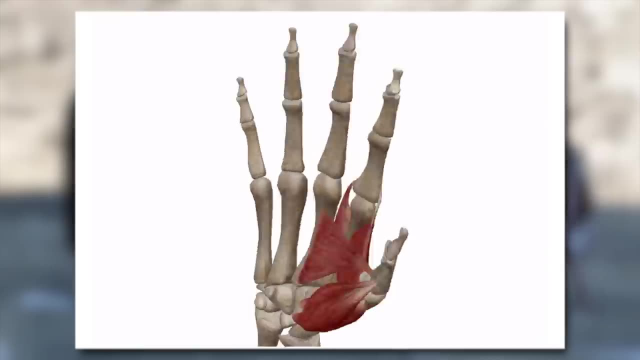 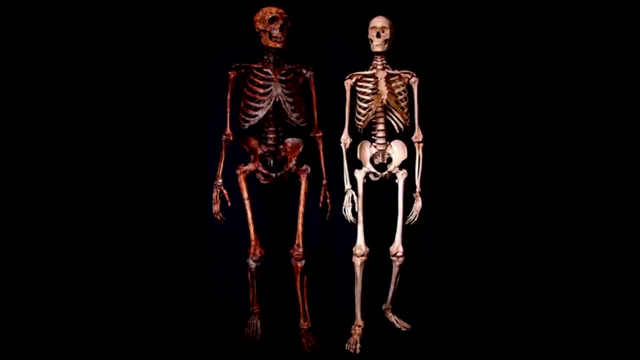 Many other small features about Neanderthal bodies differed from our own. The distal digit of their thumb was longer than modern humans. This would have provided them with a comparatively wider and stronger grip. Their rib cages were wider and barrel shaped. They had longer and straighter ribs. that may have provided them with room for a larger diaphragm and possibly a greater lung capacity. 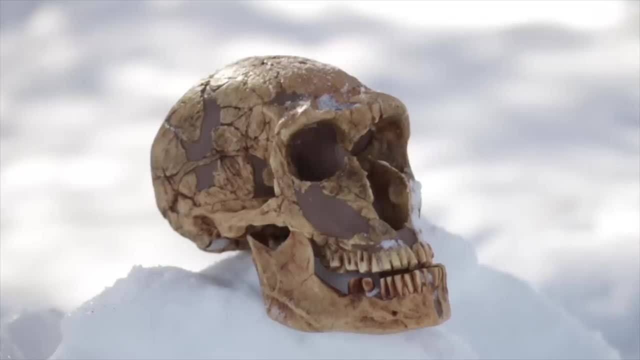 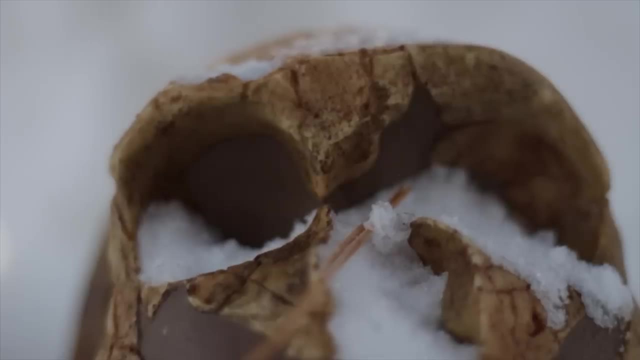 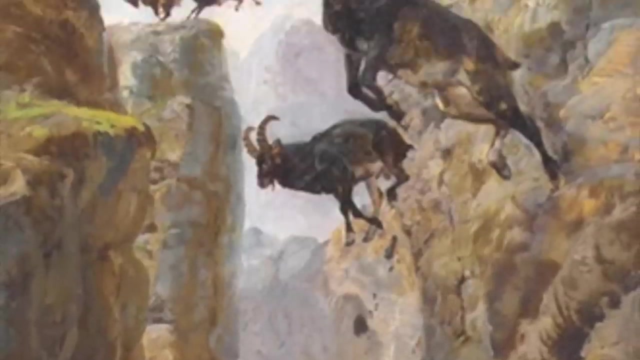 Moving up from the body. their skulls contained many interesting differences. When looking at a Neanderthal up close, the first thing you might notice is their large brow. This brow was useful at protecting their face and eyes against heavy blows from animals, rockfalls and other environmental hazards. 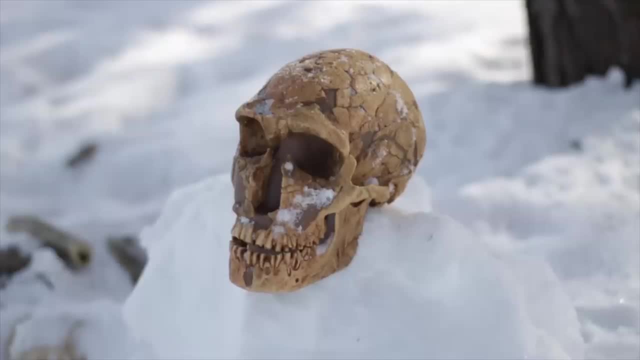 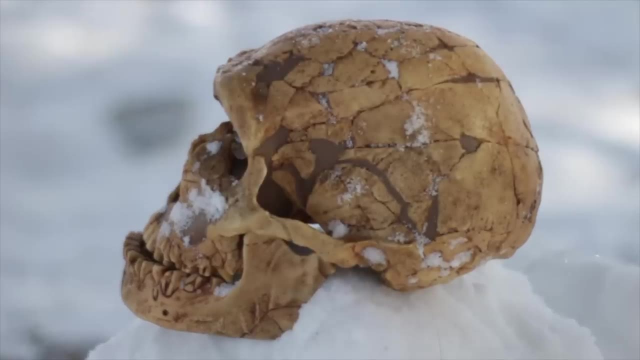 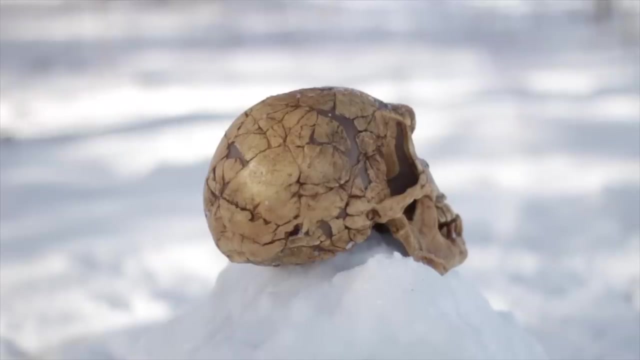 You may notice their large eyes, larger than any modern human you have met. Along with these eyes, they also had a bump on the back of their skull called the occipital bun. This feature may be responsible for a number of purposes, but one of them may have been to make room for the larger occipital lobe in Neanderthals. 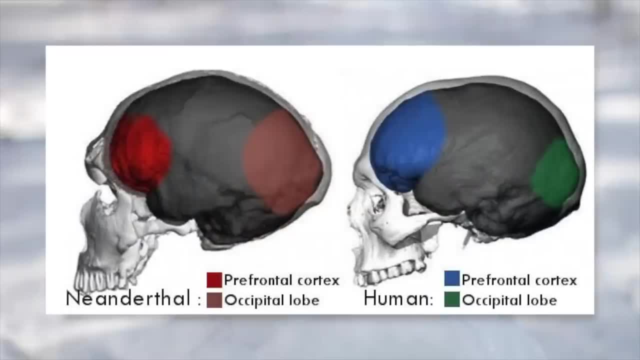 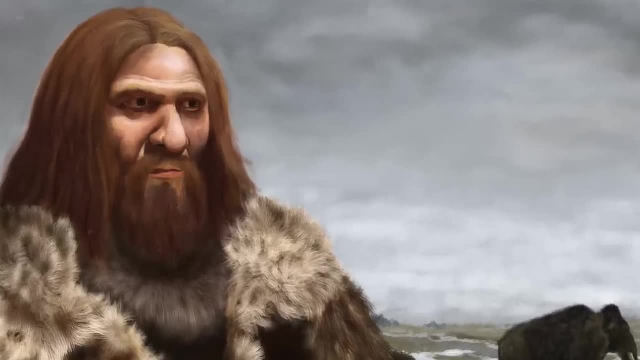 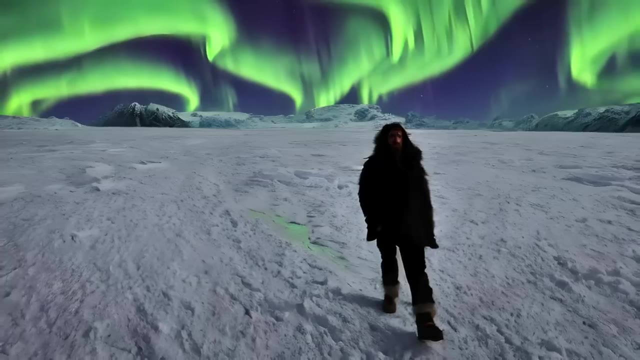 The occipital lobe is responsible for visual perception. Their large eyes, in conjunction with their large occipital lobes, would have given them better vision, especially in low light conditions. This may have considerably helped them hunt during dawn or dusk. They also had large sinuses and olfactory bulbs, which would have provided them with a good sense of smell. 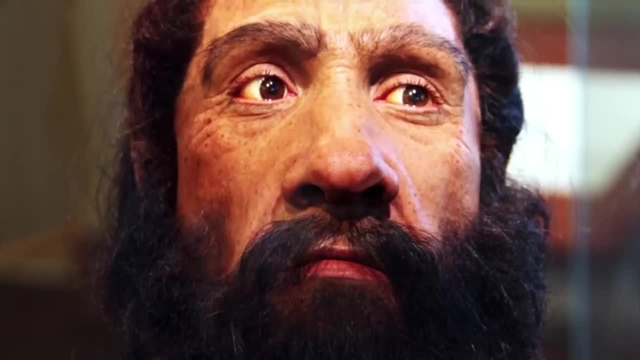 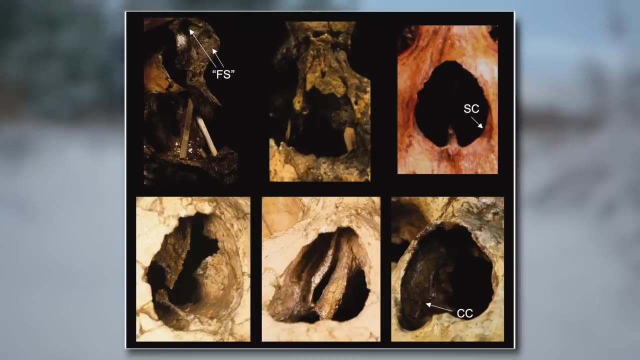 Sometimes they are depicted with very large noses, but in reality their noses would have been similar in size to modern humans, though their sinuses were nearly a third larger than living populations. They would have been able to take in almost twice as much air as modern humans through their noses. Their sinuses may have also been used to warm up air before it entered their lungs. In fact, their sinuses show some similarities with modern arctic populations. Another part of their appearance which may seem strange is their lack of a chin. We perceive a chin to be a normal part of a human face, when in fact we are the oddballs for having them. 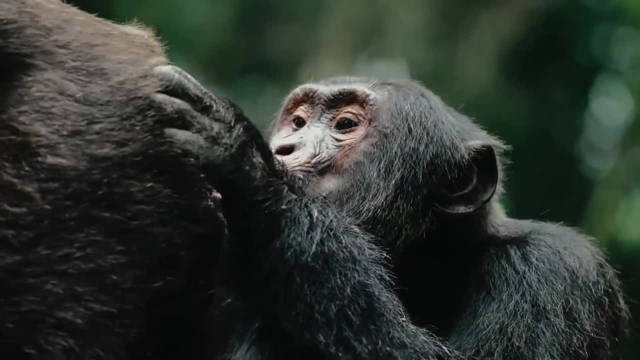 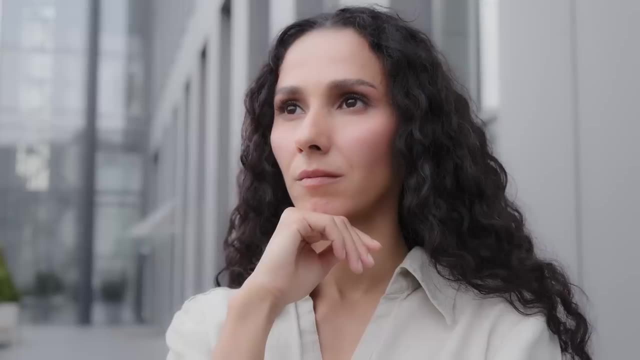 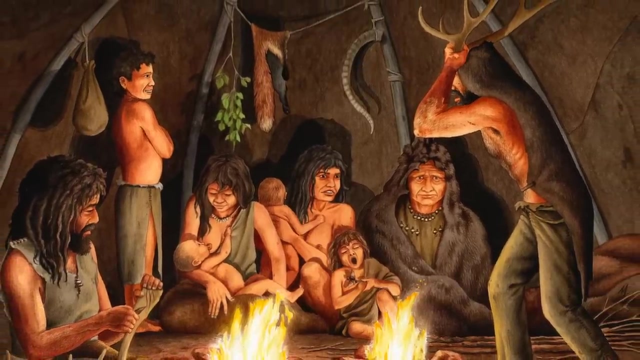 Every other species of hominin and primate lack a chin, because chins are pointless, They do not help with chewing or anything mechanical. They are purely for show. Some believe that they developed as our species became increasingly social and less aggressive. This process of self-domestication may have decreased testosterone levels. 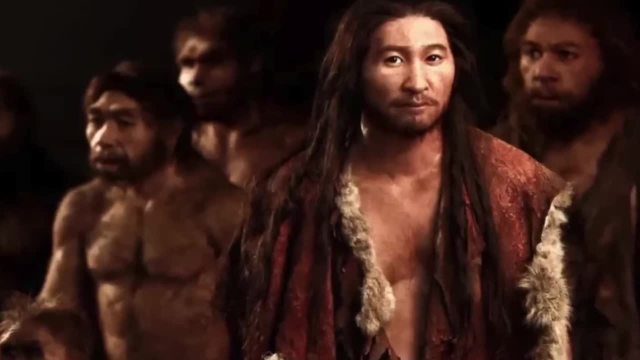 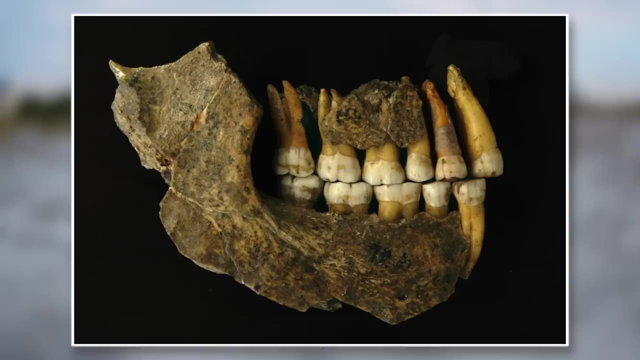 in males and created our modern facial structure. We do not know for sure what the role of the chin was, but we know that Neanderthals didn't have them, Though without a chin. their actual jaws were quite large, They had shovel-shaped incisors and large molars. Their molars also differed from modern humans in that they had an enlarged pulp. Infant Neanderthals also got their teeth up to four months earlier than modern humans. This would have allowed them to eat solid foods significantly earlier. The last feature of the Neanderthal skull that you would notice quite easily. 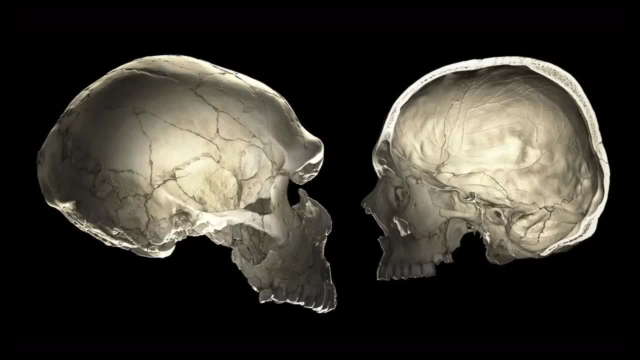 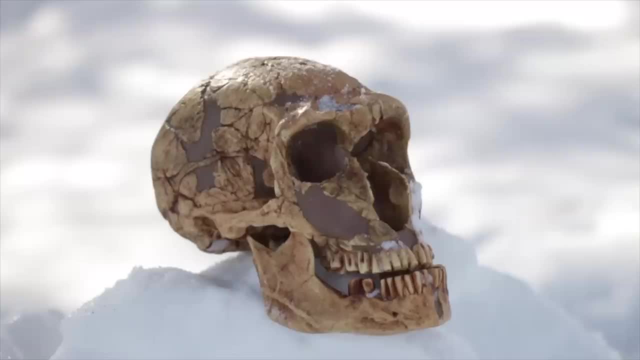 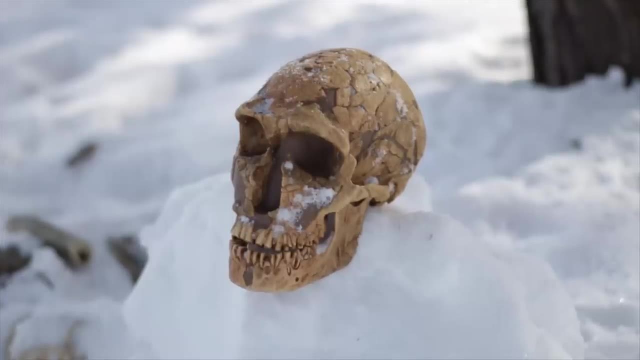 is their sloped back flat skull. Unlike modern humans, which have a globular skull, Neanderthals had a flatter, elongated skull. This skull, of course, housed their large brain. Male Neanderthals averaged a brain size of 1,640 cubic centimeters. 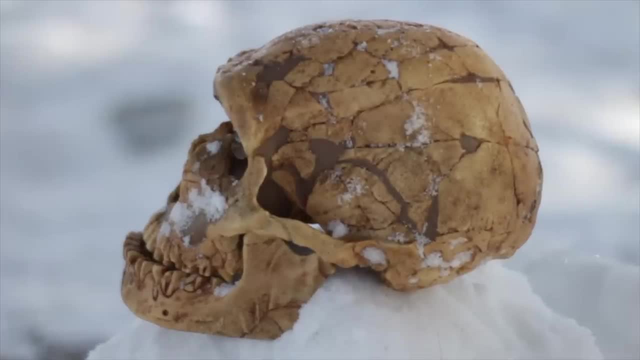 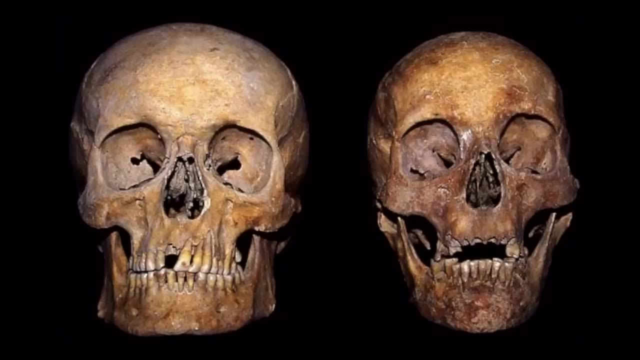 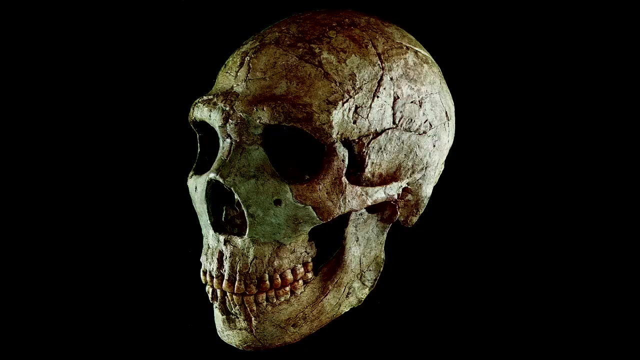 while females averaged 1,460 cubic centimeters. In comparison, modern European males averaged 1,360 cubic centimeters, while females averaged 1,200 cubic centimeters. The largest Neanderthal brain case, A-Mod. I had a brain size of 1,736 cubic centimeters. 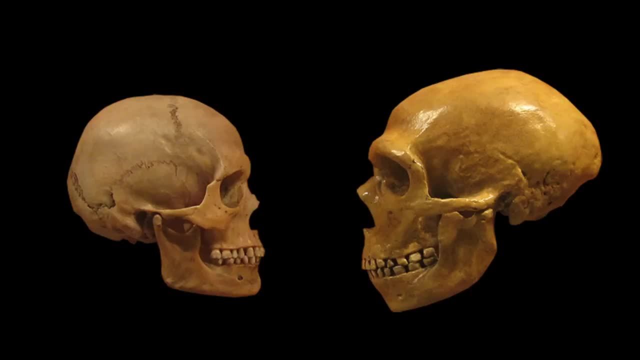 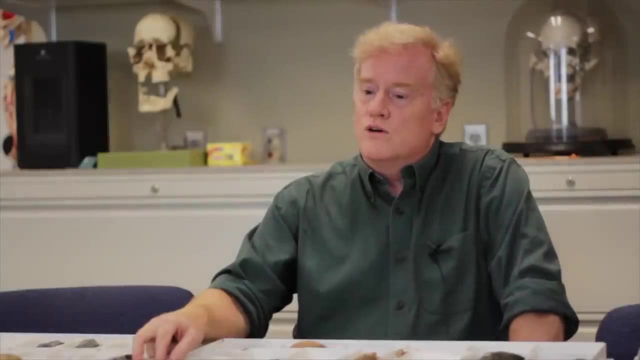 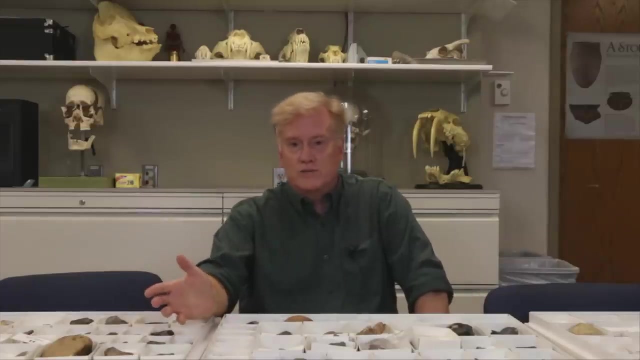 At face value, it seems that Neanderthals had significantly larger brains than our species, but it is more complicated than that. Brains were very large, but they actually weren't as large as some people actually portray them to be, So they're frequently described as being the largest in terms of cubic centimeters. 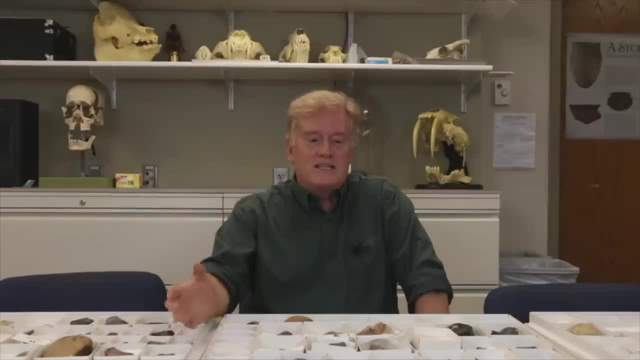 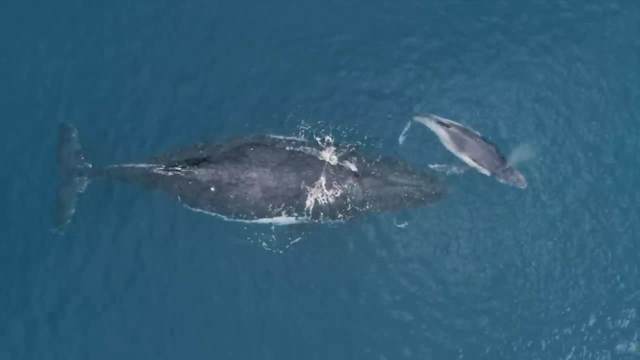 in the hominin lineage, but brain size is actually related to body size, So whales have much bigger brains than we do, but they also have bigger bodies, And so if you control brain size to body size with Neanderthals- and this is usually done by looking at the size of the orbit of the eye- 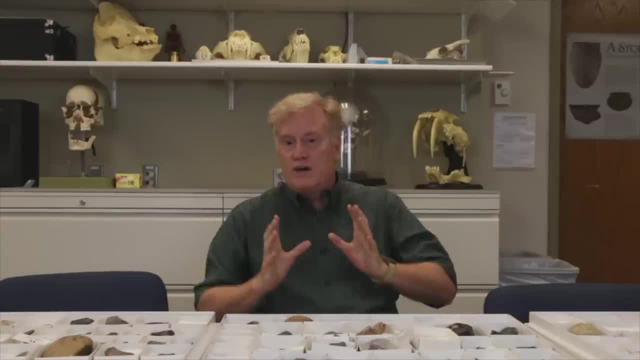 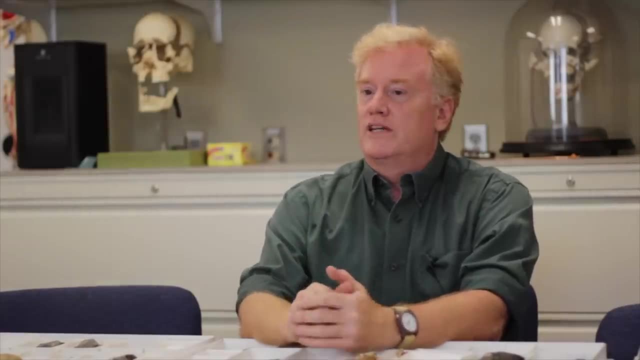 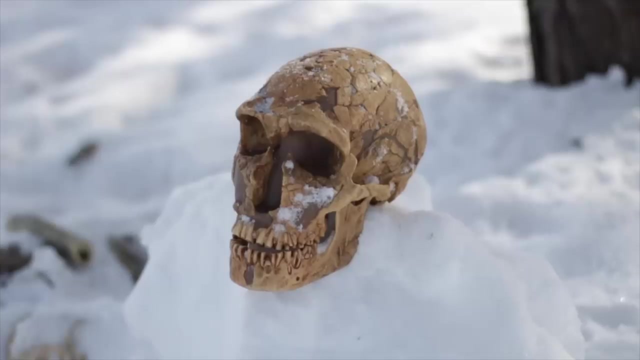 which reflects body size, more so than the rest of the cranium. Neanderthals are a little bit less big in brains, relative to body size, than modern humans are, So they're not the brainiest of the hominins, but then again there are many humans alive today who have smaller brains by body size than Neanderthals. 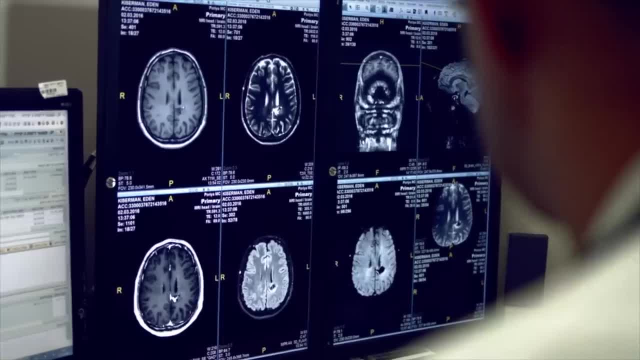 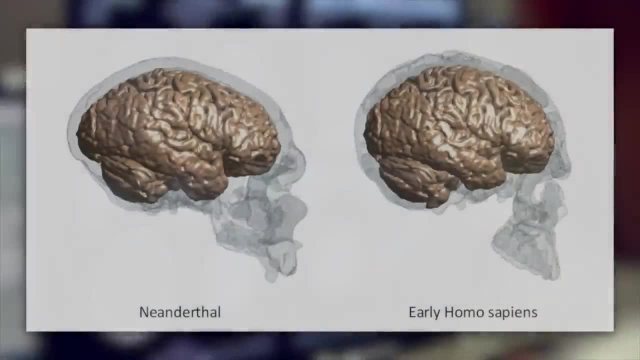 so they're within the range of a modern human. Besides overall size, the organization of a brain is another very important aspect to its function. Endocats of their brain have shown that they had smaller parietal lobes and a smaller cerebellum. 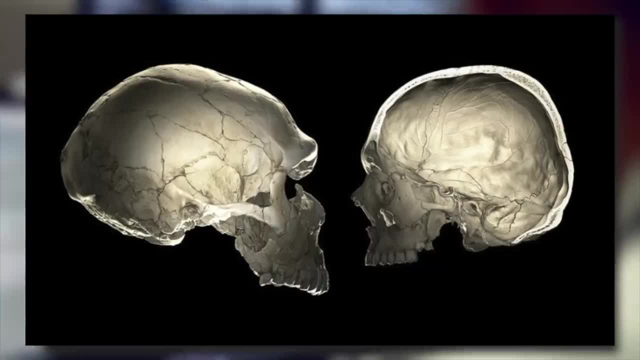 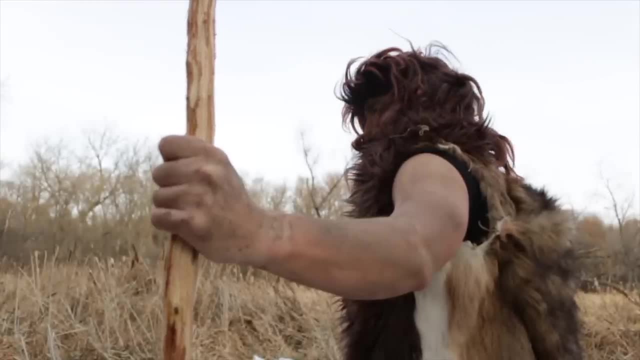 Both of these areas of the brain are very important for a number of things, including creativity, muscle memory, language and social abilities. This does not mean that all Neanderthals were necessarily less intelligent in these areas, but it does mean that there were differences. 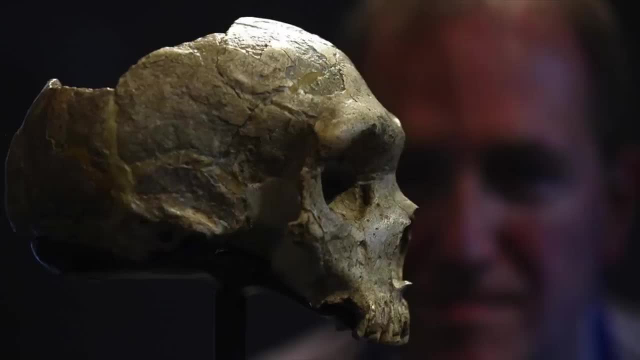 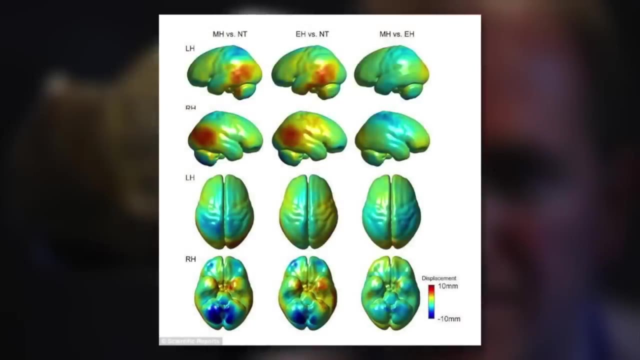 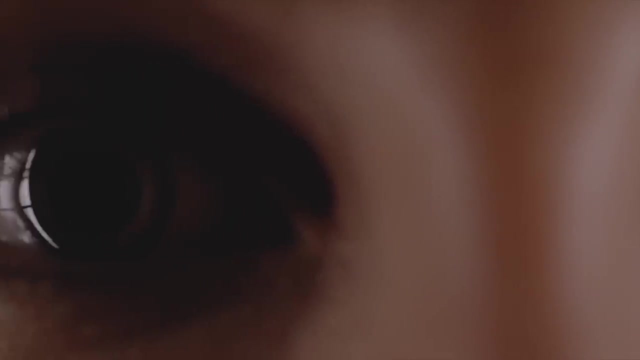 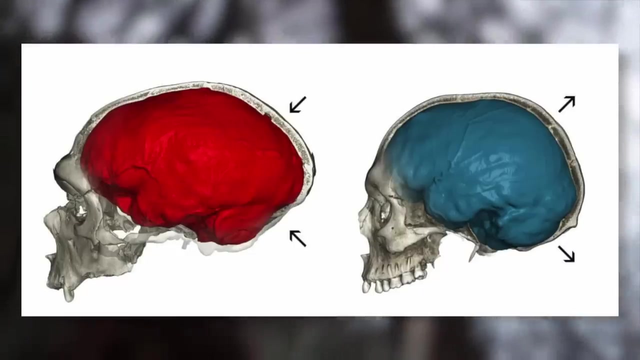 The temporal lobe is associated with processing language, pattern recognition, perception and memory acquisition. As mentioned earlier, they had larger occipital lobes and olfactory bulbs. These structures are responsible for seeing and hearing, among other things. Compared to modern humans, a greater proportion of the Neanderthal brain was devoted to visual and somatic systems. 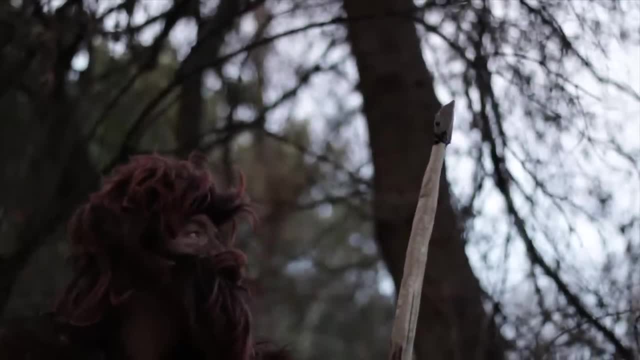 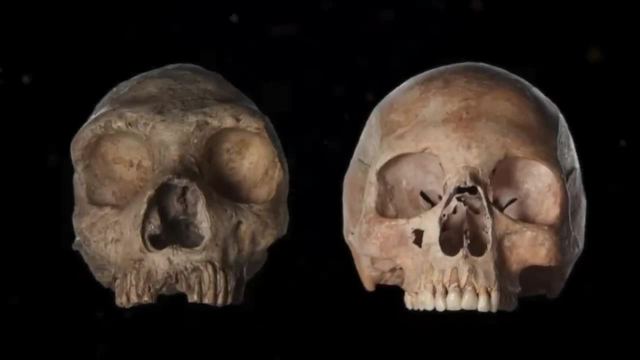 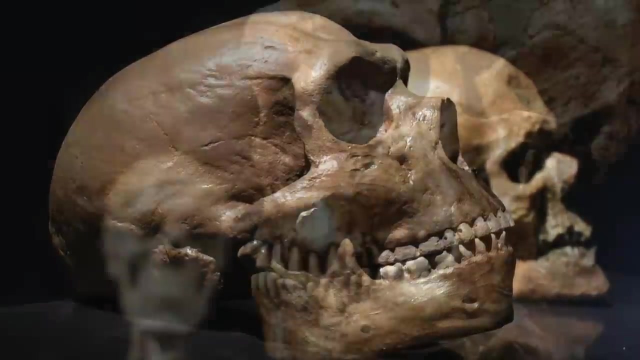 This left less neural tissue over for other areas of the brain in Neanderthals. Homo sapiens, on the other hand, have smaller than expected visual areas for a primate of our size. Therefore, it wasn't that Neanderthals had abnormally large eyes and visual cortex. 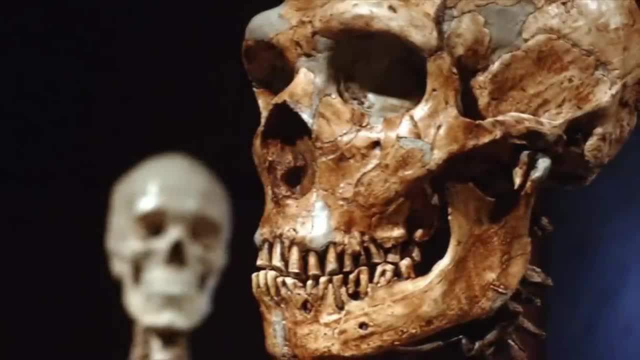 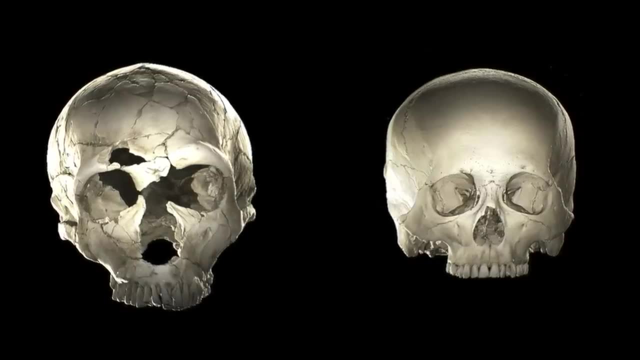 but that Homo sapiens actually have abnormally small visual systems. This seems to have left sapiens with more neural tissue to devote to other regions of the brain. Neanderthal skulls show different rates of brain growth, with individuals reaching maturity faster than in modern humans. 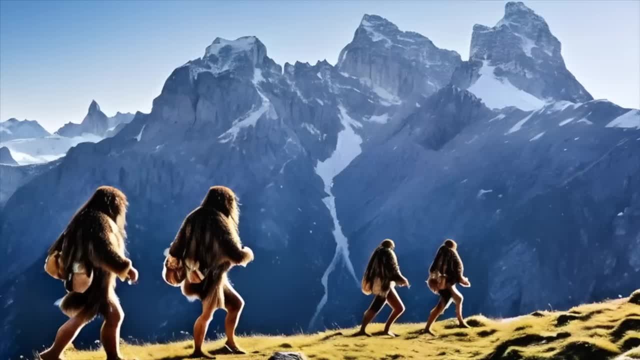 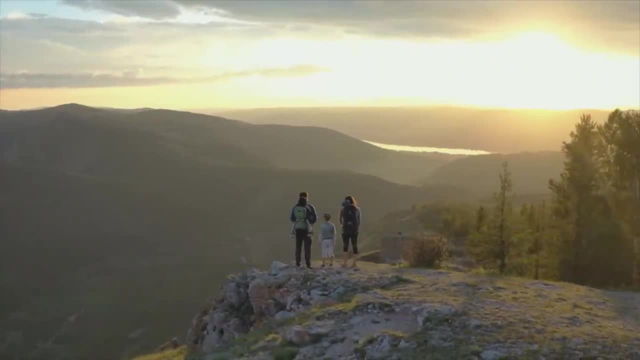 with individuals reaching maturity faster than in modern humans. It would have taken a Neanderthal around 15 years to reach adulthood. That is nearly a decade earlier than it takes modern humans to reach adulthood. The brains of Neanderthals are not comparable to any modern human. 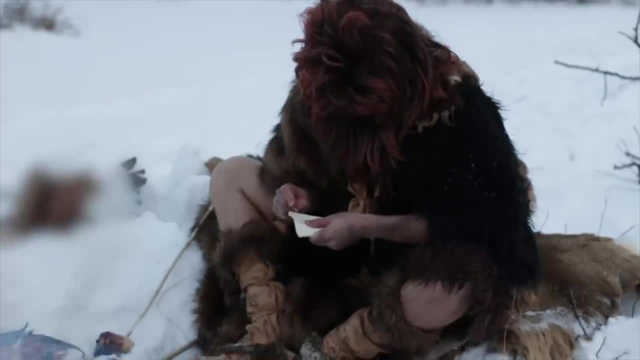 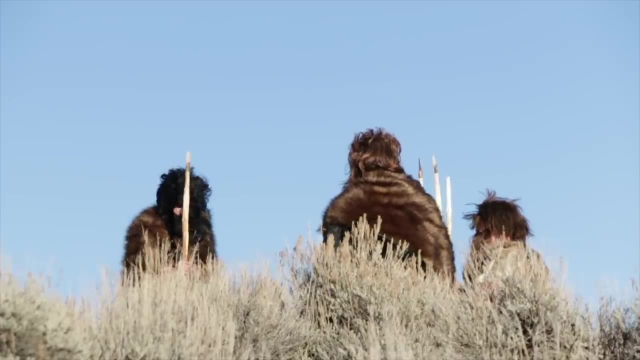 The differences they had are undoubtedly responsible for the different traits that they left in the fossil record. It is easy to focus on all the similarities that Neanderthals had with modern humans, but we cannot let them overshadow the fact that they were different. 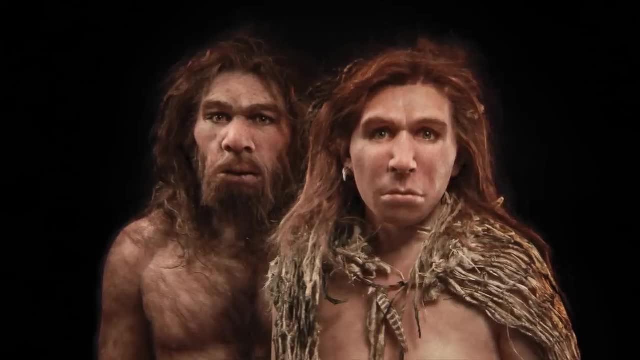 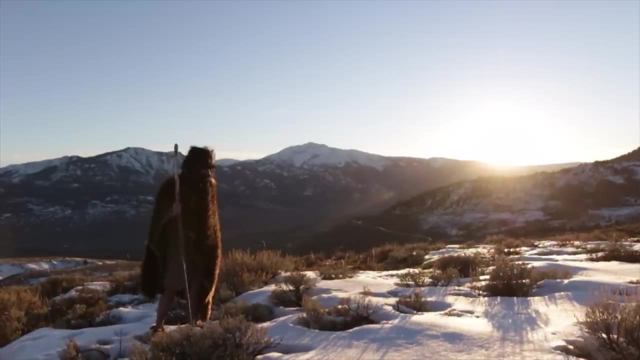 Though another way that Neanderthals were similar to our species is that they had a range of skin, hair and eye colors. This is due to the fact that they occupied a wide geographic range. A Neanderthal from France would have looked quite different than one from the Middle East. 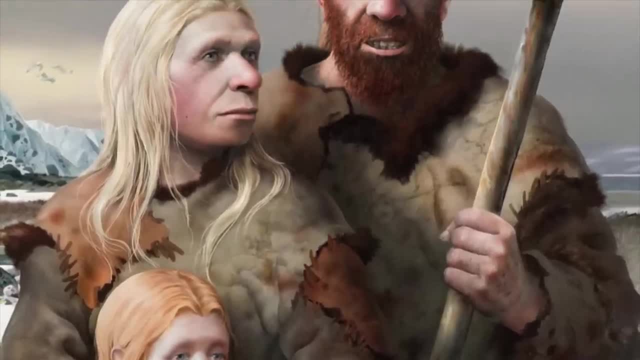 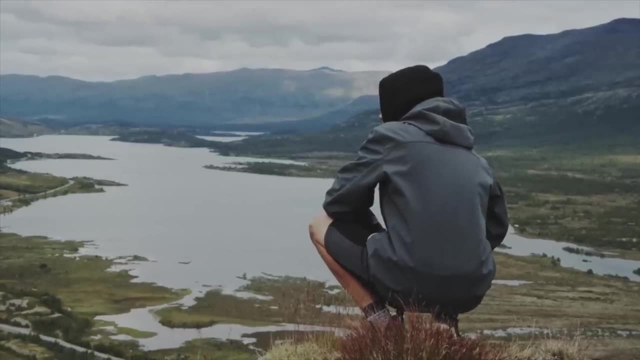 Even Neanderthals in the same populations would have had varied appearances, just like modern Europeans. However, we must be careful in assuming that if modern humans living in a region had light skin, then Neanderthals that once lived there had light skin too. 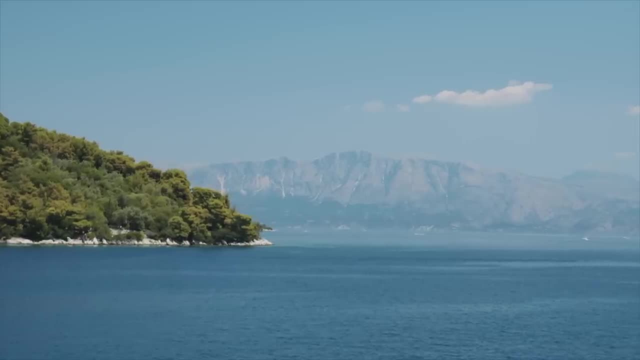 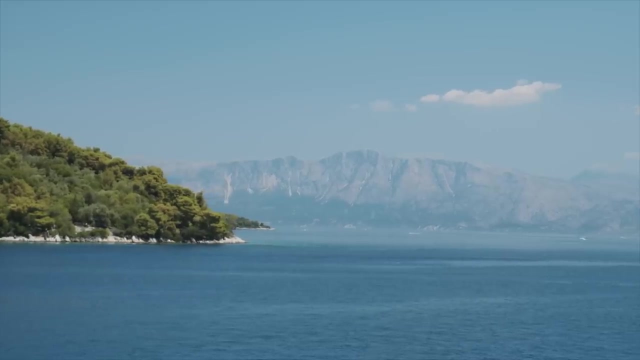 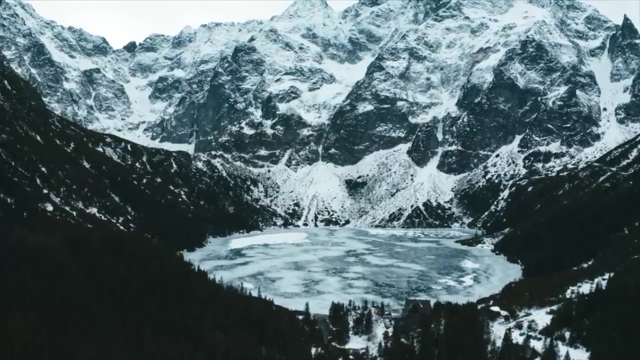 DNA analysis from three Neanderthal females from Southeastern Europe indicates that they had brown eyes, a dark skin color, with two of them having brown hair and one of them having red hair. Other Neanderthal populations living in the Middle East and even in Siberia had dark skin, eyes and hair. 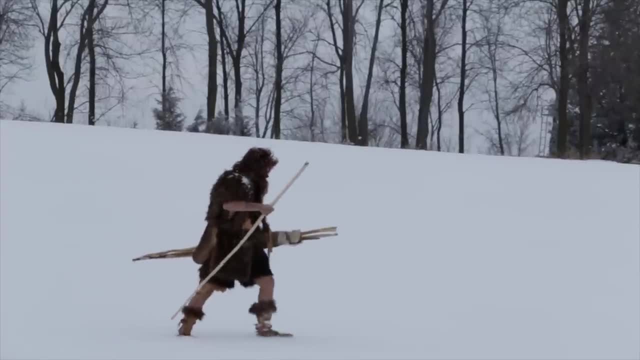 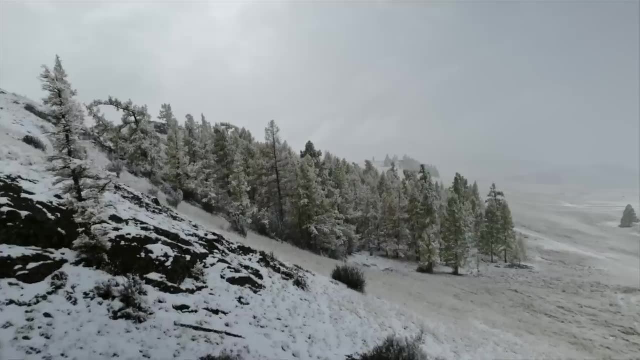 Even though lighter skin is more frequent at higher latitudes in modern Homo sapiens, the same wasn't necessarily true for other human species. Both the Neanderthals and Denisovans living in the Altai Mountains of Siberia had a dark complexion. 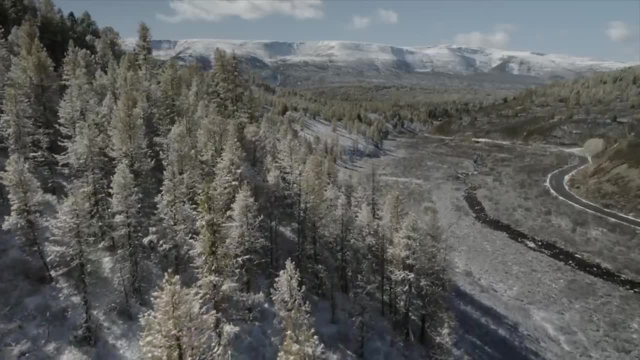 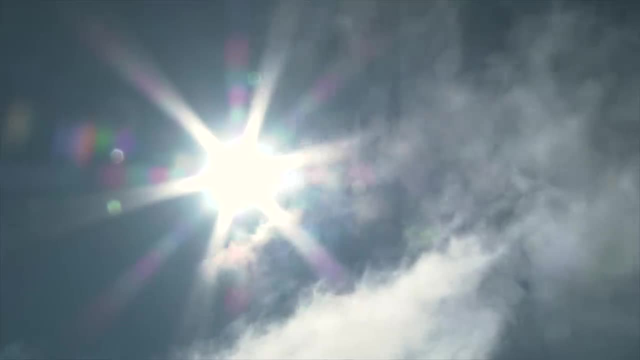 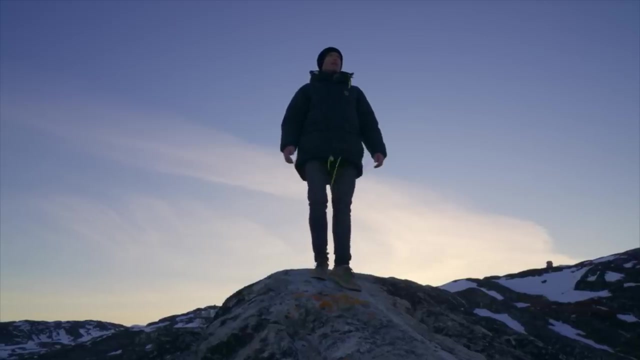 The reason that light skin is more common at higher latitudes in modern humans is generally explained by the lack of sunlight in these environments. Humans need sunlight to synthesize vitamin D. Since sunlight is less intense at higher latitudes, light skin is evolved to absorb more sunlight when available. 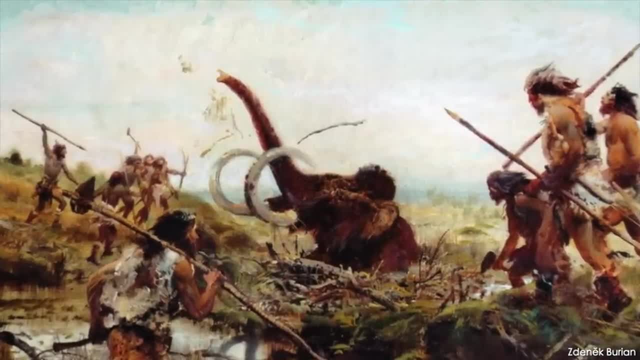 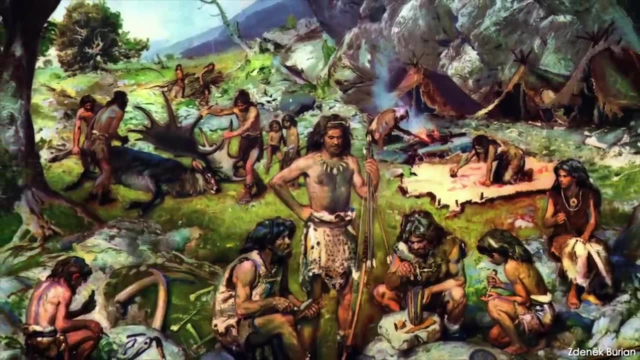 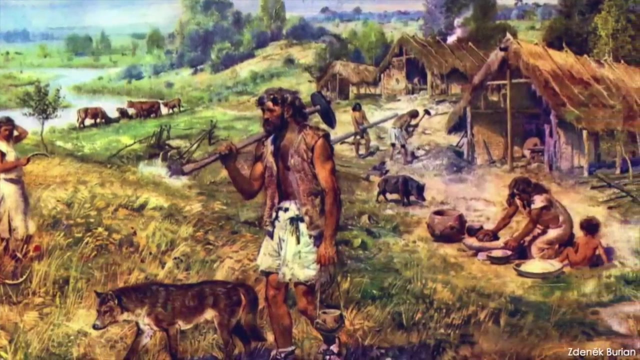 However, Neanderthals and even early Europeans got a lot of vitamin D from their rich diet. It was only in the past 10,000 years that Europeans actually evolved light skin. The prevalence of light skin in populations in the modern day is generally due to agricultural diets. 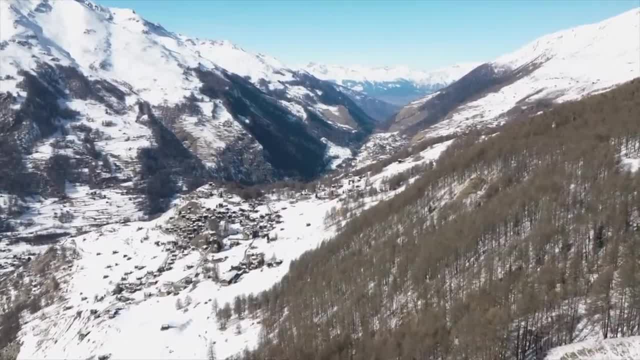 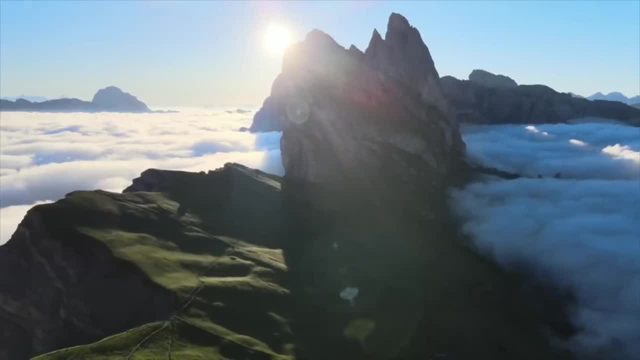 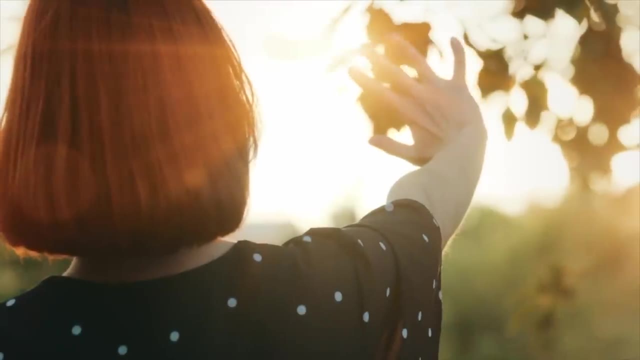 Due to this, it isn't surprising that many Neanderthals living in Europe would have had relatively dark skin, though not all did. Two different Neanderthal individuals from Italy and Spain both provided fragments of the MC1R sequence. In modern humans, this gene is responsible for light skin and red hair. 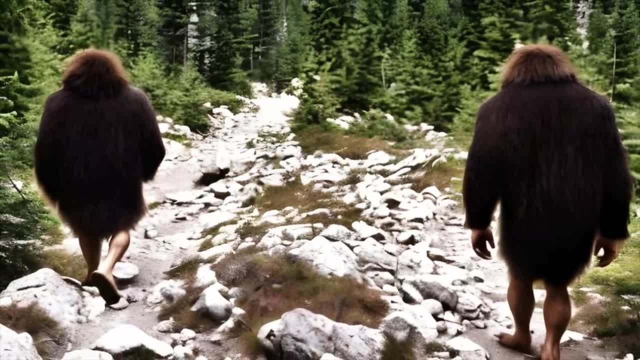 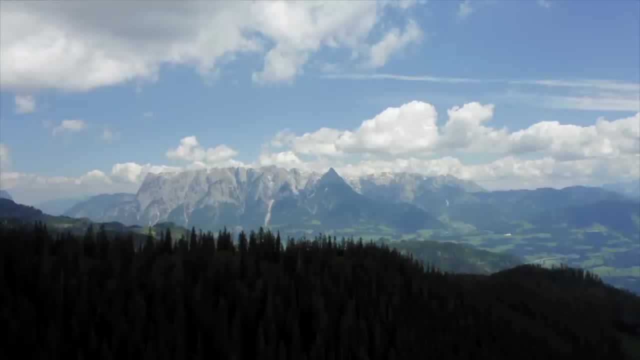 However, the MC1R gene that the researchers had found was different than the one found in modern humans. In order to test if this gene would have had a similar effect in Neanderthals, they inserted the Neanderthal gene into human pigment cells. 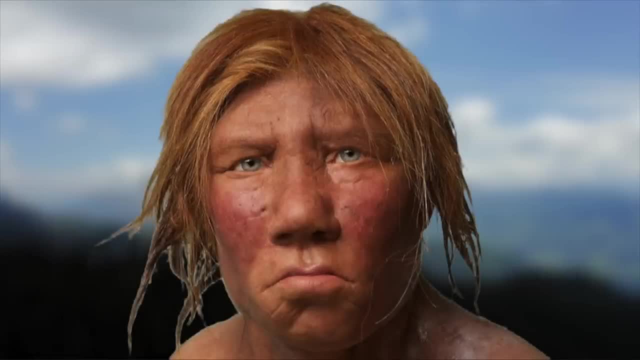 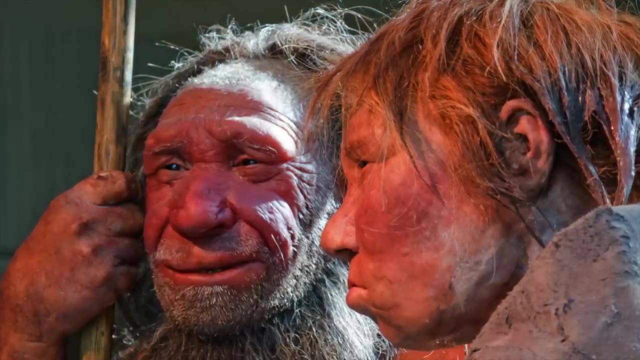 The gene produced the same loss of function that gives redheads their unique coloration. This study provided solid evidence that some Neanderthals did indeed have light skin and red hair, though the frequency of this phenotype remains unknown, Just as in modern humans. 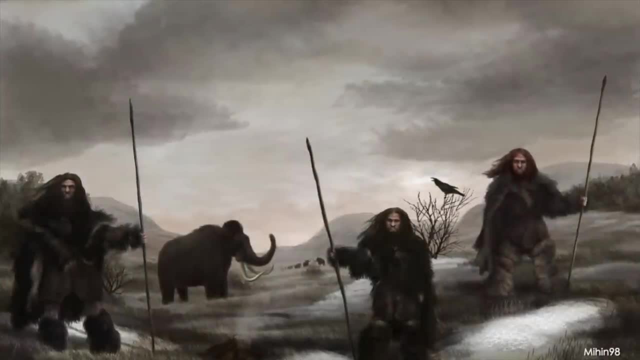 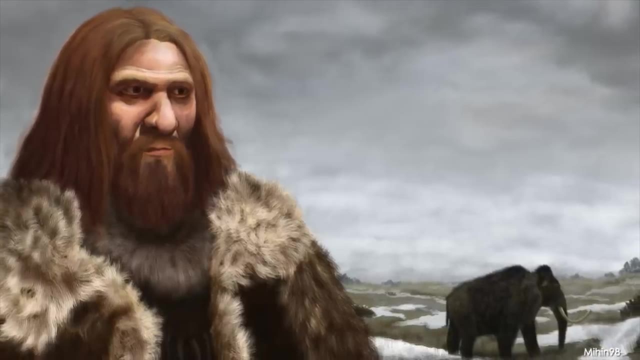 red hair was probably not very common in Neanderthals, as it was not present in other sequenced individuals. The phenotype was likely more common in northern regions, just as it is today. Neanderthals undoubtedly had a wide array of skin, hair and eye colors. 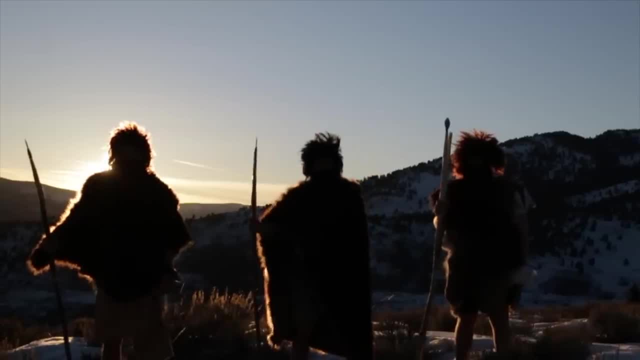 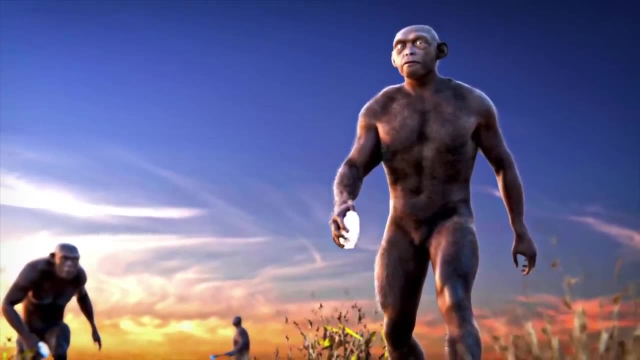 Another question regarding their hair is: how much body hair did they have? From genetics, it is known that the genes that make modern humans furless date back to around 1.7 million years ago, Since this is well before our last common ancestor with Neanderthals. 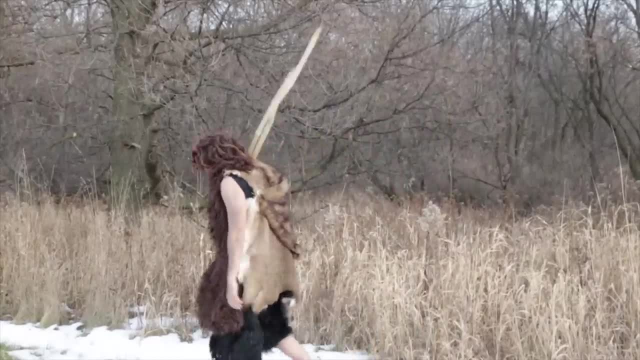 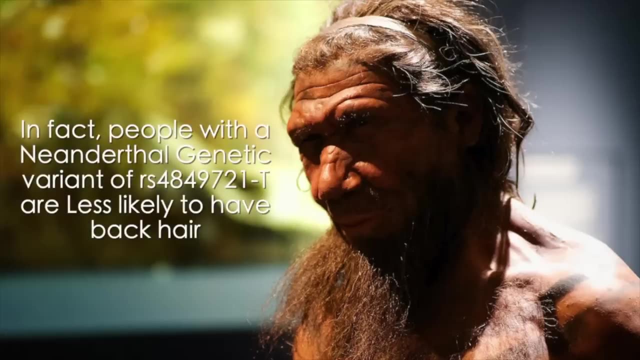 we know that Neanderthals would have had furless skin. Genetics also corroborate this. Just like us, they still had body hair, but even the hairiest Neanderthals would not have had actual fur. Anatomically, Neanderthals are fairly similar to modern humans. 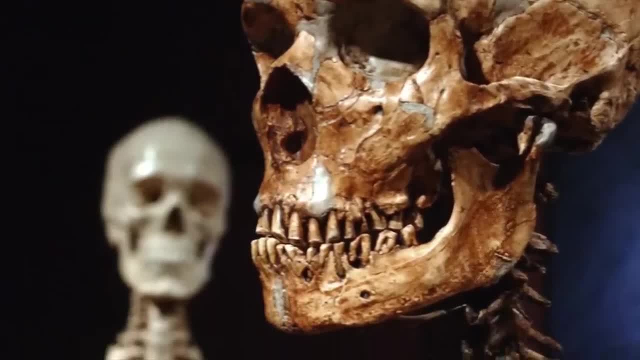 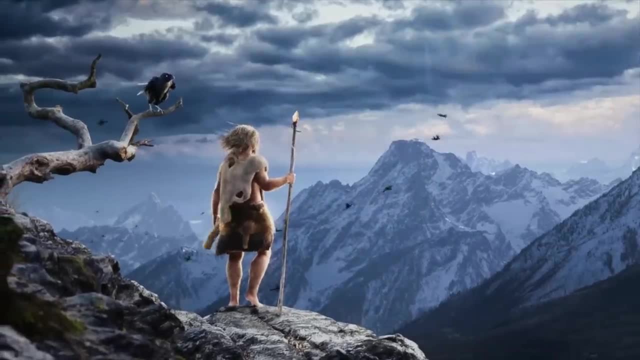 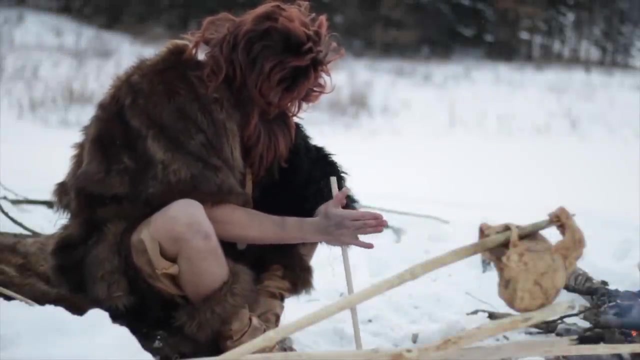 though their differences cannot be overlooked. Their anatomy was far different than any modern human alive today, even if at the surface we vary so much. Neanderthals used a vast array of technologies to survive their challenging world. Many materials and techniques were used to create a lot with very little. 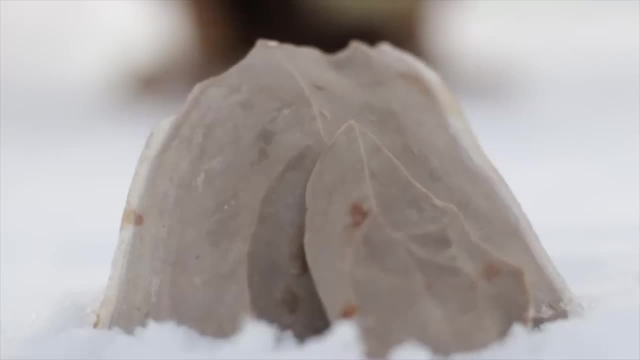 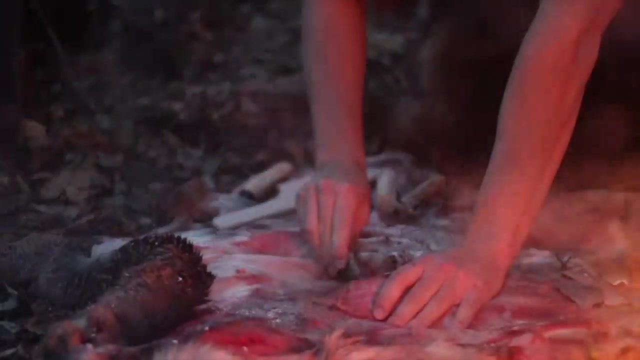 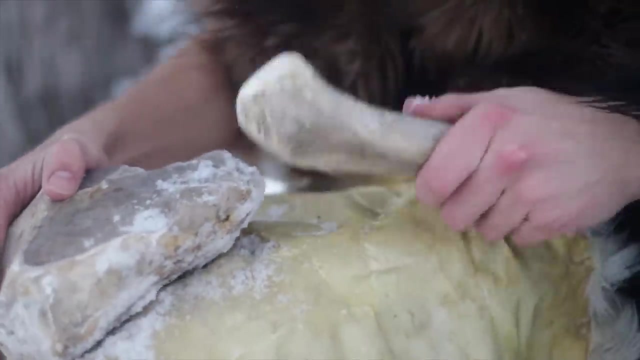 Since stone does not decay like biology, thousands upon thousands of Neanderthal stone tools have been recovered. This has allowed us to learn an incredible amount about their lives. To understand these tools, we must first understand the evolution of stone tool technology in general. 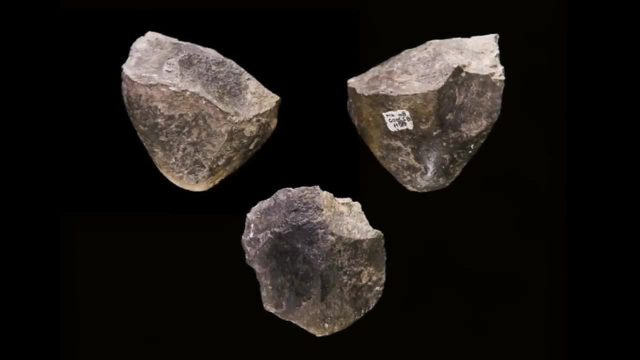 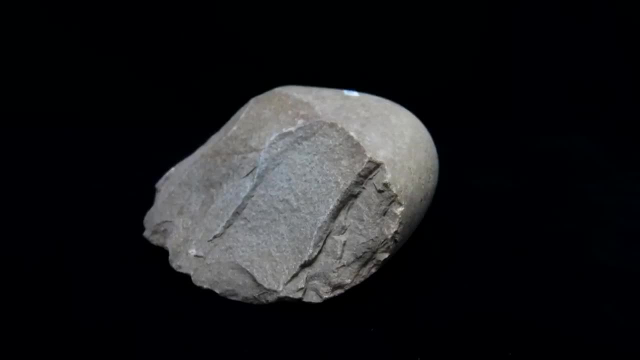 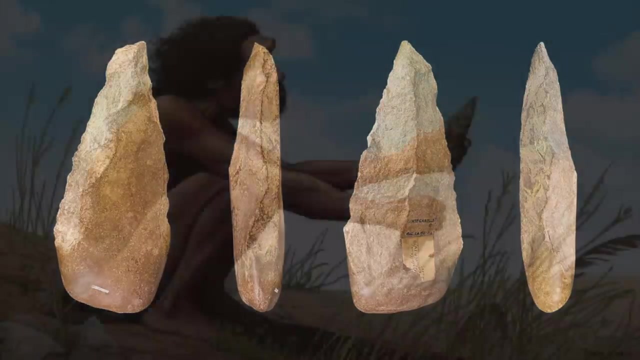 As mentioned earlier, the first stone tools made by our ancestors were simple hand axes with a few flakes taken off. This simplistic technology is considered mode one by archaeologists. Mode two technology, also known as Acheulean technology, would appear with Homo erectus around 1.7 million years ago. 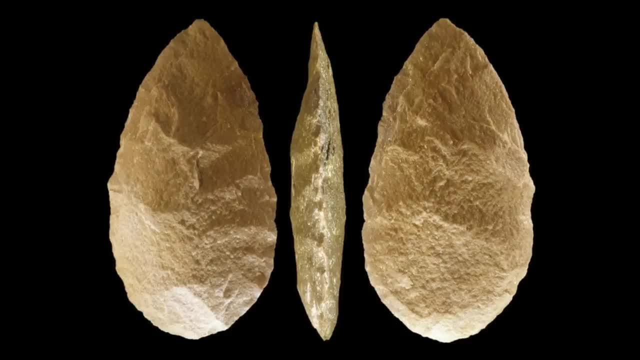 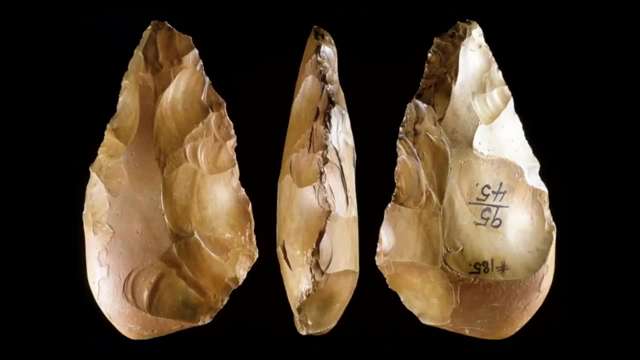 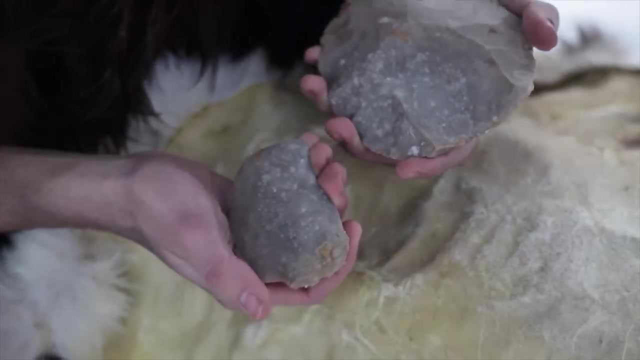 Stone cores were worked symmetrically on both sides to create much more refined hand axes. There was not much of a strategy to creating flakes or to utilizing the material effectively. This would change roughly 300,000 years ago with the emergence of Levallois technology. 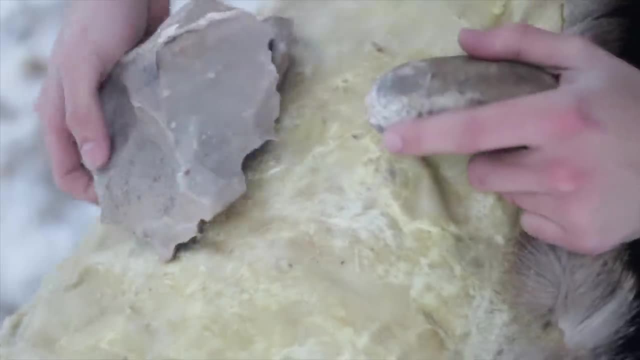 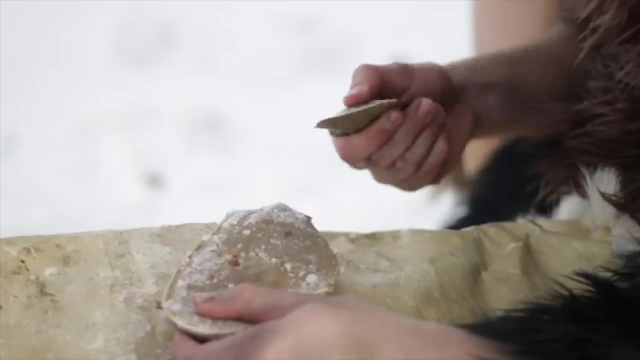 The Levallois technique, also known as mode three, appeared throughout Europe, the Middle East and North Africa during the appearance of the first anatomically modern humans and some of the earliest Neanderthals. The creation of the technique lay independently in various regions. 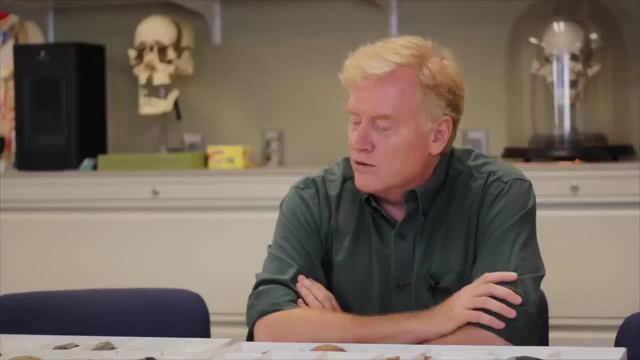 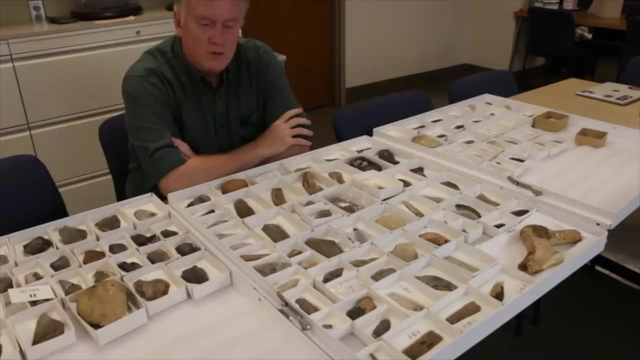 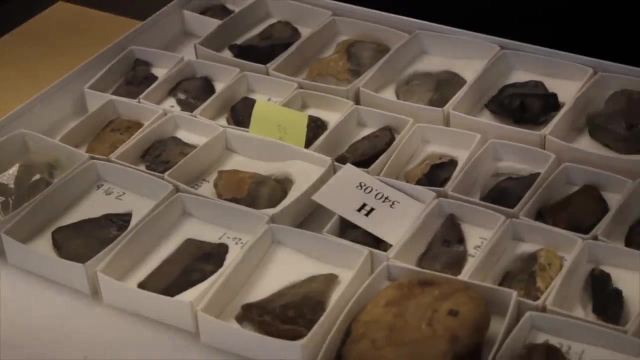 though it is often credited to the Neanderthals. When we first see the classical anatomical forms of Neanderthals, let's say 250,000 years ago, they were utilizing a Middle Paleolithic technology, which is based upon taking a core and striking flakes off the core. 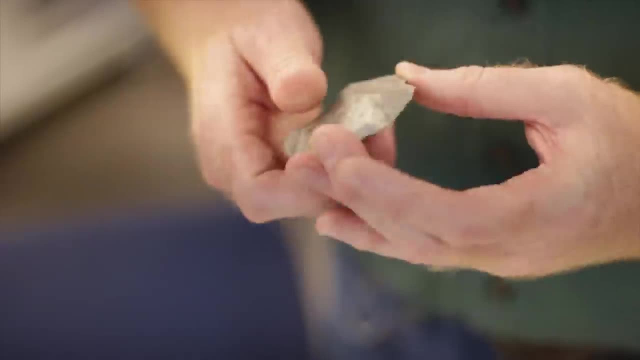 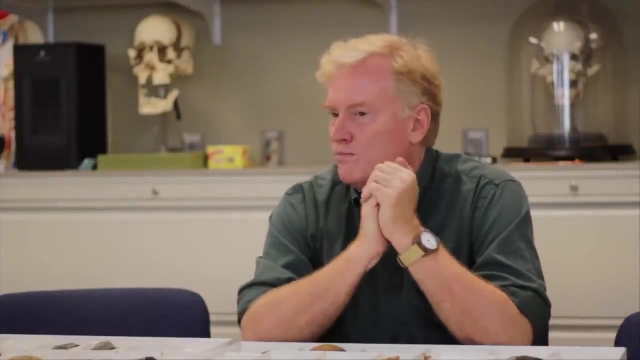 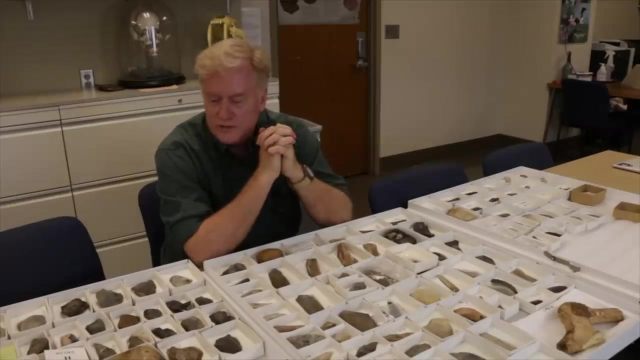 and then utilizing the flakes to do things in terms of whittling wood to make spears with which they could dispatch animals, mostly by throwing, sometimes by stabbing. This Middle Paleolithic technology of cores and flakes is slightly different from what we see in the Lower Paleolithic. 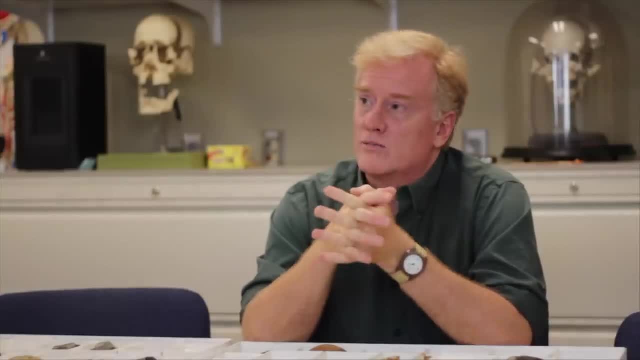 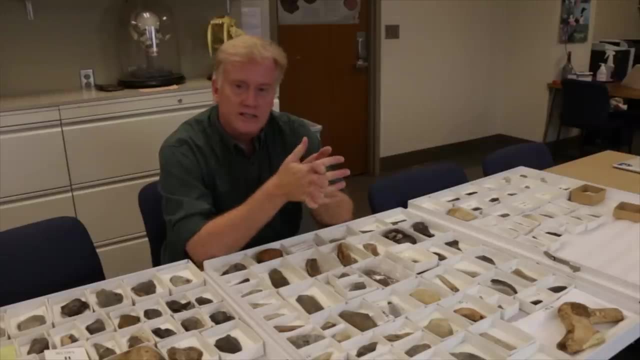 which is what we get mostly with the, let's say, Homo erectus and Homo heidelbergensis, who was immediately before Homo neontalensis, who were using hand axes of what we call the Acheulean culture or technocomplex. 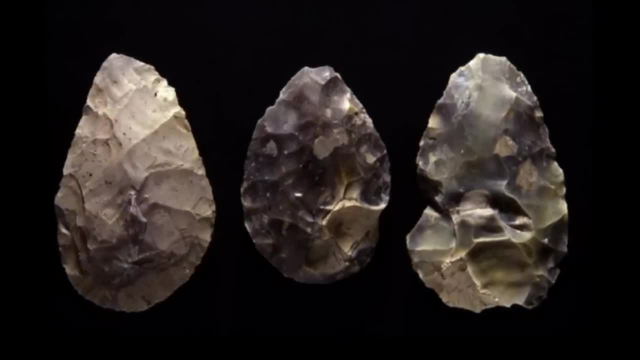 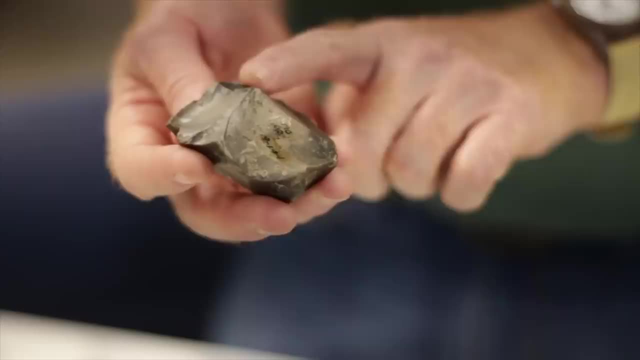 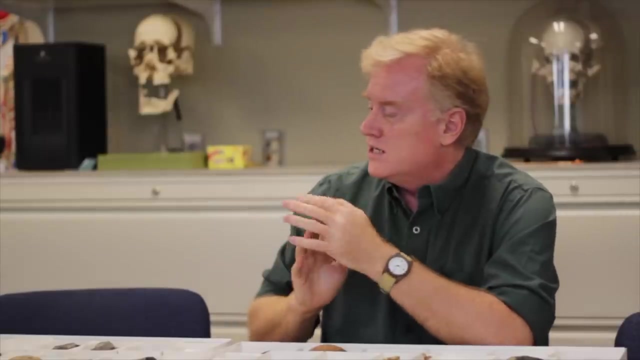 And there they were using a hand axe core that in and of itself was actually usable as a sharp implement for cutting, for pounding and for butchery. The cores in the Middle Paleolithic were not tools in and of themselves anymore, and so the shaping of the flakes. 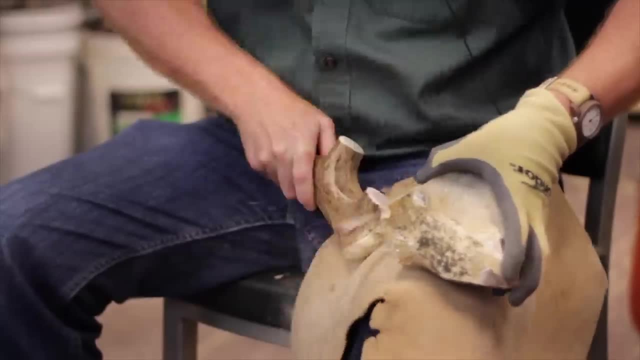 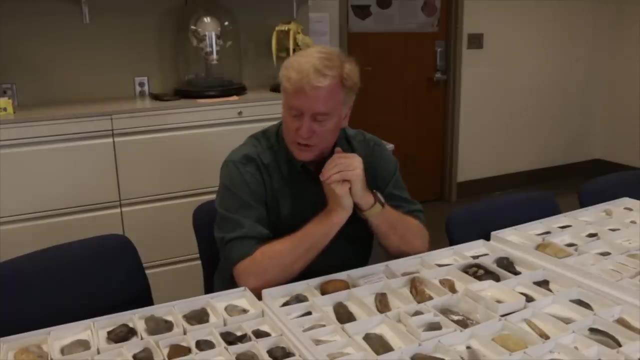 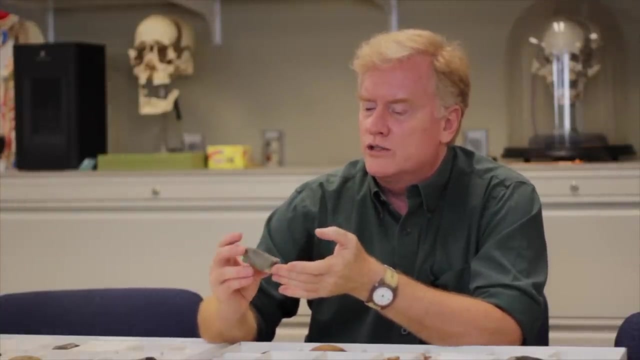 with particular types of reduction patterns. by reduction meaning literally, you're taking flakes of stone off of a core that characterizes what Neanderthals were doing in that time period, And so we can find objects such as this flint core, which was probably originally a nodule of flint. 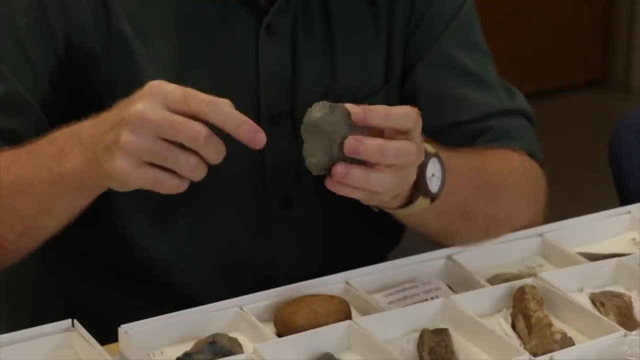 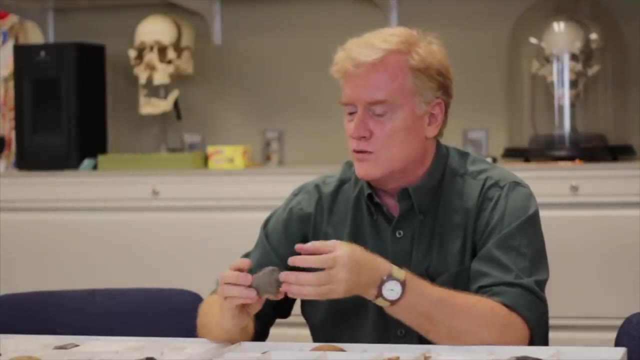 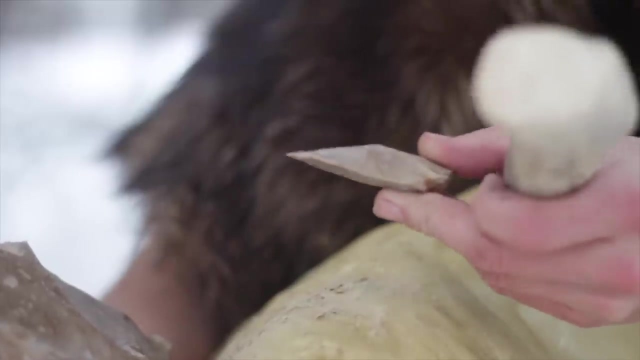 that was subsequently struck with a certain pattern that allows removing flakes that were then utilizable for butchery or for working other materials like wood. The technique itself consisted of striking preferential flakes off of prepared lithic cores. The core was shaped in a specific way. 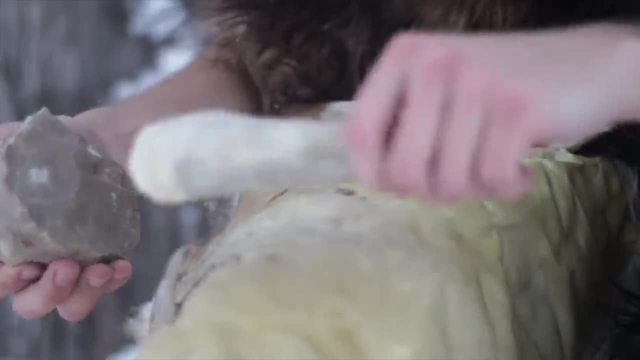 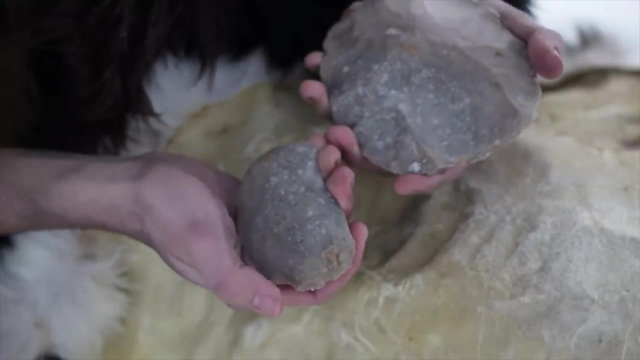 to create a dome-shaped core, known as a tortoise core. A platform was prepared on a high spot which, when ultimately struck, created a large preferential flake. This flaked nearly the entire underside of the core, effectively utilizing much of the material. 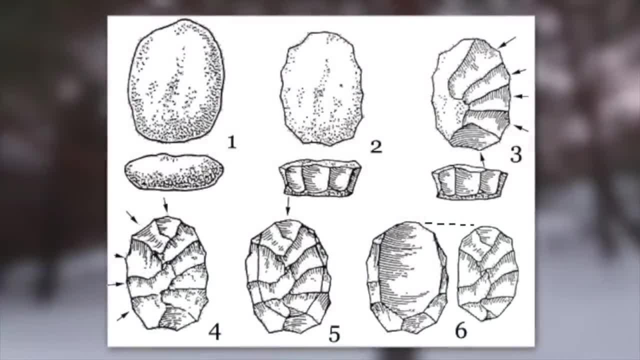 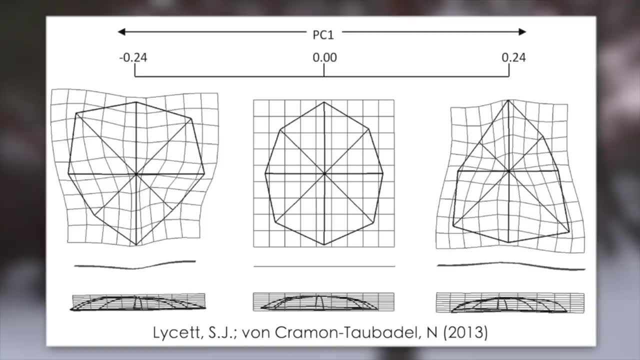 Experiments have shown that the Lavalois core is an economic optimal strategy of raw material usage. It can create the longest cutting edge per weight of raw material. This would have allowed the Neanderthals to be highly mobile, as they could get the most out of their material. 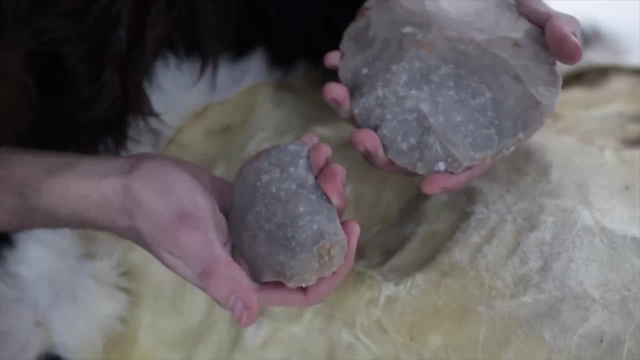 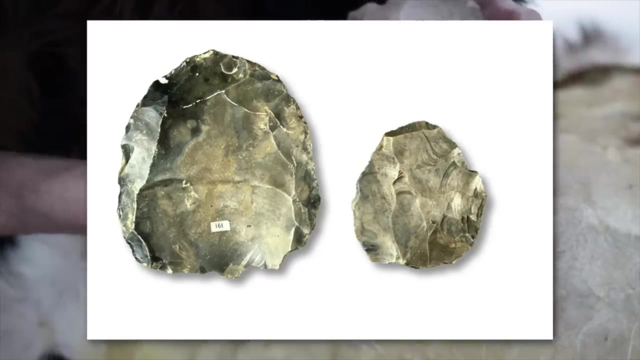 The actual Lavalois flake produced was very sharp on all sides. It would have been very efficient as a butchering tool, much more so than a hand axe. Neanderthals still used hand axes, though for more generalized purposes. 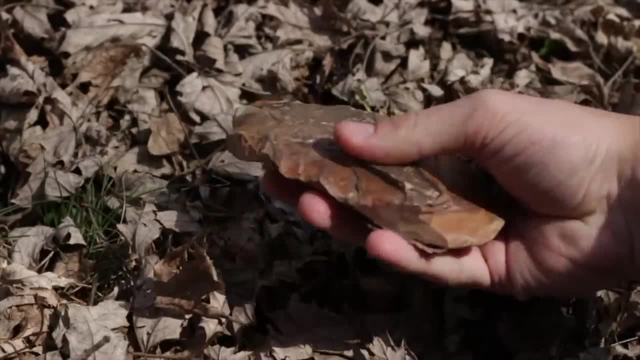 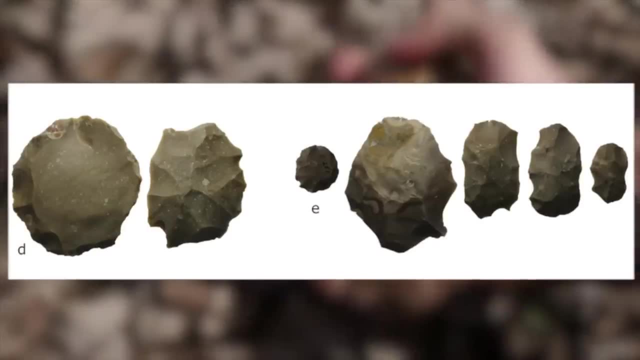 Hand axes are not the most effective butchering tools because of their often steep edges and limited resharpening potential. Lavalois flakes, on the other hand, are quite thin and can be retouched easily. Most of the technology that we see with Neanderthals. 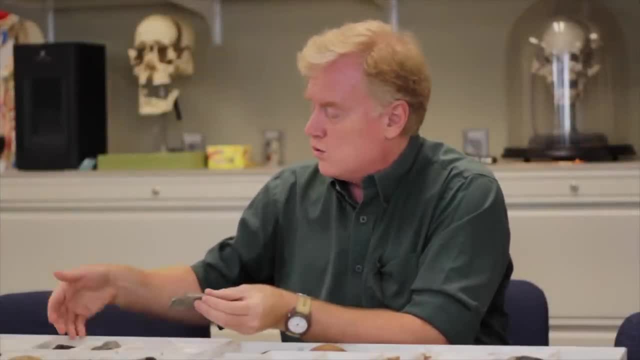 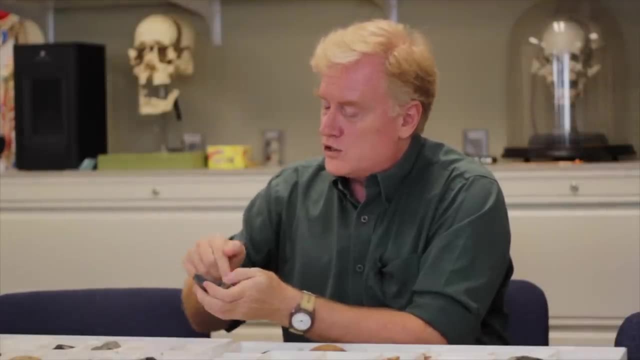 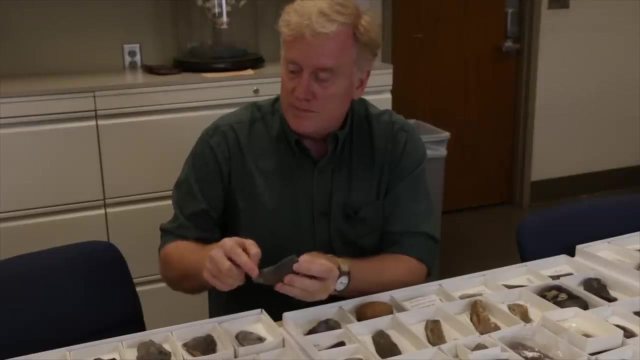 is taking flakes coming off of prepared cores like Lavalois or Discoital, and then the flakes are immediately utilized or they might be subsequently resharpened or their morphology changed by little removals off of the surface such that it makes a different shaped edge. 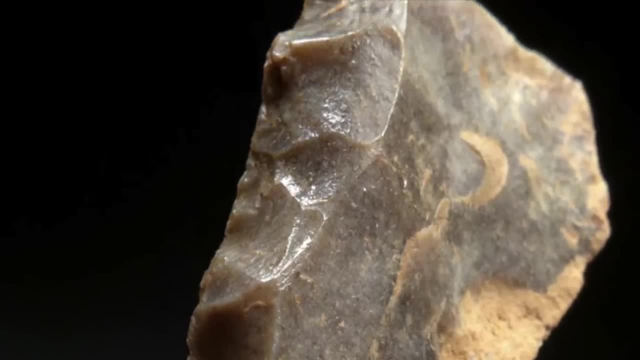 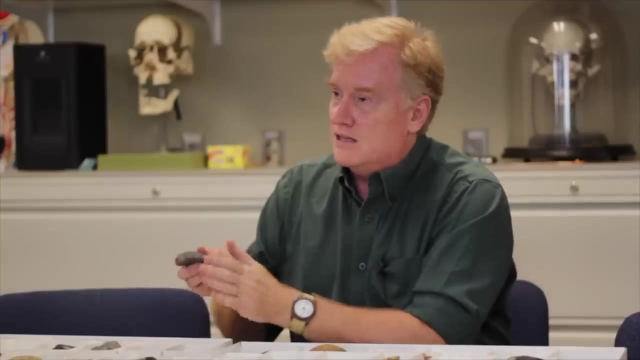 When you make these little removals it makes the edge more acute, so it's not actually sharper. but if the edge has been damaged by use, then by making these little removals you are resharpening it to some extent, And so most of the tools that we get. 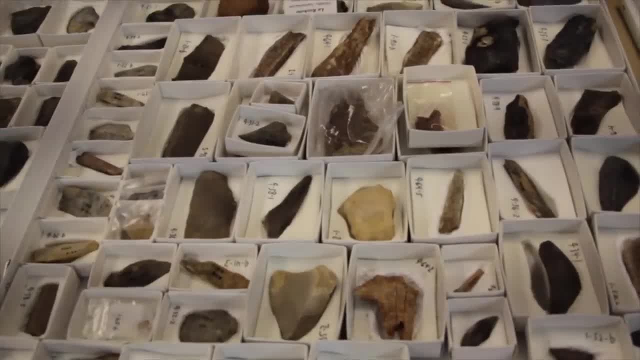 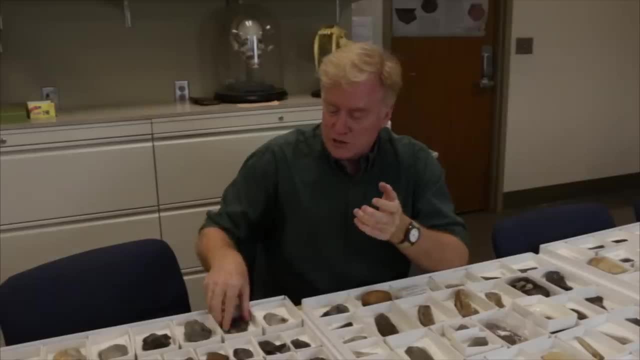 in the Middle Paleolithic that Neanderthals were using are flake tools, meaning that they are not very long relative to their width, and so they're something that you would just hold in the hand and utilize without a haft, meaning there's no handle. 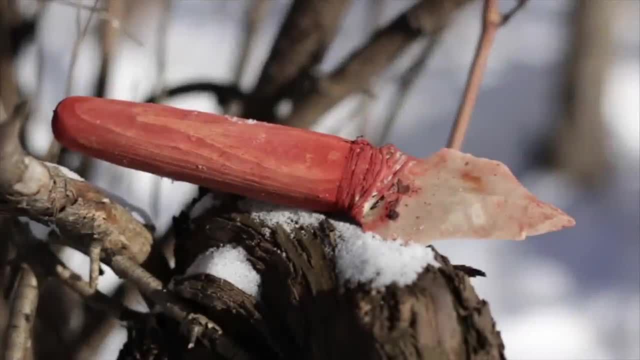 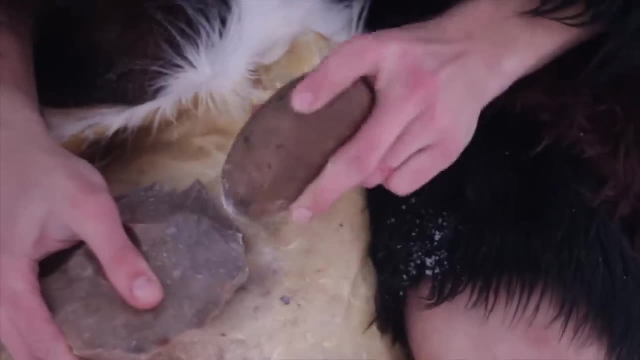 A sharp flake could originally be used as a knife and then later be resharpened into a hide scraper or other tool With the Lavalois method. other types of flakes could also be created by isolating two converging ridges. 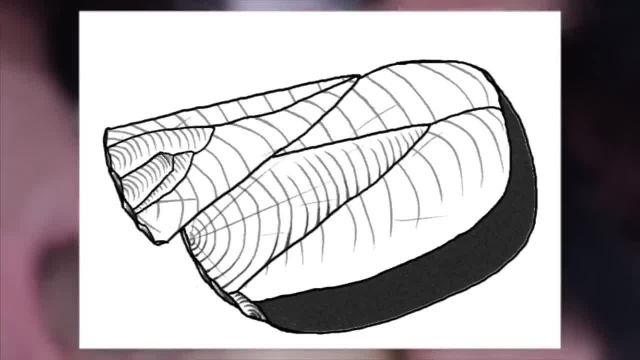 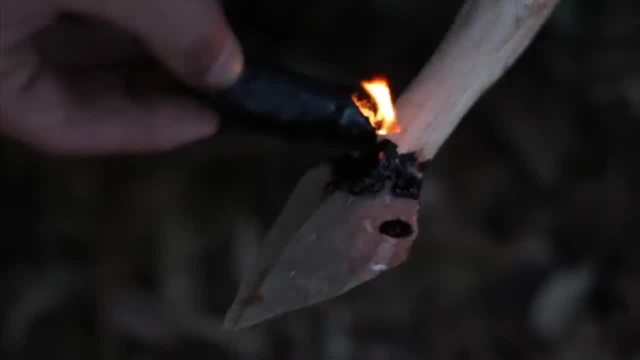 and striking beneath them, a Lavalois point could be made. These points are unsymmetrical but come with very sharp converging edges. Once hafted, these points could be very deadly weapons. We do know that Neanderthals were hafting tools also. 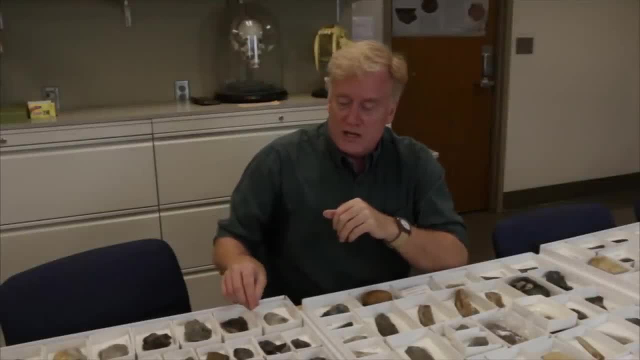 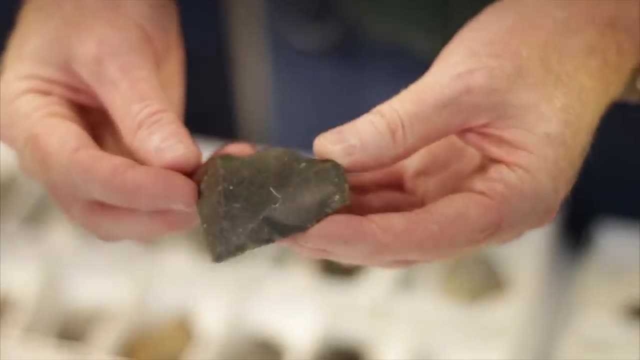 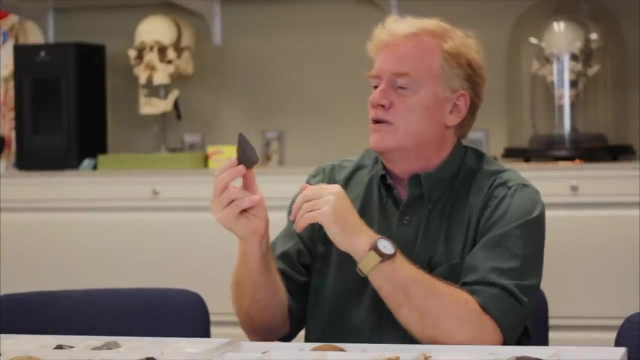 particularly points that were made with usually Lavalois technology that would allow the form to take a different shape. We also have convergent edges that come into a point. This is actually not such a classic Lavalois point, but it's pretty close. 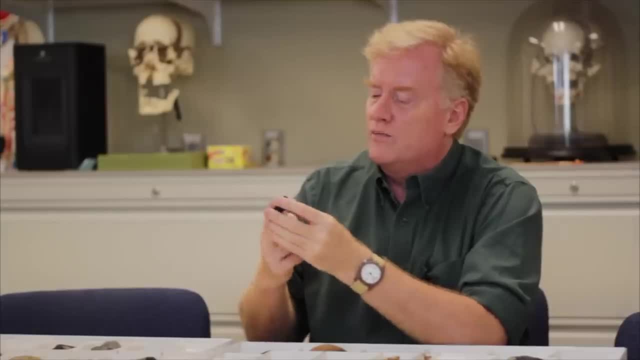 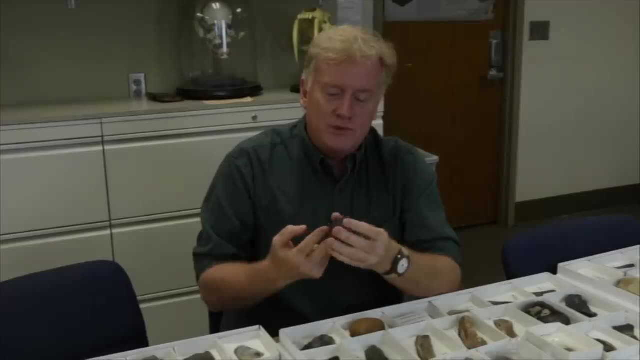 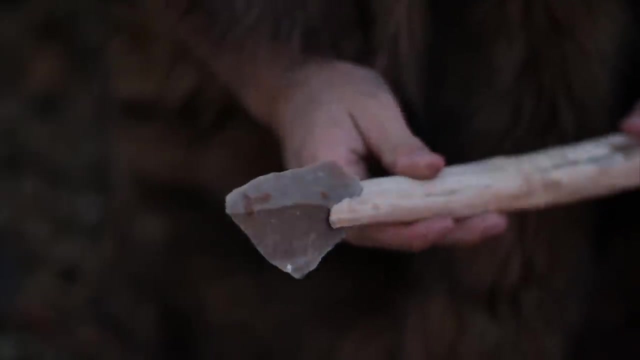 with the two convergent edges. In terms of how it would be hafted, it would be stuck into a haft like this, And we have examples of very crude hafts from around 400,000 years ago where they're just shoving into a crack in the wood. 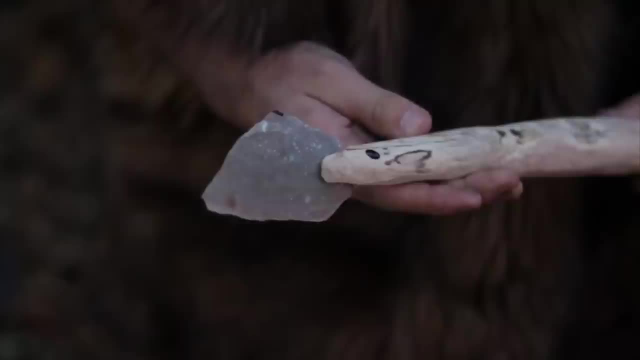 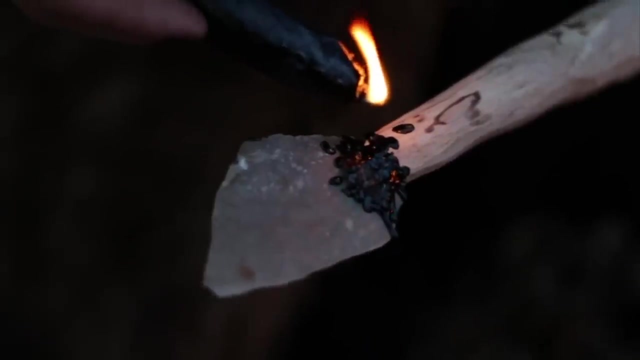 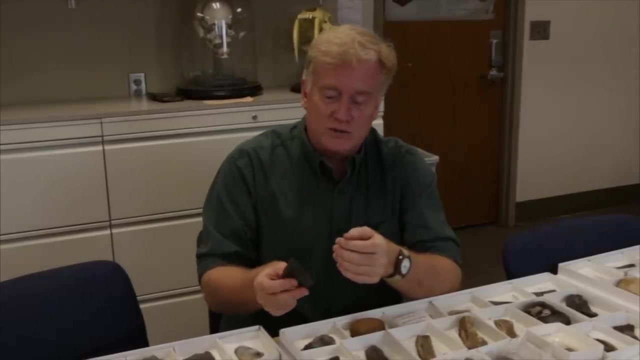 Otherwise, we have evidence that from abrasion on the edges and surfaces of the stone and also forms of glue, natural asphalt that was used to glue stones into a haft, that they were hafting things in the Neanderthal time period. 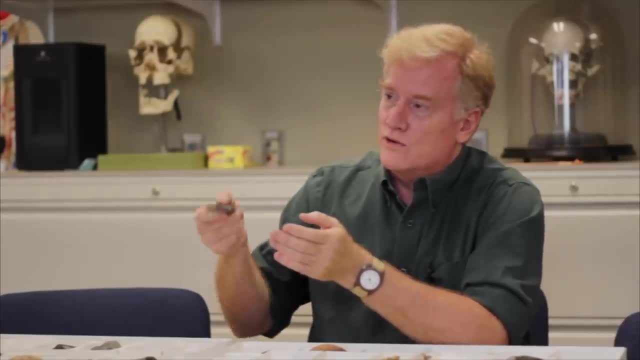 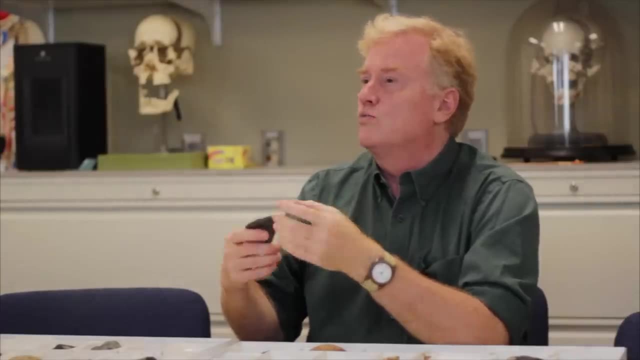 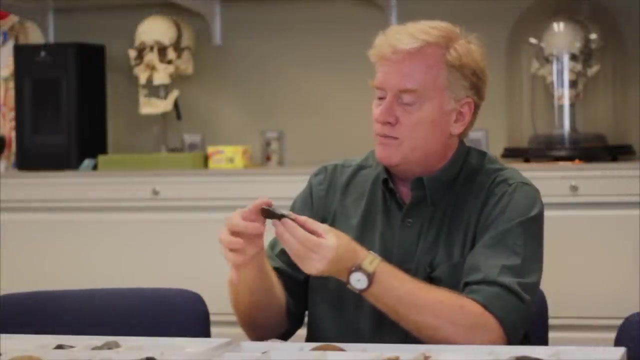 Whether they were doing it for using as knives or for large stabbing spears, those are more likely than, let's say, than a true projectile technology. Throwing them would have been also easy. but the actual tip area, cross-sectional area of a projectile tip like this, 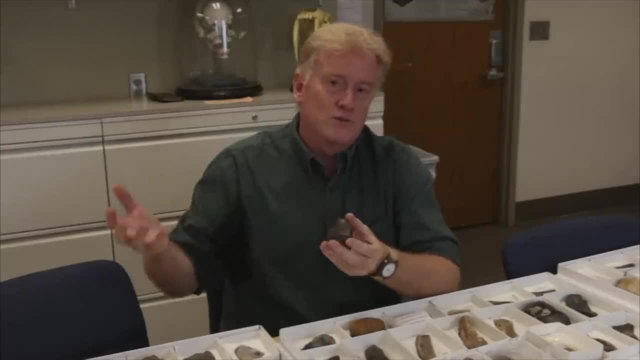 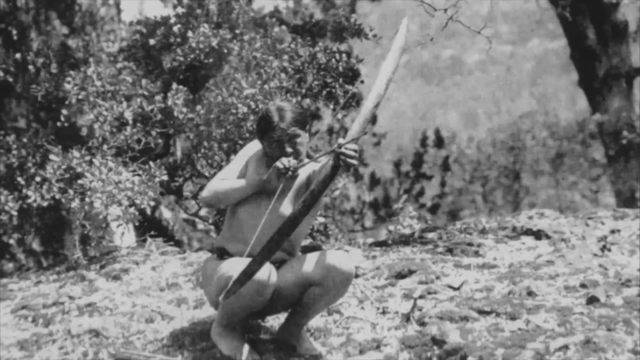 tends to be a bit larger than what we would see in a modern human society. they're using for either a projectile technology like a spear thrower or an atlatl, or even a later technology like a bow and arrow, So these look more like stabbing spears. 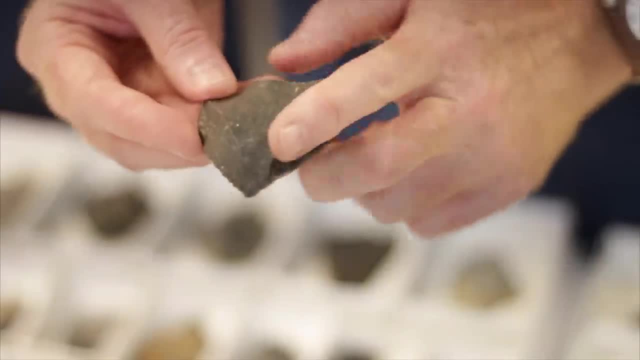 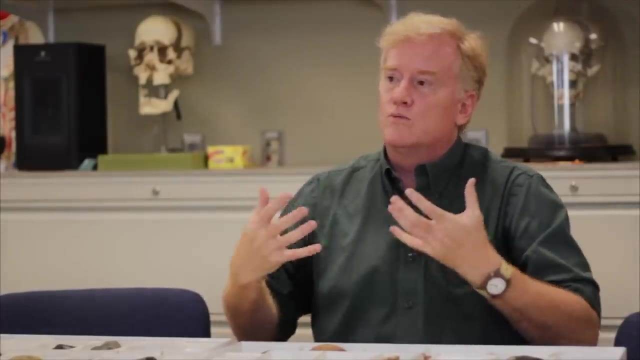 than they do something that would fly through the air and really take out an animal at a distance, And that's part of the argument that why Neanderthals were so much more muscular in terms of their skeletal structure, in terms of just having thicker cortical bone, than moderns. 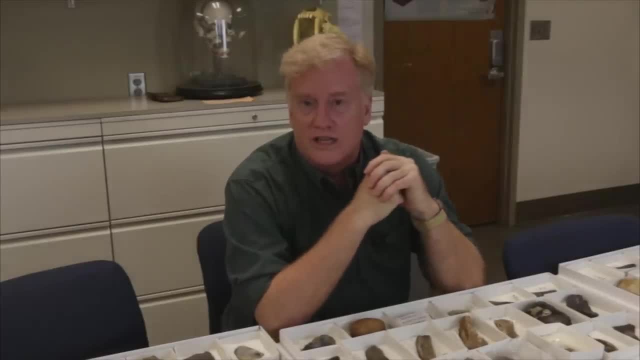 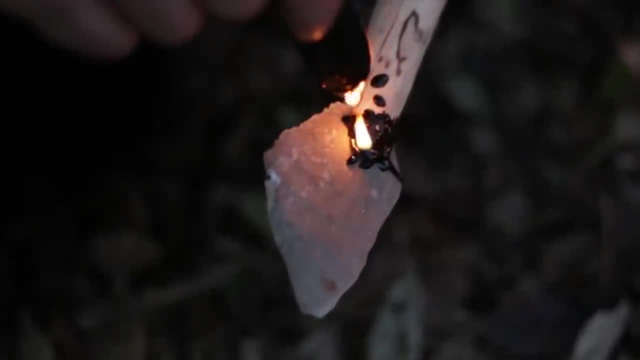 is that they were just engaging in much harder life, which could have been including, you know, confrontations with violent animals that they were trying to kill. The Valhalla points were almost certainly hafted. However, they may have been hafted in a very rudimentary way. 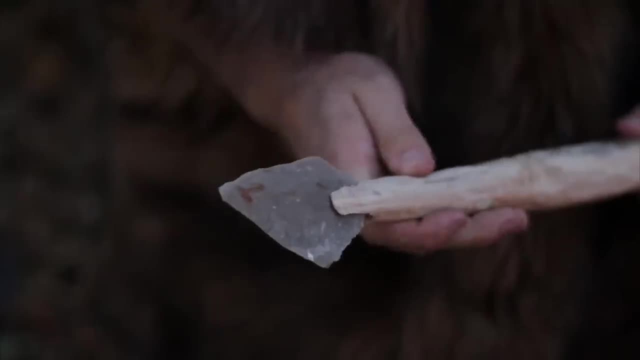 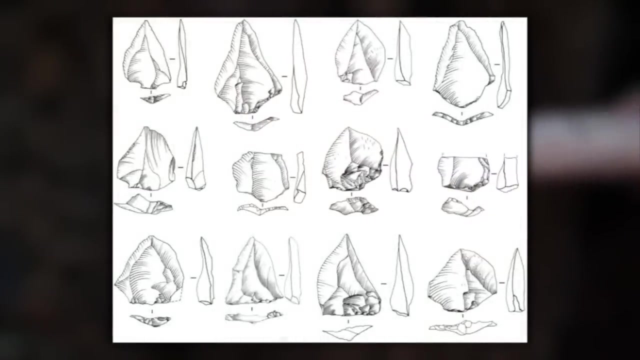 We will talk more on this later. In a study on 117 the Valhalla points, eight points displayed use-wear damage. Two of them were used for woodworking activities. six of them are associated with butchery, while one point was distinct from the others. 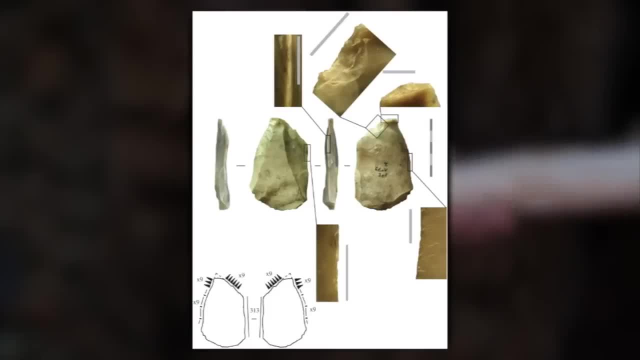 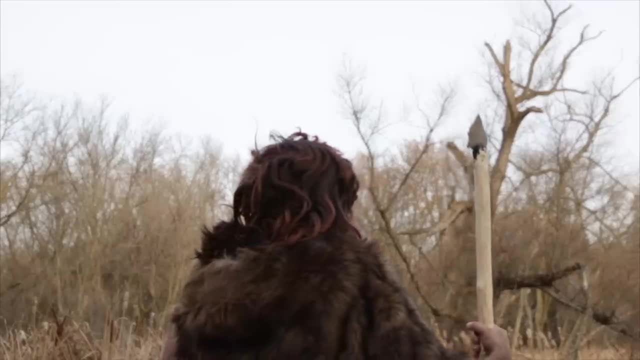 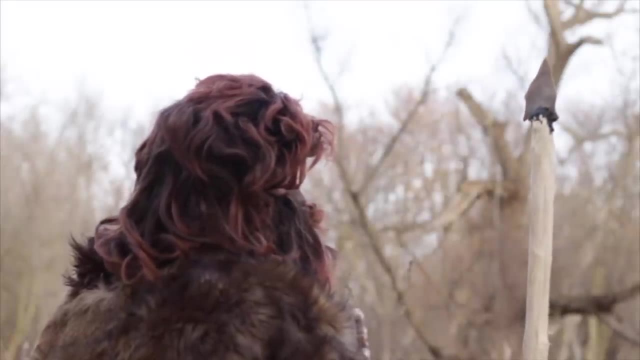 An examination of the points showed a chipped and denticulated left edge. This damage denotes violent penetration into an animal carcass and is consistent with contemporary tests of hafted spear points, Though this study does not show that the points were used as spear points. 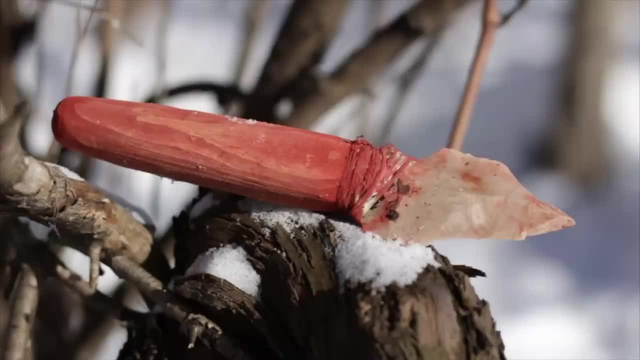 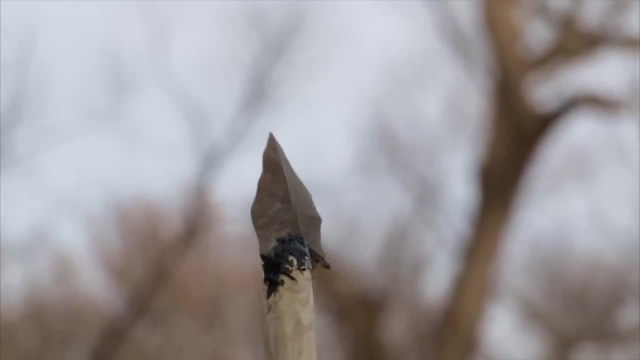 it also suggests that most weren't, Many of them would have been used for woodworking or for butchery. Nonetheless, this does not diminish the significance of these tools. on the tips of spears, Fossil remains with impact damage consistent with the Valhalla points. 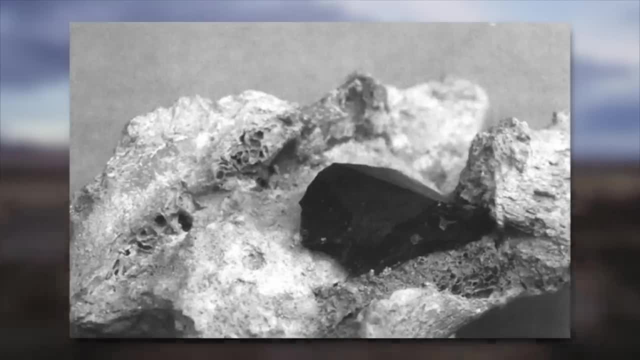 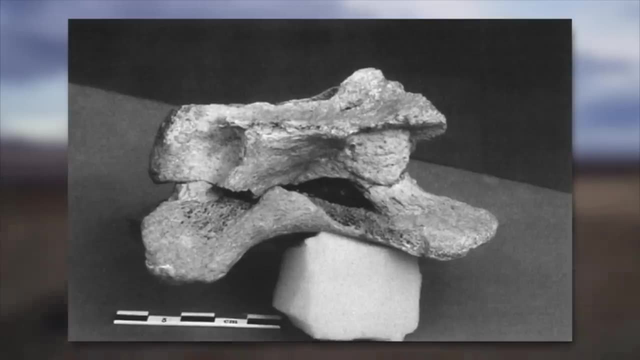 as well as fossils with literal Valhalla points embedded in them, confirms the use of this technology in hunting activities. A find like this is extraordinary for the time period. We will talk further about the use of these spears when we discuss how Neanderthals would have hunted. 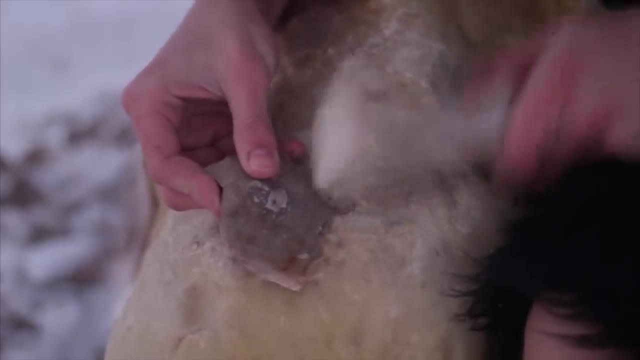 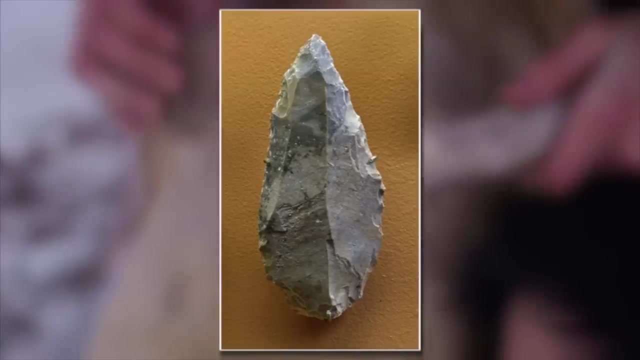 The Valhalla points were commonly made by Neanderthals, but other types of points were also used. Triangular flakes resulting from less standardized platforms were often utilized. These flakes could be turned into convergent scrapers, As their name suggests. 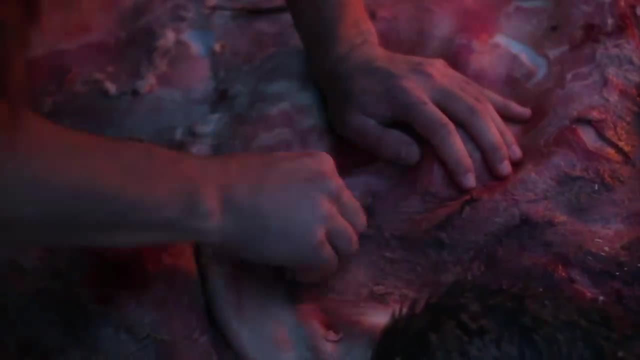 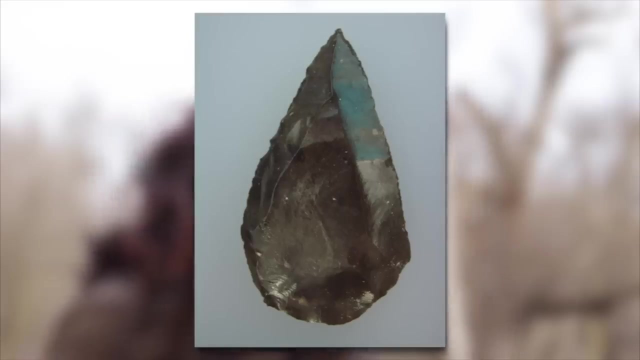 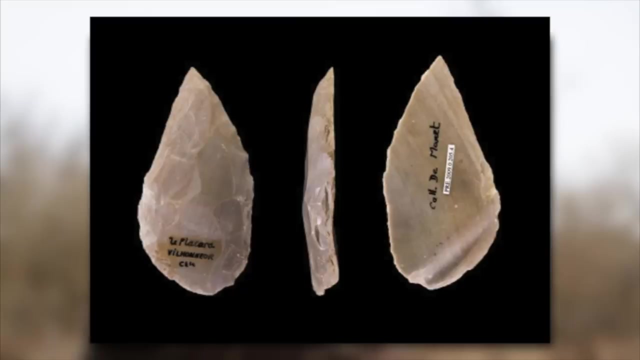 they were primarily used as scrapers, though they may have also functioned as spear points. Mousterian points were another point. created from triangular flakes or Lavalva flakes, They were modified by taking off additional flakes. This created a more symmetrical point that was often easier to haft. 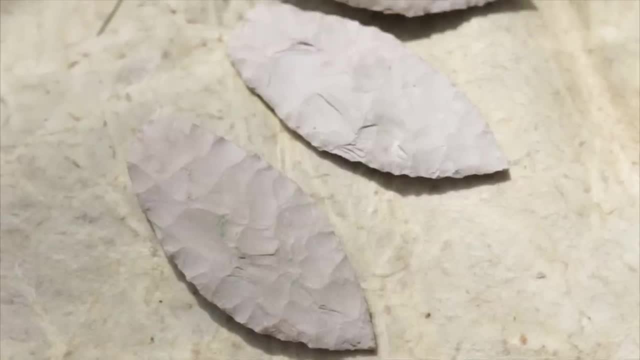 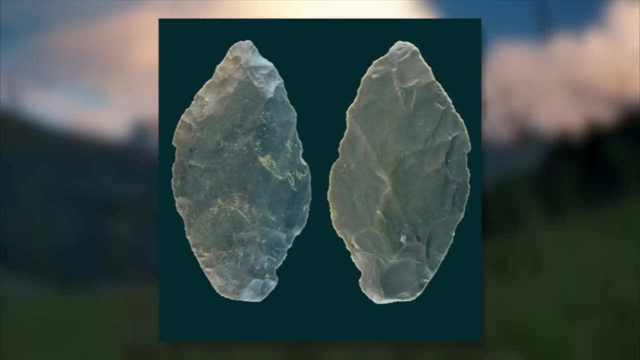 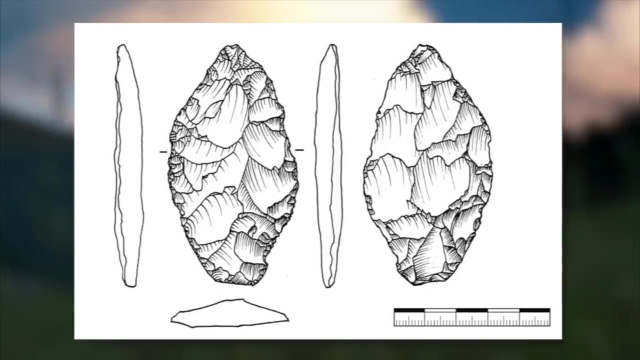 Later, Neanderthal points, dating to the twilight of their existence, were even bifacial and highly refined. Bifacial points from Hohfels, Germany, were made with considerable skill. This point in particular was certainly used for hunting. It was commonly hafted and used as a spear point. 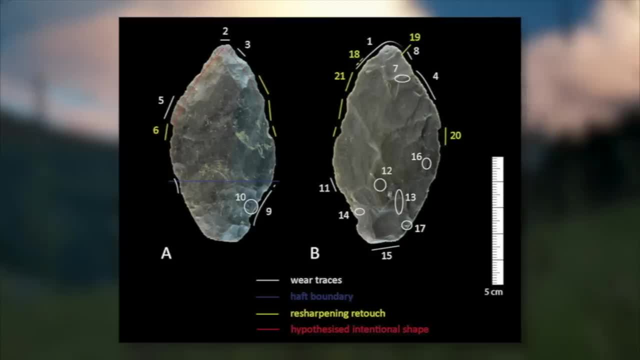 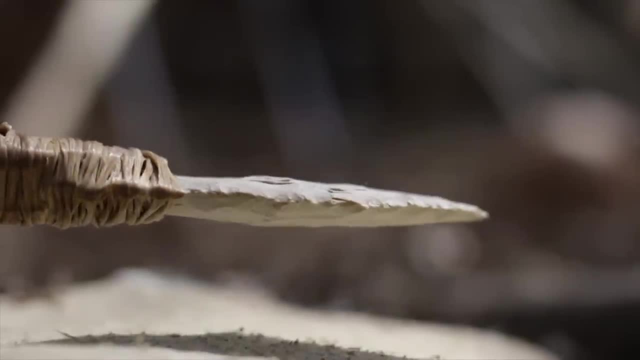 It was re-sharpened multiple times until it was no longer useful and likely discarded. Though it may look rough now, during its original creation it would have looked similar to this. Another point from a cave in Switzerland preserves a more pristine bifacial point. 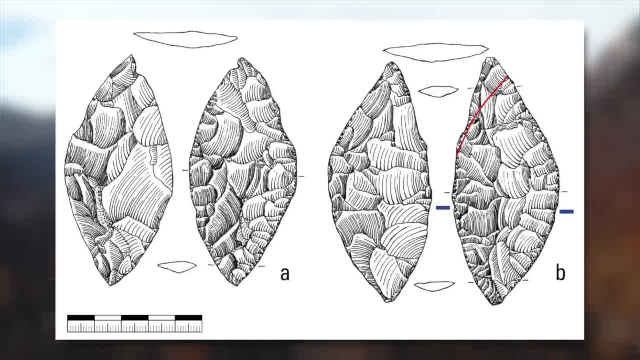 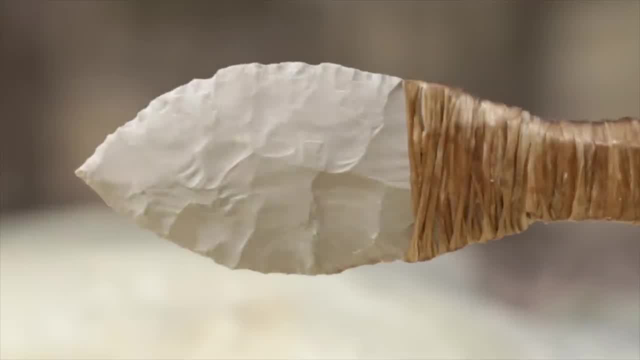 These points indicate that Neanderthal stone point technology did reach a considerable complexity towards the end of their time. Most, if not all, Neanderthal points were created with the intention of being placed on thrusting spears. The points were just too large to be part of a projectile. 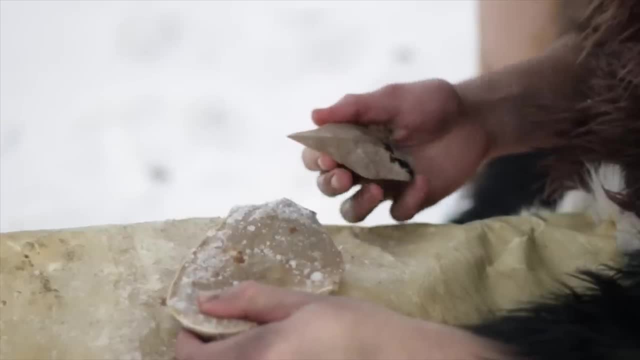 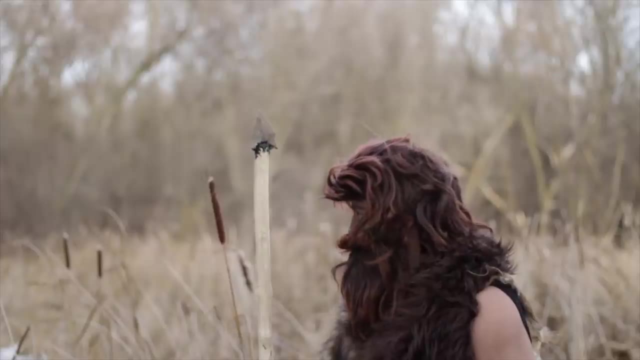 such as an arrow, atletal dart or javelin. Their thrusting spears would have likely been very robust and primarily for stabbing. This does not mean that they couldn't have been thrown, though Some evidence of wounds caused by Lavalva points. 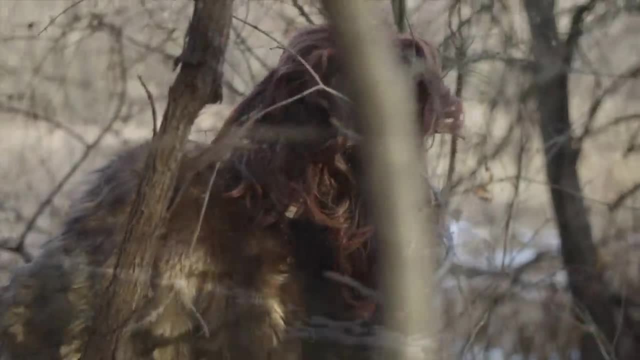 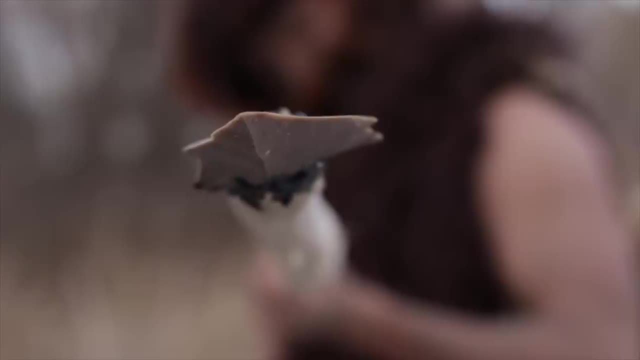 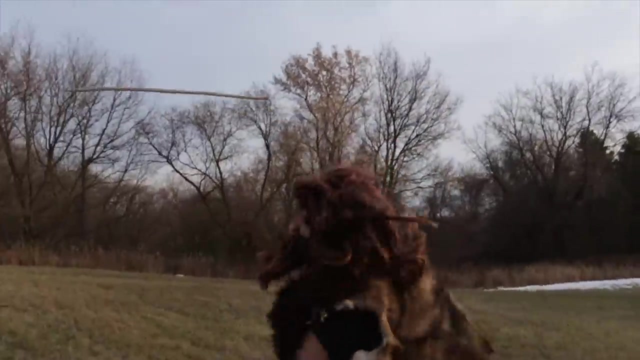 suggests that they were used as projectiles. These spears would have likely been thrown at times, but only short distances with the mass of a robust Lavalva point and a heavy shaft, these spears would have packed a considerable punch when thrown in close quarters. 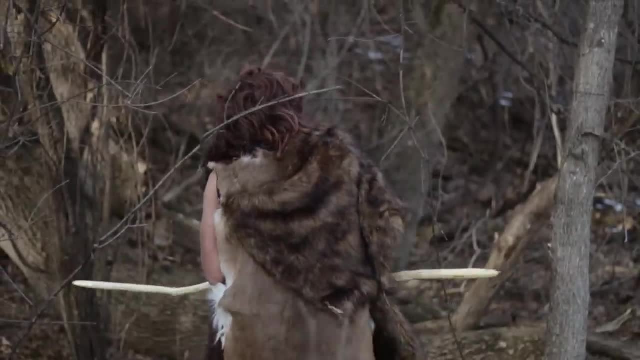 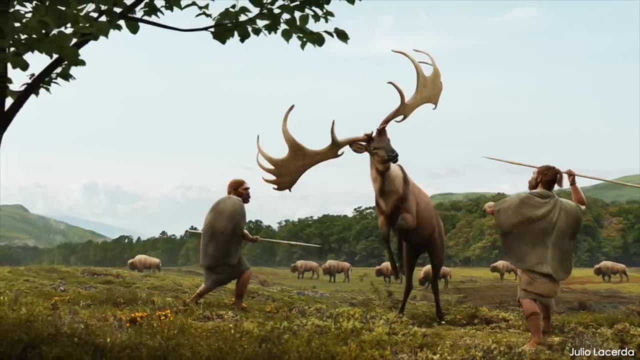 Though a Neanderthal may have preferred to hold onto their weapon and deliver most of their blows by hand, This is supported by the high rate of Neanderthal injuries, suggesting that they got very close to their prey. As mentioned previously, Lavalva points and other Neanderthal points. 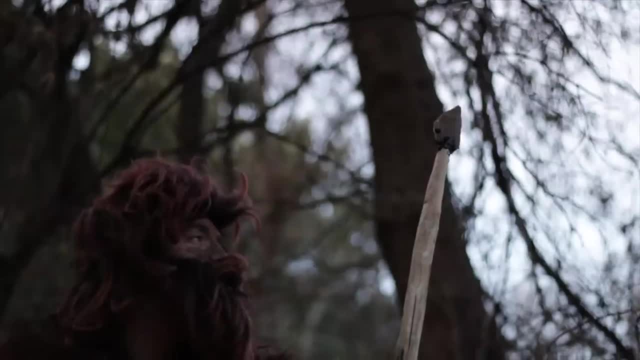 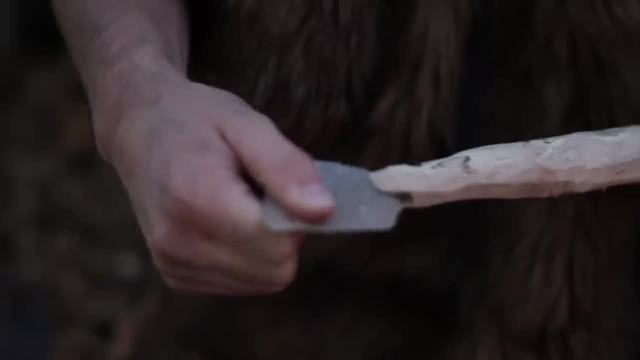 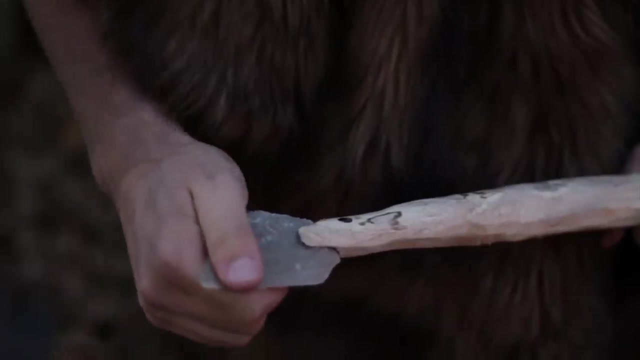 would have been hafted to spears. Another question we must answer is how were these points actually hafted? Points from earlier periods were left with unground edges. This is important because the sharp edges of a Lavalva point would cut through any cordage wrapped around them. 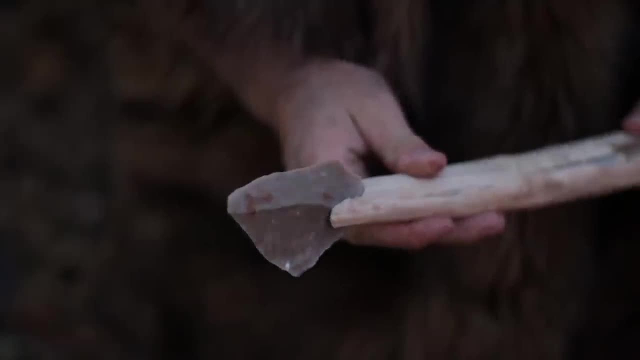 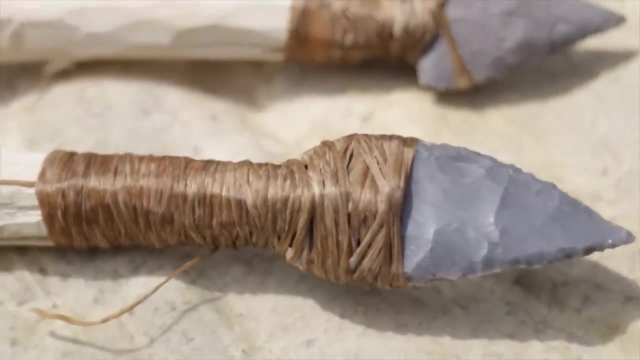 This suggests that early Lavalva points were simply placed into a wooden slot with, perhaps, the aid of an adhesive. Later Lavalva points, as well as Malsterian and bifacial points, had ground edges which would have been wrapped with some kind of wrapping or cordage. 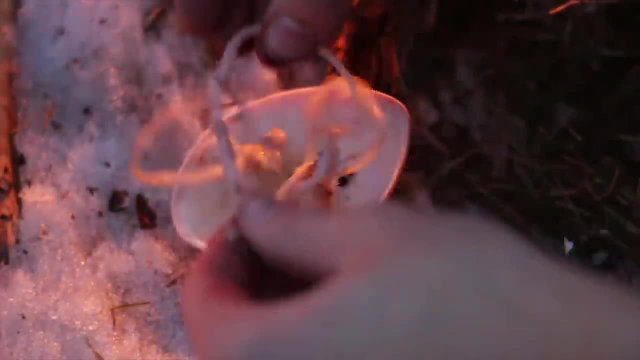 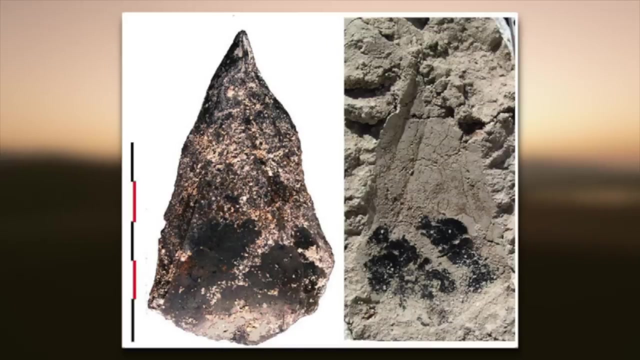 Strips of leather plant fiber, cordage, sinew and gut would have all been great materials to hold points in place. Chemical analysis from a Malsterian point and two Lavalva points from a site in Syria have shown that a natural glue was present on the base. 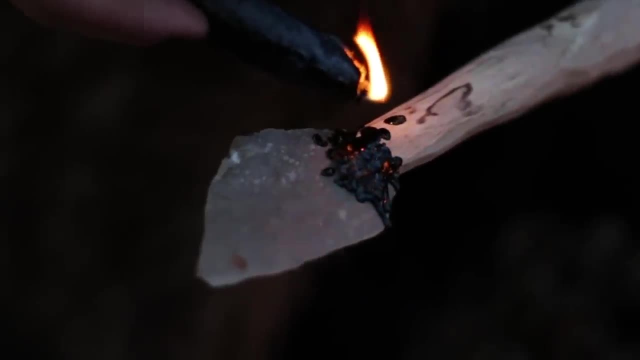 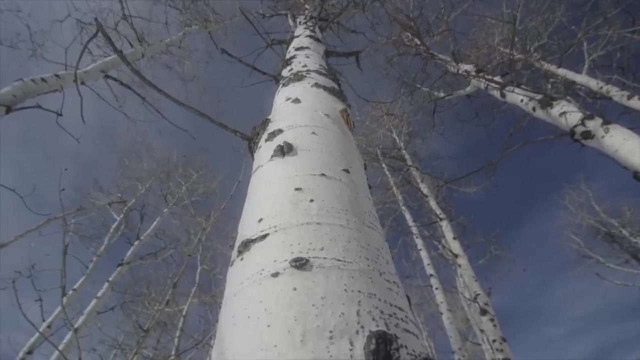 Adhesives such as pine tar, birch tar and bitumen have all been found at Neanderthal sites. The oldest evidence of adhesive use attributed to Neanderthals comes from two pieces of birch tar that date to around 200,000 years ago. 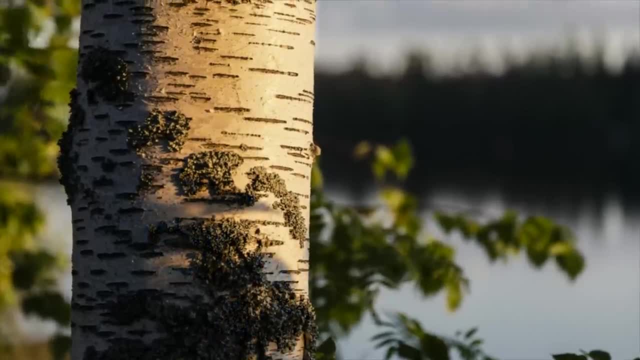 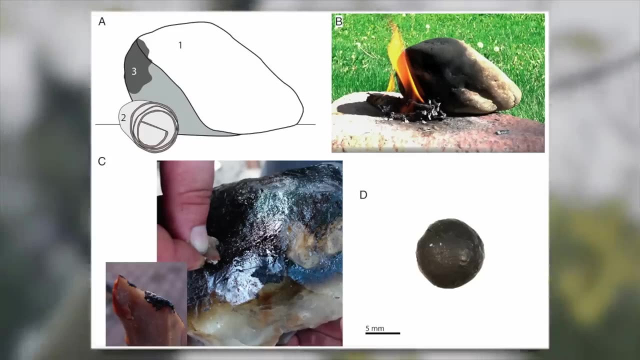 It was once thought that Neanderthals needed a complex container or methods to create birch tar, but a recent study has proven that birch tar could have been made simply by scraping burnt bark off of cobbles. The resulting material is a great adhesive. 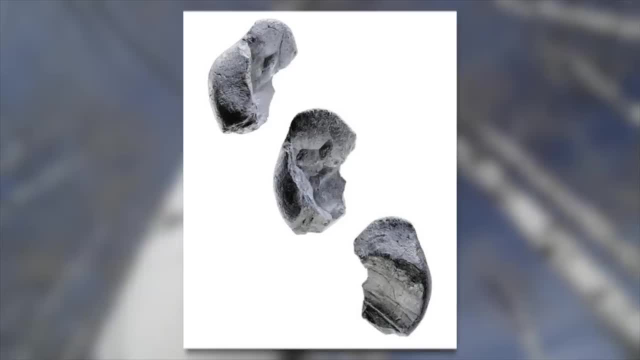 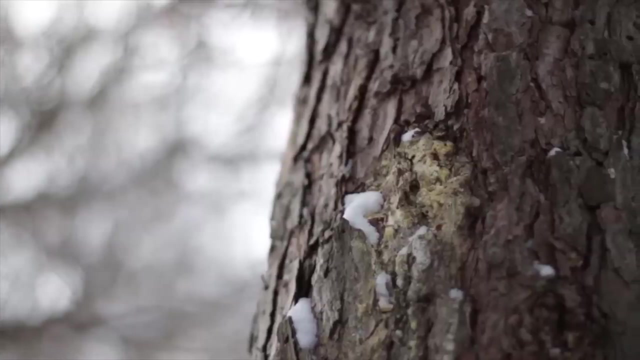 and is quite shock-absorbent. An amazing piece of birch tar from Königsau Germany preserves imprints of wood, stone and even a Neanderthal fingerprint. Evidence of halfting couldn't get much better than this. Another quite easily obtained adhesive would be conifer resin. 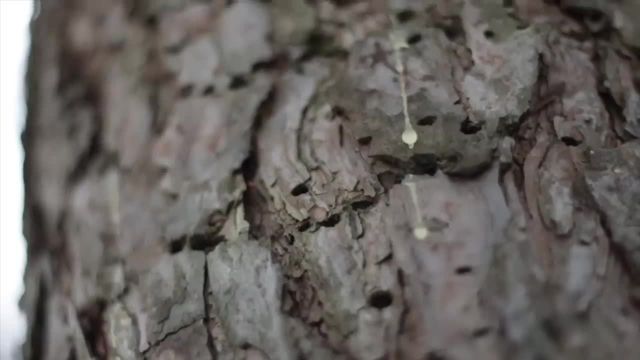 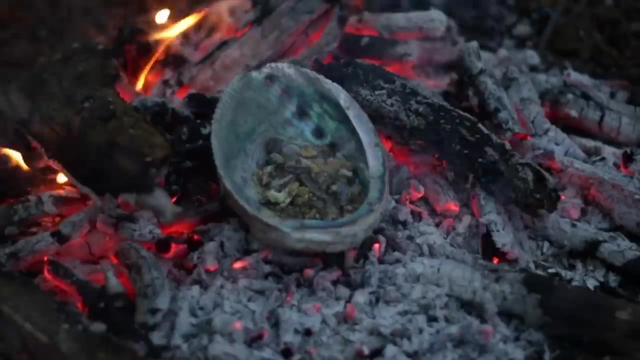 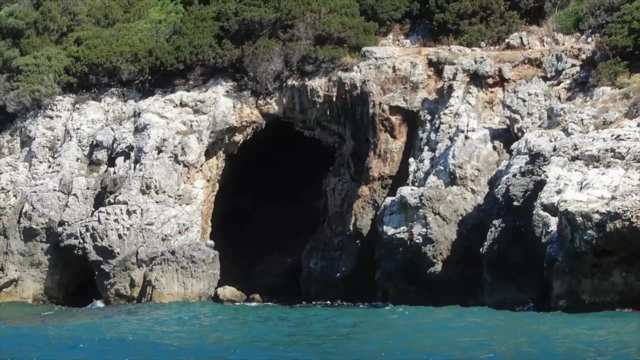 also known as pine sap. It can be used straight from the tree, though it is not very shock-resistant, As primitive technology enthusiasts may know. adding beeswax makes it an exceptional glue, and Neanderthals knew it too. Residue from 10 stone tools from Grotta del Fossilone. 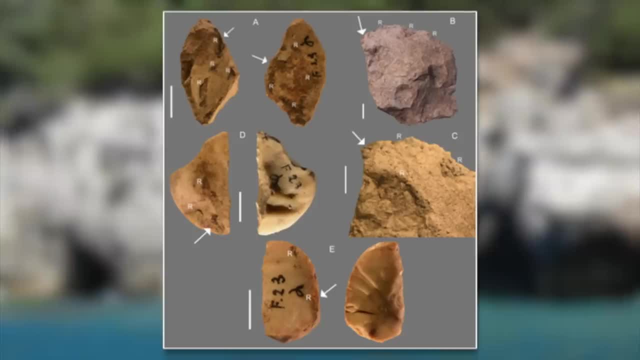 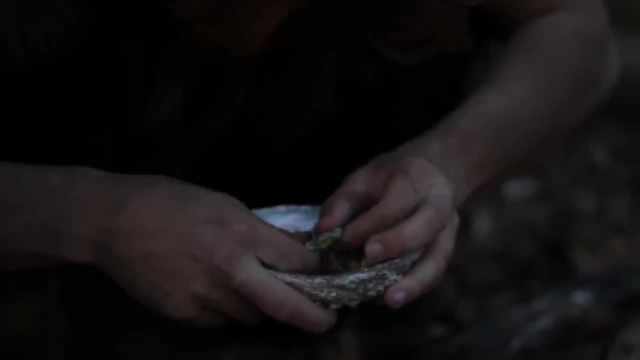 and Grotta del Santa Agostino contained the chemical signatures of conifer resin, and one contained chemicals from beeswax. Other sites containing pine resin and beeswax have strengthened the idea that Neanderthals purposefully mixed these components to create a strong adhesive. 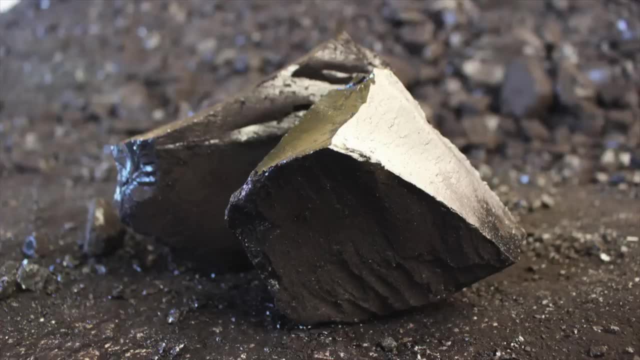 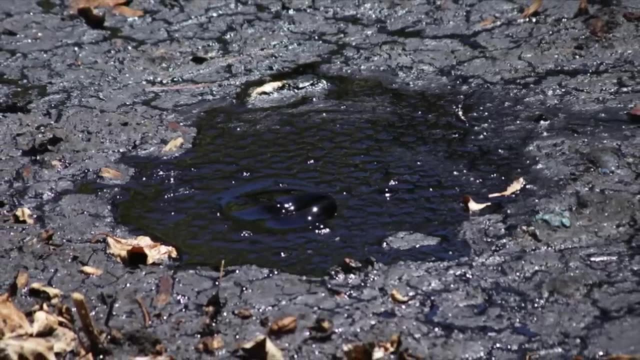 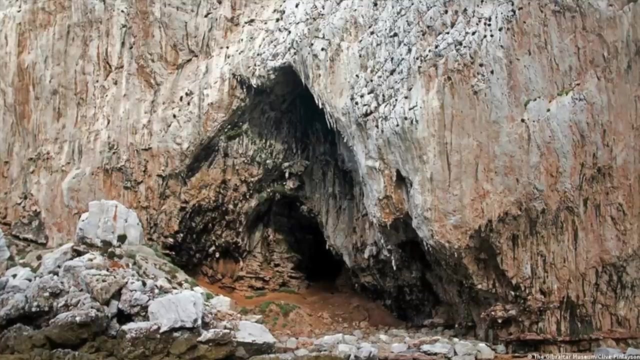 The last adhesive used. bitumen is a sticky, highly viscous form of petroleum that may have been harvested from Neanderthals in natural deposits across Europe. In its natural state it is sticky and ready to use. Neanderthals from Elsadrone Cave in Spain. 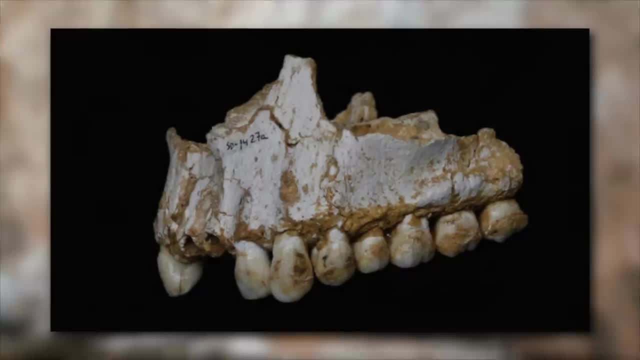 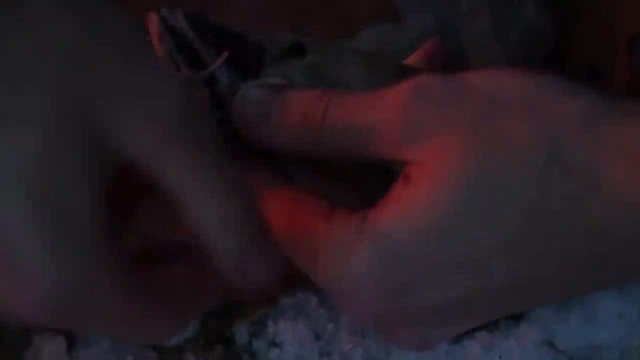 were found to have bitumen in their dental calculus. It has been hypothesized that this may have occurred by using the mouth to aid in the halting of tools, Perhaps by clamping their teeth down on the haft, holding the lithic in one hand. 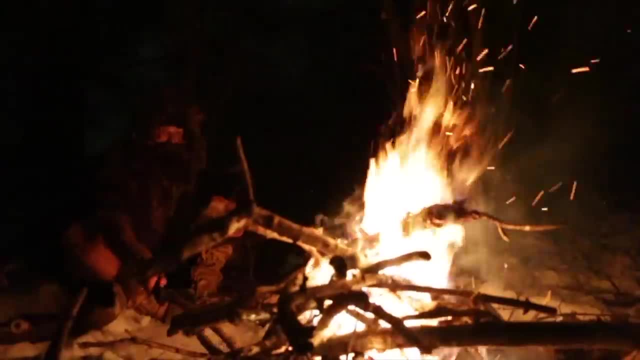 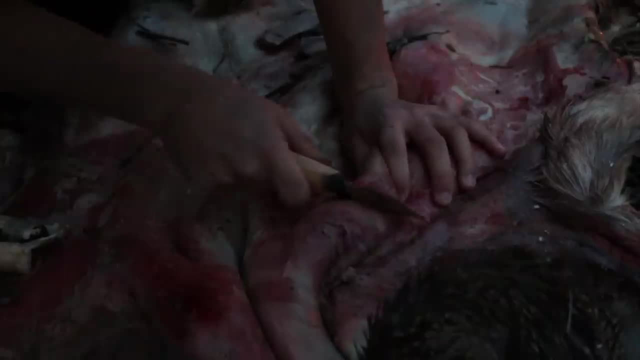 and applying the adhesive with the other. Another form of adhesive that may have been used but we don't have evidence for is hide glue. Hide glue can simply be made by cooking bits of hide or sinew next to a fire with indirect heat. 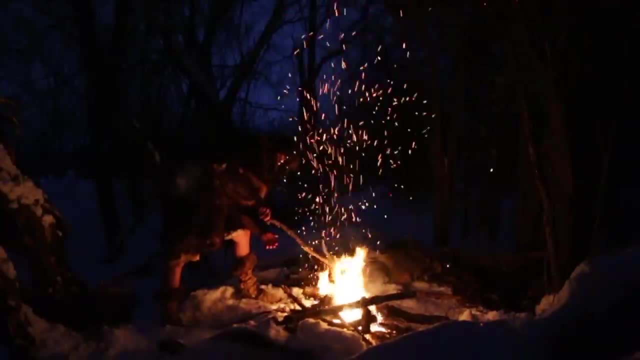 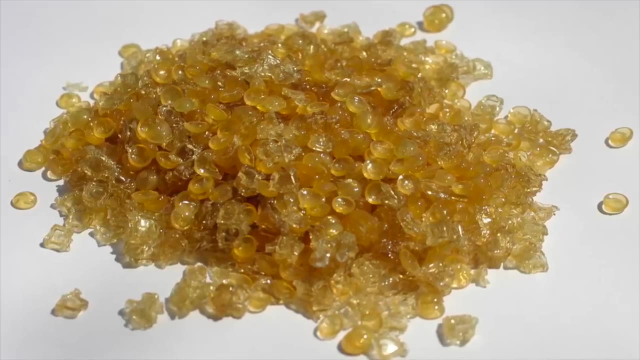 Neanderthals would have likely noticed the adhesive properties of bits of hide or sinew on the meat that they were cooking. The glue produced by this method is quite strong, but, more importantly, it binds sinew, gut and leather together. 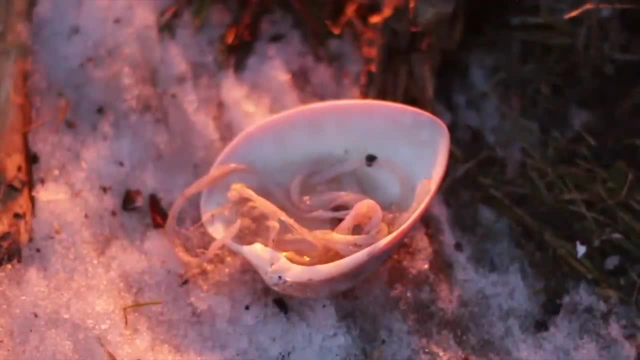 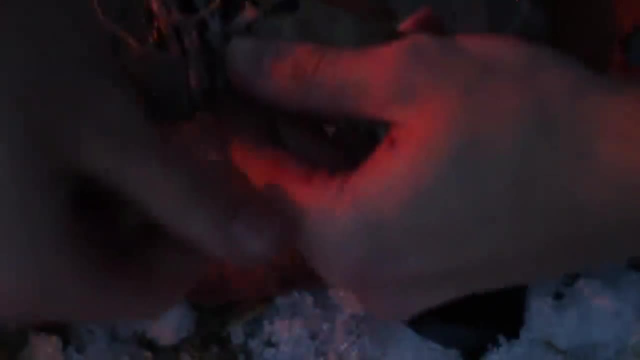 Hide glue is essentially protein that can be used to adhere bindings together. Neanderthals may have used it on their bindings to keep their spear points in place, though we do not have evidence of its use. Still, it is important to consider technology. 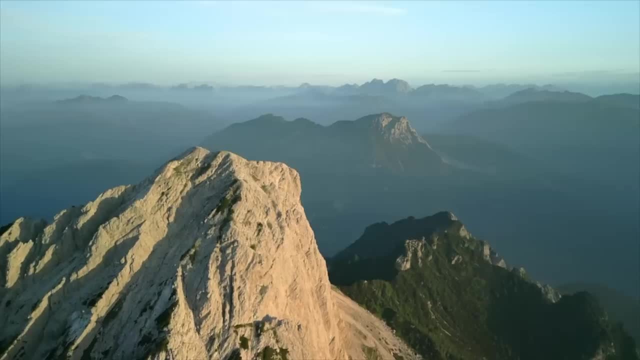 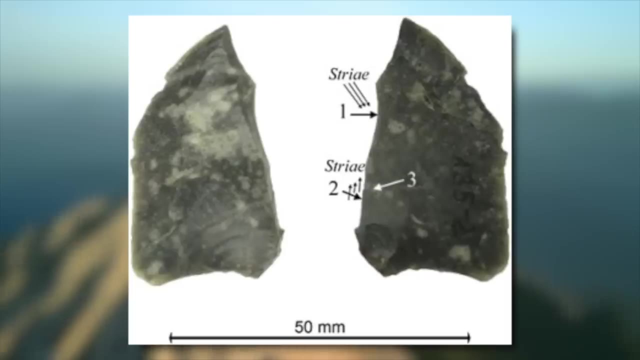 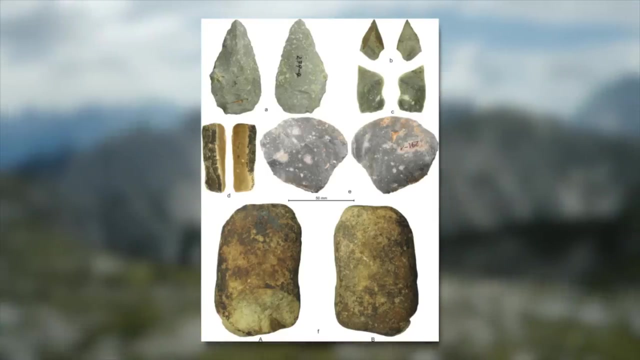 that we do not have direct evidence for. Another important form of evidence for halting comes from polishes. Halting a tool with adhesive creates clear signs on the stone. Many artifacts, including points, retouched tools and even random flakes, were hafted. 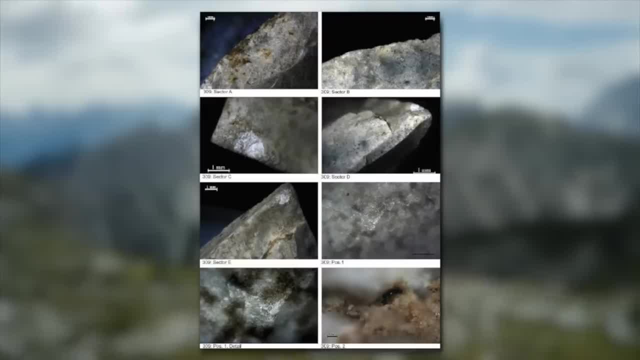 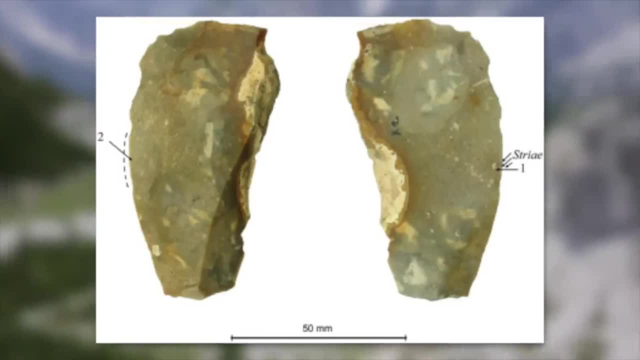 In some sites nearly half of the artifacts had halting micro-polishes. Many other sites show that halting stone tools was quite common in the Neanderthal world. When looking at Neanderthal tool remains, they may appear quite crude and simplistic. 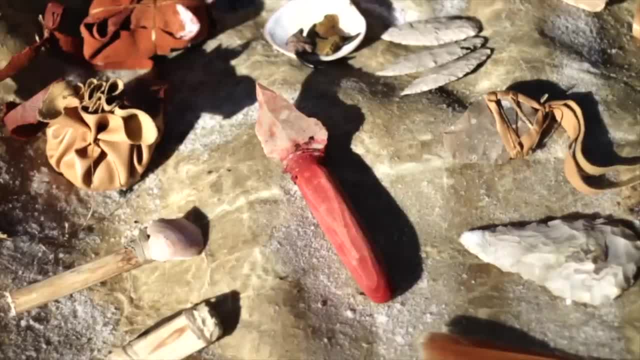 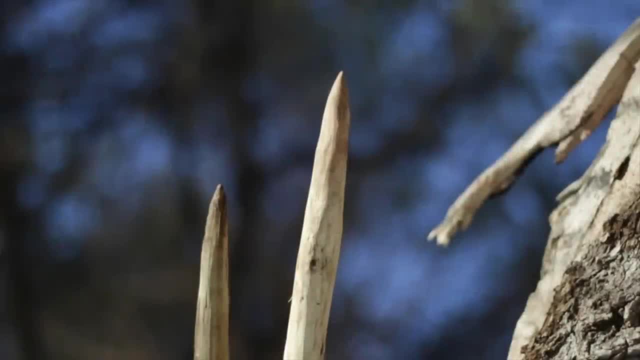 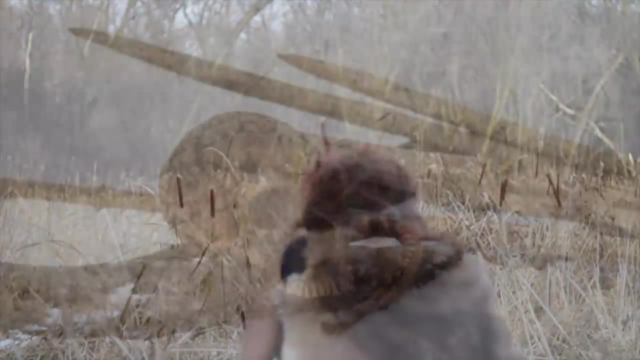 but imagining them hafted on various handles and grips sheds light on the complexity of their tools. Another underrepresented aspect of Neanderthal technology were their wooden weapons and tools: Actual projectiles as well as many weapons such as thrusting spears and throwing sticks. 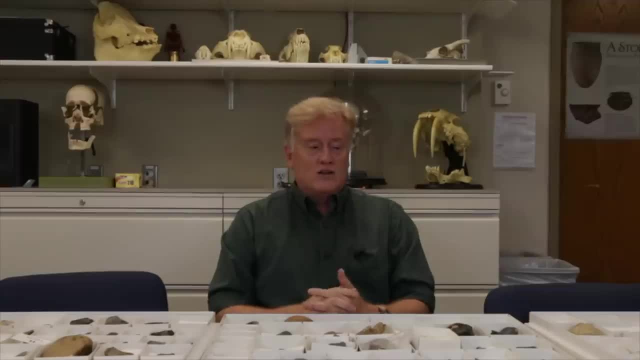 were made of wood. In terms of the technology involved, Neanderthal technology tends to be focused more on using stone to carve wooden objects as implements for hunting, But the modern humans in the Upper Paleolithic tended to haft their stone tools more frequently. 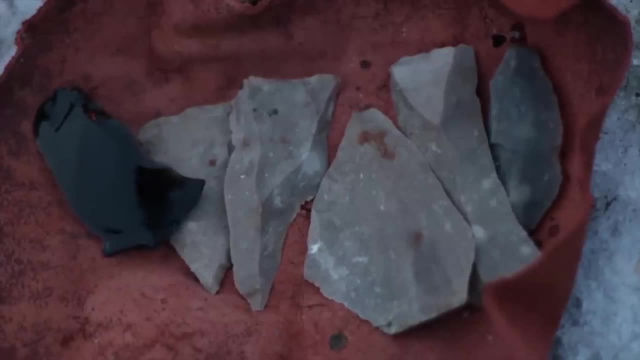 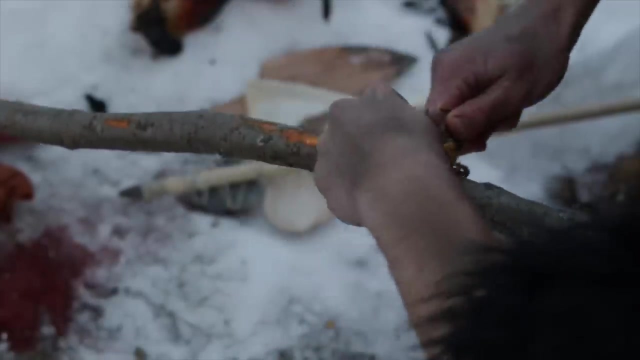 Wood was worked with a number of stone tools. Lavalwa points and blades were efficient tools for shaving wood. Backed knives would have also worked well. Notch tools were effective at shaving wood, while denticulate tools could be used to saw wood. 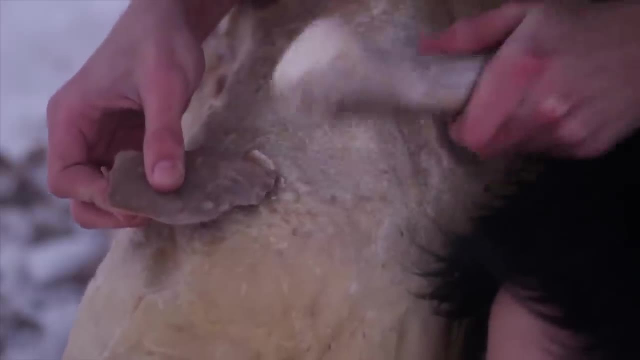 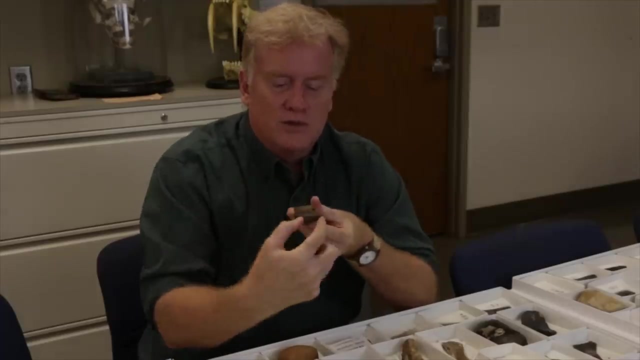 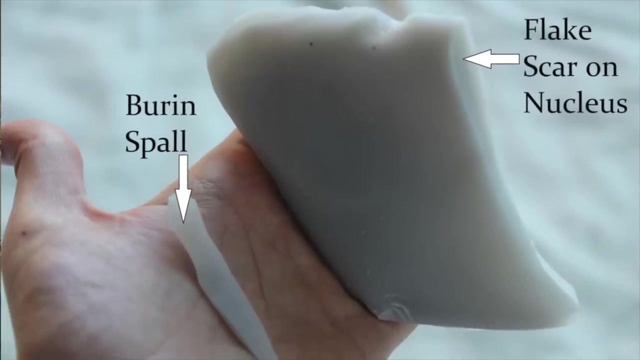 Blades could also be turned into tools called bierens. This is a fairly thick blade that was retouched here, so it was probably longer, and the end was taken off to make a little platform, to then make a bierenspaal come off here. 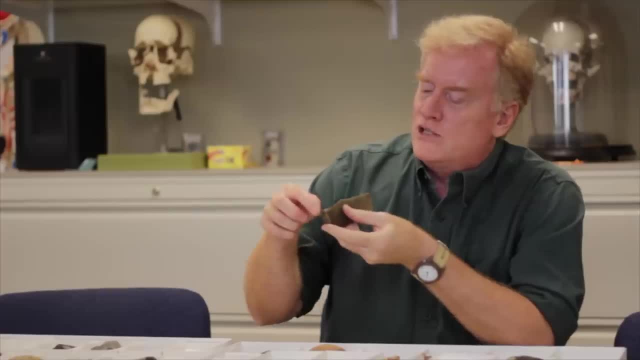 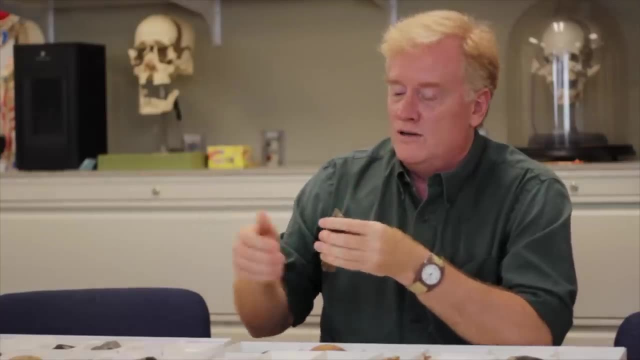 The bierens themselves were actually good little barbs, but the actual scar left on the blade, this becomes the bieren and the part that comes off is called the bierenspaal. This is actually excellent for graving bone and wood. 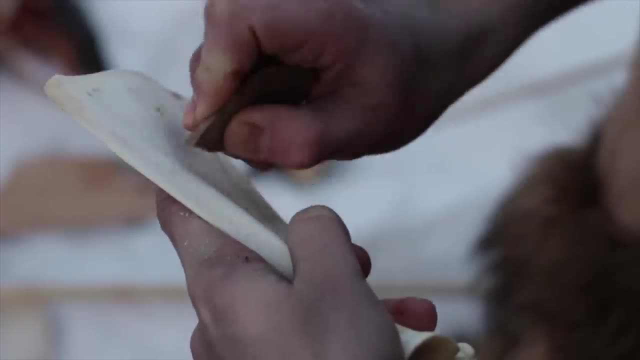 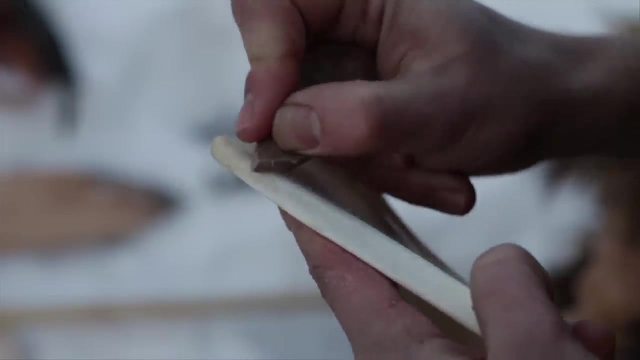 So you can literally shave bone with this edge, because it's both sharp but also fairly robust. And stone is very sharp but it's also very brittle, And so if you're trying to work something that's very hard, you need a steeper edge. 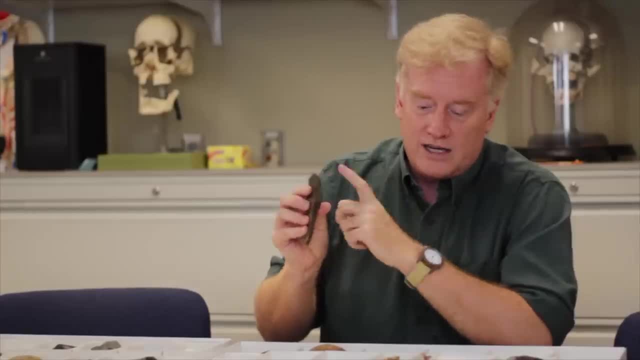 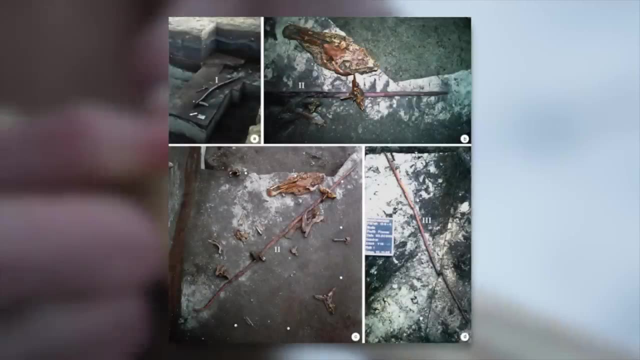 And so a bierenspaal edge is really very useful for that. With their array of woodworking tools, they were able to create very refined wooden technology. The amazing discovery of the Schoeniggen spears in 1994 recovered 10 wooden weapons dating to over 300,000 years ago. 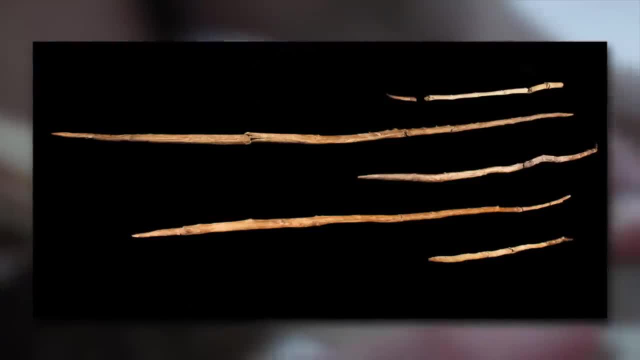 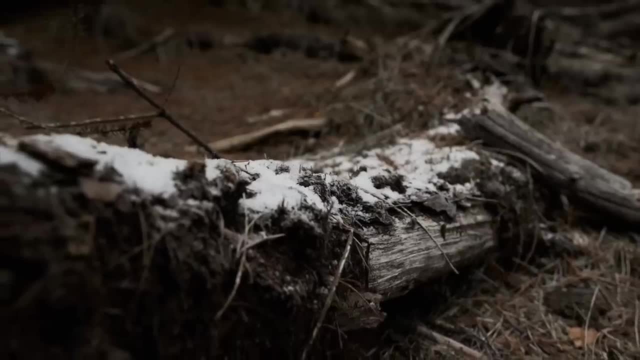 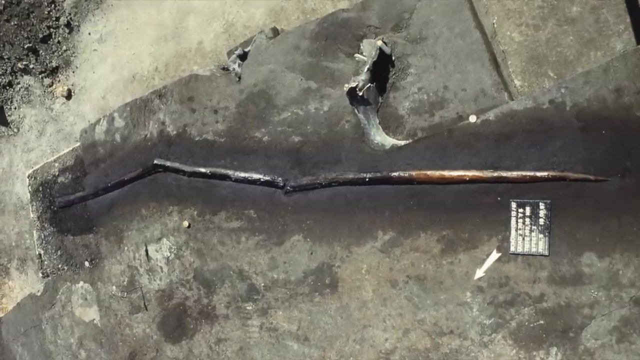 They are the oldest complete wooden tools ever discovered and were either made by early Neanderthals or late Heidelbergensis. Wood degrades in only a few years in most cases, but the rapid sedimentation and waterlogged conditions of the site provided the precise conditions for preservation. 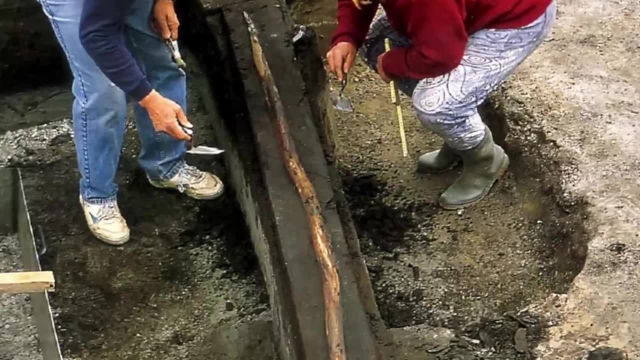 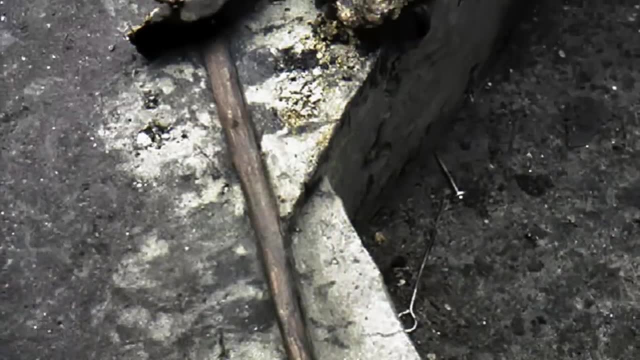 The site was once a lakeshore that eventually became buried with sediment with the retreat of the Elsterian Ice Sheet. The spears and other wooden tools were found in direct association with animal remains and stone and bone tools. The wooden tools take a variety of shapes. 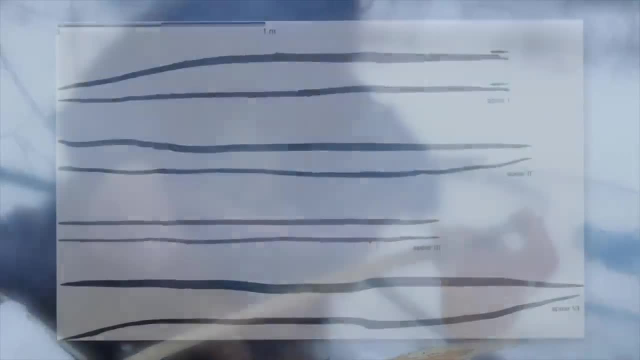 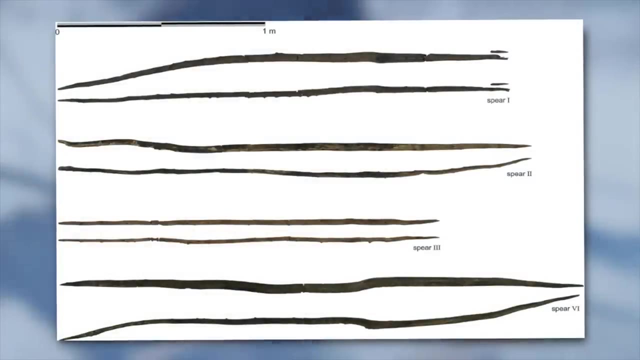 Seemingly designed for different purposes. The spears are between 1.84 to 2.53 meters, or 6 to 8.3 feet in length. The majority of the spears were made from slow growing spruce trees, while spear 4 was made of pine. 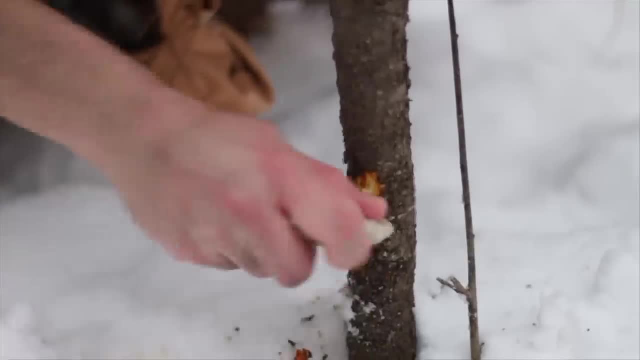 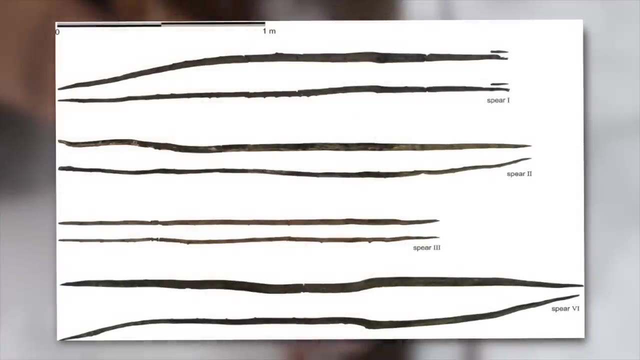 The points of the spears were carved from the bases of the trees, which are denser. All the spears were tapered on both ends, except for spear 6.. Spear 6 also has a natural kink. It has been interpreted as a thrusting spear. 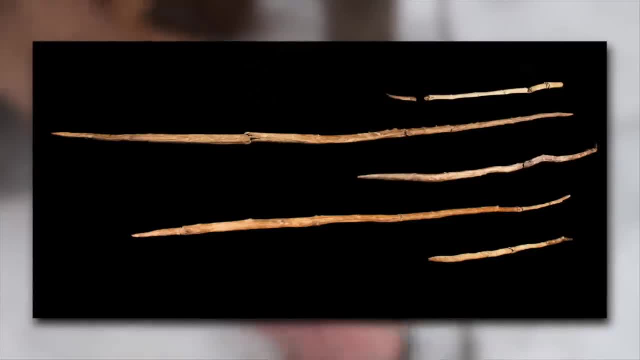 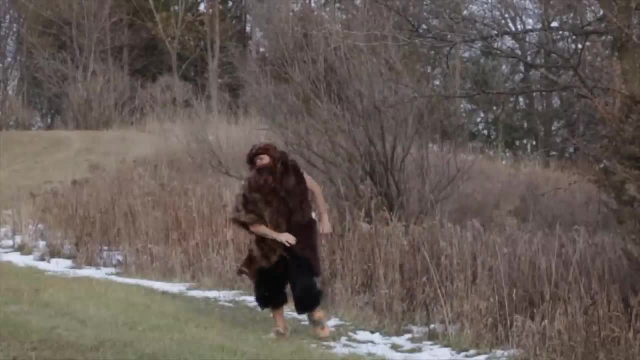 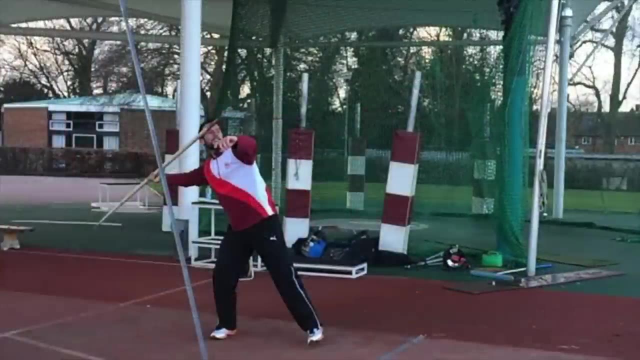 However, the other spears taper aerodynamically and are weighted with the center of gravity in the front third of the shaft. Their design and weighting suggests that they may have been used as javelins. Contemporary experiments using replicas demonstrated that Spear 2 could be thrown as far as 20 meters or 65 feet. 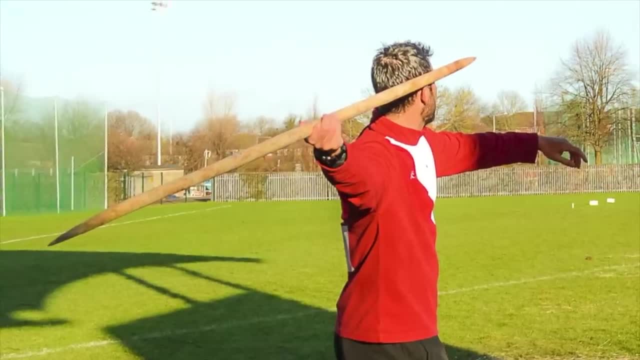 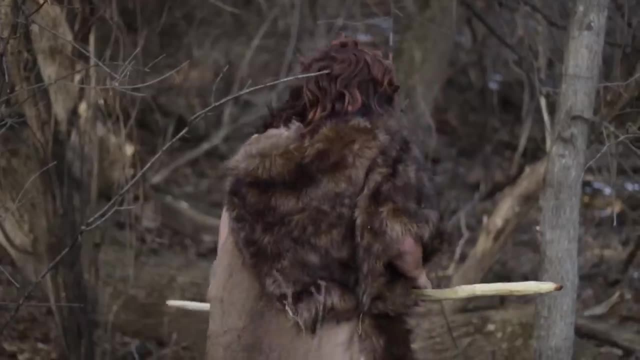 The spear, performed similarly to modern javelins. The ones suspected to be javelins also performed similarly to modern javelins. The ones suspected to be javelins also performed similarly to modern javelins. They were likely used in multiple ways. 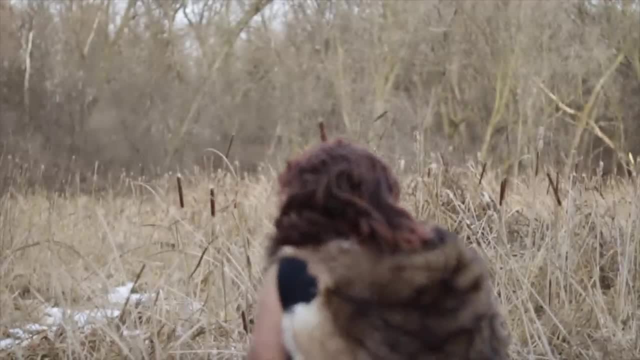 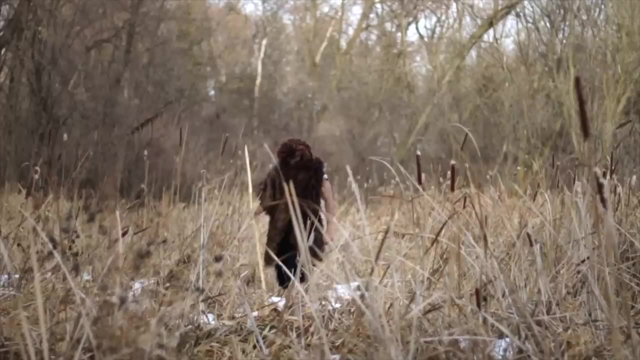 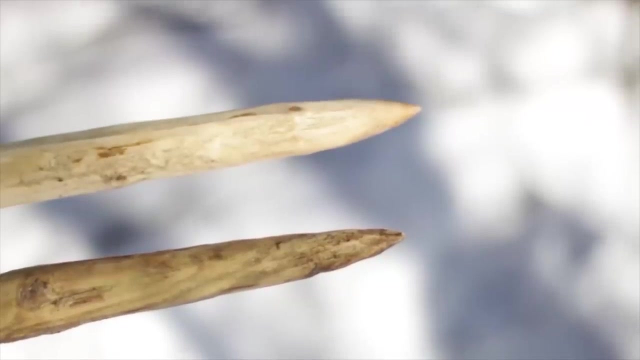 The evidence suggests that some of the spears would have been efficient for throwing, while others- especially Spear 6, was made for thrusting. All of them would have been useful for hunting or defending against predators. What is interesting about these spears is not one of them had a hafted point. 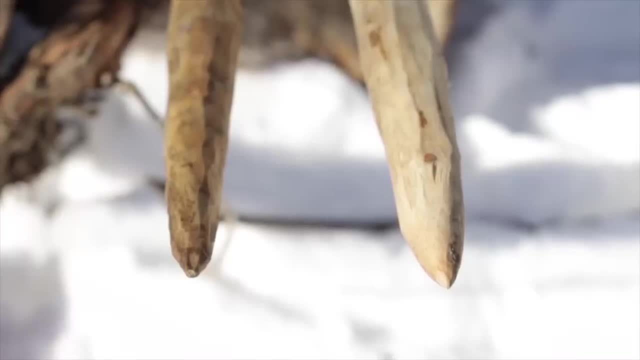 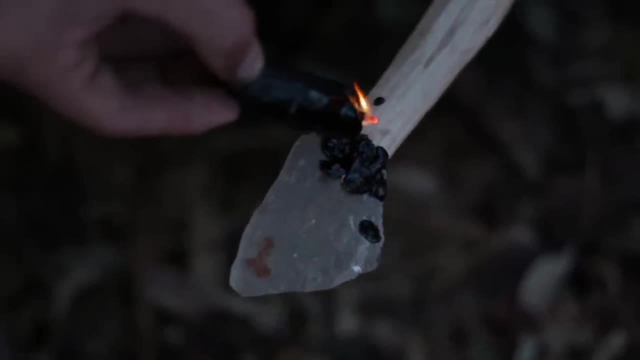 Though this is not surprising considering the date between 300 and 330 thousand years ago. Though this is not surprising considering the date between 300 and 330 thousand years ago, Hafted points would become more frequent in later time periods. In addition to the spears, there were other wooden objects. 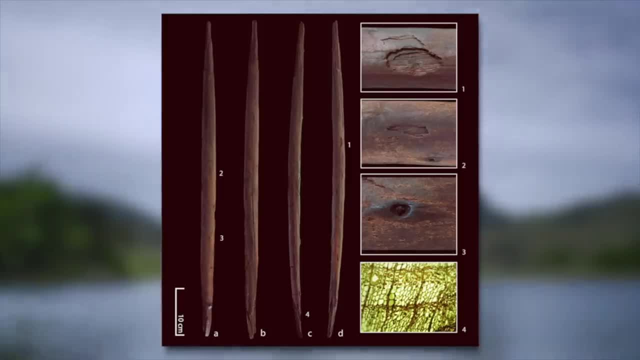 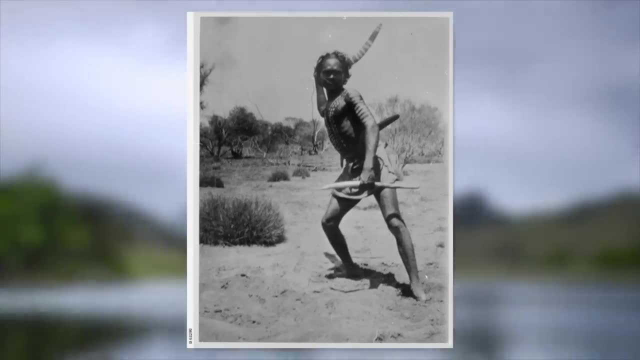 Double pointed sticks of 64 centimeters or 2 feet long are suspected to have been used as throwing sticks. Double pointed sticks of 64 centimeters or 2 feet long are suspected to have been used as throwing sticks. Throwing sticks have been used across many human societies to target small game or to drive large game. 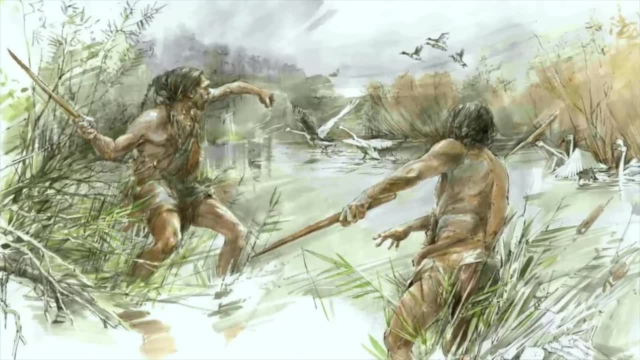 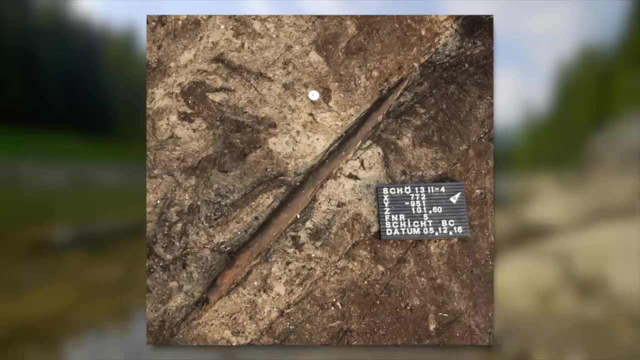 The Neanderthals at Schoenaghan may have been targeting waterfowl with these weapons. Another wooden tool found at the site was a charred wooden stick that has been interpreted as a skewer for roasting meat. The last wooden objects yet to be mentioned were short work shafts with notches cut into. 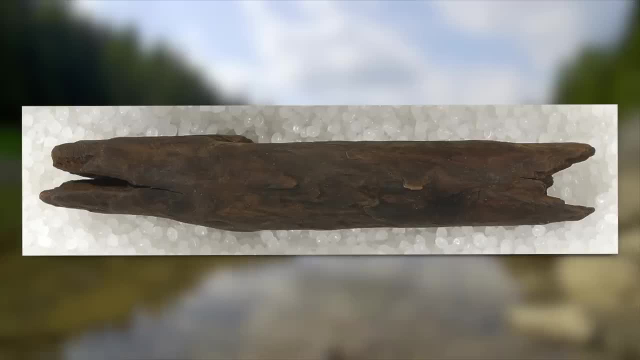 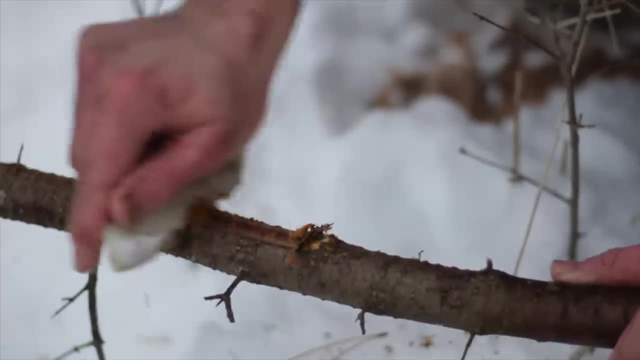 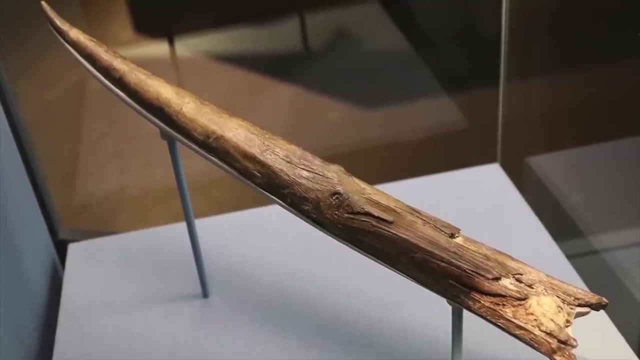 them. They have been inferred as handles for stone tools. They were likely paired with a sharp flake that would act as a knife. Other wooden tools created by Neanderthals exist, though they are very rare. The oldest wooden tool that is either attributed to early Neanderthals or their ancestors is 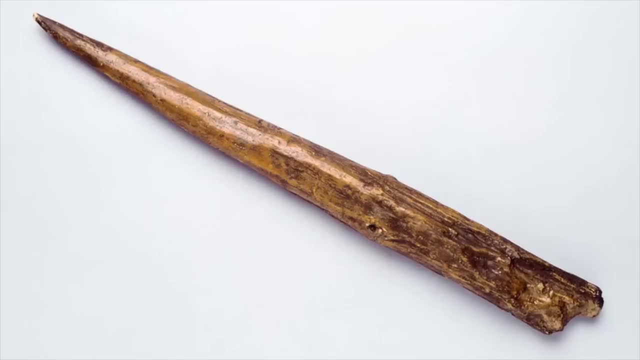 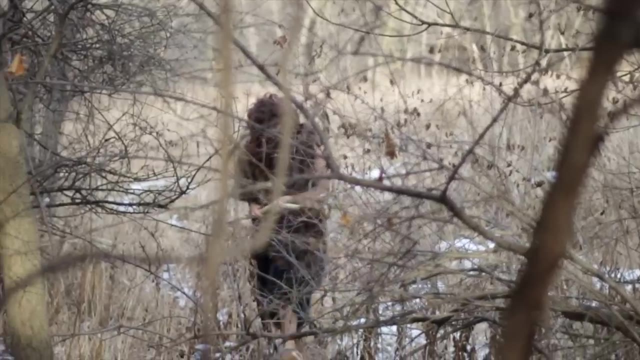 the Clacton spear. It was discovered off the coast of England and has dated to around 420,000 years ago. Since the spear only consists of a tip, it is unknown if the spear would have been suitable for throwing, though it certainly could have been used for thrusting. 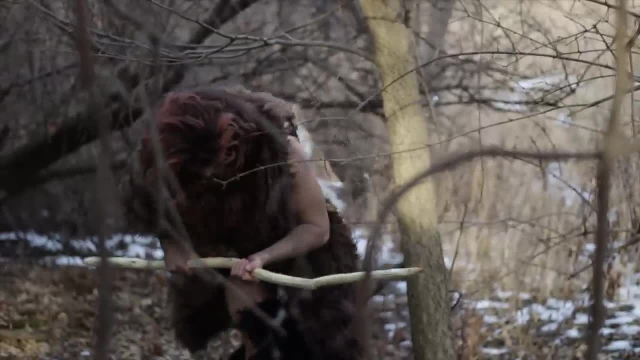 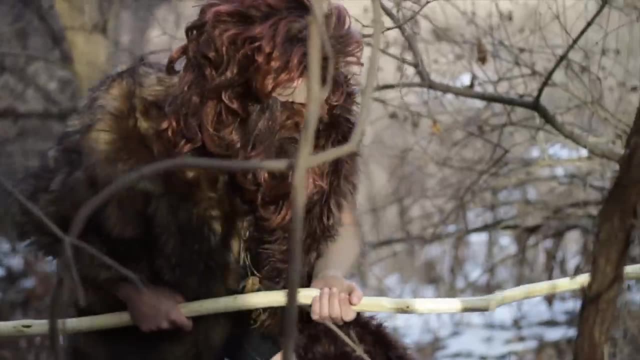 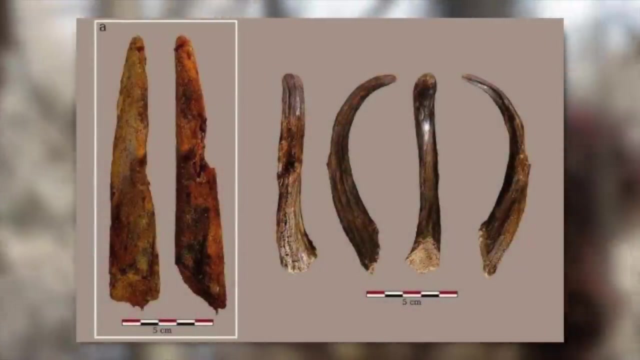 The existence of this technology predating the appearance of true Neanderthals and its appearance here is unknown. Scientists in Germany, 100,000 years later, suggest that most, if not all, Neanderthals would have used wooden spears. Other Neanderthal wooden objects have been found, including another spear, though their 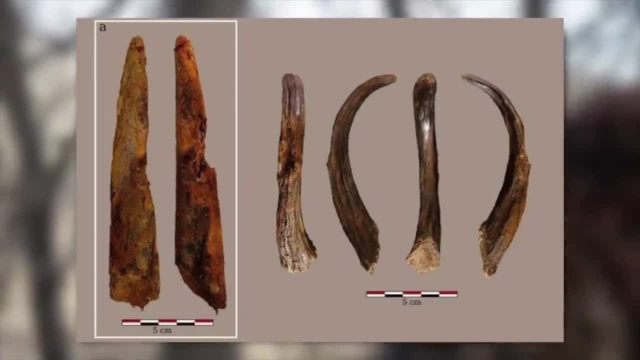 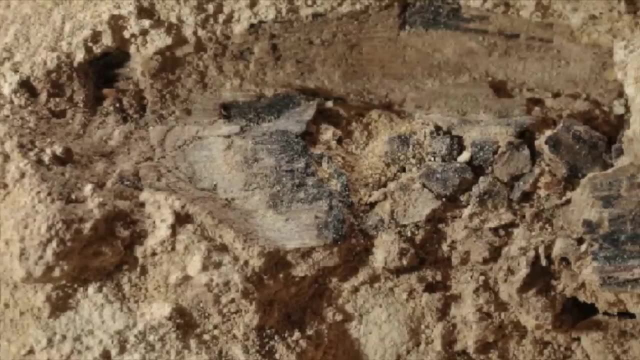 preservation is poor and their purpose is debatable. The site of Ebrek Romani preserved the imprints of many wooden objects. Though the wood has long since decayed, the travertine has preserved a cast with incredible detail. A few flat wooden dikes have been found here. 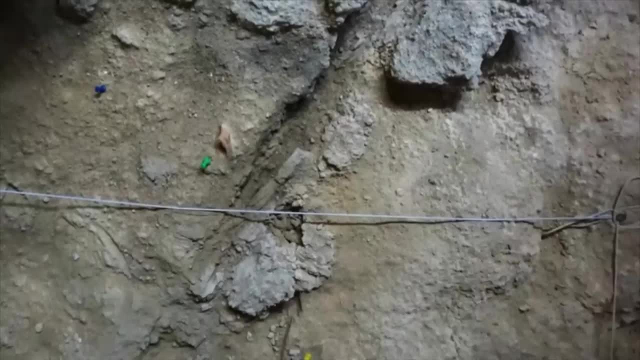 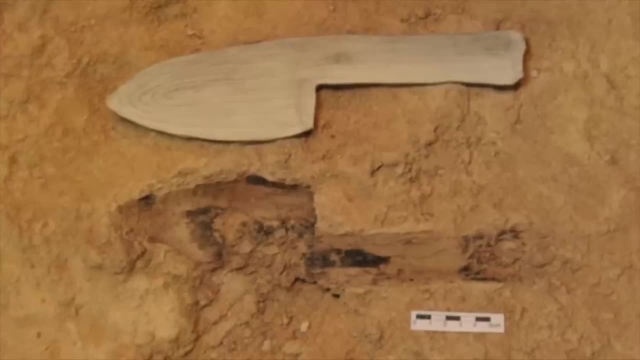 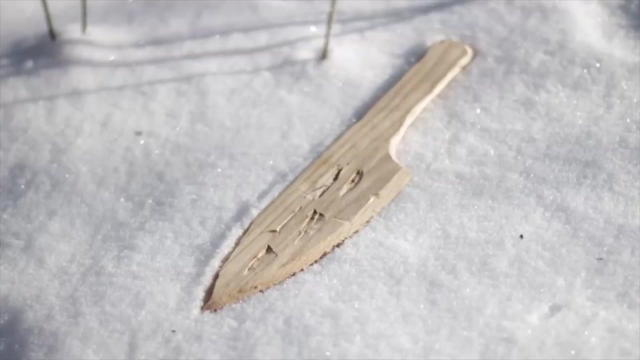 A large pole, 5 meters or 16 feet long, may have been part of this structure. An impression of a very interesting knife or spade-like object was also found. The object is very unique, as it is not something that we see in contemporary indigenous societies. 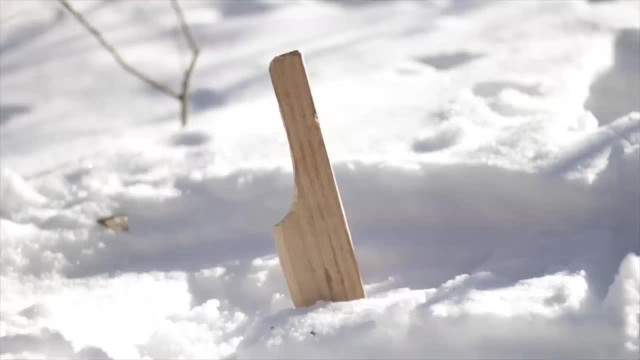 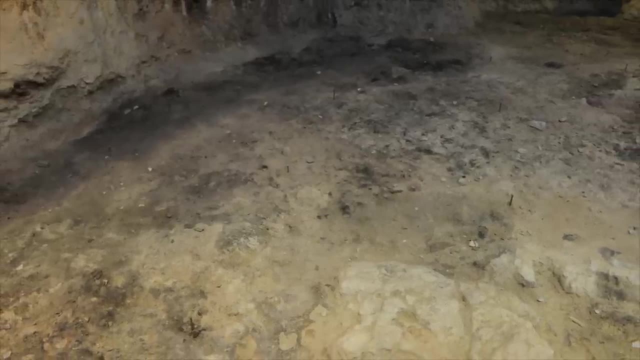 It may have been used as a butchering tool, or perhaps a digging tool. We will never know for sure. There are a handful of other impressions from wooden dikes. There are a handful of other impressions from wooden tools that are more enigmatic. 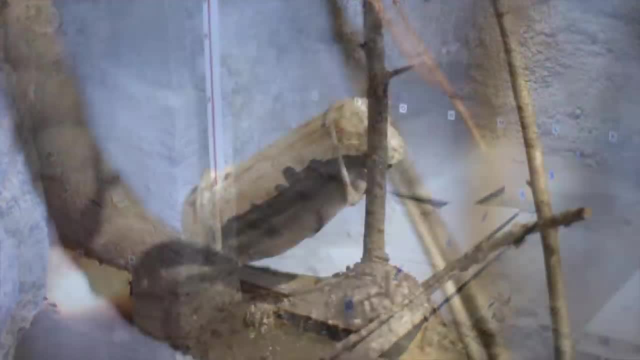 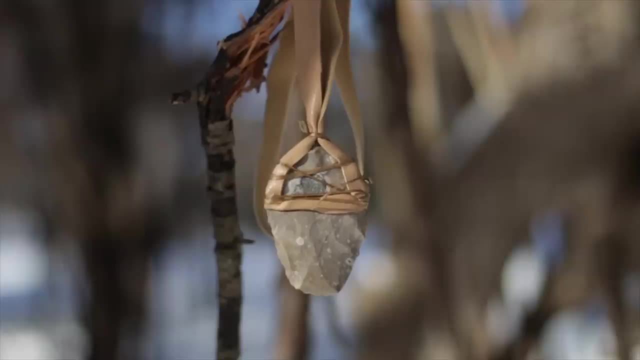 Overall, the findings at Ebrek Romani have taught us that much of the items made and used by Neanderthals would have been wooden. Besides spears and handles, many unique objects would have been made. Those stones have stood the test of time. 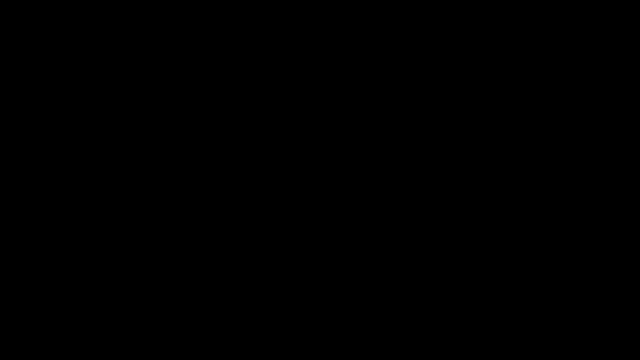 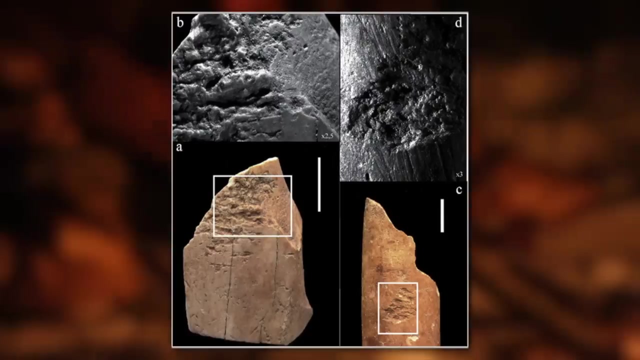 Wooden tools were just as essential to Neanderthal survival. Neanderthals also utilized other materials when creating tools. Bone and shell tools were used, though they were not used in the original Neanderthal tools. They were not used in the original Neanderthal tools. 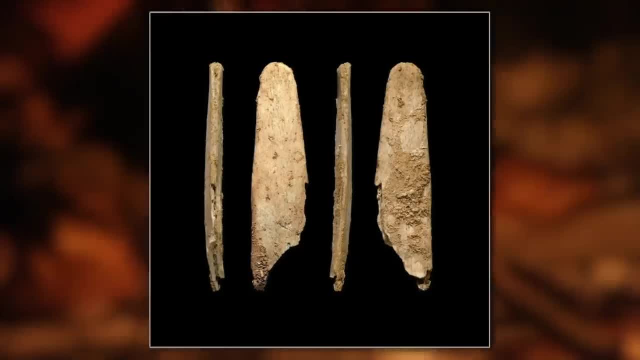 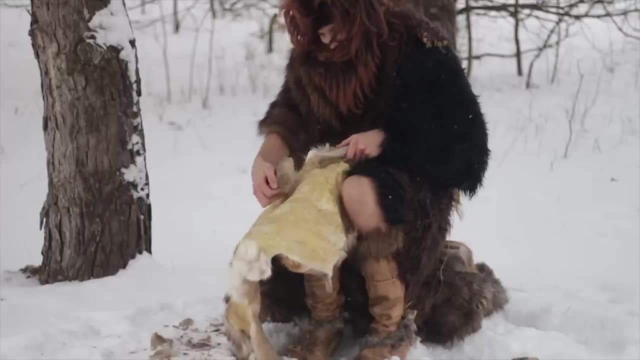 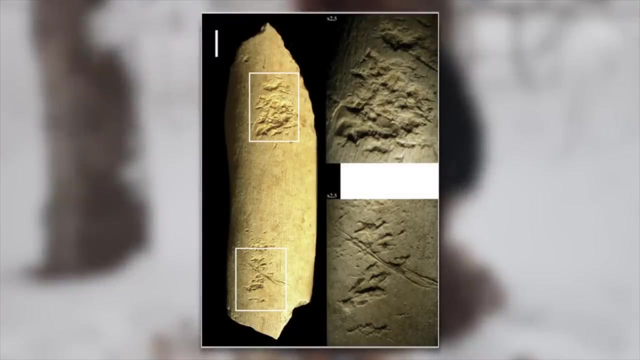 They were used in limited ways. Bone tools were mostly limited to lissois and flintknapping tools. Hammers, often made of animal limb bones, were great tools for striking flakes off of cores. Smaller broken bone shards, called retouchers, are quite common throughout Neanderthal sites. 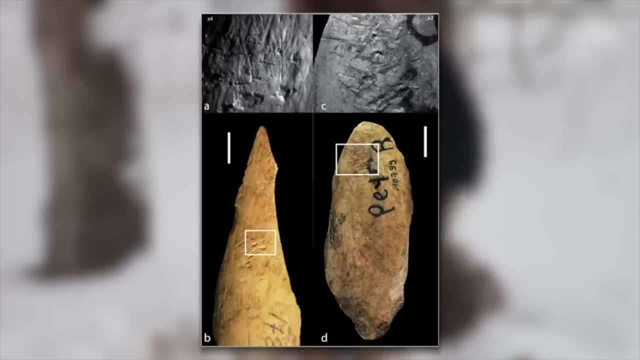 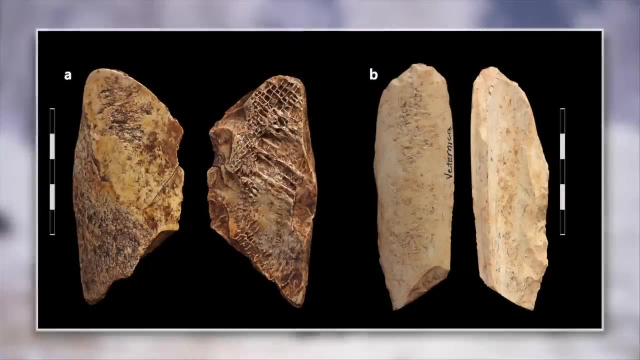 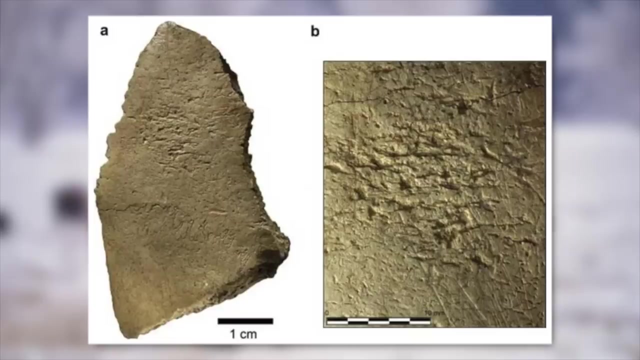 They vary in construction, but Neanderthals generally preferred the bones from the rear limbs of large animals such as aurochs, horse and bison. Tools such as jaws, horn, cores and mammoth ivory were also utilized. In one case, even another Neanderthal skull fragment was used as a retoucher. 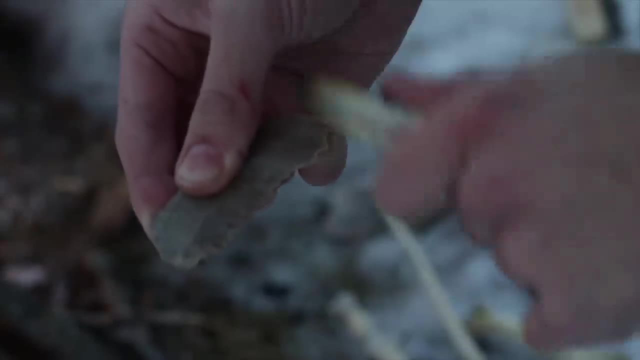 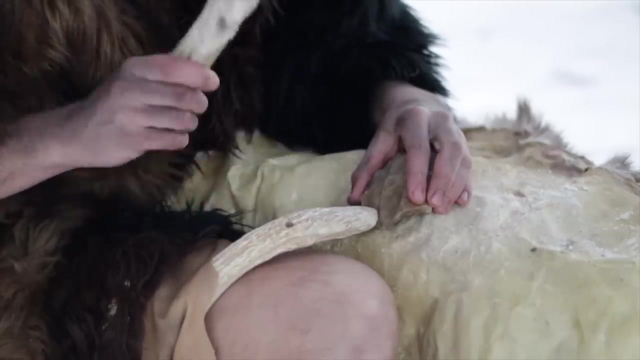 These tools would be used to resharpen stone edges by hitting off small flakes. Other bone tools display evidence that they may have even been used for indirect percussion flintknapping. This advanced flintknapping technique consists of two tools: a tool contacting the stone, 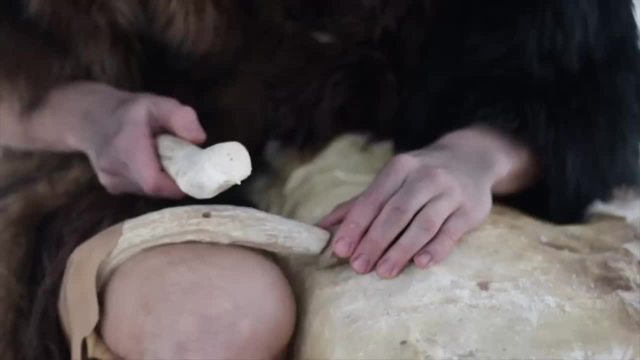 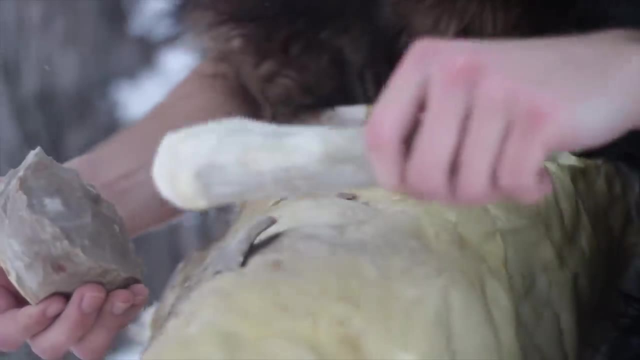 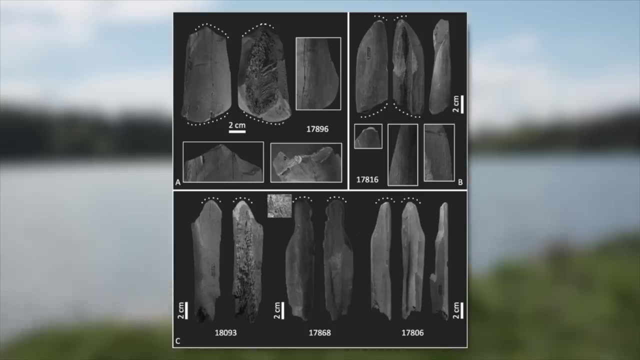 core and a tool to hit the other tool. This technique accurately focuses a lot of force into a small point. It is a very effective technique that allows for making much better stone tools. At the Schoenigen site, sharp bones may have functioned as knives to cut flesh. 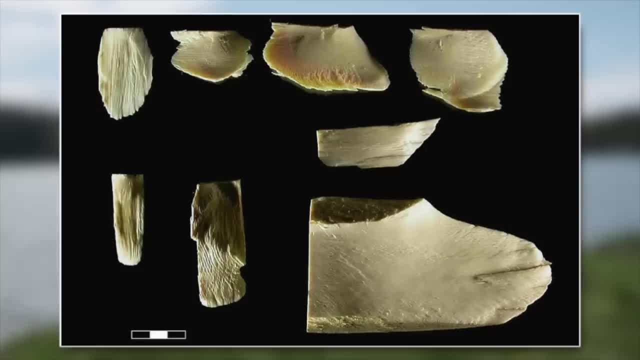 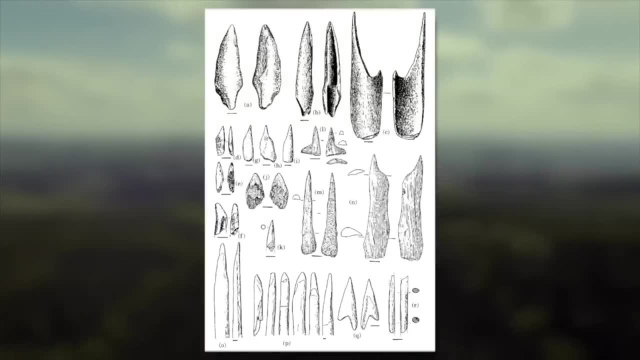 In other sites. mammoth tusks seem to have been split and napped into scrapers. At one site in Germany, over a dozen bone artifacts dating to over 60,000 years ago have been found. Some of these have been points. 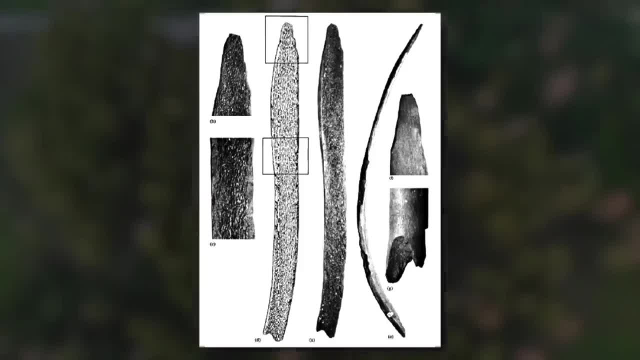 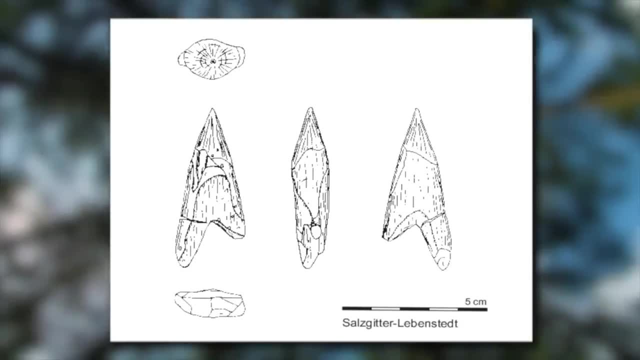 Flattened mammoth ribs with pointed tips may have functioned as spear points. A smaller point made of reindeer antler was almost certainly a spear point. It is light enough that it even could have been hafted on a javelin or a dart. 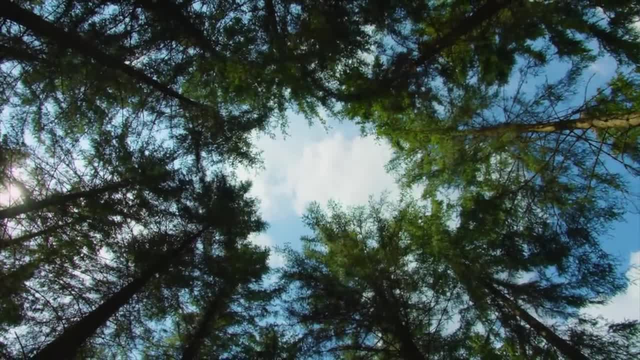 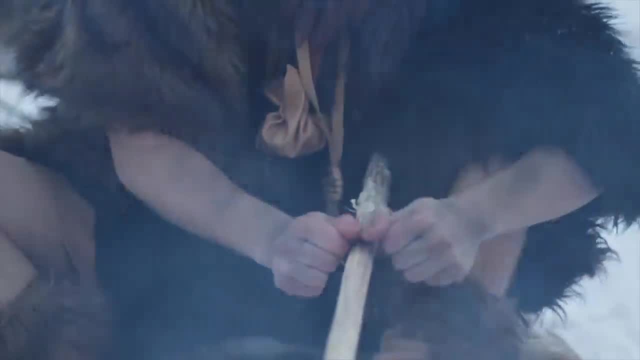 It is possible that a point of this size could have been hafted on an arrowhead, though our evidence does not suggest that Neanderthals ever used this technology. It certainly could have been part of a light throwing spear or possibly even an atlas. 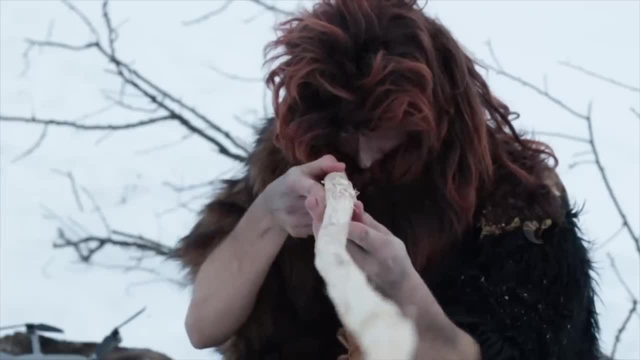 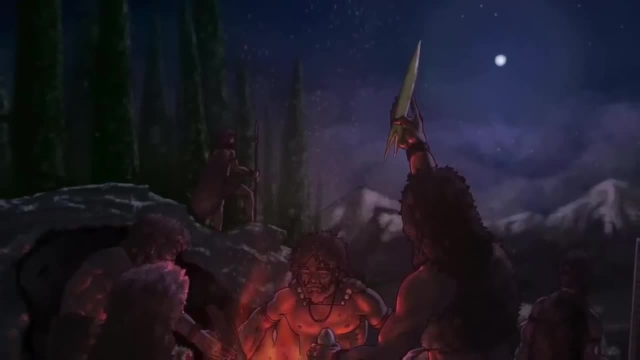 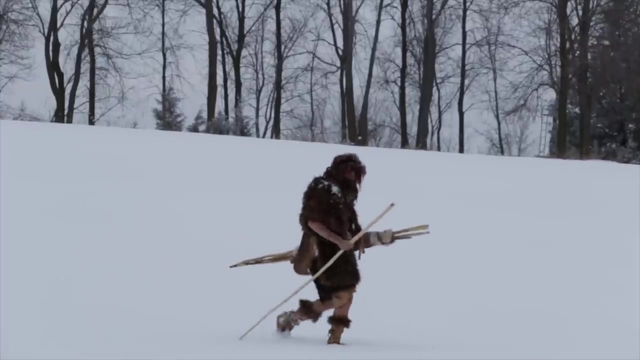 The point has been made, of a piece of iron. This idea is lacking any support, but it is an interesting idea to consider. The appearance of hafted bone points throughout Europe is largely correlated with the appearance of modern humans, but their existence in Neanderthal sites tells us that Neanderthals were certainly 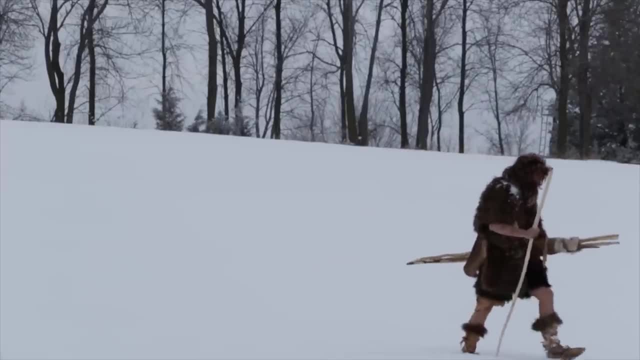 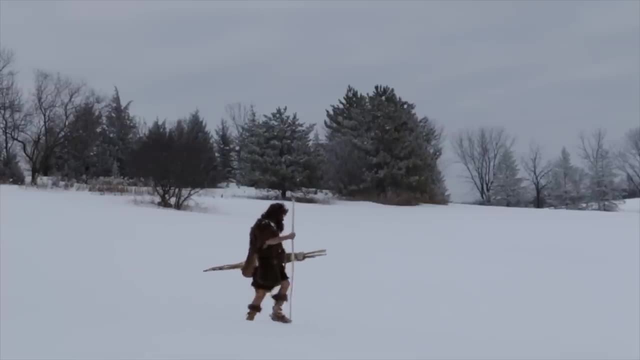 aware and capable of this technology to some extent. This technology is only found at one site in Germany, but bone does not always stand the test of time. It is possible that bone points were used elsewhere and left little trace, though we just don't know. 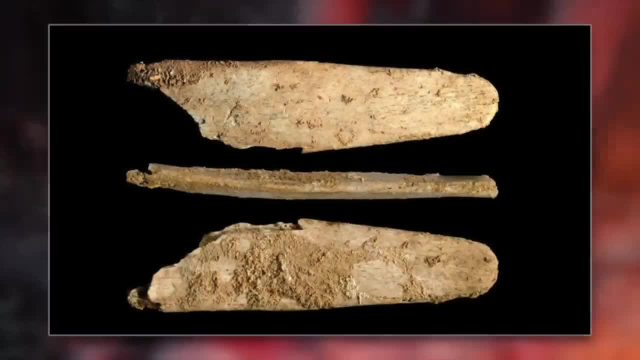 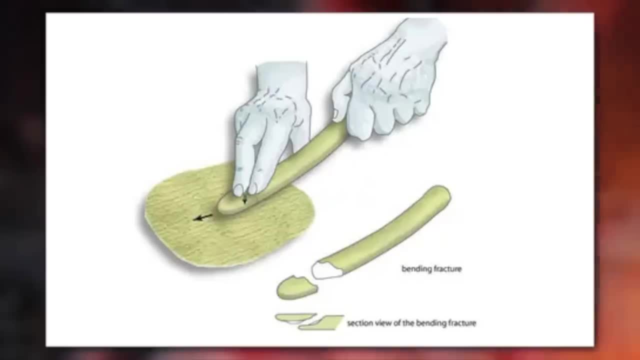 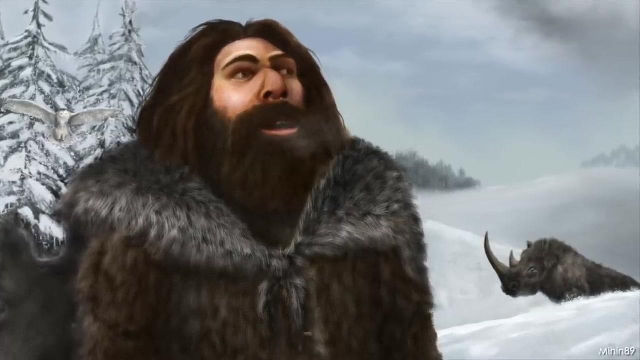 Another tool made of bone found at various Neanderthal sites were leatherworking tools called lissois. These tools, also known as slickers or burnishers, are used to rub into hides to make them softer and more water resistant. Neanderthals chose the ribs of large herbivores to make these tools. 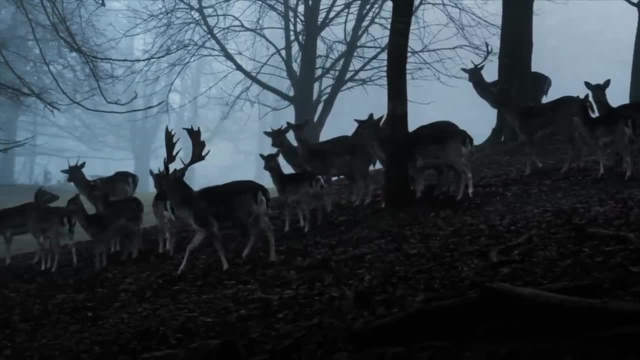 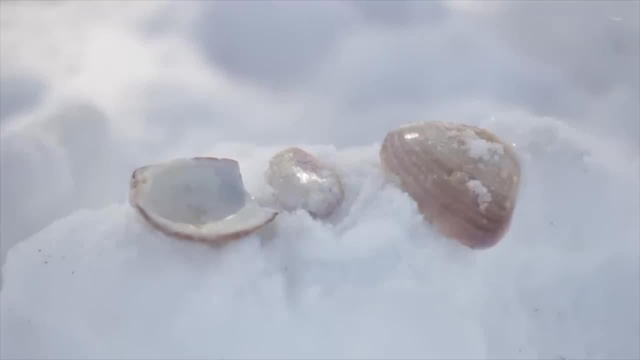 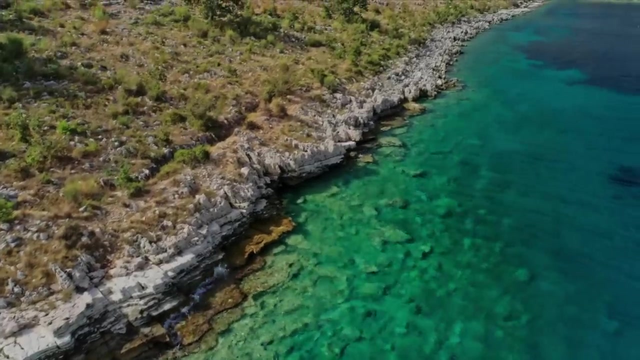 Though these lissois could be made with the abundant reindeer from which they hunted, they preferred the more uncommon bison and aurochs ribs. Besides mammal bones, shell was also heavily utilized by various populations of Neanderthals, particularly in the Italian peninsula. 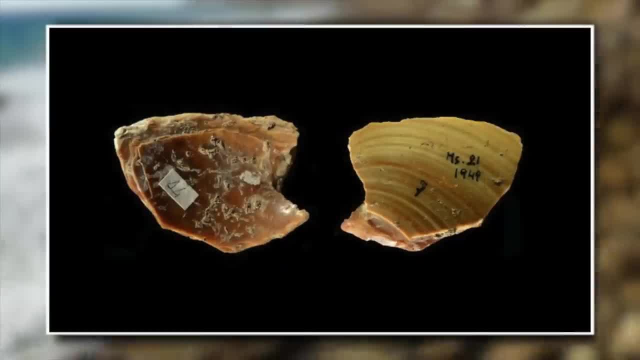 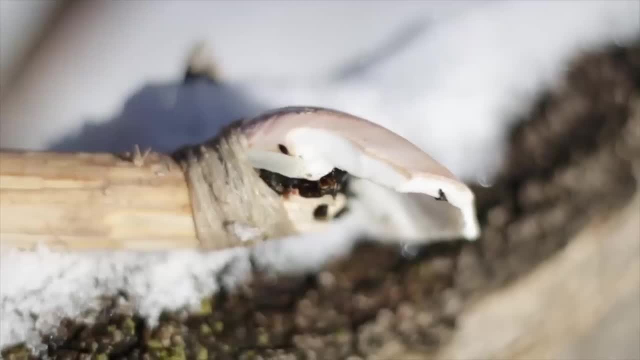 In areas of poor quality stone, we see that Neanderthals often used shell as an alternative. Shell is a hard material that can be napped similarly to stone, but can also be resharpened simply by rubbing against an abrasive stone. 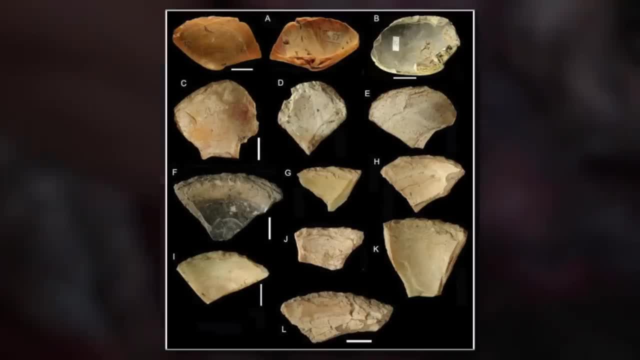 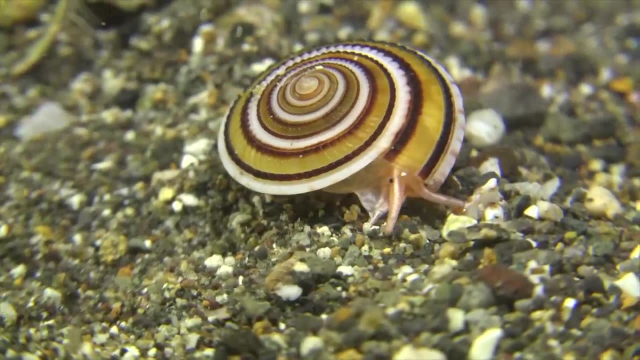 More than 70 work shell tools were found at Grotta dei Moscherini alone. Out of these shells, about 24% of them were gathered alive from the sea floor, meaning that Neanderthals had to wade or dive into shallow waters to collect them. 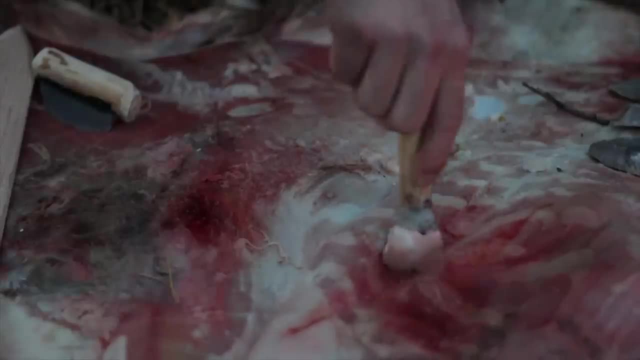 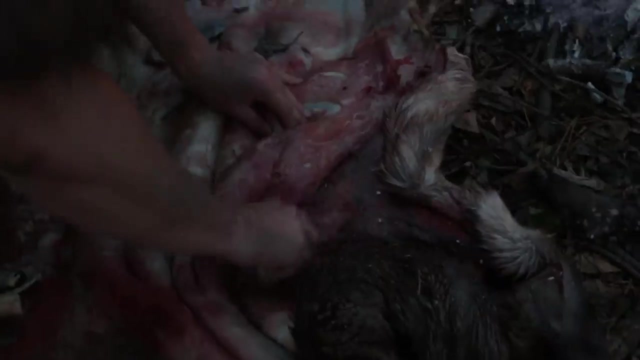 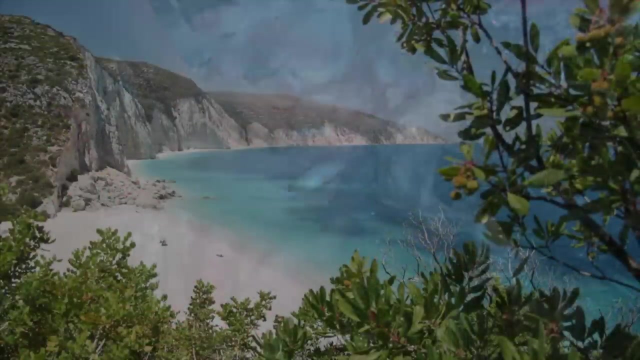 These live clams have stronger and more robust shells than unoccupied specimens. They also offered a small snack every time they needed another tool. Across various sites, these tools were used for cutting meat, scraping bones, etc. Shell tools were also found in parts of Italy and Crete, but are absent from other. 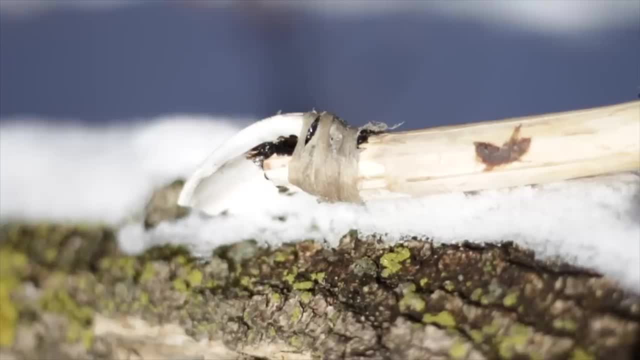 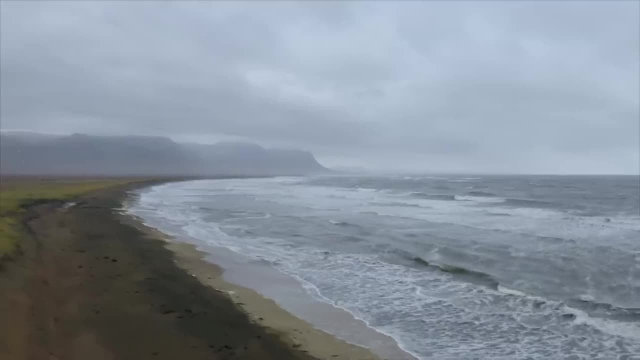 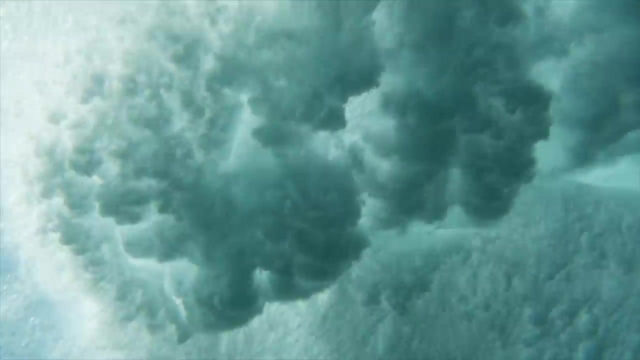 Mediterranean sites. Considering that Neanderthals were certainly using aquatic resources elsewhere, it is strange that shell tools were not more common. It is possible that these sites exist, but lie beneath the ocean's surface. The ocean undoubtedly conceals many other facets of Neanderthal life. 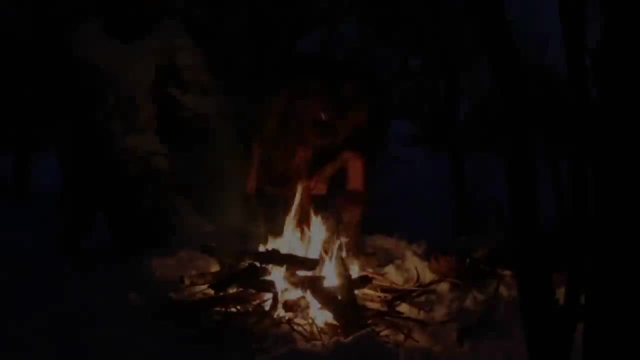 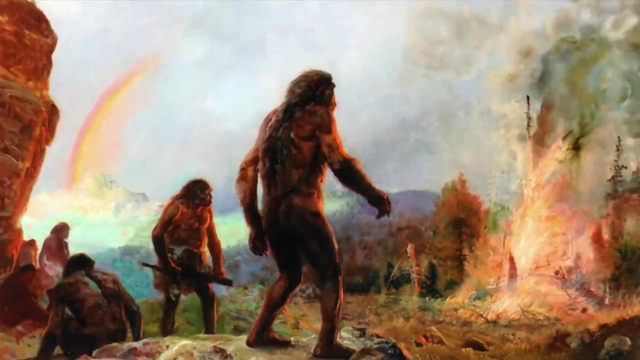 Again, this is very dangerous of an open title. Any questions about how these materials came around changed the Mog seperti world. The use of fire was clearly a major technological development for our genus. Evidence of the use of fire by our ancestors extends more than a million years into pre-history. 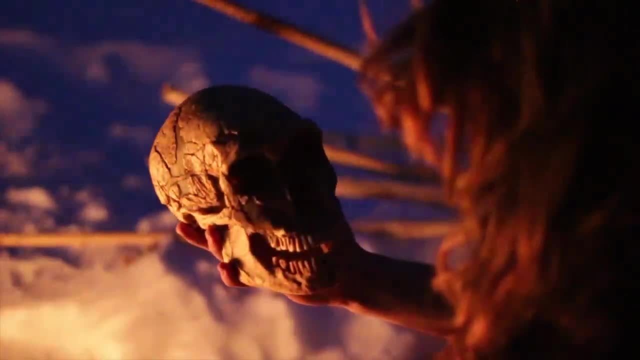 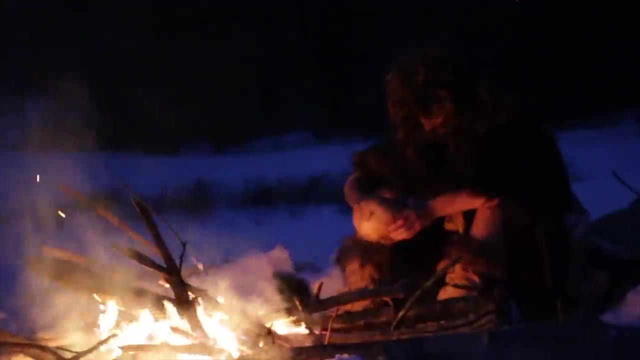 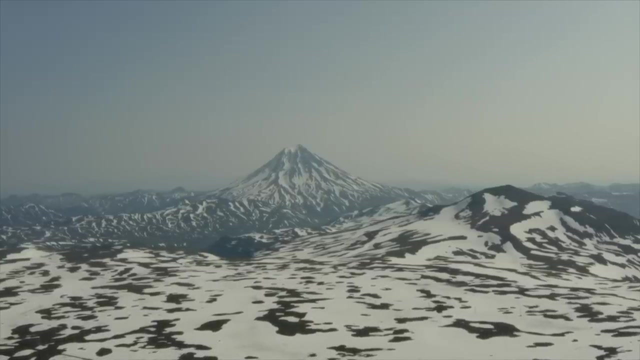 To understand the significance of this technology, we should take a further look into why exactly it was so advantageous. First and foremost, fire provided heat. Neanderthals lived across a range that was quite often cold, depending on the current environmental conditions. Other ways to stay warm existed, such as clothing, but fire provided direct heat. 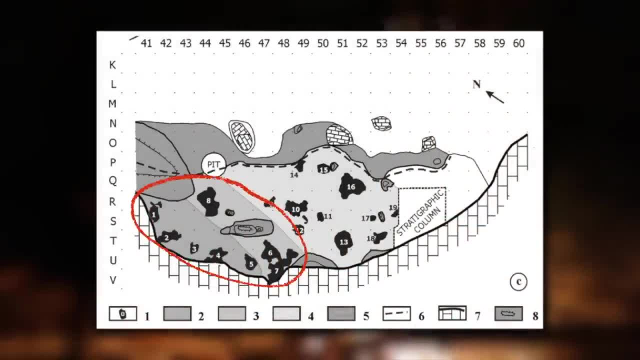 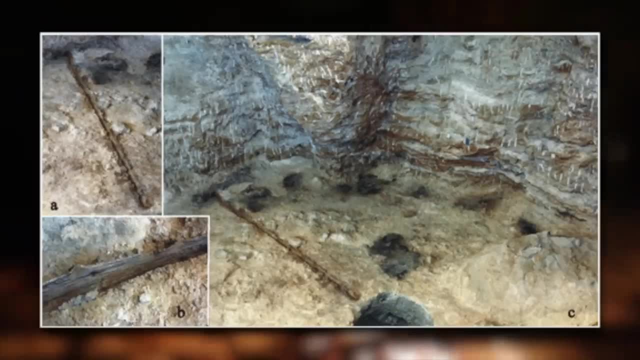 At the site of Aberich Romani, there are eight evenly spaced hearths aligned against the rock shelter wall. These hearths have been interpreted as personal fires to keep individuals warm while sleeping. Similar constructions have been observed by Australian desert aboriginals. 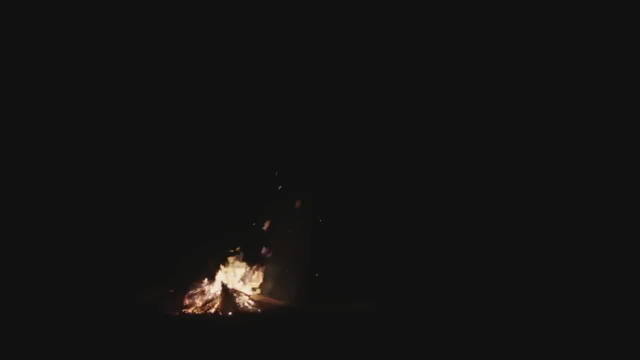 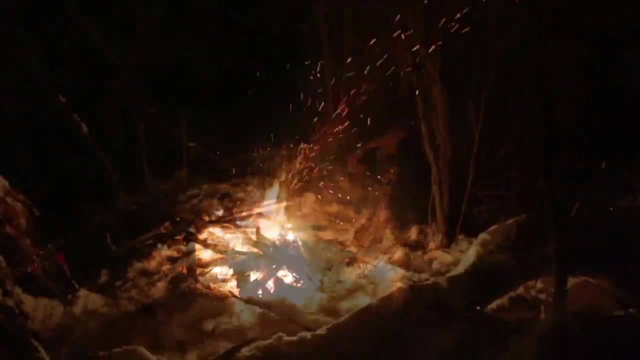 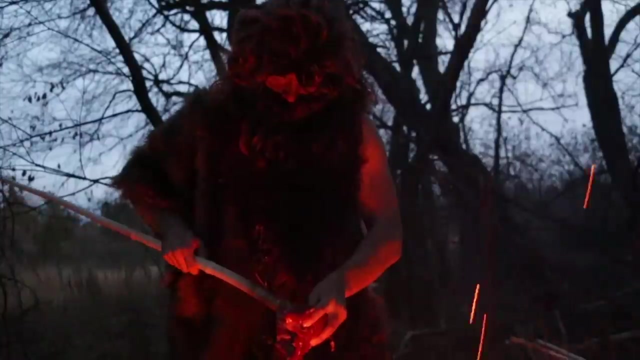 They would sleep with little glowing campfires on either side of them. The altering position between each individual and fire provided an economical way to stay warm. Other Neanderthal sites show similar constructions. The advantage of fire, arguably more important than warmth, was its use for cooking. 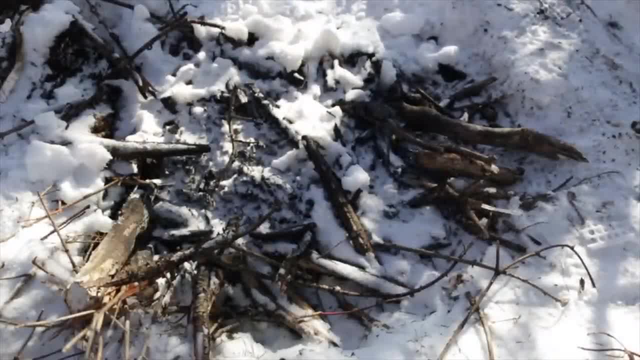 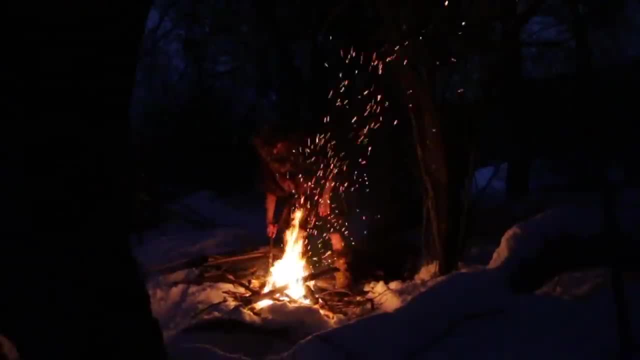 Jarred bones that may have been cooked are widely known from many Neanderthal sites. They suggest that the meat and marrow were likely being cooked. Other tissues, such as organ meat, does not preserve well in the fossil record. However, they are likely to be cooked. 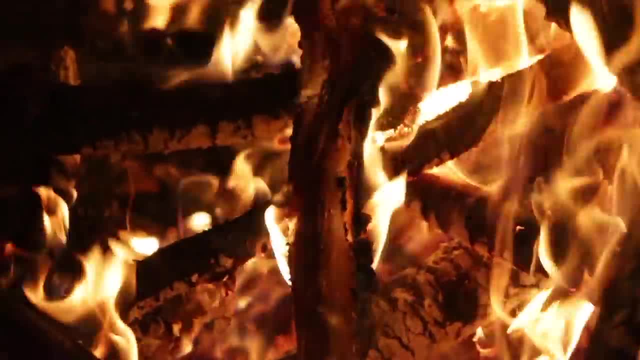 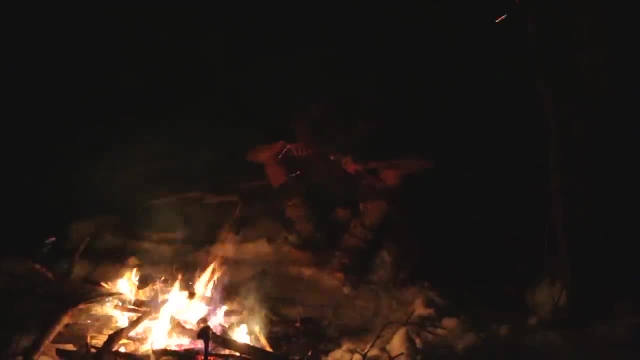 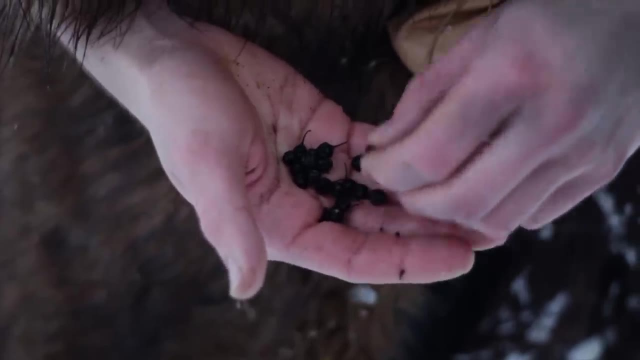 Cooking meat breaks down tough fibers and connective tissue, which makes it easier to chew and digest. It also leads to better nutrient absorption and kills any harmful pathogens. Direct evidence for cooking plants is very rare in the Neanderthal fossil record, though it does exist. 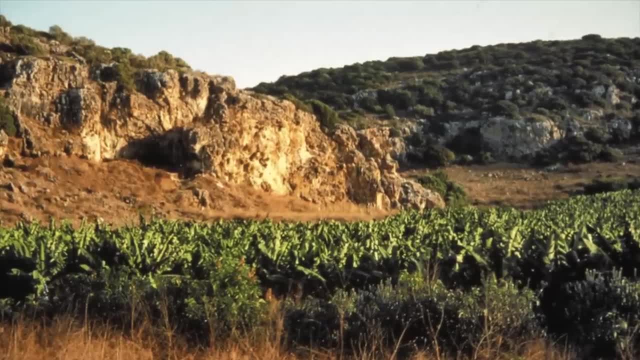 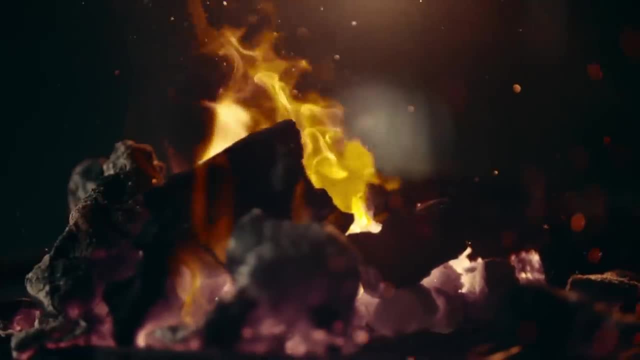 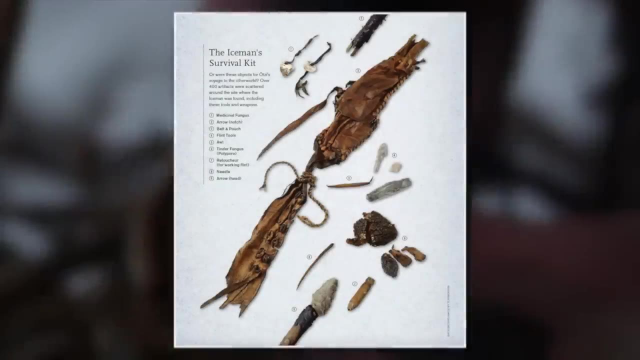 There are plenty of ways to carry an ember. A smoldering piece of wood can simply be wrapped in green leaves, though other materials, such as fungus, may be more effective. Woodsy the Iceman was found with a Tinder fungus that is suspected to have been used. 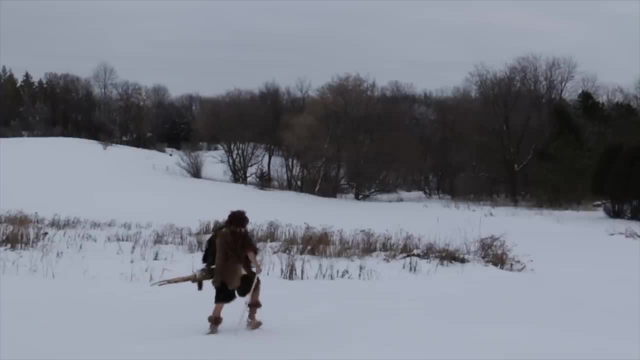 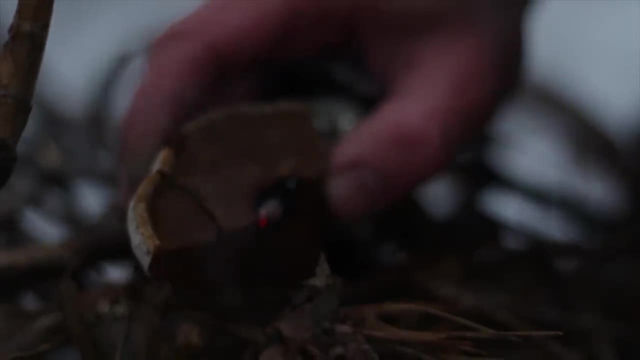 to carry embers. Once set alight, tinder fungus can smolder for hours before going out. Though we do not have evidence of Neanderthals using this technology, it is still interesting to speculate. Another technology that Neanderthals must have utilized. 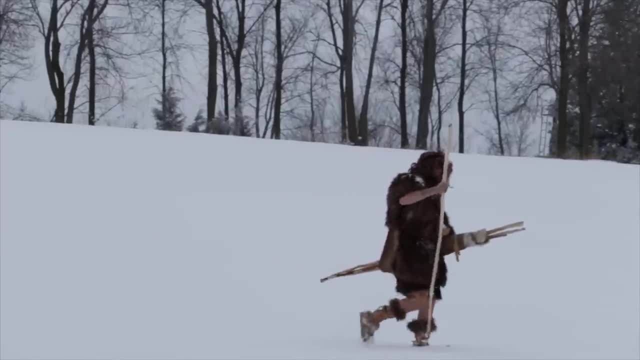 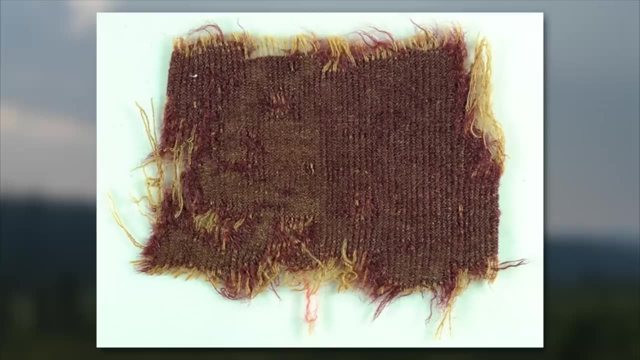 to survive the colder winter months is clothing. Clothing may have been used as far back as the lower Paleolithic, though direct evidence does not exist. Our oldest direct evidence of clothing is less than 10,000 years old. It just doesn't stand the test of time. 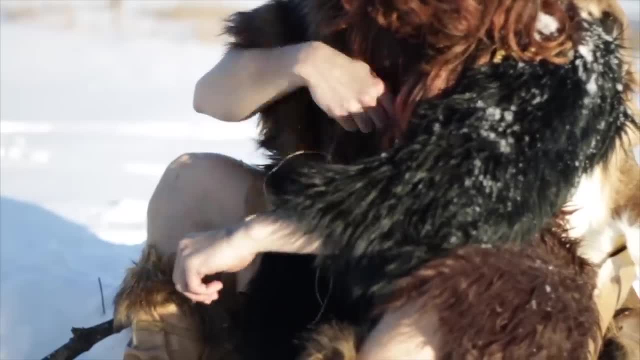 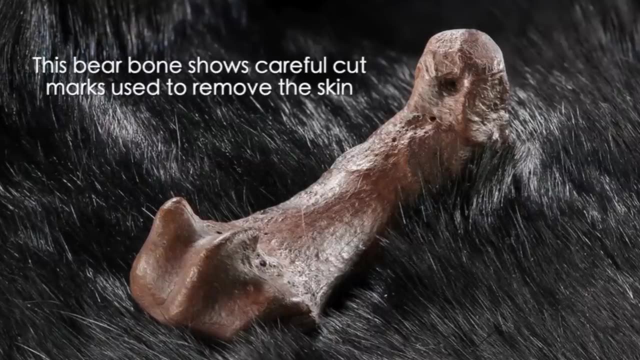 However, many forms of indirect evidence can tell us an incredible amount about the clothing that Neanderthals would have worn. The placement of cut marks on the bones of butchered animals indicates that Neanderthals were preserving the skin of their prey. 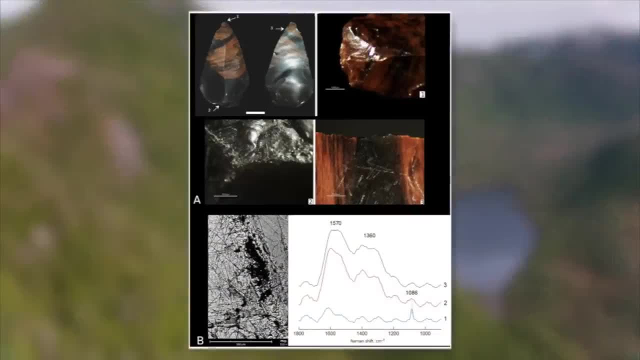 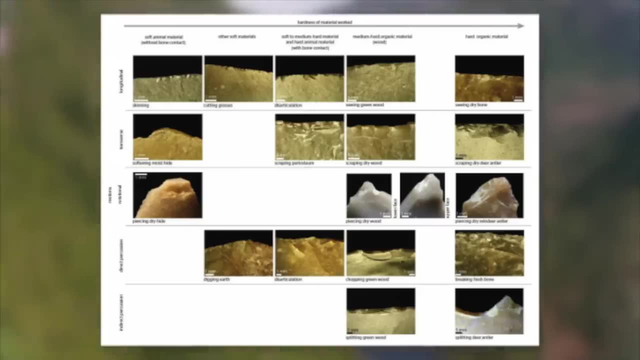 Use. wear on lithics from dozens of Neanderthal sites confirmed that they were being used on hides. Researchers are even able to distinguish lithics that were mainly used on fresh hides from ones that were used on dry processed hides. Some artifacts are so worn. 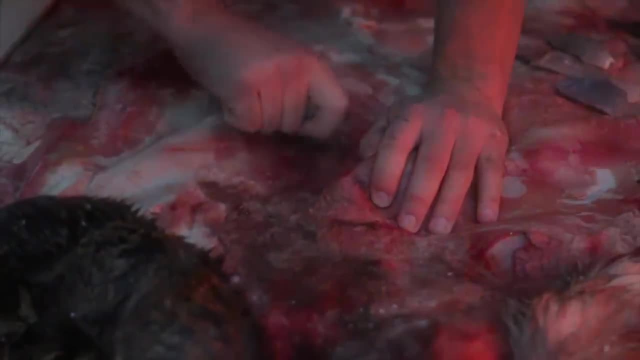 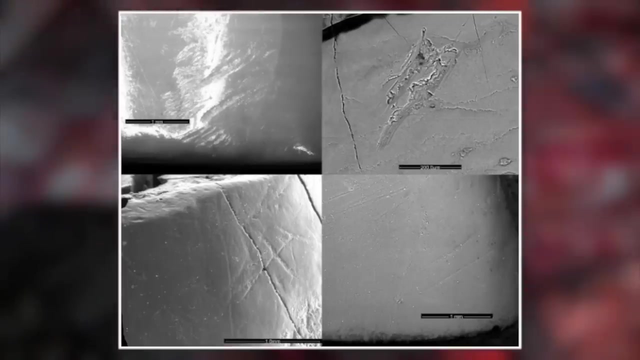 that they must have been used for many hours. Heavy wear present on the teeth of Neanderthals, similar to contemporary hunter-gatherers, indicates that they were using their teeth as a clamp to hold onto hides as they worked them. Neanderthals from colder regions. 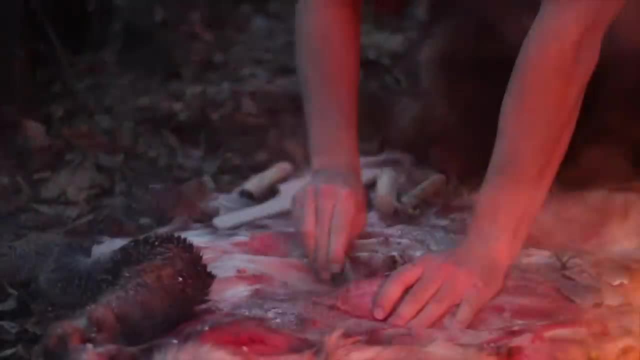 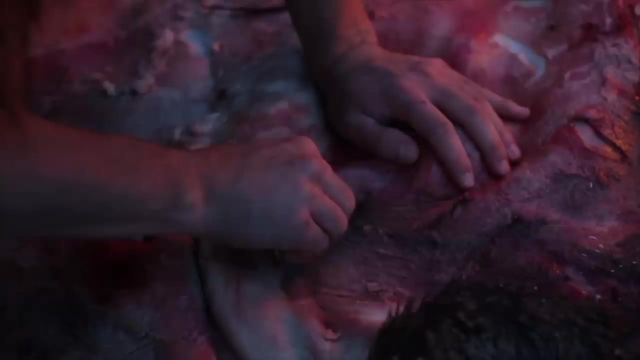 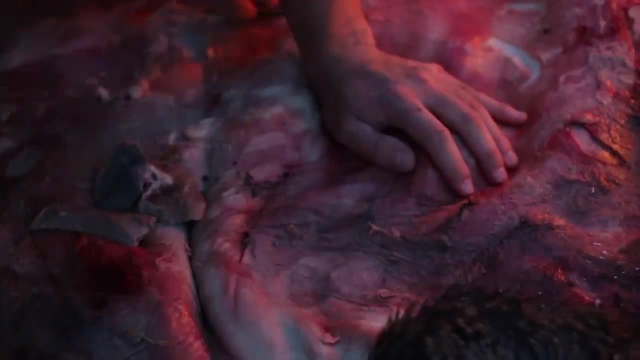 even show significantly more wear on their teeth, suggesting that hides were being worked at a higher frequency. Hide working is a hard, time-consuming process. First, all fat and muscle tissue must be cleaned from the hide shortly after butchering an animal, or else the hide will rot. 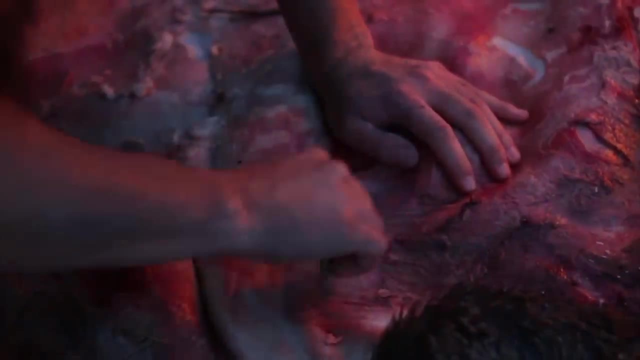 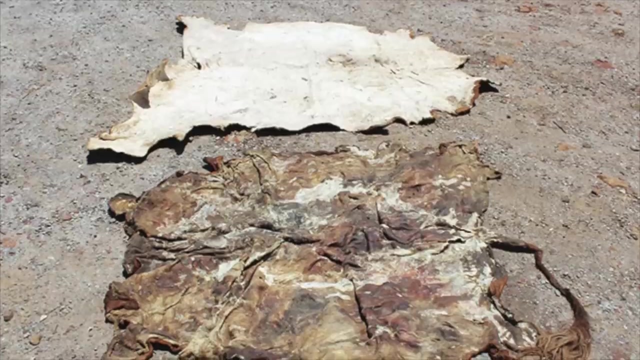 This process is very time-consuming and physically demanding. This is what happened to Neanderthals. This is what hide scrapers would have been used for- a very common tool in Neanderthal assemblages- After drying in sunlight, by a fire or in a dry cave. 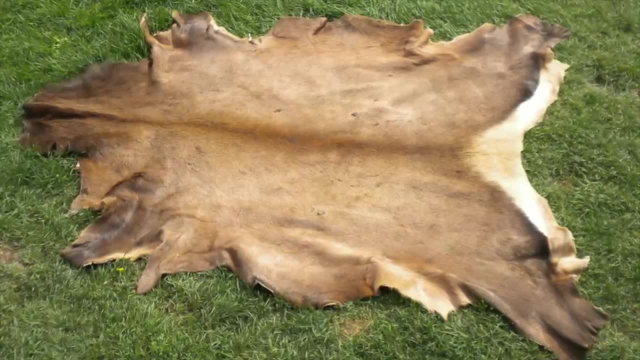 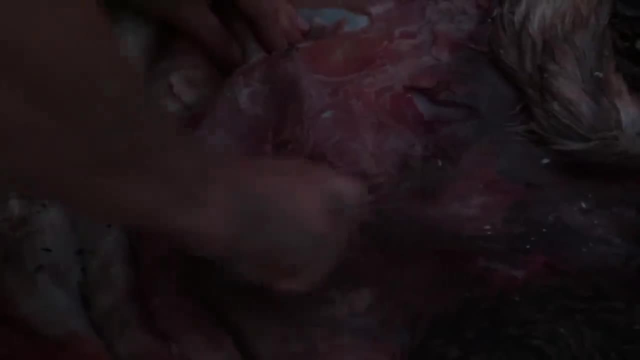 the hide can be stored indefinitely without spoiling. But a dry hide can be as stiff as a board. It must be worked further. The hide must be soaked in a water source to become pliable once again. Once wet it is easily stretched. 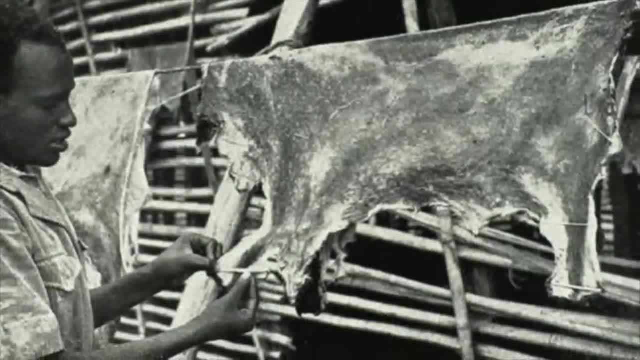 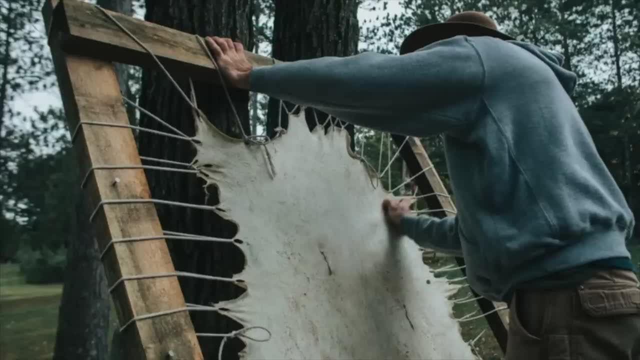 This can be done over a hard surface or even by hand. After sufficient stretching, it can be left to dry once more. The next step would be to work a fatty substance into the hide. This waterproofs the hides and makes them even softer. 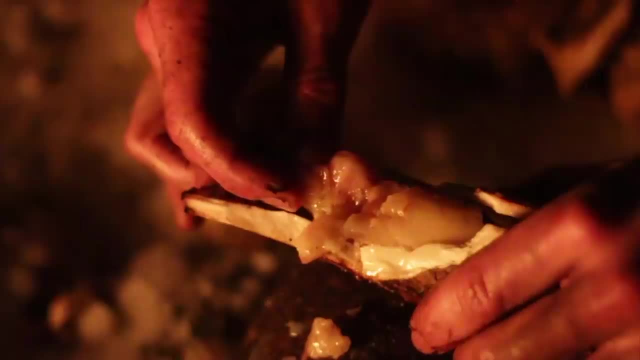 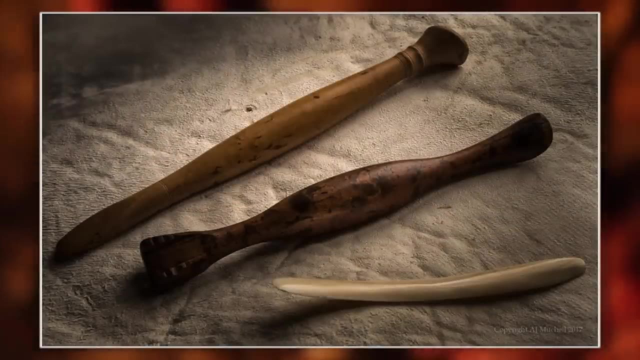 Any kind of fat could be used, but bone marrow and especially brain work much better due to their natural chemistry. At this point lissois could be used to further work the hide. They are not essential, but they make a much finer product. 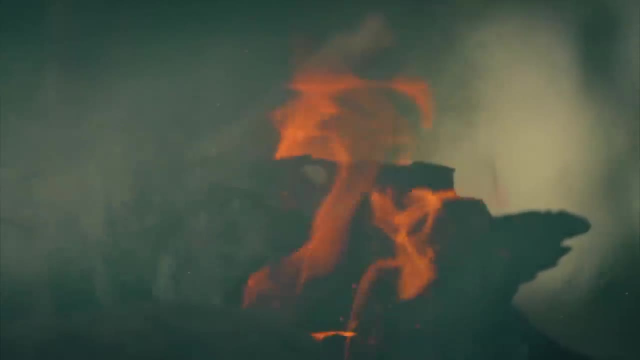 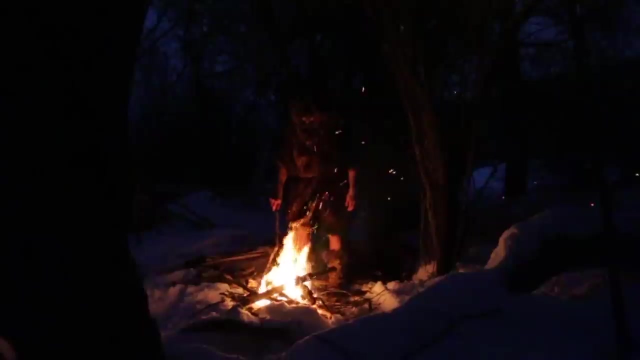 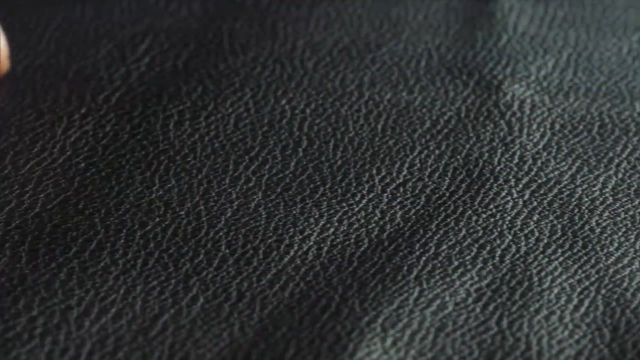 The last step that may have been used is smoking. Smoking a hide drastically increases its longevity and durability. It is not essential, but Neanderthals were likely aware of its effects on their hides. Evidence from the site of Newmark Nord suggests that Neanderthals even tanned their hides to make leather. 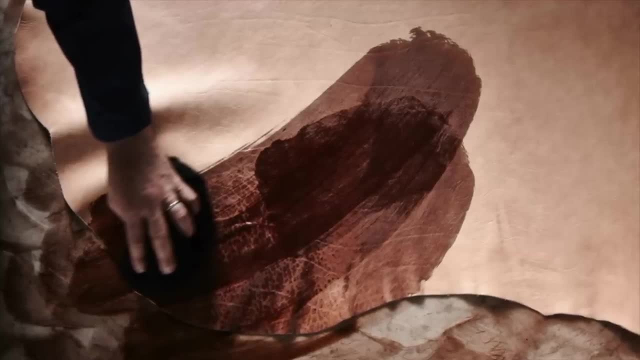 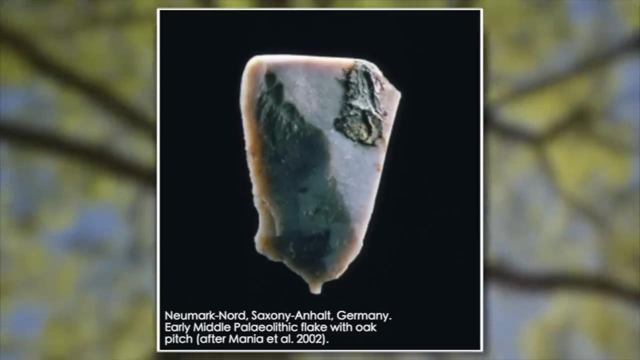 Hides must be exposed to tannins in order to stabilize the proteins to resist decay. Tanning seems to have been done at this site with boiled oak and chestnut bark. Soaking the hides in this solution would have not only improved the quality of the hide but also the quality of the protein. Soaking the hides in this solution would have not only improved the quality of the protein, but also the quality of the protein. Soaking the hides in this solution would have not only improved the quality of the protein, but also the quality of the protein. 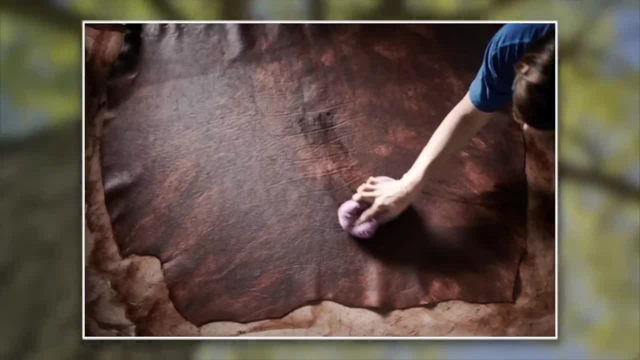 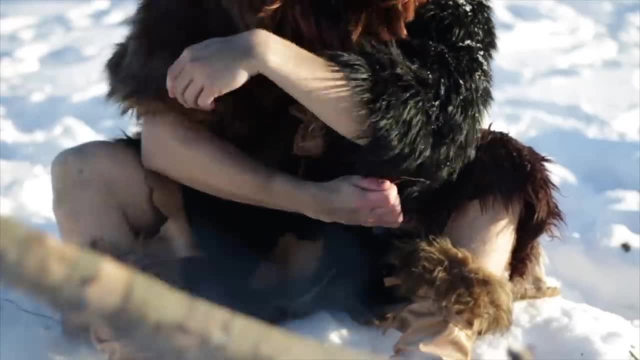 The process was often used to make the hides more delicious, but also made them last much longer. This process may have been used at other sites, though further evidence is required. Hides may have been used for a number of things, but clothing was certainly an important process. 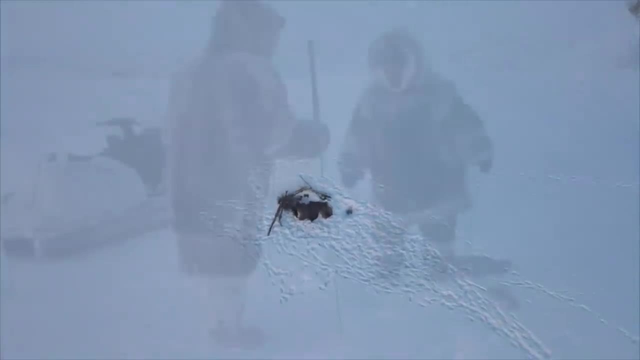 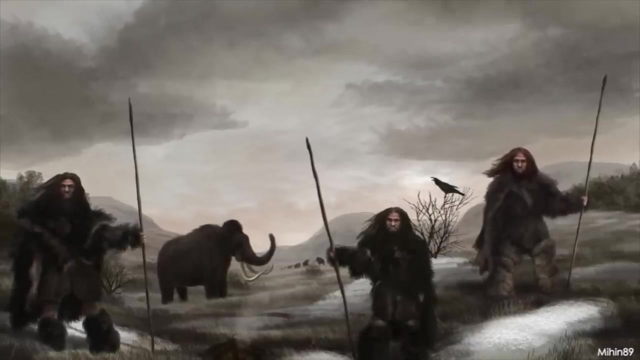 Neanderthals lived in colder environments than contemporary hunter gatherers that wear parkas and other heavy clothing. Thermal modeling has shown that Neanderthals must have covered much of their body in colder regions to survive, Though Neanderthals were stockier than moders. 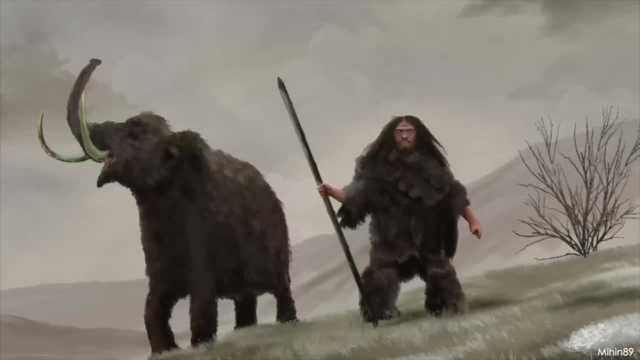 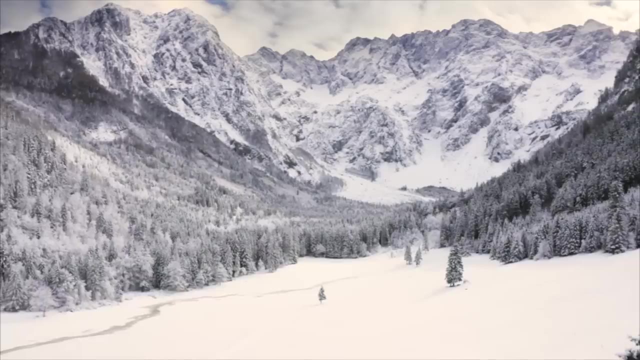 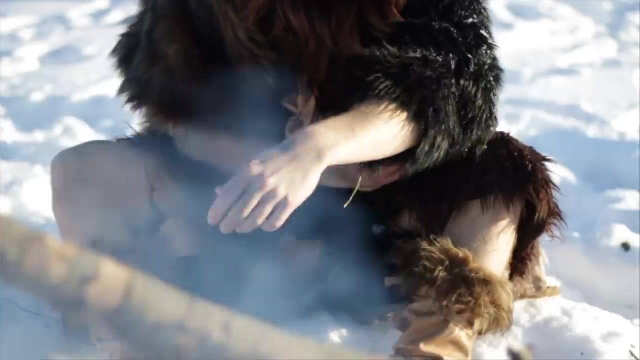 Neanderthals were stockier than moders, than modern humans, and able to deal with temperatures four degrees celsius colder. taking this into account, wales et al 2012 compared the climate that the neanderthals lived in to 245 modern human hunter-gatherer groups. the resulting data predicted that, on average, 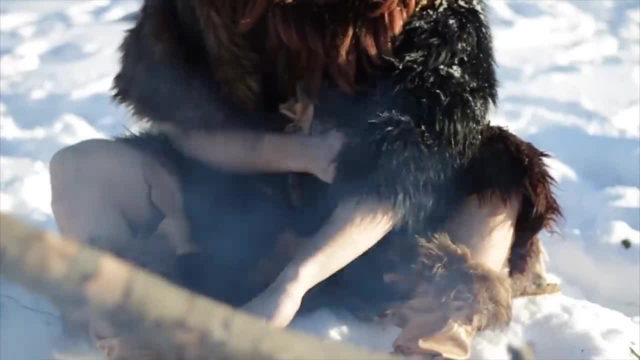 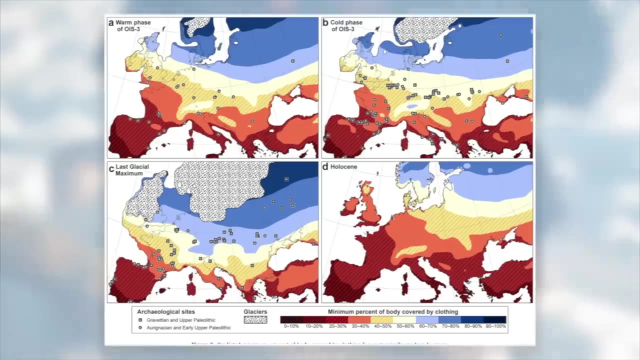 neanderthals would have had to cover up to 80 of their bodies during winter. the amount of clothing they would have needed heavily fluctuates from region to region and depending on whether or not the world was in a glacial or interglacial period. 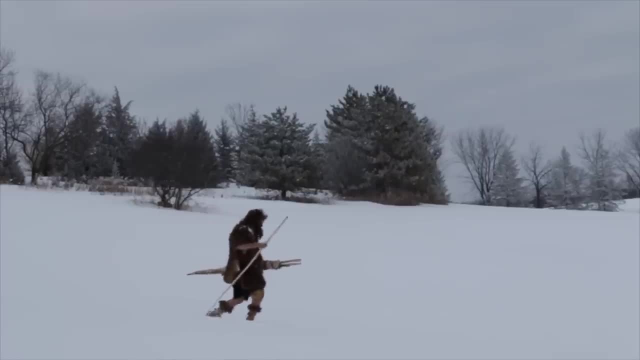 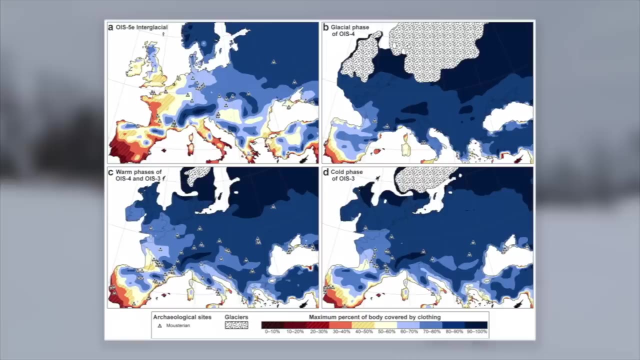 neanderthals living in central europe during glacial periods would have had to cover over 90 percent of their bodies. during the winter, though, even in the coldest periods, neanderthals living on the coast of the mediterranean would have had to wear much less clothing. 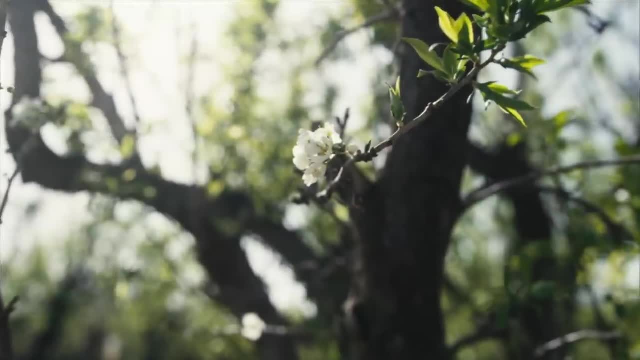 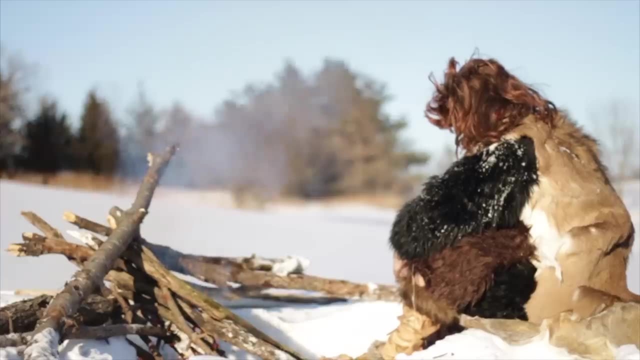 clothing would have certainly fluctuated from season to season and, in larger scales, with climatic changes. as for the actual clothing itself, it is hard to say what exactly the would have worn wales at all did suggest that hands and feet must have been covered in colder. 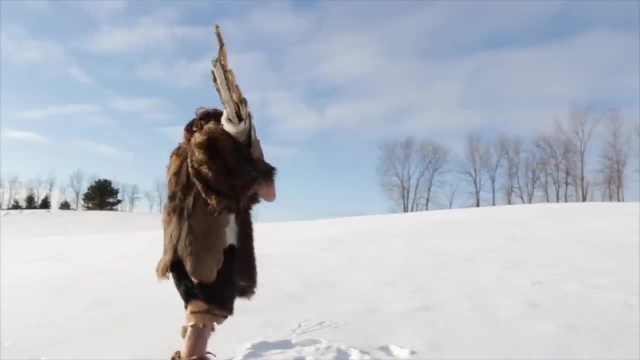 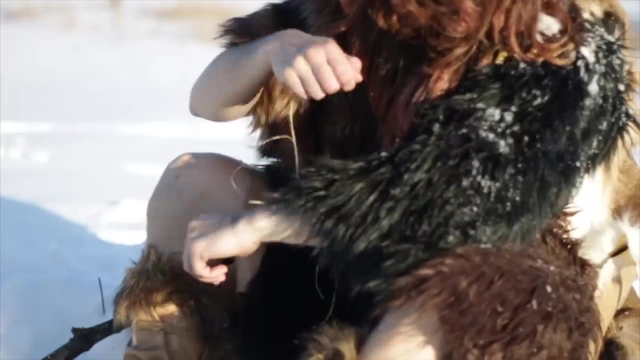 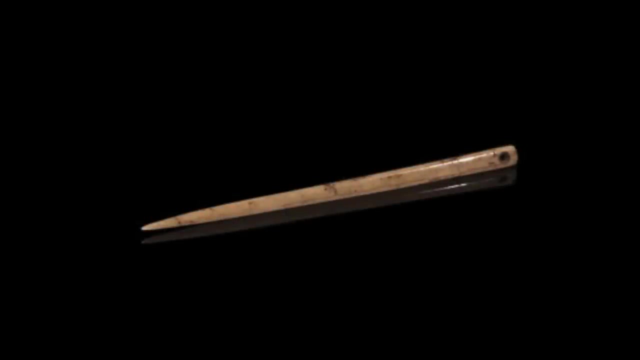 periods to survive. clothing did not necessarily have to be fitted, but it certainly would have helped. that brings us to a big question about neanderthal clothing. was it sewn together or simply draped around the body? to date, no eyed neanderthal needle has ever been found. 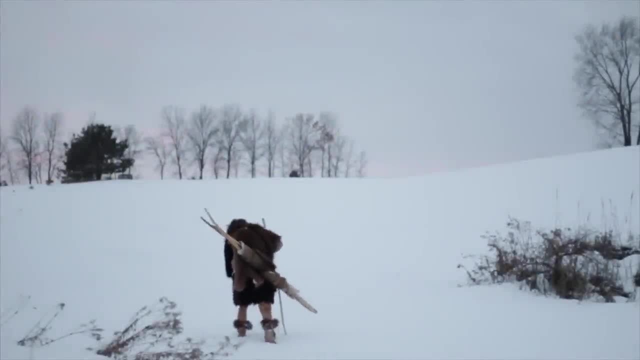 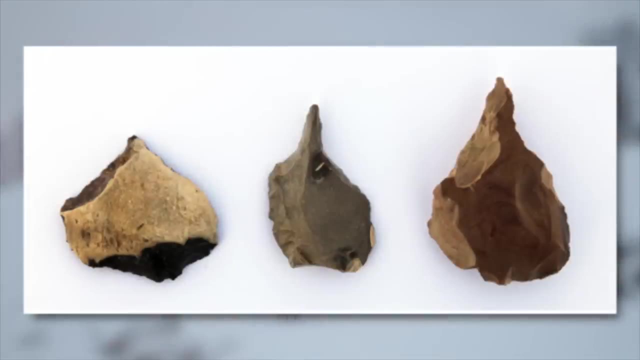 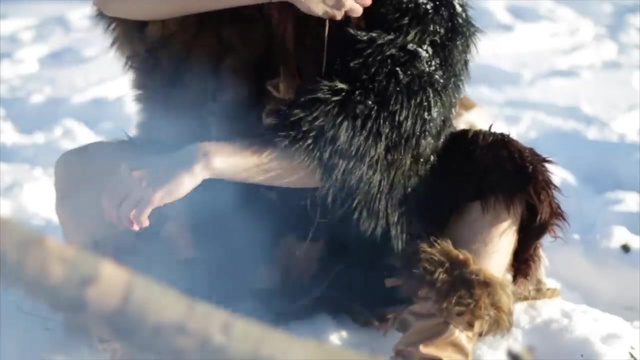 though. eyed needles are not essential for fitted clothing. all that is necessary is an awl and cord. awls could have been made of stone, bone or even wood. stone and bone objects found at neanderthal sites may have been used to make holes and hides. after a hole was made, cordage could 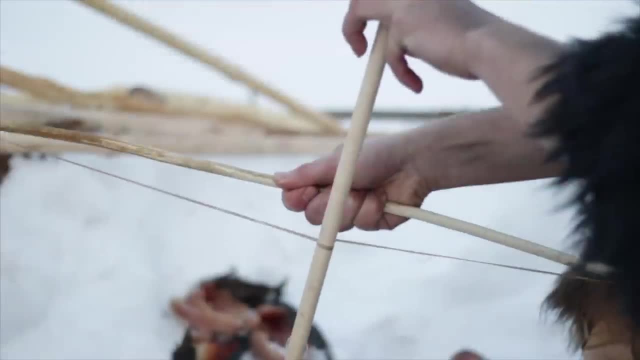 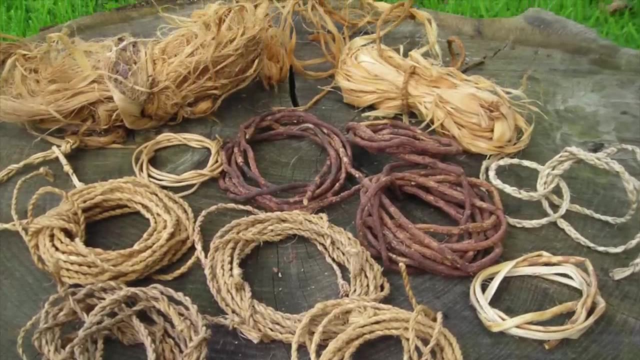 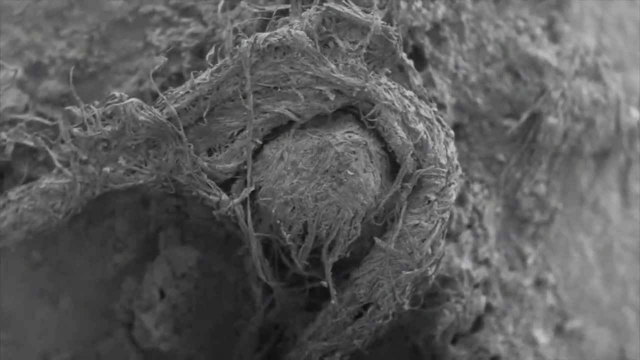 simply be pushed through. various materials could have been used for cordage. thin strips of hide, sinew and plant fibers would have all worked well. in france, there is evidence that plant fibers were being twisted into cord. around fifty thousand years ago. a small fragment was made of the inner bark of an evergreen tree. they were twisted to form a 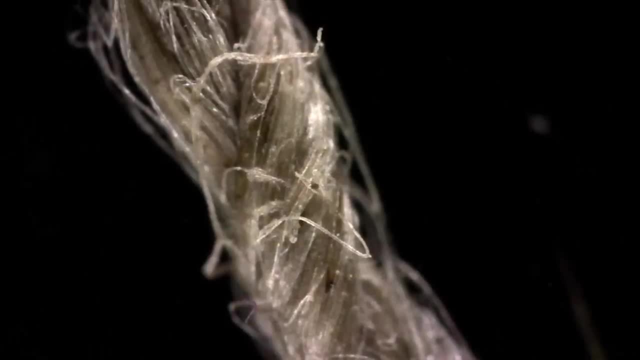 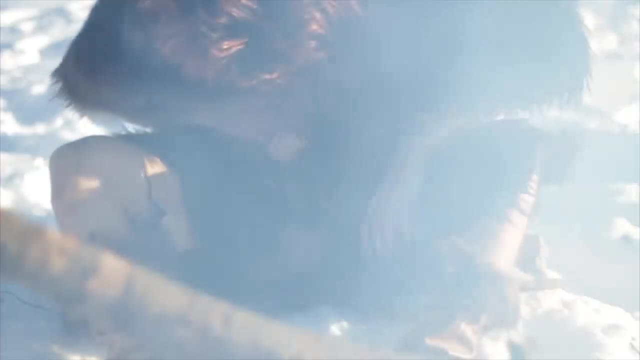 three-ply cord. this cord in particular does not appear to have been very strong, though it still would have been useful. it is unclear how widespread this technology was. considering that the materials are biodegradable and preserved very poorly, hides could have been stitched together to create fitted. 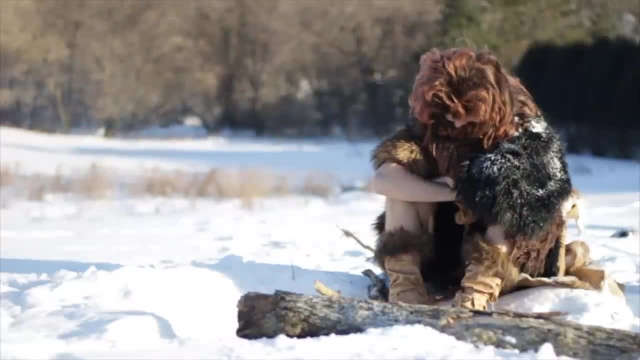 clothing. a set of neanderthal clothing, including an upper body, garment and leg coverings, would require around five large hides. a set of neanderthal clothing, including an upper body, garment and leg coverings, would require around five large hides. a set of neanderthal clothing, including an upper body, garment and leg coverings, would require around five large hides. 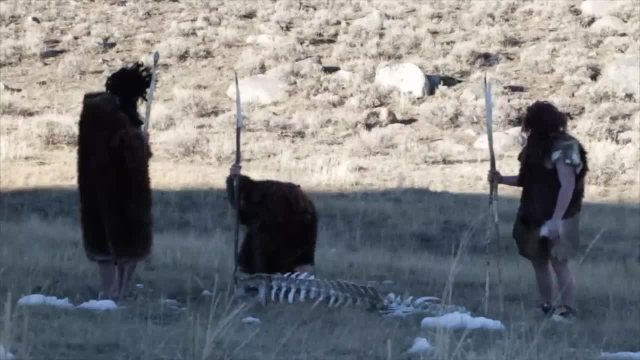 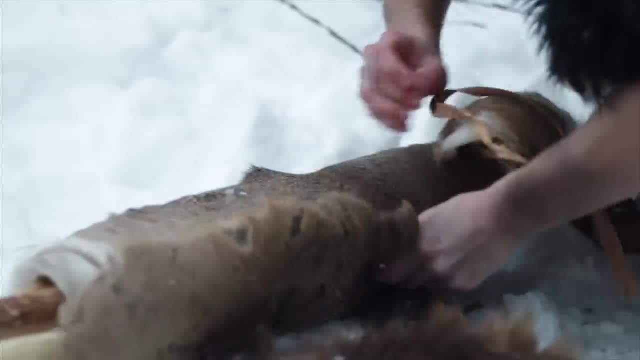 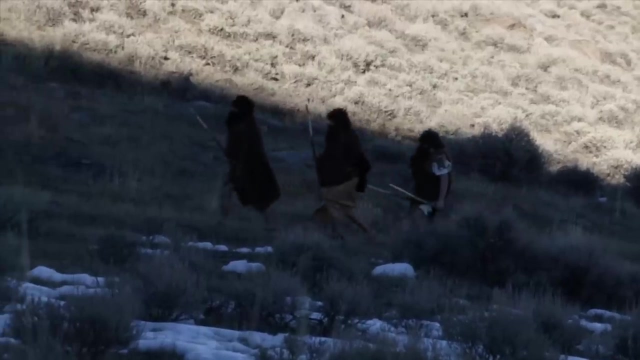 many animals would have been available. to make clothes out of their most common game of deer would have been an easy choice. but deer hair falls out of the hide quite easily. deer hides may have been made into buckskin for a variety of leather crafts and garments. specific hides were likely sought after for different garments because of their different 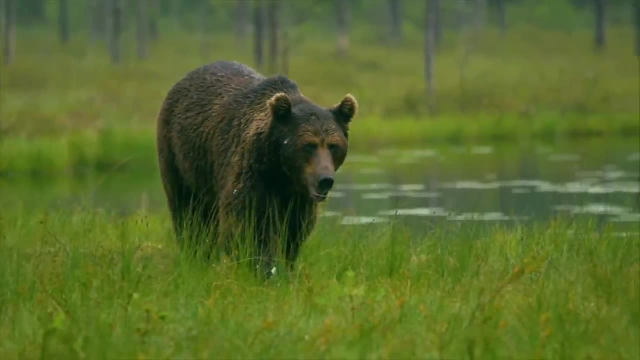 properties. thicker hides such as bear, bison and woolly rhino may have provided exceptionally warm. hides such as bear, bison and woolly rhino may have provided exceptionally warm skins. hides such as bear, bison and woolly rhino may have provided exceptionally warm skins. 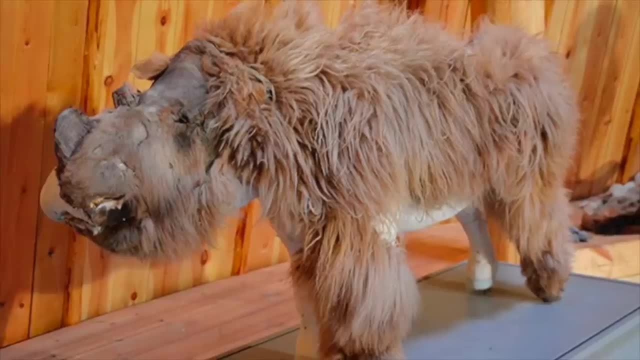 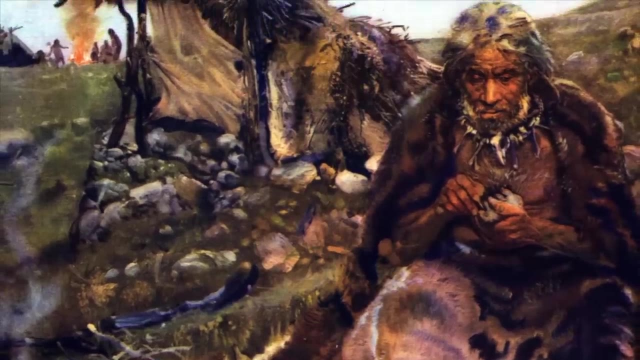 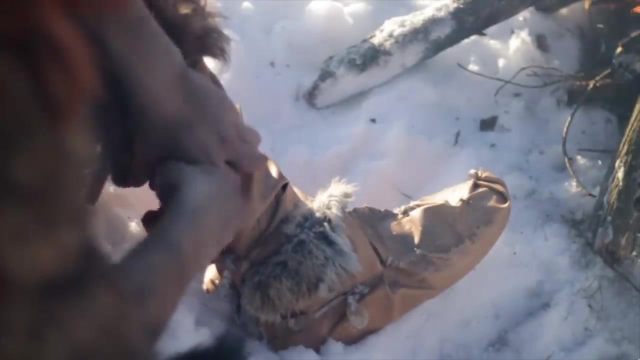 utilized for heavy coats, but some of these hides, such as woolly rhino or mammoth, may have been impractical for clothing. they may have been used as very heavy blankets or as walls for shelters. additional garments such as shoes, gloves or hats could have been made with trimmings or 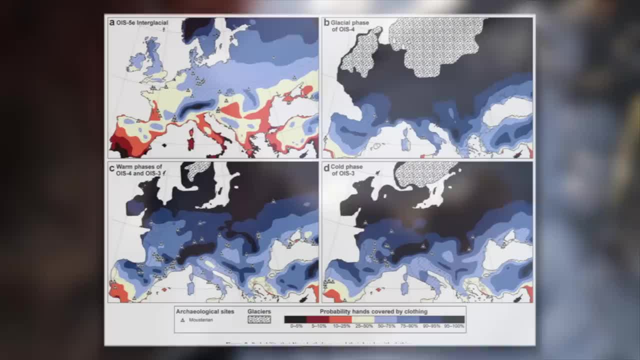 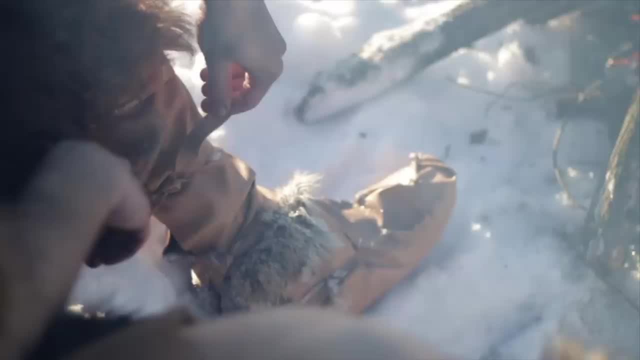 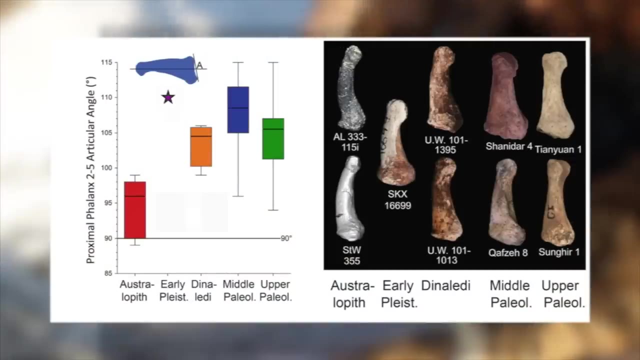 small sections of hides. shoes and hats would have only been worn in very cold periods. like contemporary hunter-gatherers, neanderthals would have had calloused feet, which would have not required shoes in most environments. an analysis of their feet and posture indicates that neanderthals did not wear hard-soled shoes. most surviving neanderthal footprints are from 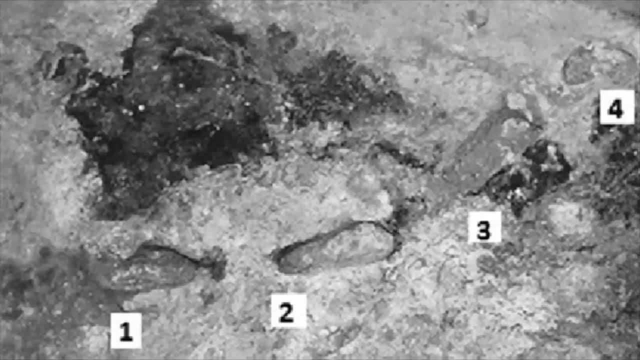 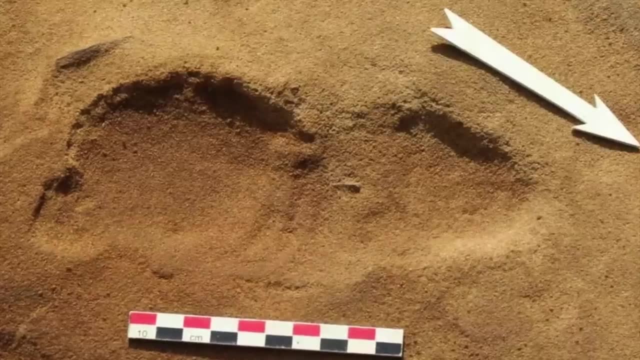 barefooted individuals, though at theopetra cave in greece, one footprint is barefooted, while the other two seem to have been covered with some sort of material. the print may support the hypothesis that simple foot coverings were worn, soft coverings made of. 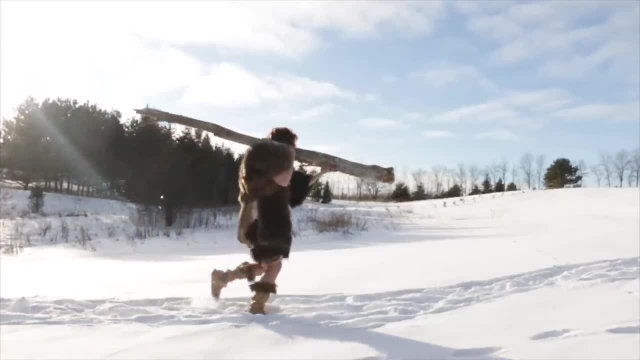 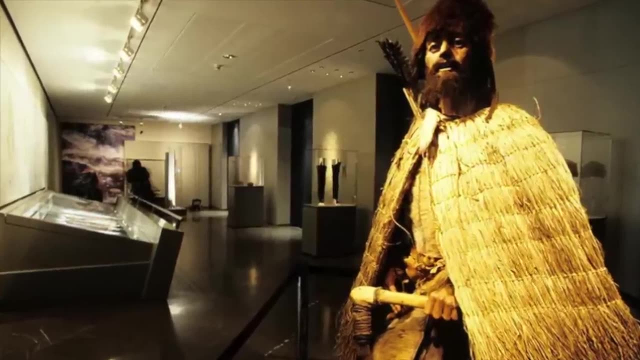 hide, or perhaps wood would have been used to cover the feet of the neanderthals if they had not been covered with hide, or perhaps woven grasses must have been used during the winter and especially in glacial periods. utzi the ice man was discovered with what has been interpreted as a grass cloak. 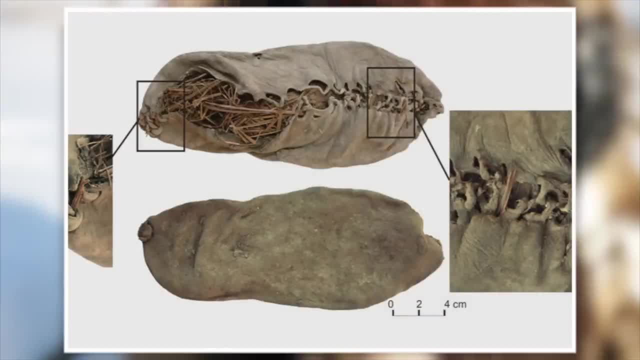 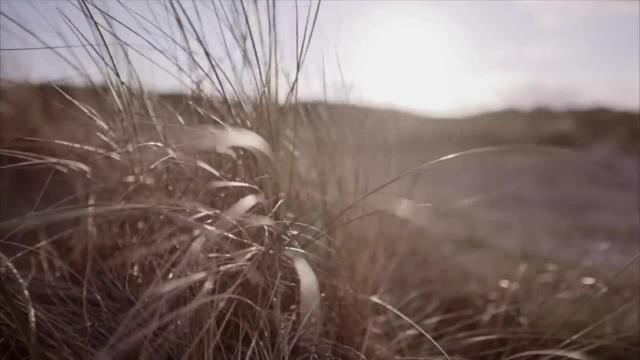 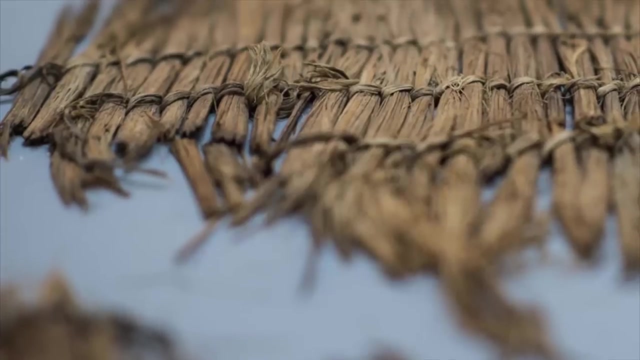 the oldest pair of shoes ever discovered were made of leather and grass, while the oldest sandals were made of sagebrush bark. it seems likely that some of their clothing and toolkit utilized grass. since we know that some neanderthals were able to create cordage, weaving is certainly not out of the question. 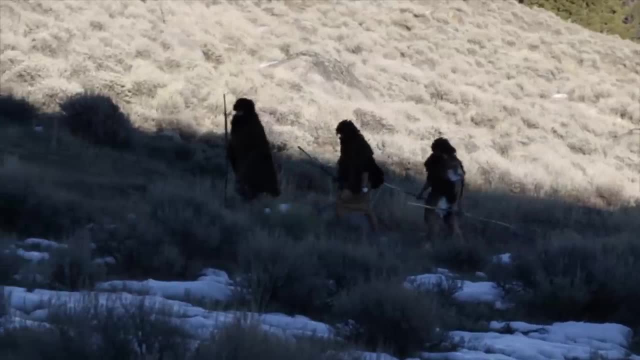 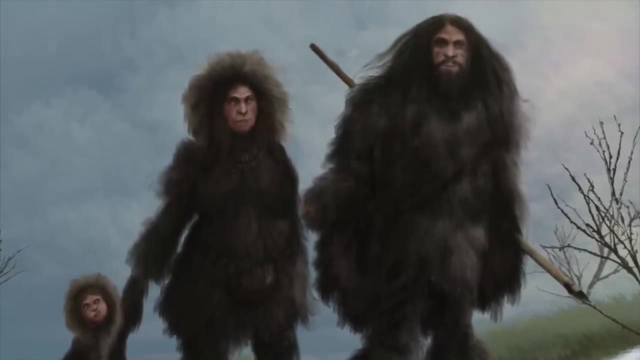 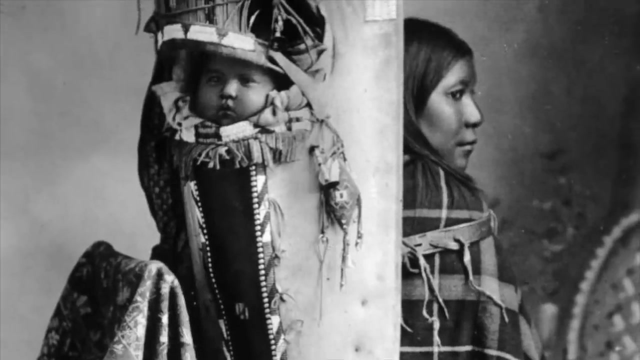 besides just clothing, hide and cordage technology would have had many other uses. warm fur pouches for carrying infants would have been essential for cold winters. babies may have been strapped to the back of neanderthal mothers as seen in inuit and native american cradle boards. fur bags and pouches would have been very useful for. 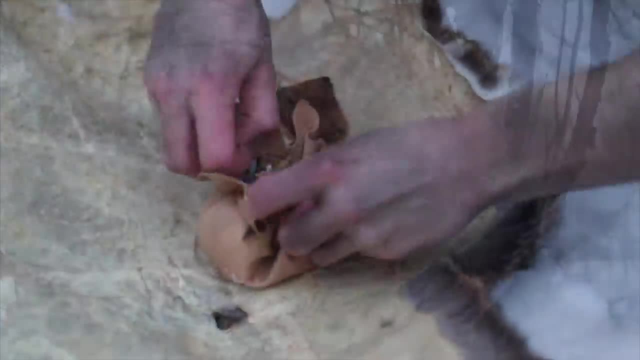 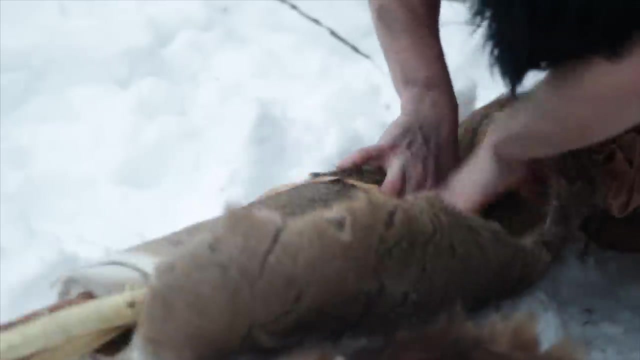 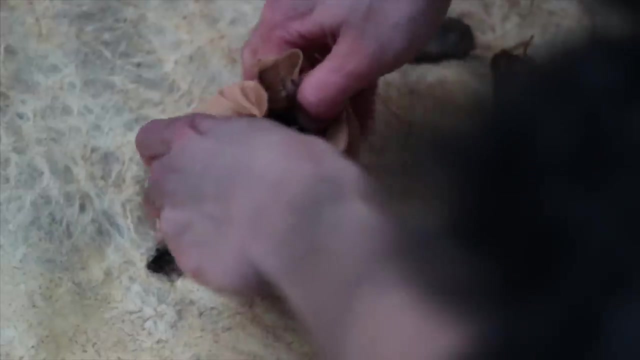 carrying around the neanderthal's toolkit. neanderthals were highly nomadic and carried everything with them in addition. hives, weapons, flint, knapping tools, stone, dried meat, bedding, fire making materials and more bags made of animal skins or stomachs would have been essential limb extremities. 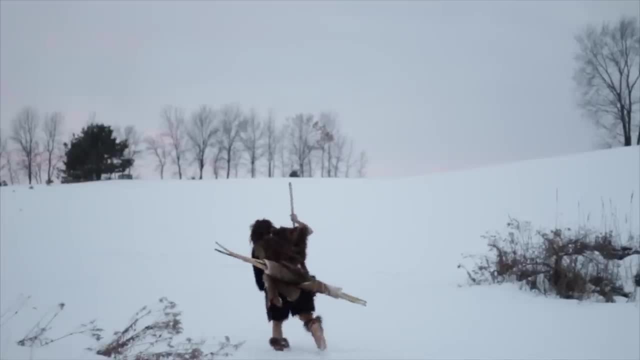 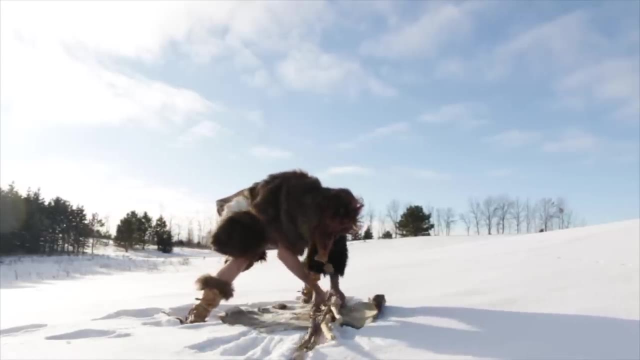 left on hides could have functioned as shoulder straps or handles. other uses of hides includes bedding and shelter. hide is a very versatile material that neanderthals certainly exploited. it was one of the many materials that neanderthals could use to keep their kids from the cold winter. 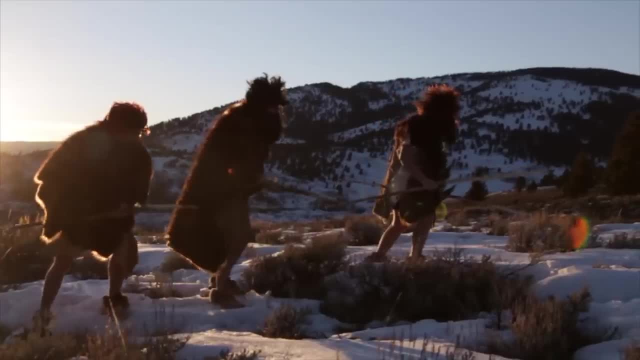 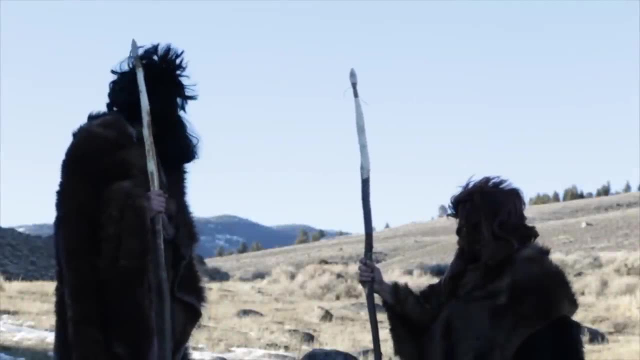 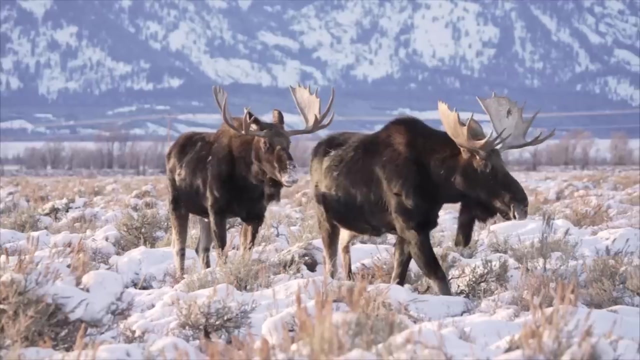 utilized, made of animal products, products that can only be procured with the death of an animal. Hunting was certainly one of their main forms to obtain sustenance and raw materials Across their vast range, both spatially and temporally, many different kinds of animals. 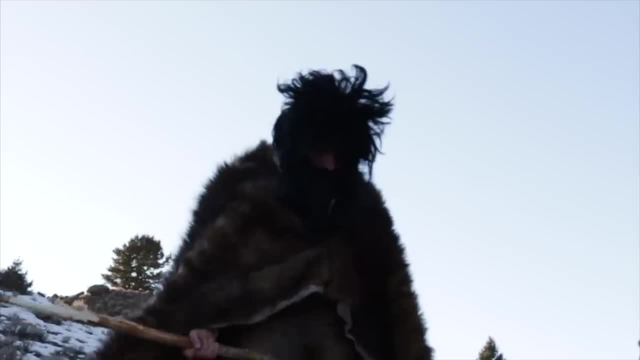 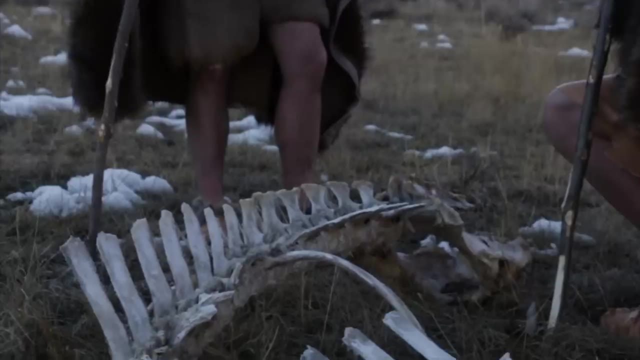 would have been hunted in many different ways. Their technology, wear on their lithics and damage to the bones of their prey can allow us to understand how hunting may have been done. Like mentioned earlier, much of their technology was focused on creating wooden implements. 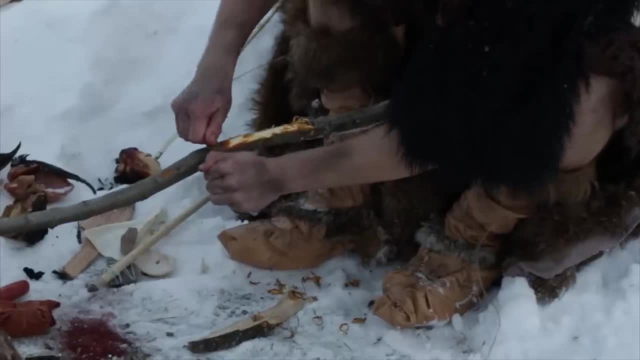 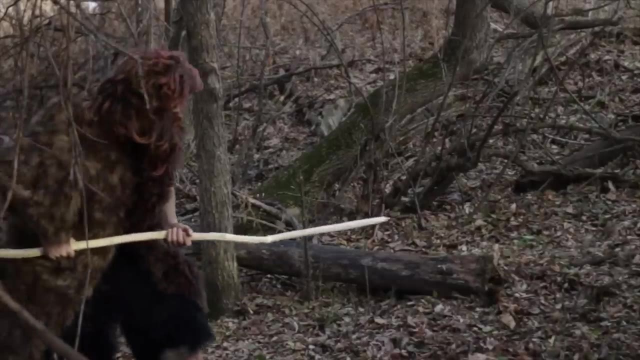 As seen at the Schönegan site, throwing javelins and thrusting spears were being created even early on in Neanderthal existence. Even a relatively simple wooden spear would have been a formidable weapon in the hands of a Neanderthal. 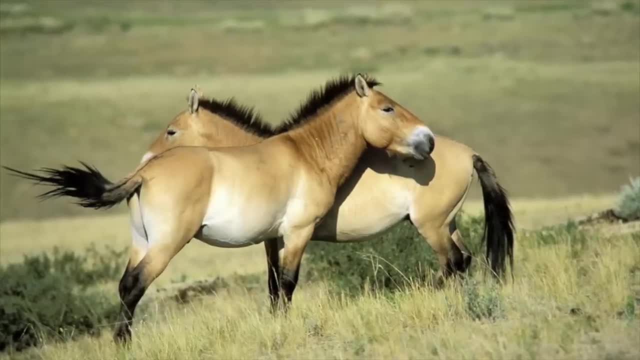 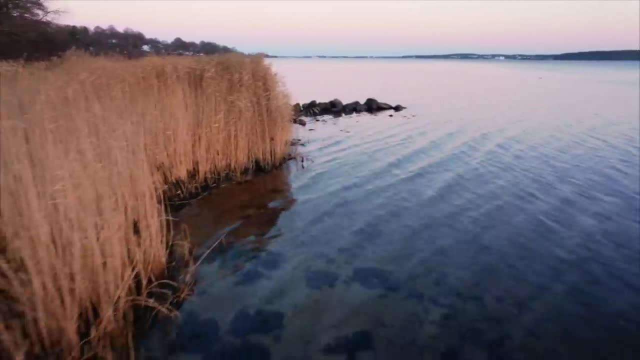 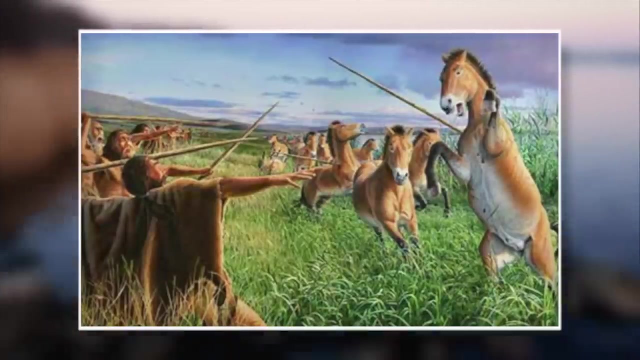 The large horses found at the Schönegan site weighed over 500 kilograms or 1100 pounds. The site is located on an ancient lakeshore where Neanderthal hunters likely ambushed their prey. It was originally interpreted as a mass killing event, but later discoveries found that the 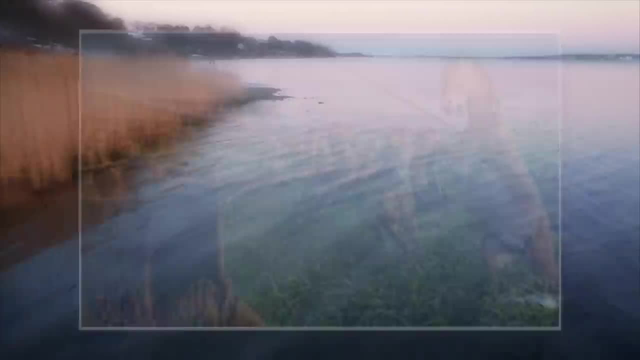 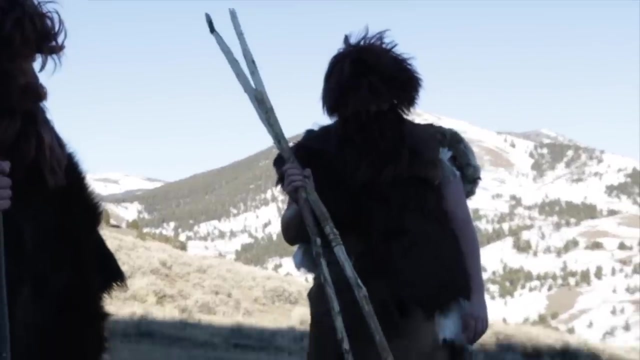 horses were hunted in separate seasons. The hunters likely herded horses towards the lake, where they were less mobile and easier to ambush. The ability to kill such large animals with such simple tools is a testament to their hunting ability, Which likely included pre-planning and an extensive knowledge of hunting. 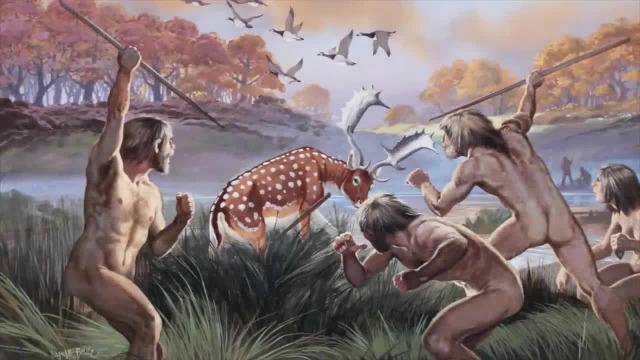 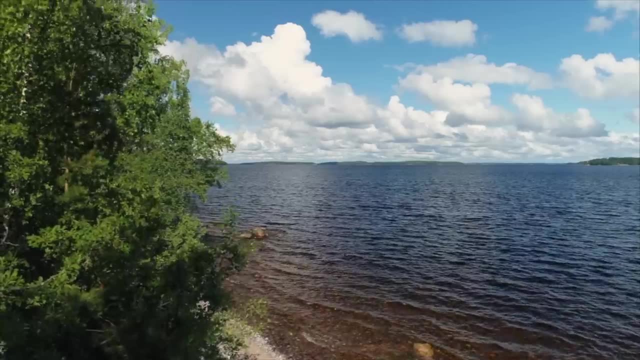 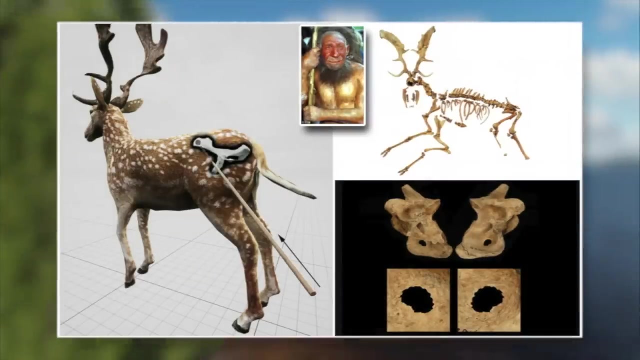 A very similar site, which also consists of an ancient lakeshore in Germany, preserves the remains of over 100 fallow deer. Out of the mostly prime-aged individuals, two different individuals have puncture wounds present on a hip and neck bone. 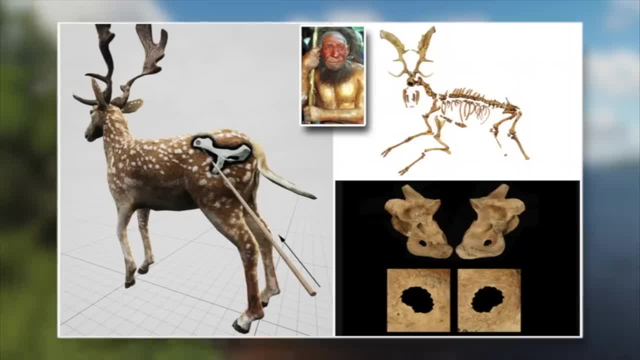 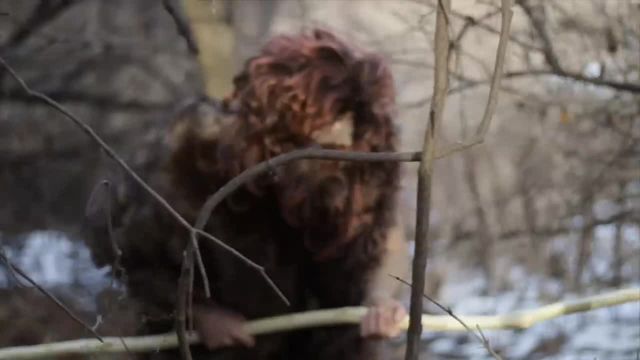 These wounds are consistent with a low-velocity thrust, likely underhanded. Getting within thrusting range of an agile deer is no easy task. These hunters would have had to conceal themselves in the middle of the lake to avoid the threat of a fallow deer. 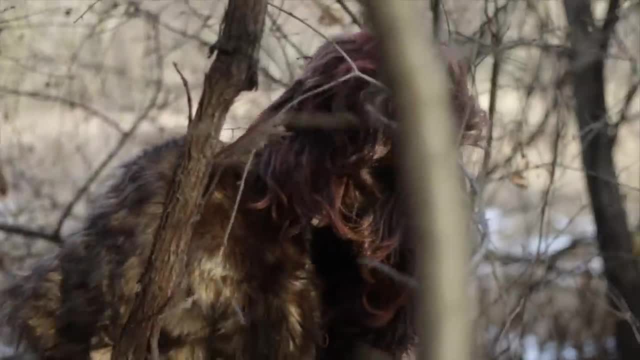 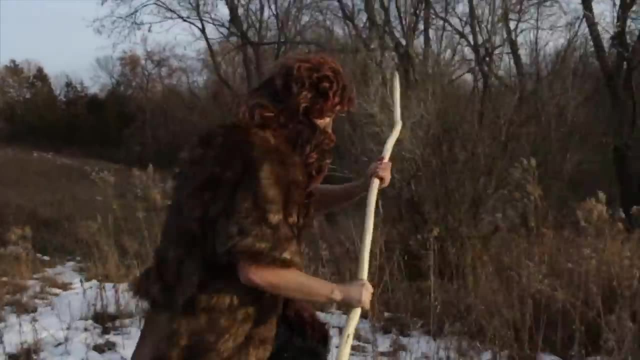 They would have had to keep their distance from the deer for hours and hours. while coordinating with multiple individuals, The powerful Neanderthal anatomy would have allowed for quick and powerful bursts of speed that would have aided them in ambushing unsuspecting prey. Though only two of the deer at the site have direct evidence of puncture wounds, it is 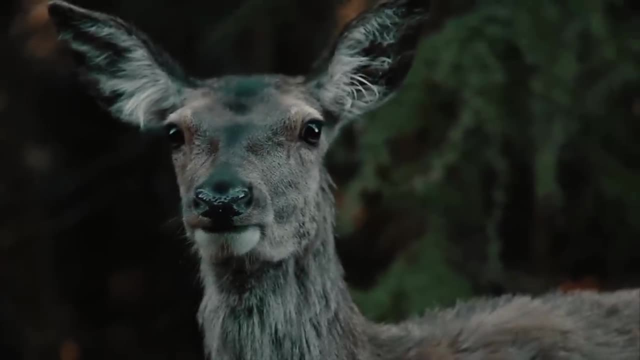 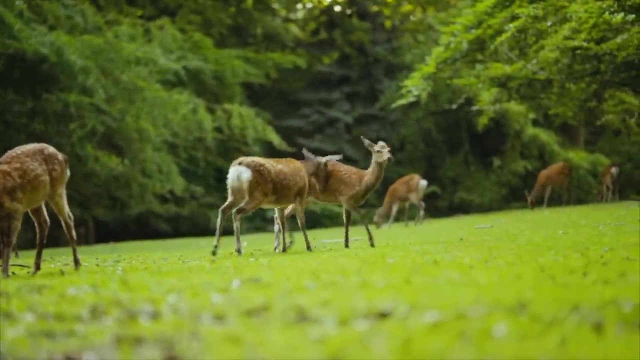 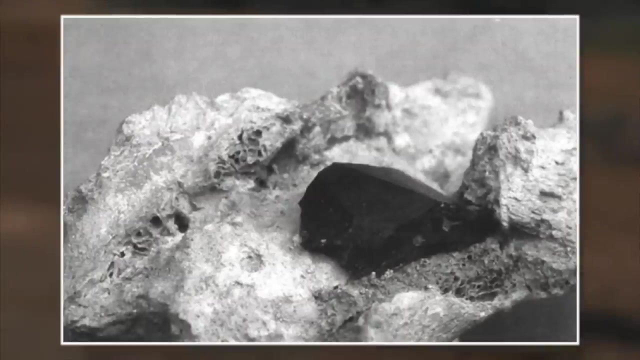 likely that most, if not all, of them were hunted. telling by the context of the site, Many wounds such as a punctured lung would not necessarily be evident in their skeleton. Other wounds are highly evident. The vertebrae of an African wild ass from Syria has a fragment of a Levallois point. 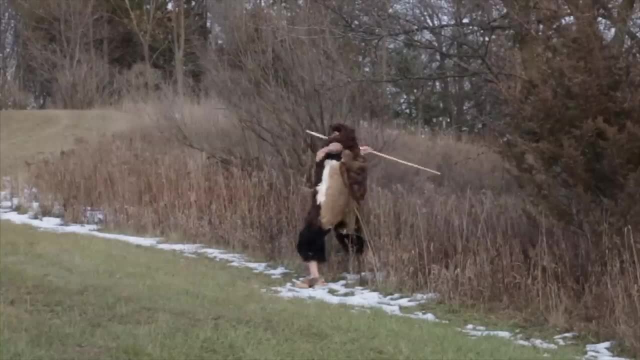 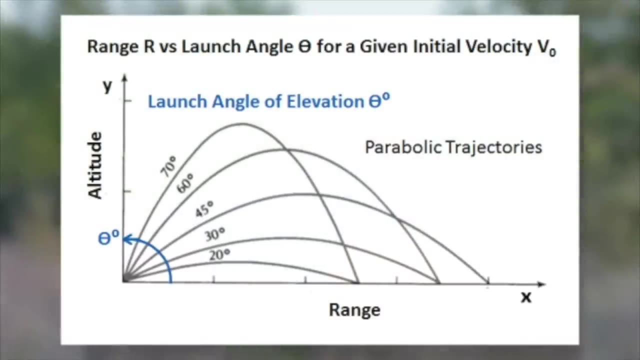 embedded in it. The fragment impacted the animal with a high degree of kinetic energy. If the animal was struck while standing, the trajectory of the weapon must have been parabolic. The high kinetic energy and parabolic trajectory suggest that this weapon was thrown rather. 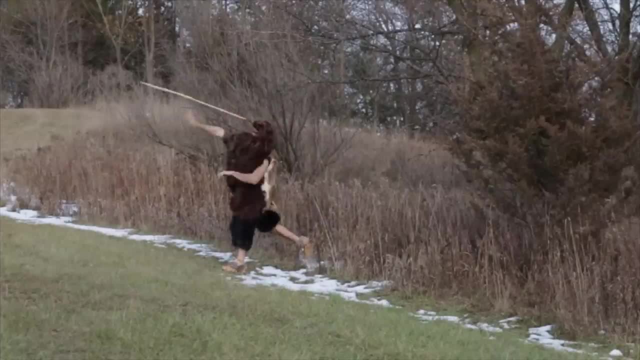 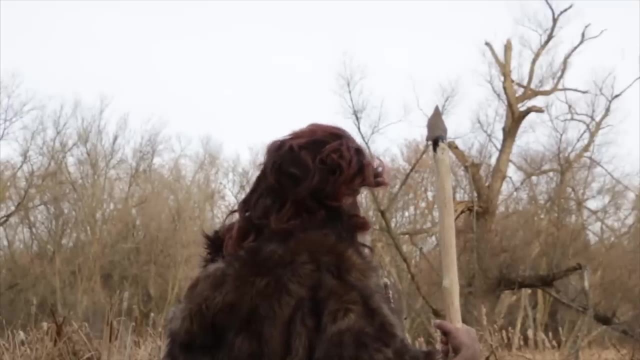 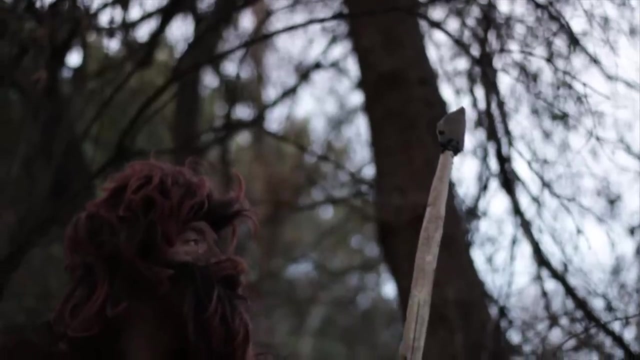 than thrusted. This wound would have caused immediate paralysis of the limbs and likely a quick death. This example overturns the idea that Levallois points hafted on spears were only used as thrusting spears. Still, these spears would have been quite heavy and would have only been thrown short. 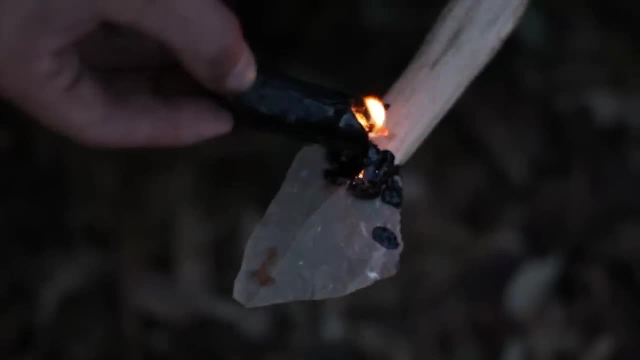 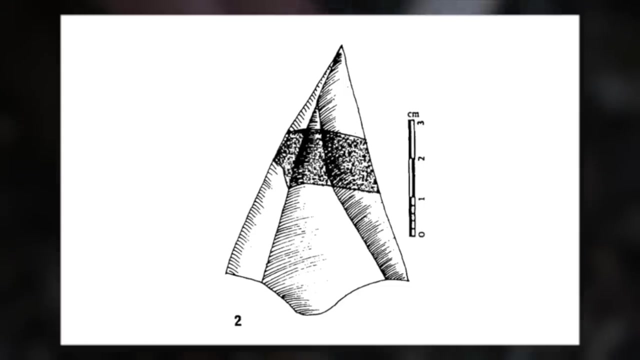 distances. Whether thrown or thrusted, the weapons would have created massive flesh wounds. The fragment found in this particular vertebrae already had a broken tip before impacting the donkey's neck. This may indicate that it was used multiple times in the same hunt or that it was used 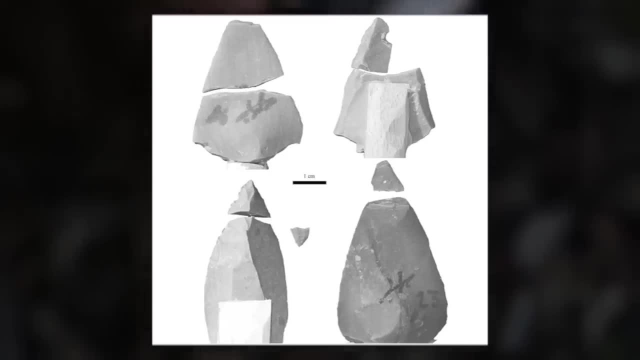 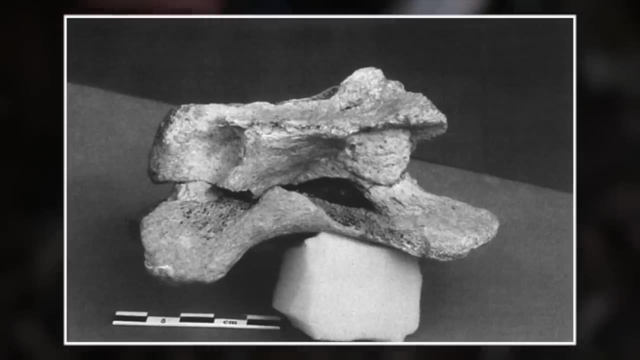 for the same purpose. However, it is unlikely that it was used for the same purpose. It may also indicate that it was damaged from a prior hunt. Whatever the case, even with a broken tip, it was able to deliver a fatal wound. 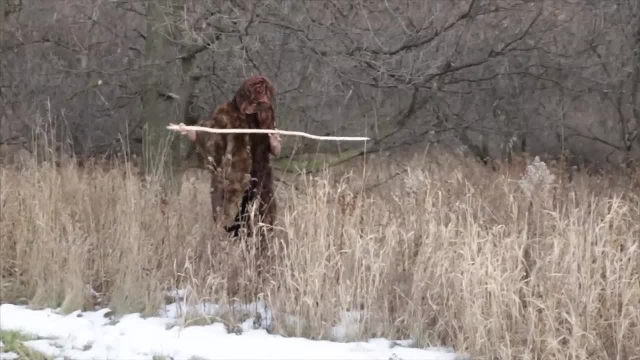 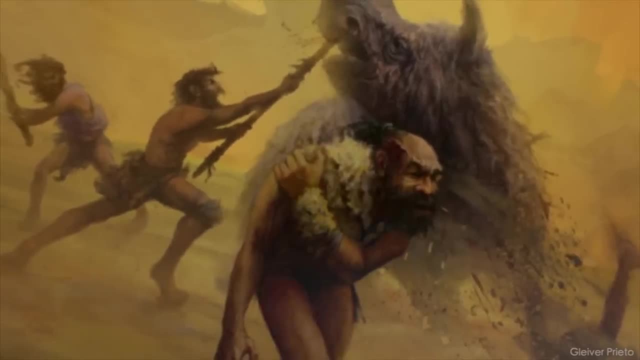 Though some of this evidence may make it seem like Neanderthals primarily threw their spears, in reality thrusting was more common. We know this based on artifacts, but also by the fact that 79-94% of our Neanderthal specimens 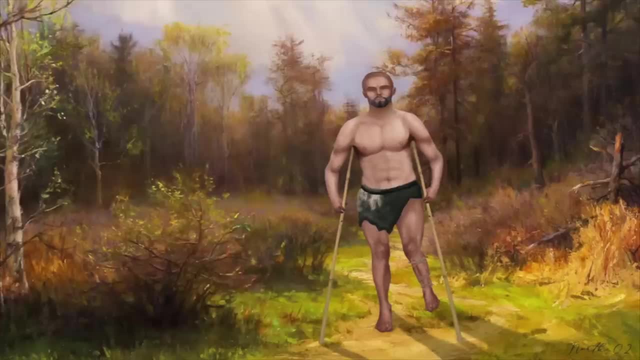 show evidence of healed major trauma. Up to 50% of Neanderthals were injured throughout their lifetimes. We know this based on artifacts, but also by the fact that 79-94% of our Neanderthal specimens show evidence of healed major trauma. 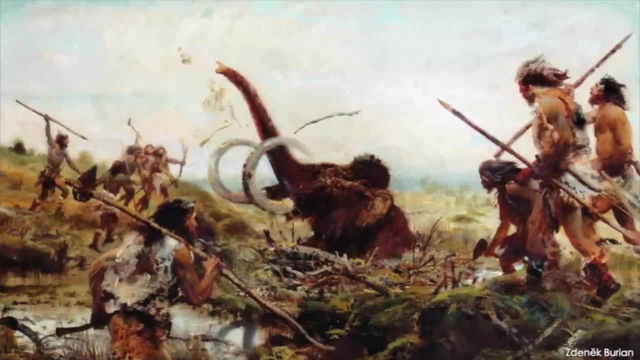 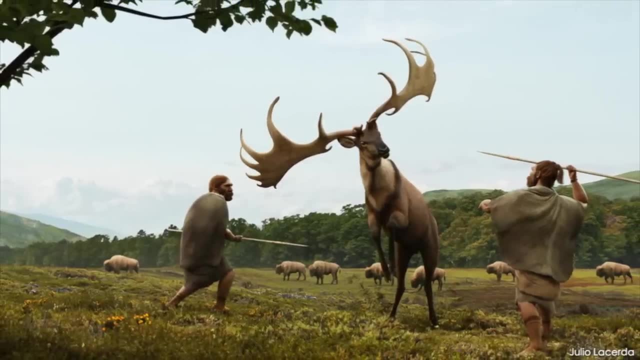 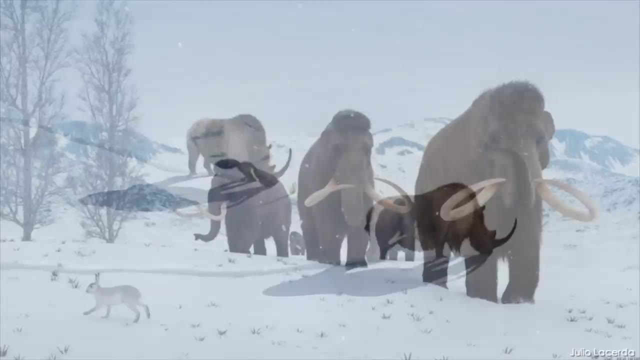 Confrontations with large dangerous game is generally the explanation for such a high injury rate. Even game not typically seen as dangerous, such as deer, can cause life-threatening injuries at close range. Very large animals such as moose, woolly, rhino and mammoth would have been very deadly. 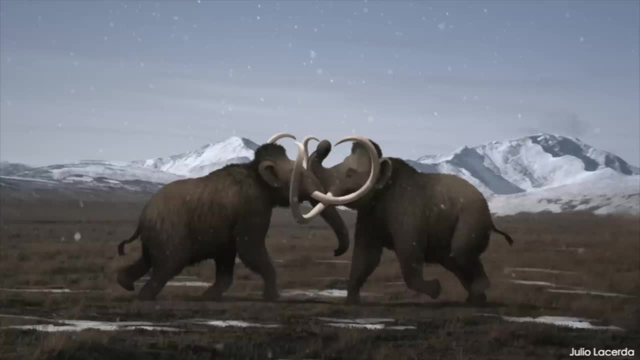 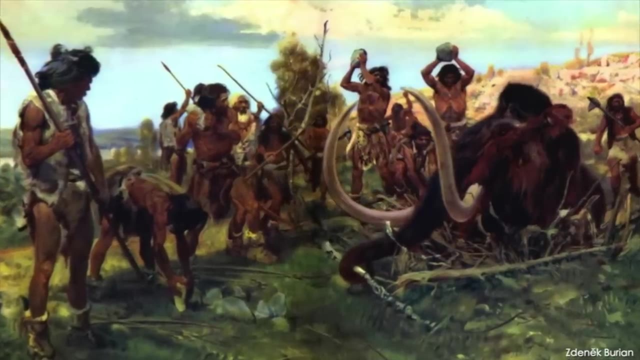 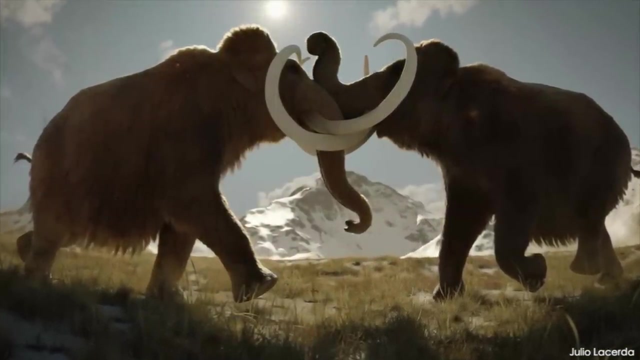 Due to the risk of hunting these animals and their pure bulk, some question whether hunting them would have even been possible In place of seeing Eurasia, there lived both the woolly mammoth and the straight-tussed elephant. Woolly mammoth were around the same size of modern elephants, while the straight-tussed 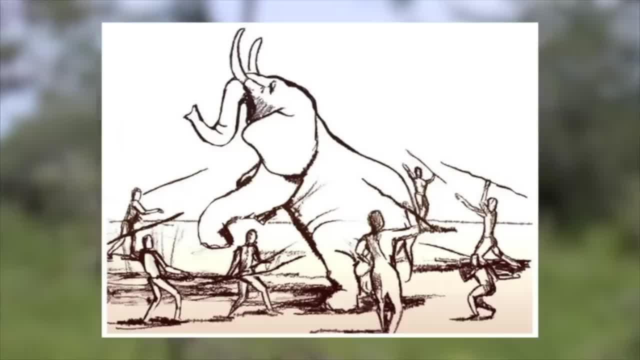 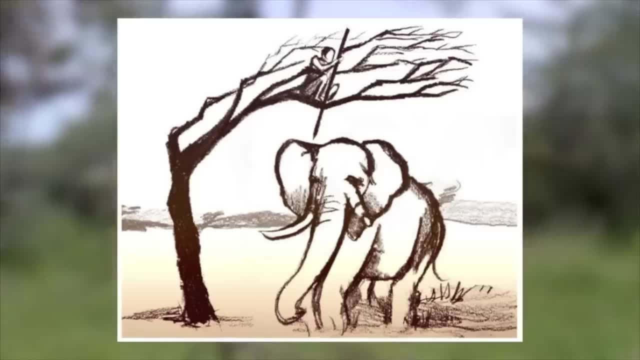 elephant was much larger. Recent contemporary hunter-gatherer populations in Africa have been known to take down adult elephants with only spears. In some cases, a singular hunter was able to sneak beneath an elephant before it was able to take it down. In some cases, a singular hunter was able to sneak beneath an elephant before it was. 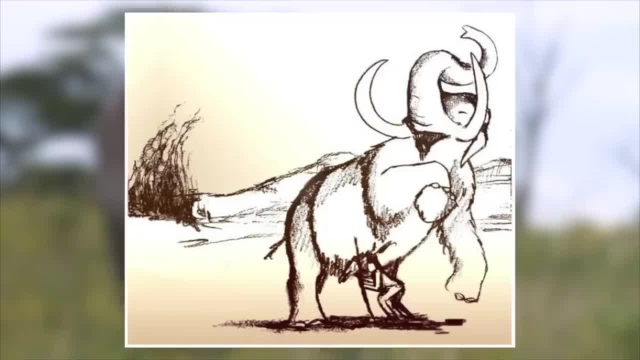 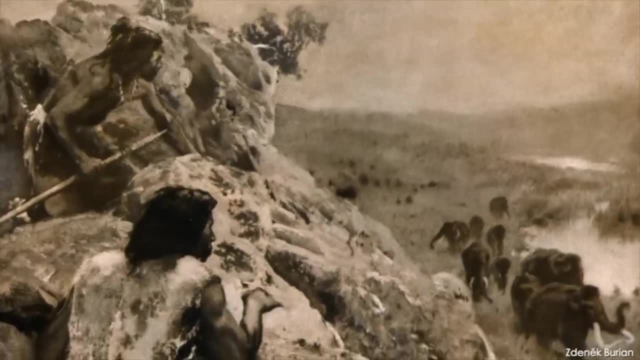 able to take it down. Some have even been said to have been able to take down elephants with spears. Because of the fact that mammoths and elephants were known throughout many neanderthal sites, it is certainly possible that some of these individuals were actively hunted. 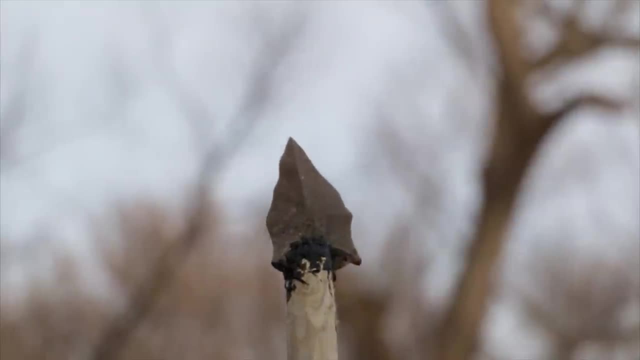 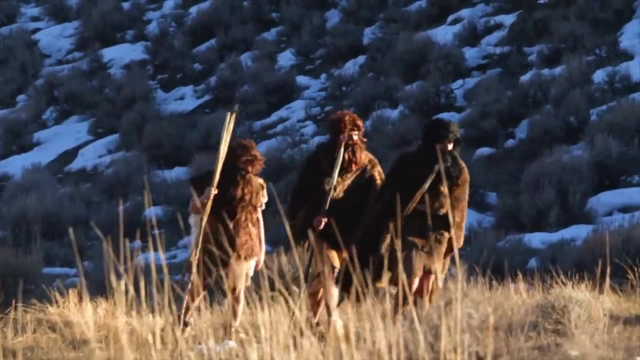 When taking into account the wide razor-sharp edges of a La Valois point in tandem with a heavy shaft, the idea of a group of neanderthals taking down a mammoth or elephant seems much more plausible. Perhaps mature mammoths were only hunted in times of scarcity or difficulty. 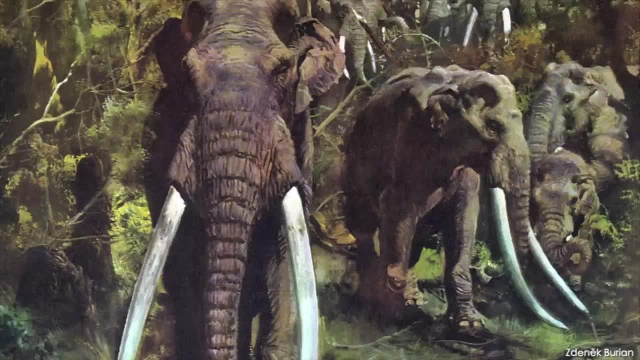 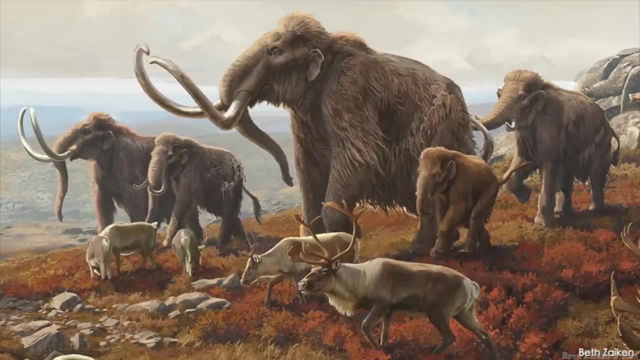 However, the number of mammoths in the world is small: scarcity or perhaps before winter, though it can be said that they were not relied upon or were the usual prey of most Neanderthals, Though young mammoths and elephants may have been preyed on. 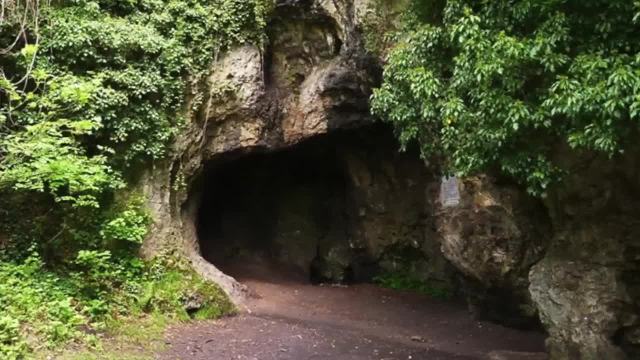 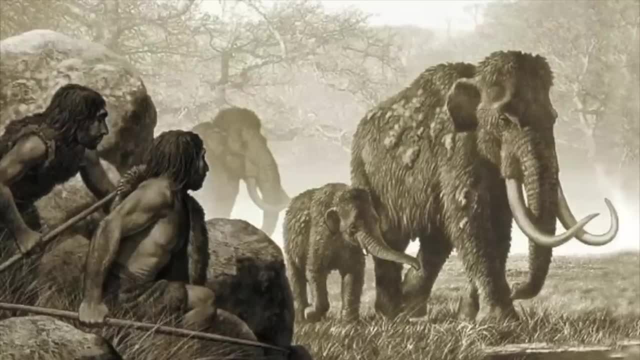 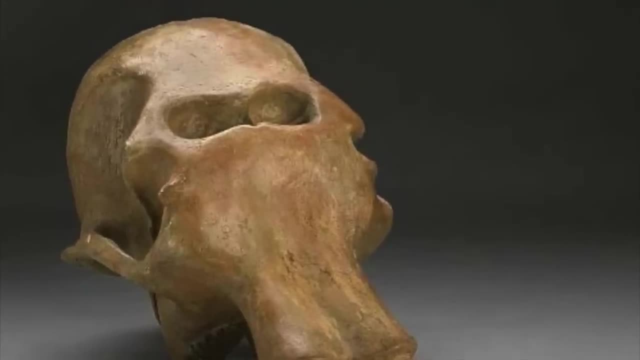 much more often. A fascinating site in Belgium called Spy Cave has evidence that Neanderthals preyed upon young mammoths. The site has many interesting remains, but the mammoth remains are peculiar. There is an abnormally high frequency of young mammoth skulls. In a very interesting paper 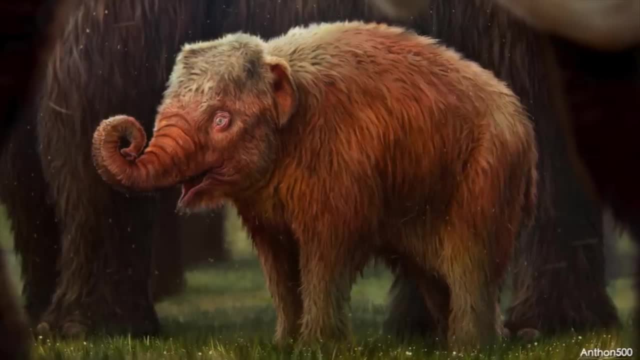 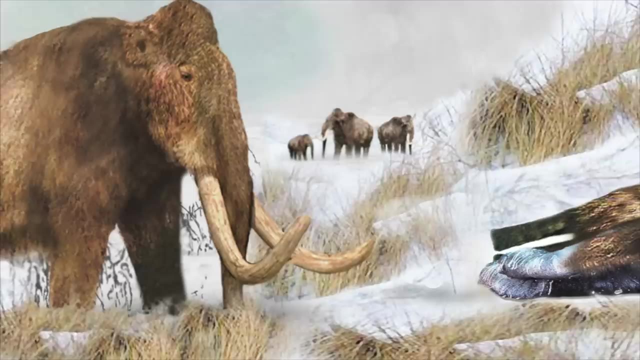 it is hypothesized, young mammoths were targeted by these Neanderthals for their brain matter. The brains of young mammoths provided essential long-chain fatty acids. It was found that Neanderthals were less efficient than some modern humans at creating. 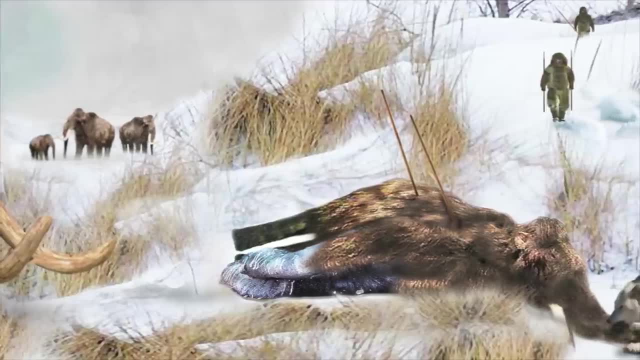 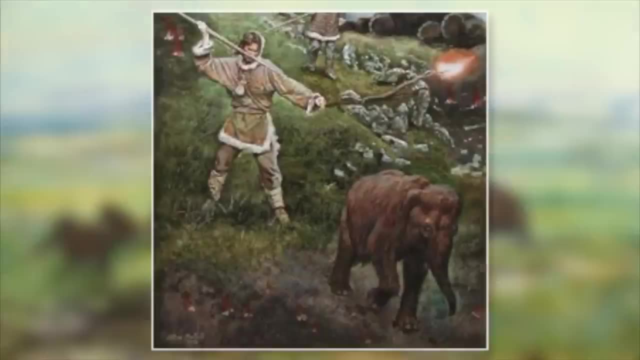 these fatty acids, which are very important for neural growth. Mammal brain tissue is one of the richest sources of fatty acids in the world. It is believed that the body of a mammoth is the source of these long-chain fatty acids, Therefore eating these mammoth brains actually. 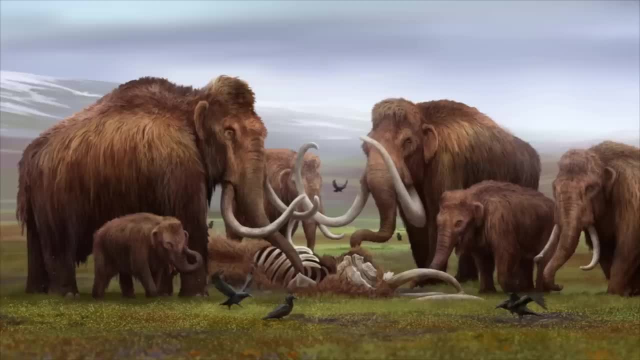 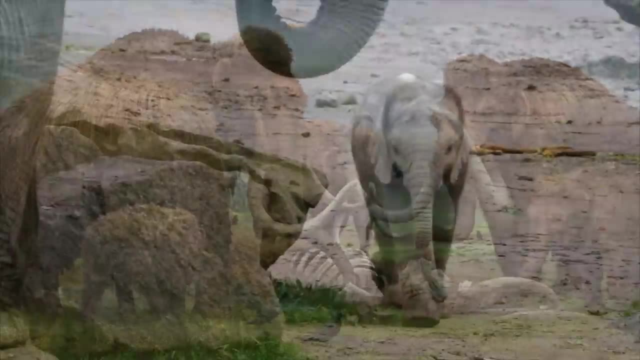 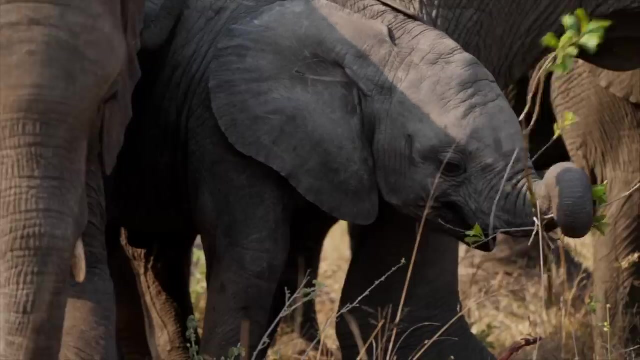 helped them in their own brain development. Another interesting thing about baby mammoths or elephants is that they are not naturally afraid of humans. Young elephant calves have no instinctive fear of humans and are known to attach themselves to them. It is possible that 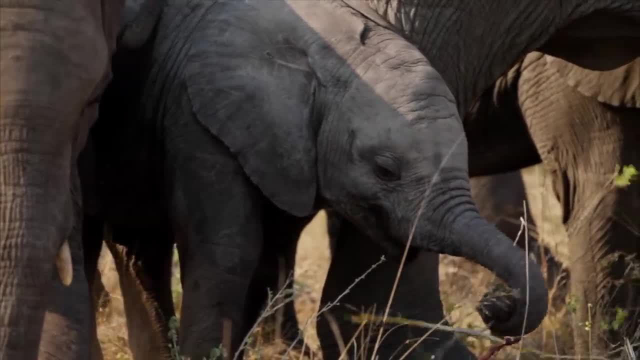 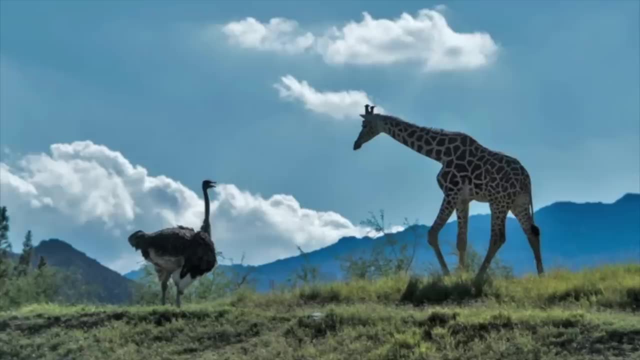 baby proboscideans were even kept as some kind of pets in rare instances, Though we would assume that these people would have just hunted a helpless animal mercilessly. even relatively unintelligent animals are known to form strange bonds with animals that they may typically see as prey. 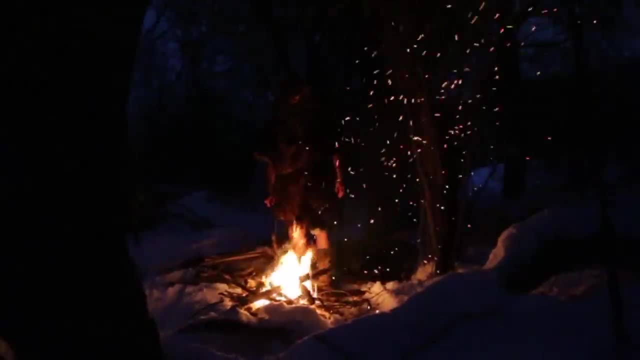 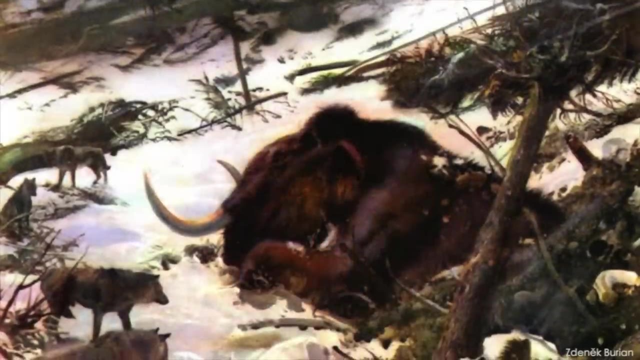 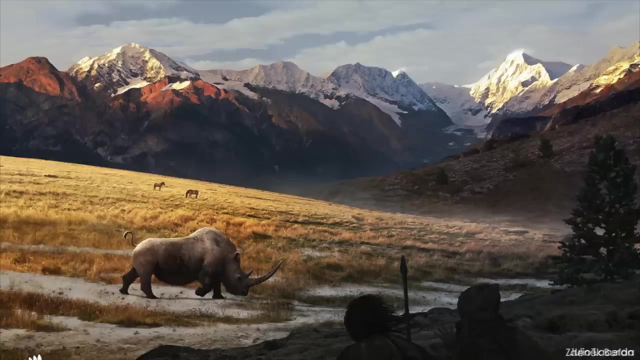 It is not out of the question that a group of Neanderthals, well-off with food, may befriend a young mammoth to possibly eat later or even just as a pet. Besides proboscideans, other very large animals were hunted. Multiple rhino species called to your up home, The woolly rhino weighed. 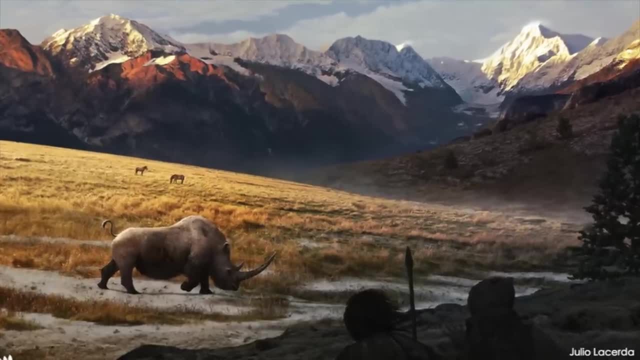 around 3,000 kilograms and weighed about 1,000 kilograms. The baby proboscideans were also found to weigh around 3,000 kilograms or 6,600 pounds. Merck's rhinoceros and the narrow-nosed 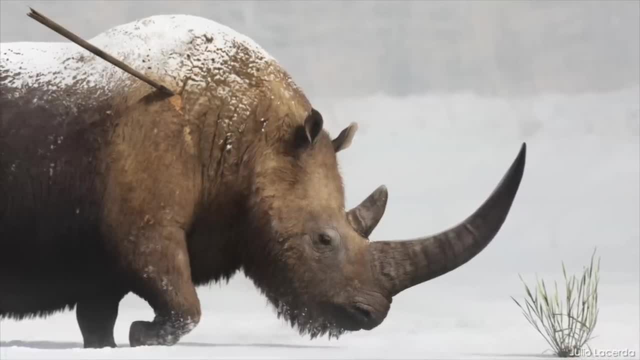 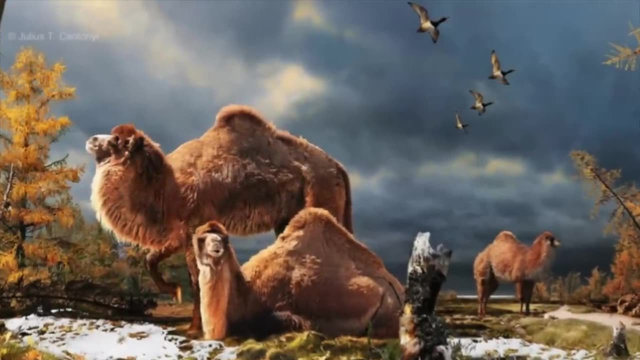 rhinoceros. both weighed around 1,800 kilograms or 4,000 pounds, At around half the weight. Camelus noblaki was much taller, at 3 meters or 10 feet. The aurochs, the undomesticated ancestor of cattle weighed as much as 1,500 kilograms or 3,300 pounds. Megaloceras was a giant species of deer with the largest antlers. They were also found to weigh about 3,000 kilograms or 6,600 pounds. 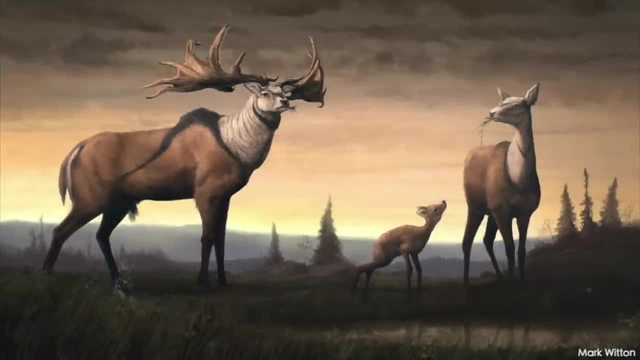 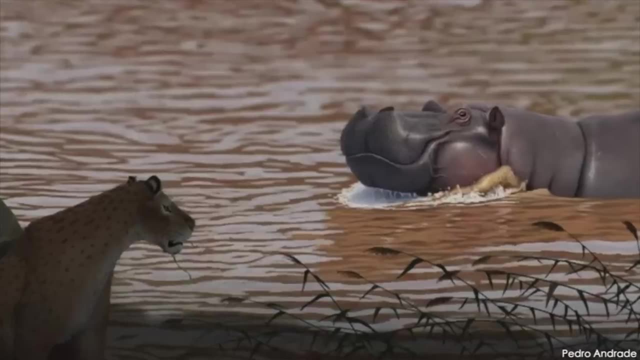 The hippopotamus. a species of hippopotamus, was also found to weigh about 3,000 kilograms or 6,100 pounds. They weighed as much as 700 kilograms or 1,500 pounds, and would have certainly been a sight to see. During interglacials, hippopotamus moved all the way up into central Europe. 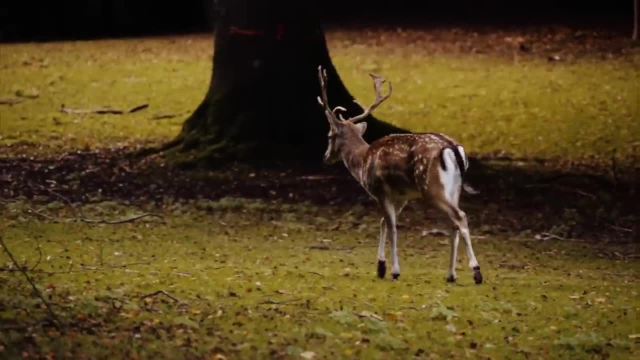 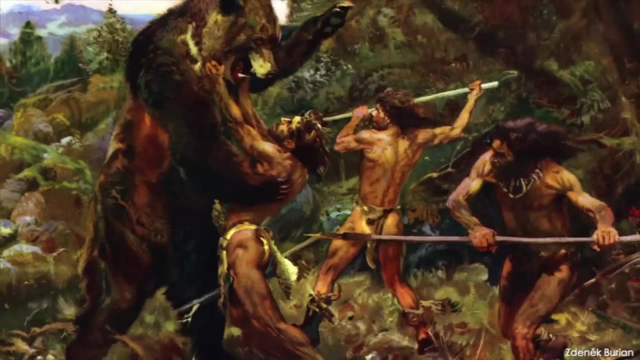 Extinct species such as red deer, reindeer, ibex, moose and bison were all hunted. Carnivores also seemed to have been hunted. There was evidence of direct brown and cave bear hunting in and out of hibernation. Bear are not an easy animal. 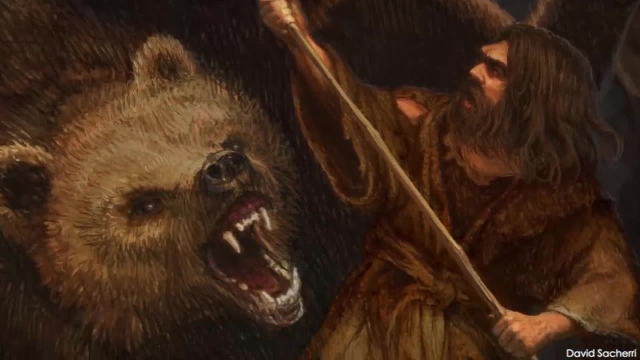 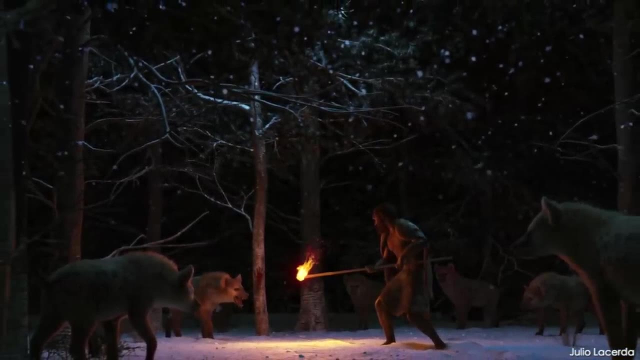 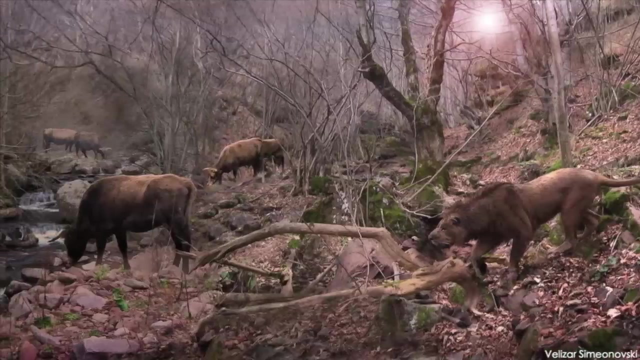 but they become much more vulnerable when hibernating. Other large predators, such as cave lions, cave hyenas and wolves, would evolve in prey occasionally. All of these animals would technically be considered megafauna. Megafauna are just animals that weigh over 45 kilograms or 100. 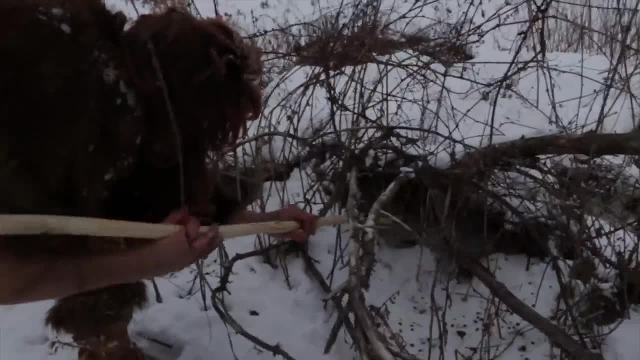 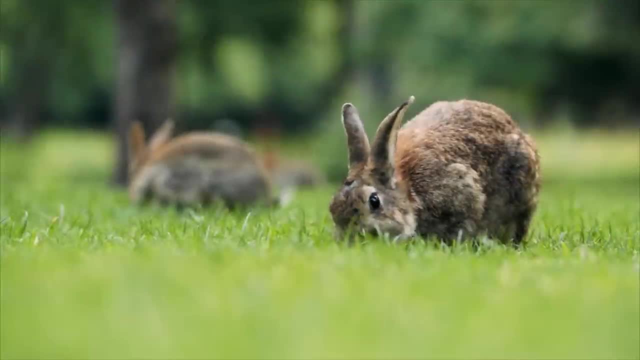 pounds, But Neanderthals hunted a much larger variety of prey. Smaller animals such as birds, small mammals and reptiles were also hunted. Small animals such as birds, small mammals and reptiles were hunted more than we once thought. Because these animals are smaller, their remains do not. 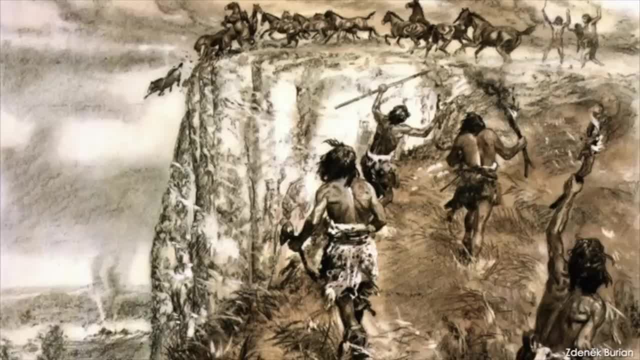 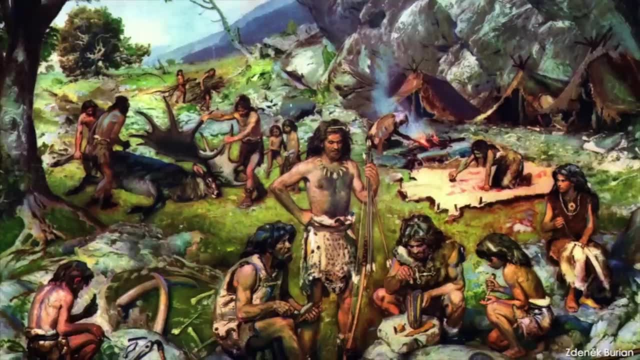 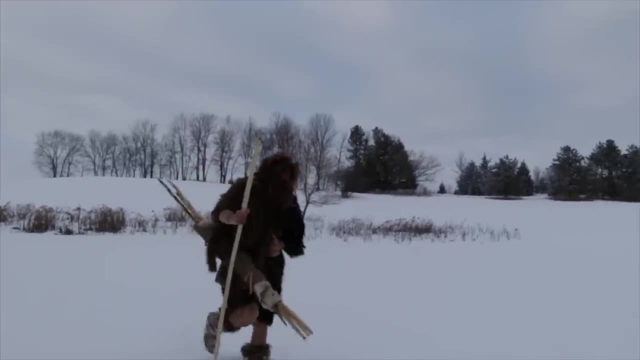 tend to preserve as well in the fossil record Due to this, preservation bias made us think that Neanderthals only hunted large game. We even thought that homo sapiens may have out-competed them because they had an over-specialized diet. However, recent evidence has suggested otherwise. 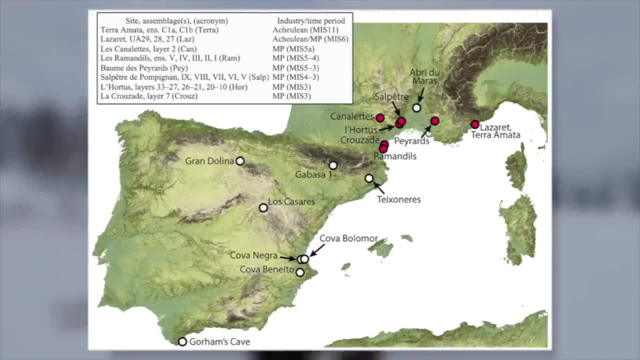 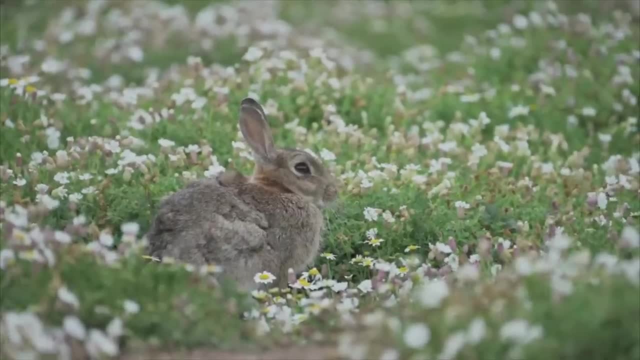 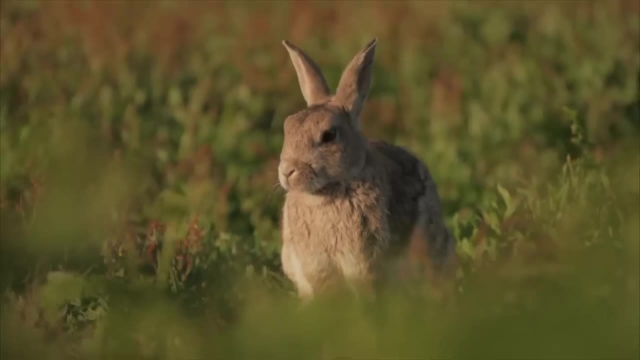 A team led by paleoanthropologist Eugene Morin examined the fossil rabbit remains from eight Mediterranean sites. What they found was that most of the rabbit remains were adults. This suggests that they were not targeting the rabbit's homes, but instead hunting them individually. Rabbits do not provide very many calories and were likely only a snack. 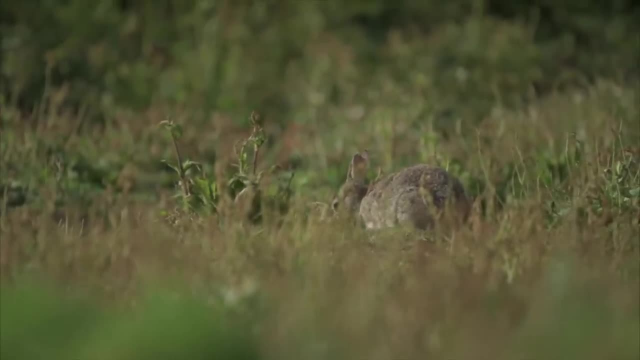 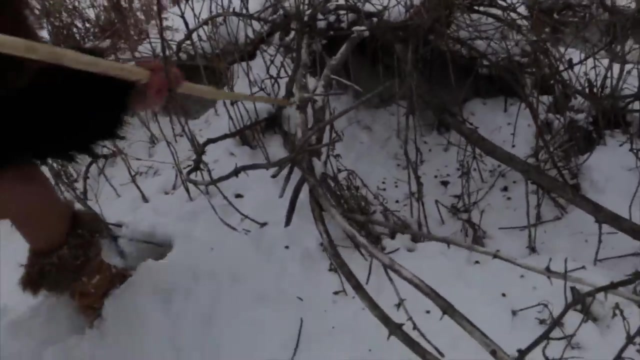 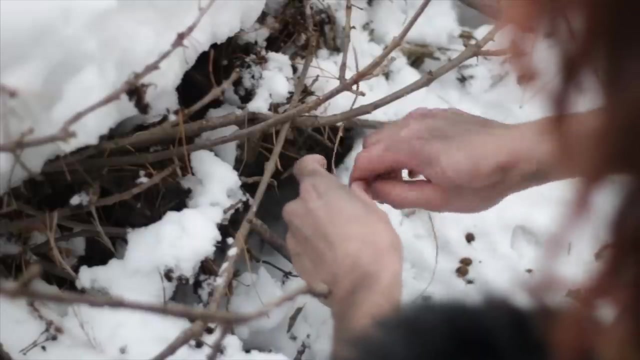 but the fact that Neanderthals were able to catch these animals is interesting. Rabbits are extremely difficult to catch by hand and are also hard to hunt with traditional weapons. Throwing sticks may have been used, but traps are generally more effective. Neanderthals were certainly cognitively advanced enough to create 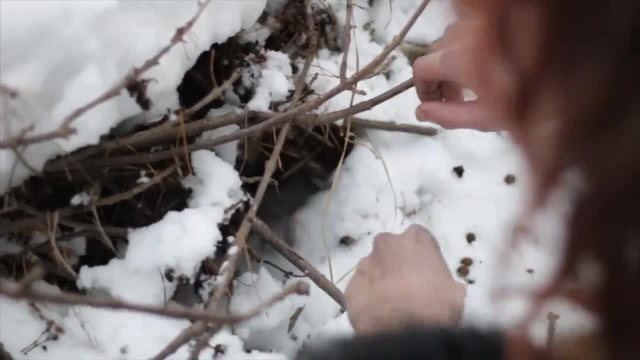 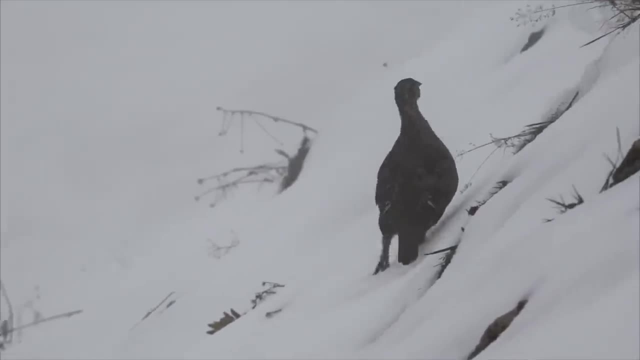 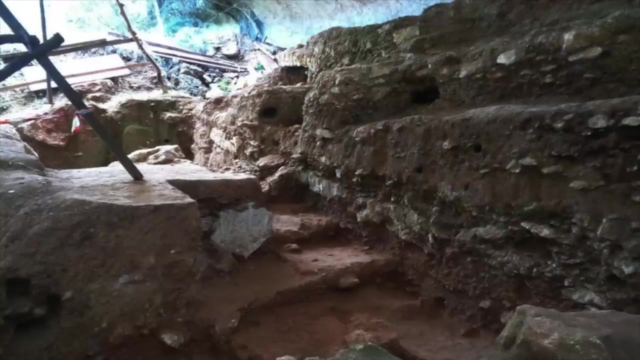 a variety of traps- Small game very well- may have been caught with snares or deadfalls. The high rate of bird remains at their sites raise a number of questions regarding how they procured them. Birds are another animal that could have been caught with traps. The high rate of bird. 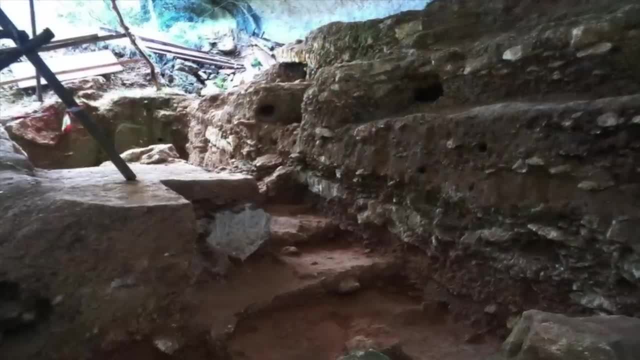 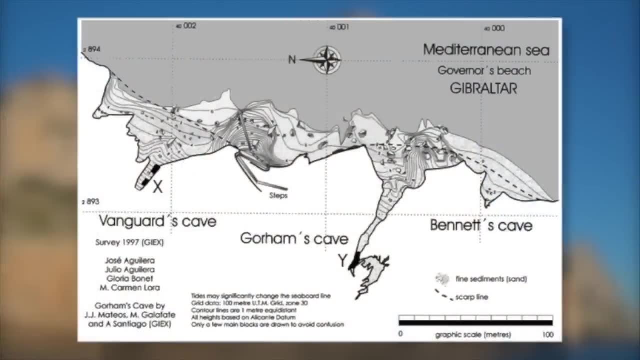 remains at their sites raise a number of questions regarding how they procured them. At sites in Gibraltar, Neanderthals were more likely to be caught with snares or deadfalls than with rabbits. The remains of 143 different bird species have been found, including ground dwelling species and. 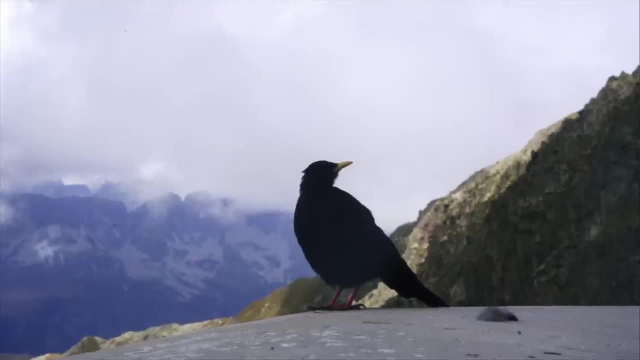 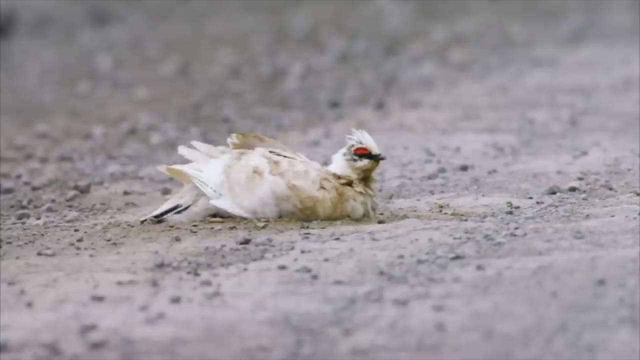 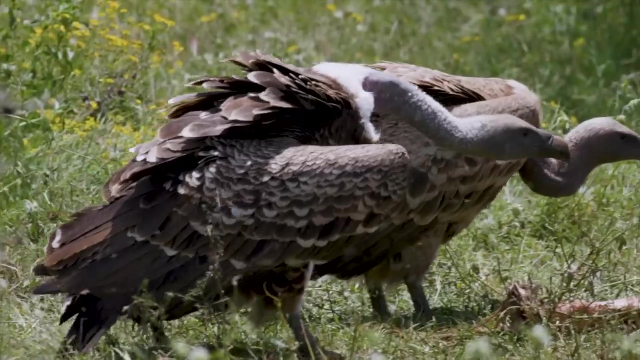 even eagles and vultures. Some bird species, such as joes, nest in caves at night and can be easily caught by hand. Ground dwelling bird species such as grouse or quail could have been taken with throwing sticks, plain old rocks or even traps. Birds of prey would have frequented carcasses. 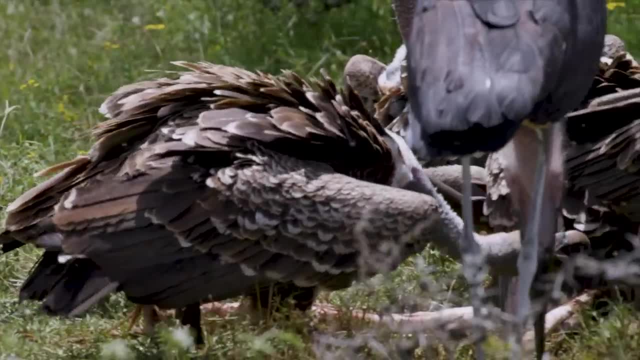 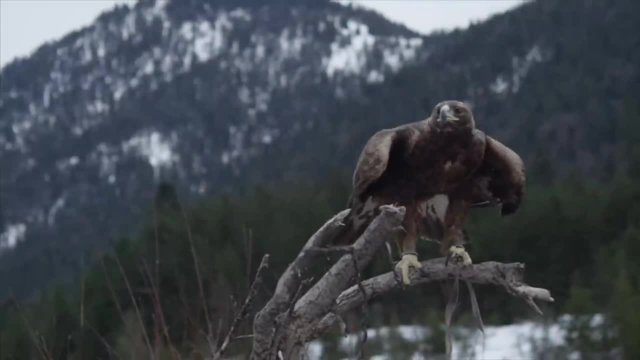 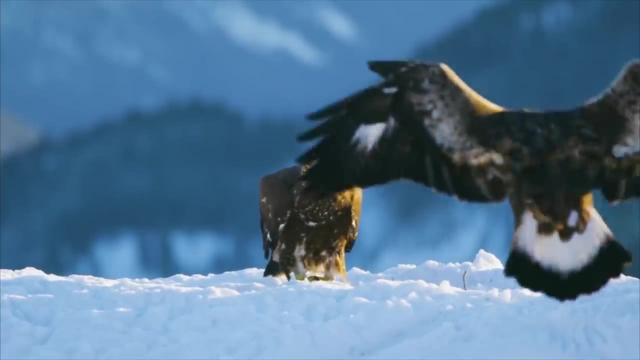 which would have made them vulnerable to being taken by a projectile. these birds are extremely intelligent and have extremely keen senses. It would have been very difficult to sneak up on them and even more difficult to actually kill them, Though the unusually high rate of eagle remains at Neanderthal sites and strange modifications to their bones. 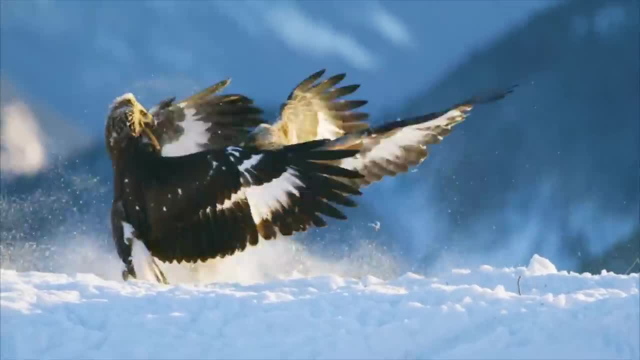 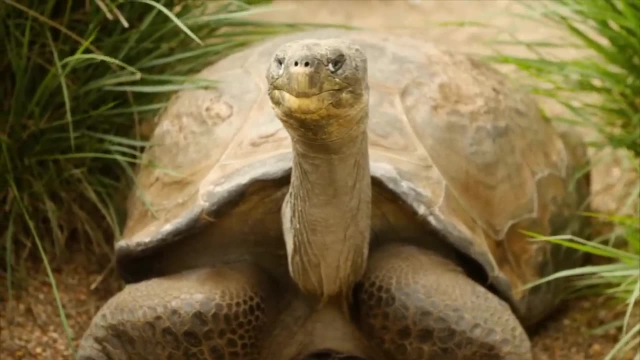 suggest that eagles may have had a symbolic meaning in their culture. Another food source were reptiles. The remains of at least 20 butchered tortoises have been found at Bolimar Cave in Spain. Tortoises from the region became significantly smaller over time. 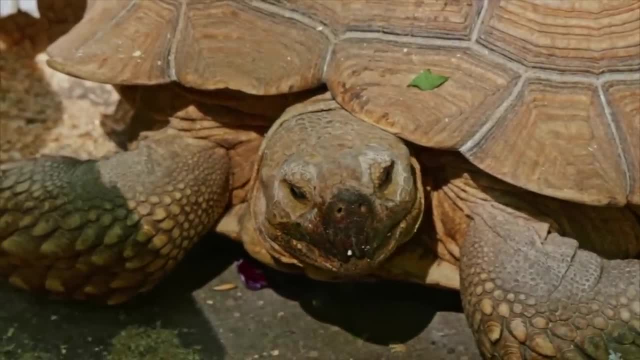 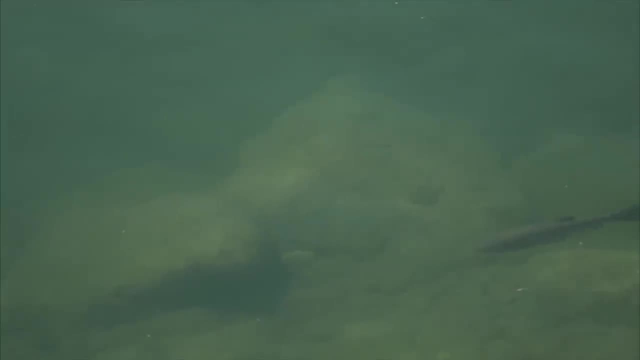 likely reflecting over-hunting, which may have led to their extinction in Iberia. Freshwater turtles were also caught at an ancient lake in Israel. Aquatic resources in general were quite an important part of the diet of some Neanderthal populations. Neanderthals seem to 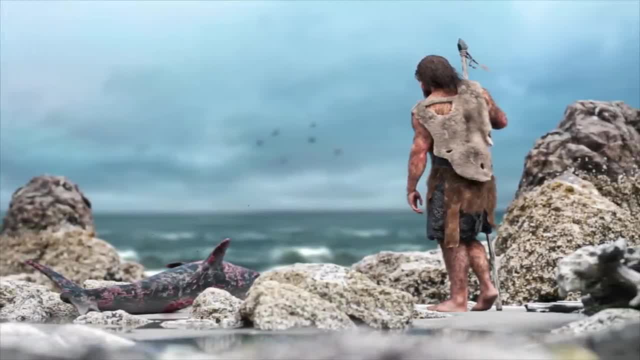 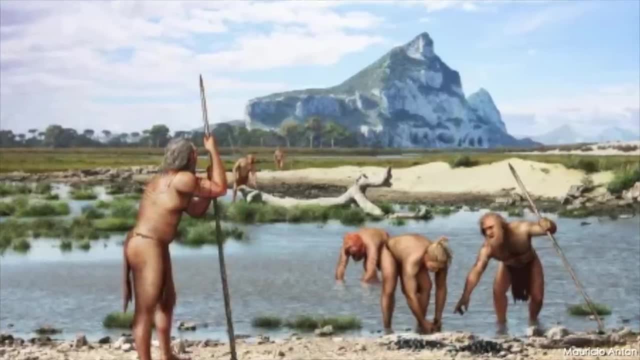 have exploited aquatic resources to a similar degree as our own early ancestors. Neanderthals, particularly have been used as a source of food for animals and animals of all ages. Neanderthals, particularly in southern Europe, ate all kinds of marine life: Crabs, clams. 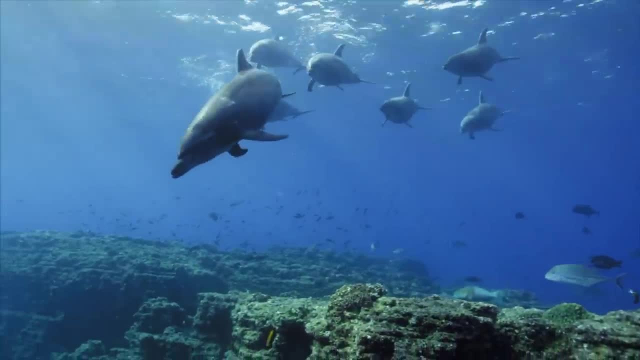 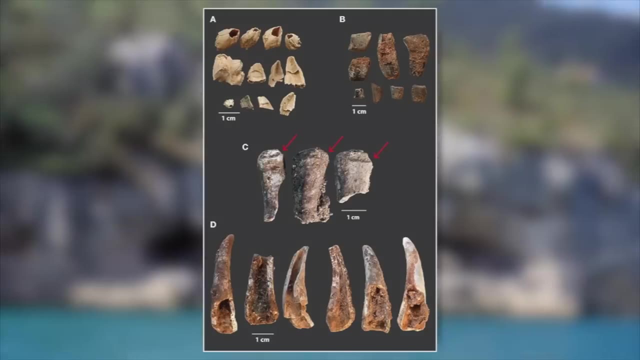 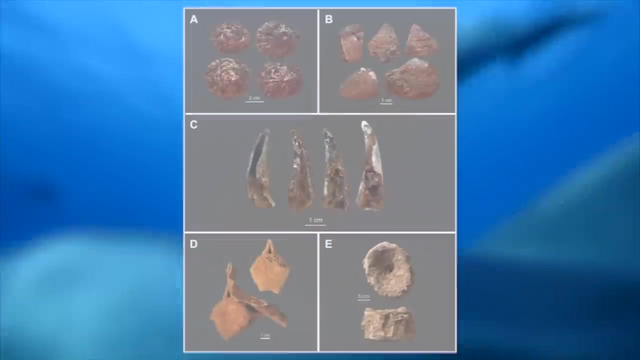 seals, many species of fish, dolphins and seabirds were all enjoyed. At Figueira Brava, Portugal, almost 800 shells of multiple species were found. This cave also preserves the remains of marine mammals with butcher marks: The remains of a monk seal, a ringed seal. 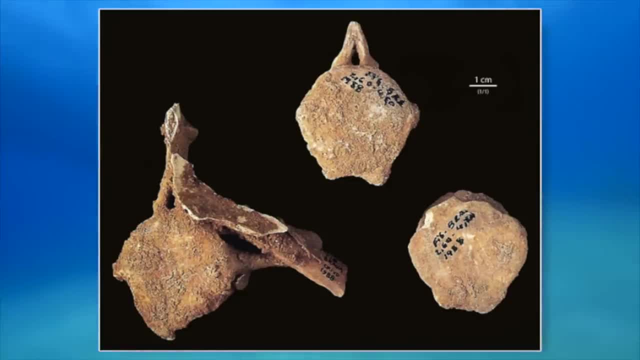 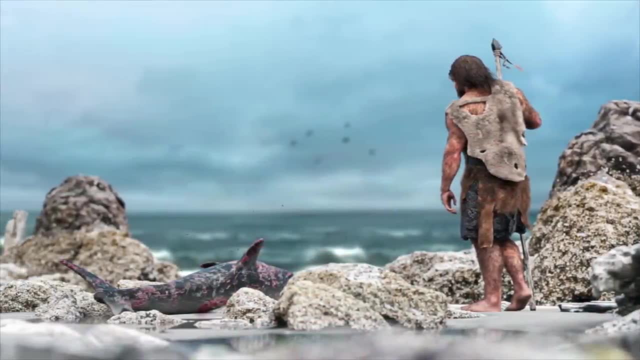 and two different bottlenose dolphins have been found. How these animals were acquired is a mystery. It is likely that they were simply scavenged, but other possibilities exist. Seal could be killed in shallow waters or while lounging on the shore. 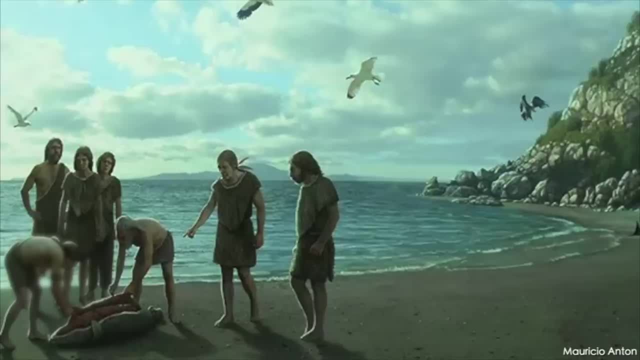 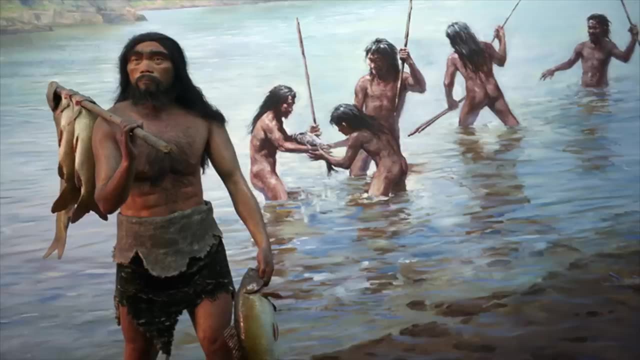 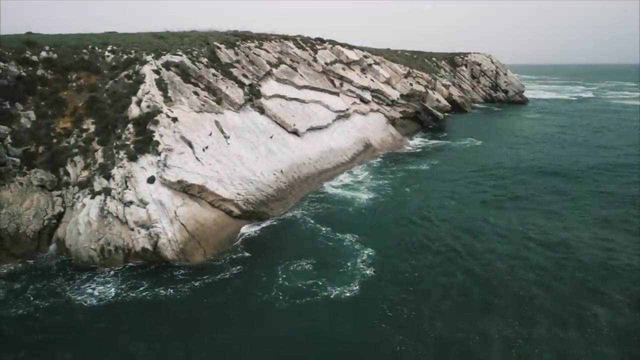 but dolphin would have been harder to encounter. A beached dolphin would have been easy prey and of course, washed-up carcasses could have always been scavenged. It is possible that they were hunted near the shore with spears. No hooks are known from Neanderthal remains, and neither are weights that could have been used for. 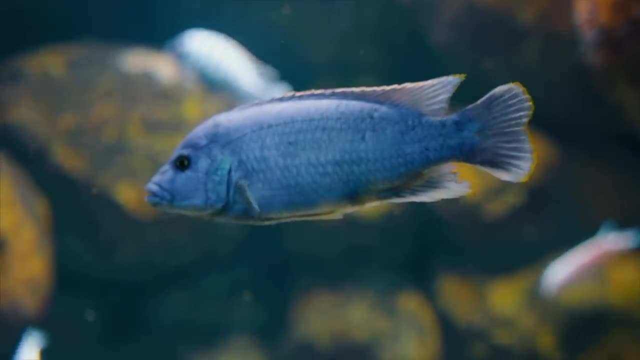 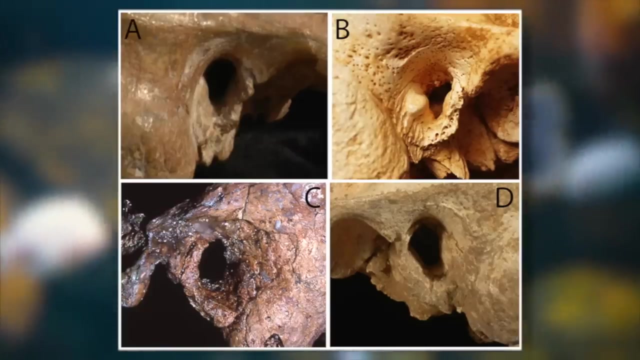 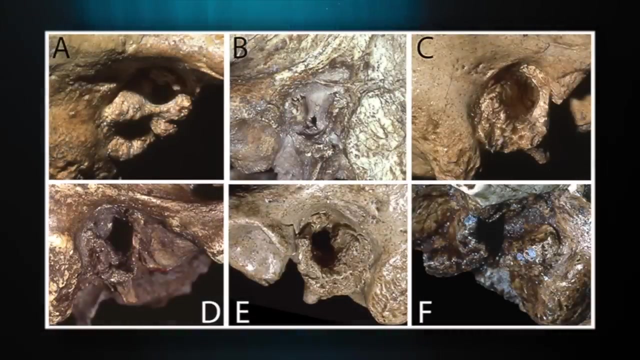 nets, Fishing methods would have likely consisted of hand and spear fishing. However, bony growths on Neanderthal skulls may suggest otherwise. Surfer's ear is a condition where the ear canal begins to grow bony protrusions in response to exposure to moist and cold conditions. The presence of this condition on many Neanderthal 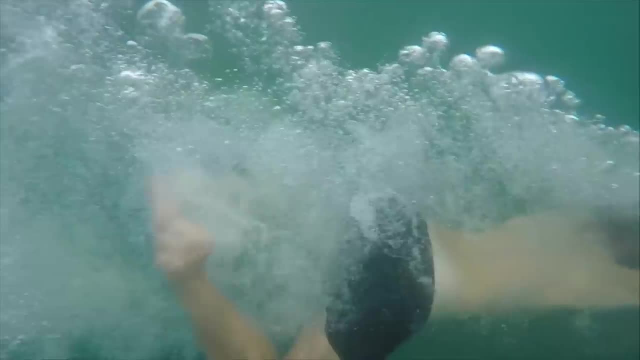 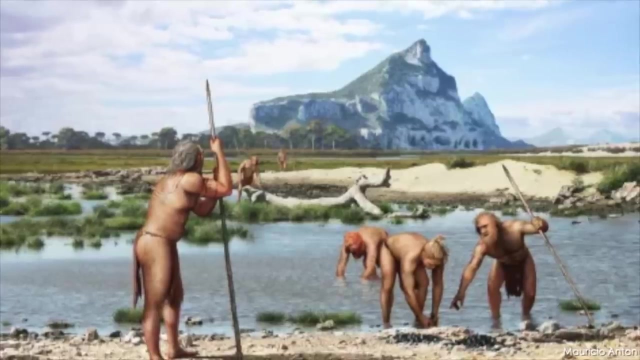 skulls may support the idea that they were diving. The abundance of shells at their site suggests that they were primarily foraging, but the presence of shells on the surface of the water may also indicate that they were foraging. Neanderthals also harvested fish in freshwater. 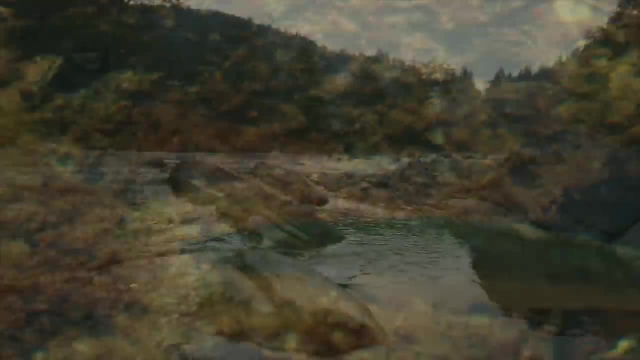 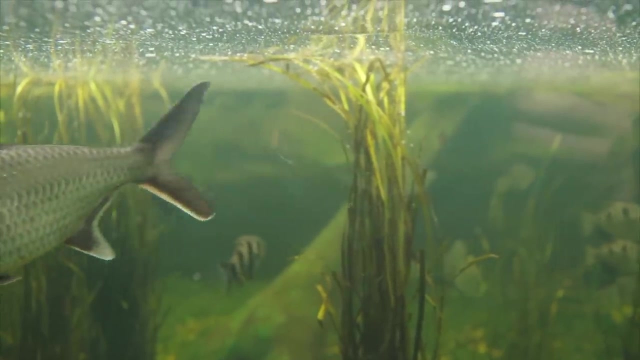 Trout, chub and eel have been found in Grotta di Castelcivita, Italy, which is on a river. Multiple sites in France have evidence of chub and European perch, Kodaro Cave. Russia even has evidence of Black Sea Salmon. 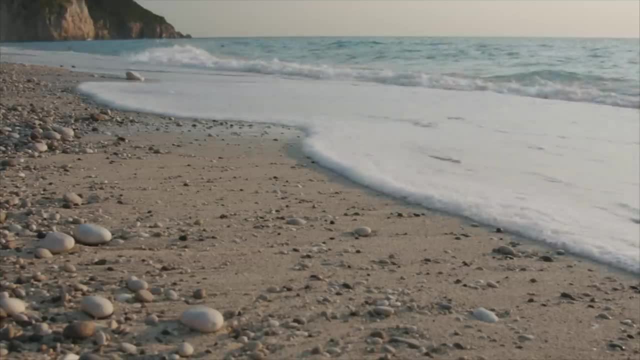 It is generally thought that a lot of the evidence of Neanderthals eating fish is lost due to the sea level rising and covering up cold waters. However, there is no evidence of any fish eating fish. It is generally thought that a lot of the evidence of Neanderthals eating fish is lost due to the sea level rising and covering up cold waters. 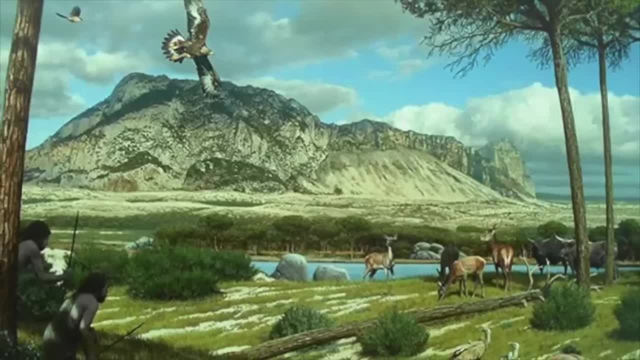 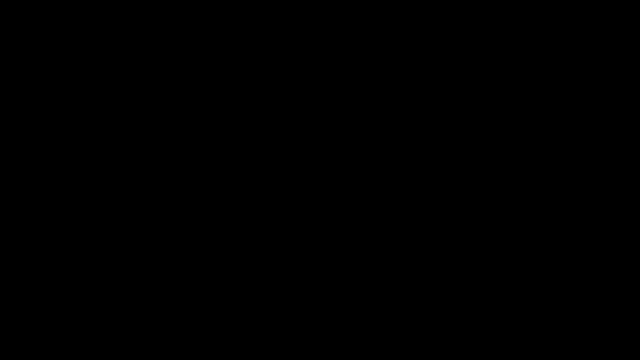 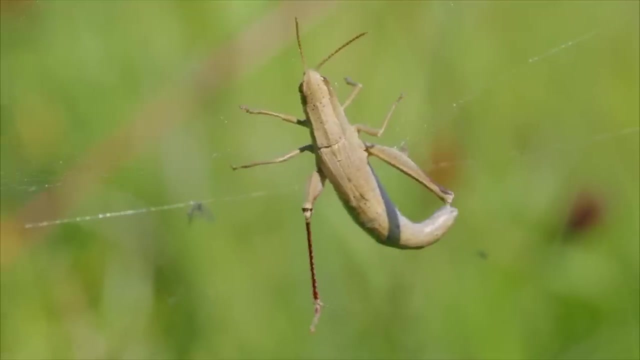 Even with the evidence we have, it is clear that some Neanderthals exploited aquatic environments for food and resources. One such lesser-talked-about food source would be insects. Eating insects may be frowned upon in some modern societies, though in others it is extremely common. 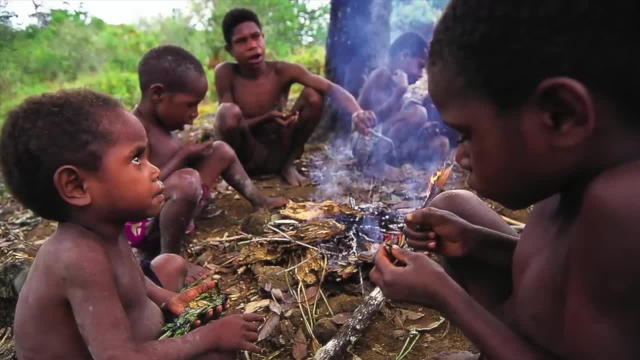 Hunter-gatherer societies are known to recognize the importance of insects. A variety of bugs can simply be caught by hand or with a simple stick. A variety of bugs can be caught by hand or with a simple stick. A variety of bugs can be caught by hand or with a simple stick. 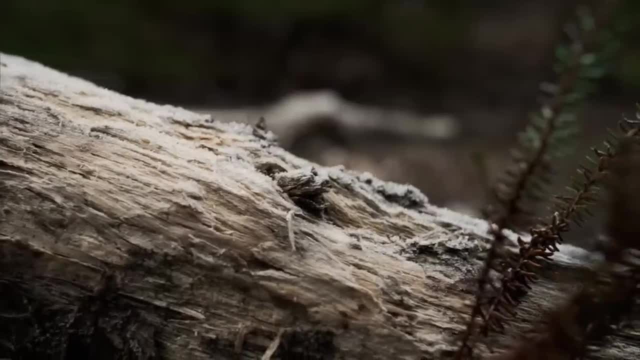 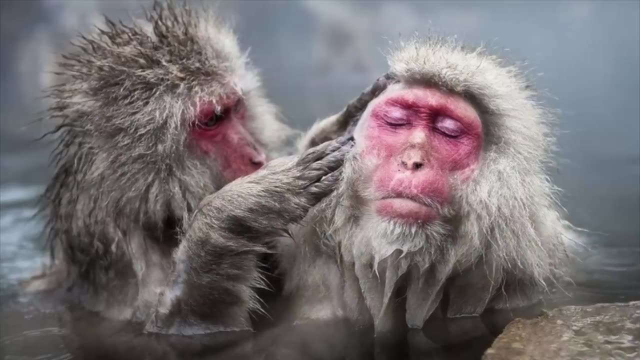 Smashing open rotting logs or scavenging grubs from carcasses could have easily provided valuable nutrients, especially in times of scarcity. Parasites on their prey and on themselves may have served as a quick snack. Some arctic people have considered the parasites on the. 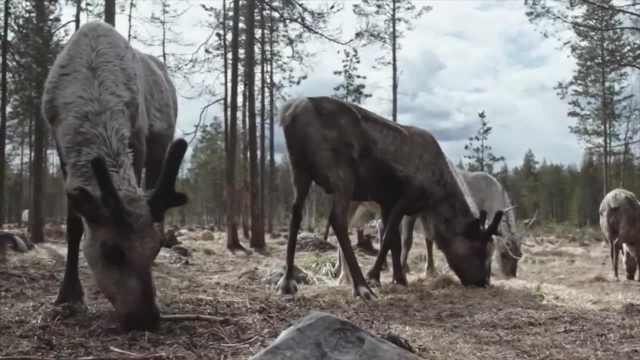 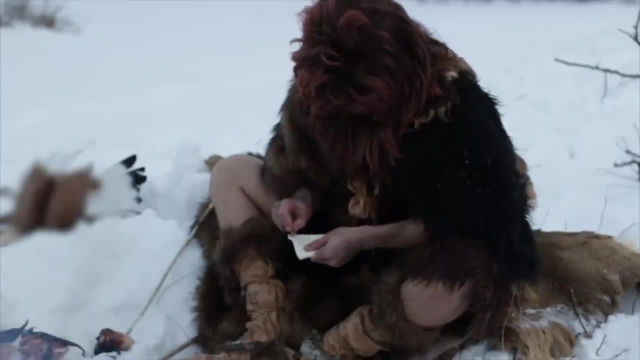 inside of caribou pelts to be a delicacy. There is currently no evidence of insect exploitation, though insects generally do not fossilize well, so that is not surprising, Since beeswax was mixed with some of their adhesives. 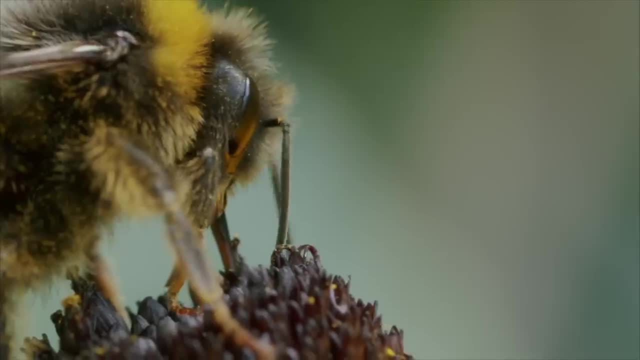 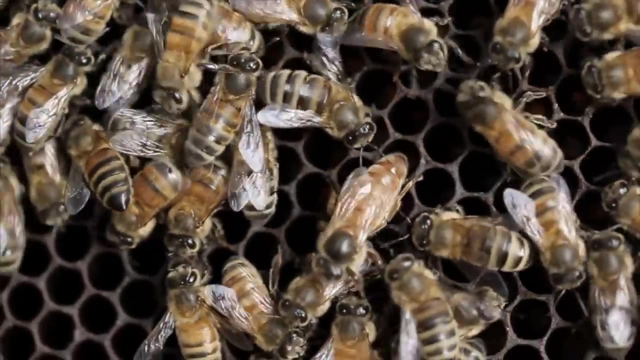 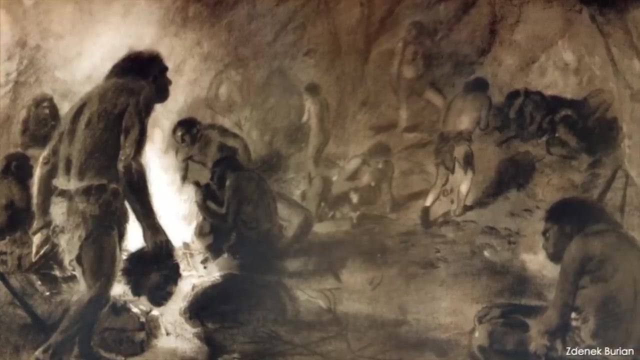 we can assume that they were also harvesting honey. Contemporary hunter-gatherers are known to be obsessed with honey, even if they get stung a little bit. Beehives would have provided them with tasty honey, nutritious larvae and useful beeswax. The last food source we will be talking about is other Neanderthals. 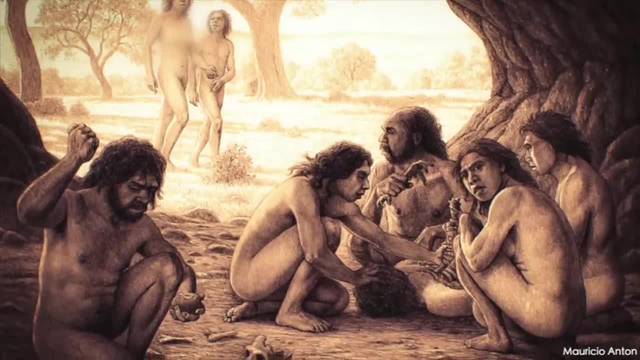 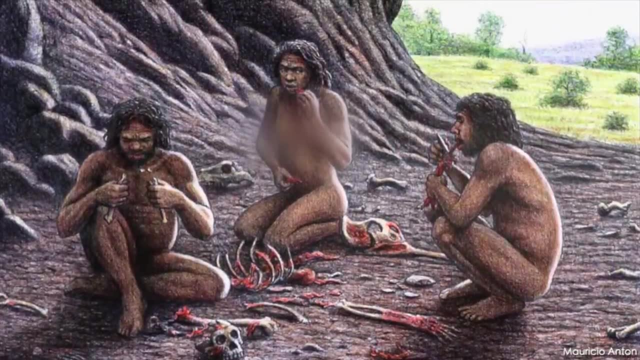 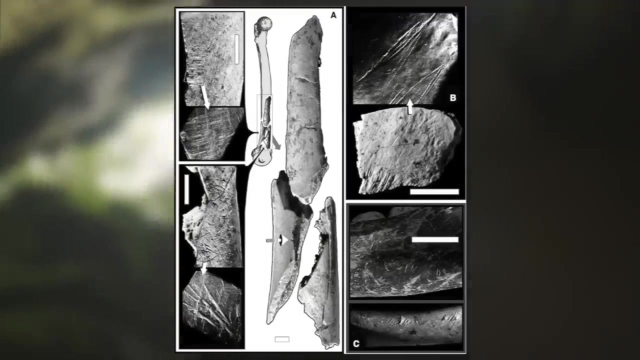 Neanderthals, just like Homo sapiens, practice cannibalism from time to time. The oldest evidence of cannibalism from Neanderthals comes from 120,000 years ago At Moulaghercy in southeastern France. the remains of at least six cannibalized individuals have been 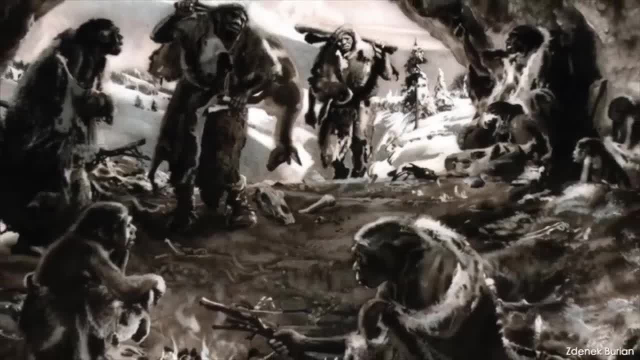 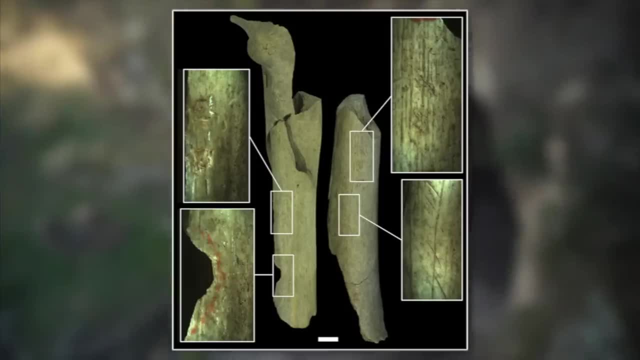 found Two adults, two teenagers and two children. Their flesh was cut and scraped from the bone, and their bones were smashed and thrown among the remains of their other prey. Many of the Neanderthals at Moulaghercy seem to have suffered from malnutrition. 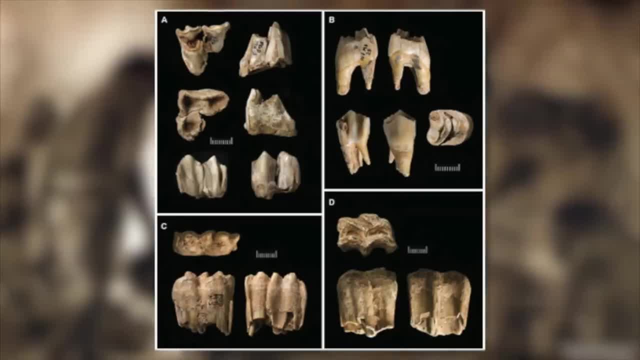 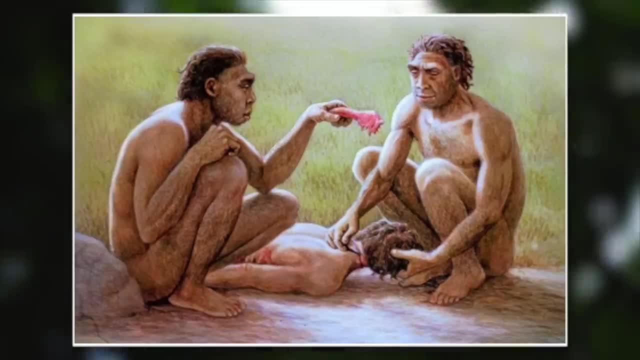 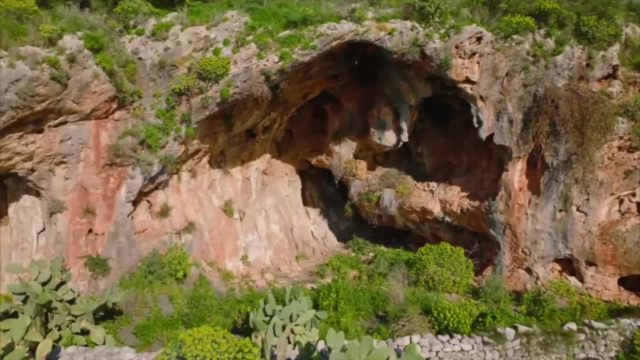 This is evident by the thinner bands of enamel on several teeth from Moulaghercy cave. Only the remains of six individuals were cannibalized at the site, and subsequent layers of habitation do not include cannibalized remains. Two authors of a 2019 paper about the site said: 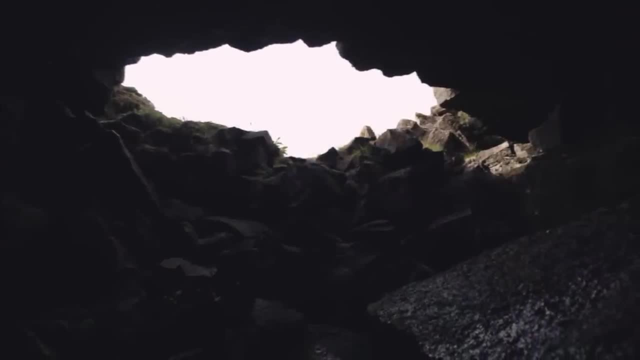 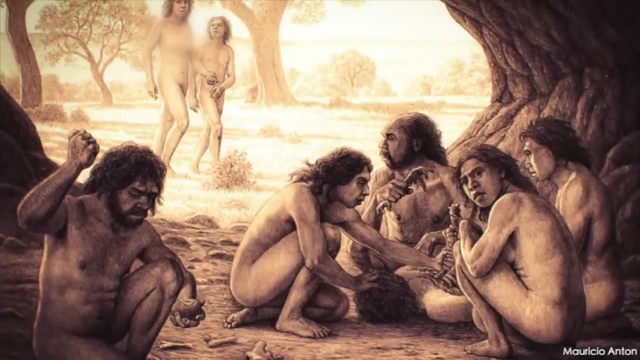 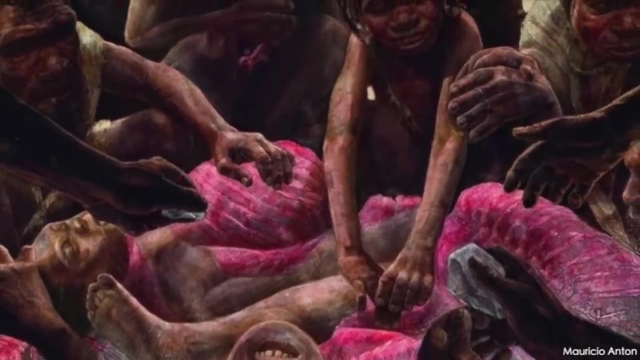 The cannibalism highlighted at Moulaghercy is not a mark of bestiality or subhumanity. If anything, it's a gut-wrenchingly human story. It's a story of hard choices and desperate times. At the end of the day, our bodies are edible and many will choose survival over starvation. 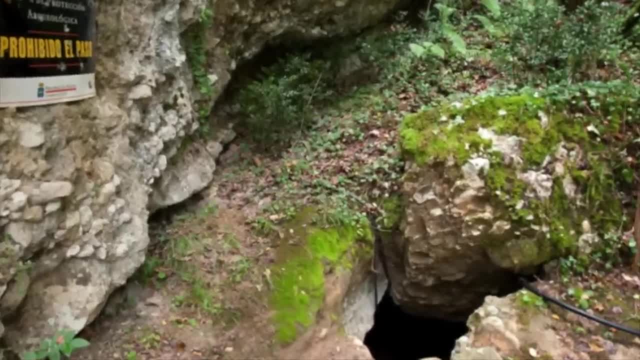 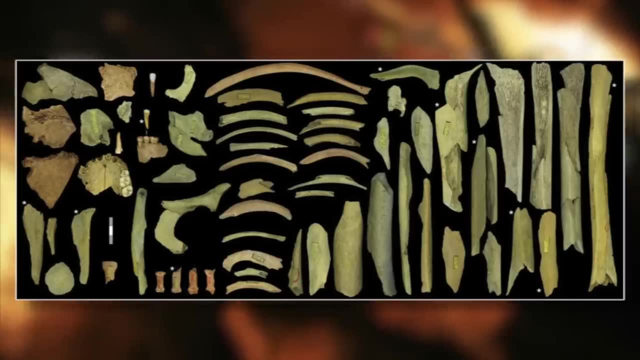 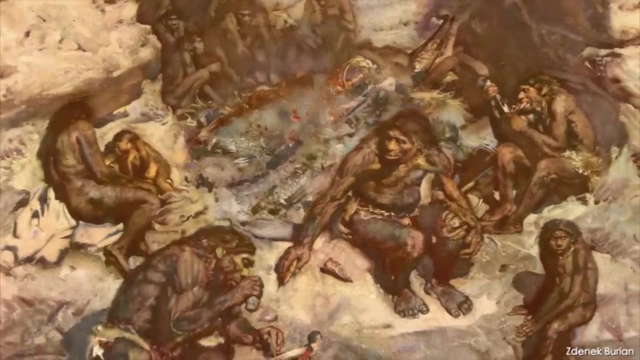 Another cave in northern Spain paints a grimmer picture. At El Cidron Cave, an exceptionally well-preserved assemblage of bones preserves the remains of 13 individuals. They include three adults, four adult females, three adolescents, two juveniles and one. 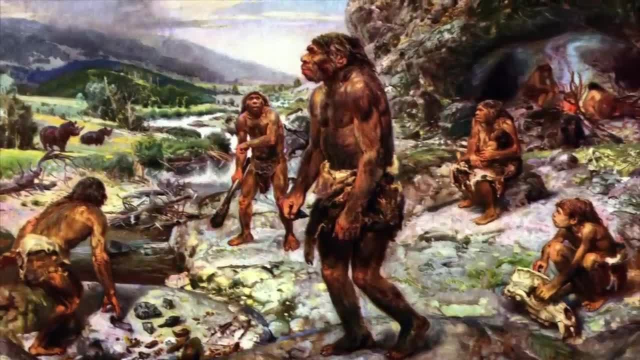 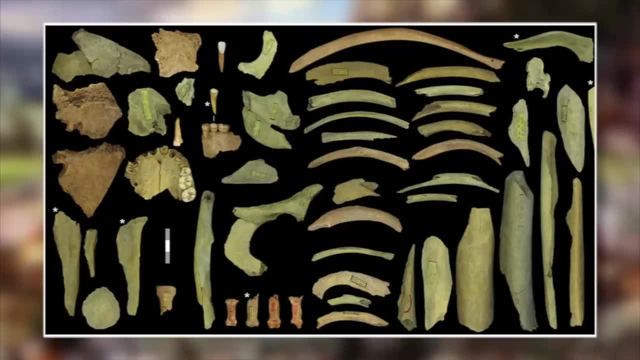 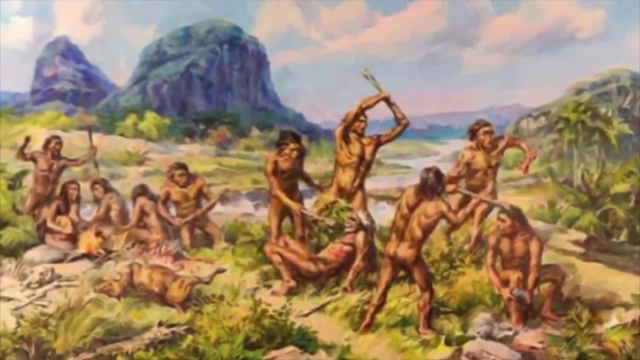 male. Analysis of their mitochondrial DNA supports a hypothesis that the 13 individuals represent one cohesive family group. The bones are full of cut marks and have been smashed to bits. This family was almost certainly murdered and cannibalized by another group. The group only had three adult males, which may have been easily overpowered. 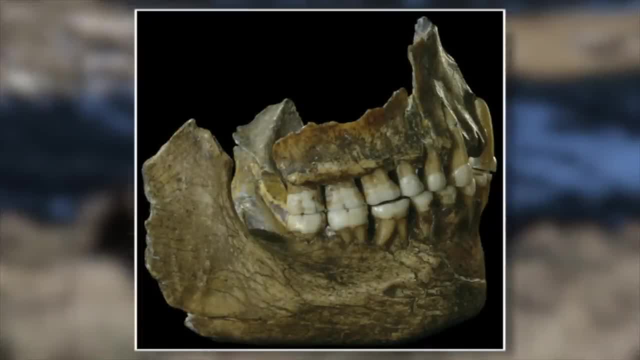 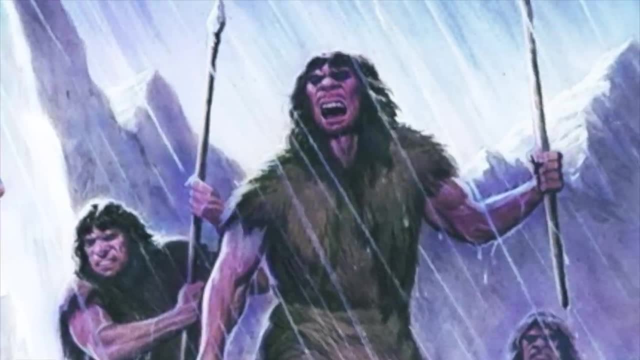 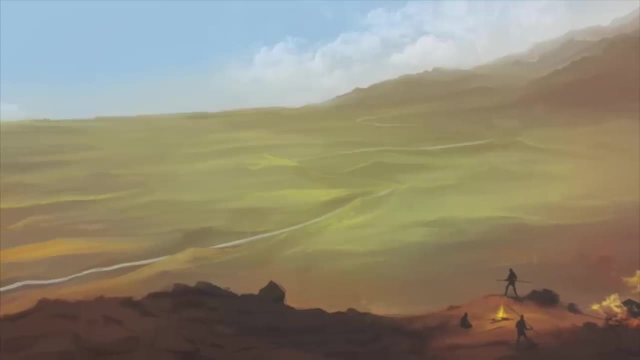 Even the adult men and women seem to have been quite young, as seen by the wear on their teeth, successfully targeted as a food source by a larger, stronger group. The remains of this family also indicate that they had been suffering from nutritional stress for their entire lives. 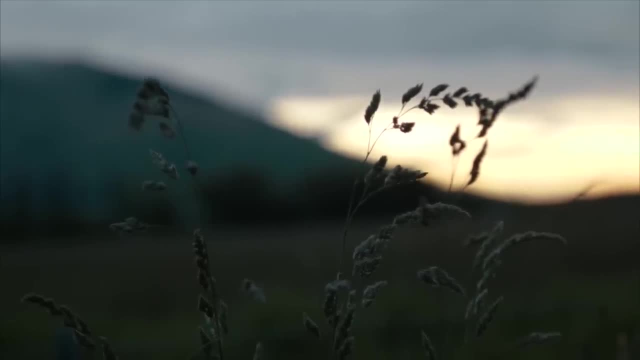 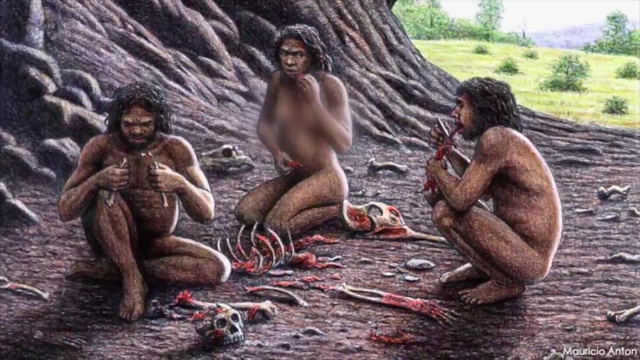 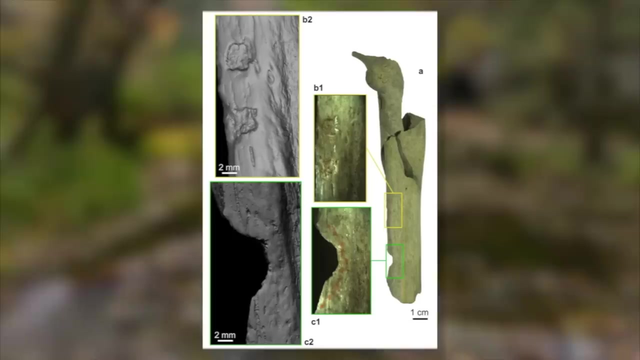 Their diet seems to have been made mostly of plant seeds, tubers and a smaller quantity of meat. They may have been targeted by another tribe that was having trouble filling their stomachs. Another site in Belgium has grisly evidence of Neanderthals being butchered. 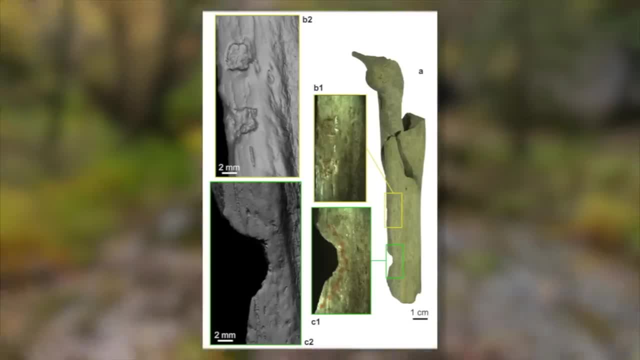 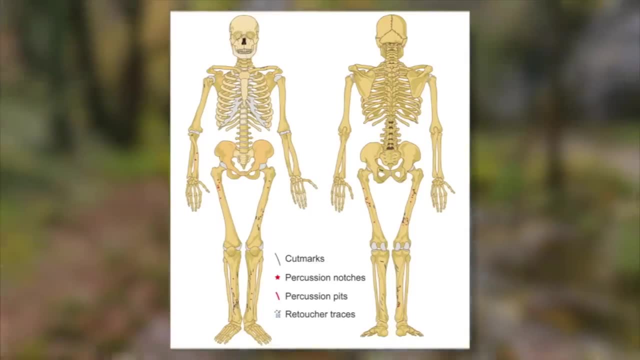 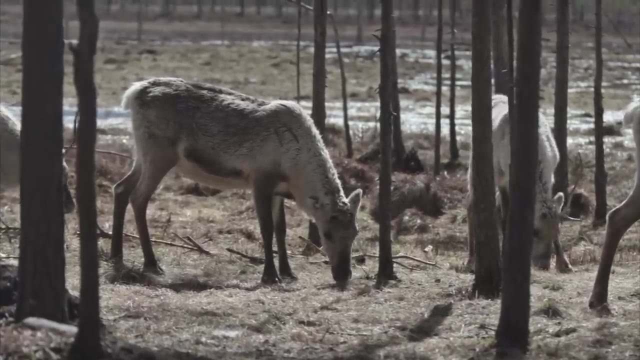 Through the cut marks present on their bones, it was determined that the upper limbs were disarticulated, the lower limbs were defleshed and smashed, and the chest was disemboweled, among other smaller cuts. Their butchering was conducted in a very similar way to their normal prey of reindeer. 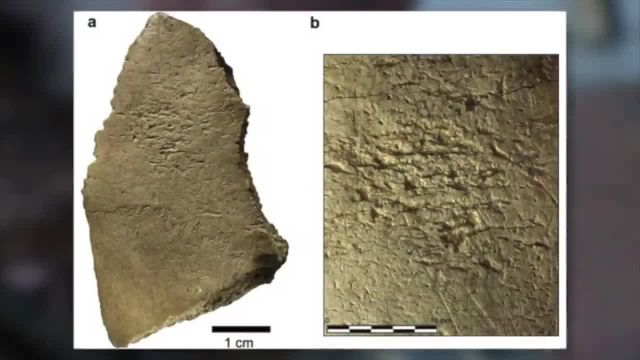 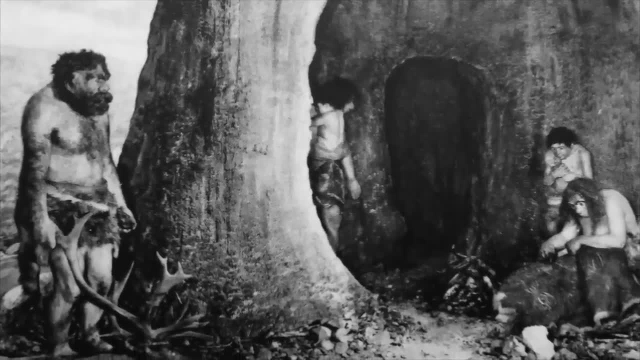 Some Neanderthal bones were also used as retouchers to freshen up the edges on their stone tools. 2. Cannibalism: The aforementioned examples may be painting a picture that is not necessarily accurate. Neanderthals were expert butchers. 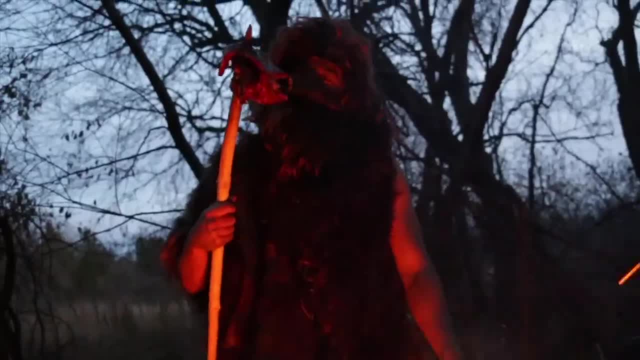 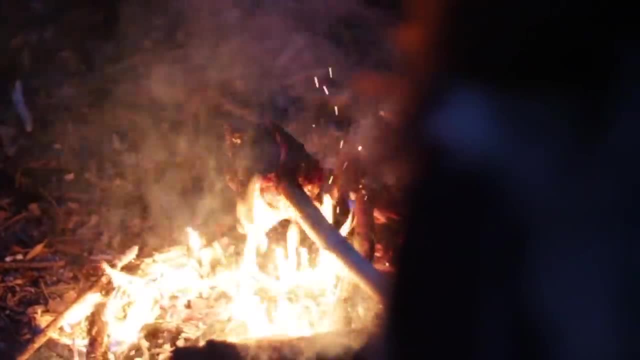 If they were consuming other Neanderthals on a daily basis, you would see much fewer cut marks on these remains. Cannibalism would have been reserved mainly for starvation. When considering all of our Neanderthal remains, it is apparent that Neanderthals practice. 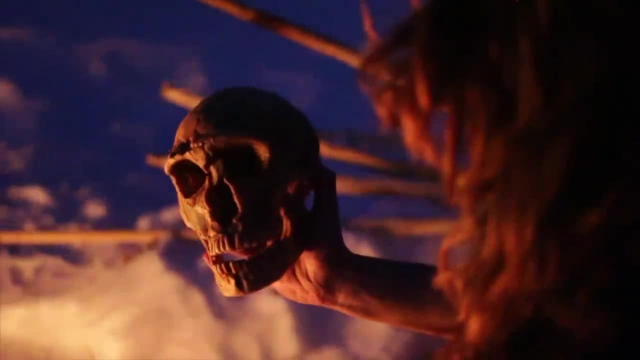 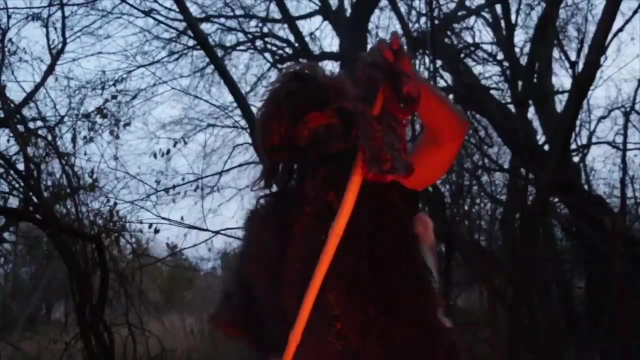 cannibalism to a similar degree as our own species. To label them all as cannibals is as follows: 1. Cannibals- The term cannibals is as inaccurate as calling all homo sapiens cannibals. Regardless of what they were eating, we know that they needed plenty of calories to survive. On average, Neanderthals were shorter than modern humans, though their stockier bodies required comparably more nutrition. Their shorter legs meant more steps and deep snow would have been hard work. to move through Cold environments without highly tailored clothing would have used a lot of energy, just 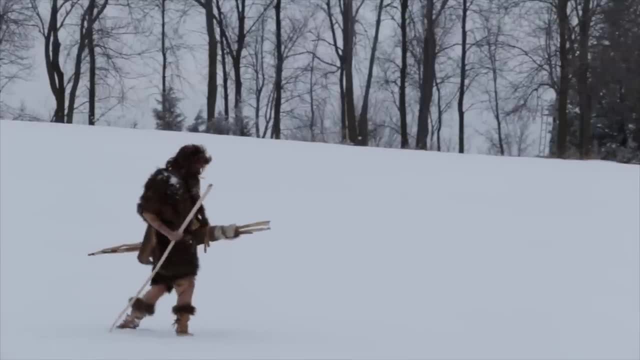 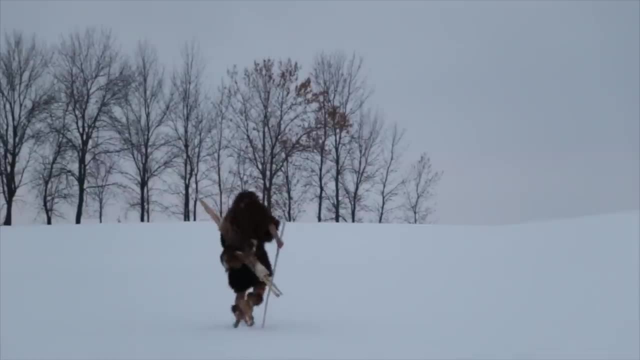 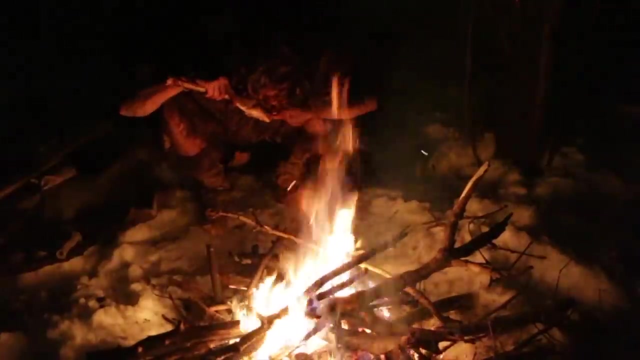 to stay warm, Carrying equipment, babies or injured friends would have been even more taxing. Larger brains, hearts and digestive tracts would have passively burned a lot of energy, whether active or not. Between 3,500 to 5,000 calories would have been required daily. 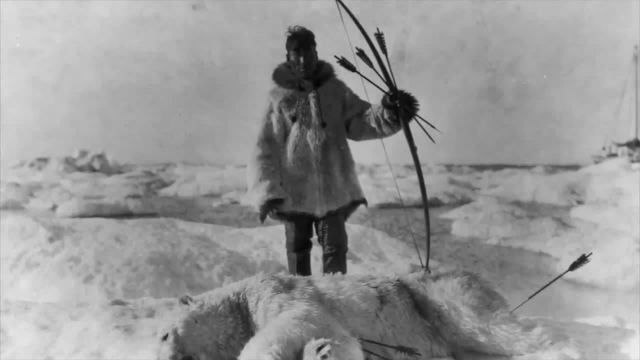 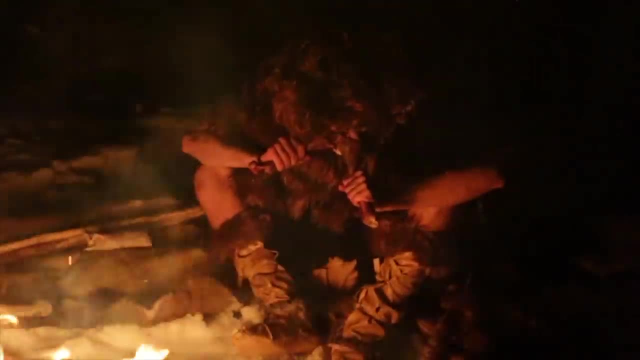 Contemporary hunter-gatherers living in similarly cold environments are known to eat over 3 kilograms or 6.5 pounds of meat each day. That is a rough estimate: 2., 5., 8., 8., 9., 9.. 10., 10., 11., 11., 12., 13., 14., 12., 14., 15., 16., 15., 16., 17., 17., 18. 19.. 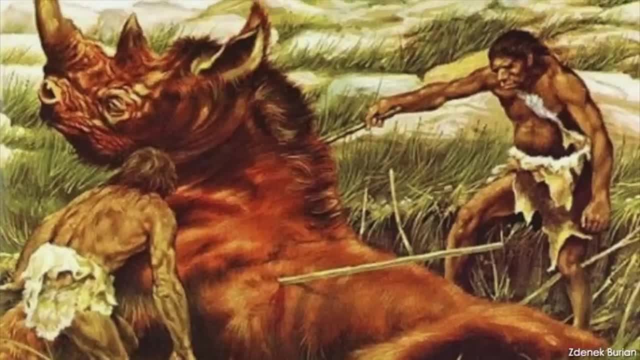 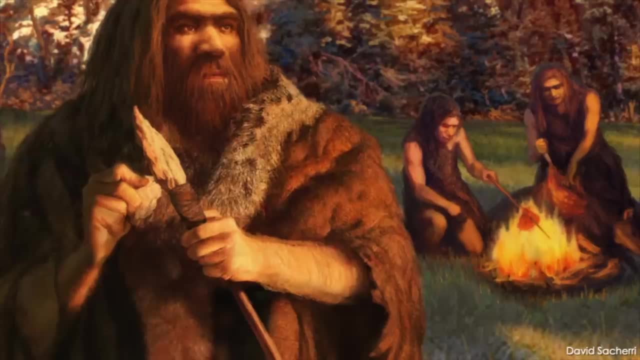 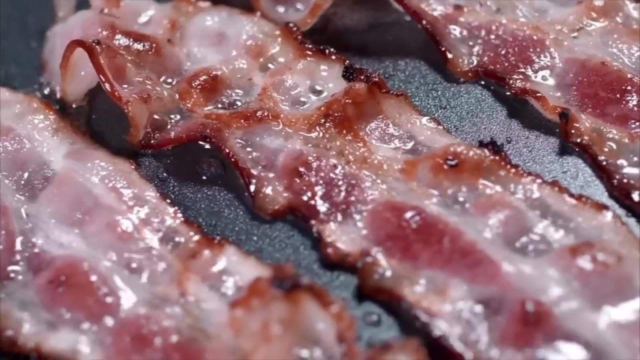 19., 20. 23., 24. 25. 21. 22. an average group for over two weeks. However, massive quantities of lean meat can actually lead to a form of malnutrition called protein poisoning. Many people get confused with the term protein poisoning because of the popularity of carnivorous. 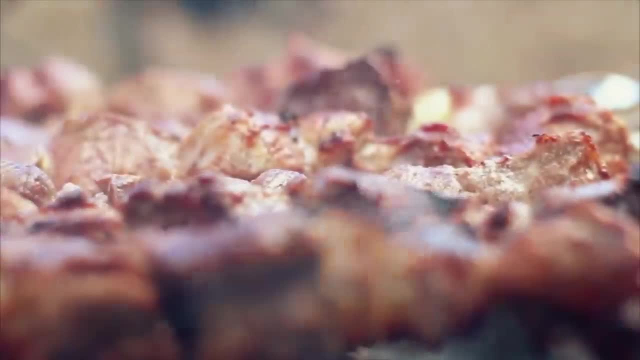 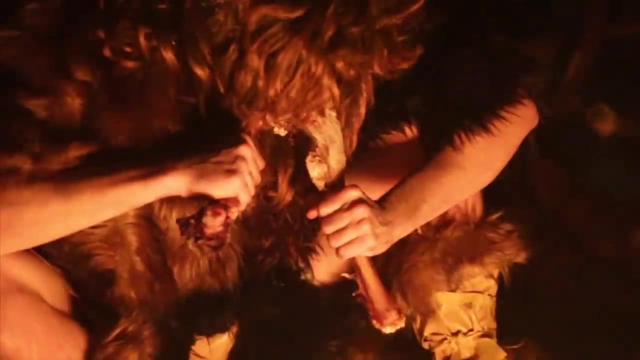 diets. Protein poisoning does not occur from just eating meat. It occurs when almost all calories consumed come from protein in lean meat. The lack of other nutrients, specifically in lean meat, can lead to health problems such as dysentery and even starvation. 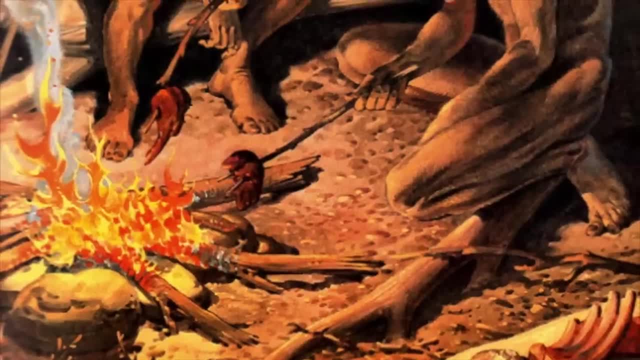 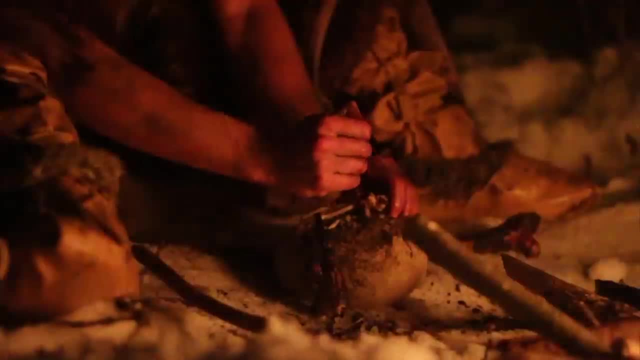 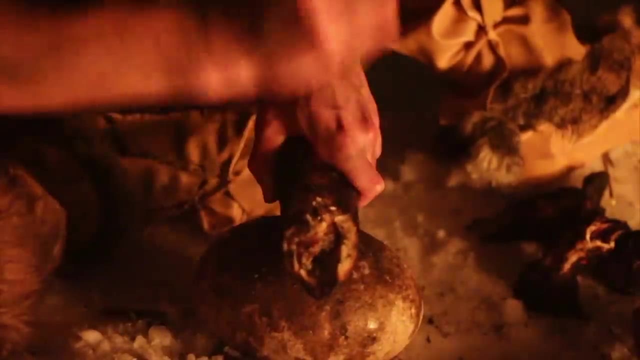 In order to have a heavily animal-based diet, Neanderthals would have certainly needed to consume eyes, brains, tongue, fat marrow and other fatty organs. Fat in general is a very valuable resource in hunter-gatherer societies. Considering they heavily processed long bones and skulls, it appears they highly valued. 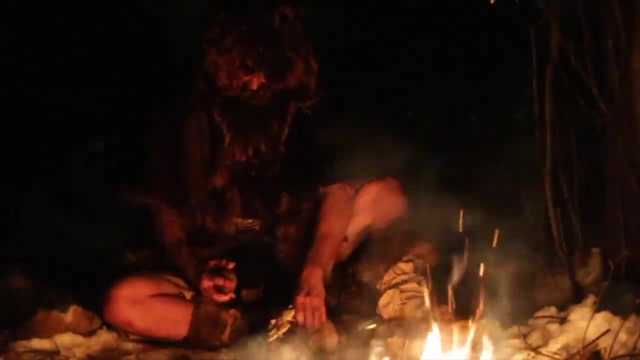 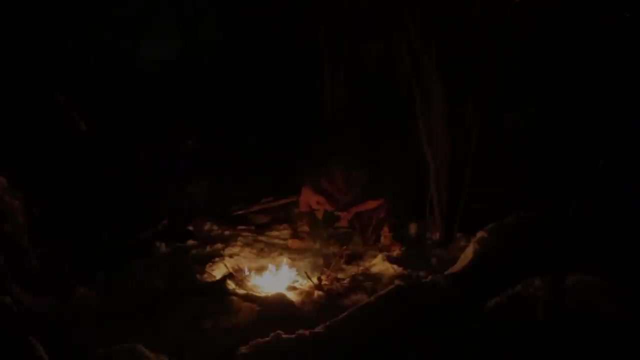 fat and marrow. Neanderthals may have even eaten the partially digested content of meat. The fat content is found in the stomachs of their prey, as seen in contemporary hunter-gatherers. An important question about the diet of Neanderthals is what proportion of animal products did? 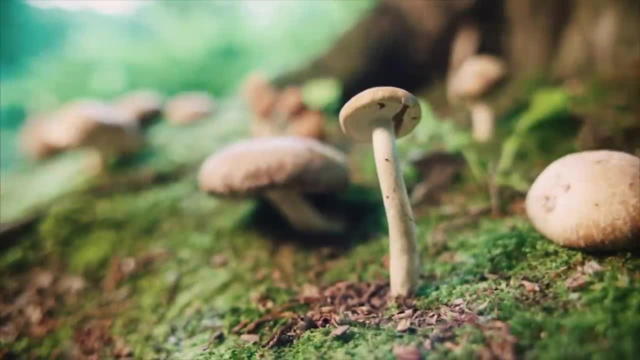 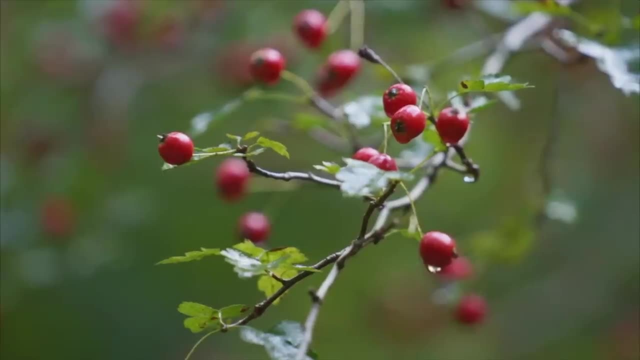 they eat. in comparison to other foods such as plants or fungi, Plants would have certainly been an important part of the diet of Neanderthals, though we have to consider the limitation of plants as a whole. Many wild plants are not very calorically dense. They offer a wide array of nutrients. Neanderthals would have typically been concerned with warding off starvation and not feeling marginally better. Edible plants also do not grow at a high frequency during the winter, meaning that meat intake would have increased during these months. 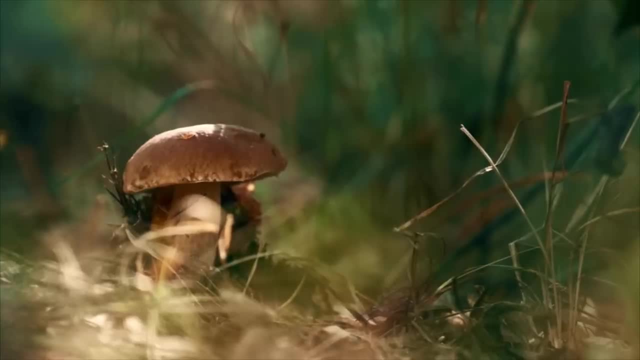 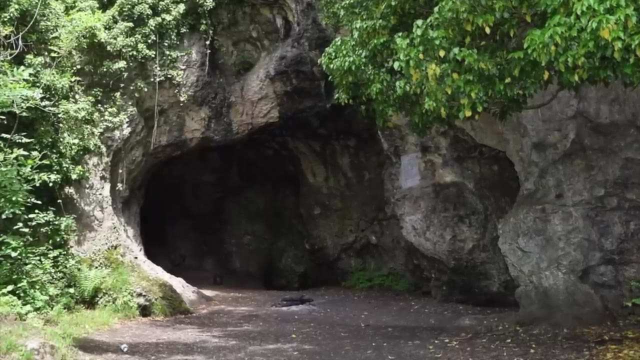 Nuts, moss, tree barks and mushrooms would have been some of the few plants and fungi available during the winter. Dental tartar from Grote des Spa in Belgium indicated that the inhabitants had a diet including mouflon, sheep, woolly rhinoceros and mushrooms. 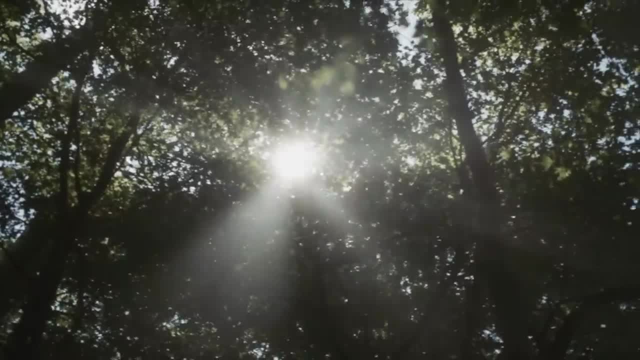 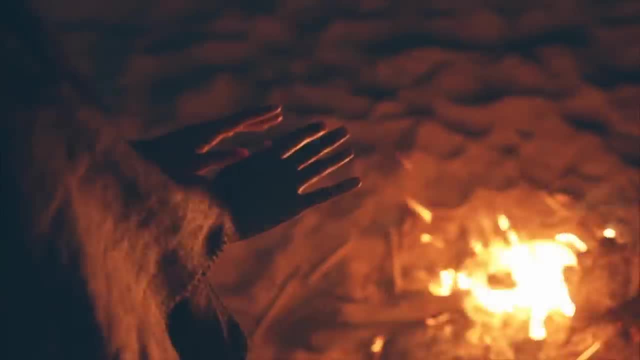 Neanderthals would have typically been concerned with warding off starvation and not feeling marginally better During warmer interglacial periods. plants seemed to have played a larger role in Neanderthal diets. Middle Eastern sites preserve the remains of charred nuts, including acorns walnuts. 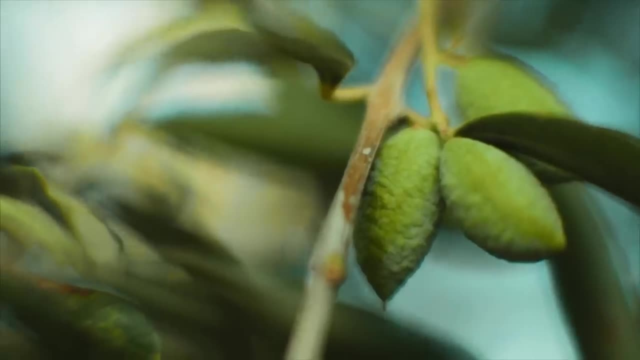 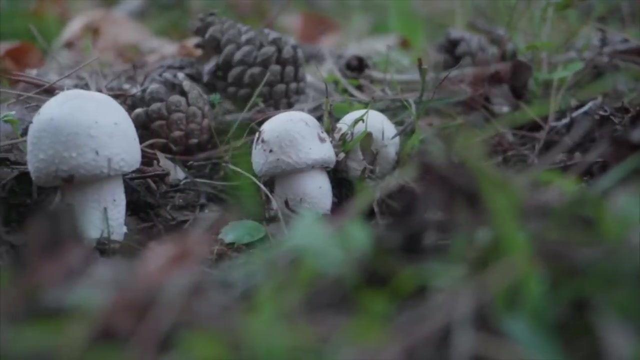 pistachios, and hazel and pine nuts. Fruits including dates, figs, olives and grapes can also be found. A large variety of plants found at these sites suggest that they had a knowledge of many plants and knew how to get to them. 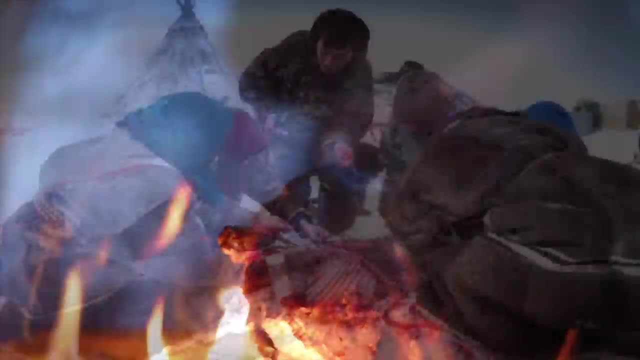 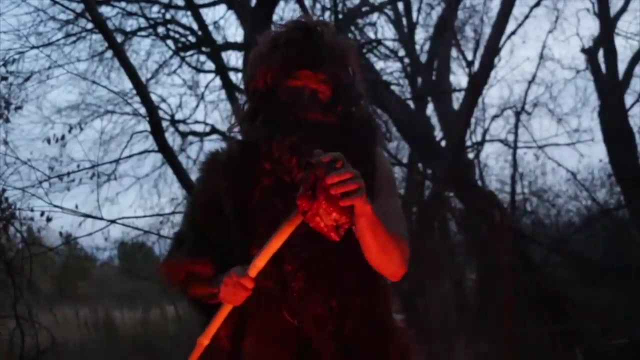 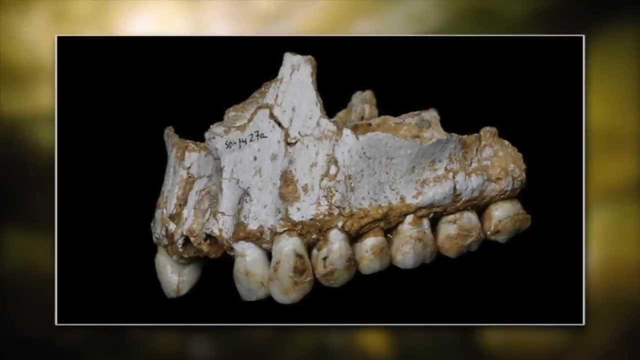 They also said that the animal products were the primary source of nutrients. However, their wear is not like that of arctic people who exclusively eat meat. It is more similar to populations with a relatively varied diet. The dental calculus of an individual from El Cedron Cave had no evidence of large mammal. 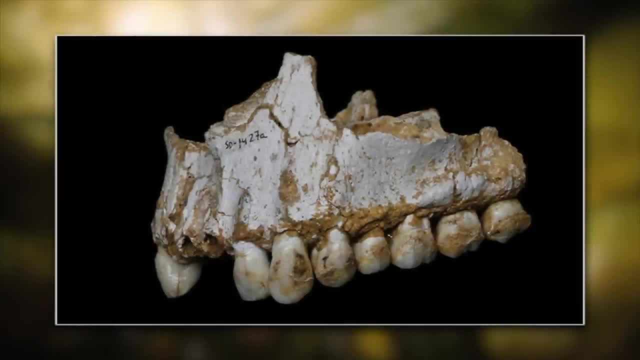 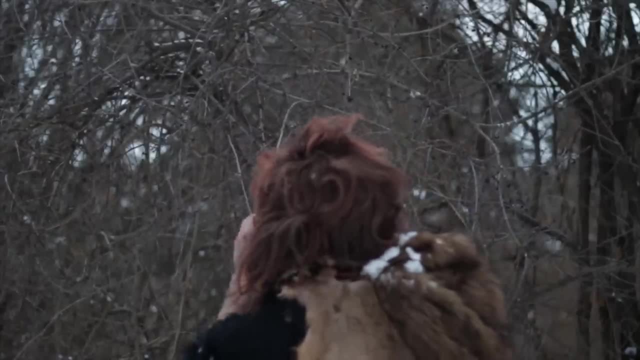 DNA, but it did have evidence of pine bark, mushrooms and moss. This discovery created claims of vegetarian Neanderthals all over the internet, though the truth is more complicated. The DNA found in Neanderthals is more complex than in animals. 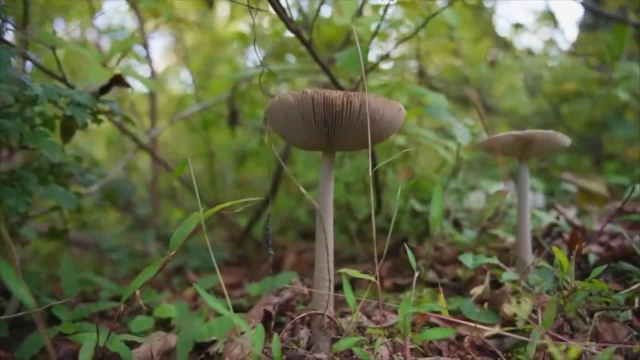 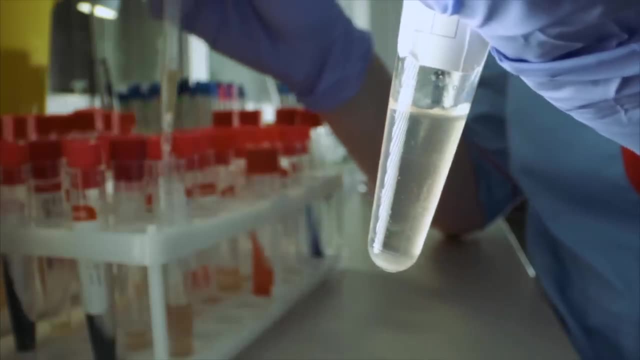 The DNA found in Neanderthals is more complex than in animals. The DNA found in the calculus matched mushrooms from the area, pine bark from East Asia and a moss with little to no nutritional value. The moss and pine bark may have gotten into the test through contamination. 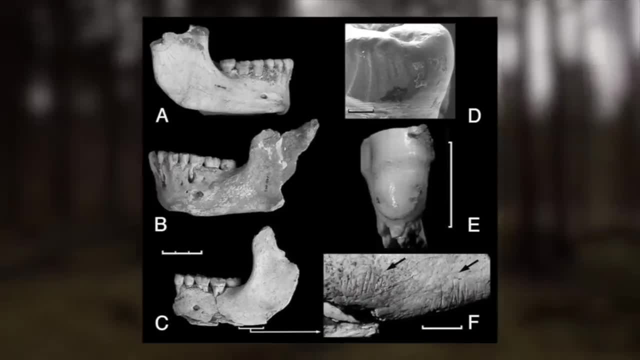 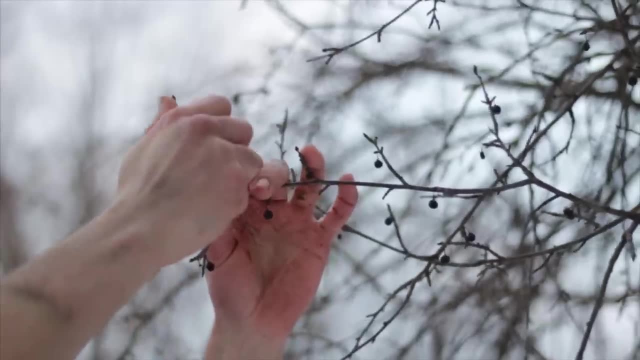 The actual dental wear on the remains of this individual and others at El Cedron suggest a varied diet, including plants and animal products. The idea of a purely vegetarian Neanderthal seems to be a product of our modern imagination rather than a reflection of reality. 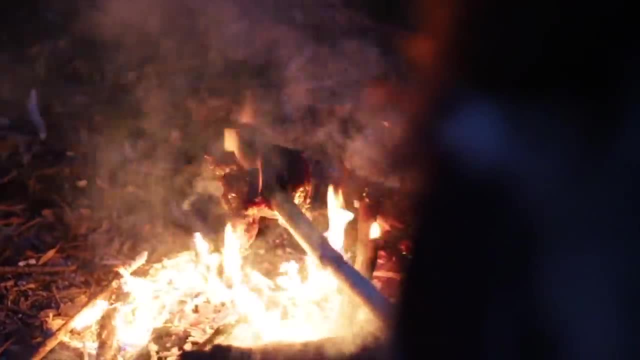 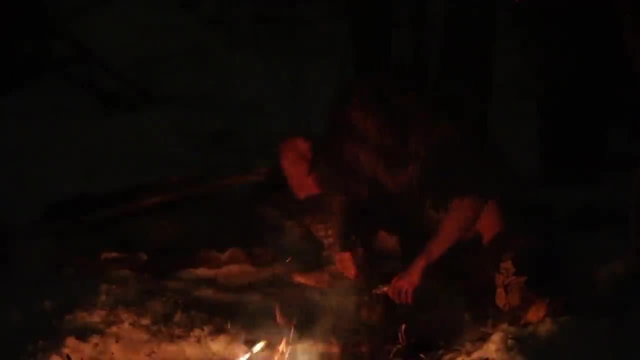 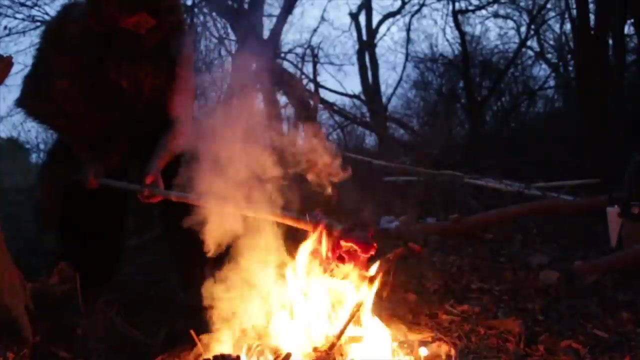 When considering Neanderthal diets, we must also consider how the food was actually prepared. As already mentioned, cooking food breaks it down and thus increases its nutritional value, along with other benefits. But how was meat actually cooked? Roasting meat on skewers would have been a good way to quickly cook up a piece of meat. 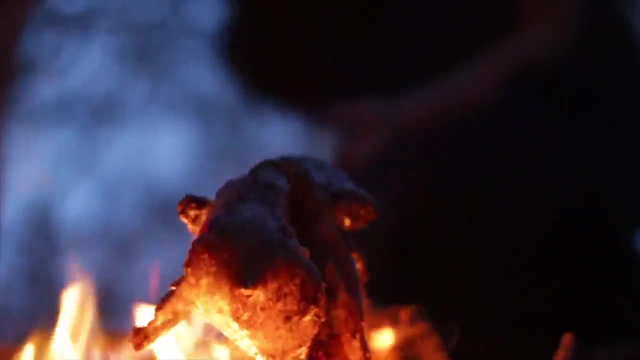 A stick from the Schoeniggen site even appears to have been used for that exact purpose. The problem with roasting a piece of meat over the fire is that precious calories are not enough to cook up a piece of meat. The problem with roasting a piece of meat over the fire is that precious calories are. 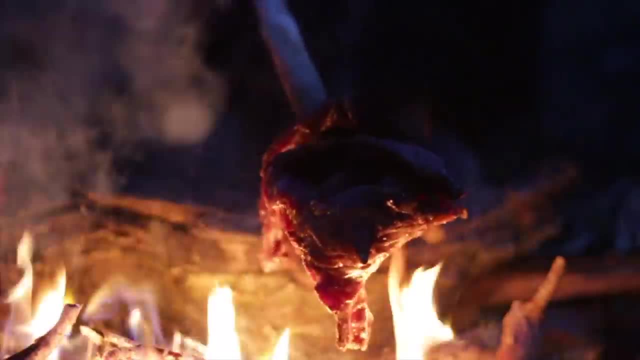 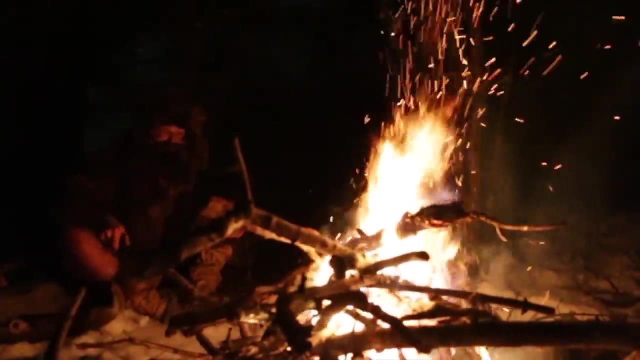 not enough to cook a piece of meat. The problem with roasting a piece of meat over the fire is that precious calories are not enough to cook up a piece of meat. The meat still remains tough. Other methods, such as making stews or baking by throwing a large piece of meat directly. 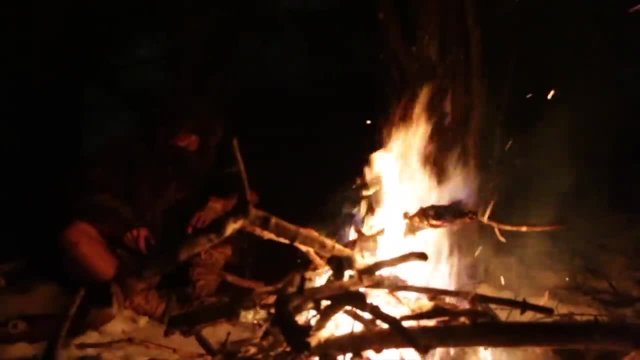 on the coals and then burying it would have provided more calories than an oven on the scale of an egg. Other methods, such as making stews or baking by throwing a large piece of meat directly on the coals and then burying it, would have provided more calories. 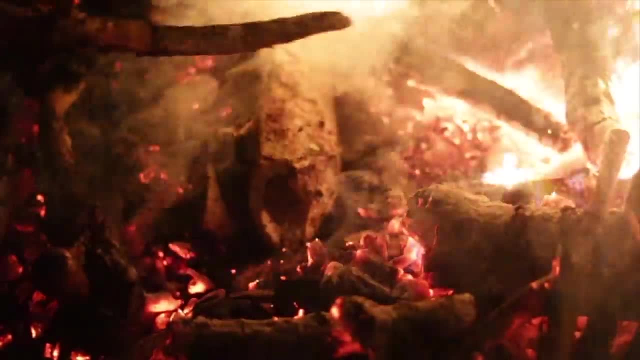 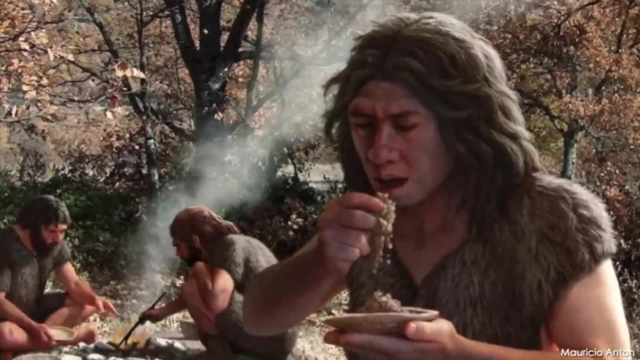 It is easy to bury meat in a fire and to let it cook, but creating some kind of stew or soup is much harder. It requires a waterproof container that can also withstand a lot of heat. Rocks heated in the center of a fire can be placed into any container of water to boil. 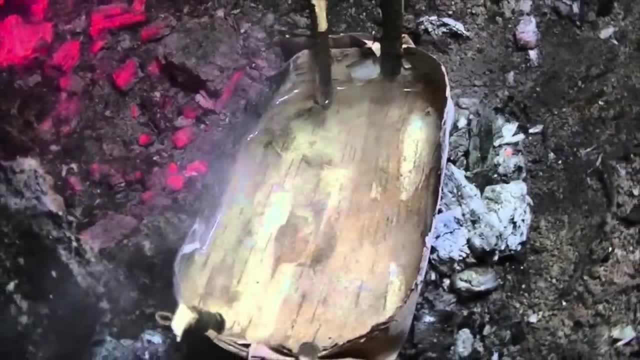 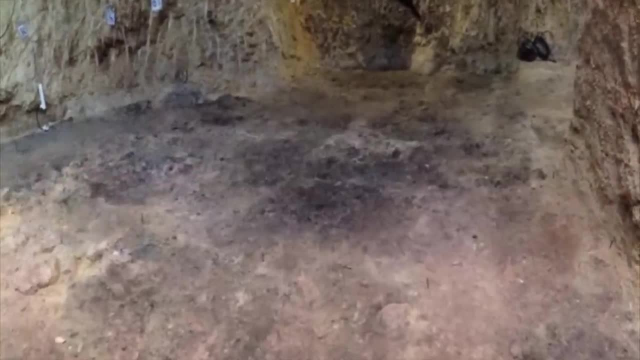 it. A bark bowl, animal stomach or skull could have been used for this purpose. There is even a rock structure from Abric Romani that may have been used as a container to boil liquids. A hole in the rock capable of being filled with a liquid is located right next to a high 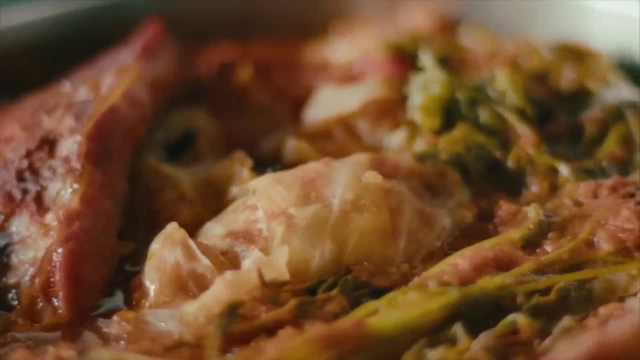 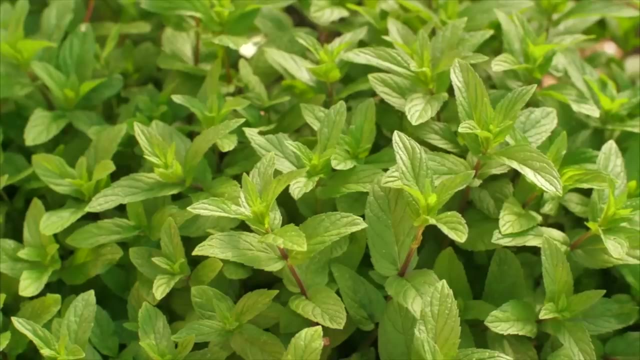 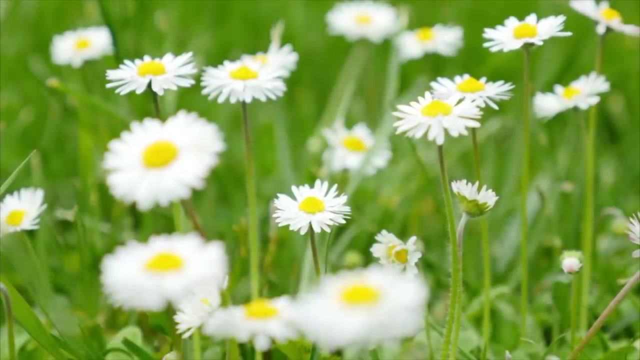 quantity of hearths. It may have been used to boil stews or steam meat. Plants remains from other sites also appear to have been cooked Along with caloric staples. Neanderthals may have seasoned their food with wild herbs. In the calculus of a Neanderthal from El Sajon Cave, researchers found chamomile and yarrow. 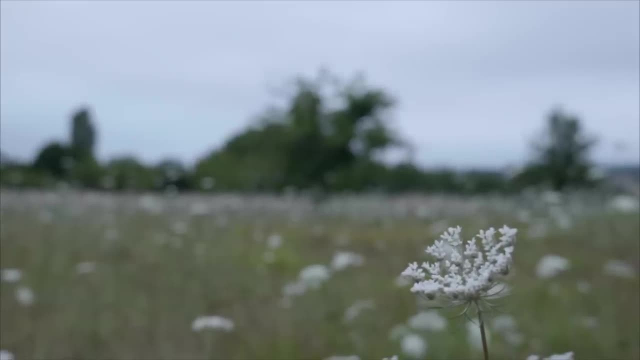 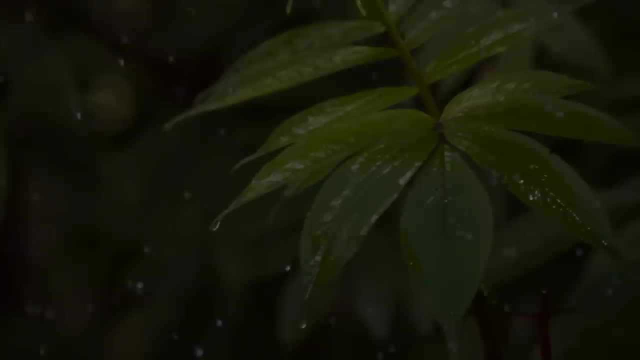 Neither of these plants have any nutritional value, though they do have strong flavors. They may have been used to add flavor to their food, though they may have also been used as a form of medicine. Besides immediate use, we must also consider how Neanderthals have been used to make their food. Neanderthals would have stored perishable goods such as meat or even some plants. Killing or scavenging a woolly mammoth would have left a Neanderthal band with literally millions of calories- enough to feed a group of Neanderthals for months. 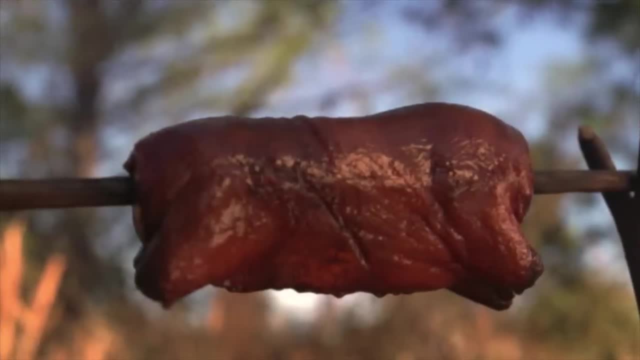 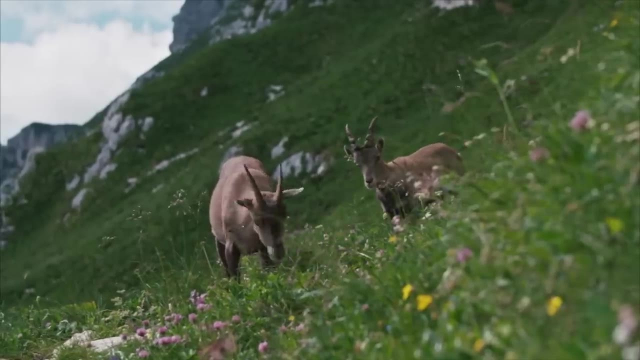 Even an abundance of relatively smaller animals may have warranted preservation. At Grotte du Lazaret, France, a total of 23 red deer, 6 ibexes, 3 aurochs and 1 roe deer appear to have been hunted in a single day. 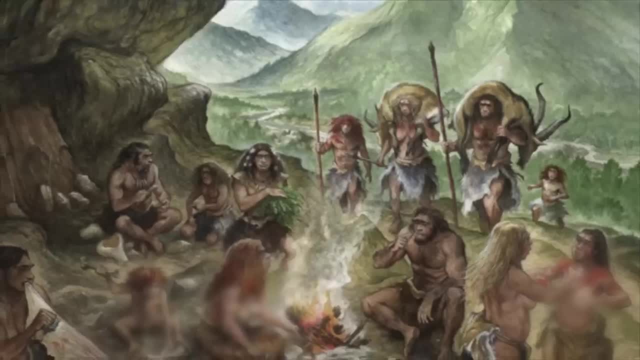 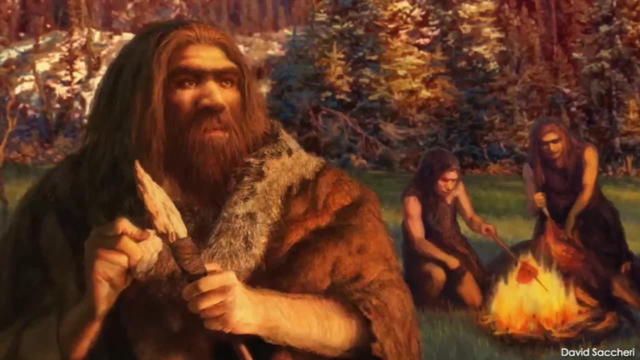 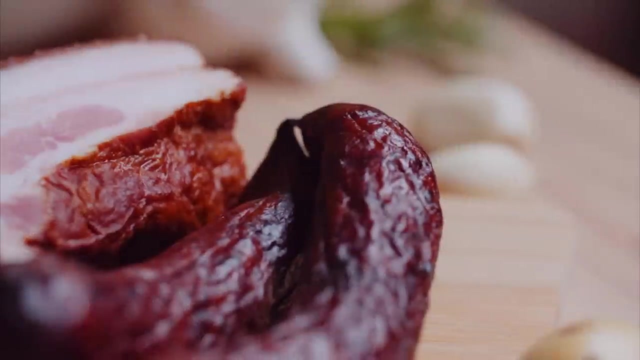 The entire carcasses appear to have been transported to the cave and then butchered. Because this is such a large amount of food to be consumed, it is possible these Neanderthals were curing and preserving it before winter. set in Curing meat could have been accomplished in a few ways. 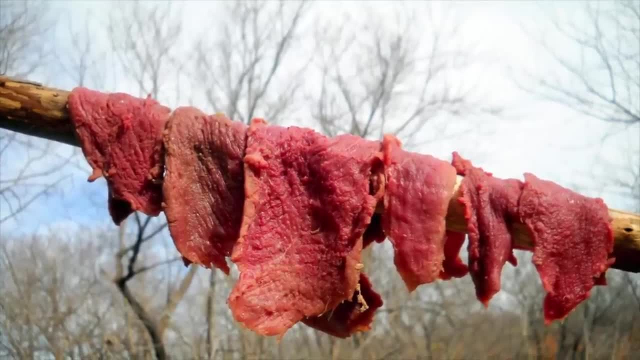 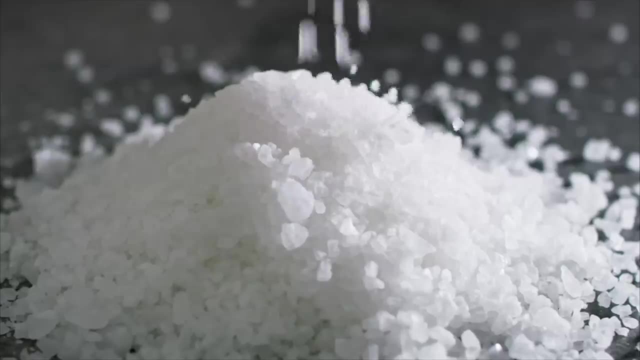 Meat can simply be air-dried in the right conditions to preserve it. Neanderthals could have simply hung their meat over a fire, which is a very effective way to preserve it. It is a very effective way to preserve it. Salt may have been used, but it is hard to come across in significant quantities in. 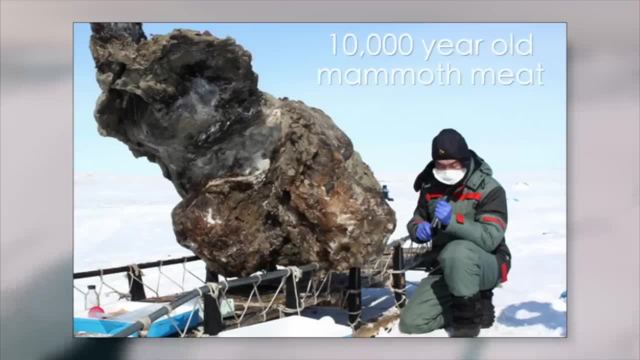 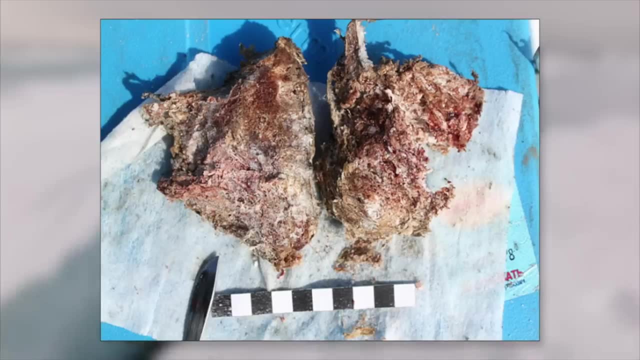 many places. If it was cold enough outside, meat, of course, could have just been frozen. It could have stayed frozen for many months during glacial periods, possibly even in the summer, depending on how cold the period was. Meat may have also been fermented. 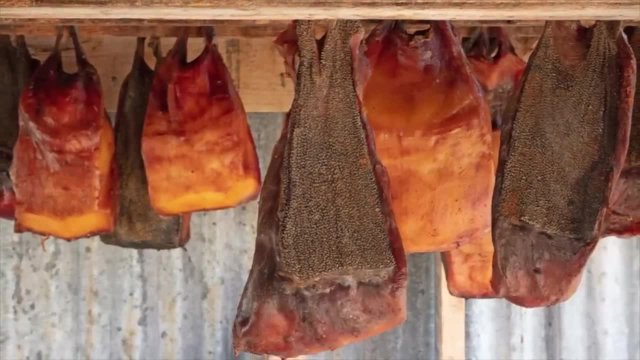 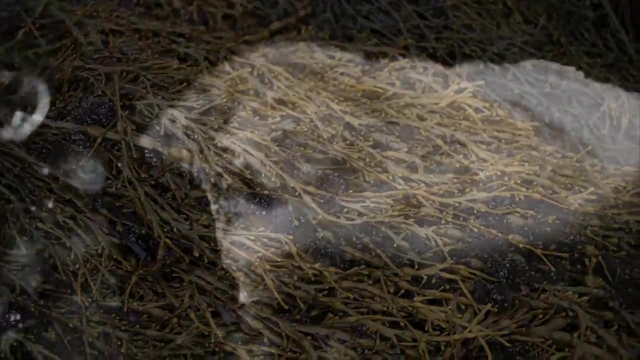 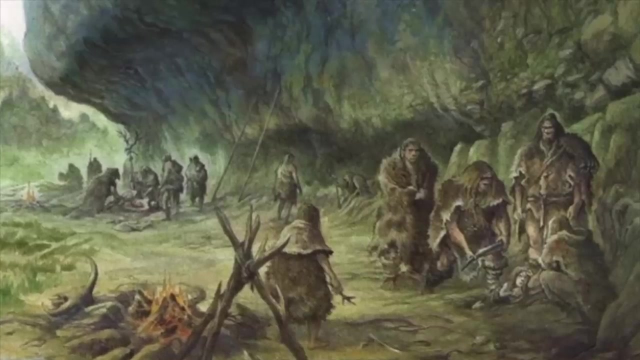 Many recent indigenous peoples fermented meat and other foods At Cueva de los Aviones, Spain. the remains of shellfish and seaweed may indicate that water-soaked seaweed was being used to keep shellfish alive or to keep them fresh. There are many ways which Neanderthals may have preserved their foods and our evidence. 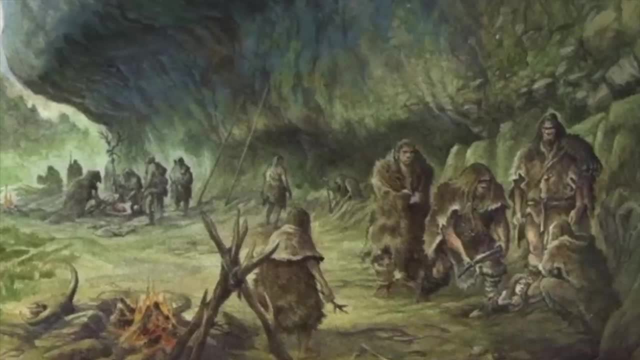 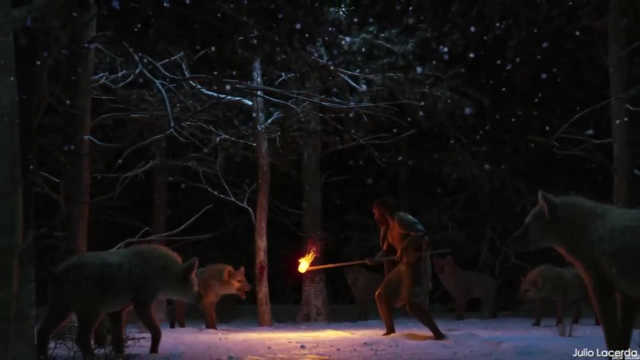 does suggest that food preservation may have been going on. By procuring all these food resources, Neanderthals made themselves a target for carnivores and scavengers. Neanderthals were a dynamic part of their wider ecosystem that we cannot overlook. 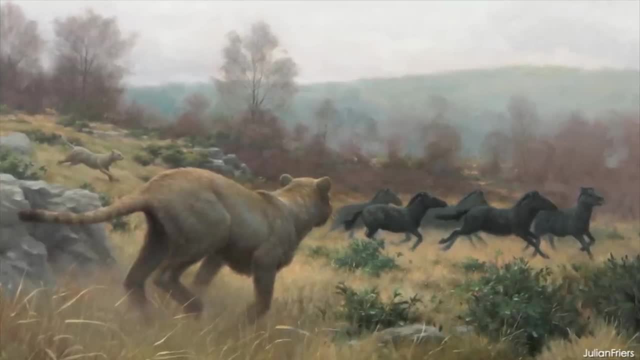 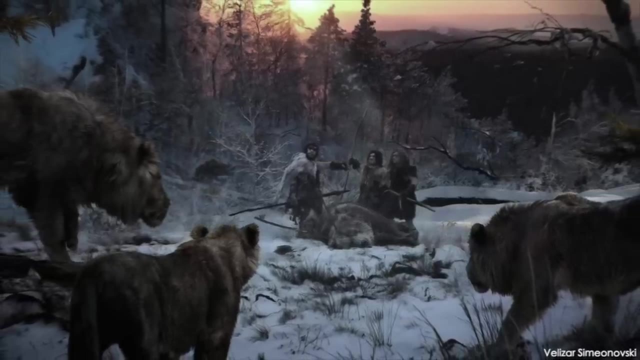 Cave lions as big as the biggest tigers, target Tigers, targeted horses, large deer, aurochs and bison. Brides of such lions would have certainly been a threat for any Neanderthals butchering prey. Homotherium, also known as the scimitar cat, hunted young mammoths and other fairly large 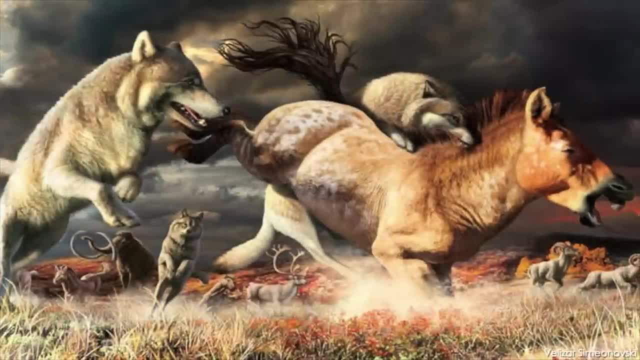 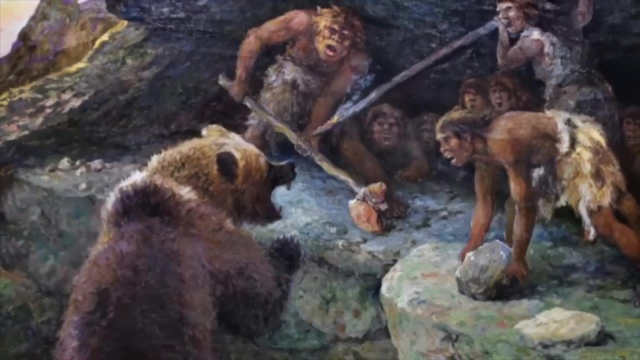 game. Wolves and leopards hunted a variety of prey. Multiple species of bear would have ran into Neanderthals on many occasions. Bears may have attempted to steal carcasses from Neanderthals or even target individuals. The species of bear is known to be the most aggressive of the Neanderthals. It is believed that the Neanderthals were the most aggressive of the Neanderthals. Bears in general do not typically target humans as a food source, though surprise encounters or defensive mothers often trigger attacks. The massive cave bear stood 3.5 meters, or nearly 12 feet tall. 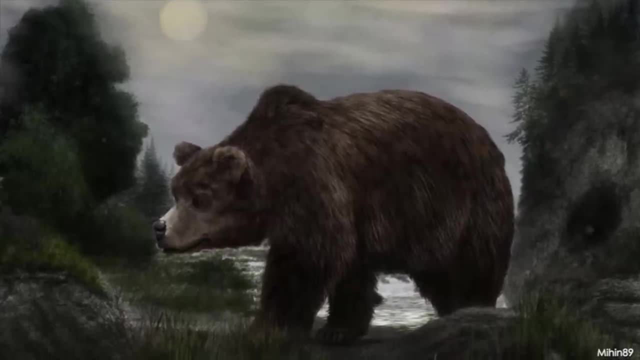 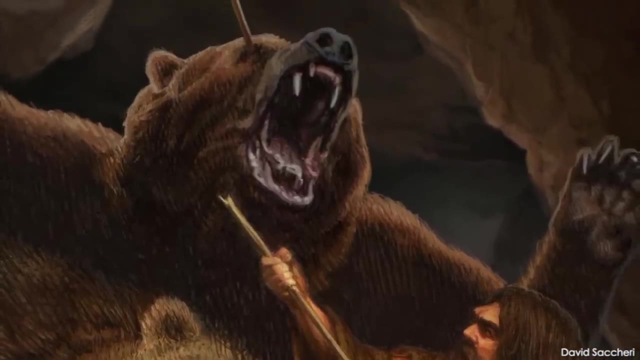 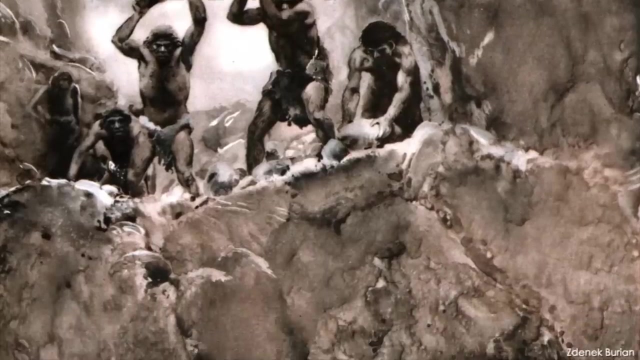 They also weighed up to 1,000 kilograms or 2,200 pounds. As their name suggests, they would have competed with Neanderthals over cave space. Other bears like the brown bear and the step bear also occupied caves. Bears are vulnerable while hibernating and may have actually been more of a food source. 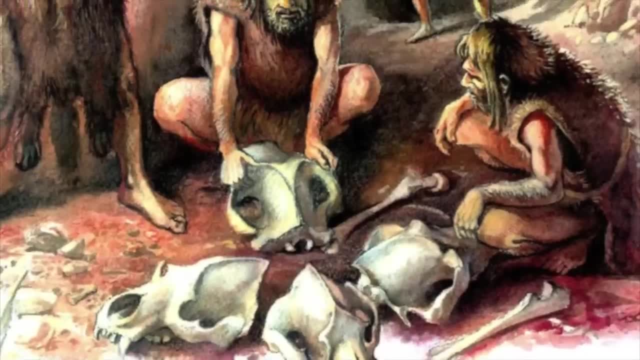 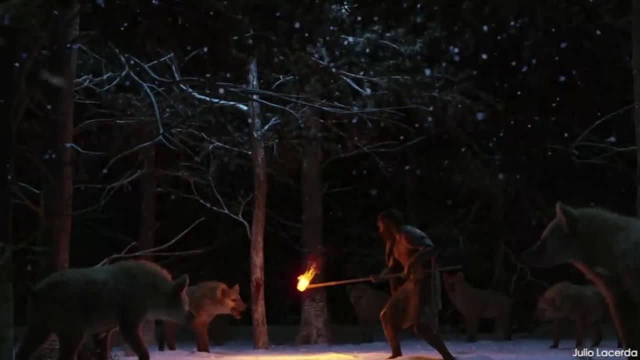 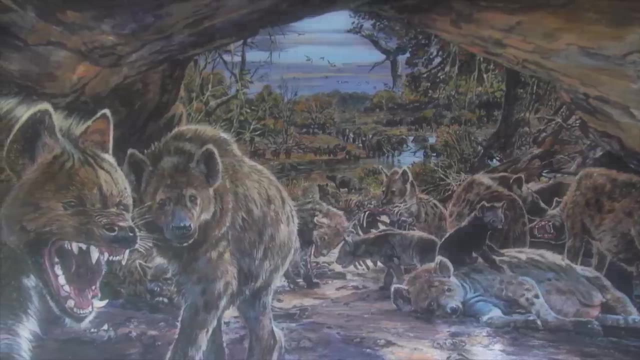 than a competitor in the winter. Some remains even indicate that bear hunts may have been a cultural practice among some groups. Another predator that Neanderthals would have frequently ran into were cave hyenas. Neanderthals and cave hyenas had very similar niches, though they may have exemplified niche. 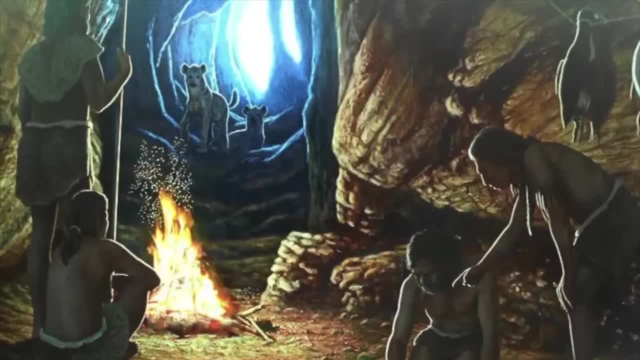 differentiation. They would have been able to find their prey in the same place, but they would not have been able to find their prey in the same place, Though, going after the same prey and living in similar places, they may have exemplified the same thing. 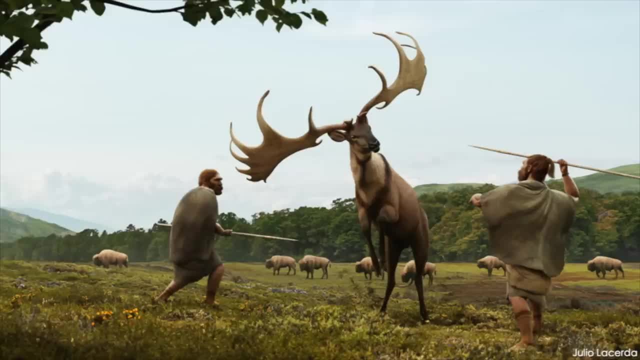 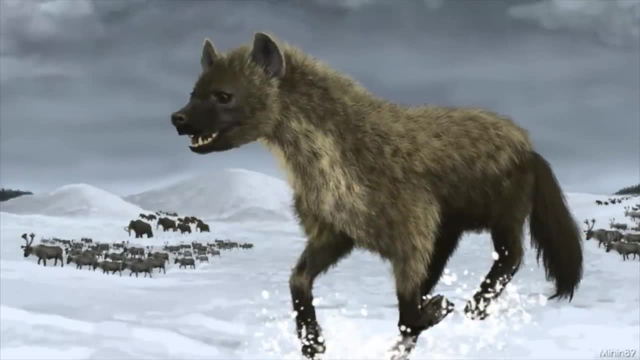 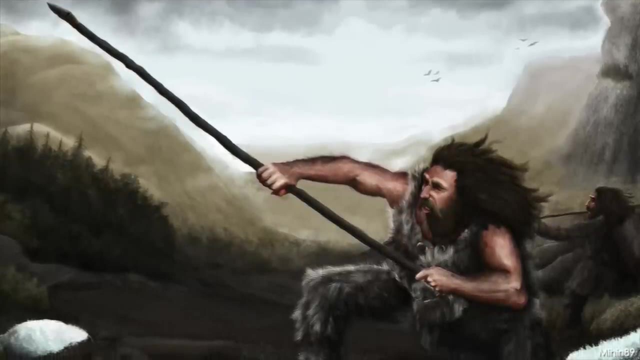 They may have actively avoided each other. Animal remains from Neanderthal caves indicate that they targeted prime individuals, while hyenas hunted weaker and younger prey. Nonetheless, hyenas are often known to steal kills from other animals with intimidation tactics. Remains of Neanderthals even indicate that they were either preyed upon or scavenged. 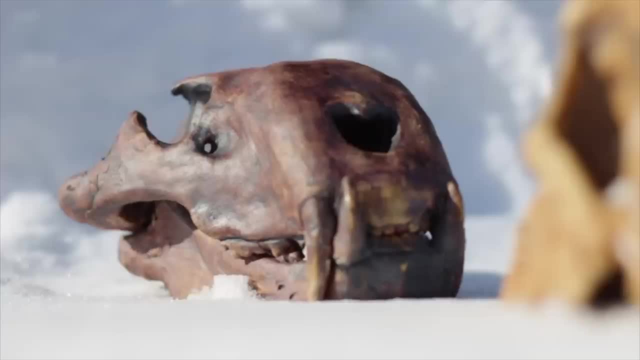 by these powerful beasts from time to time. With a world full of hungry beasts, Neanderthals certainly had a lot of fun. They were also very active in the wild. They were very active in the wild. They were also very active in the wild. 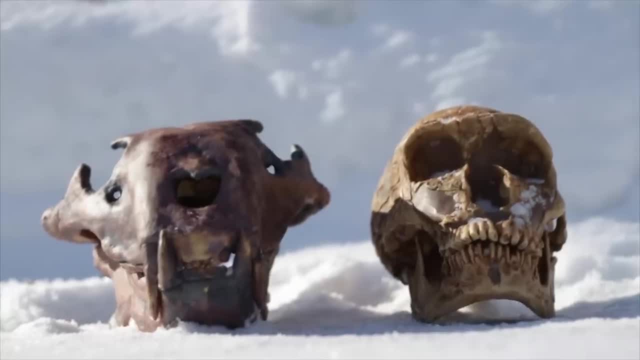 They were very active in the wild. They were also very active in the wild. They were very active in the wild. Cameros2016 looked at 124 Neanderthal specimens and analyzed the source of their skeletal trauma. Cameros2016 looked at 124 Neanderthal specimens and analyzed the source of their skeletal 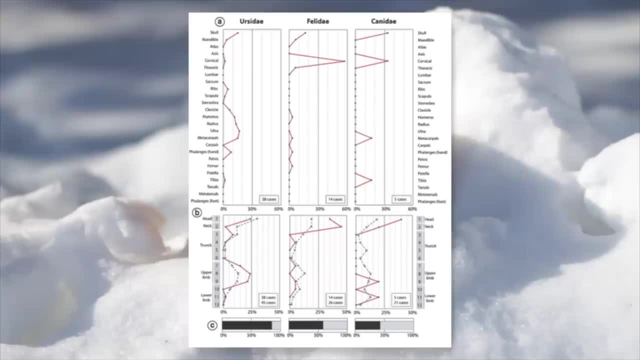 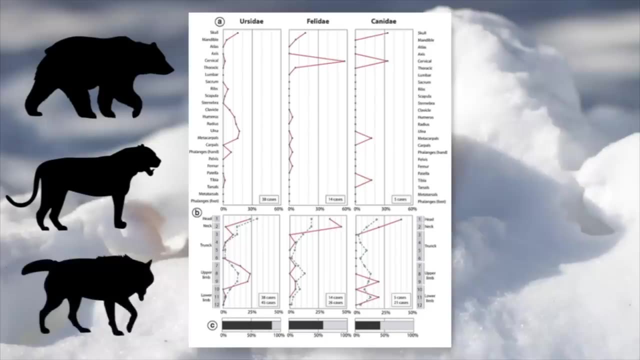 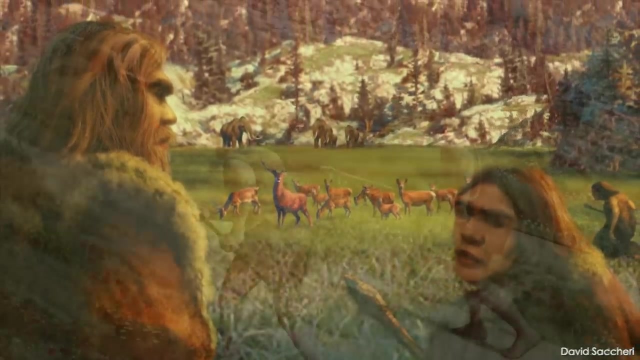 trauma. 36% were victims of bear attacks, 21% were attacked by big cats. 17% had evidence of wolf attacks. Interestingly, none of this sample were victims of hyenas, though other Neanderthals certainly were. These conflicts may have happened for a number of reasons, and many of them are possible. 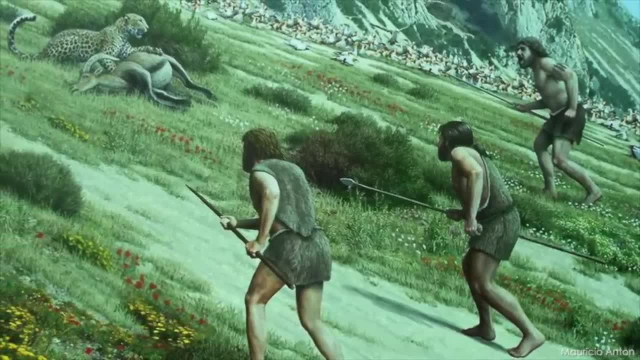 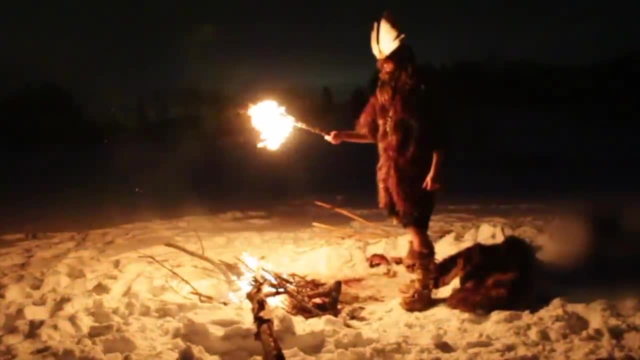 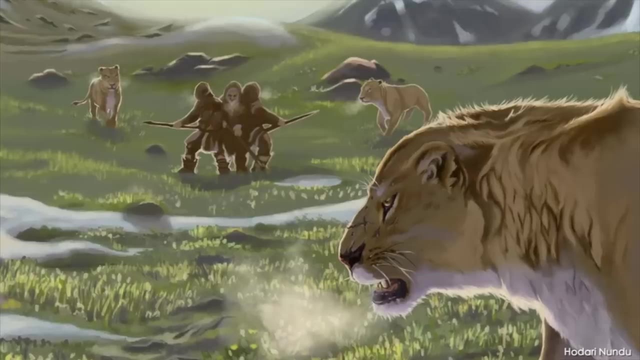 number of reasons, and many likely involved carcasses. With such stiff competition, Neanderthals certainly had ways to defend their kills. They likely engaged in intimidation tactics such as yelling, arm waving and stone throwing. It is possible that they even lured carnivores to their kill sites to also target as prey. 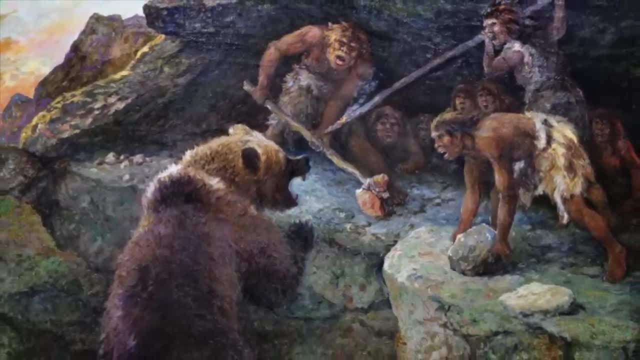 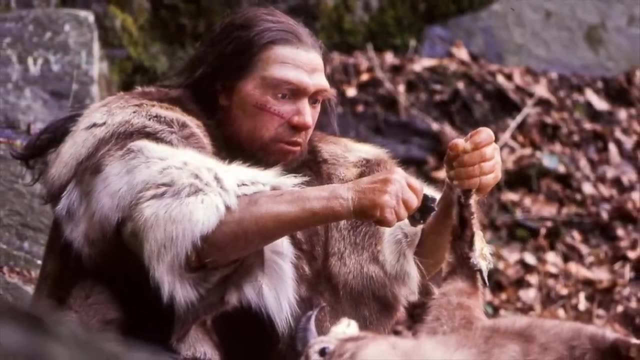 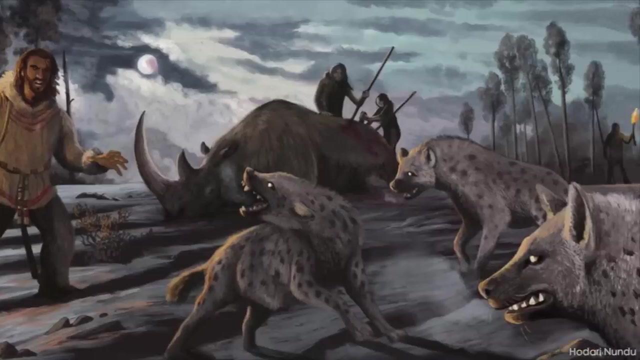 This may explain why carnivore remains are found at their sites. Still, these animals are very dangerous. Being able to quickly harvest game would have been a necessity. Deer and other medium-sized game would have been dragged off, but larger game would have put them at higher danger of encounters with lions or hyenas. 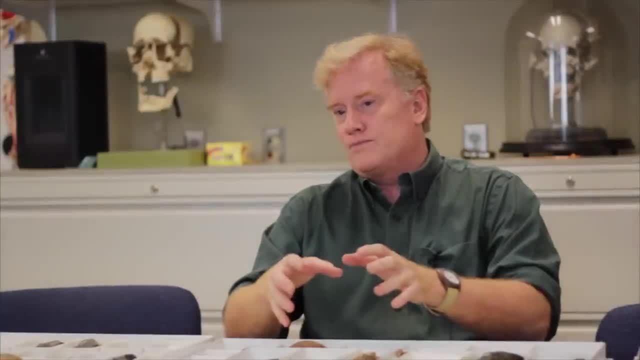 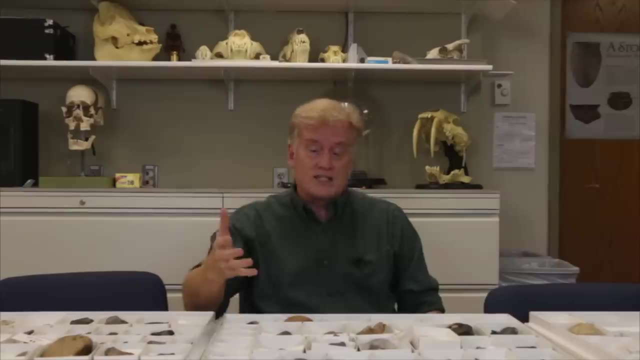 We would think that, in fact, the Neanderthals would come to the carcass, to the kill site, rather than dissecting the carcass and bringing it to their locations of residence, their base camps, which are frequently rock shelters and cave sites, as well as some open air sites. 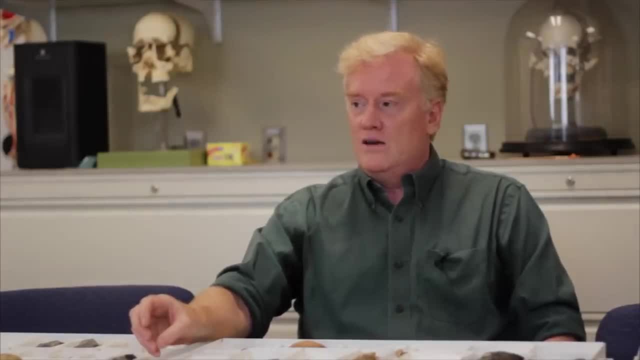 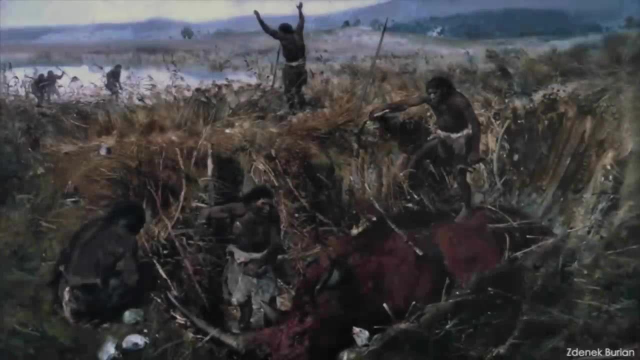 Modern humans. when they take large animals like that, they will bring the people to the carcass rather than bringing the parts of the carcass to the people. Campsites formed around large animal carcasses may have been nerve-wracking to live in, but 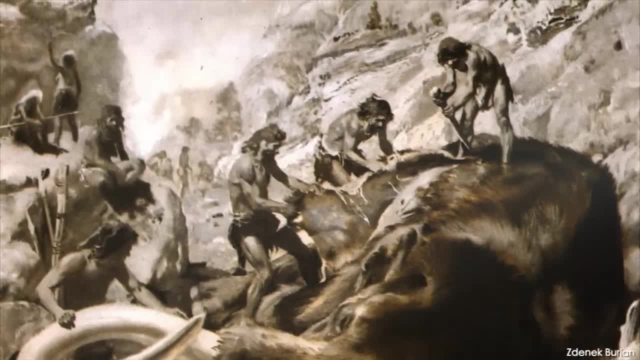 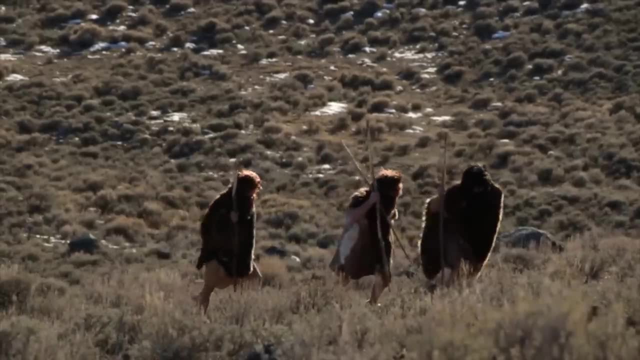 it would have been the most calorie efficient way to process a large animal. The idea of Neanderthal campsites conjures up questions about how they actually moved through the landscape. Neanderthals are most commonly pictured as cave dwellers. This is not just a stereotype. 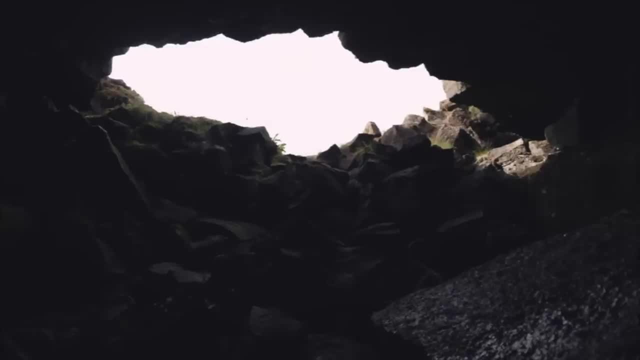 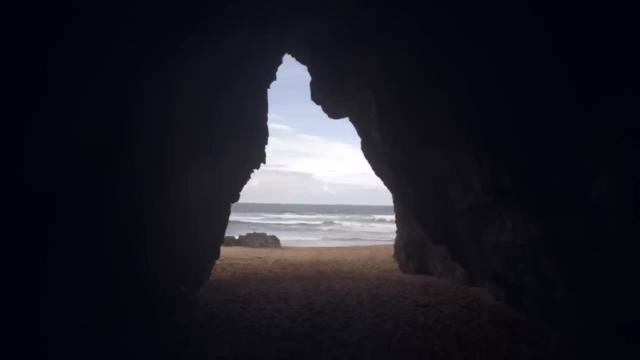 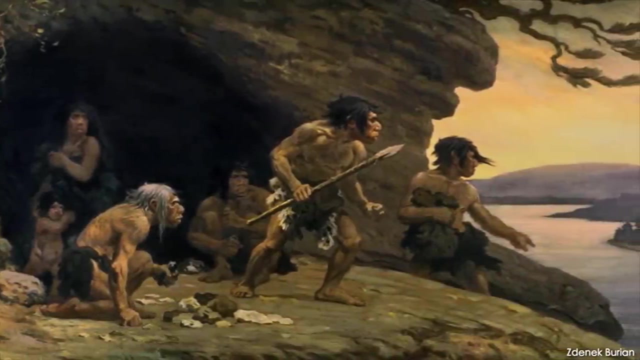 Caves were certainly heavily utilized, Though, due to their ability to preserve remains, they are over-represented. Depending on their structure, caves can provide protection from all sides and have a stable temperature. Fires were typically made near the entrance of the cave to, of course, prevent breathing. 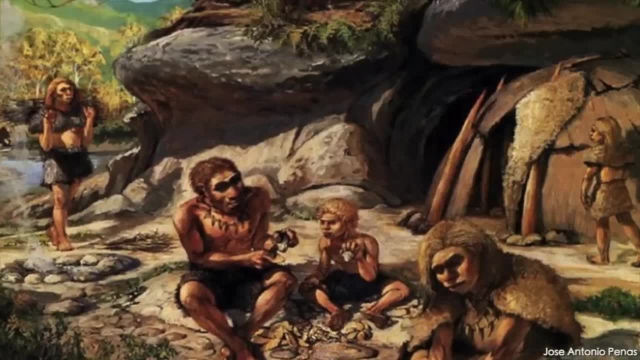 hazards. It is possible that some form of wall or barrier was put at the end of caves to keep the cold out and to keep any predators from coming in. Many caves at Neanderthal campsites were built in the early 1800s and early 1900s. 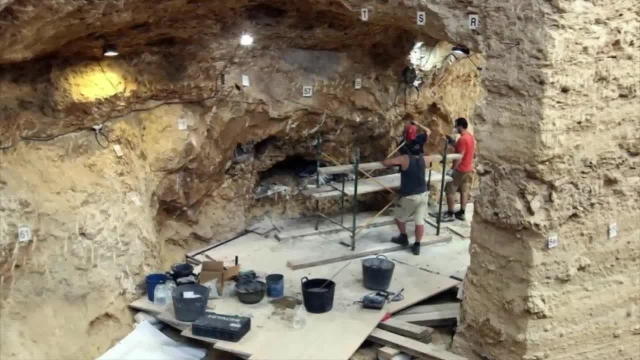 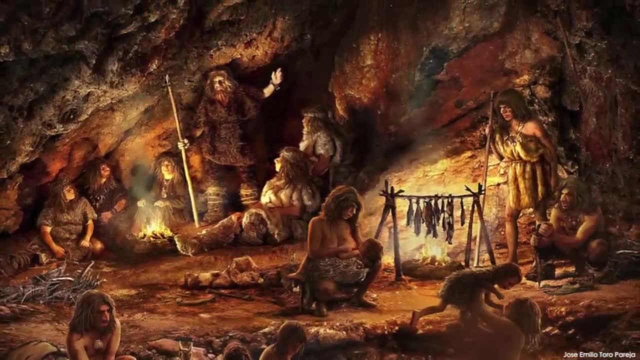 Many caves at Neanderthal campsites were built in the early 1900s and early 1900s. The structure that Neanderthals used had an obvious organizational pattern: Dedicated areas were designed for sleeping, napping, butchery and, of course, the hearth. 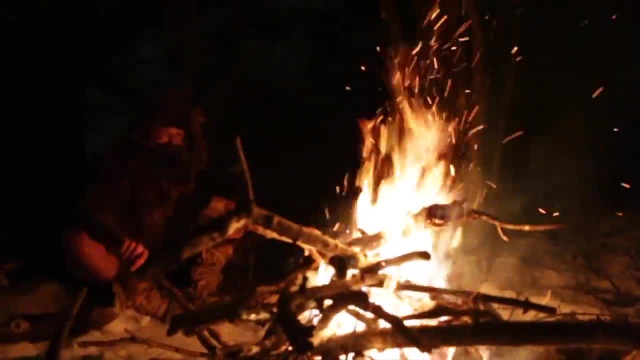 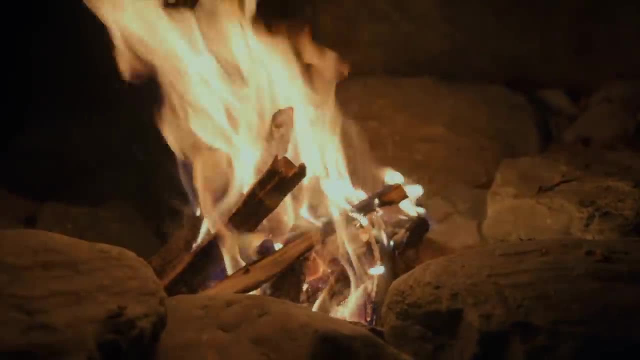 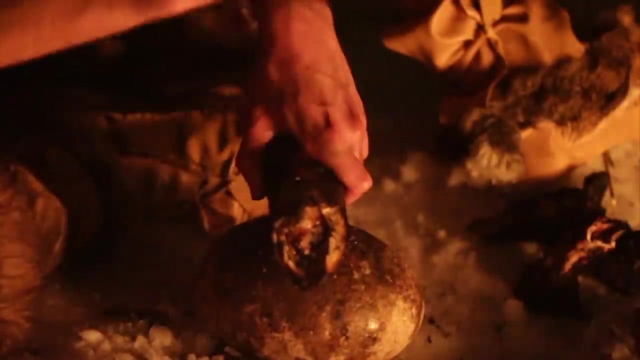 In some caves, specific hearths were reused for many generations. Some even have rocks around them that could have been used to contain the fire or maybe for butchery. Large blocks of stone are known from various Neanderthal sites. Some are surrounded with the remains of skulls, suggesting that they were used as an anvil. 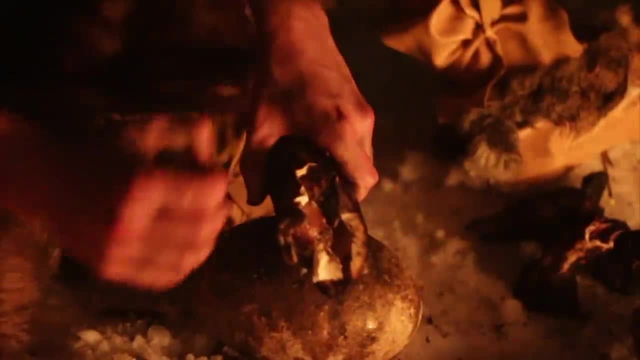 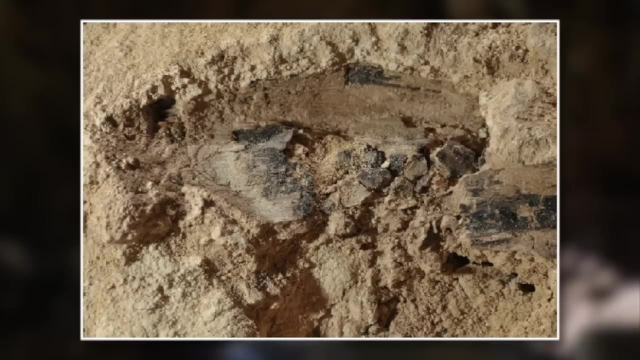 Some are surrounded with the remains of skulls, suggesting that they were used as an anvil. Others that are not near animal remains may have been used to sit on or perhaps to rub hides against Travertine from Abric. Romani has preserved the remains of large pieces of wood. 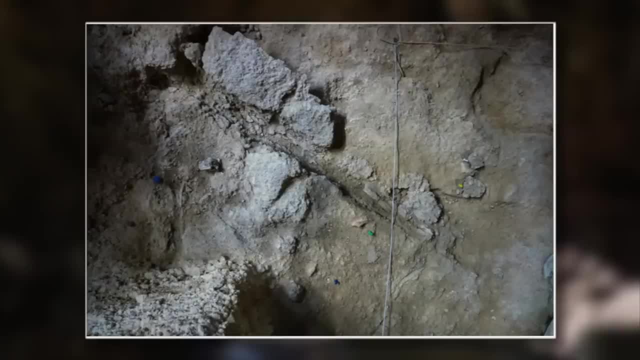 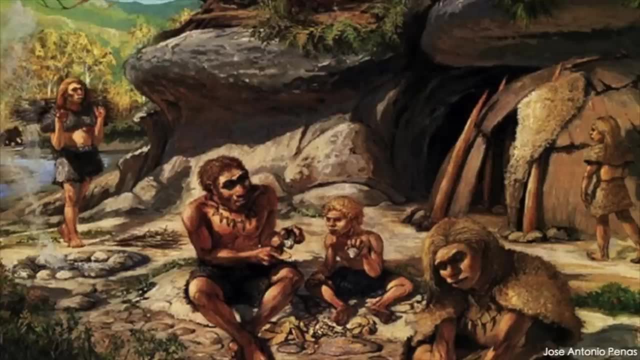 The wood may have been backup firewood, though it also may have been some kind of furniture or structure. Some caves have the remains of what seem to be post holes inside. Perhaps shelters were made inside of caves. There is also evidence that hides were placed on the inside of caves. 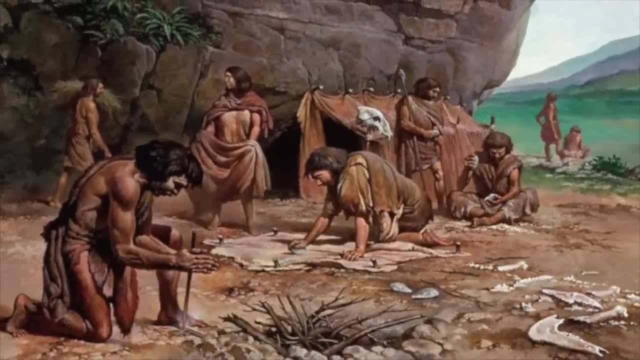 Some caves have the remains of what seem to be post holes inside. Perhaps shelters were made inside of caves. There is also evidence that hides were placed on the inside of caves, Perhaps the remains of what seem to be post holes inside. Some caves have the remains of what seem to be post holes inside. 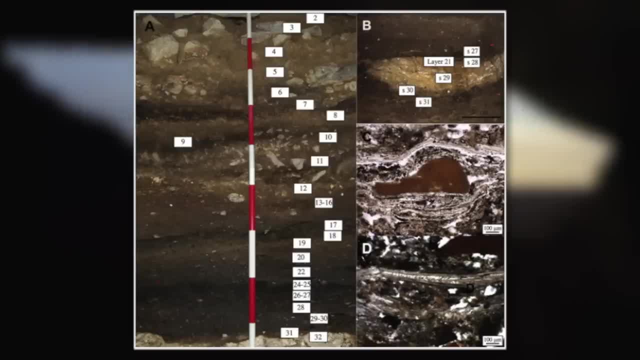 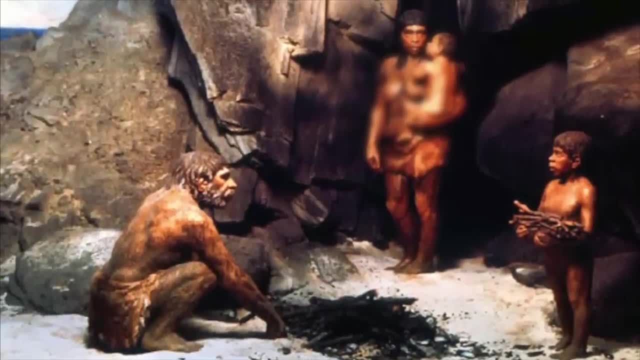 There is also evidence that there was a place that a expecting person had put them in so that it might have been their building. Other caves have evidence of grass beds nearby a hearth, which were likely used for sleeping. Images of cold rocky caves with Neanderthals crouching on a dusty stone floor may not necessarily 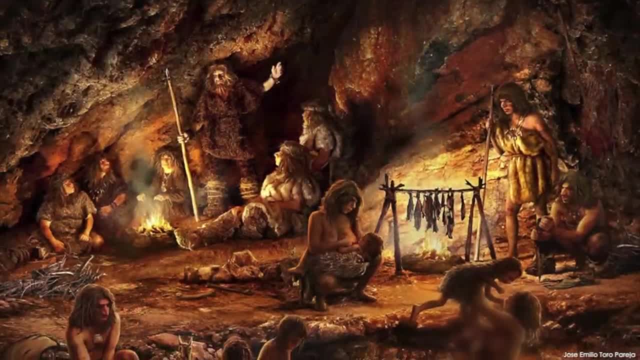 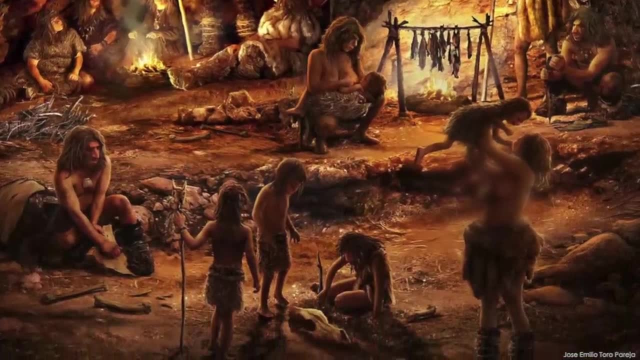 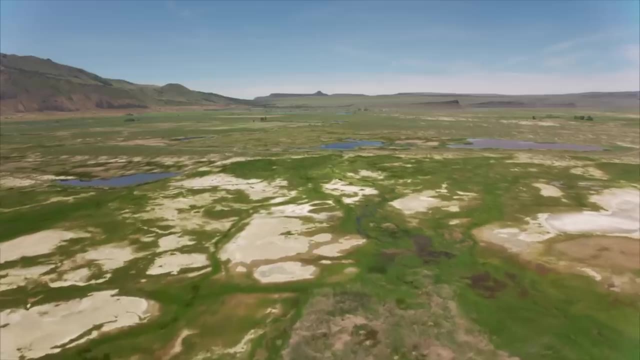 be very accurate. Instead, fire lit living spaces with tents, rugs and other furnishings may be a more accurate depiction of some of these caves. Though even well established caves like value principalmente have evidence of its existence, established caves like Abercrombie were only used temporarily. Neanderthals were highly nomadic and only stayed for a period of weeks, not months or years. Only so many animals exist in one area and once they were exhausted, Neanderthals moved on. Many animals also follow seasonal migrations and Neanderthals would have moved with them. A site in Spain known 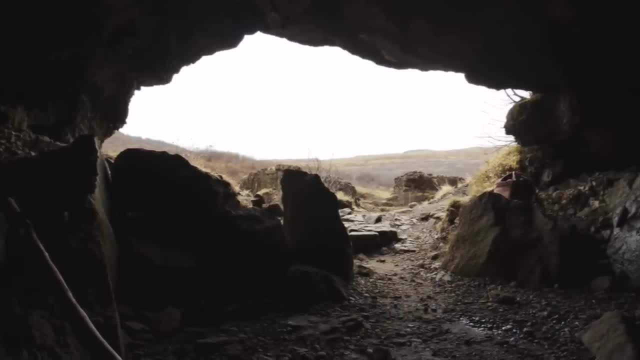 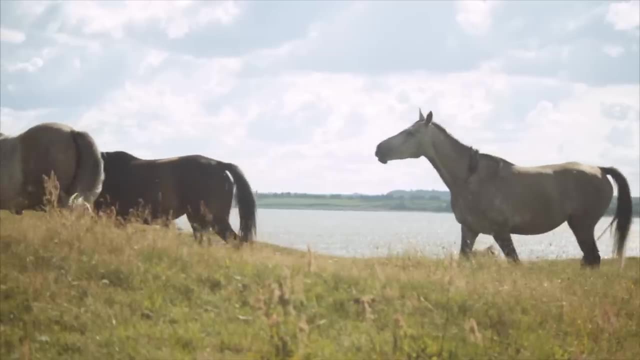 as Texenaires Cave may preserve a seasonal hunting camp. Horses are found at the site, but only during the late spring and early summer periods, A time when horses mate and are generally more vulnerable to predation. The site also had fewer hearths and stone. 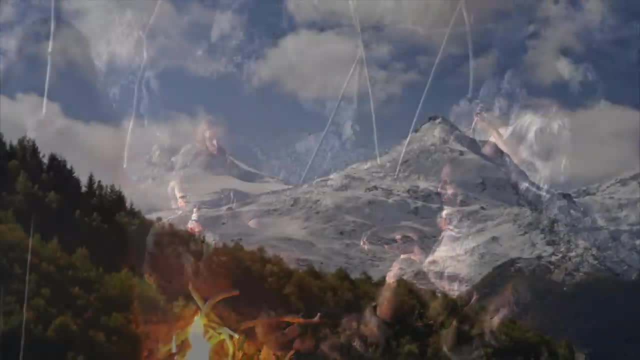 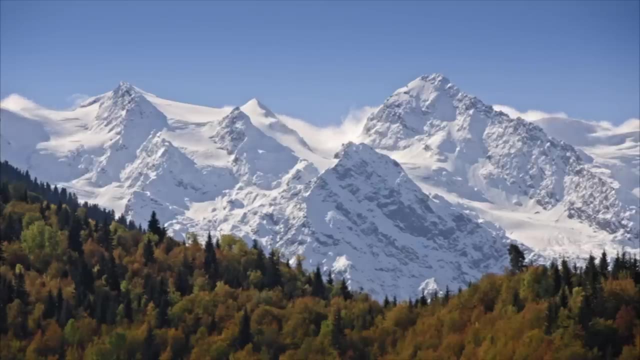 tools than we would expect from a Neanderthal home. The site seems to have only been stayed at for a few days at a time, certainly not a place where generations of Neanderthals grew up. Other sites also show individuals living in the area. 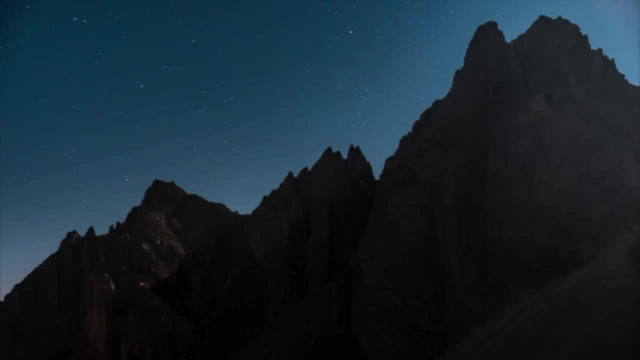 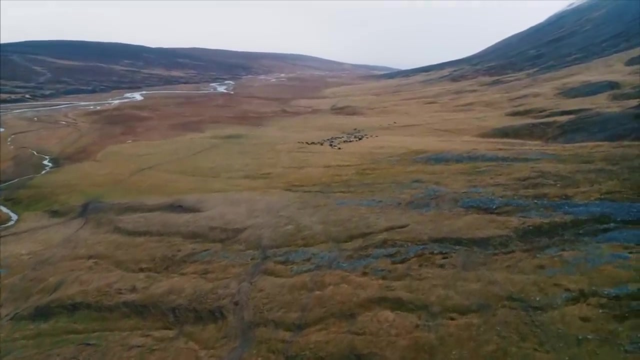 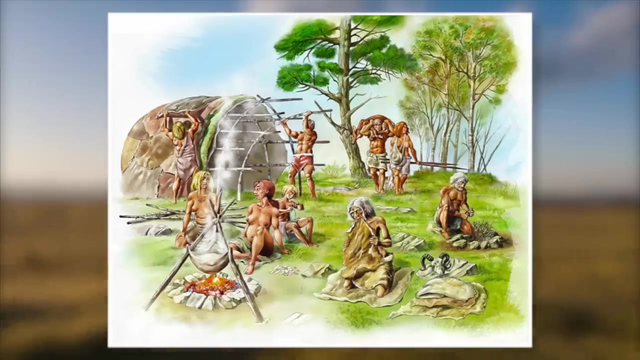 occupation periods that could have only been a couple of nights at most. Since there are not caves everywhere, Neanderthals would have certainly had to construct shelters. At the French site of La Folie, it appears that large wooden poles were rammed into the ground and supported with large stone blocks. The 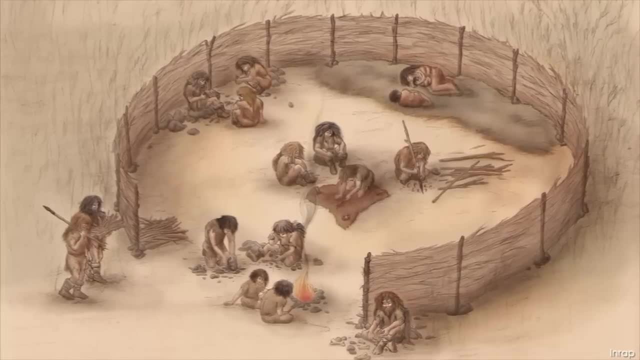 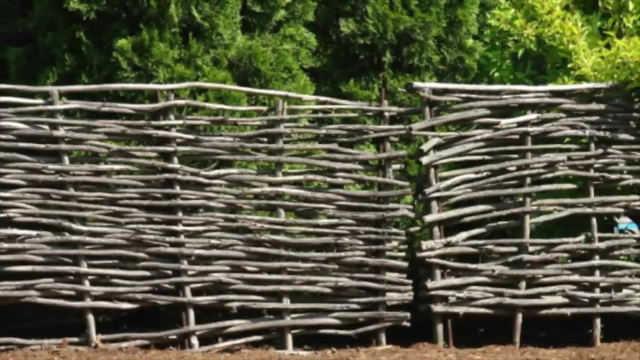 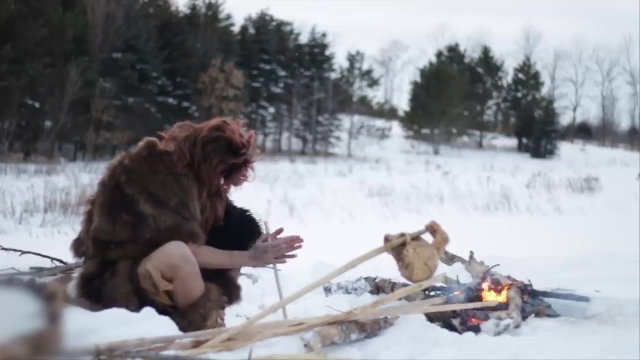 space was around 10 meters or 32 feet in diameter and was likely not roofed. Perhaps thin sticks were woven between the large poles to create a wall to protect from wind and predators. Within the structure there is evidence of different areas of activity, including a butchery station, leather working area. 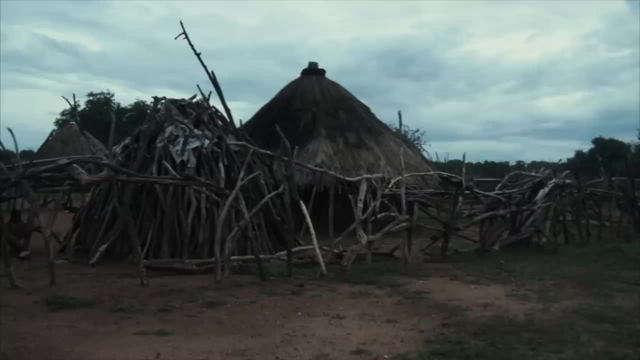 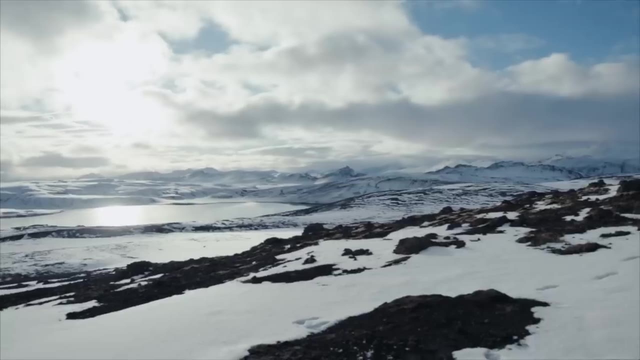 flint, knapping space and a bedding area. Even though they had to invest a lot of time making this structure, they only seemed to have stayed for a few weeks at most. At another site in Ukraine, a ring-shaped structure made of mammoth. 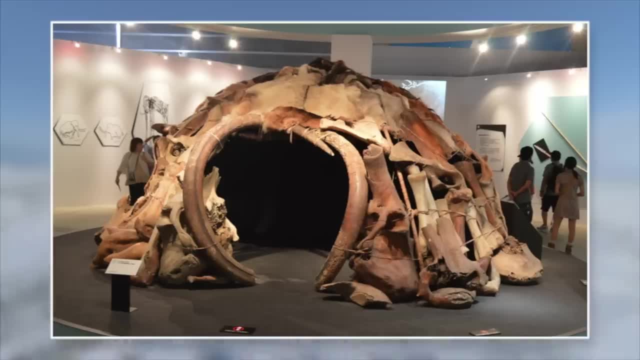 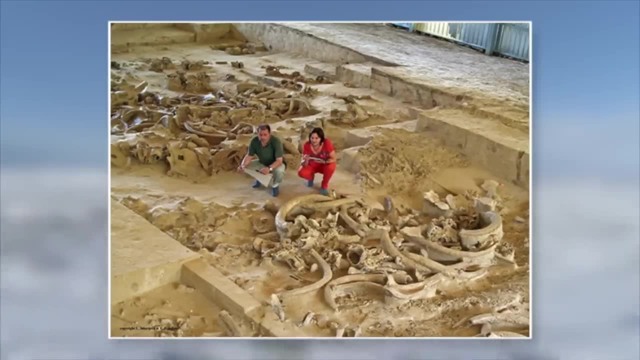 bones was found. It was 7 by 10 meters or 23 by 33 feet. It contained hearths, a crafting area and a cooking area. This structure is similar to later modern humans from the Russian plains With little wood to go. 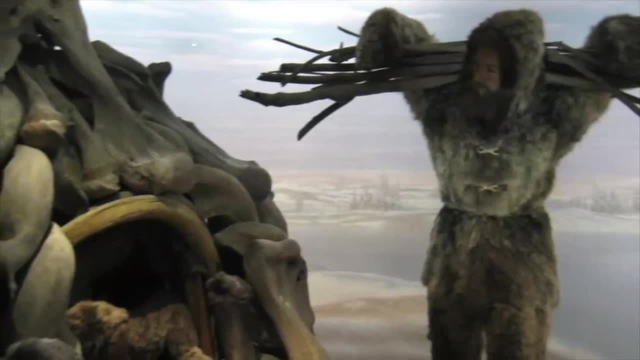 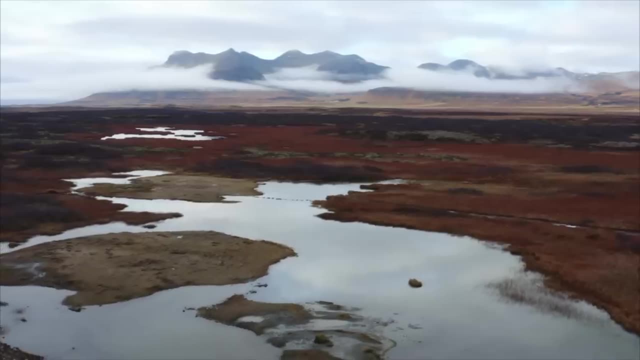 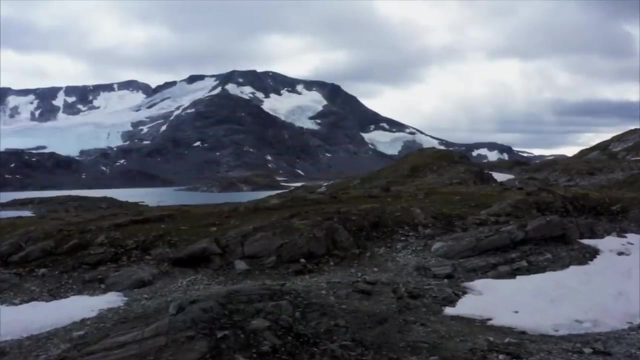 around mammoth bones were some of their only building materials. It is unlikely that all of these mammoths were directly hunted, but some of them likely were. Neanderthals likely created many small shelters across their broad landscape. that would not necessarily preserve any evidence in the fossil record. A simple 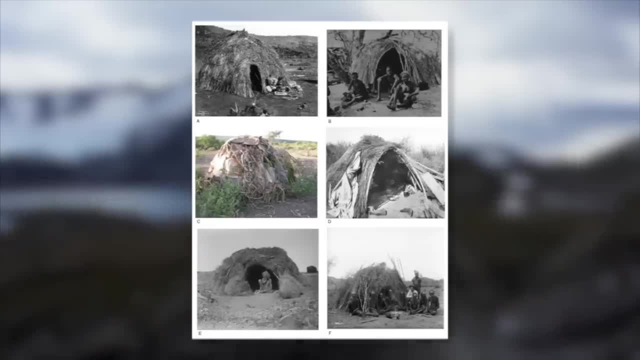 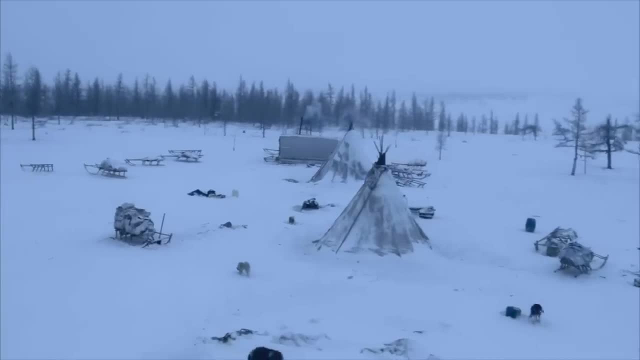 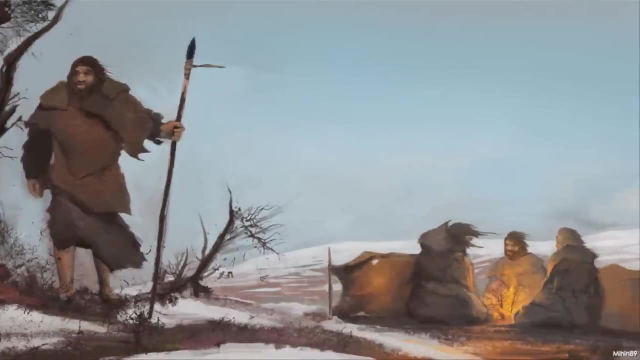 shelter made of sticks and shrubs would not leave much evidence. Portable shelters such as teepees or hide tents may have been made. However, the large teepees that were made by the plains Indians required horses and dogs to be moved efficiently, Since Neanderthals had neither of these animals at their will, their portable 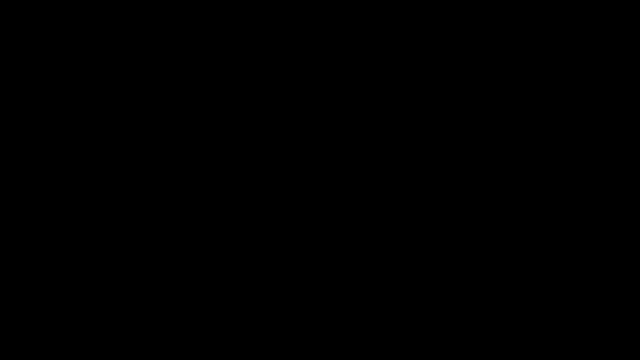 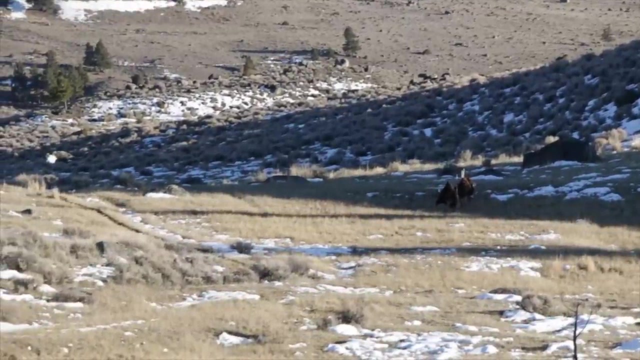 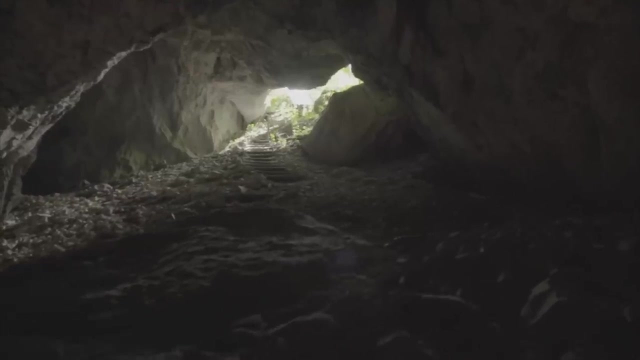 shelters would have been limited in size. Neanderthals seem to have moved across their landscape in yearly cycles from one shelter to another. Some sites were repeatedly returned to for thousands of years. Occasionally, some of these sites were abandoned for decades or even hundreds. 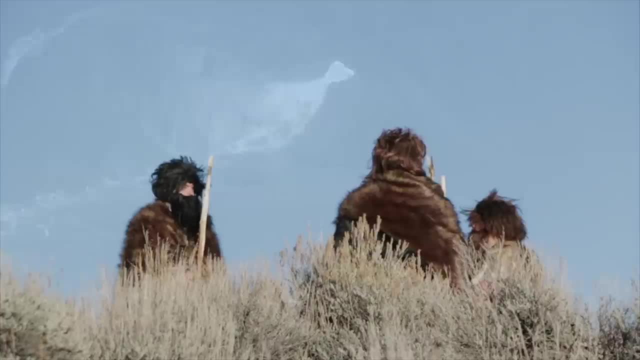 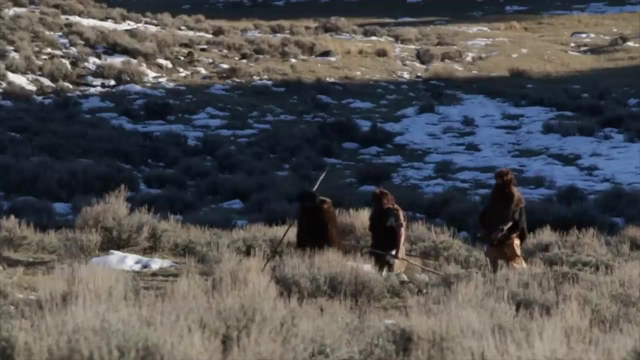 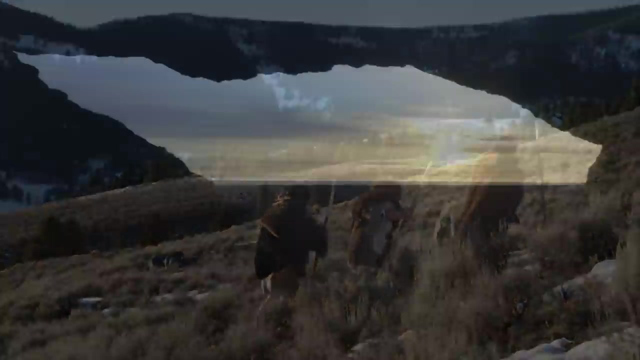 of years before being reoccupied. Perhaps their inhabitants died out or perhaps they found greener pastures elsewhere. It is hard to reconstruct their yearly cycle, but considering they returned to the same caves, there was certainly a rhyme and rhythm to their movement. Neanderthals did not seem very concerned with other 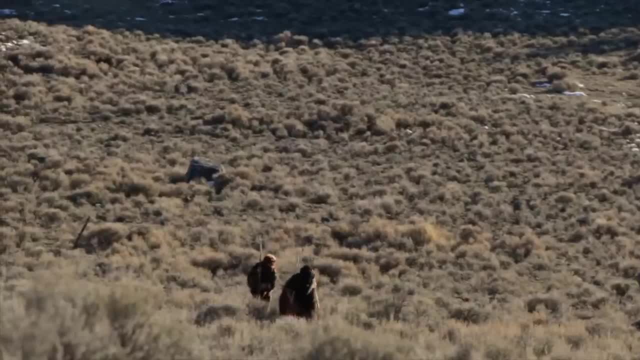 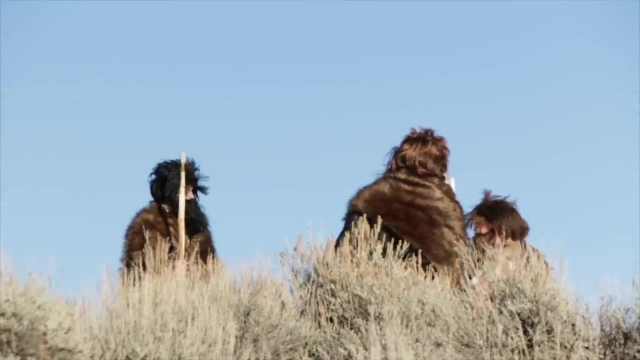 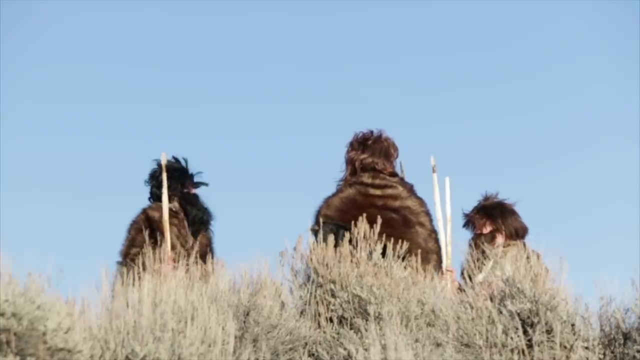 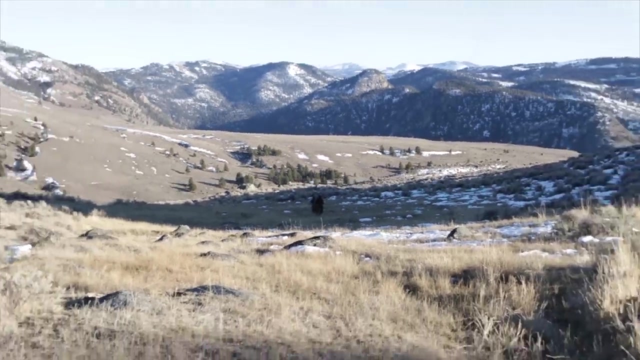 Neanderthals taking their caves. This is likely because Neanderthal populations were always quite low. Analysis of Neanderthal DNA suggests that Neanderthal populations hardly exceeded 10,000 individuals and never exceeded 15,000 individuals. Populations were separated into small, isolated groups, with some being fairly inbred. 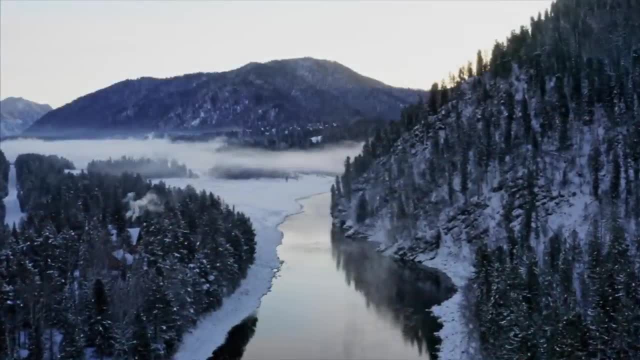 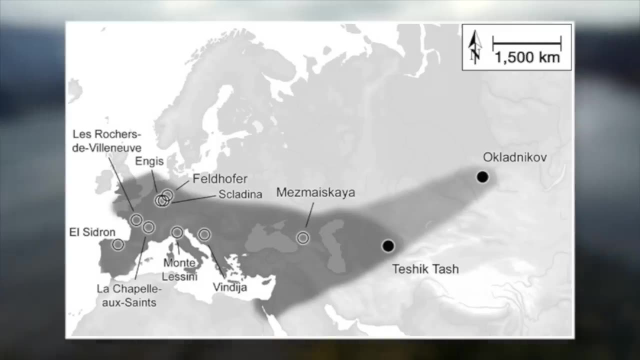 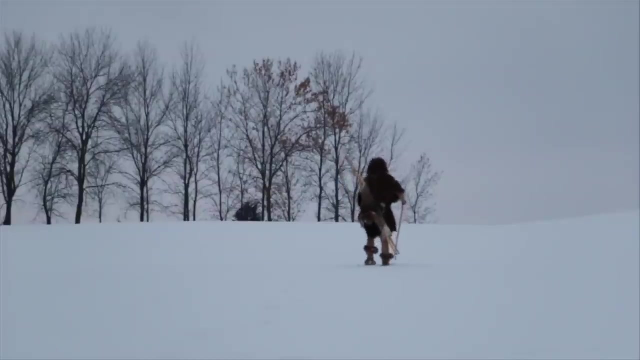 The Neanderthals had a massive range from Britain to Siberia to the Middle East. Their overall range was as much as 26 million square kilometers, or 10 million square miles. Despite their massive range, their population density was only 0.0002 individuals per square. 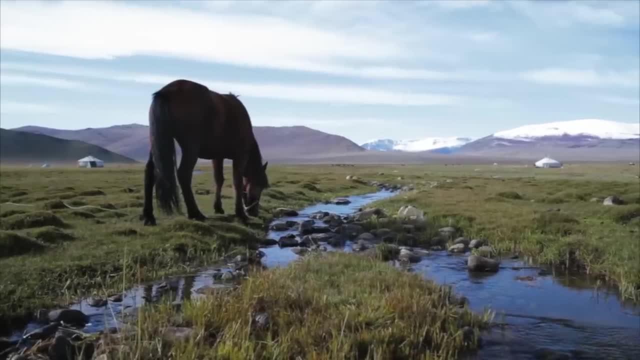 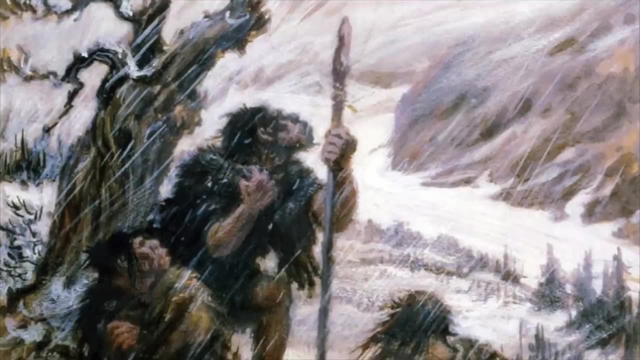 kilometer. Mongolia, the least populated country, has a population density of 2.07 individuals per square kilometer. To add to this, their population was only one-tenth of the size of the population of Homo sapiens, who would eventually move into the Neanderthals. 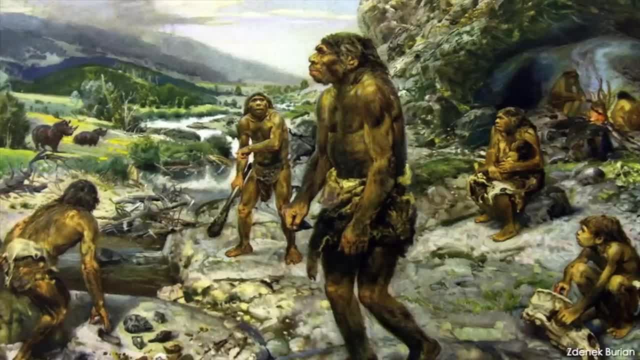 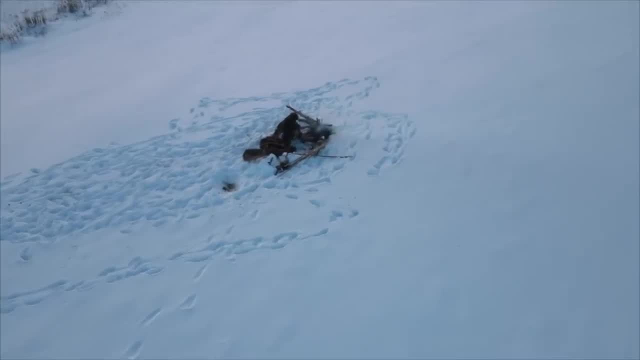 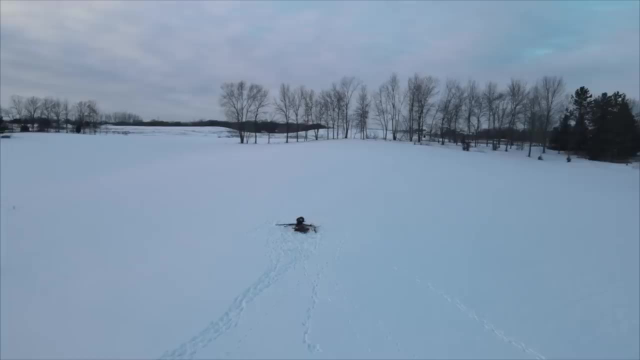 The only reason the Neanderthals were able to move into their territory was due to their high fertility and high infant mortality rates. This allowed for the proliferation of harmful gene variants, which in turn, may have kept the population low. We will talk about their population further when we talk about their decline. 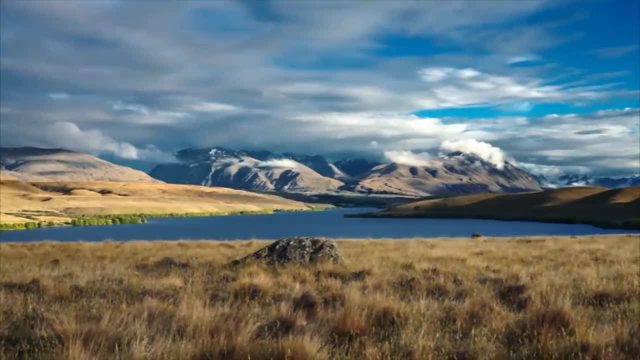 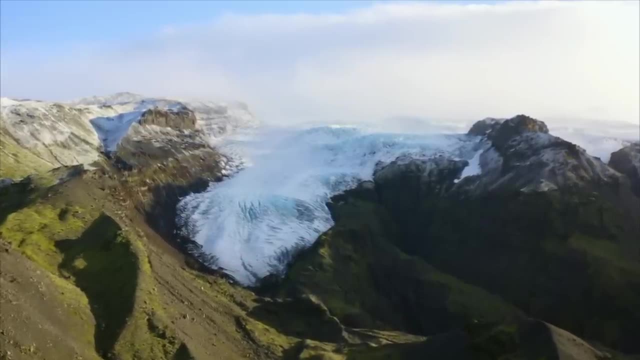 Another aspect about their world that we must consider is how it changed over a large time period. To give you an idea of where the population came from, First of all, there was no list of existing populations for roughly 2.5 million years. 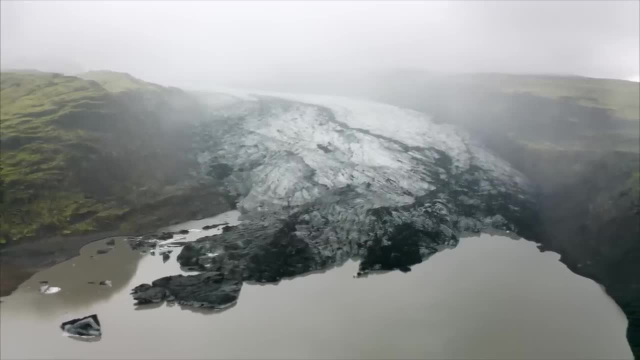 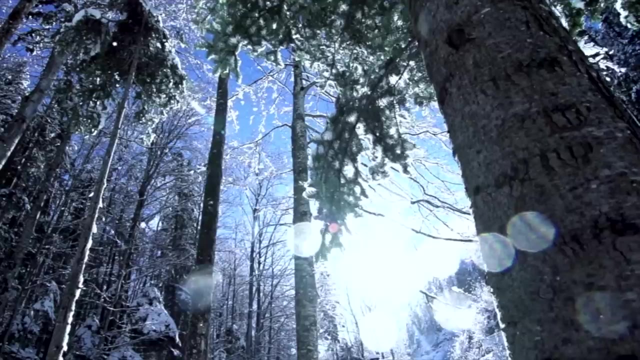 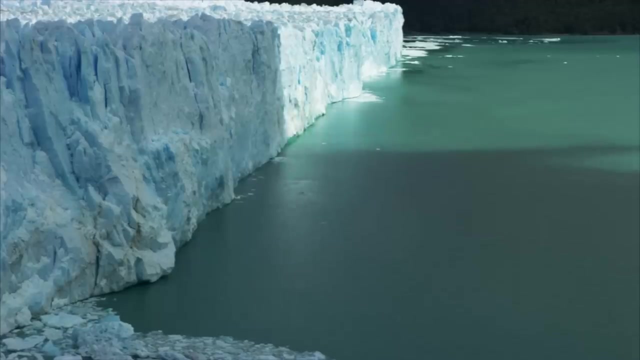 What most people think of when we talk about ice ages is the last glacial period. A glacial period is a cold period caused by variations in the Earth's orbit that affects how much solar radiation the Earth receives. The last glacial period lasted from 120,000 years ago to 11,500 years ago. 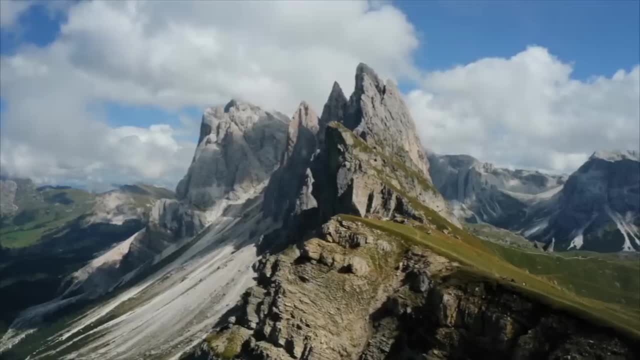 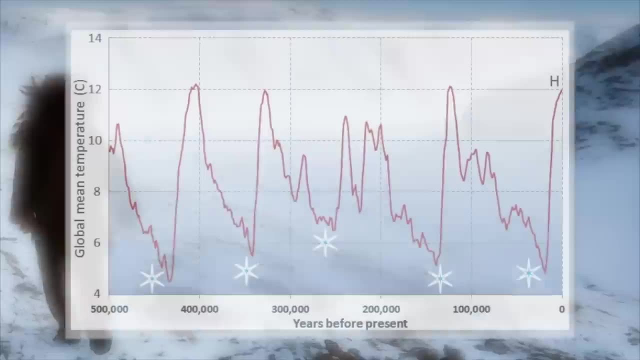 They are then followed by a warmer interglacial period. We are currently in an interglacial period. During the roughly 400,000 years of Neanderthal existence, four different glacial periods occurred, with four different interglacials between them. 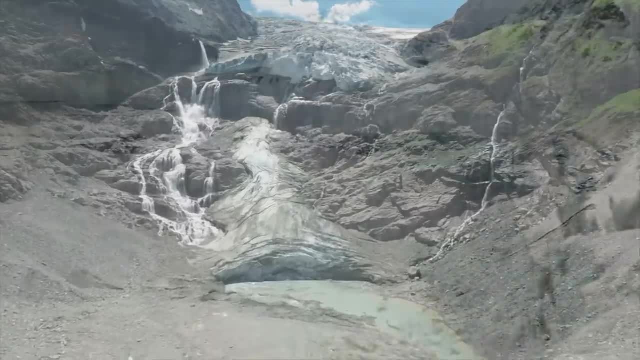 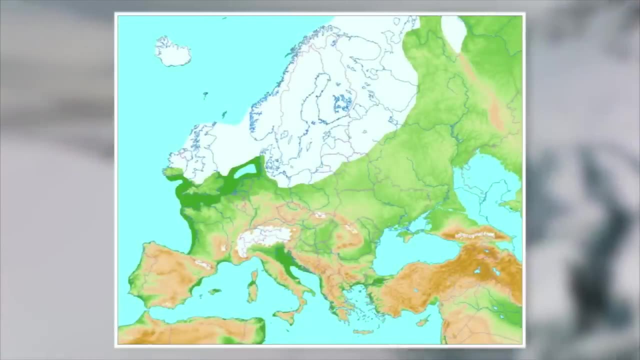 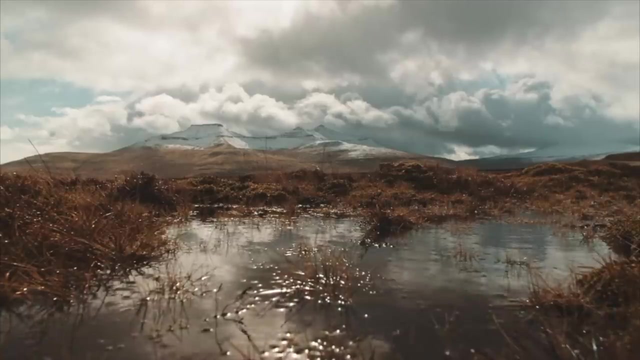 These periods are far too long to be noticeable within a lifetime, though. Neanderthal existence was undoubtedly dictated by these climatic changes. In glacial periods, northern Europe and much of the British Isles were covered by large glaciers. Central Europe was left as mostly barren tundra. 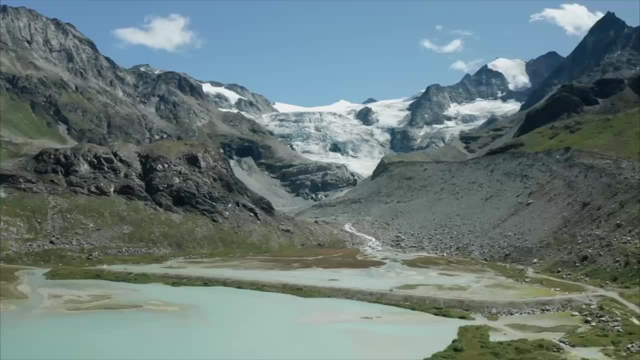 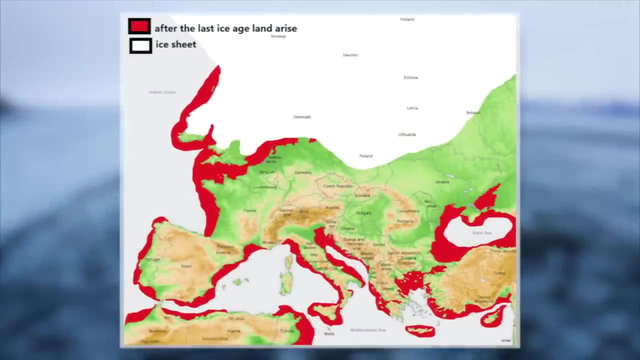 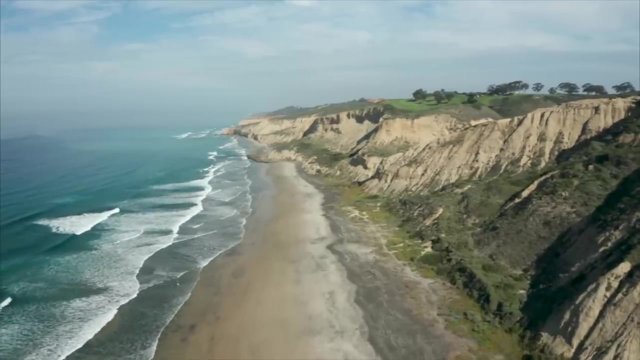 While the Alps were also covered in glaciers, Many Neanderthal populations were forced to move south Due to so much ice being locked up in glaciers. southern Europe swelled in landmass during these periods. Some islands could be simply walked to and coastlines everywhere expanded. Inversely, warmer interglacials would have allowed Neanderthals to move farther north, though territory would have been lost to rising sea levels. Interglacials in general were much more tolerable to live in. Neanderthals had greater success during these times. 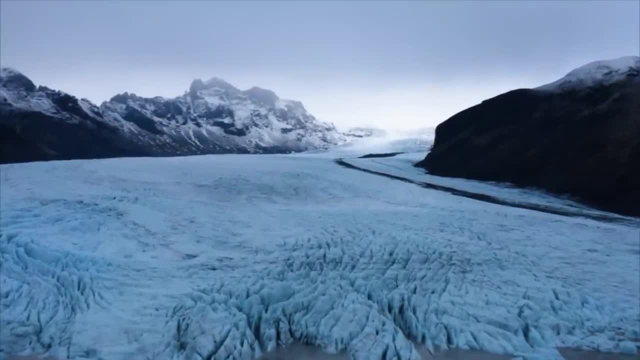 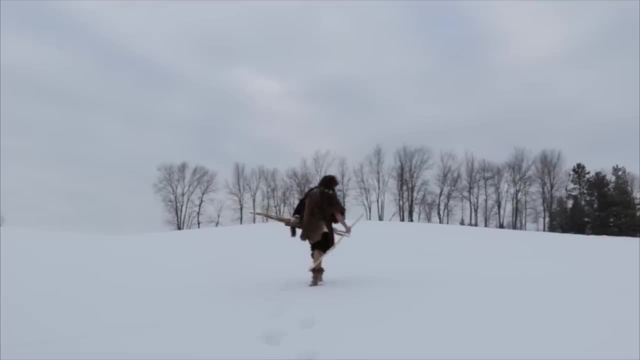 Understanding these climatic changes can help us understand the larger picture of Neanderthal life. The last aspect of their landscape that we must consider is: how did they actually move through it? Neanderthals were very adaptable and could live at sea level all the way up to relatively. 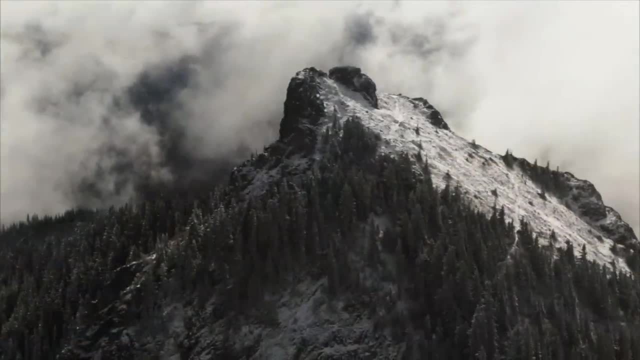 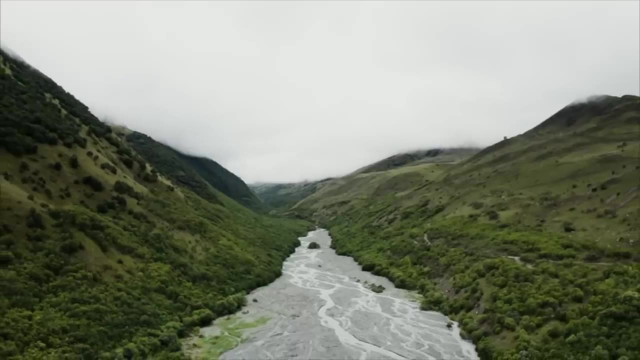 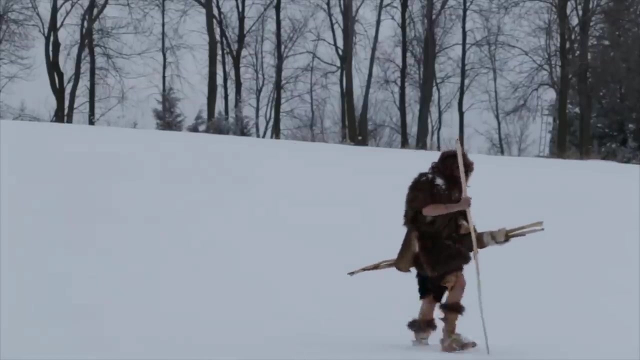 high altitudes. They were certainly not discouraged by high mountain ranges or low valleys. Just like modern human hunter gatherers- hunter-gatherers, they would have had a detailed mental map of their range. They would have been able to navigate many miles based on familiar landscapes. and perhaps the stars, Stars must. 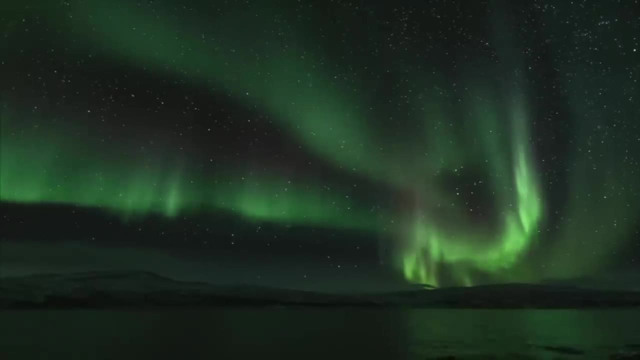 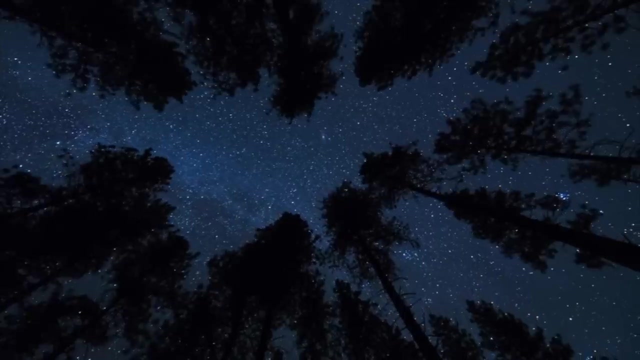 have been a thing of wonder for these people. Perhaps a symbolic meaning was attached, or maybe they were even seen in a more practical light. Regardless, we know that they would have been very familiar with them, and navigation is a possibility From analyzing how they use stone. 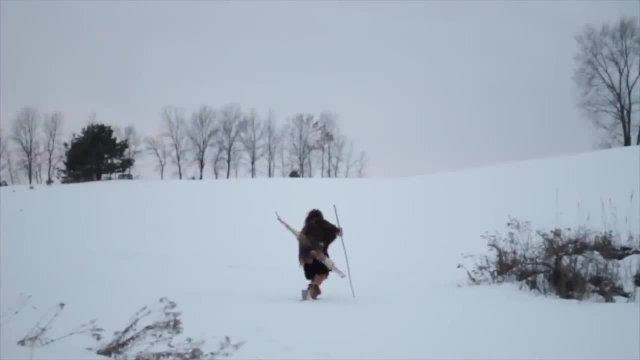 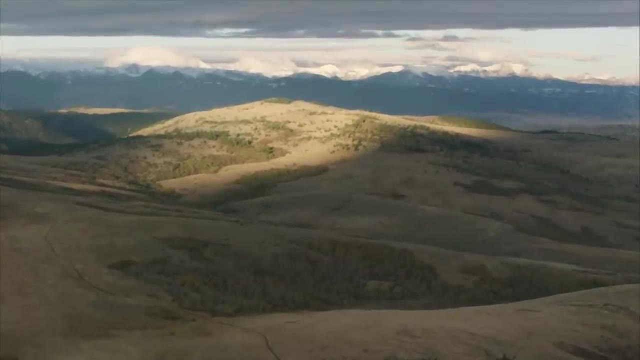 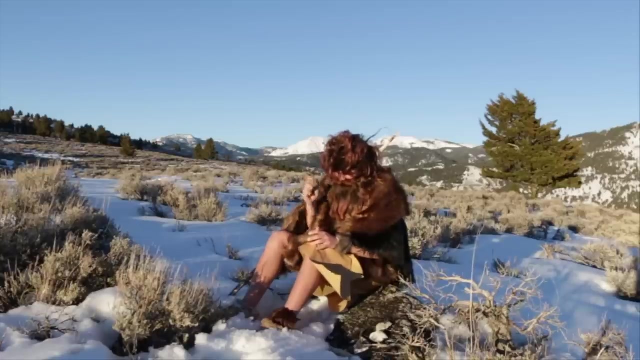 we can get a hint about how they moved through their landscape. From their sites, poor quality stone is usually sourced within about 5-10 kilometers or 3-6 miles. This range may represent their typical foraging area. once they reached a site, Poor quality stone was typically left. 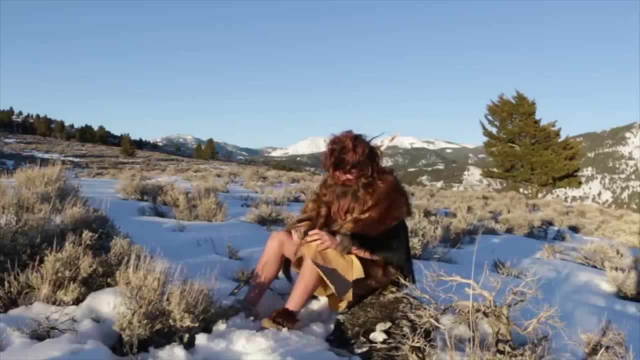 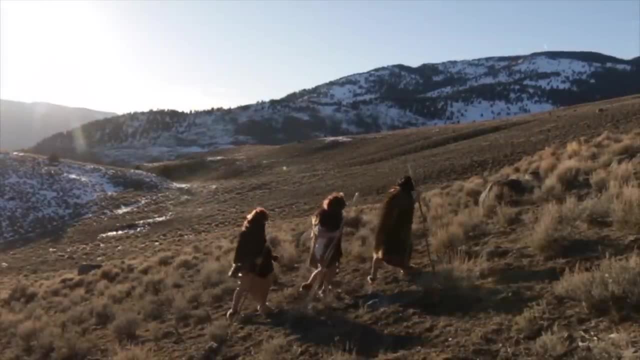 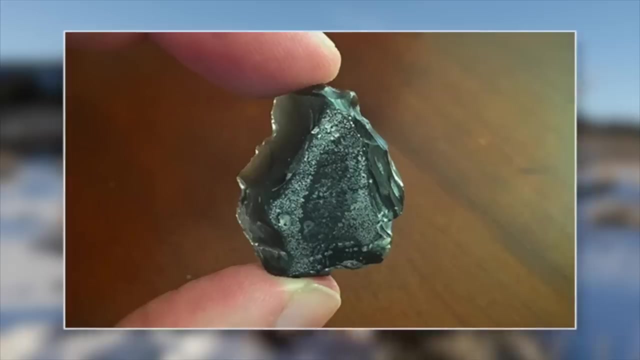 within this range after the Neanderthals left, Only high quality stone would have been carried. further. Quality flint was often carried more than 60 kilometers or 40 miles from its source before it was sourced. The highest quality flint and the sharpest rock obsidian were carried more than 300 kilometers or 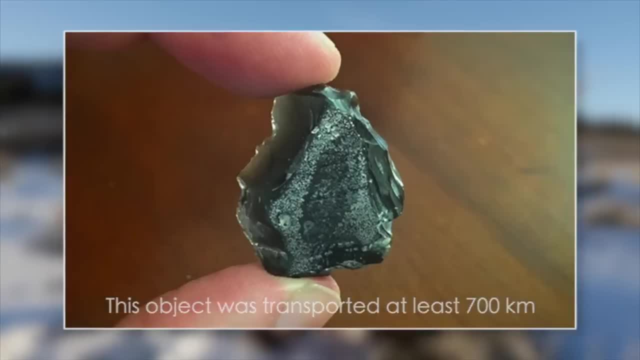 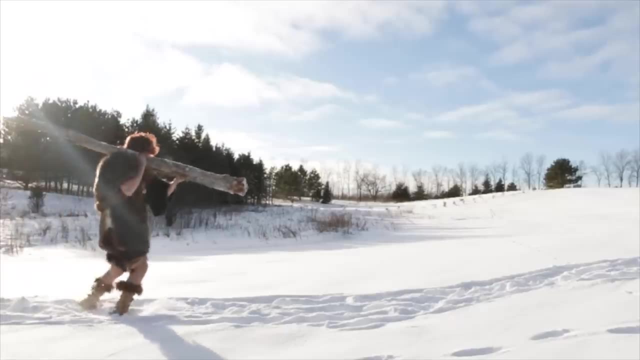 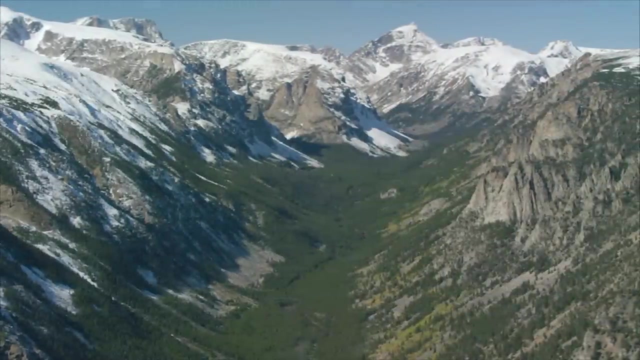 190 miles before being discarded. These tools may represent the existence of long-distance trade networks. Neanderthals likely did trade with other groups, though they were so nomadic that it is hard to rule out actual movement. Moving such distances would have required crossing significant obstacles. 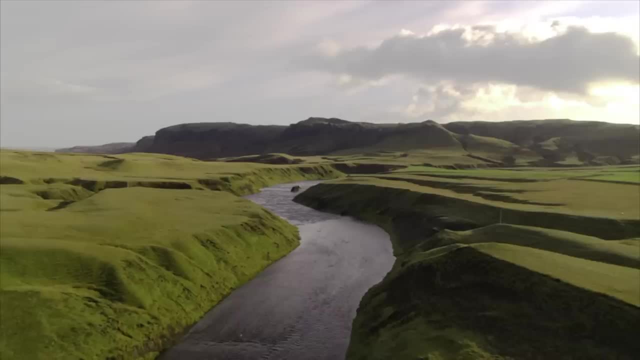 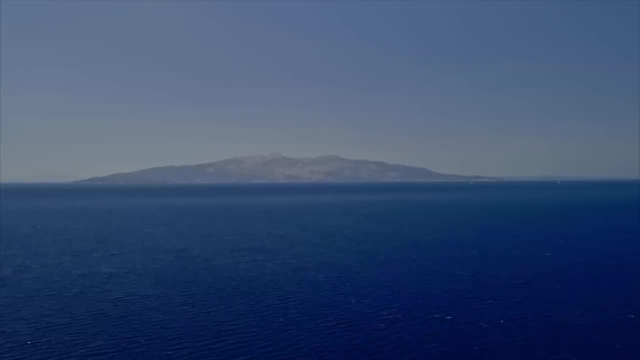 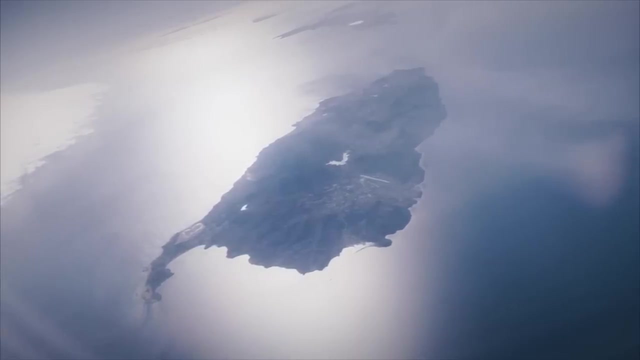 Streams and small rivers may have been simply walked or swam across, though larger rivers and oceans would have been difficult to cross. Despite this, Neanderthal remains are found on islands separated from the mainland by many miles. The only way to get to these islands would have been to swim, or perhaps 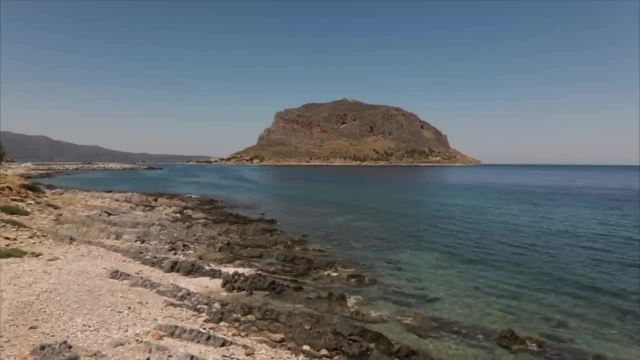 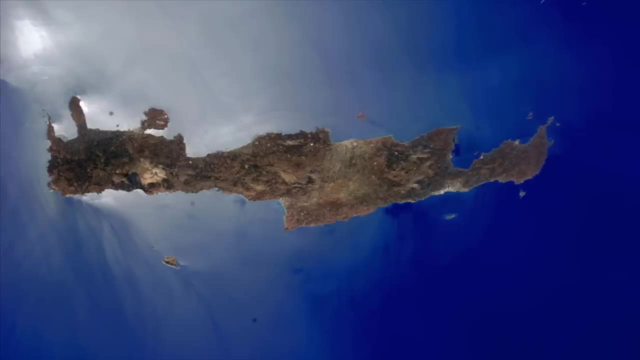 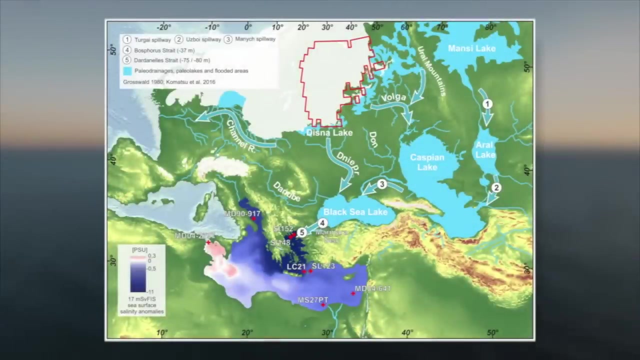 to use some sort of flotation device. Artifacts on Crete date back to between 130 and 107,000 years ago. Crete has been an island for some 5 million years and is 40 kilometers from its closest neighbor, Even during glacial periods, when the sea level was much lower. it would have been nearly the same distance. 40 kilometers is quite a long distance to swim. Neanderthals would not have necessarily have been the best swimmers. Their high muscle mass and dense bones would not have made them very buoyant and their short limbs would not have been the best. 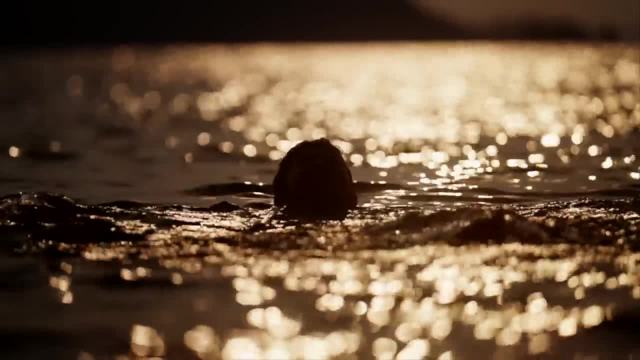 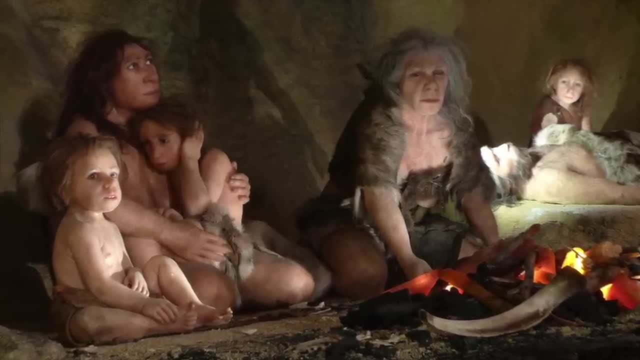 to propel them. We must also consider that not all Neanderthals were full-grown adults. Teenagers, toddlers and infants were not the best swimmers. The only ones who were able to swim were the adults Neanderthals. toddlers and infants were all part of a Neanderthal group at any given time. 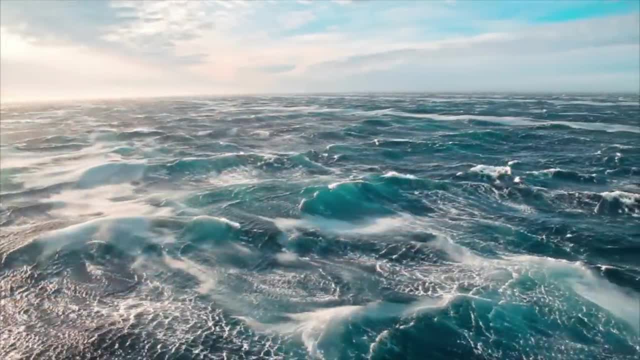 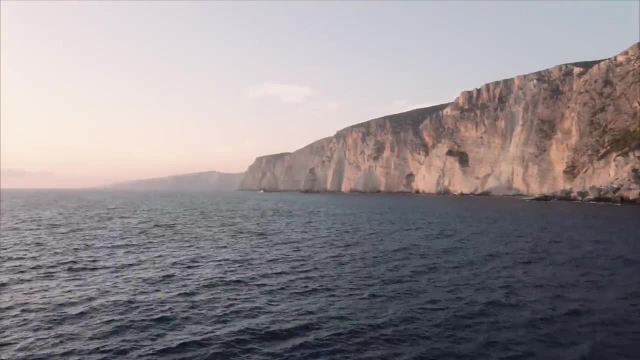 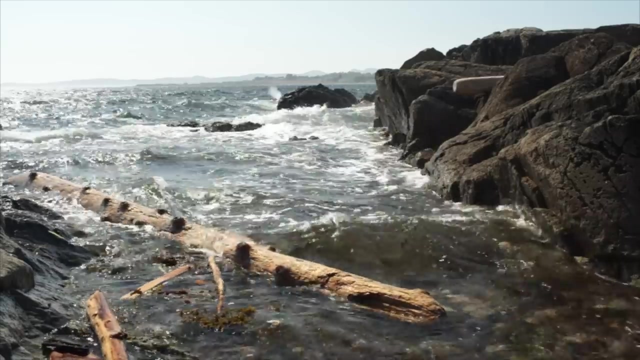 Depending on their age. it would be nearly impossible for young Neanderthals to swim this far. Ambitious journeys such as crossing over to Crete were almost certainly highly planned affairs. Some type of flotation device may have been necessary. Buoyant logs may have been held onto while children sat atop them. 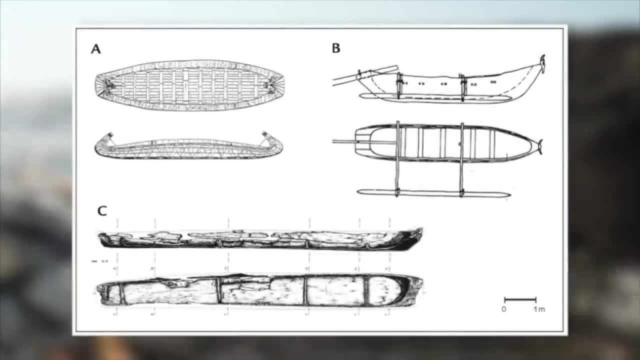 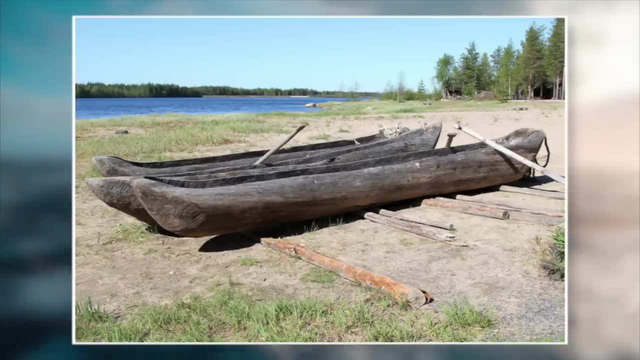 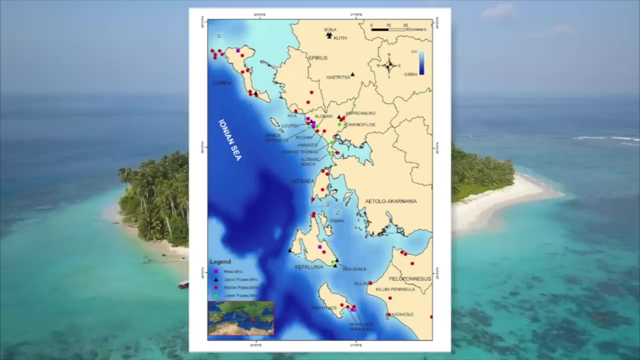 More complex constructions may have certainly been used, considering their crafting ability. However, an above-water boat is unlikely, considering how challenging they can be. to make A dugout canoe would have been extremely labor intensive, though some type of reed boat could have been made. Other islands also show evidence of long distance travel over the Mediterranean. Zakynthos and Cephalonia also have artifacts older than 100,000 years. These islands were still islands during periods of low sea levels. Other islands in the Mediterranean may have also been inhabited for centuries. Other islands in the Mediterranean may have also been in. 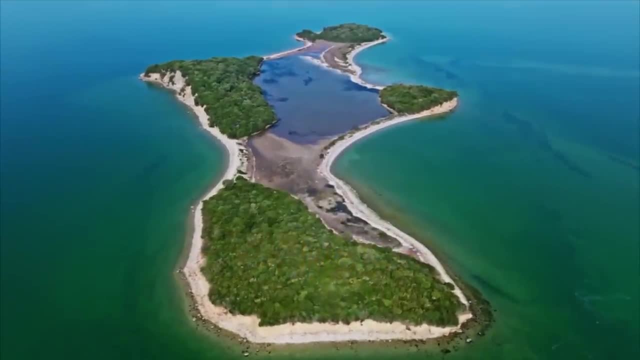 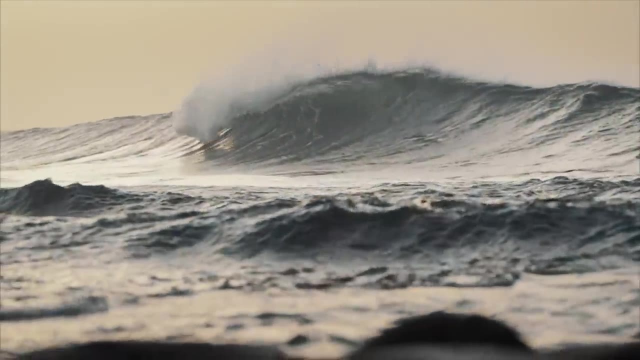 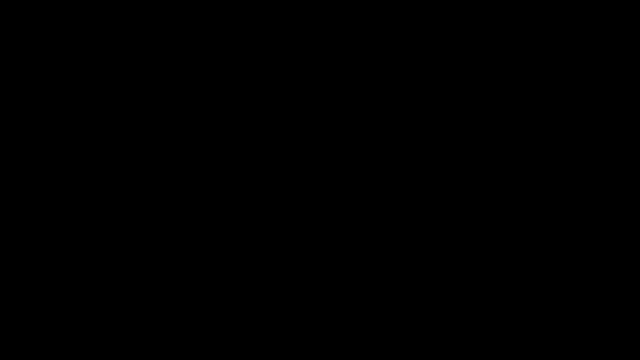 inhabited, and others do have artifacts present on them. Even the strait of Gibraltar may have been crossed. If they really did cross the seas, their ability to engineer boats and navigate through open waters would speak volumes to their advanced cognitive and technical skills. Considering their world was quite lonely, we must consider what their social lives were. 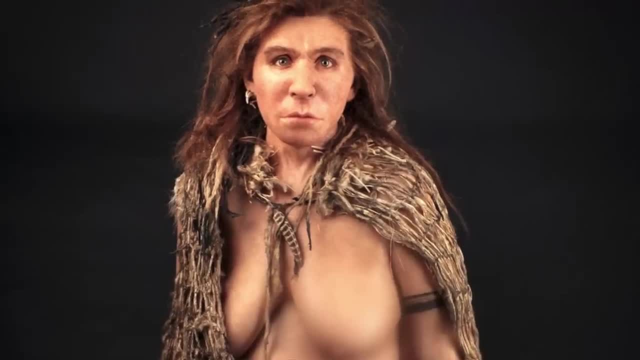 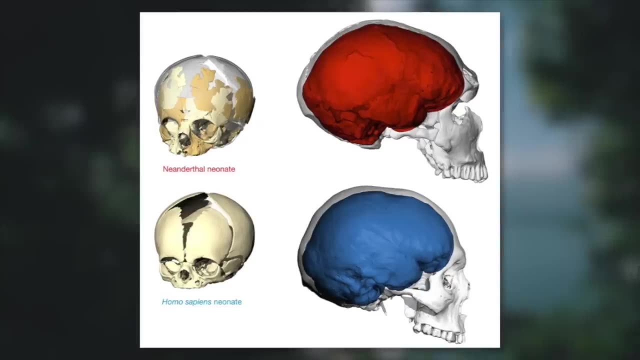 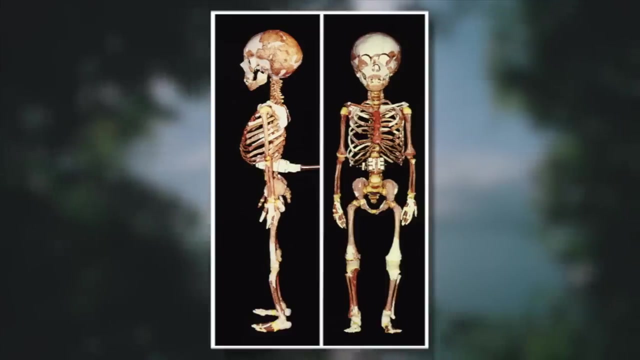 like. First, we must consider the lives of pregnant women. Human birth would have been about as dangerous as it is for modern humans. Neanderthal infants were born with a brain volume of about 400 cubic centimeters, Similar to modern human babies, though their skeletons were much more robust. Female Neanderthals had larger pelvises than modern humans, but infants also had long and more robust skulls. Pregnant Neanderthal mothers would have likely sought after shelters such as a cave or a rock shelter when their time was near. Since most Neanderthals had long and more robust skulls, pregnant women would have had. 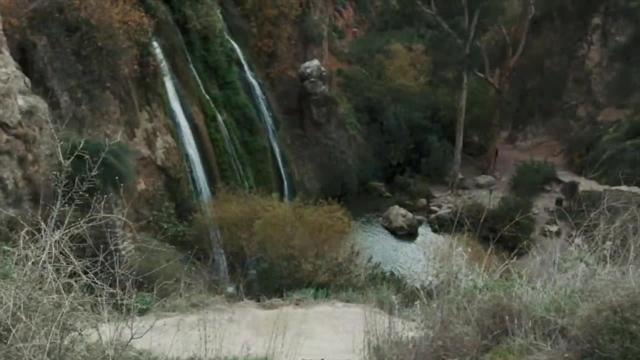 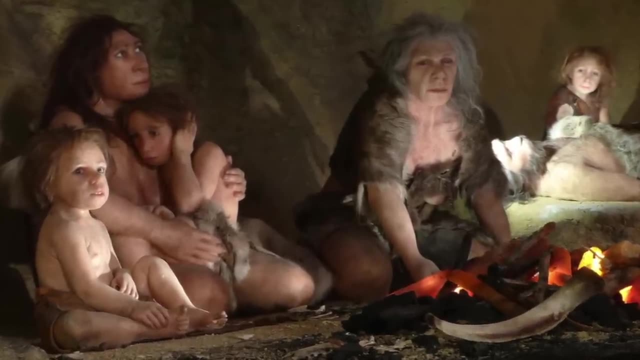 a hard time finding a place to live. Since Neanderthals seem to have been born in the spring, they may have planned to give birth at certain locations. Friends, parents and even grandmothers may have assisted in the birthing process. 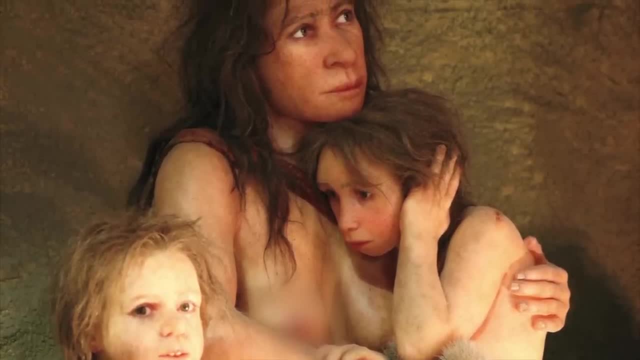 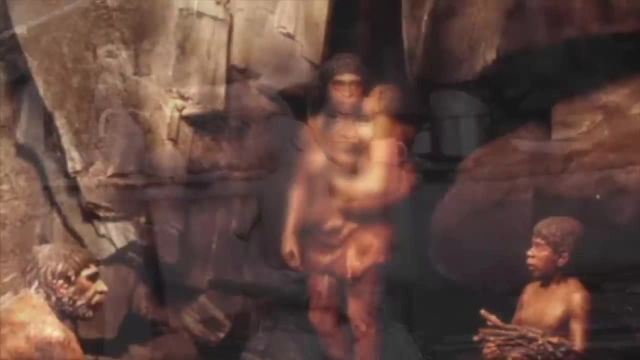 If a Neanderthal and their mother were lucky enough to survive birth, they would have been breastfed for up to two and a half years. This is similar to modern hunter-gatherers. An extra 500 calories on average would have been needed for Neanderthal mothers to feed. 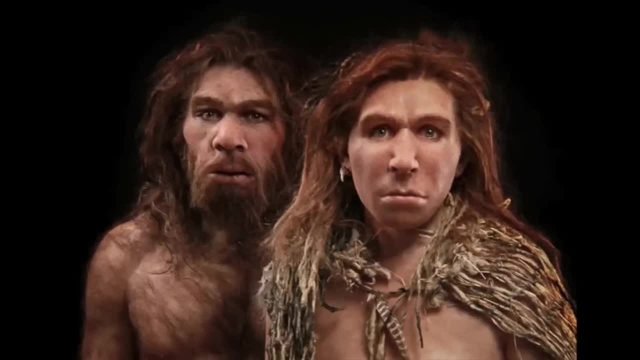 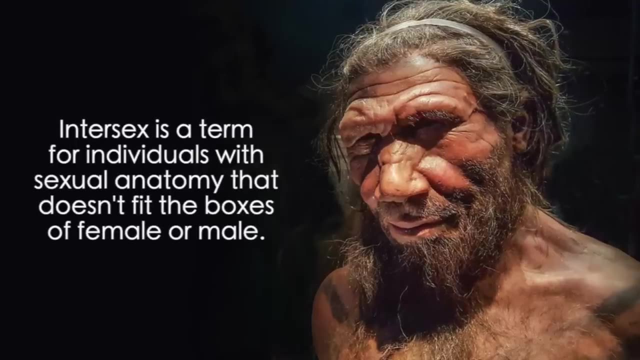 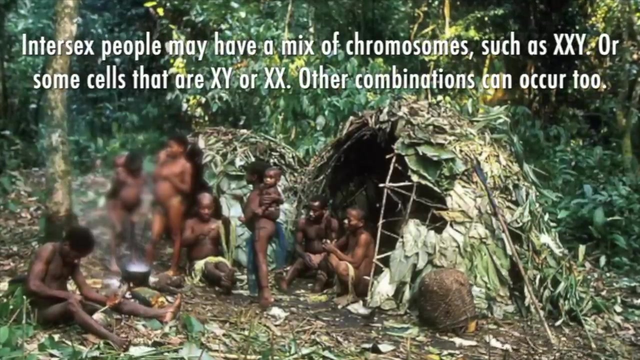 their infants. In terms of living people, an estimated 1 in 2,000 Neanderthals would have been born intersex- A low number, but statistically significant considering their population size. These individuals are almost ubiquitously accepted across hunter-gatherer societies. 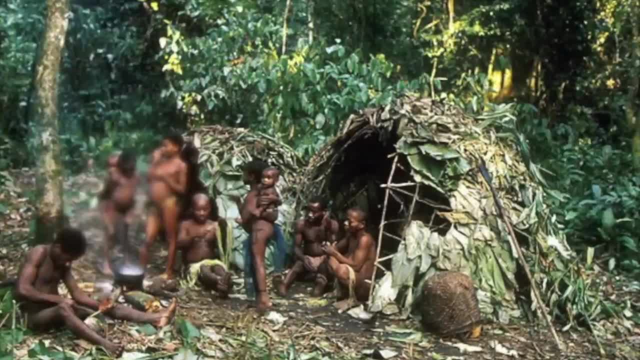 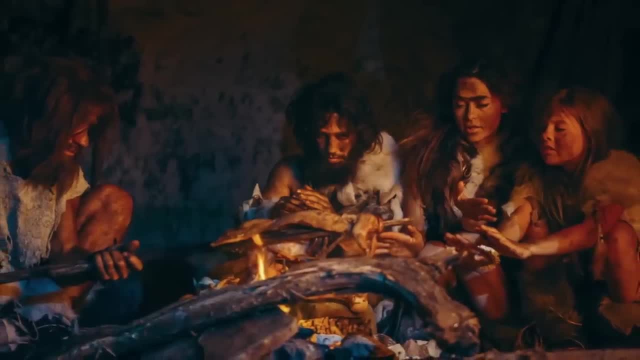 as another set of hands and their actual role in society varies. Considering these individuals certainly existed, it is interesting to imagine how they would have fit into the Neanderthal social structure. Due to a high level of ailment sensitivity, Neanderthal mothers would have been able to. 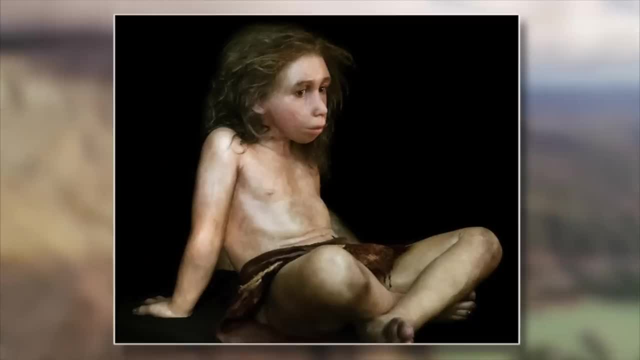 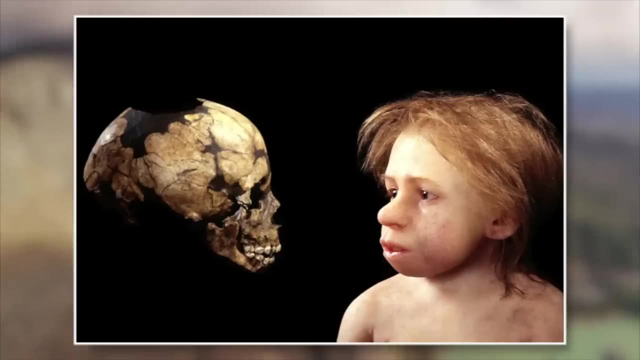 handle the ailments at a young age. It appears that young Neanderthals were immediately put to work helping the group. Both male and female Neanderthal children show a similar rate of a highly active life. They would have had many skills to learn, many of which were physically exhausting. such 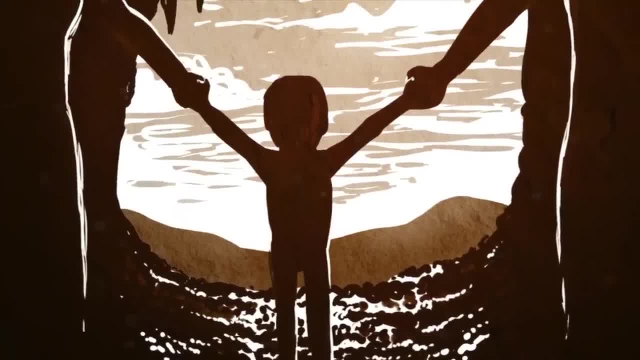 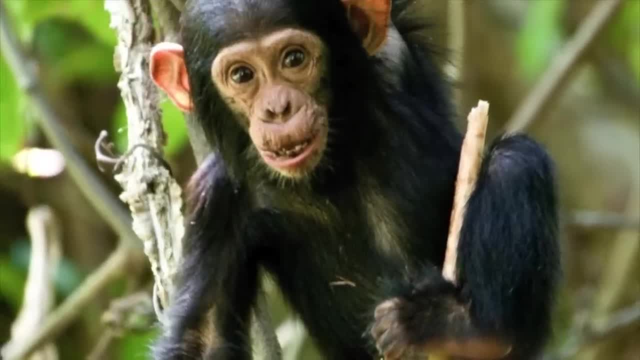 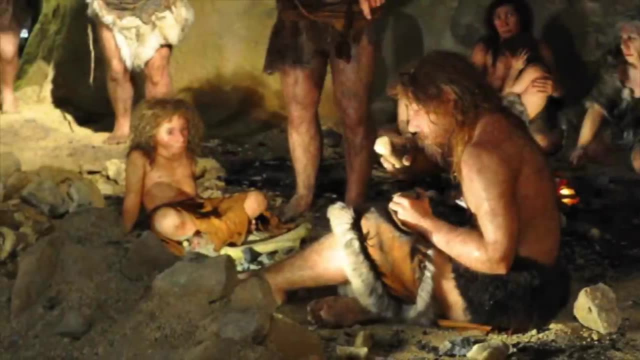 as working hides, though a childhood with toys and plenty of laughter is not out of the question. Young chimpanzee females are known to carry around objects to mimic infants. young Neanderthal girls may have also played with some sort of makeshift dolls. Both sexes may have been given their own stone tools to play with at a young age. 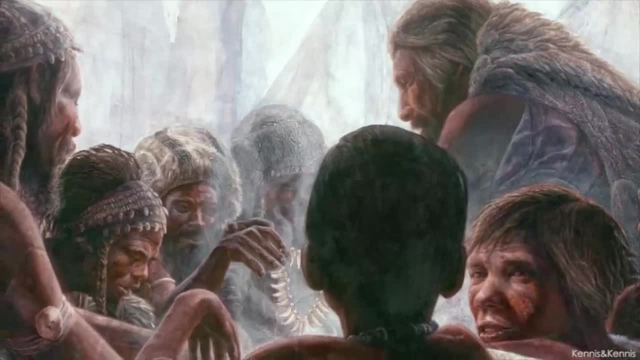 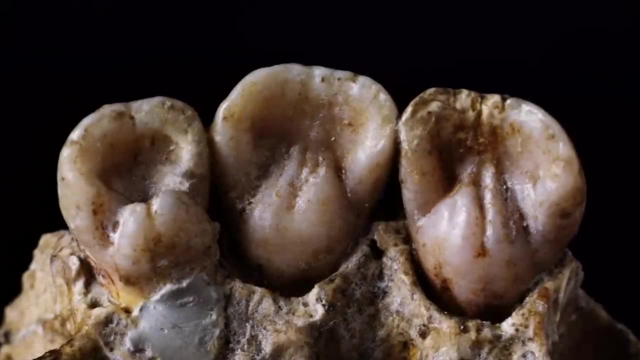 As men and women matured, their tasks would have diverged. Tooth wear patterns in Neanderthals differ from men and women. Women seem to have commonly used their teeth for carrying things around, while men have more wear on their upper teeth. 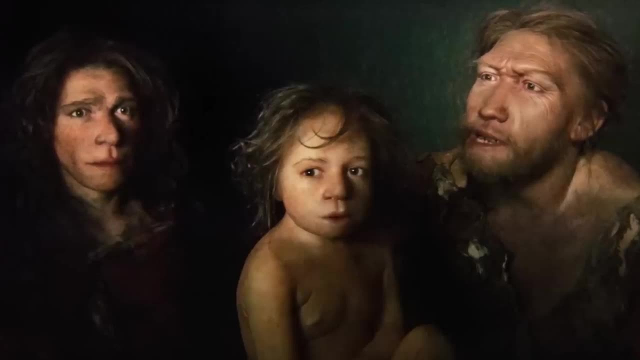 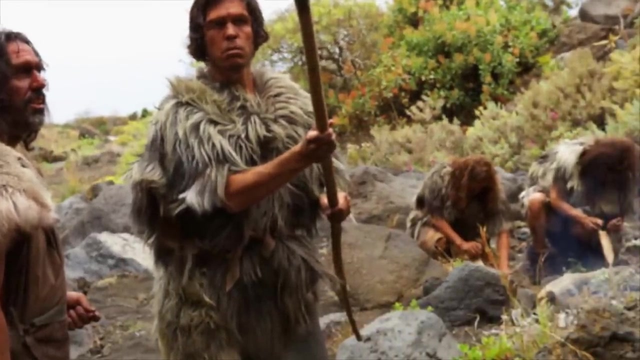 We do not know exactly what they were doing, though it is clear that there was a sexual division of labor. 3. Hunting Large Game. Though the typical picture of men hunting large game while women foraged harmless berries does not seem to be true, 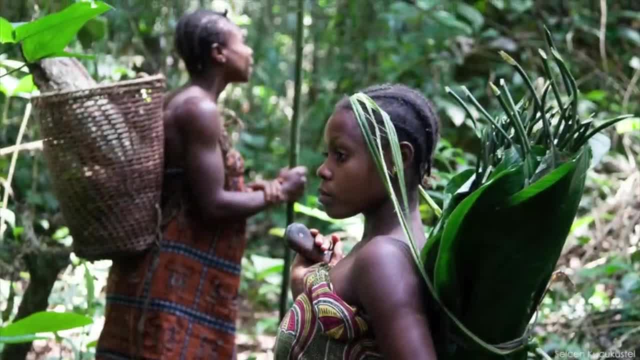 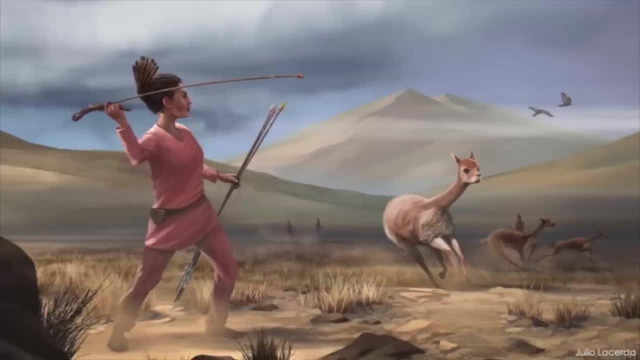 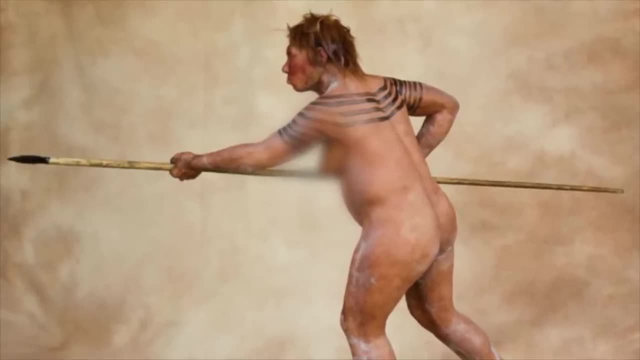 First of all, this idea is not really even true for modern human populations. Across hunter-gatherer societies, women often hunt small game and even sometimes medium to large game. Neanderthal women were stocky and strong and would have certainly been capable of hunting. 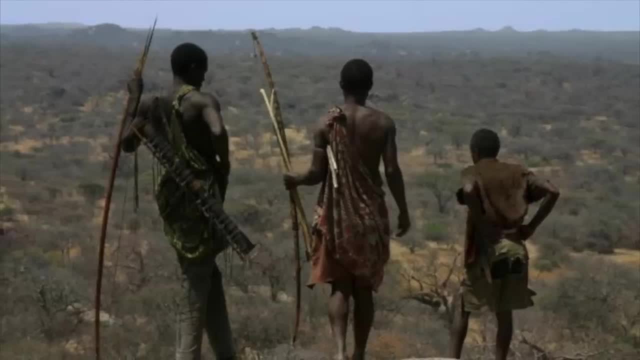 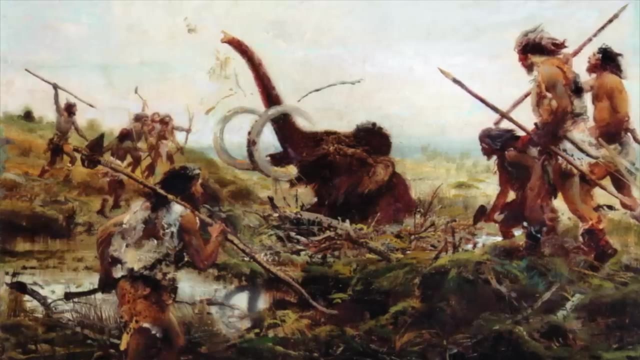 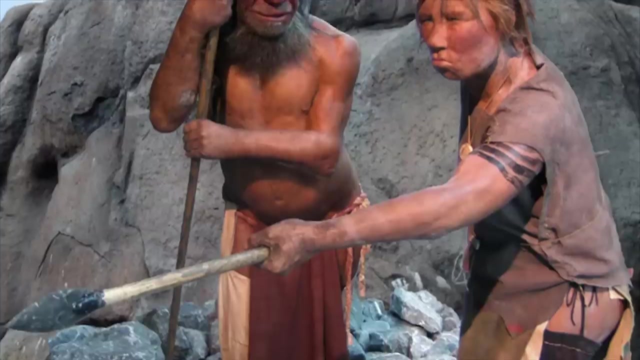 Though based on hunter-gatherer societies, the larger the prey and the farther away it is, has a direct correlation to a higher proportion of male hunters. Neanderthal women may have not taken part in some of the larger, more dangerous hunts, but they were still certainly getting injuries from dangerous animals. 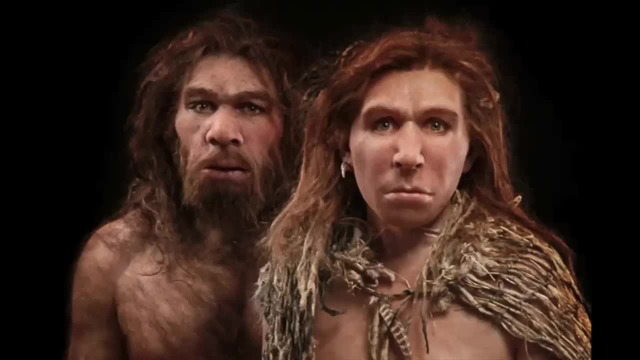 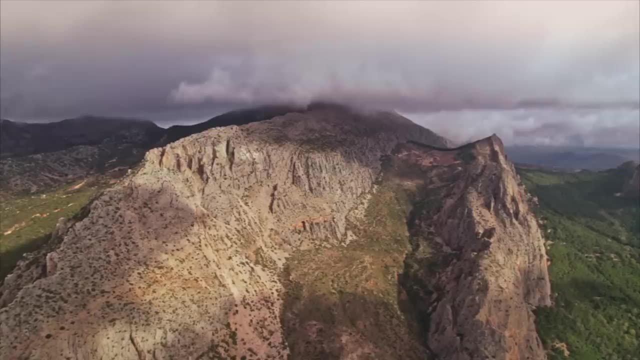 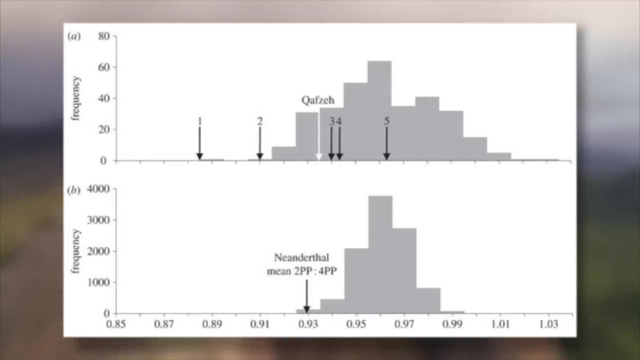 Some hunts undoubtedly included men and women. Another question we must ask regarding Neanderthal relationships is what their sexual relationships were like. It is, of course, a very difficult question to ask with the remains that we have. Funny enough, A way to test this comes from finger length ratios. 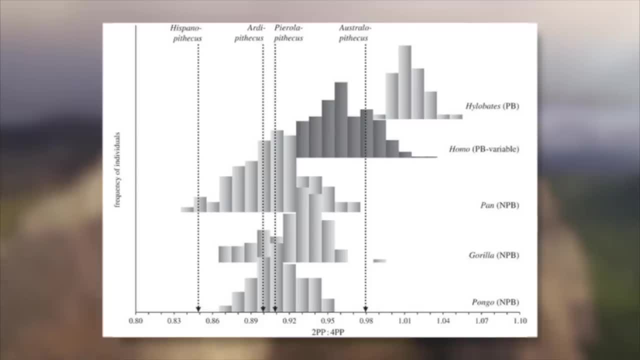 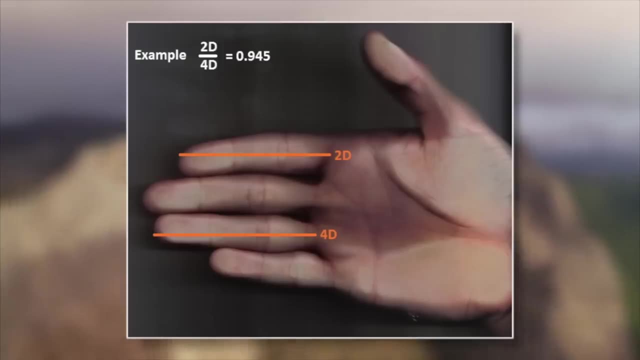 It is thought that finger length ratios are affected by androgens such as testosterone in the womb. High levels of hormones increase the length of the fourth finger in comparison to the second finger. Neanderthal finger ratios were lower than most populations of living humans. 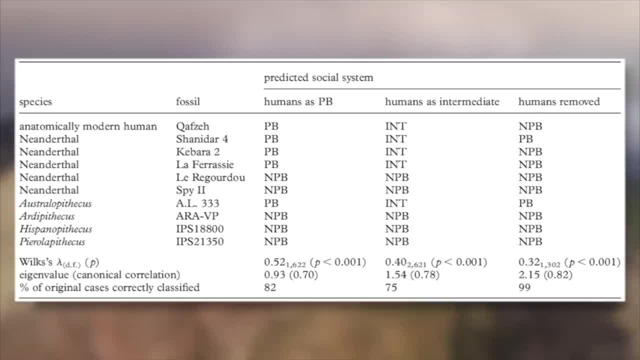 This means that males were likely very competitive for mates and more promiscuous than modern humans. They may have formed more polygamous relationships than modern humans. The reason for this is that Neanderthal females were more likely to be competitive for males than modern humans. 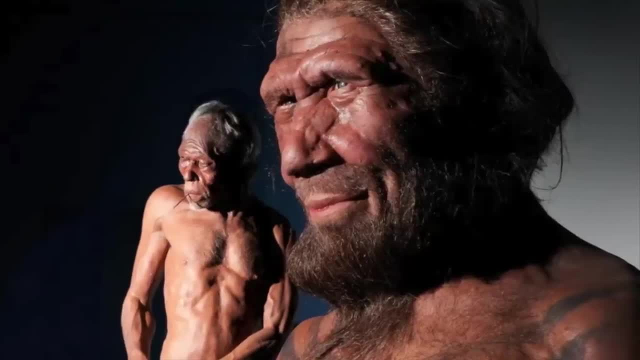 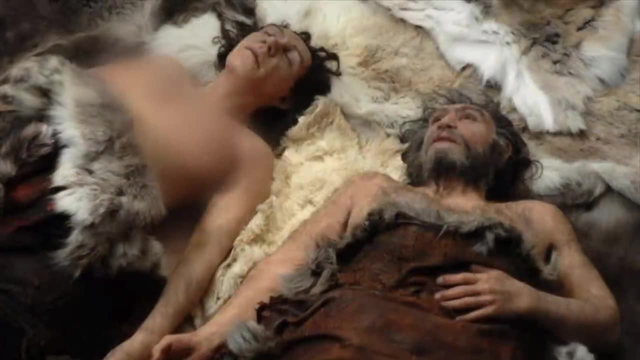 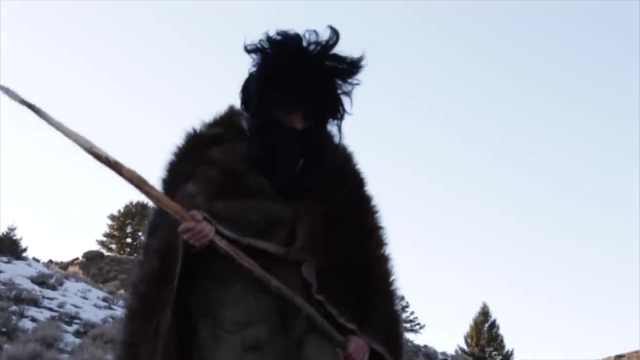 Some contemporary hunter-gatherers, though, of course, take this with a grain of salt. Due to their relatively similar rates of sexual dimorphism as modern humans, they probably commonly had pair-bonded sexual relationships, and these relationships were likely even same sex from time to time. 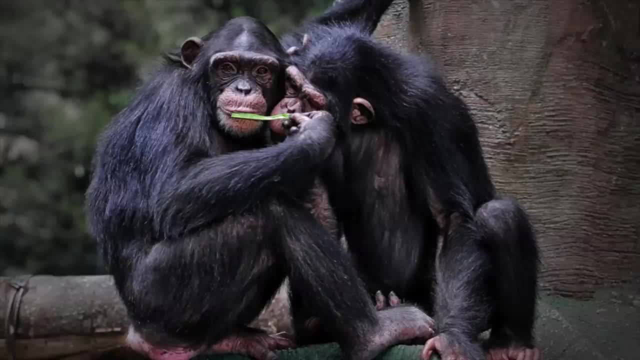 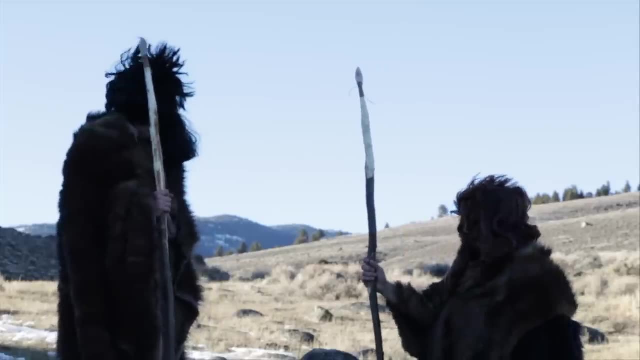 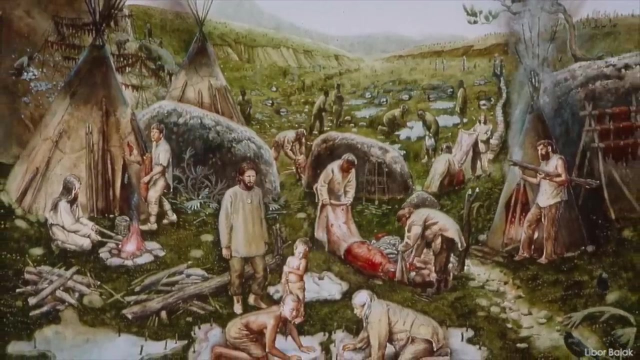 Same sex relationships are quite common across the animal kingdom and have been reported in every species of great ape. There is no doubt that this would have been the same for Neanderthals. Beyond thinking about individuals, we must think about the larger Neanderthal community. 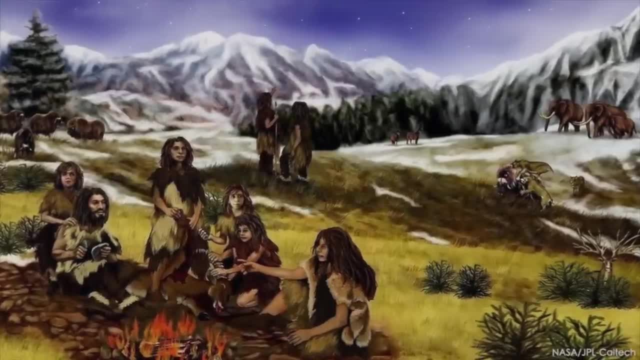 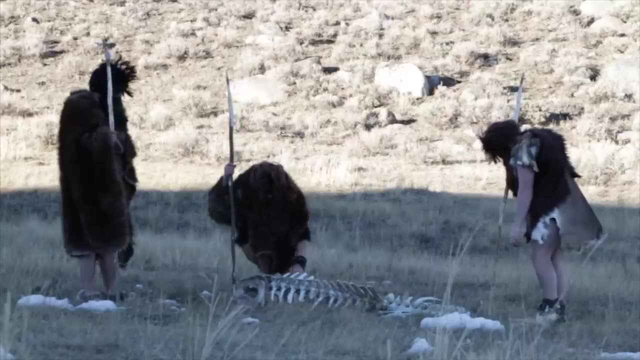 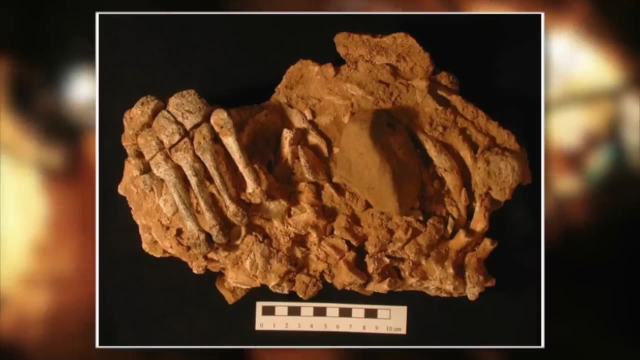 Their group sizes averaged between 10 to 30 individuals. Smaller groups seem to have splintered off for specialized hunting and gathering tasks. Some sites show only three individuals stayed for short periods. The previously mentioned family that was cannibalized at El Cedron has told us a lot about Neanderthal. 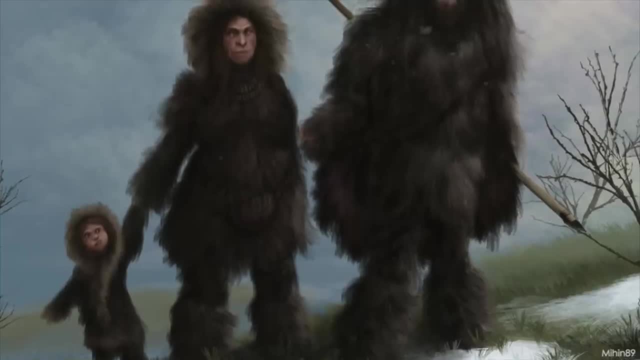 family organization. 7 of the 13 individuals stayed for a short period of time. The group that was cannibalized at El Cedron has told us a lot about Neanderthal family organization. 7 of the 13 individuals, of which six were men, share the same mtDNA haplotype. 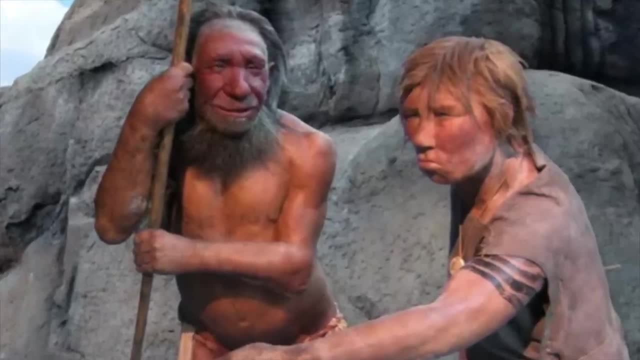 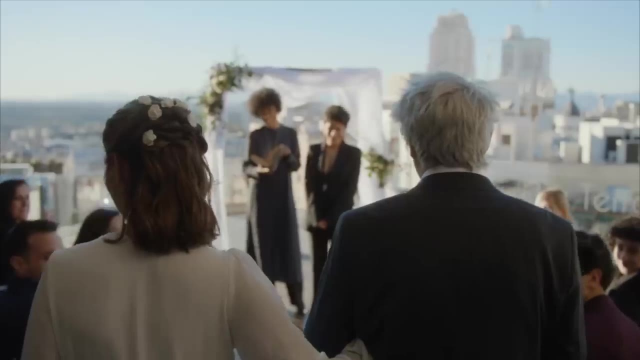 Three of the four adult females have different mtDNA lineages. This suggests that the men were all closely related, while the women were from an outside group. This group likely practiced patrilocality, meaning that the women moved to the male's group instead of vice versa. 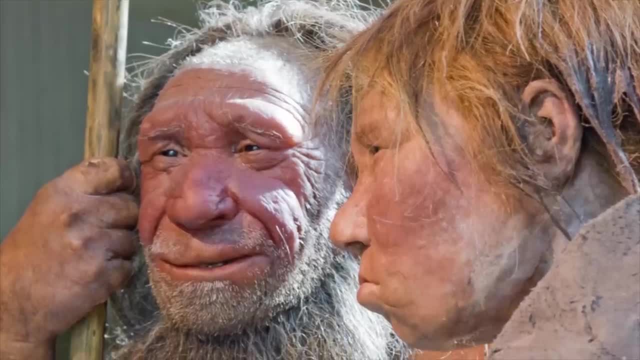 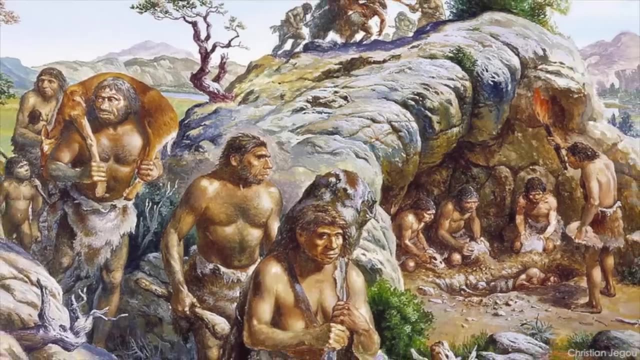 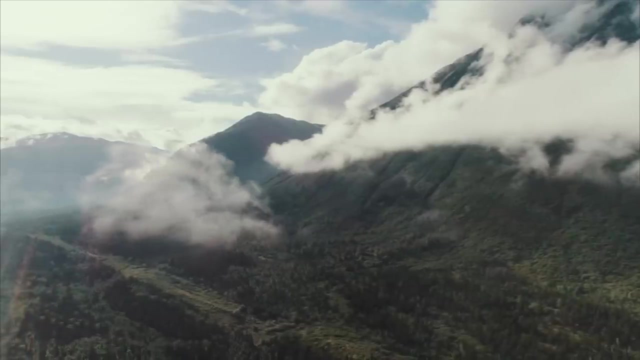 Though we must be careful when coming to any concrete conclusions. other groups may have had much different customs and habits. Neanderthal groups were likely part of a larger network of similar groups. In order to avoid interbreeding, this larger network would have had to be around 500 individuals. 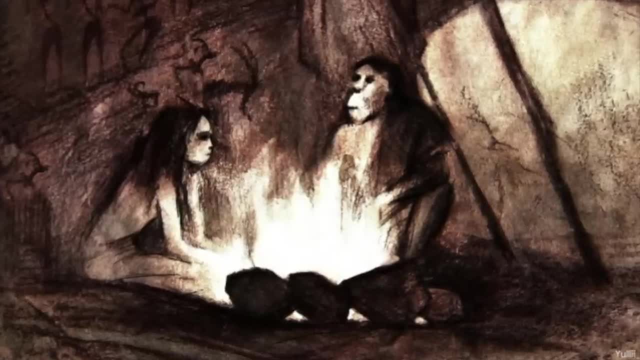 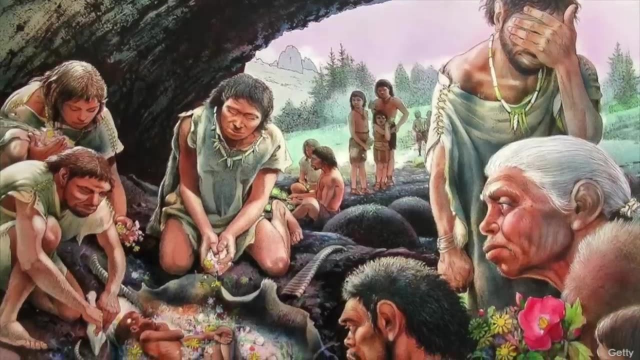 Genetic evidence tells us that a fair amount of Neanderthals may have been inbred, Though based on artifact transfer. Neanderthals seem to have been capable of creating expansive ethno-linguistic tribes. Many tribes in a region may have been able to directly communicate through a similar 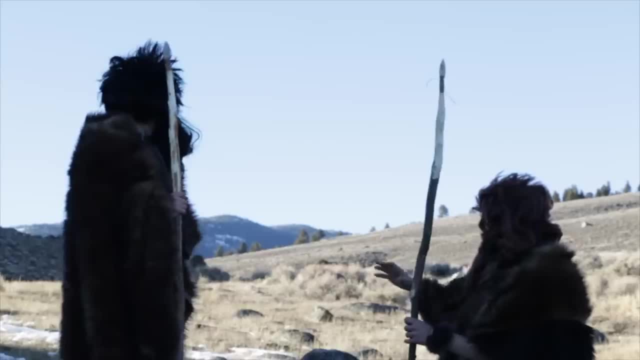 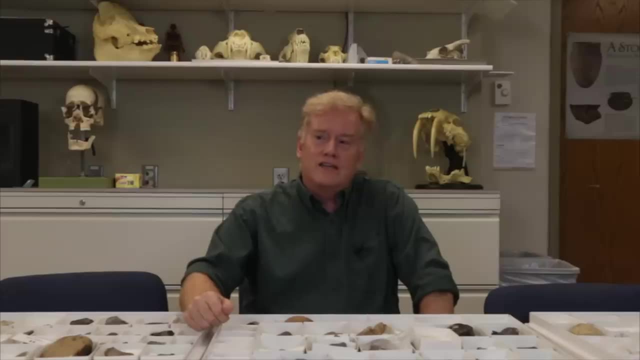 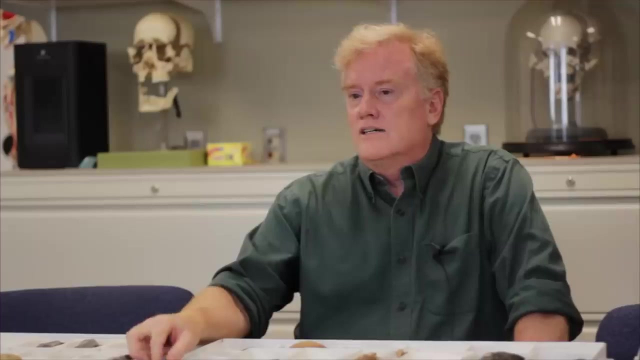 language. Due to their technical and cultural complexity, it is reasonable to assume that some kind of language was spoken. They had language. Their language, in terms of their speech, was slightly different from ours, but we don't have any reason nowadays to assume that, in fact, the language was so different that it 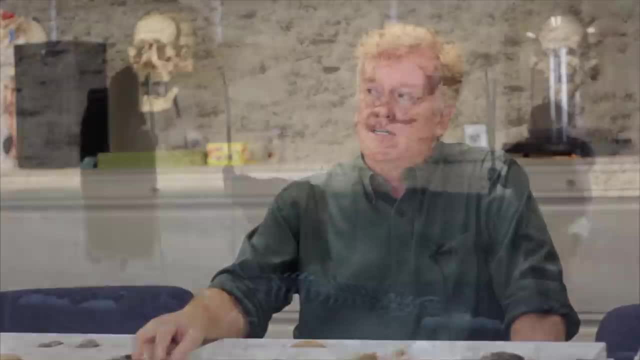 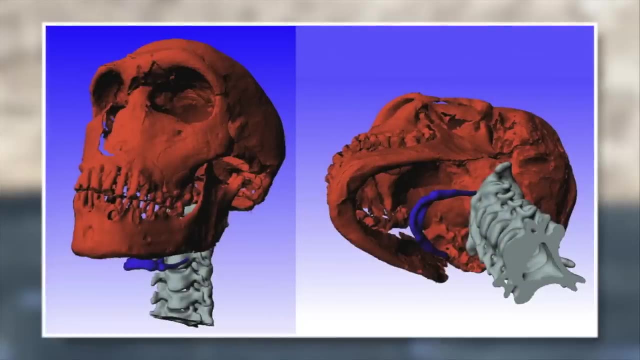 could not have performed like a grammatical language. A fairly complicated language was likely necessary to navigate their complex world. The hyoid bone is a small bone at the front of the neck which is used to support the tongue and is very important for speech. 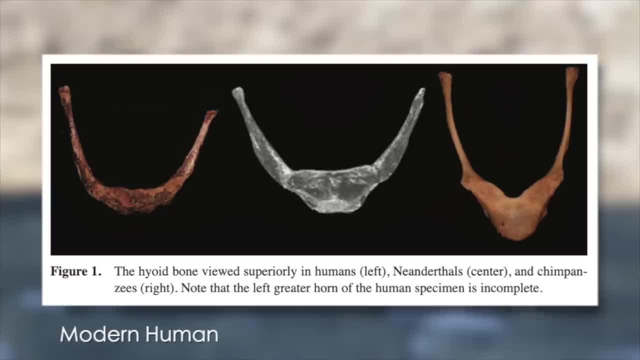 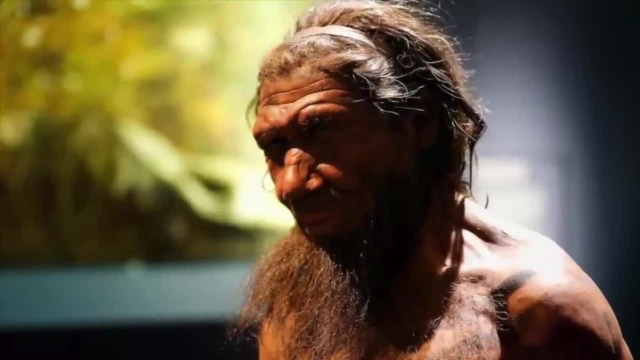 A Neanderthal hyoid bone found in Israel is nearly identical to the hyoid of a modern human. Some have claimed that Neanderthals would have had high-pitched, squeaky voices. However, multiple studies on the morphology of the Neanderthal vocal apparatus proved 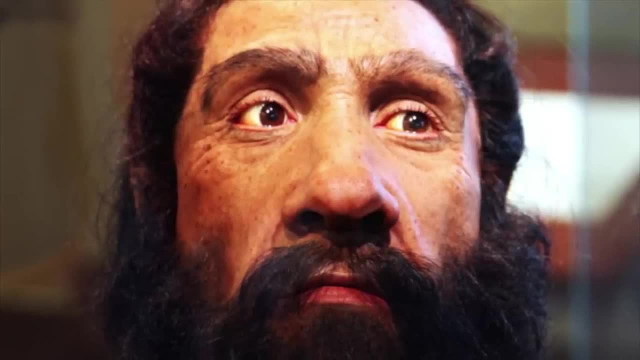 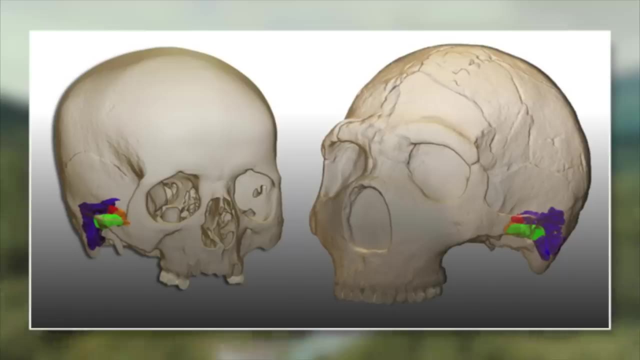 that they could produce a similar range of sounds as modern humans. Neanderthals' ear bones also suggest that they were capable of hearing a similar range of sounds. Beyond being able to make and hear complex noises, a complex brain is needed to process. 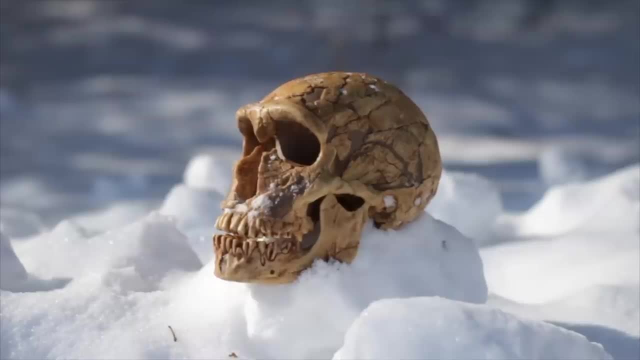 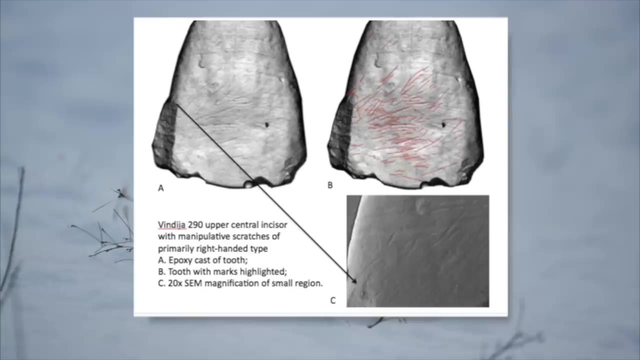 them. Neanderthals had an expanded Broca's area of their brain, which, in modern humans, is associated with the formulation of sentences and speech comprehension. They had similar rates of right-handedness as modern humans, which reflects asymmetry of the brain and supports language ability. 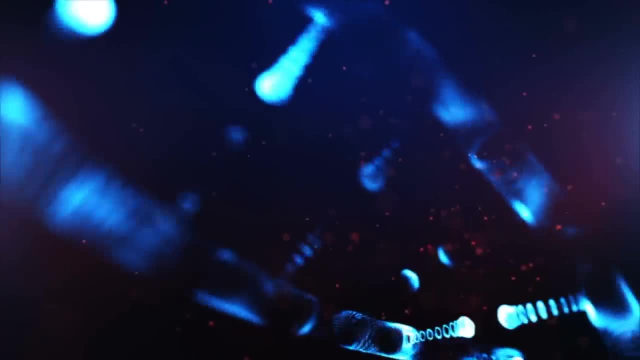 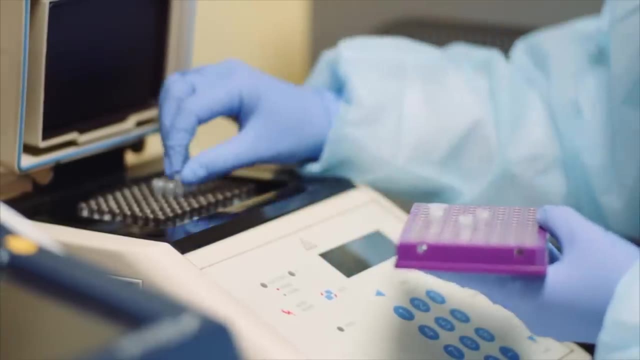 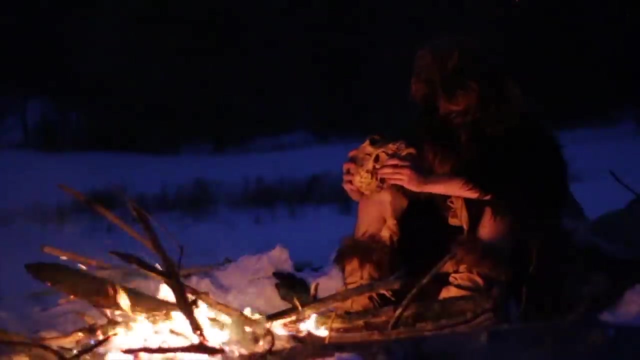 DNA. DNA can offer us a more detailed look into what they may have been capable of. Among 48 genes associated with language in modern humans, 11 of their genes differ from modern humans. These 11 genes do not necessarily inhibit complex communication, but they do differ. 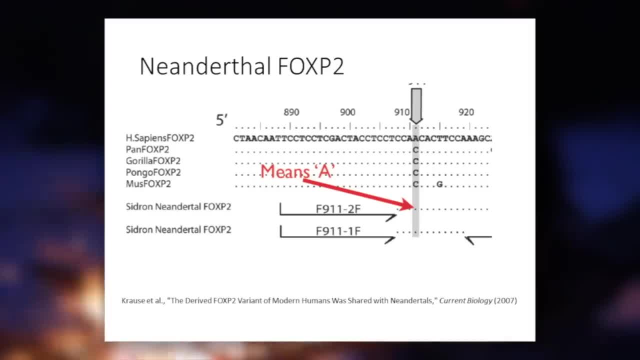 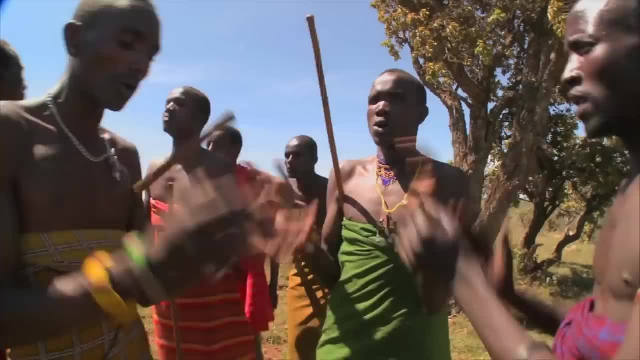 Of the similar genes. Neanderthals had a FOXP2 gene, but it was not the same as our modern variant. This gene is associated with speech and language development. Overall, Neanderthals had a very similar range of sounds. In general, DNA evidence suggests that modern humans have a stronger ability to express. 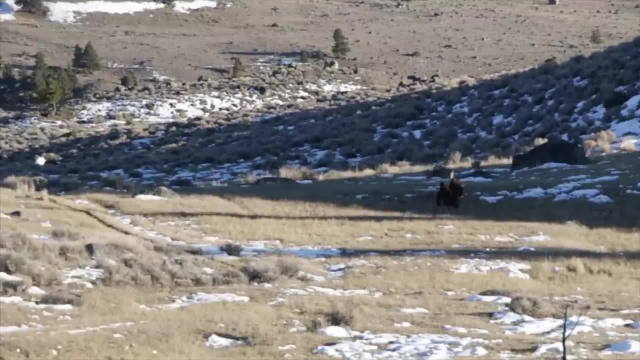 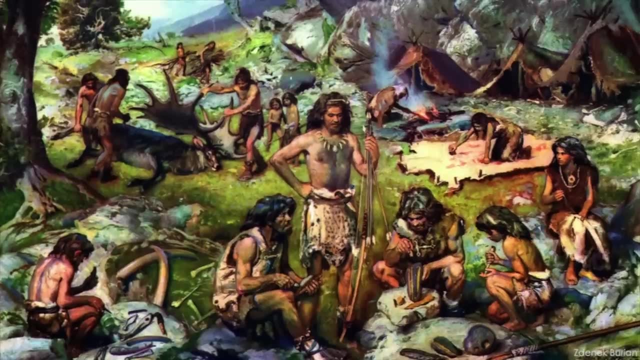 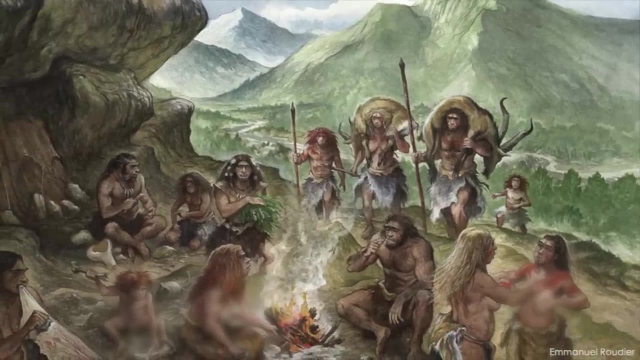 language than our Neanderthal cousins. This makes sense considering that Neanderthals lived in secluded groups and overall had a lower population density. Modern humans in general are much more social than Neanderthals When thinking about the actual language that they spoke, it is important to understand. 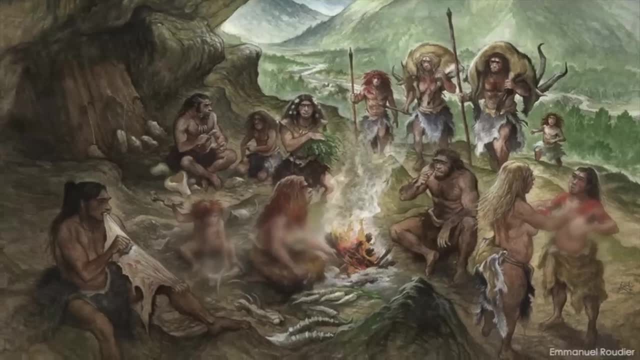 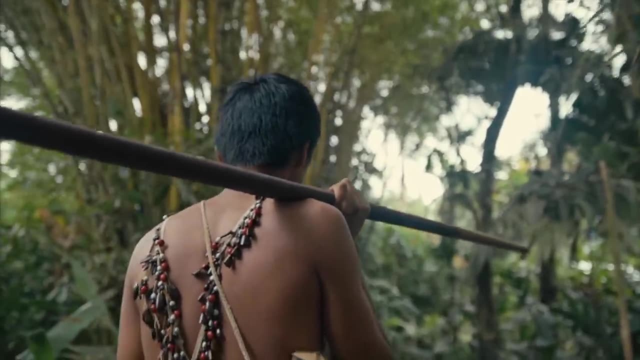 that there was not one singular Neanderthal language. Over their vast range, their languages may have used the same language as Neanderthals. However, Neanderthals were not the only Neanderthal language. Some groups may have even differed to a similar degree as contemporary indigenous people. 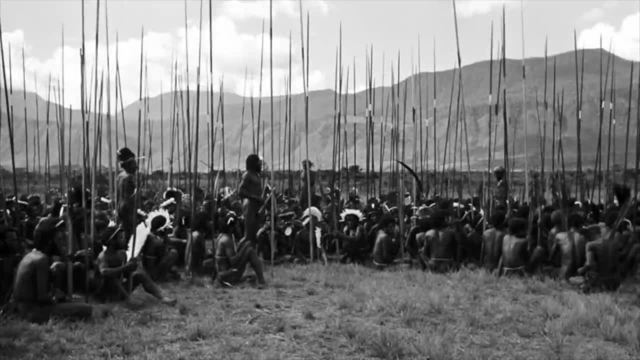 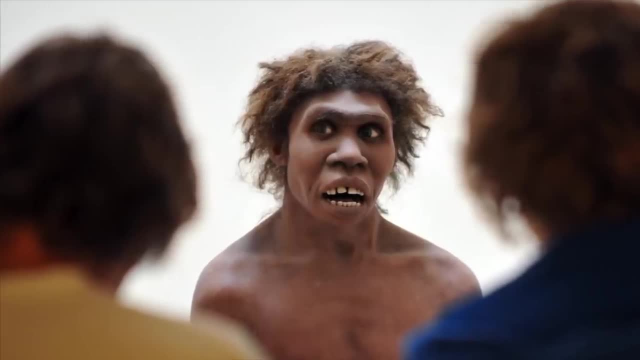 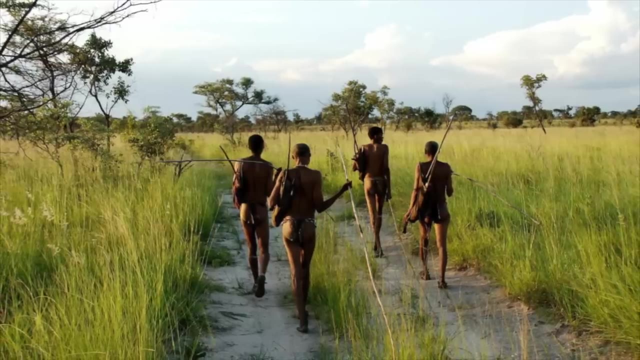 There are 839 living languages in Papua New Guinea alone. due to how isolated the populations on the island are, We can also imagine that some Neanderthal populations may have spoken very differently than we are familiar with. Some groups may have spoken with clicks, such as Khoisan languages, or possibly with whistles. 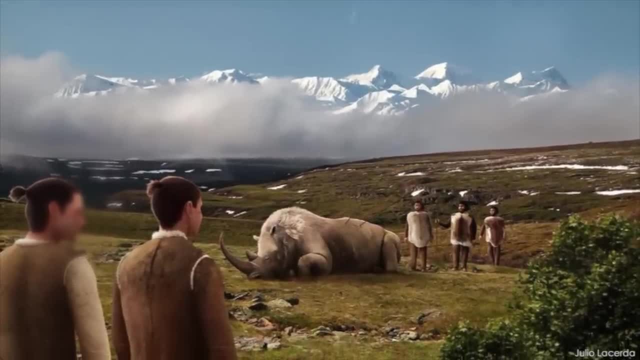 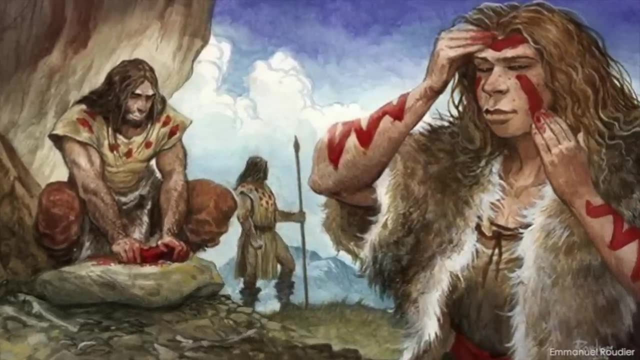 Migrating groups of Neanderthals may have had a very difficult time communicating with each other. Neanderthal groups may have even found themselves interacting with people who were very culturally different. As mentioned early on in the video, there is evidence that Neanderthal cultures from 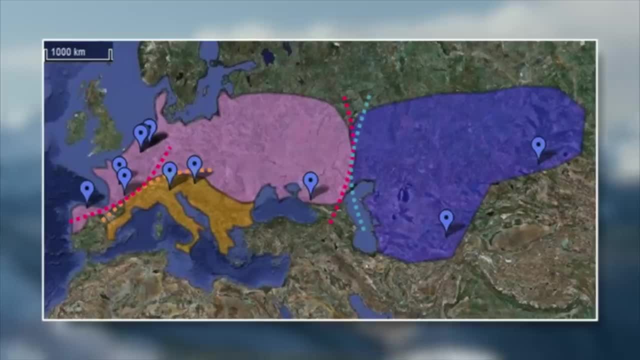 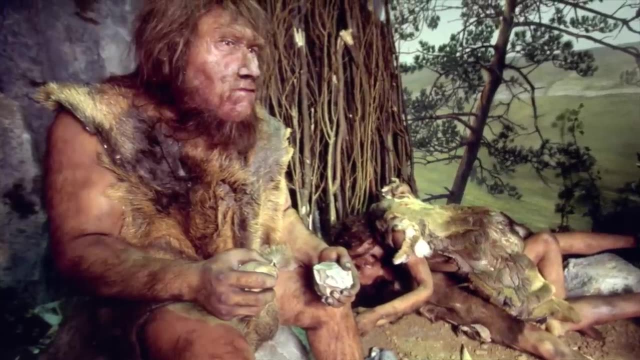 central Europe were different from southern ones and another culture east of the Altai mountains were also different. Not only did they use slightly different technology, but there was also anatomical differences. But we can't only think about culture from a geographical perspective. we must also consider: 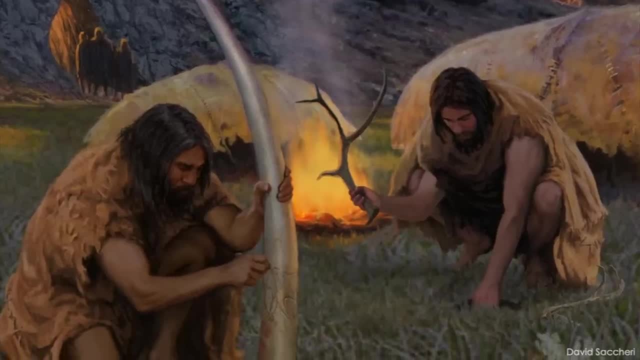 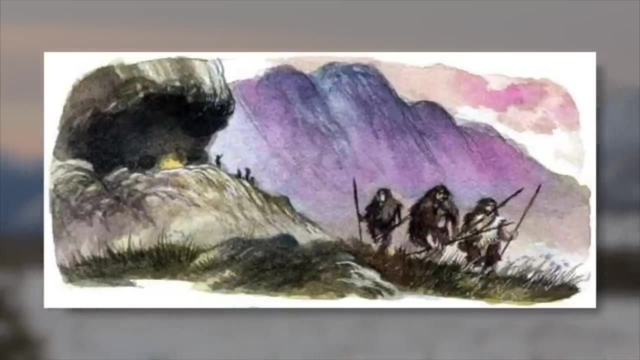 time, Different tool-making traditions and cultures appeared throughout space and time. Laquina is a Neanderthal site from France where the Laquina mousterian industry was discovered. These Neanderthals had a specific way of life that was different from other groups. 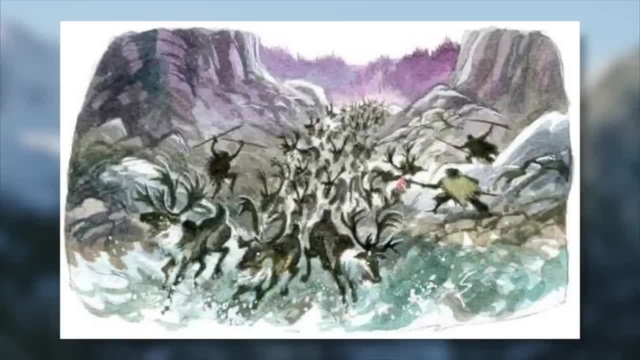 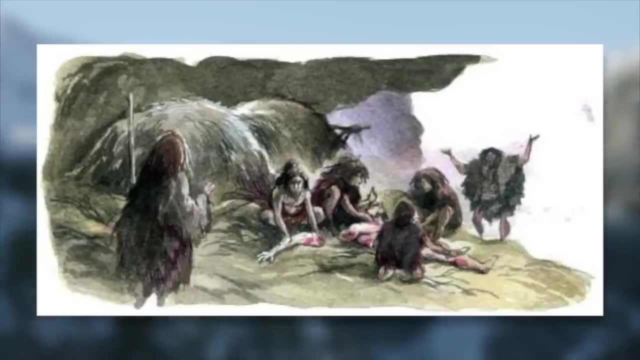 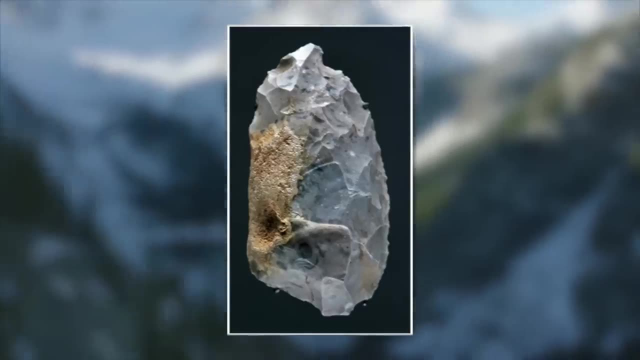 They specialized in reindeer hunting. Just like some modern cultures, they followed reindeer and lived off of what they provided. They brought their entire carcasses back to their sites and processed them with unique, thick, asymmetric tools. These tools could be retouched many times, useful for nomadic hunter-gatherers. 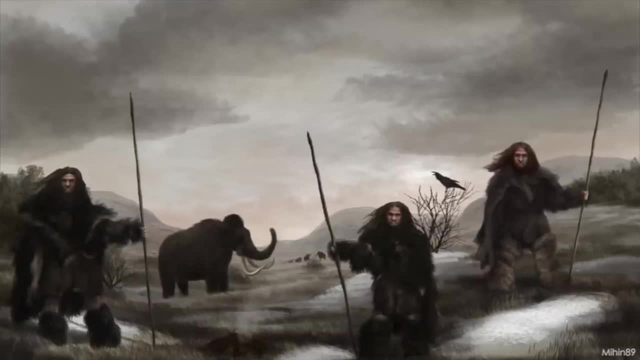 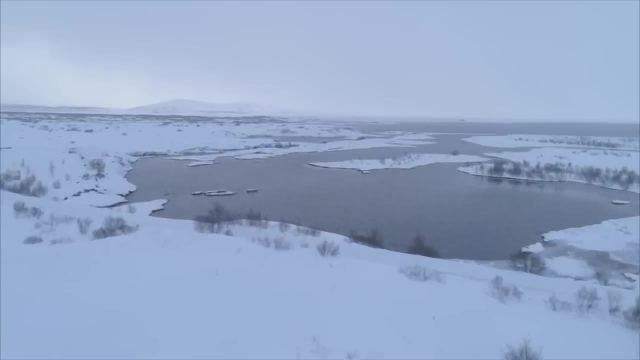 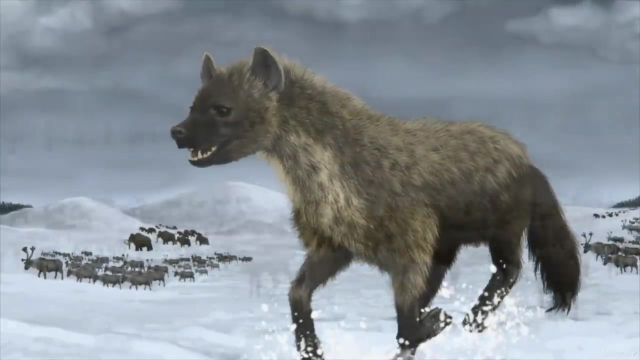 The Laquina technocomplex appeared around 80,000 years ago in southern France during the MIS-4 glacial period. This period was very cold and caused many prey animals to become regionally extinct. Hyenas also seemed to have abandoned the area, possibly because of a lack of prey. 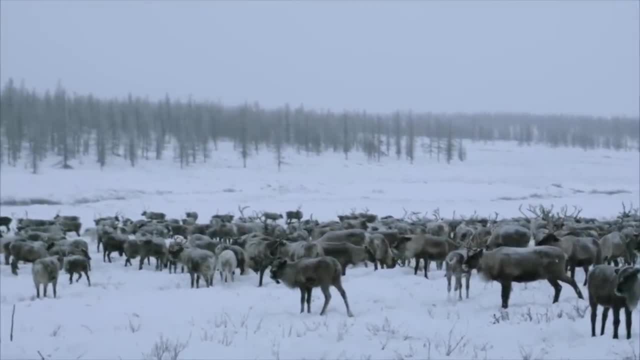 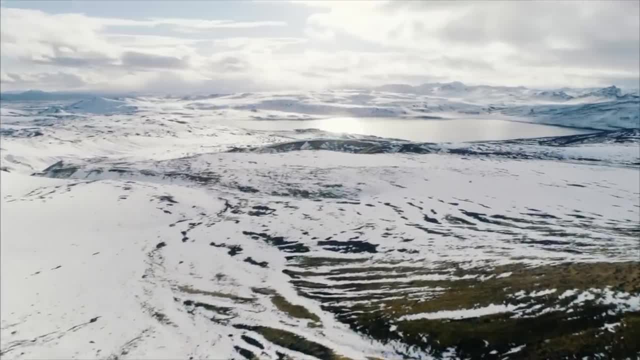 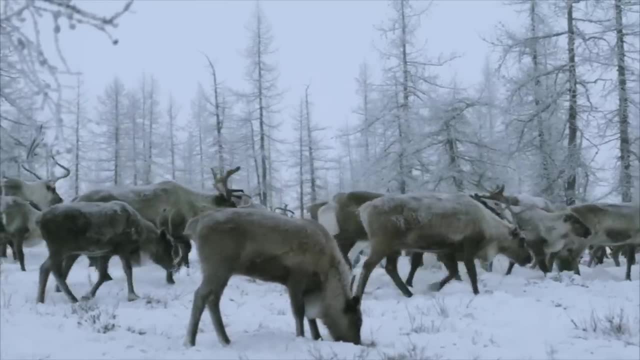 The Laquina sites were also used as a source of food for animals. This suggests that these Neanderthals did not frequent forests and were more accustomed to the tundra. Reindeer are known to be very migratory and Laquina sites appear to have hunted reindeer. 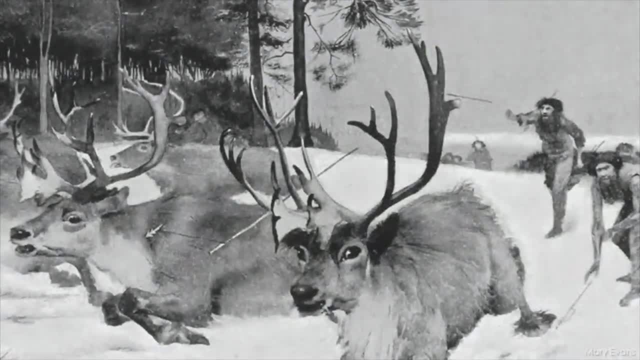 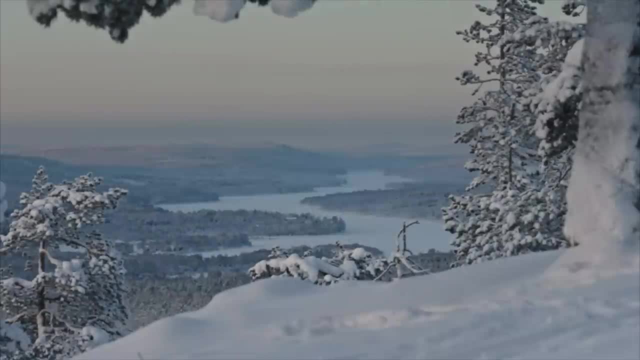 at all times of the year. This means that they were well aware of reindeer movements and either followed them or intercepted them along the way. Many Laquina sites also appear to have been intensely used, but only for short periods. The Laquina culture continued to exist after the MIS-4 glacial period. 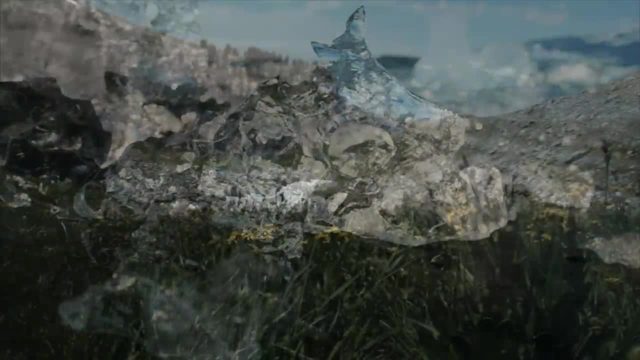 The Laquina culture continued to exist after the MIS-4 glacial period. The Laquina sites were also used as a source of food for animals. MIS-4 ended and the warmer glacial period had begun, though it would only be a few thousand. 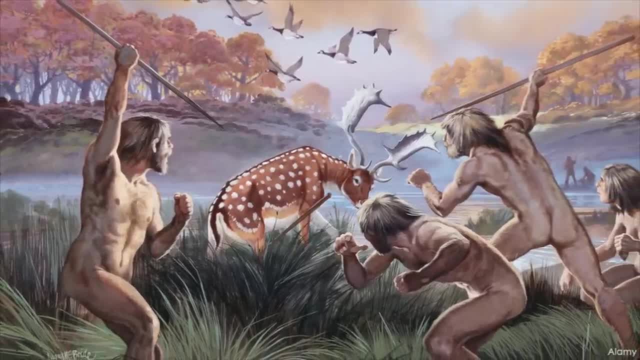 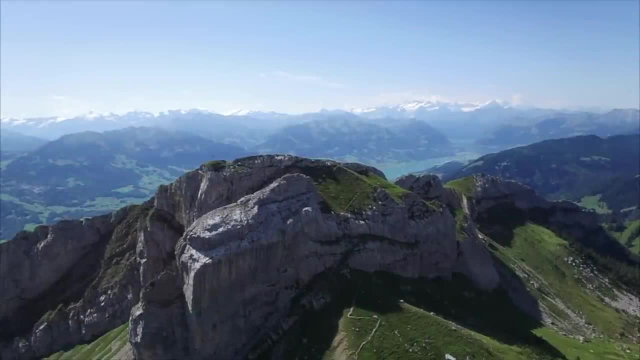 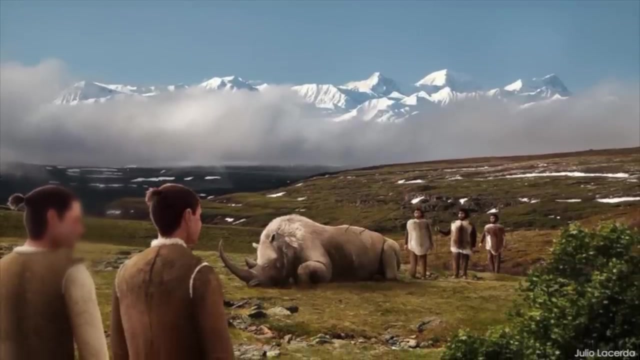 years before the culture disappeared around 50,000 years ago. The important thing to understand about this culture is that it represents how the Neanderthal world was: complex and distinct cultures formed and disbanded due to a variety of reasons. When considering how Neanderthal groups from different areas would have interacted with. 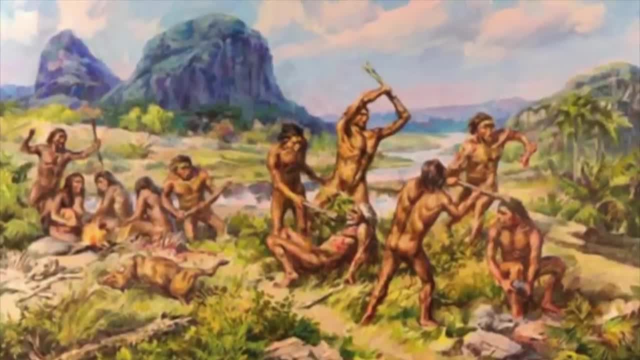 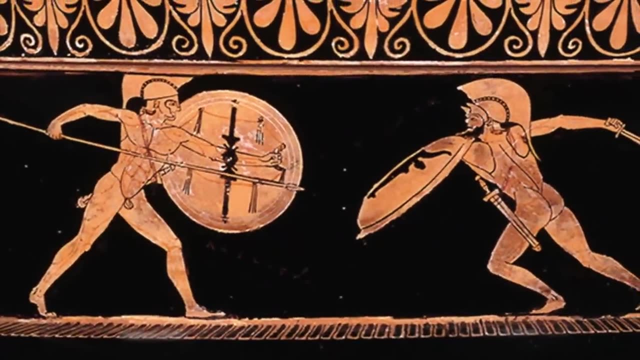 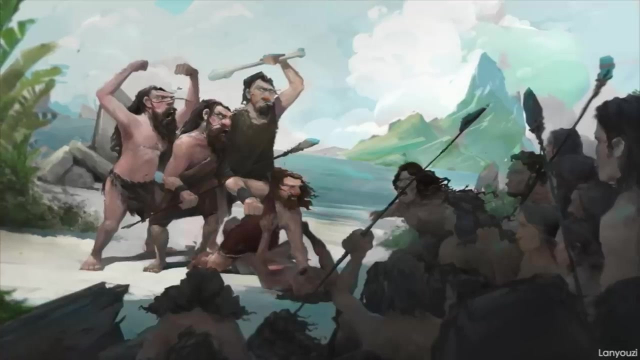 each other. we cannot overlook conflict or even war. Perhaps the ugliest and simultaneously most celebrated human cultural invention would be war. War is more or less ubiquitous across modern human cultures, and many like to speculate that it was the same way in prehistory. 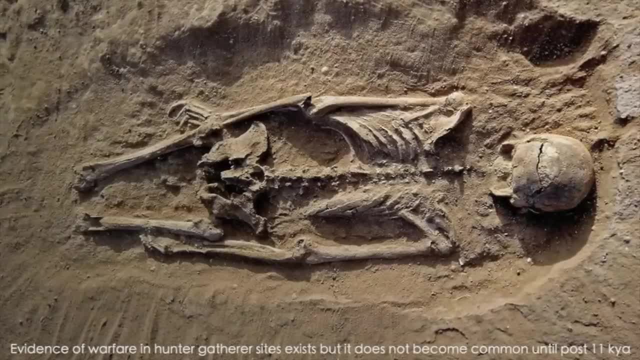 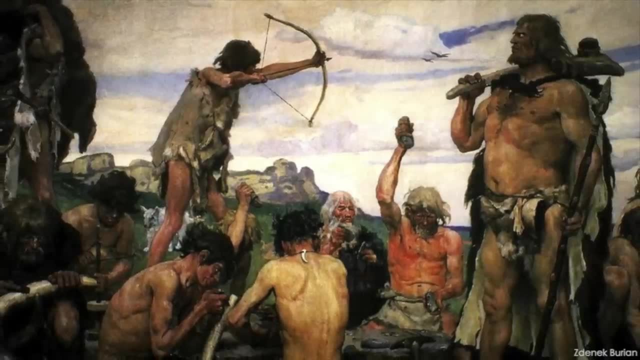 But warfare did not even appear in our own species until we started settling down and our populations rose rapidly. Some anthropologists have even considered warfare to be a form of war. War is believed to be a relatively new cultural invention, that is only around 10,000 years. 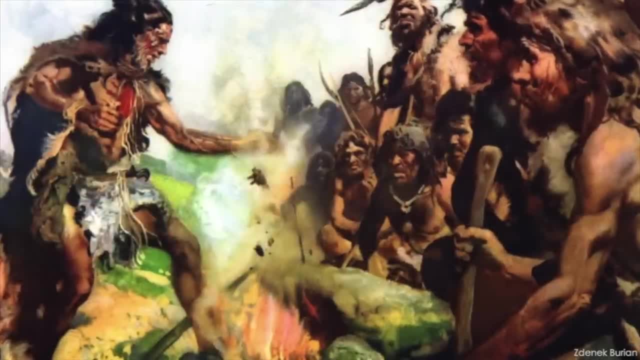 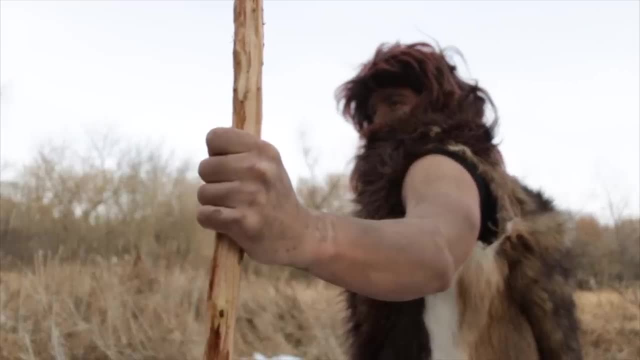 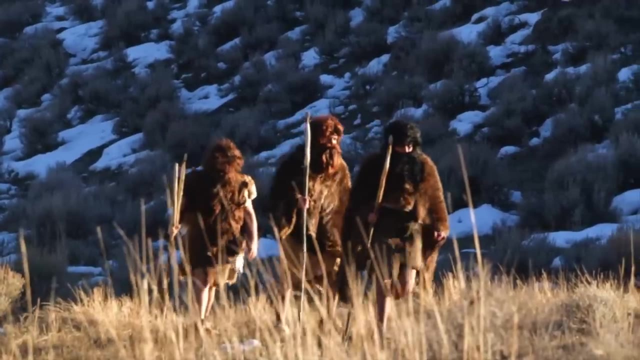 old. Though we think of warfare as fundamental to the human condition, it was actually quite rare during the Paleolithic. When considering warfare during this period, we must define what we even mean. Regarding Neanderthals, warfare would simply consist of separate groups attempting to kill. 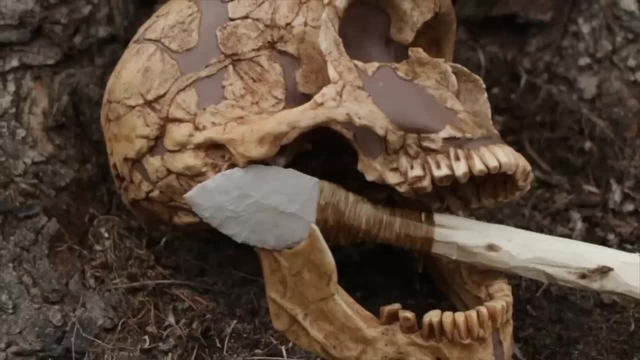 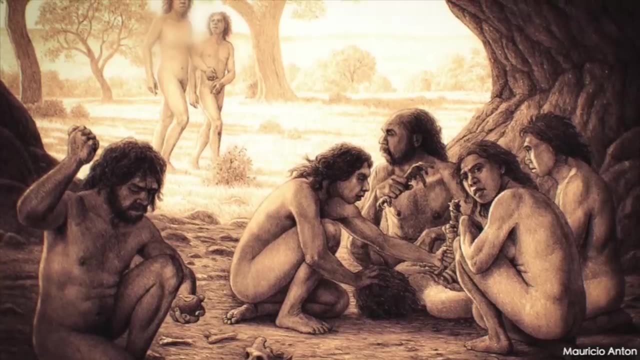 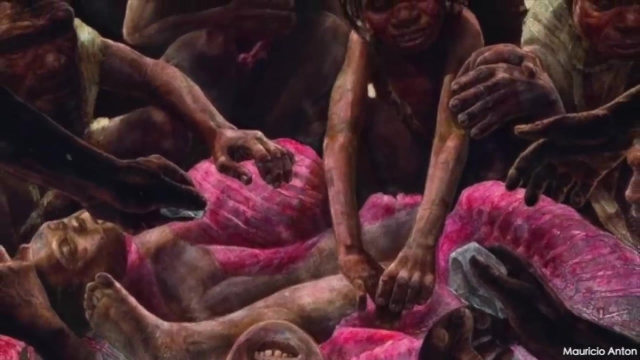 or injure members of other groups. There are only a few examples that we could point to regarding Neanderthal conflict. The Neanderthal family at El Cedron seems to be the victims of a starving group of neighbors. This example may classify as warfare, but seems to be more of a case of survival: exo-cannibalism. 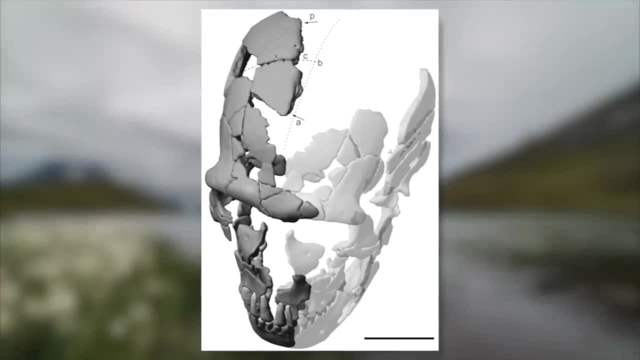 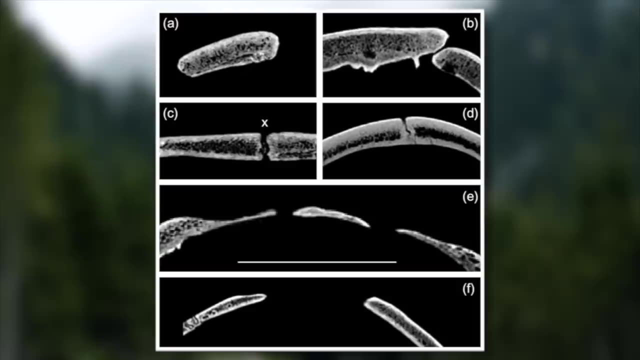 A skeleton from France preserves a healed blade wound on top of an individual's head. Based on comparative and actualistic data, Zollecoffer concluded that this injury was inflicted during an act of intra-group, interpersonal violence. The Neanderthal family at El Cedron is considered to be the victims of a starving group of neighbors. Based on comparative and actualistic data, Zollecoffer concluded that this injury was inflicted during an act of intra-group interpersonal violence. The Neanderthal family at El Cedron is considered to be the victims of a starving group of neighbors. Based on comparative and actualistic data, Zollecoffer concluded that this injury was inflicted during an act of intra-group interpersonal violence. 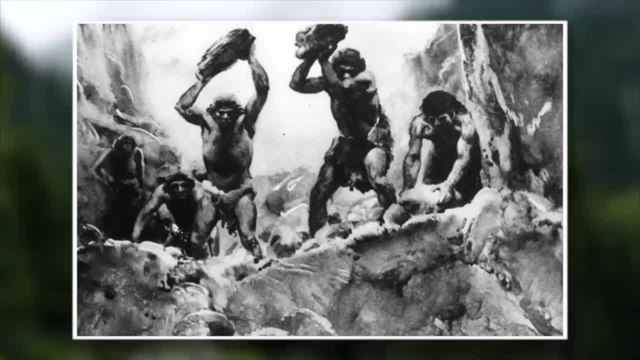 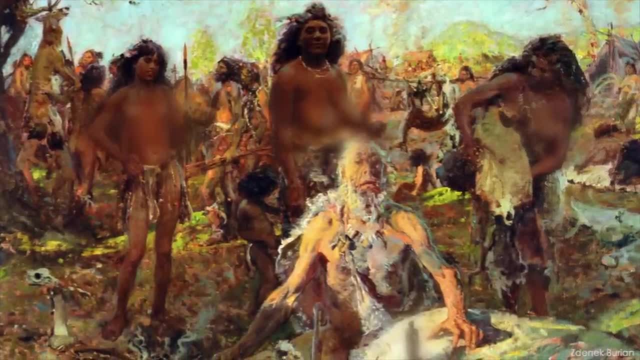 Meaning that the injury was likely inflicted by an individual within the victim's group. He was then nursed back to health by his group and possibly even by the individual that injured him. Considering the wider context, this example is not indicative of warfare with other groups. 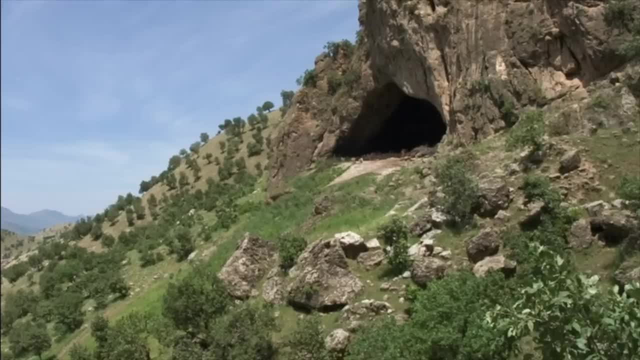 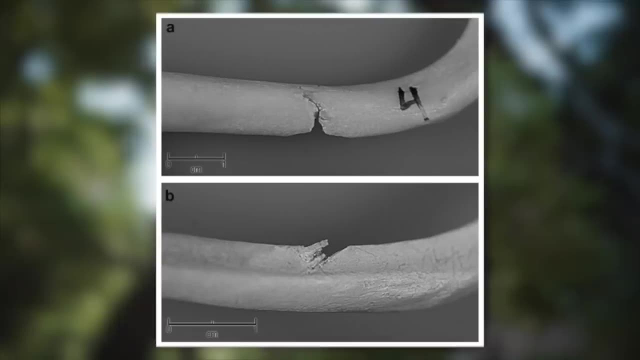 but rather violence within a group. At the Shandandar cave of Iraq, a lesion on the rib of a Neanderthal is characteristic of a projectile weapon. The morphology of this injury is consistent with a low. The morphology of this injury is consistent with a low. 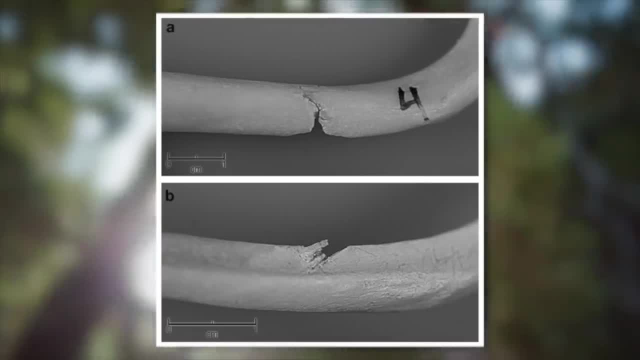 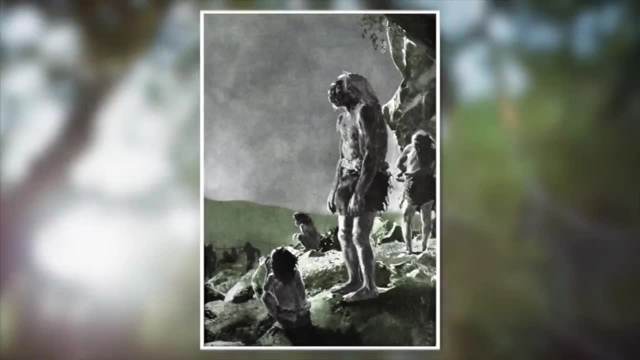 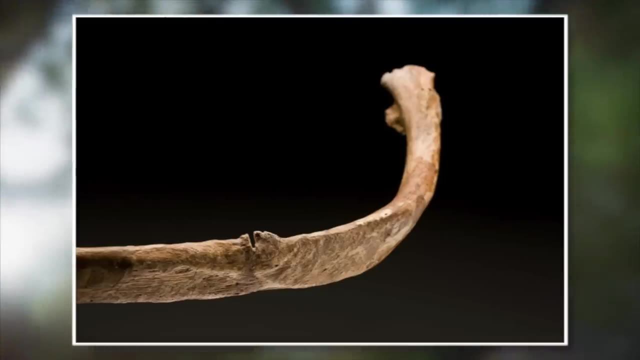 mass low kinetic energy projectile weapon. The injury only damaged one rib, but may have also damaged the individual's lung. Shandandar III was 40-50 years old and may have died due to the wound. Whether it was a hunting accident, an act of interpersonal violence, 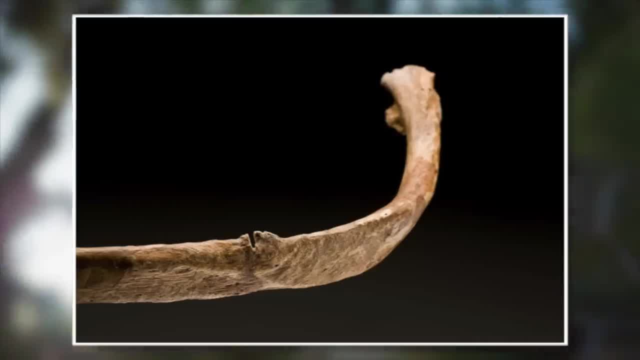 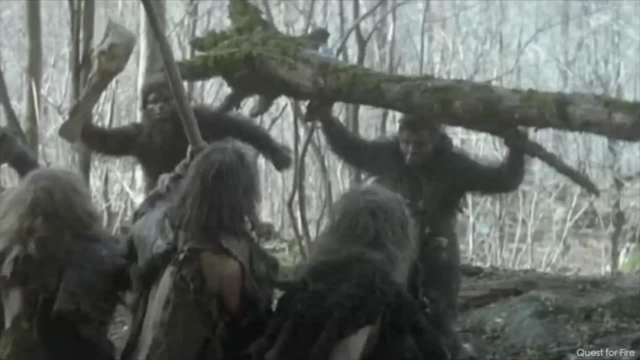 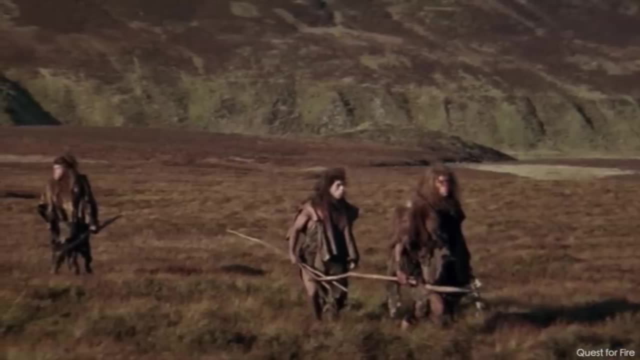 or violence from another group. we may never know. It is possible that it was even made by modern humans, though we just don't know. Overall, conflict and warfare does not appear to have been very common in the Neanderthal world. Neanderthal populations were just too low to make conflict all that common. 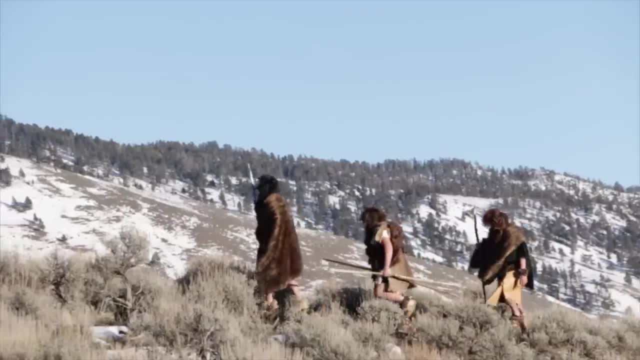 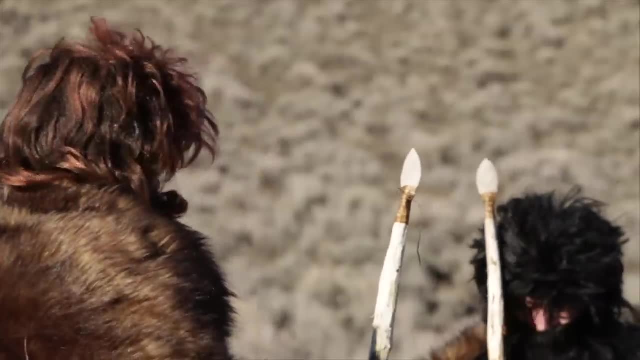 When considering their population density. there just does not seem to have been an incentive for two groups to fight. Since we have talked about the ugliest aspects of the human condition, we should talk about the most beautiful: The expression of art and culture. 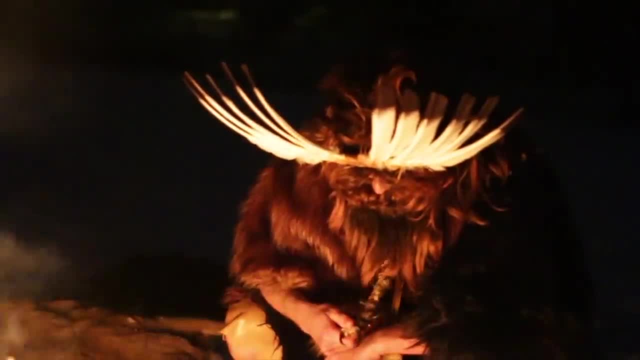 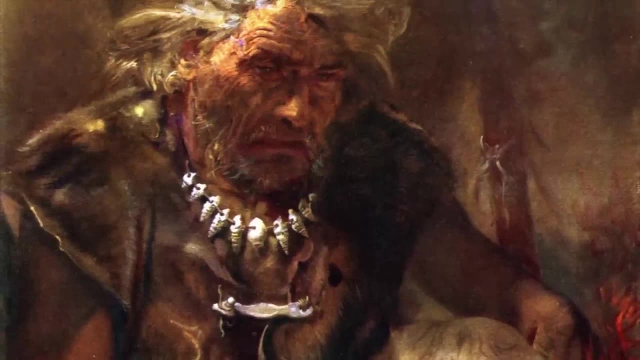 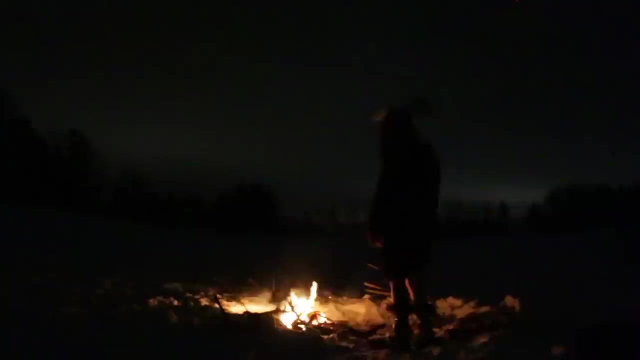 It was once thought that Neanderthals were not capable of symbolism. This was because early modern human remains are full of human remains are full of art, something that was seemingly absent from the Neanderthal fossil record. As more discoveries were made, it became apparent that Neanderthals were capable of symbolism. 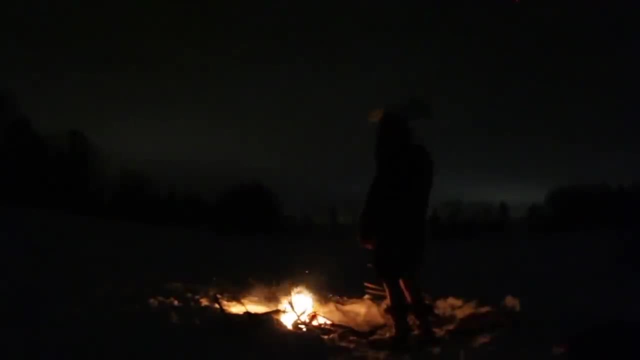 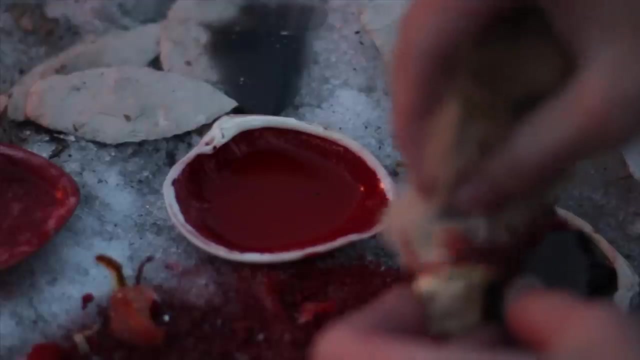 even if it was expressed quite differently than it was in early modern humans. Some of the first indications that Neanderthals may have thought symbolically came from the large amounts of red ochre found at their sites. Red ochre is a term that describes various kinds of iron oxide pigments which can be 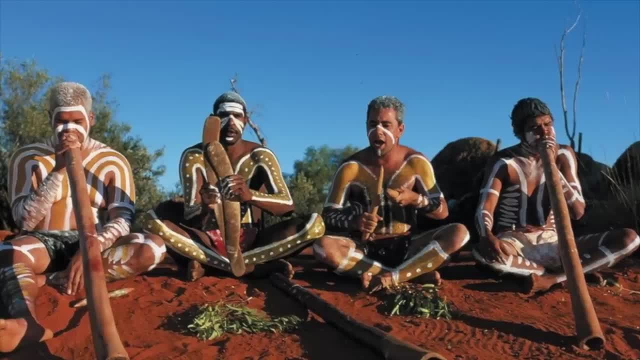 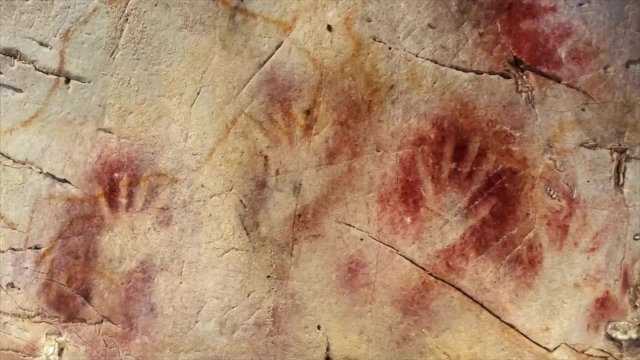 a variety of warm colors. It is still used today across many cultures as a pigment and a medicine, and it was widely used throughout prehistory. Neanderthals used red ochre over 200,000 years ago, around the same time that our own species. 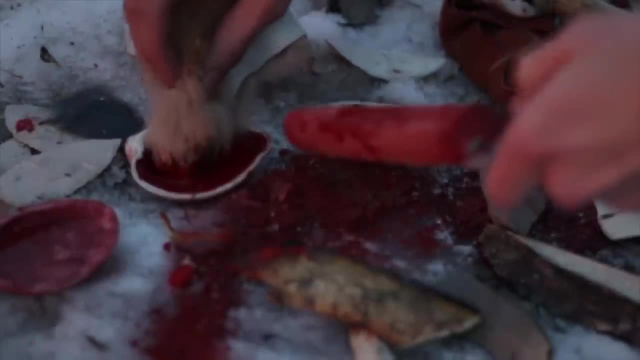 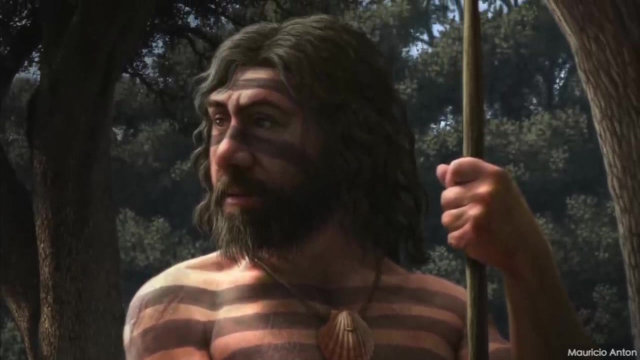 began to use it. Identifying how Neanderthals used this material is quite complicated. If they used it to paint themselves, we will never know. The Himba people of Namibia use a combination of ochre and fat to create a paste. 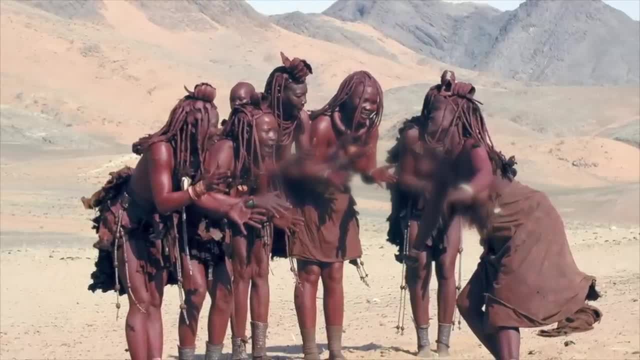 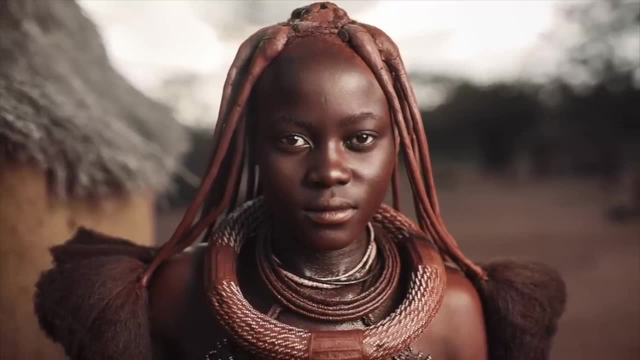 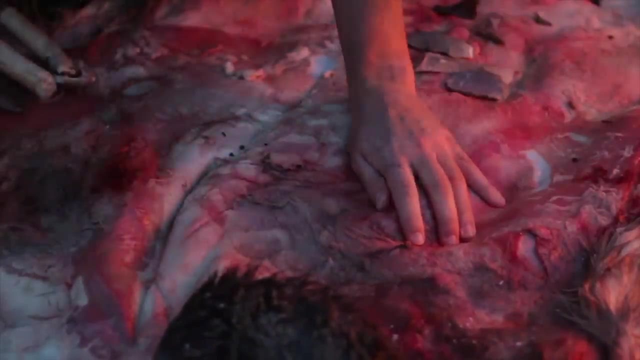 This paste is then spread across their skin and hair to protect themselves from the harsh desert climate. They also use it as a mosquito repellent during initiation ceremonies and during funerals. Other cultures have been known to use it to tan hides or even for food preservation. 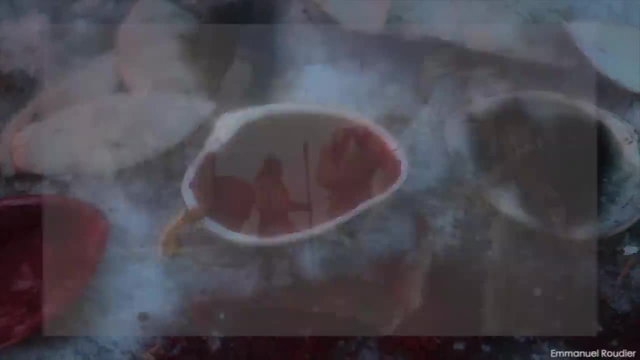 Neanderthals may have been using it in many of the same ways. They may have also used it to paint their clothes or perishable goods, both of which would not preserve well in the forest. Neanderthals may have used it to paint their clothes or perishable goods, both of which would not preserve well in the forest. 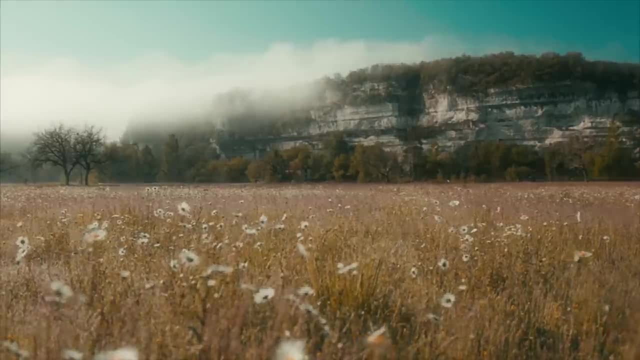 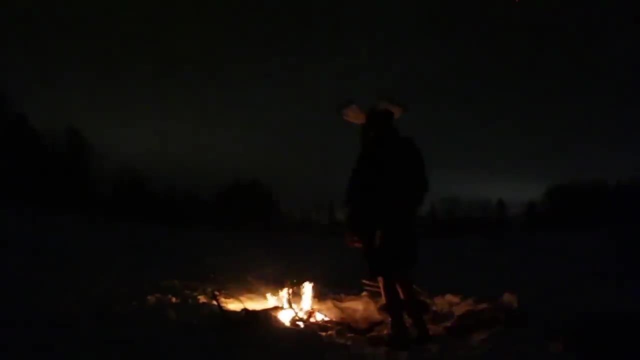 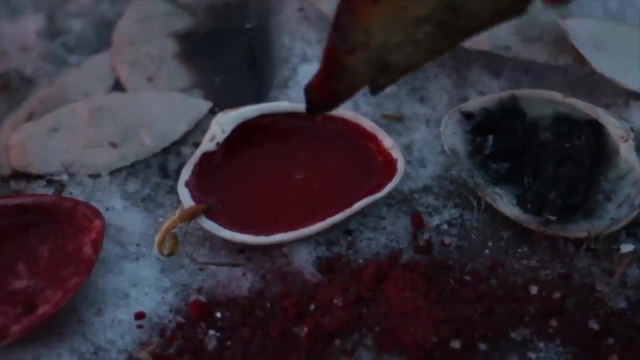 The analysis of pigments from a site in France suggests that they were applied to soft materials such as hides or even human skin. Hides may have been dyed brilliant shades of orange and red for ritualistic events or even just for daily life. Red, ochre and other pigments are also found on some objects. 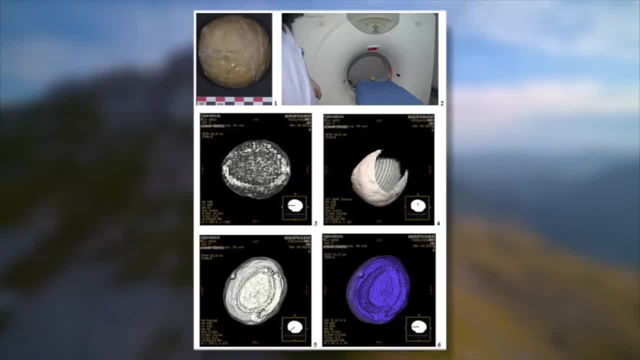 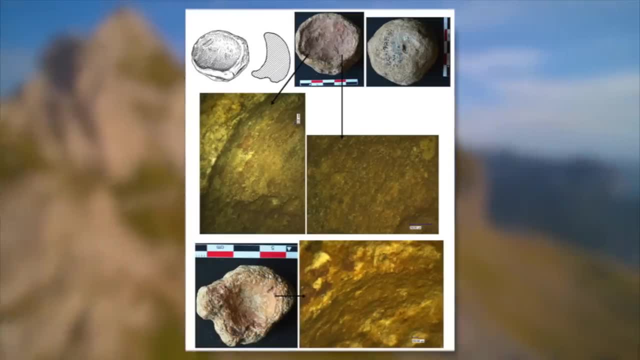 A geode from Romania was coated with red ochre. The strange object was brought back to a cave and painted on every surface. Other containers from Romania have also been laid bare before the state. Containers from the same site, made of stalagmites, appear to have been used as mixing containers. 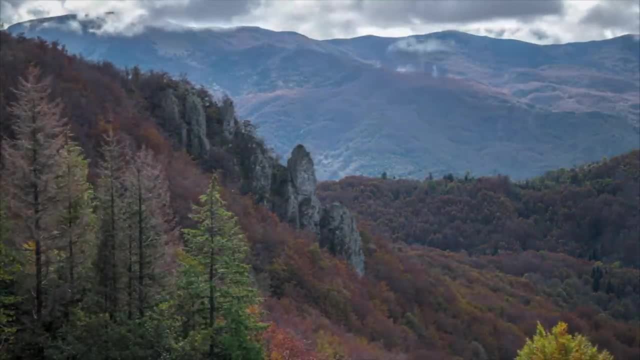 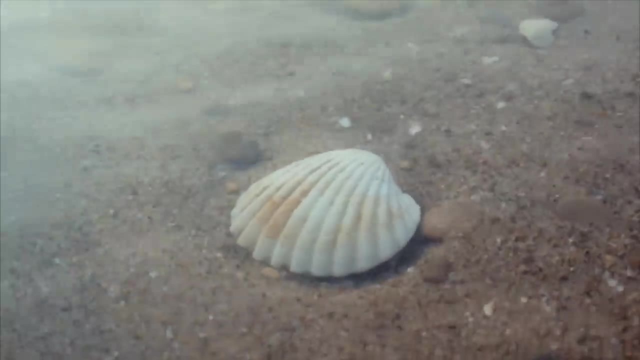 The geode had no practical use, but nevertheless it was carried back to the cave and covered in paint. Other objects that may have been pendants were painted with pigments. A fossil sea-snow shell that may have been painted red was transported over 100 kilometers. 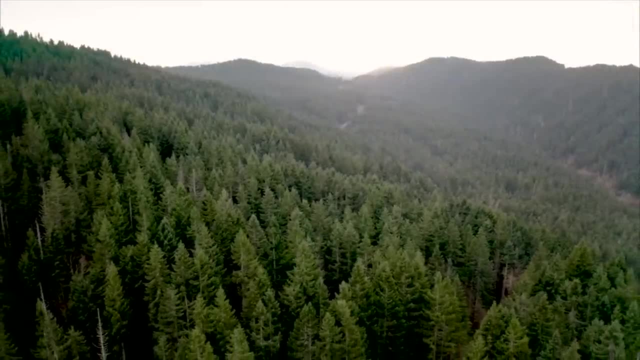 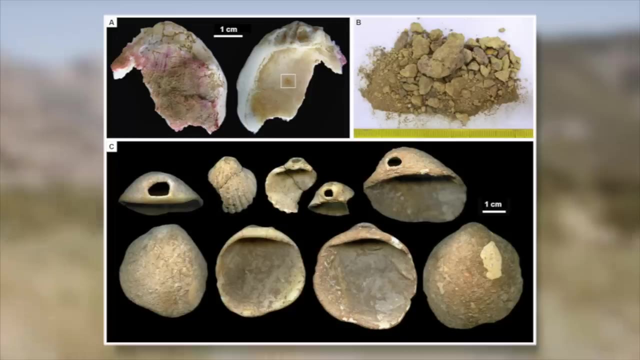 or 62 miles to a Neanderthal site. Other shells from Spain dating over 115,000 years ago were perforated and painted with black, red and yellow pigments. The shells are naturally vibrant on one side and they may have been painted to make them. 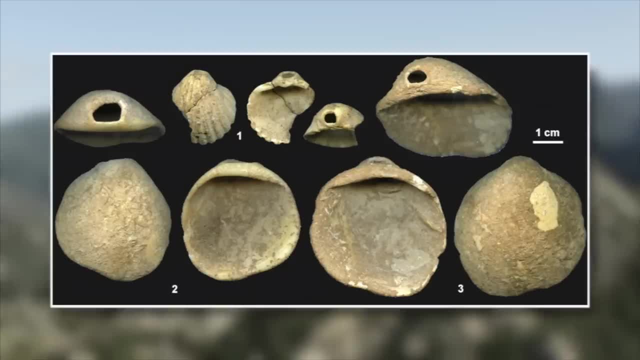 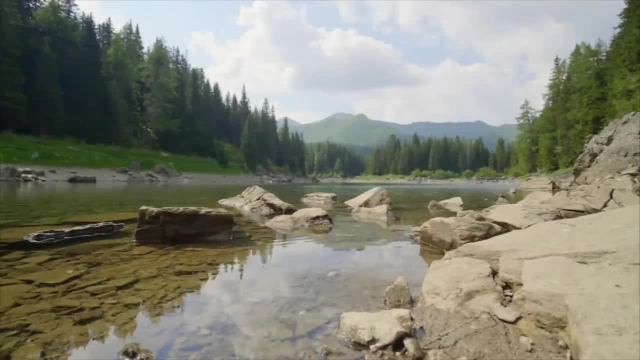 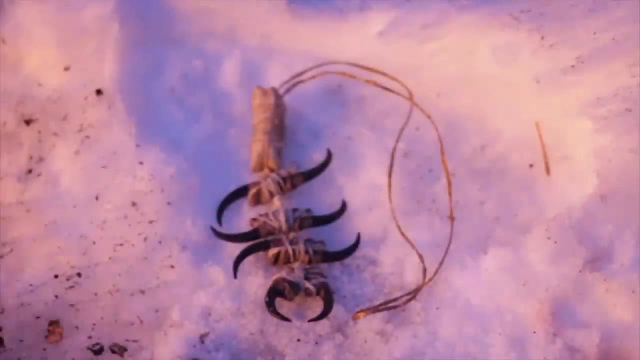 colorful on both sides, Considering they have holes present in them, they may have been strung together to make a necklace. Other evidence of necklaces exists. Perhaps the most interesting evidence comes from the Krpina site of Croatia. Here 130,000 people are buried. 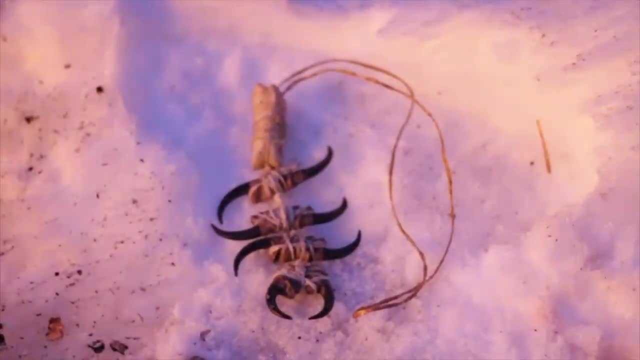 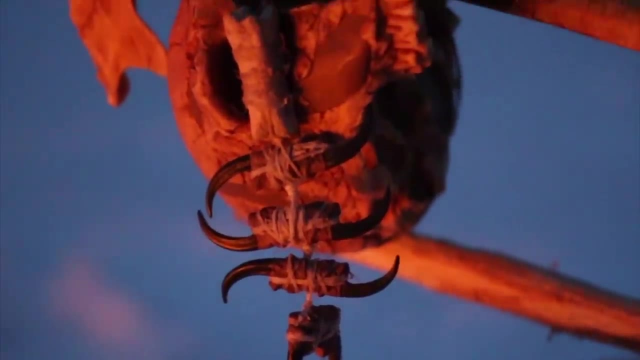 thousand-year-old eagle talons appear to have been strung into a necklace. Eight of these talons were excavated together. The necklace would have taken three to four eagles to create. It is unlikely that all of these eagles were simply found deceased: Deep notches and smooth cut marks. 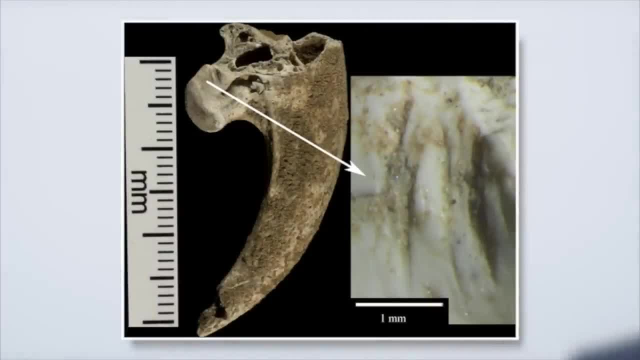 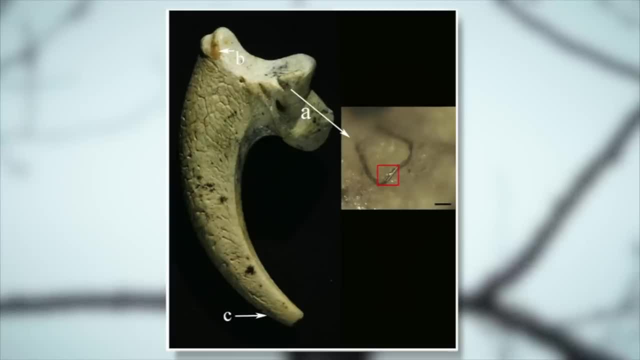 present on the base of the talons would have helped string them together. Recent analysis showed evidence of a fiber still present on one of the talons, which may be a remnant of the leather or sinew that once held it together. Some of the talons even have evidence that red yellow 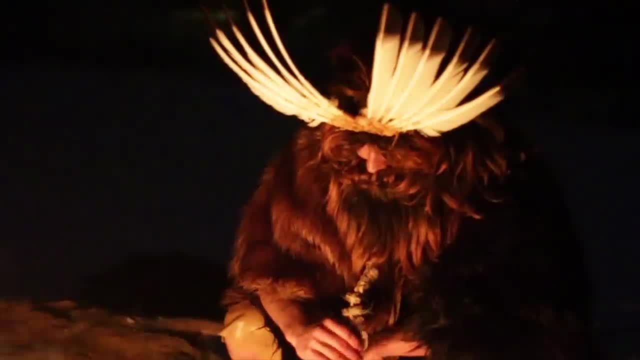 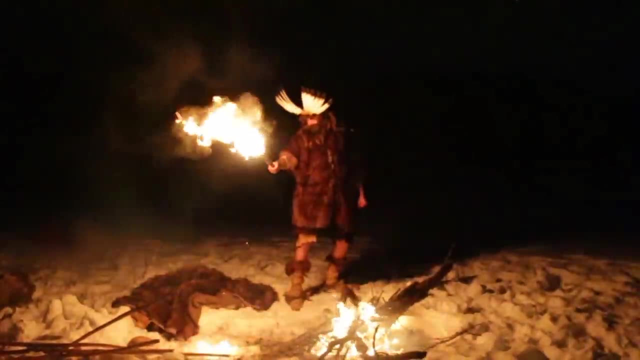 and black pigments were applied to them. This evidence may be the earliest evidence of jewelry in Europe. It may also be evidence that Neanderthals had a symbolic culture long before contact with modern humans. There is evidence of another eagle talon necklace from Spain dating to. 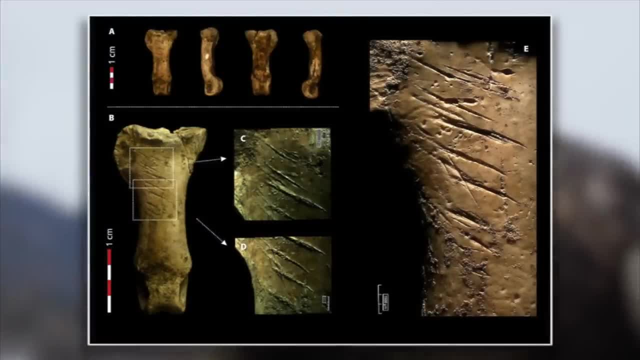 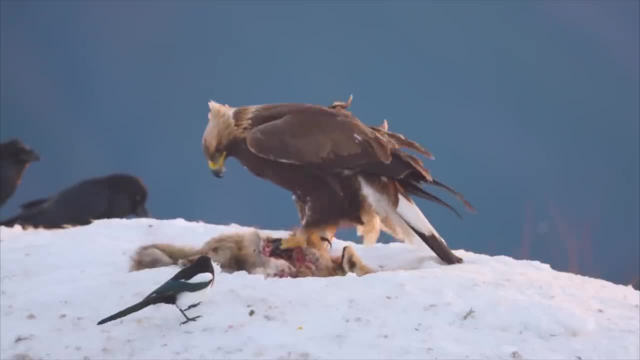 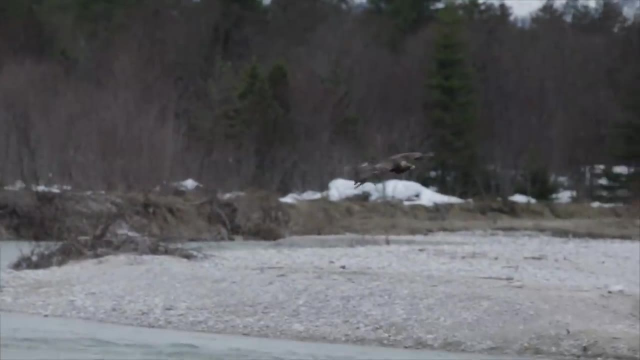 39,000 years ago, though it could have been made by modern humans. Talons are known in other sites as well: The wings of eagles- Interestingly, other parts of these birds without significant quantities of meat on them are present in many of their caves. Wings in general are vastly 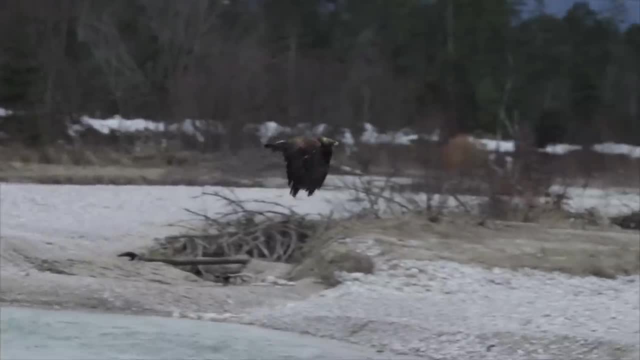 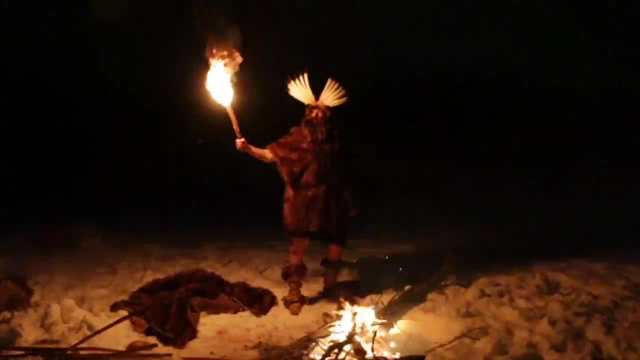 overrepresented in Neanderthal sites. compared to other parts of birds, It appears that Neanderthals mainly selected the primary flight feathers from wings. These feathers do not appear to have any practical purpose. They do not provide any warmth and they are not useful in stabilizing a projectile. 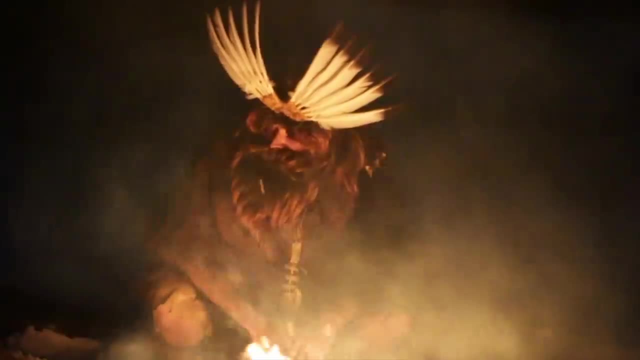 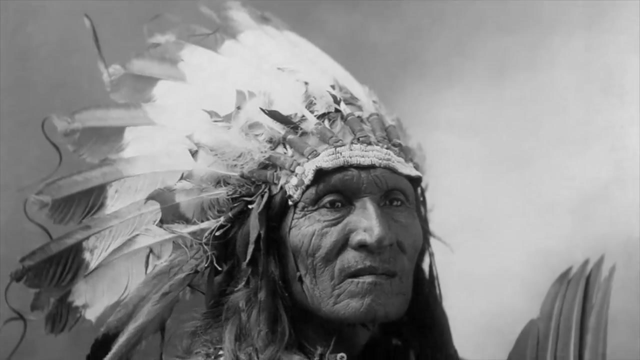 due to the size of Neanderthal spears? The most likely answer would be that they were used for their inherent aesthetic value. Feathers are commonly used throughout indigenous societies for this very same purpose. Another site in Ukraine preserves evidence of modified raven bones. 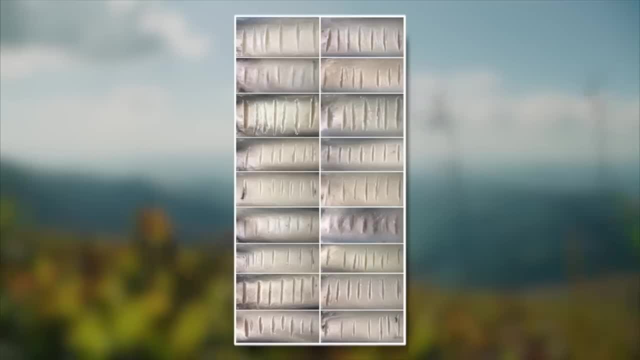 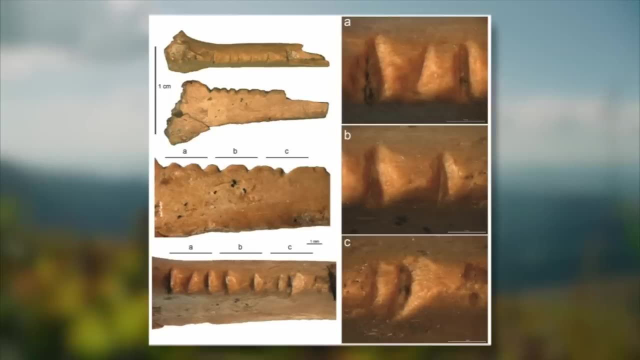 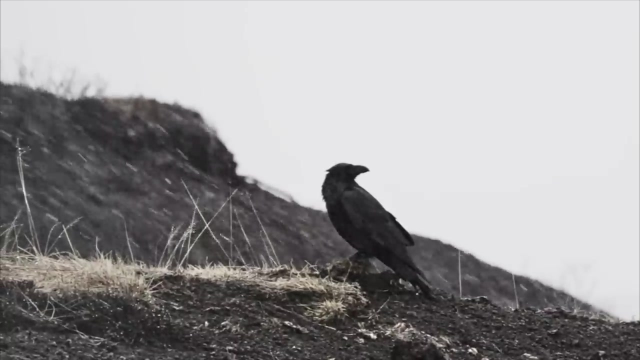 Seventeen of the bones were decorated with intentional equidistant marks. The reasoning behind this is, of course, enigmatic. They could have been made to count to aid in the grip of the bone or for some aesthetic purpose. Either way, this is further evidence of bird bones being interacted with in a way that does not have. 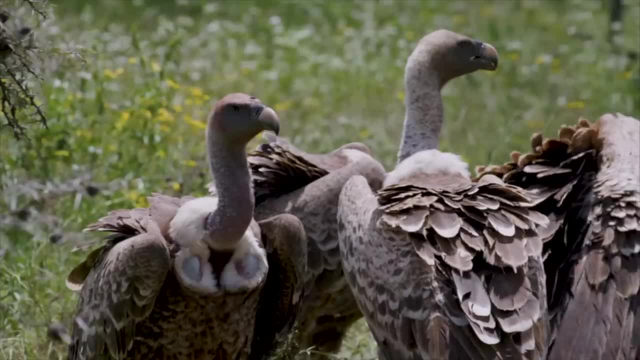 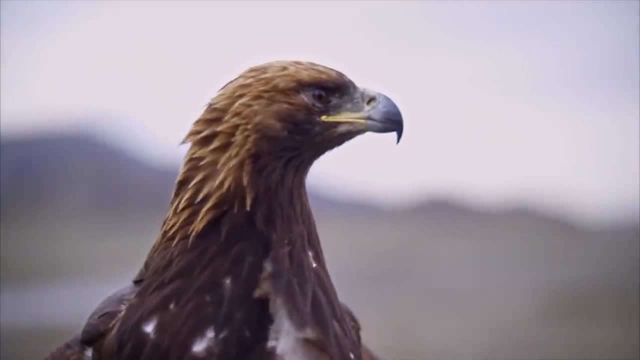 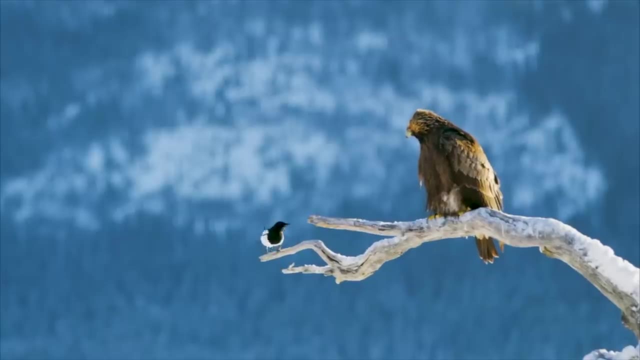 a survivalistic explanation. Birds, especially larger raptors and corvids, may have indeed had a symbolic meaning across many Neanderthal populations. Clearly, these animals are impressive not only in the way they interacted with their environment, but also in their inherent aesthetic. 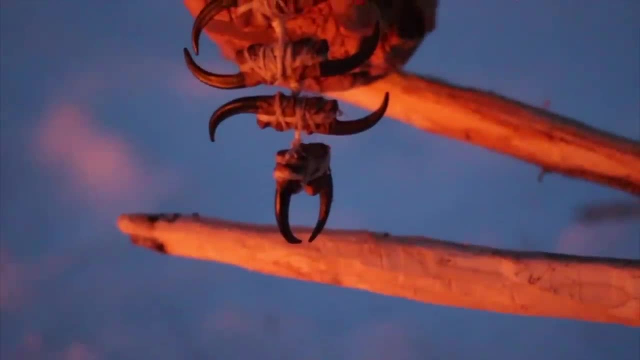 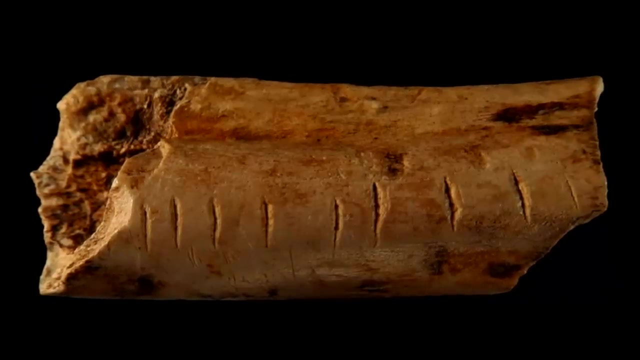 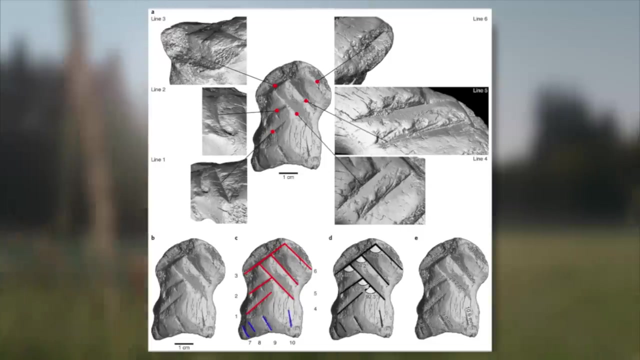 value. Bones from a variety of other animals also seem to have been treated in ways that are not consistent with butchery. A hyena bone from a cave in France has nine strange parallel incisions. Perhaps it is evidence that Neanderthals were counting things. A giant deer phalanx from Germany. 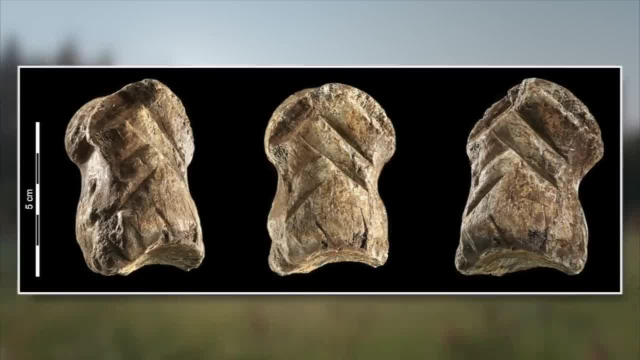 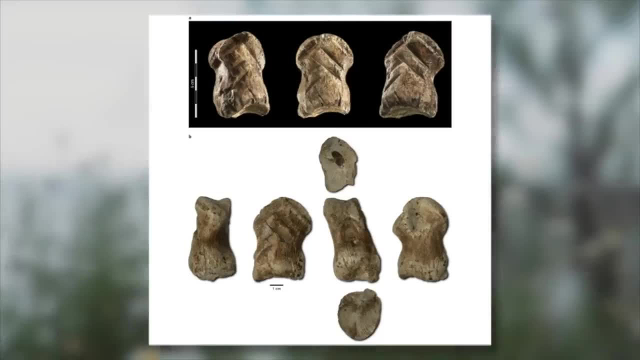 has even stranger markings. The bone appears to have been cleaned of tissue and probably boiled After drying. it was then carved with slanted intersecting lines and smaller tick marks. Carving these deep notches would have taken some time, and it was certainly not accidental. 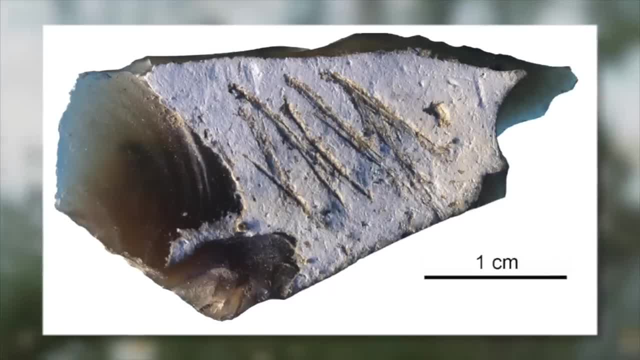 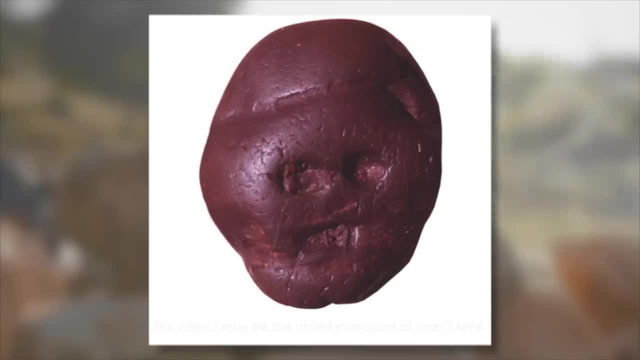 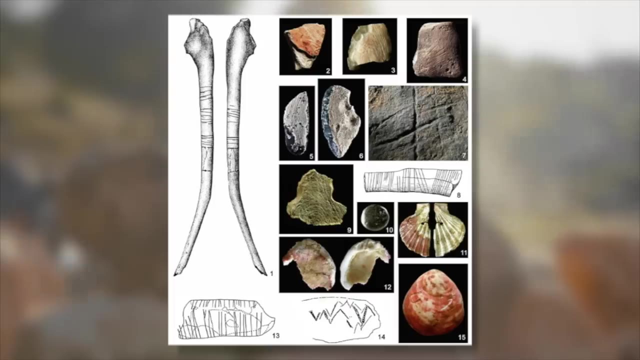 A piece of flint from the Crimean mountains has 13 deep lines scratched into the cortex. The lines would have had no practical function. Unmodified natural objects known as manuports are known throughout many Neanderthal sites. Neanderthals transported various rocks and even fossils to their sites. 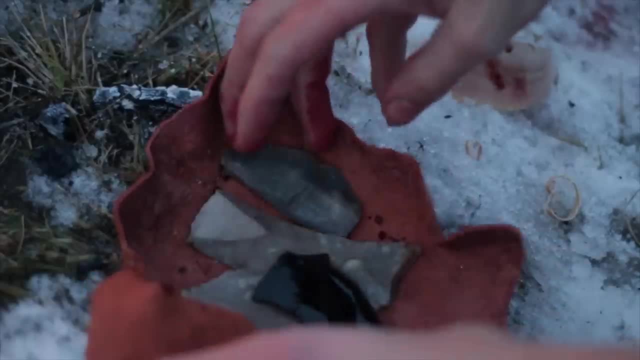 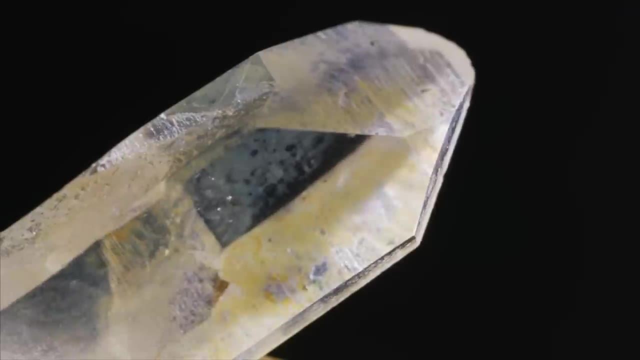 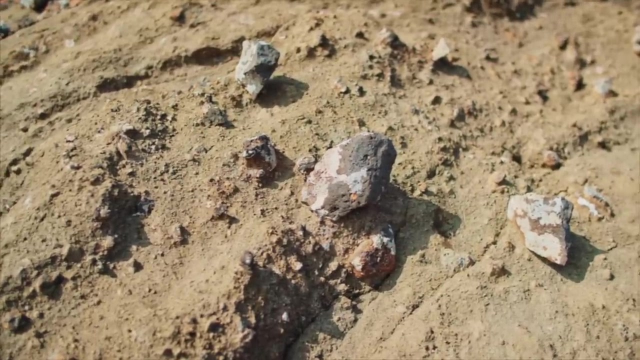 Some of these objects do have practical purposes, but we cannot look past their eye-catching looks. Quartz crystals can be napped, and Neanderthals certainly did nap them, though others were left unmodified. Other minerals that they brought into their sites include ceresite, iron, pyrite, calcite and galena, A variety of fossils of aquatic organisms. 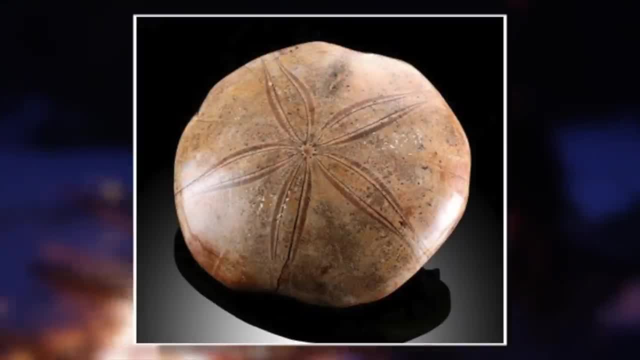 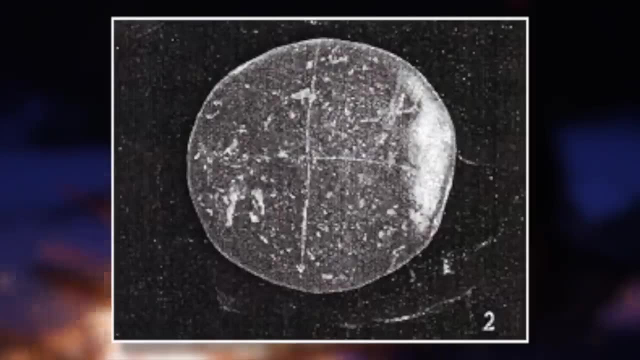 have been found at their sites, including shells, polyps, sea urchins and belemonyte beaks. A fossil pneumolite shell from Hungary even has a cross etched into it. Some of these aquatic animals would have been familiar to Neanderthals and may have been strange. 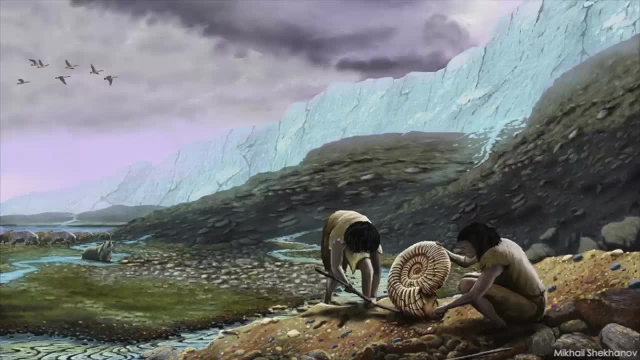 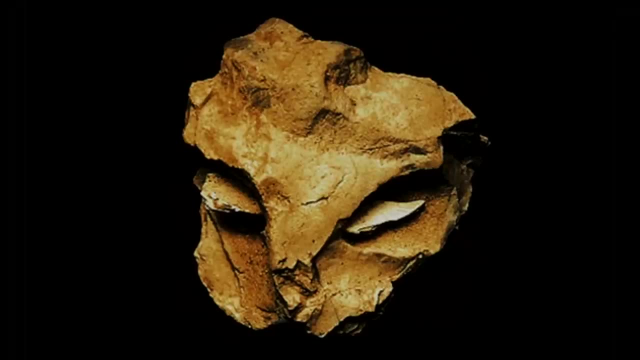 for them to see in the medium. Some of these fossils have been found at their sites, including the Neanderthal's stone. Though they did not understand how these fossils came to be, they undoubtedly found them to be interesting. Another fascinating artifact recovered from a Neanderthal site is the mask of Laroque Cotard. 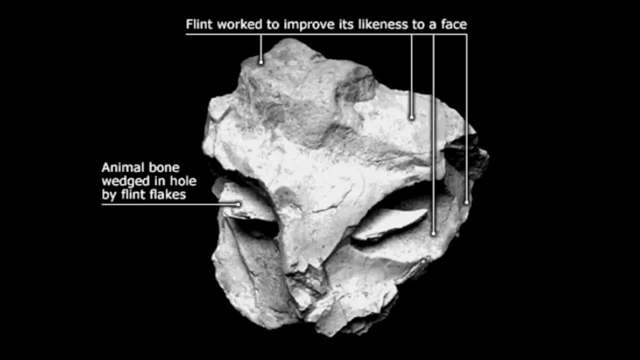 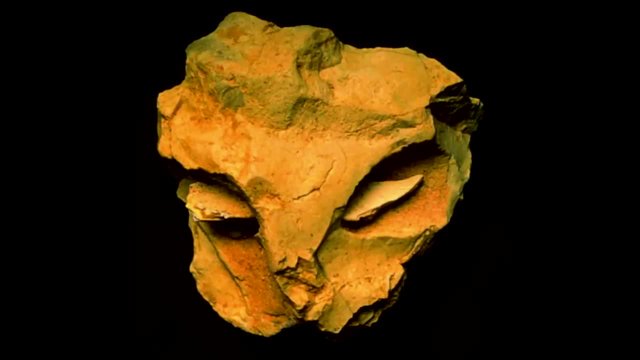 It was made of a piece of flint with a bone pushed through a hole on the midsection. It has been interpreted to resemble the upper half of the face, with the bone representing eyes. It may represent a human or even animal face. The actual function of 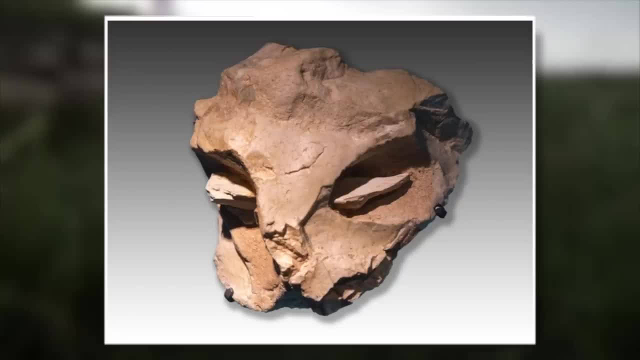 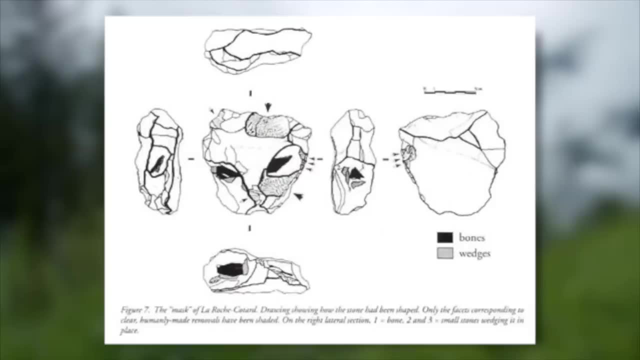 the mask is unknown. It is unlikely that this artifact would have been worn, considering it is made of a heavy piece of flint. It has been argued that it may have actually been a device for tying knots, Though it would be very coincidental that it was used for a different purpose. 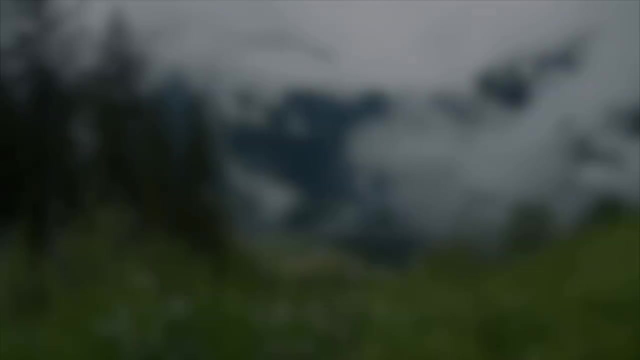 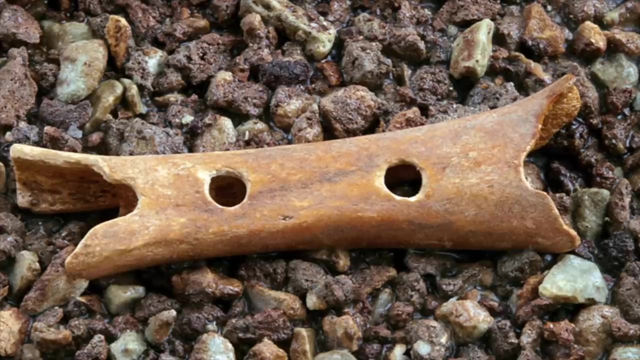 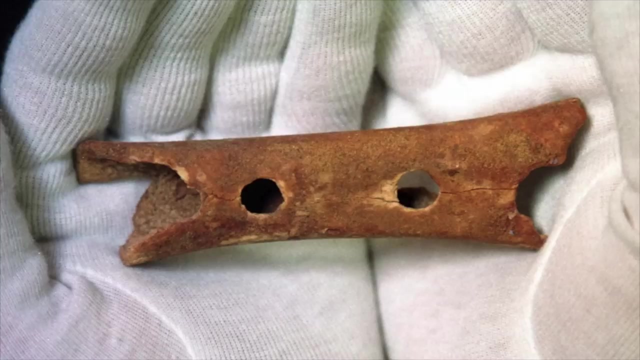 yet resembles a face. its purpose remains unknown. Another intriguing object found at a Neanderthal site is the Divje Babe flute. Canadian musicologist Robert Fink said that the original flute had either a diatonic or pentatonic musical scale. This artifact is very controversial. Some claim it. 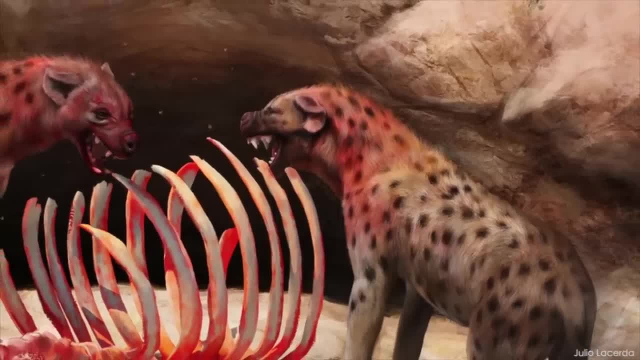 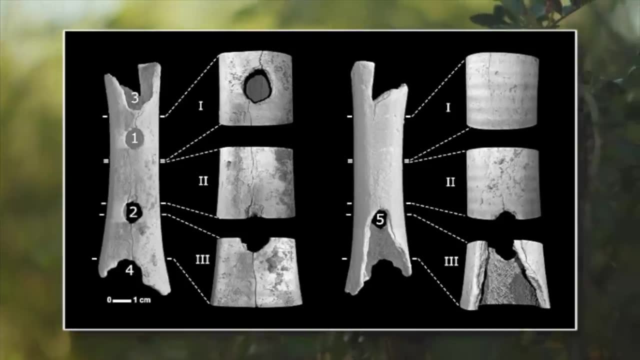 to have been made by modern humans, and others think it may have been made by a carnivore bite. The bone comes from a very young cave bear. The holes were likely made by humans and seem to have been deliberately spaced. It remains unknown whether it was a musical instrument Another. 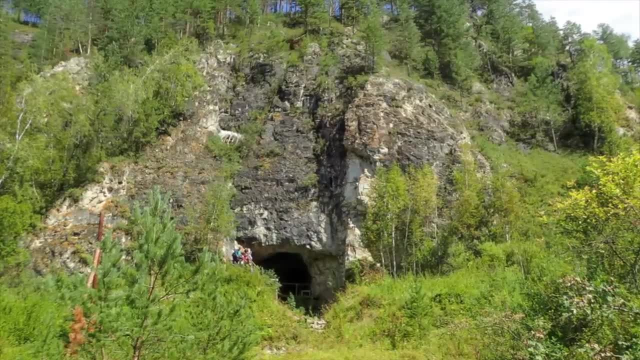 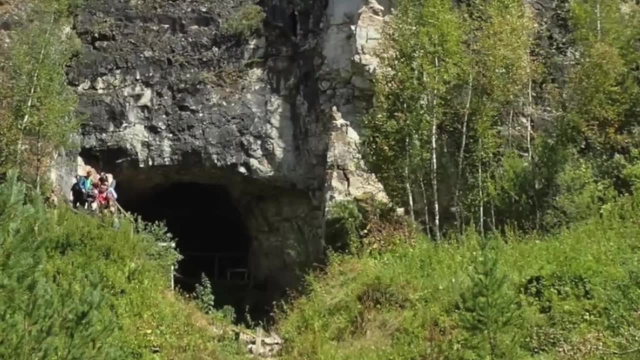 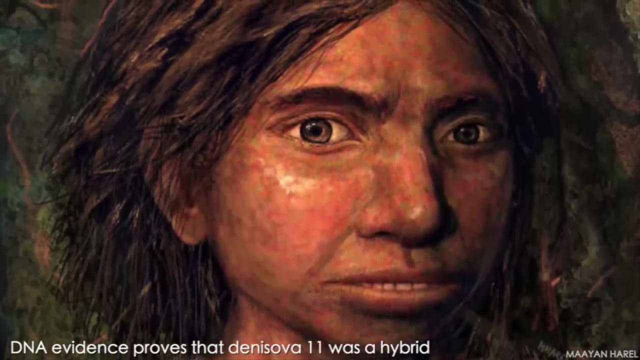 place where stunning artifacts have been found is at Denisova Cave. Though Denisova Cave is typically known as the place that housed Denisovans, Neanderthals also lived there. In fact, a girl that lived at this cave 90,000 years ago was the daughter of Denisovan and Neanderthal parents. 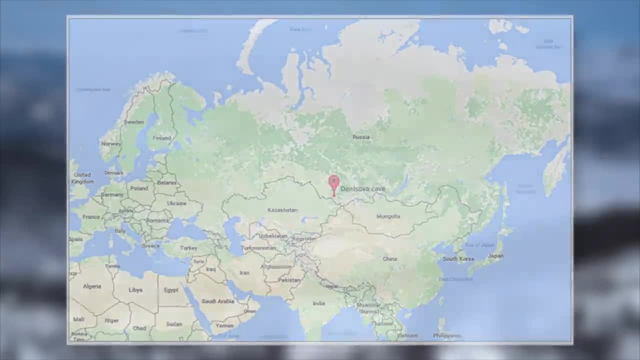 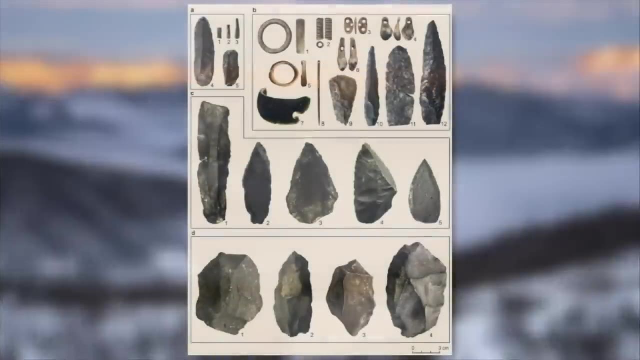 This cave is the farthest east that we know Neanderthals lived. It is hard to tell how often Neanderthals would have been in the area, but we know at certain times they were. Artifacts from this cave become exceptionally interesting in younger layers dated to around 48,000 years ago. 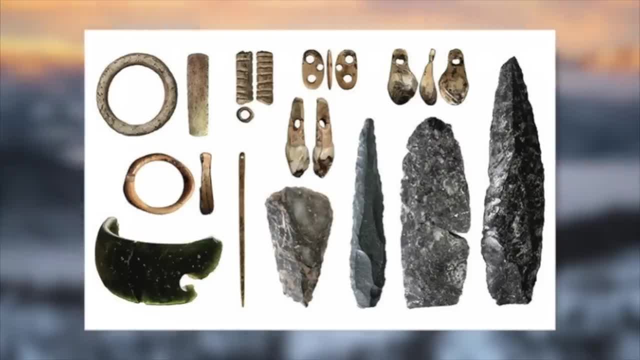 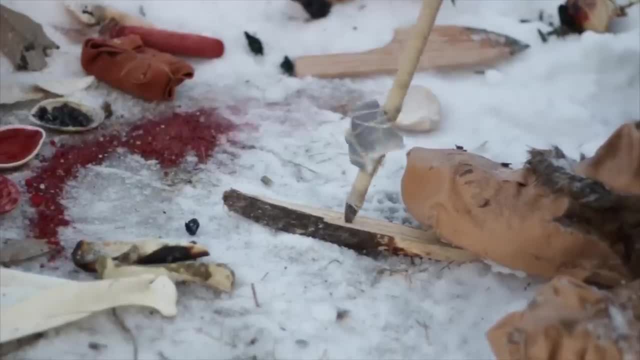 In these layers there were many pendants, ostrich eggshell beads, a beautiful stone bracelet and even a bone needle. These objects suggest that the inhabitants must have had drill technology. A stone hand drill could have worked, but a bow or pump drill would have been much better. 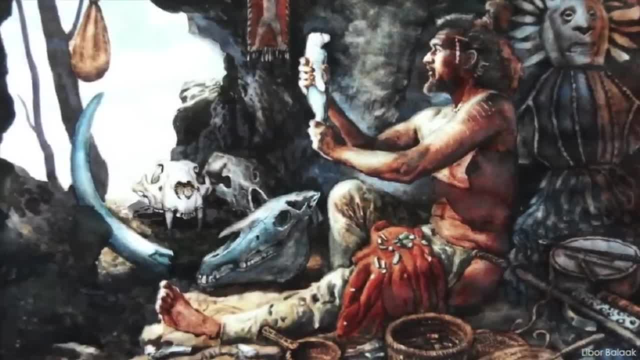 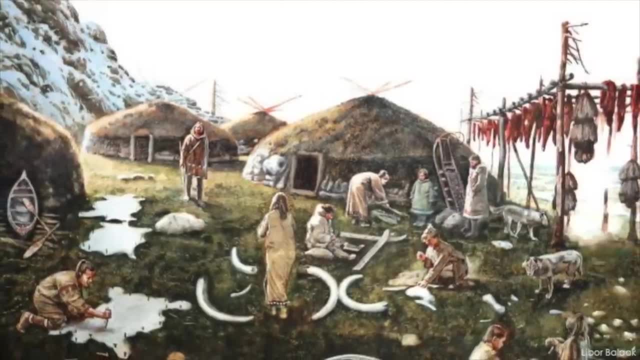 These artifacts are much more indicative of a modern human assemblage, and they may have been made by them. Modern humans were in Siberia during this time and they likely had a role in the creation of these tools, Though we cannot rule out the possibility that. 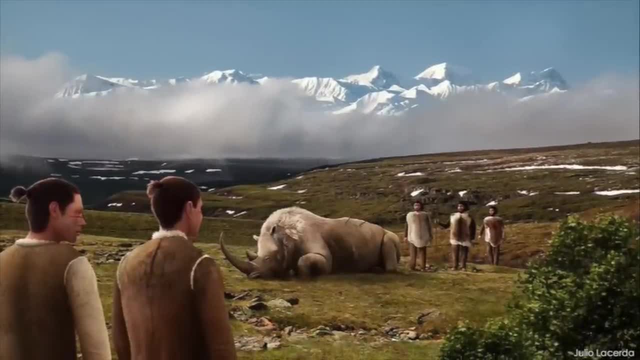 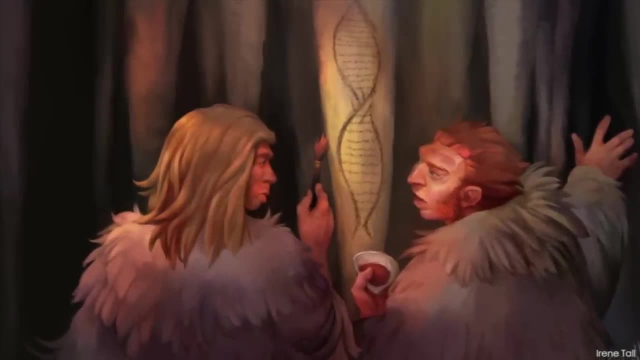 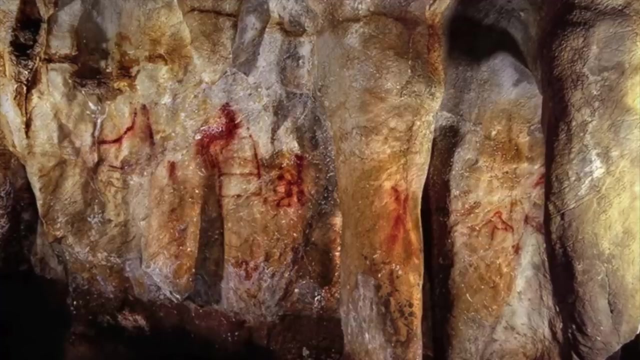 Neanderthals, Denisovans or even a hybrid population between all three of these species were responsible. Besides artifacts, Neanderthals also decorated their living spaces to some extent. Art from Maltraviso cave, also located in Spain, has been dated to 64,000 years ago. 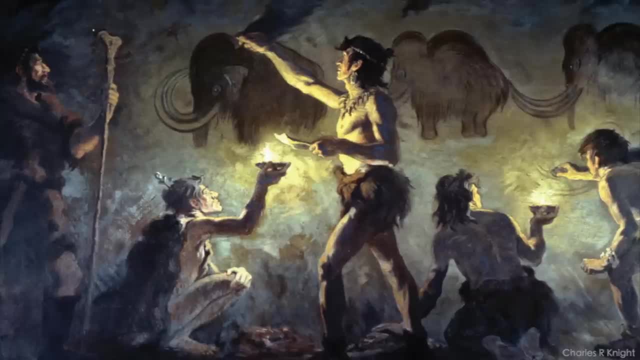 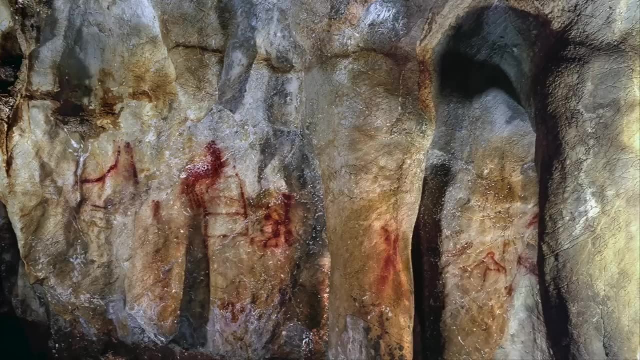 It was once thought that these paintings may have been made by homo sapiens, but after a new dating technique was used, it proved that these were the work of Neanderthals. They are the oldest cave paintings found anywhere on earth. They show abstract symbols and even what appear to be animals. 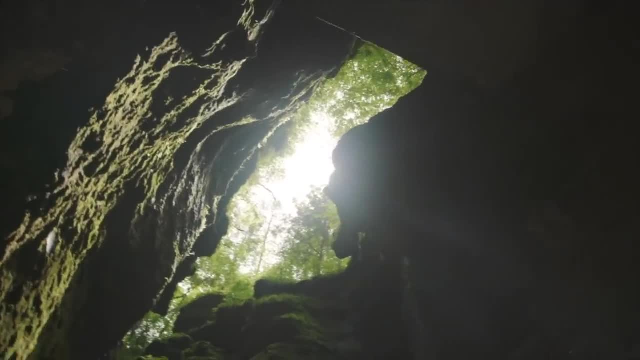 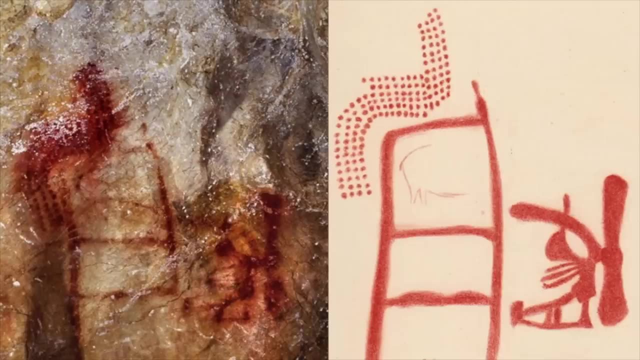 In order to create these works, they had to venture deep into the cave with the aid of a light source. Interpreting what these symbols may represent is very difficult. A geometric ladder like shape was made. Above it, over a hundred dots of paint were placed. 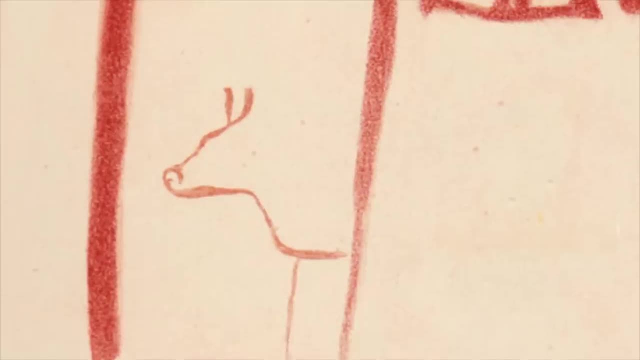 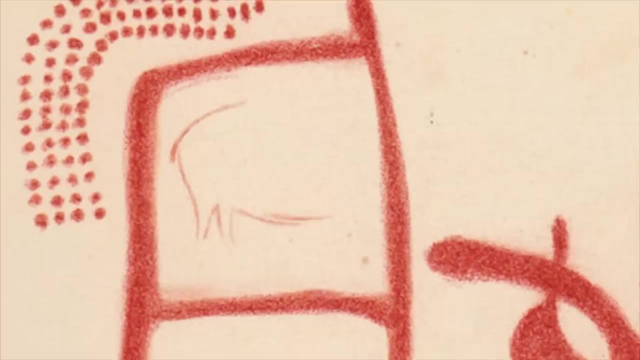 This would have taken precision and patience. Two paintings of what have been interpreted to be animals filled two of the latter's holes, Both bulbous looking herbivores, Though these paintings may have actually been made by modern humans later. Then, to the right of the work, a very strange. 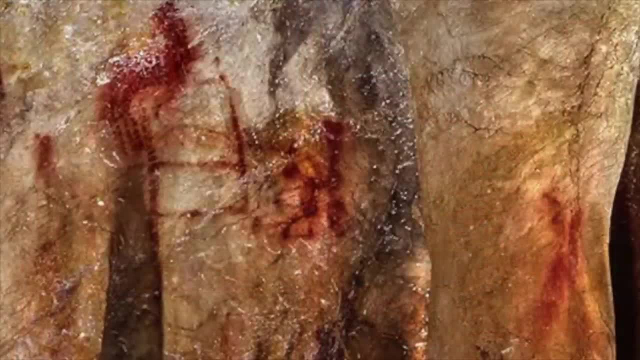 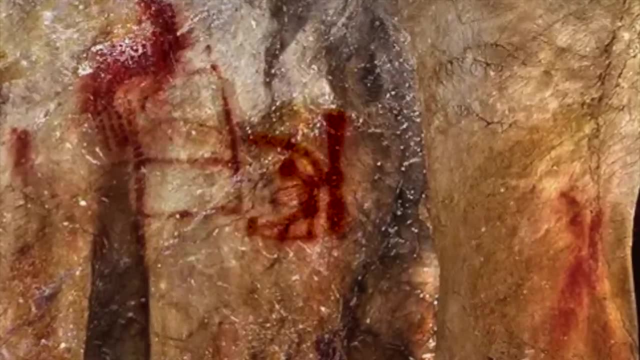 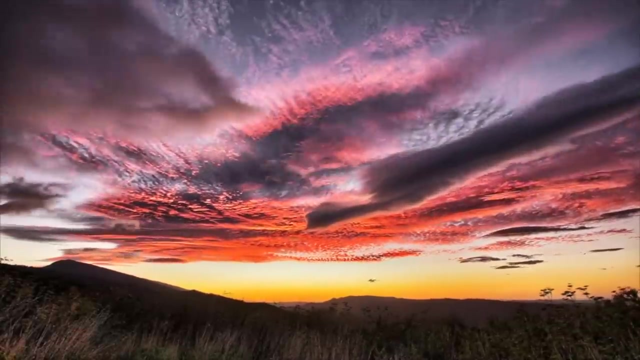 and complex symbol was made. It does not look to be a depiction of an animal or anything of the natural world, A purely symbolic creation. We can only imagine what the purpose of this painting was. Could it represent their culture or clan? A spoken word or a song? Maybe a depiction? 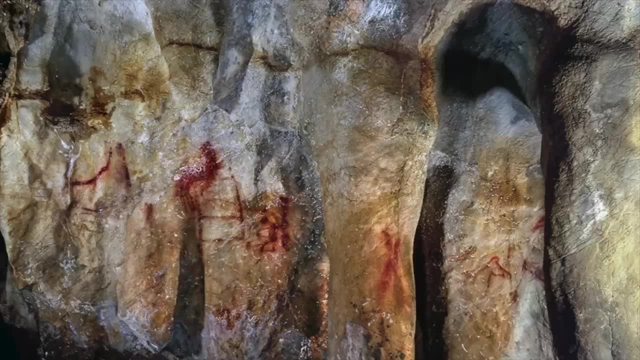 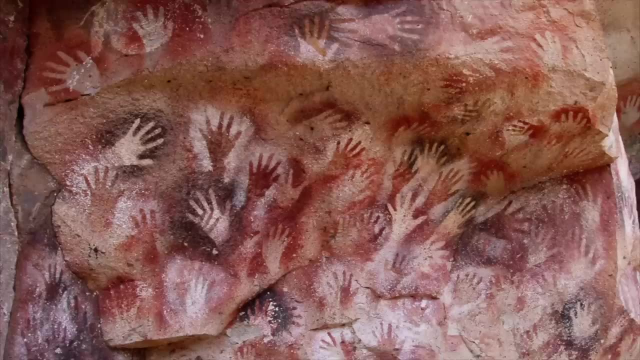 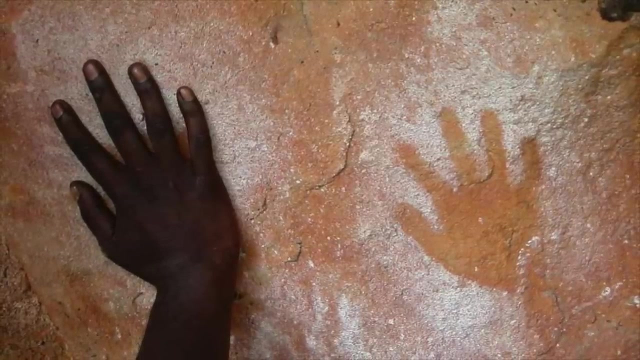 of a primordial creation deity? In truth, we will never know. In this cave there also exists a couple of red ochre hand paintings, A trend that would be very widespread throughout the upper Paleolithic. Some hunter-gatherers in Australia still practice this ancient tradition Likely. 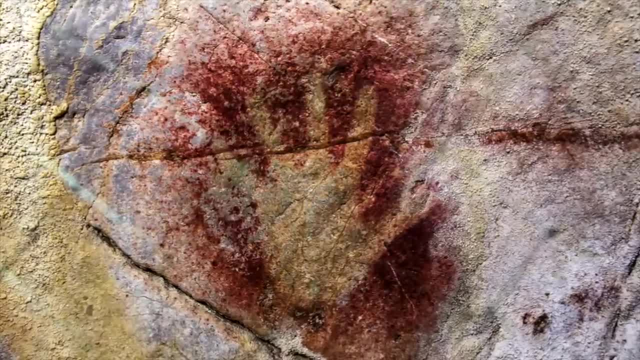 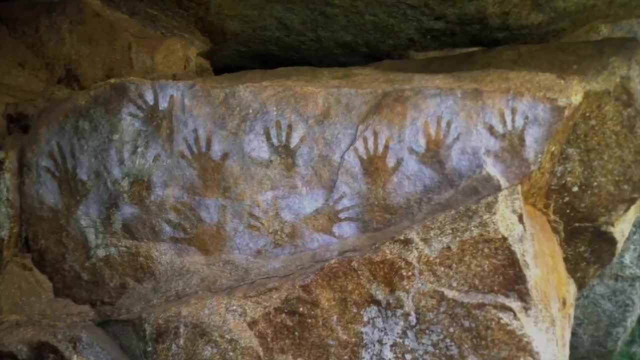 the longest living expression of art, A mark of one's hand, The stone age way of saying: I was here. Looking at walls of these handprints can sometimes be eerie. Though they were distant in time, they were no less human. Their lives were as detailed and as 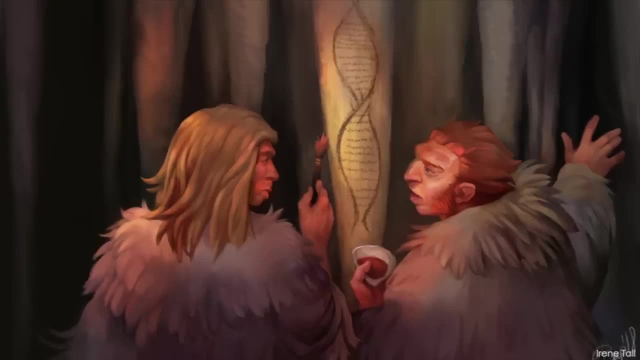 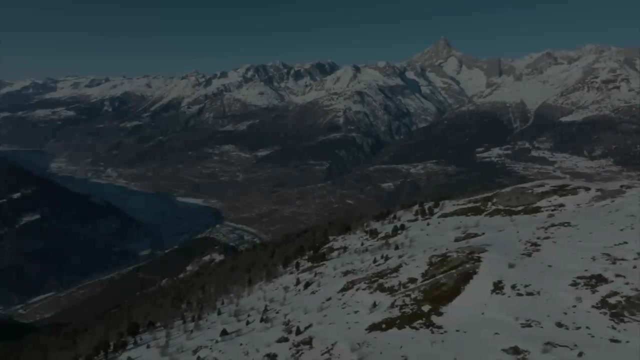 complicated as the ones we're living right now. It seems now that Neanderthals may have been the pioneers of art, rather than the artless brutes that we once thought they were. This discovery has opened the door to the possibility that other European Paleolithic art could have been created. 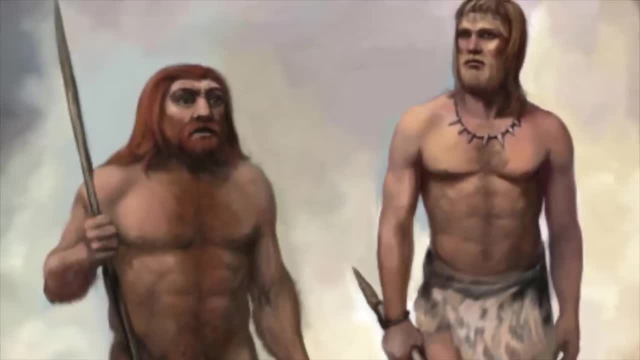 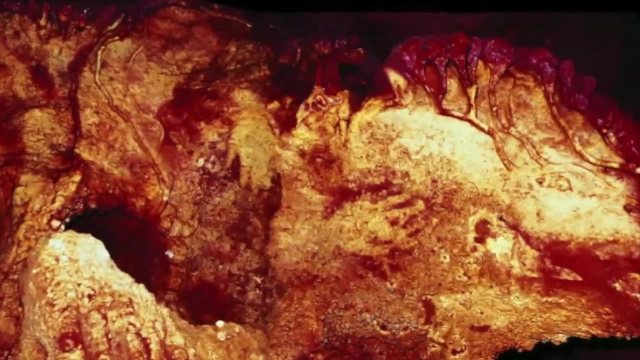 by our evolutionary cousins. Since Sapien and Neanderthal occupation overlaps, we can only say that the art of Neanderthals is not the same as the art of Neanderthals. The art of Neanderthals was undoubtedly Neanderthal if it was older than about 44,000 years old At the site of Leroux-Cotard. 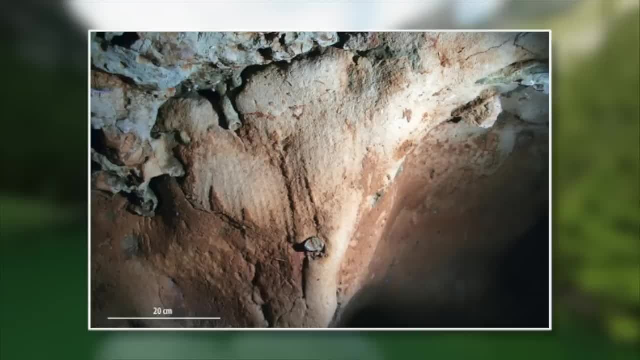 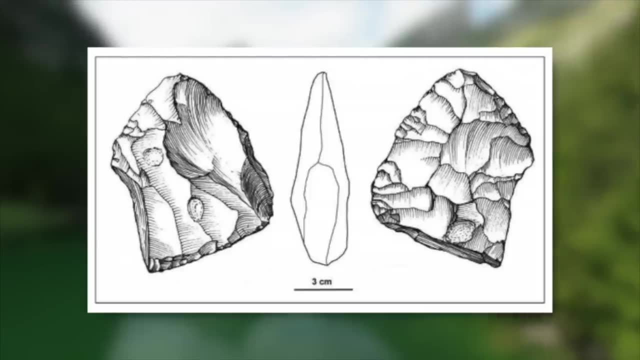 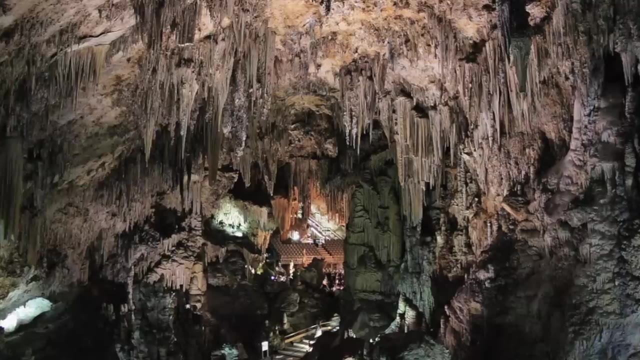 the same site as where the mask was discovered. evidence of red pigment on the walls, as well as finger marks, were likely made by Neanderthals. The site has tools characteristic of Neanderthals, as well as faunal remains dating to over 44,000 years old. Another cave in southern Spain. 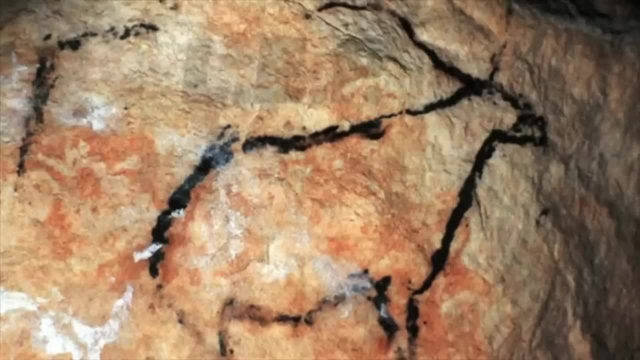 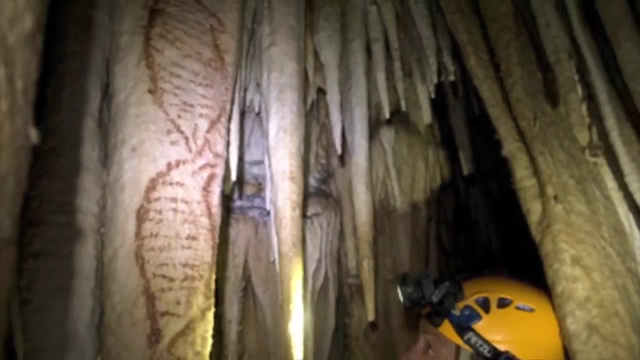 called the Cave of Nerja, has various works created over the past forty-some thousand years. Recent dating methods have shown that some of the paintings are well over 42,000 years old. This has led some to speculate that they may be Neanderthal in origin. 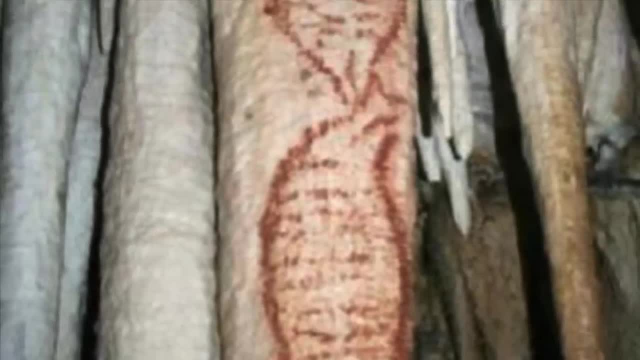 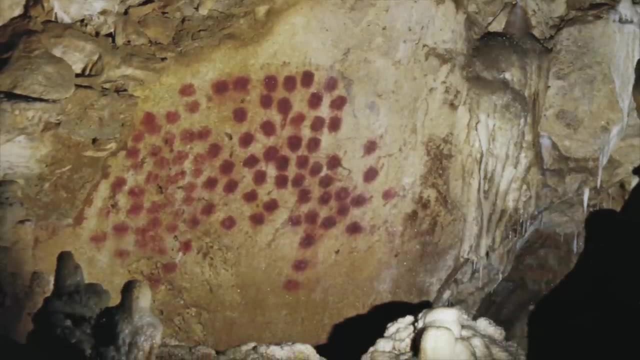 The paintings of two seals are among the oldest in the cave, which is an animal not commonly seen in cave art. Other cave art found around southern Europe could have been made by either Neanderthals or modern humans. These species both co-existed in the region for a few thousand years. 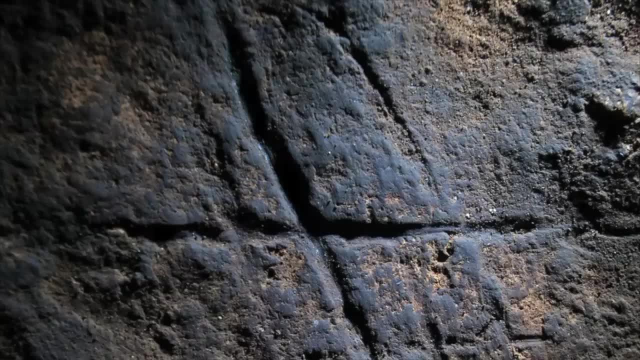 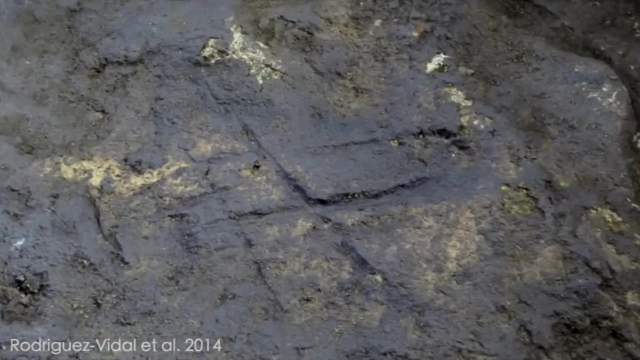 At Gorham's Cave, Gibraltar. scratch marks on the floor have been interpreted as art. Thirteen intersecting lines were scratched deep into the stone over 40,000 years ago. It would have required an estimated two to three hundred scratches to produce this pattern. 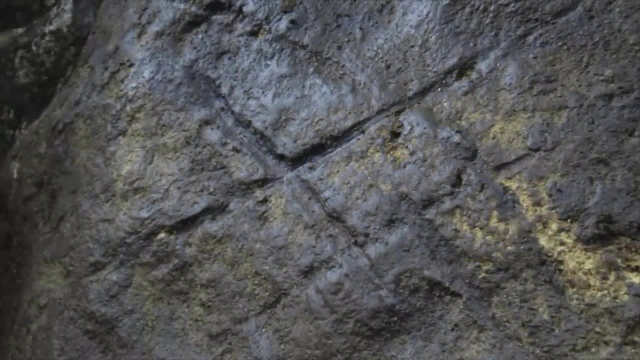 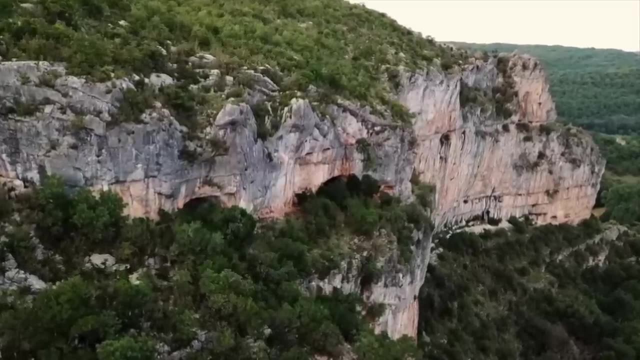 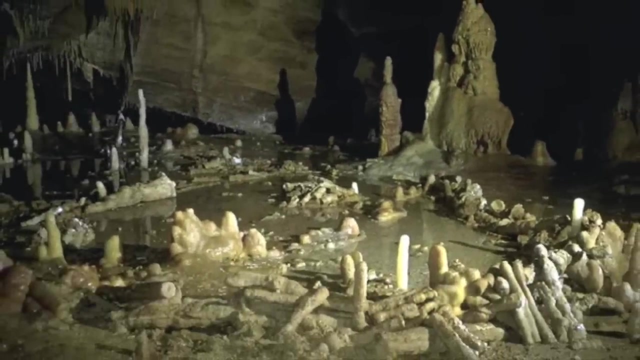 Such a structure had no practical use, perhaps a mark of property or a careless doodle. A far stranger's site was discovered within the French cave of Brunequel. Three hundred meters or thousand feet down, a bizarre arrangement of stalagmites was found, Over four hundred of. 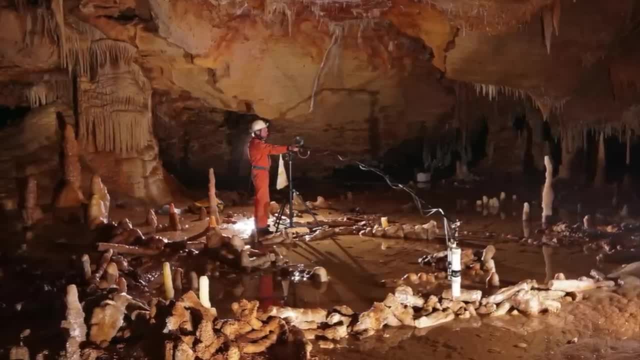 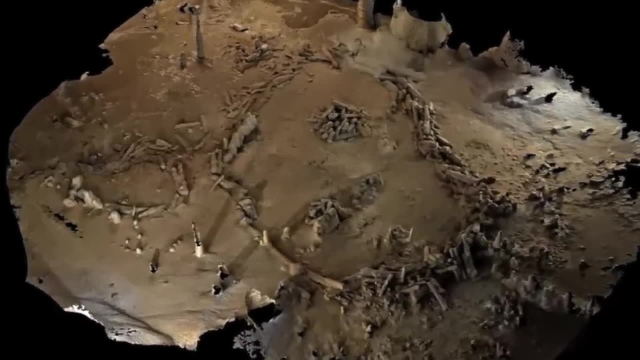 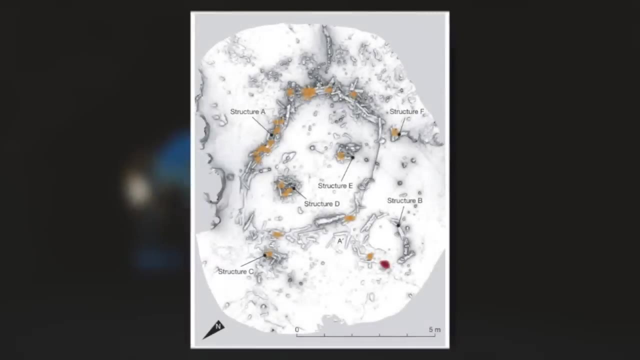 these stalagmites were broken off and placed into two main rings. The larger ring has a diameter of about five meters or sixteen feet. Two piles of stalagmites made by four distinct layers sit within the larger circle. Evidence of fire was found on multiple points of the structure. 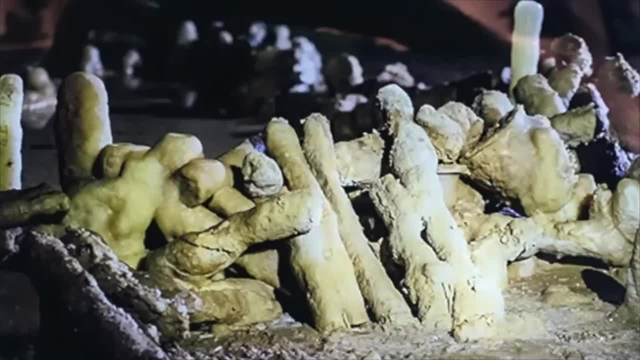 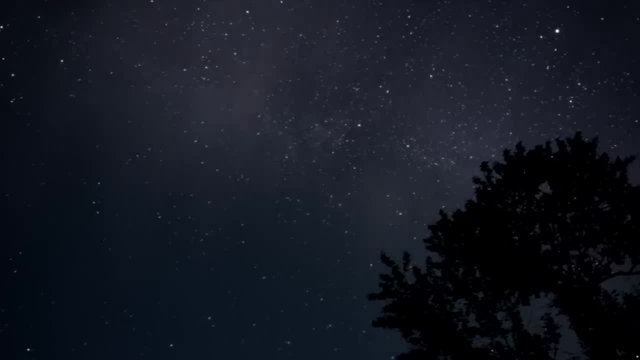 Around a quarter of the stalagmites were burned. The floor of the cave is covered in stone, but beneath it are other hearths. It seems that the site may have been visited repeatedly for at least hundreds of years. The total weight of the stalagmites moved is over two tons. 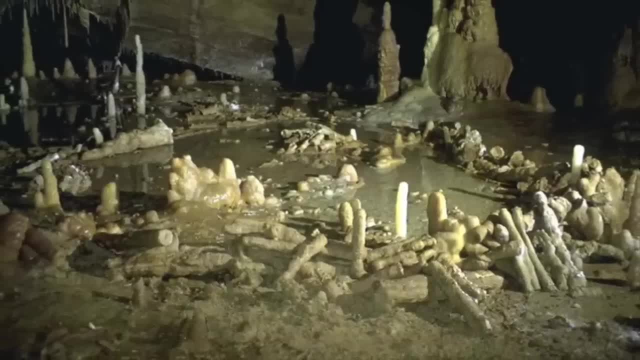 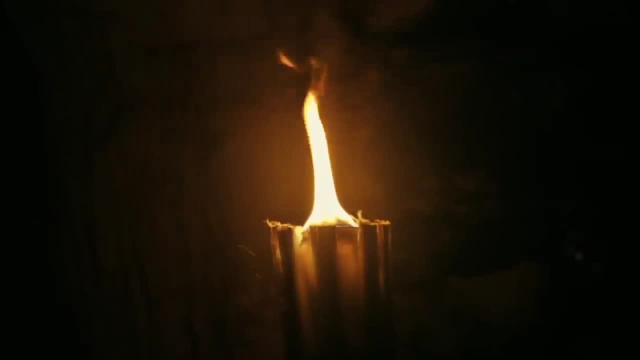 It would have taken hours to build, likely over multiple sessions. Artificial light would have been needed to see perhaps a torch or possibly the fires on the structure. When looking at the bigger picture of the site, it appears that it was some kind of ritual or sacred cave. 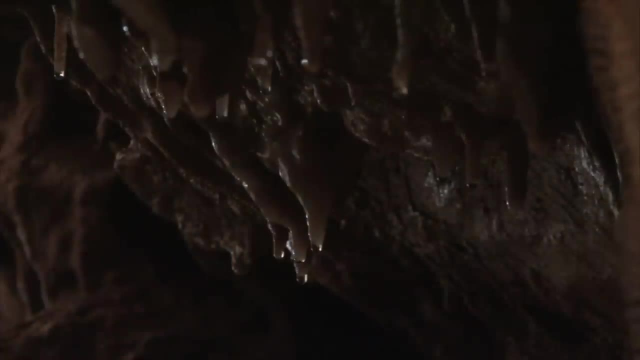 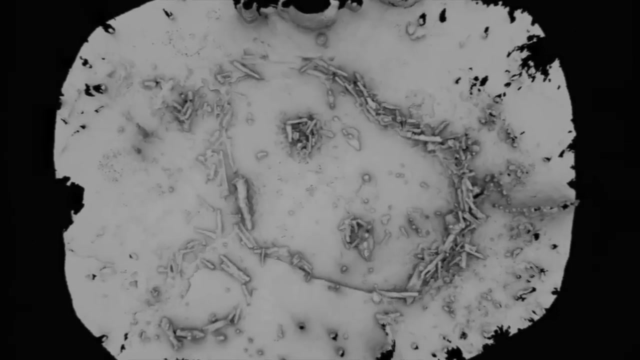 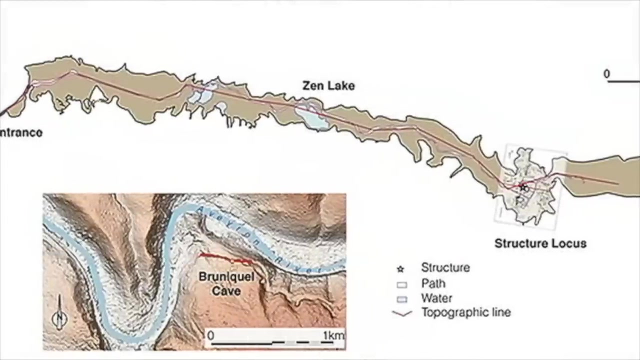 A group of Neanderthals spent hours deep underground, choking on smoke, working on a seamlessly pointless structure. Some have claimed that it may have been a sort of shelter. Perhaps the stalagmites were used to anchor a tent of some sort. However, the structure was so deep underground that it would have been impractical to live in. 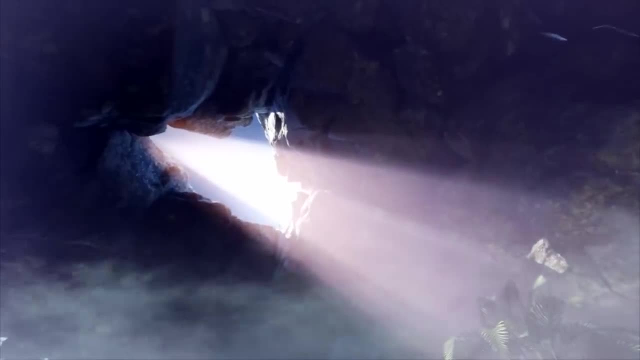 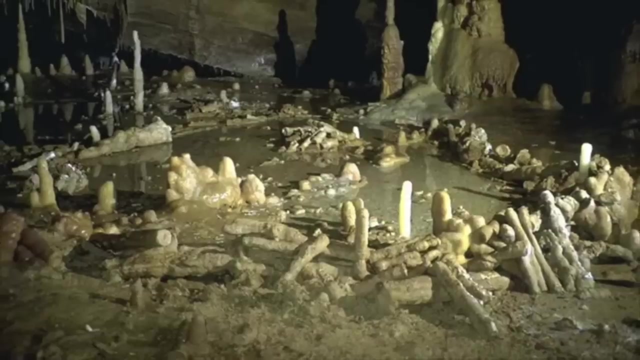 Starting a fire for cooking or warmth would have choked the inhabitants with smoke. Fires were also had within the structure and on the walls. This contradicts the idea that the stalagmites supported some kind of tent or pole. Furthermore, there is no lithic or 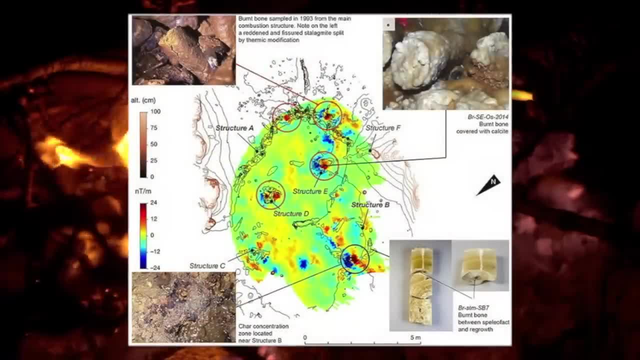 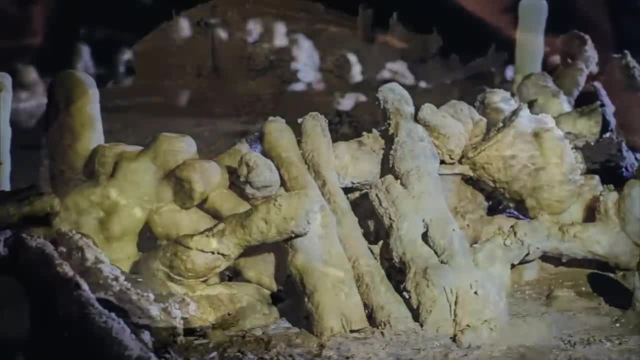 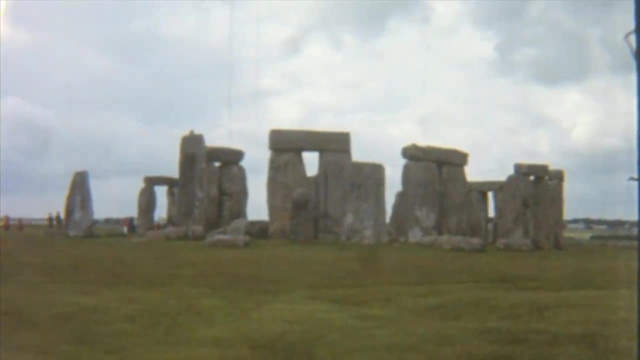 butchery waste. There are some bones, but they could have been fuel for a fire just as much as a snack. The structure is dated to 174,000 years ago and is the only monumental stone structure ever made by the Neanderthals. Modern humans around the world made large megalithic structures. 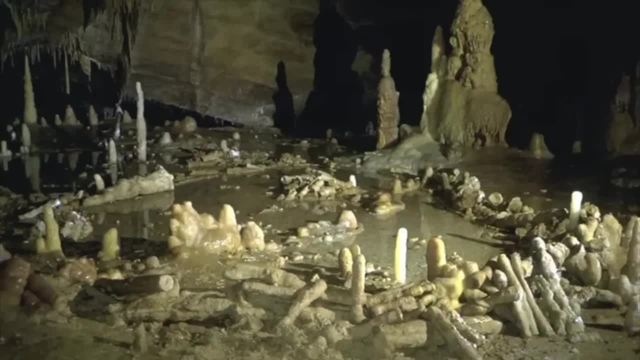 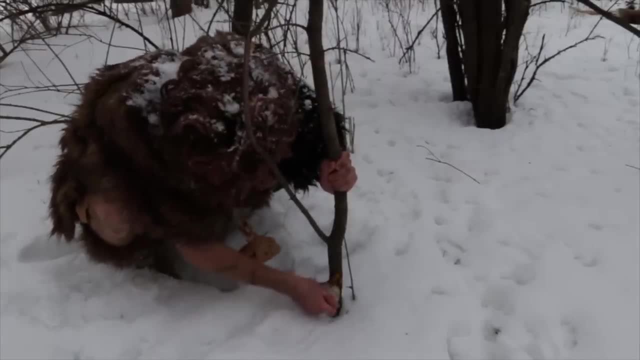 often for spiritual reasons, and Bernuquell may be the Neanderthals' take on the same pulses. Though it is easy to think of Neanderthals as busy hunter-gatherers with little time to think abstractly, the reality is that they were human and had complicated emotions and ideas. 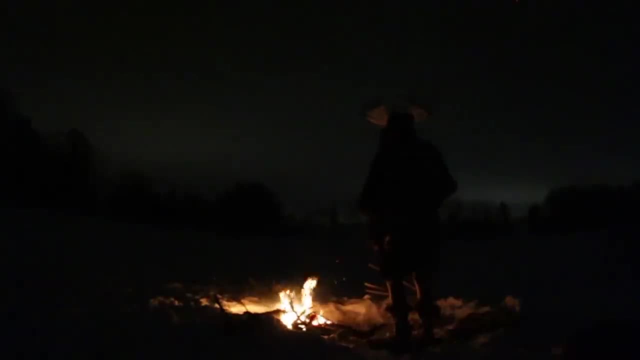 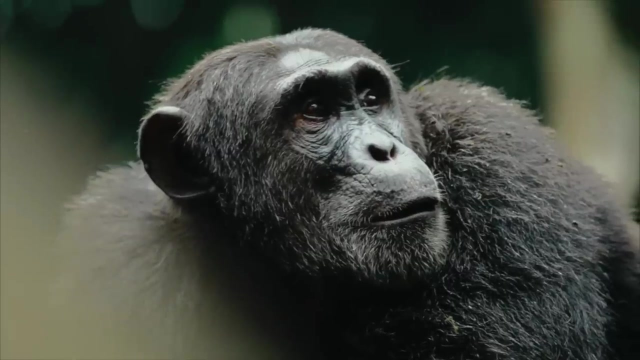 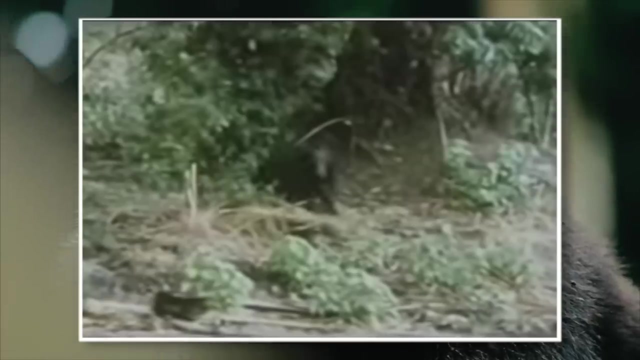 Attaching words such as religion or spiritual to Neanderthals can be contentious. Even doing so to early modern humans is a tricky affair. But there are even examples of chimpanzees' symbolic or ritual behavior, such as so-called sacred trees, or reacting strangely in the face of 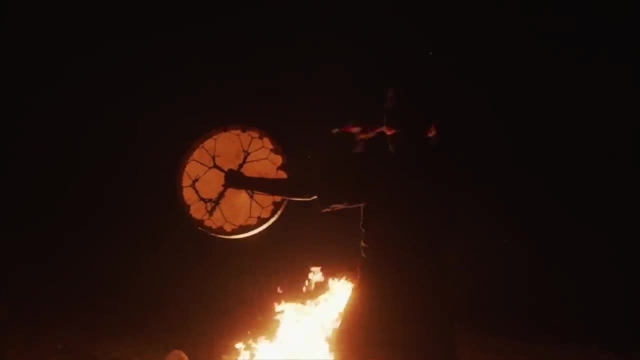 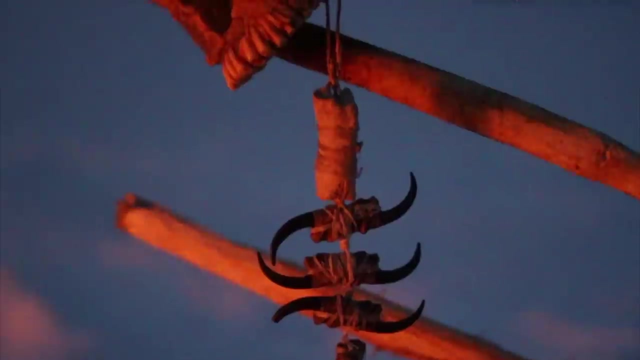 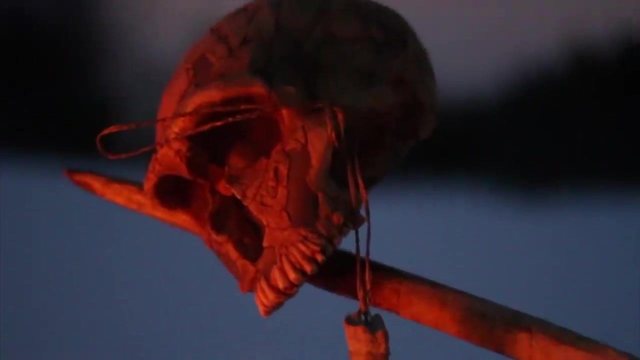 storms or wildfires. These behaviors may be the most primitive predecessors to our modern religions and rituals. Though we cannot pin down any classification of shamanism or animism, we can imagine that they would have had similar impulses to act based on existential thoughts. 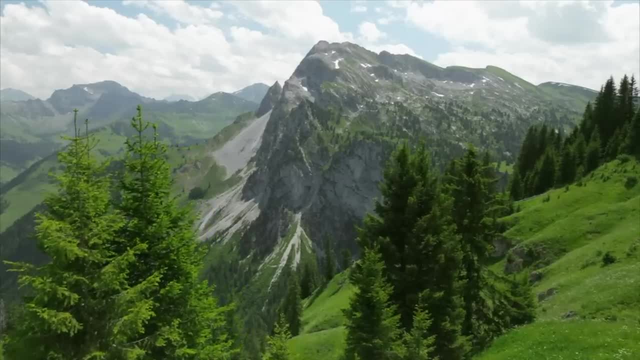 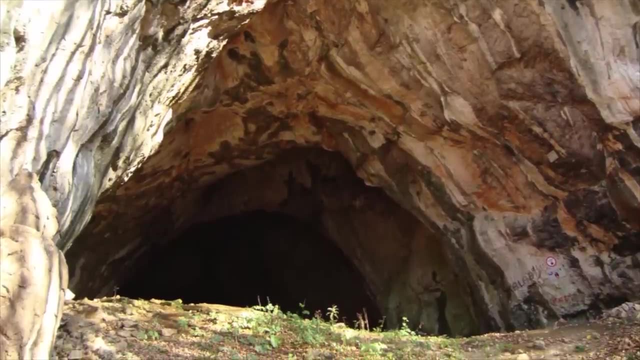 In the early 1900s, the cave of Dreckenloch in Switzerland was excavated. The cave was full of bare bones, which was not very surprising considering it was used as a den, But the bones appeared to be arranged in very strange ways. 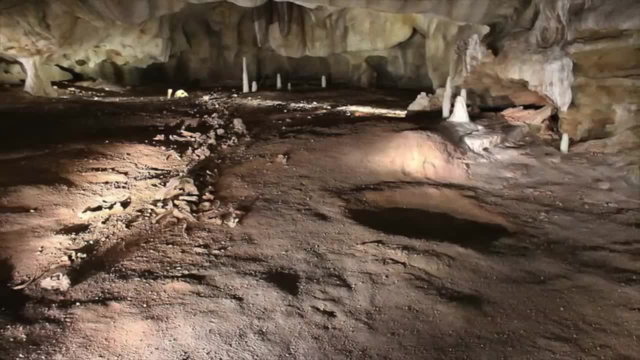 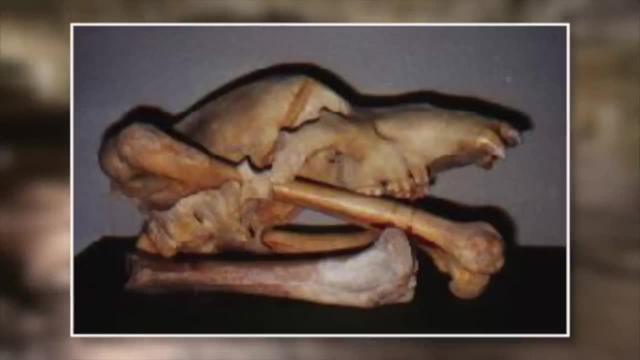 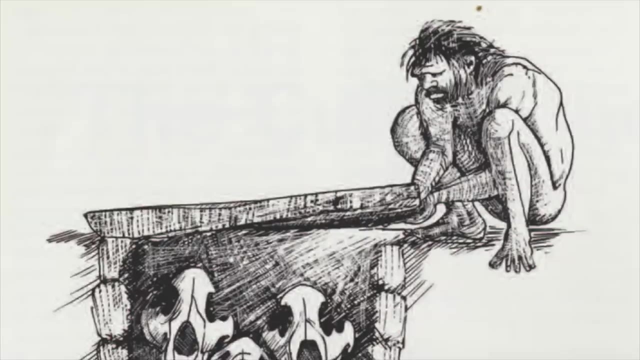 Low stone walls next to the cave walls seemed to hold back bare long bones and complete skulls. One skull even had a shin bone stuck between its cheekbone. Elsewhere in the cave, six chests or boxes made of sandstone contained bare bones. One contained bare skulls and was 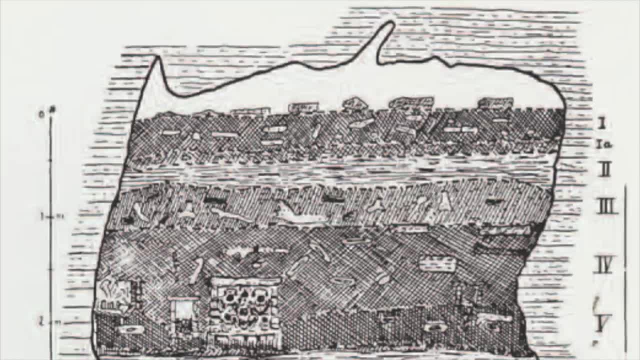 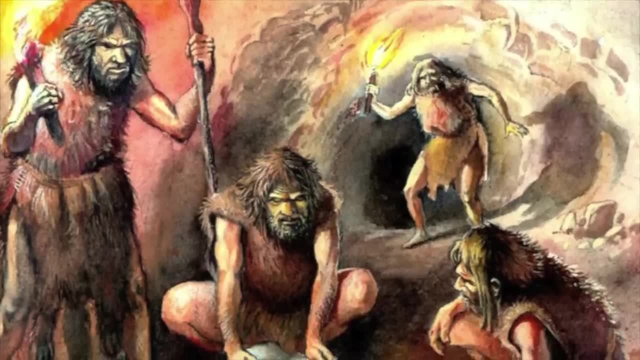 covered with a limestone slab. Workmen then reportedly dismantled much of the site before it could be photographed. The cave walls were covered with bare bones and complete skulls. The cave walls were thoroughly excavated and only sketches remained. The discovery and rumors associated with the cave immediately caused speculation that it 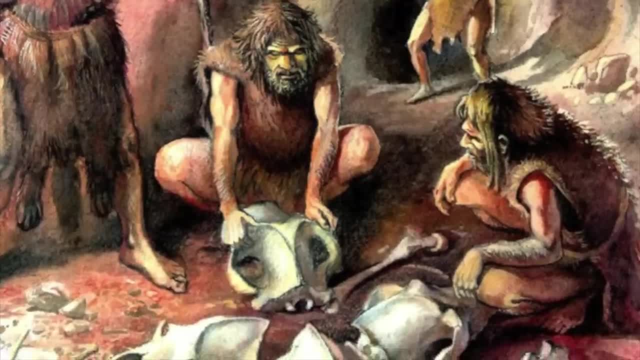 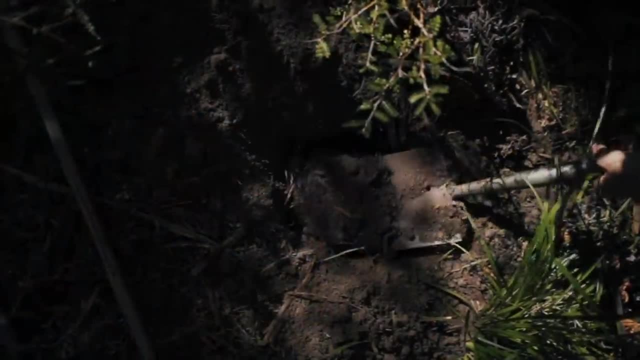 was used as a ritual center for some sort of cave bear cult. The romantic idea quickly caught on, though some were still skeptical. The cave was excavated hastily by workmen who were only supervised by archaeologist Emil Bacler for part of the time. 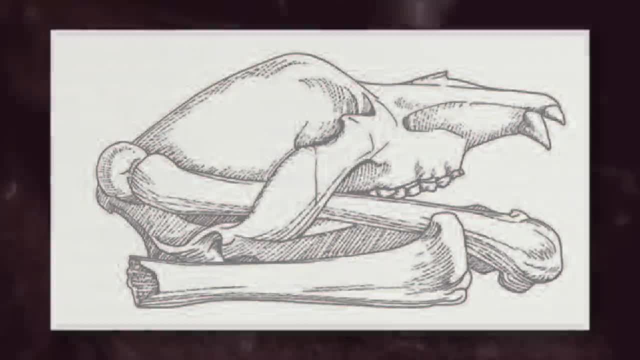 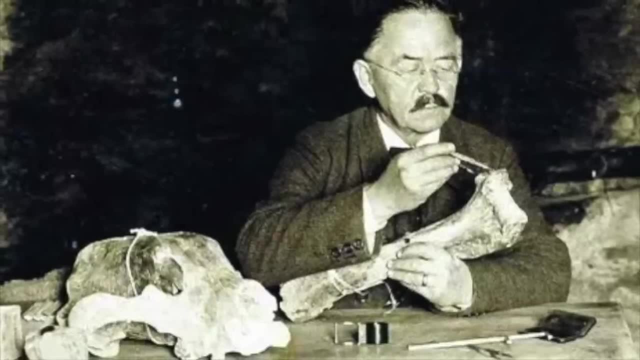 They discovered the skull with the long bone through it and some of the chests, without any professional presence. There was no clear reason for the cave's existence. The cave was also not present. No photos of the chests were taken and our only evidence comes from what Backler says. 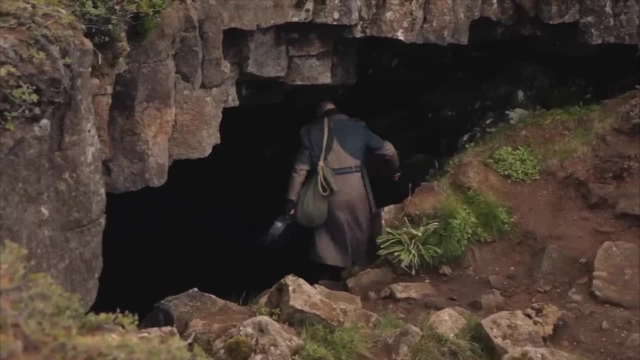 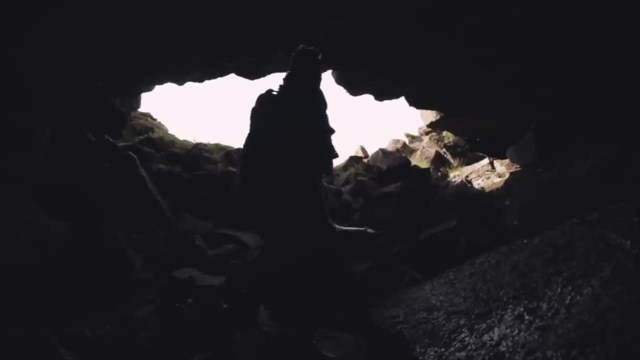 he found. The men who saw these chests in their resting state do not even agree what they saw and as time went by their accounts changed. Field notes from one man say that the structures may not even be man-made and may just be accumulations. 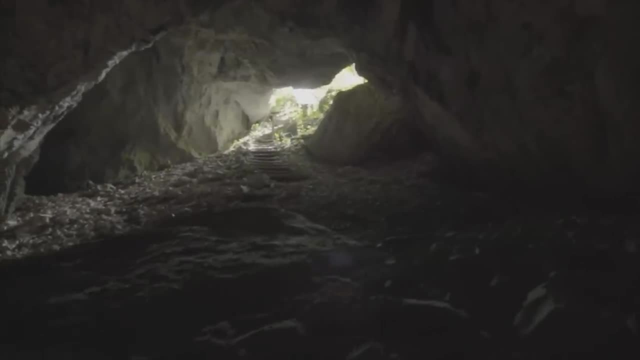 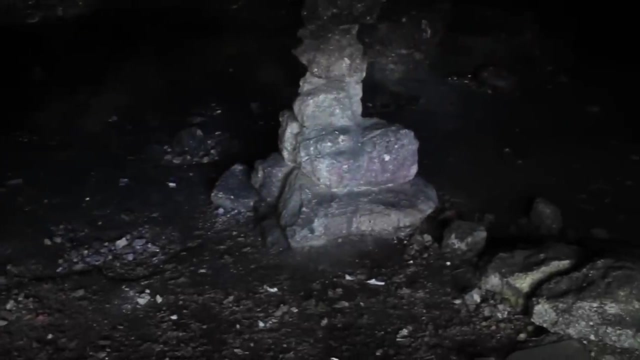 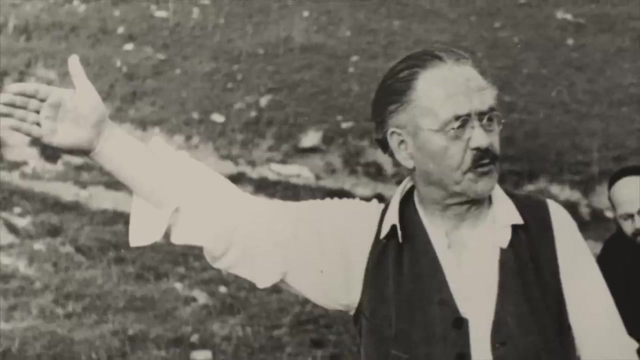 of fallen rocks. He also made no mention of stone chests, but rather cavities in the floor with bones covered up by limestone slabs. Such an accumulation could certainly be the work of nature and not the hands of a cultist. Backler's account is undeniably flawed. 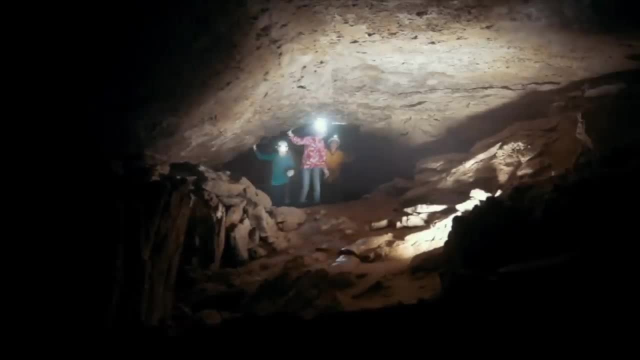 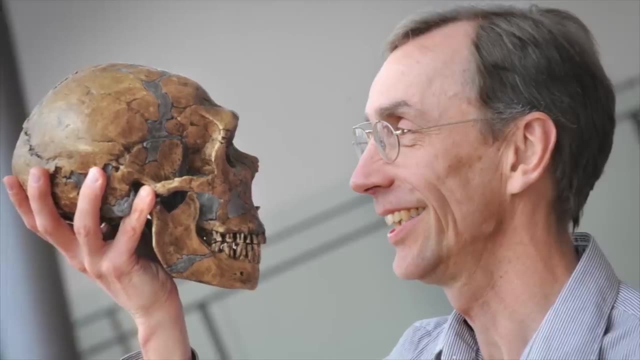 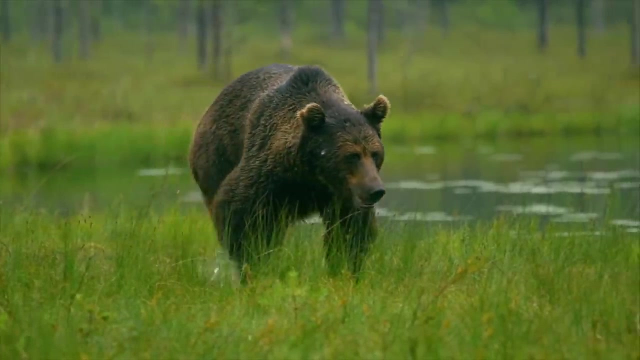 Unfortunately, we will never really know, because the site has been so badly damaged. This example is important because it displays the danger of placing our own preconceived notions on remains that we may not fully understand. Neanderthals very well may have had various cults based on bears, birds, the seasons. 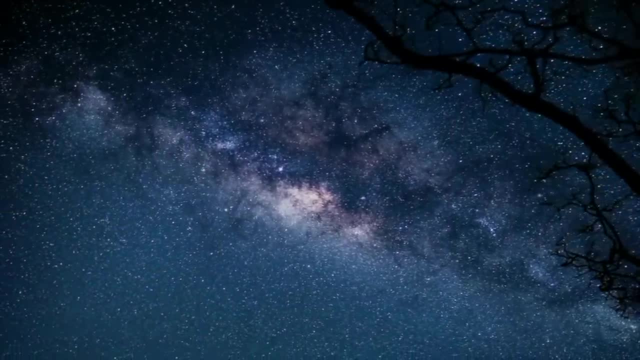 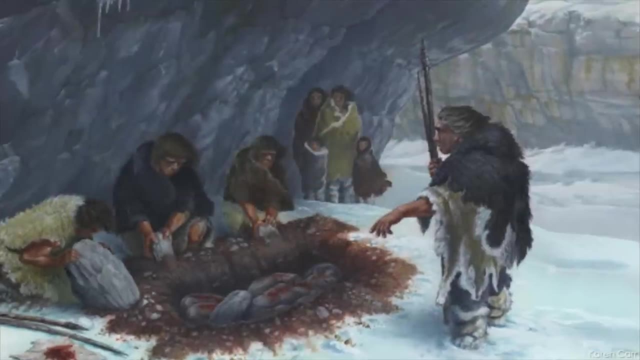 or even the stars, Though our evidence is far from conclusive. Perhaps the best evidence that they may have thought ritually or spiritually comes from the burial of their dead. Neanderthals did bury their dead. this much we can say for certain, though we do not know. 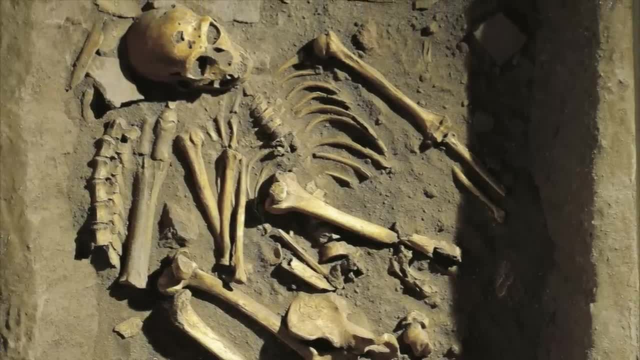 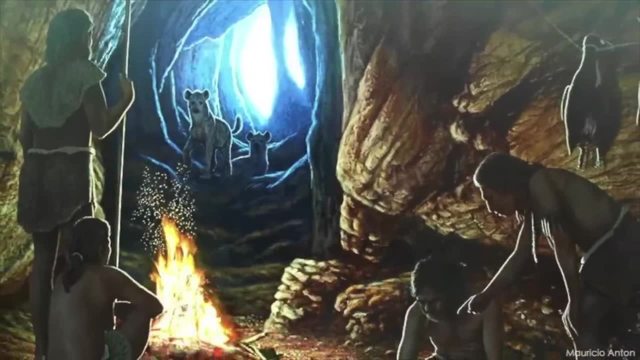 if their burials were symbolic funerals or just some form of predator prevention. From a practical standpoint, burying a dead member of your group prevents attracting dangerous animals. It can also prevent the spread of dangerous diseases and the spread of the virus. 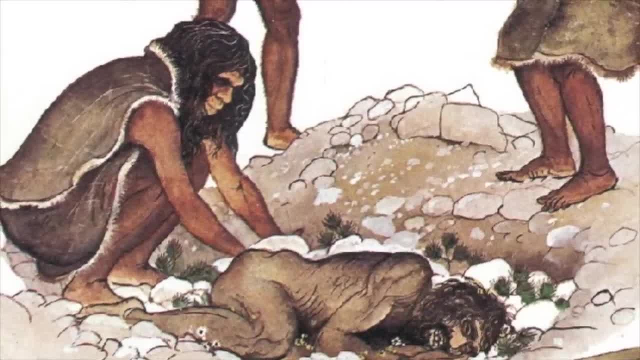 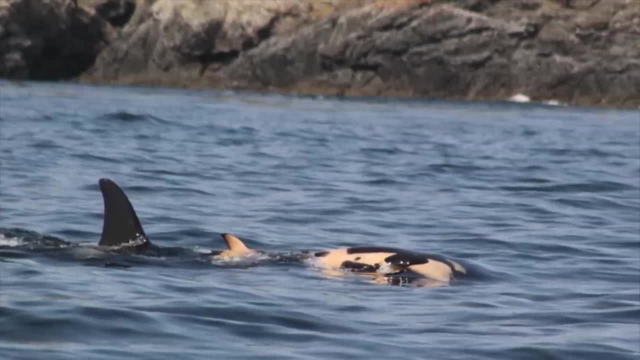 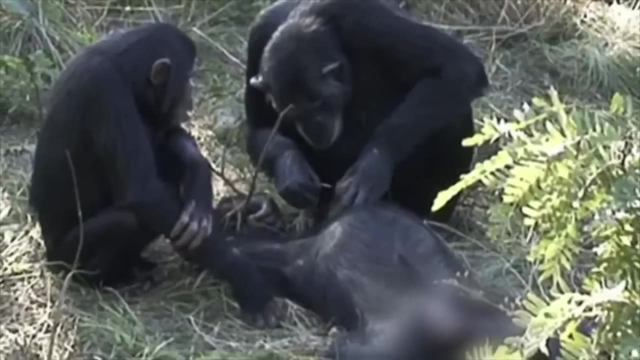 Neanderthals are the best example of this. or even just an unpleasant smell, though chimpanzees, elephants and even whales are known to display mourning behaviors. Chimpanzee mothers are known to carry around their deceased children, while in one case a chimpanzee used a grass tool to clean out the teeth of a dead friend. 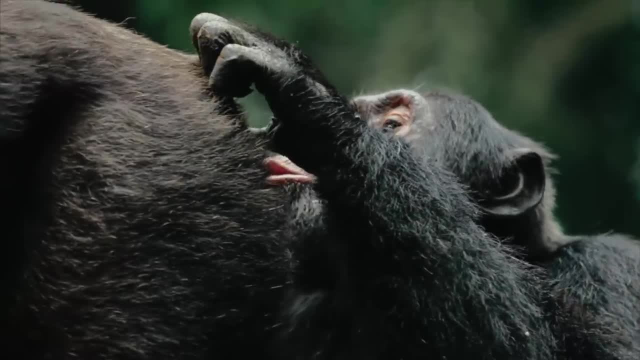 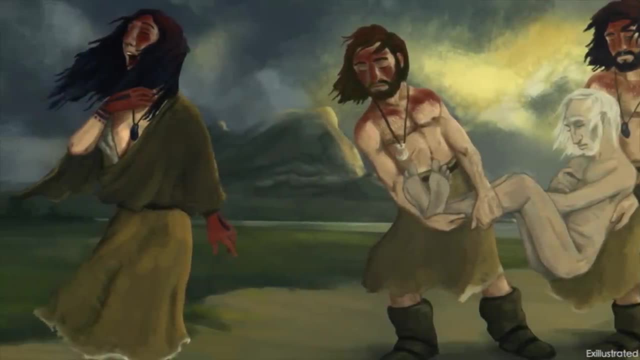 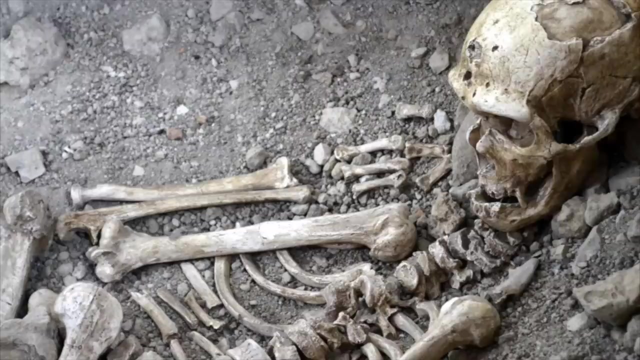 This would not necessarily classify as symbolic, but rather just a display of immense emotion. There is no doubt that a Neanderthal would have mourned the loss of a loved one, but we must look for further evidence of symbolism. The first evidence of possible deliberate burial by Neanderthals comes from an individual from 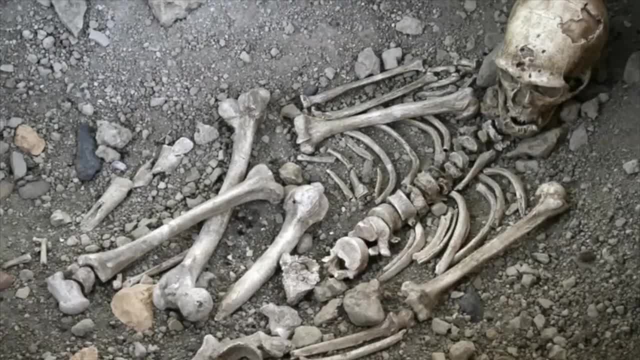 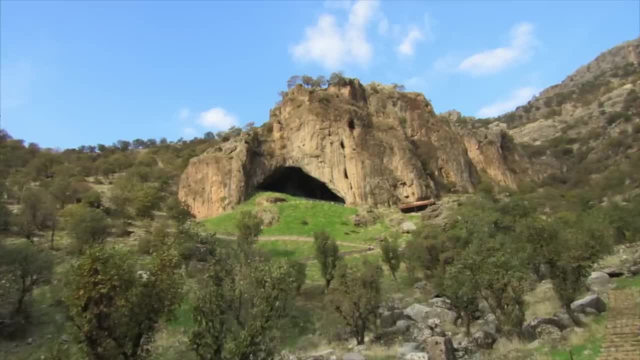 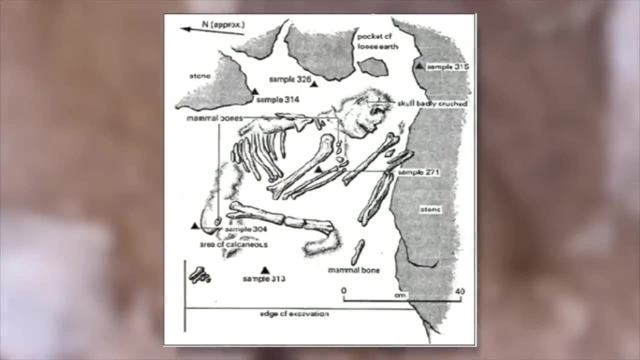 La Chapelle aux Sens, France. The remains seem to have been preserved in an artificial hole within the cave. Further evidence emerged from excavations in the 1950s and 60s. The cave yielded the remains of 10 Neanderthals, including one dubbed Shannondar IV, which was found with clumps of pollen. 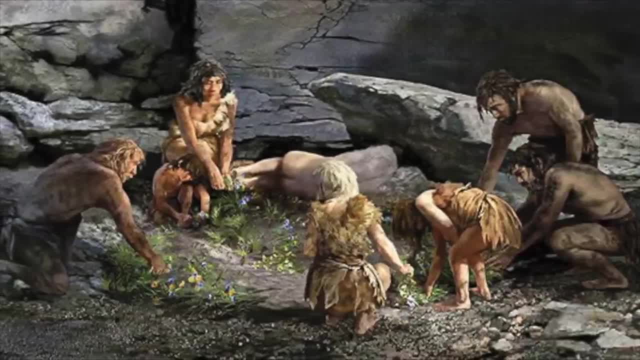 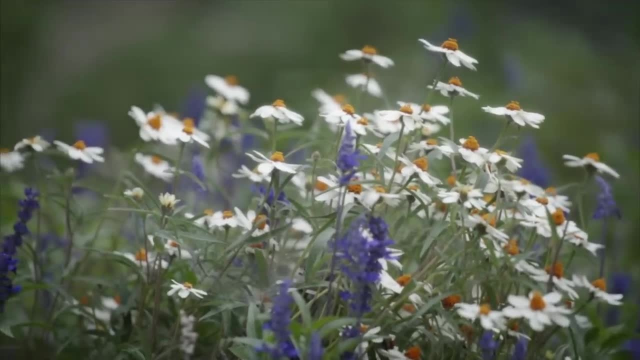 This suggested that the body had been deliberately placed in a grave and a variety of flowers were scattered on it. Interestingly, some of the flowers may have medicinal properties. This led some to believe that the individual may have been a shaman or a healer. 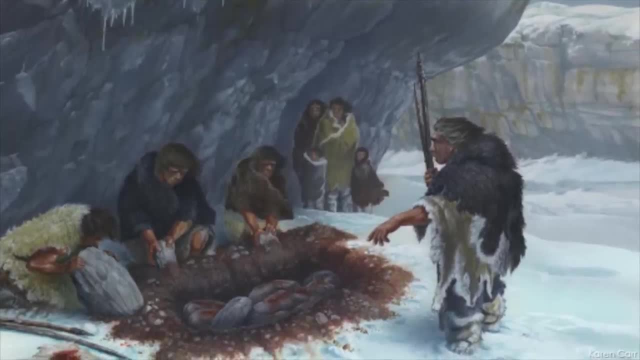 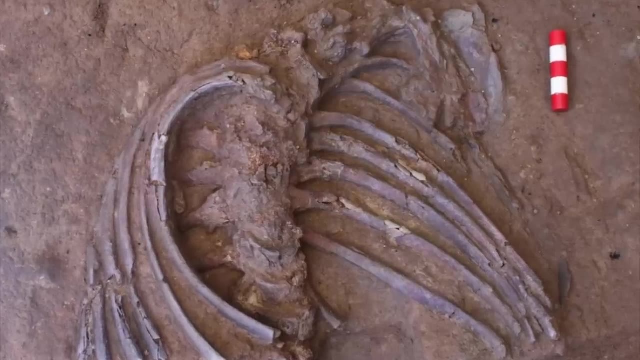 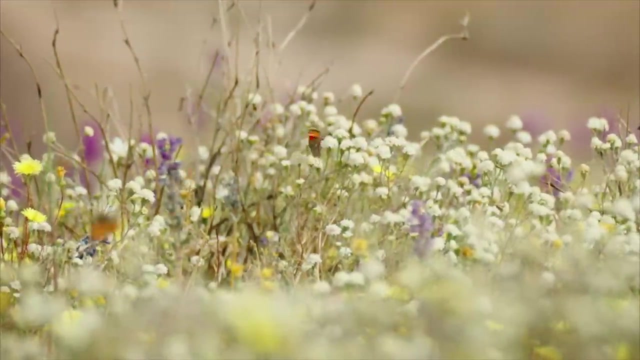 A finding was one of several lines of evidence that has led to a reassessment of Neanderthals as highly intelligent and social people. The idea of burial has been controversial, and the idea that flowers were placed on the graves seemed even more unlikely. Flowers may have just grown nearby or been blown in with sediments. 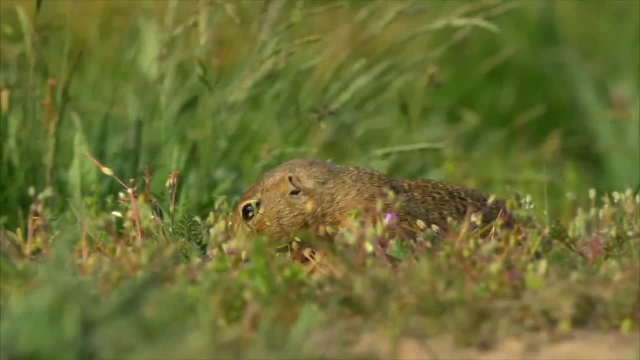 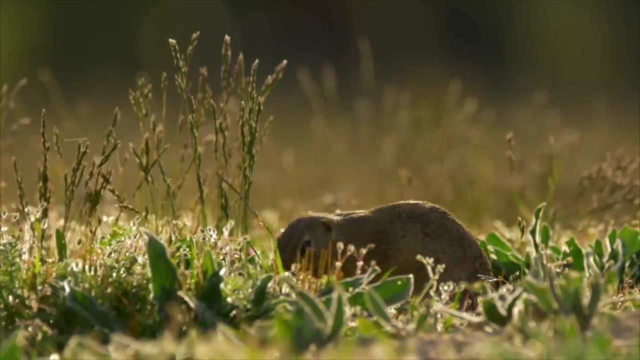 and some rodents are known to deposit various plants in caves. Deliberate placement of flowers remains a possibility, though rodent remains within the deposit are a more likely explanation. Reexamination of the site discovered another Neanderthal individual right next to the famous 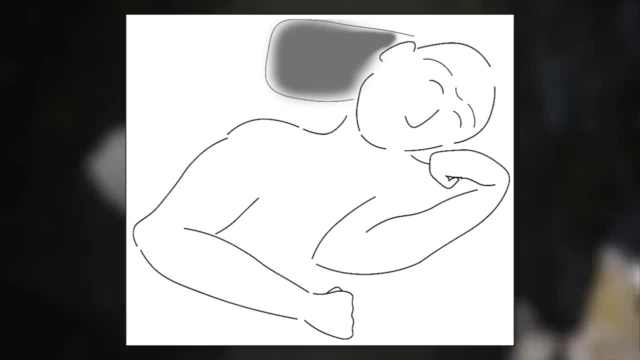 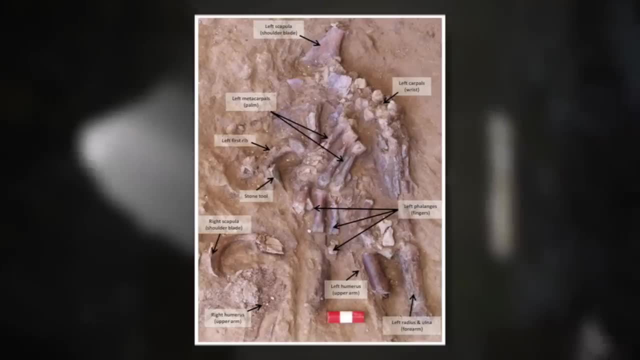 flower burial. These new remains show the upper half of a Neanderthal in an anatomical position. But what are the outside conditions to do to kill neanderthals? Mere data, Multiple lines of evidence, indicate that the Neanderthal was deliberately buried, including 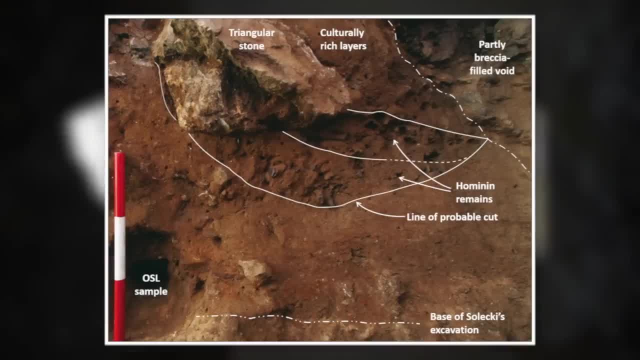 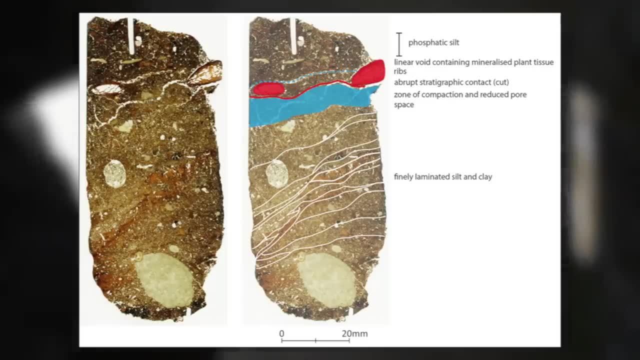 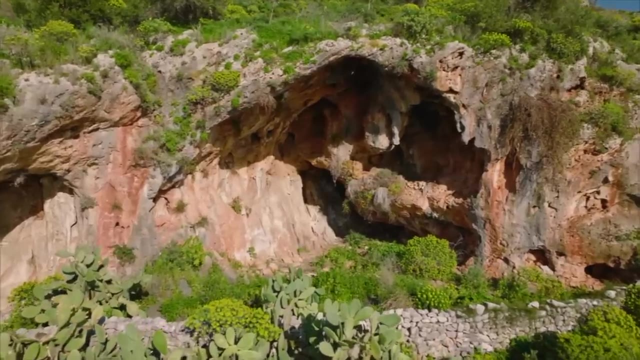 the fact that the sediment layer around the body is visibly different from the layer below, Evidence of digging and replacement within the sediment is strong evidence for burial. A variety of other Neanderthal sites preserve evidence of burial, though it can sometimes be hard to rule out cave-ins or rockfalls. 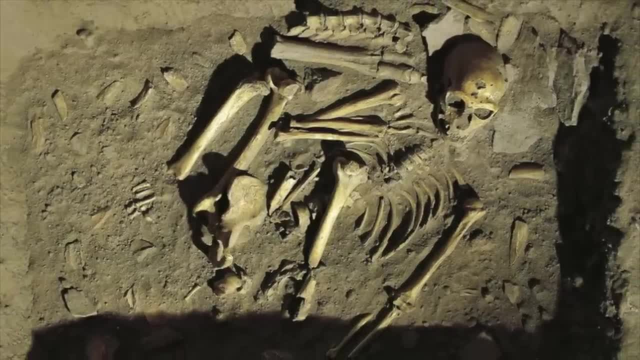 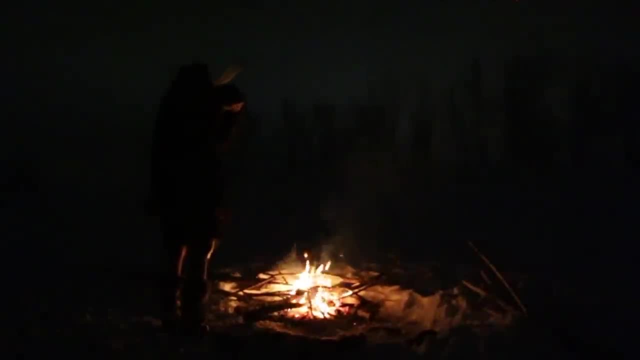 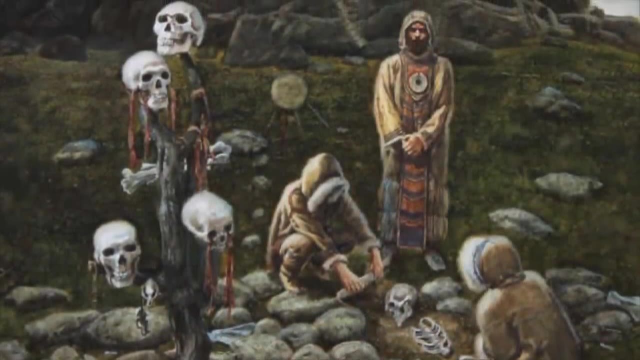 Actual, deliberate Neanderthal burials typically consist of shallow graves and sometimes include lifegoods. Some sites, such as Shannondar Cave or La Farassee, may actually have been important mortuary centers for Neanderthals. Mortuary centers are known throughout many modern human cultures. 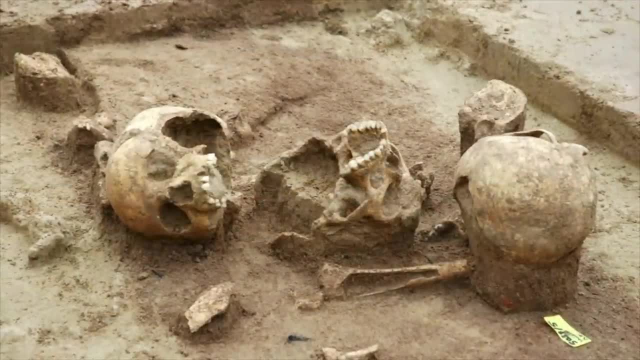 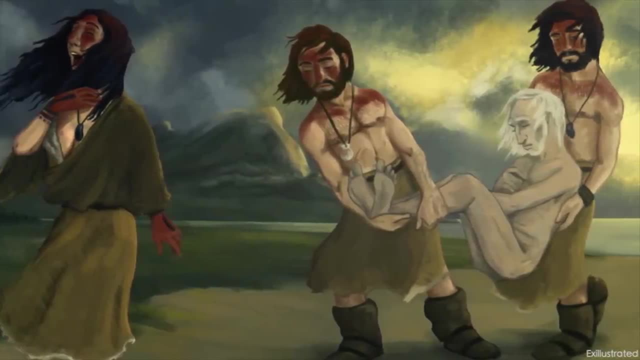 Neolithic Europeans would bring their dead from far and wide to the site of Herxeme. It is possible that Neanderthals would have made similar travels to these sites to put their loved ones to rest. Children and infants in particular seem to have been buried with great respect. 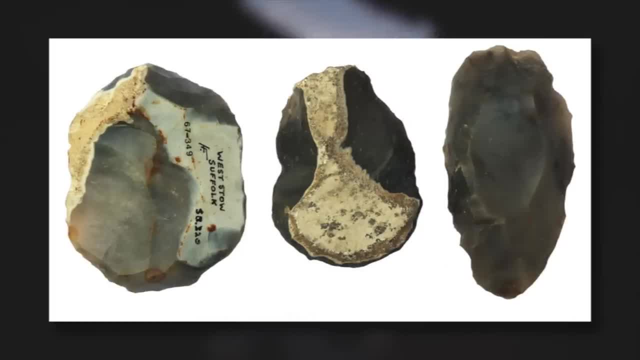 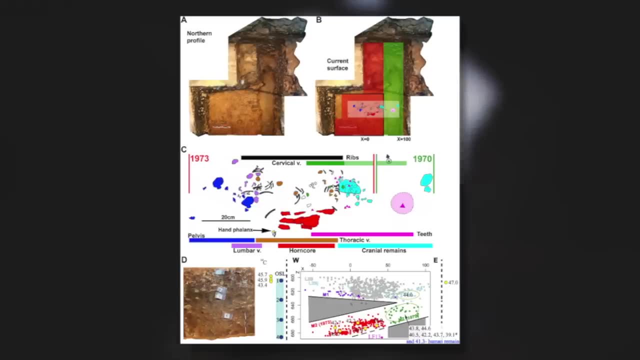 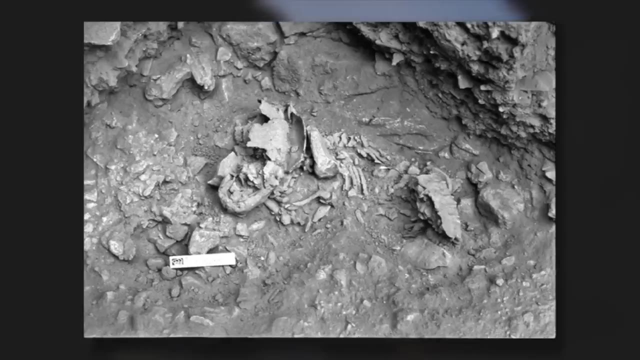 An infant from La Farassee, France, had three flint scrapers buried with it. Its head was also left higher than the rest of the skeleton, perhaps indicating that Neanderthals deliberately piled sediment to raise the head At Emote Cave, Israel, a child is clearly associated with a red deer jaw, while the other 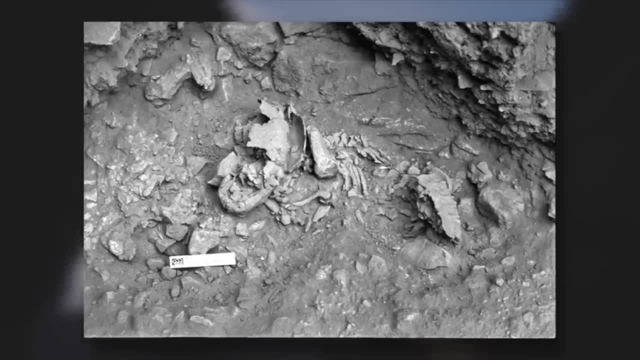 remains of this animal are absent or pulverized. At Dederiah Cave in Syria, two infants were buried. One of them was buried laying on its back with a stone slab next to it. The other was buried on its back with a stone slab next to it. 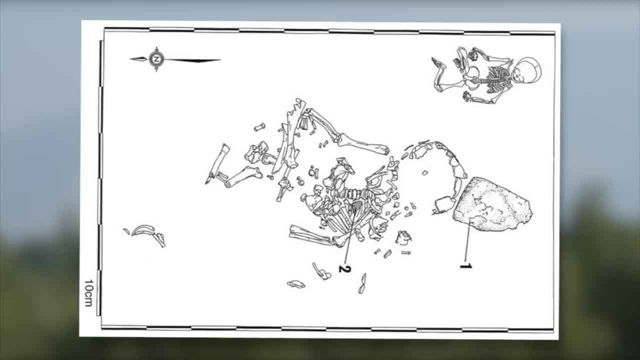 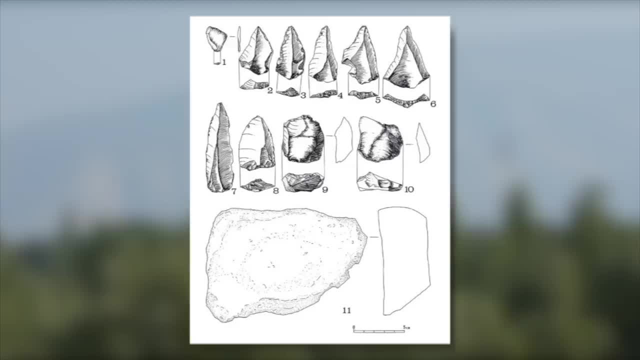 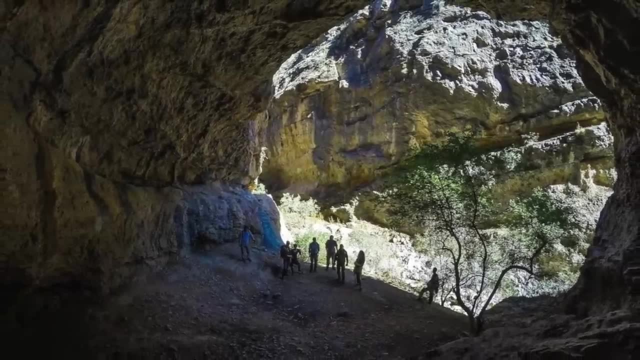 flint on its chest. The other was associated with faunal remains and over a hundred pieces of knapped stone. At the site of Tashik Tash in Uzbekistan, a child was placed in a circle of ibex horns with a slab of limestone to support its head. 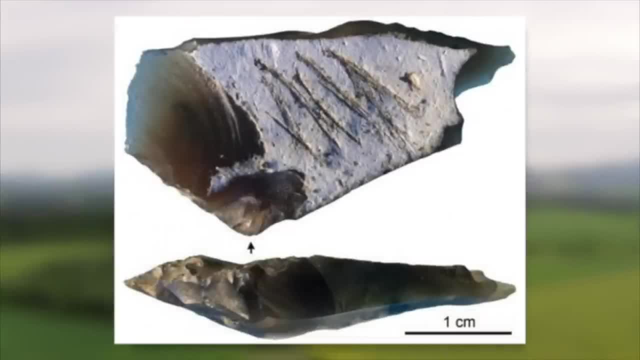 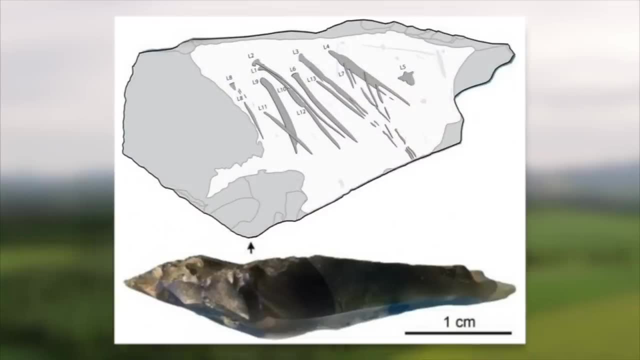 Finally, at the site of Kilkoba in Ukraine, a child was buried with a flint flake with etchings on it. This is the same flake that we talked about earlier. Considering that almost any parent would have been devastated by the loss of their child, 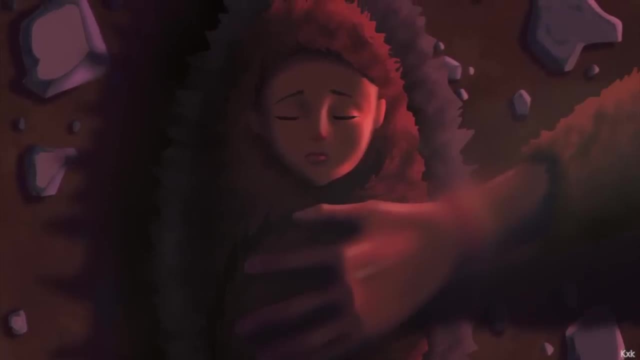 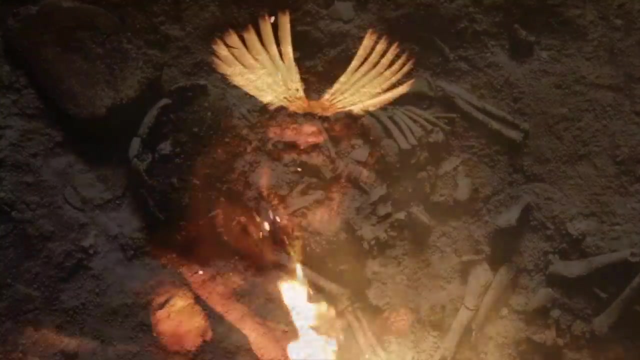 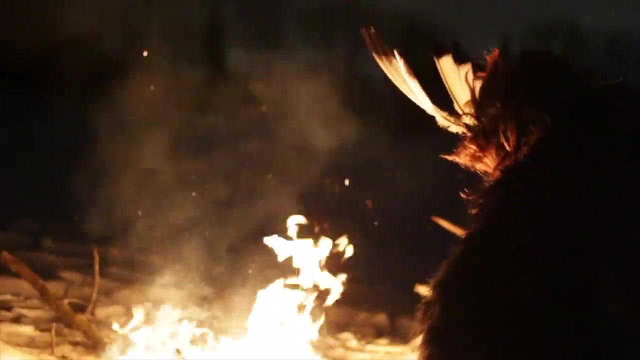 it makes sense that deceased infants were treated with so much respect. The association with grave goods at infant graves is indicative of a deeper symbolic meaning. There very well may have been a ritual being performed at these burials. Once again, we must be careful not to apply our modern ideas of spirituality or religion. 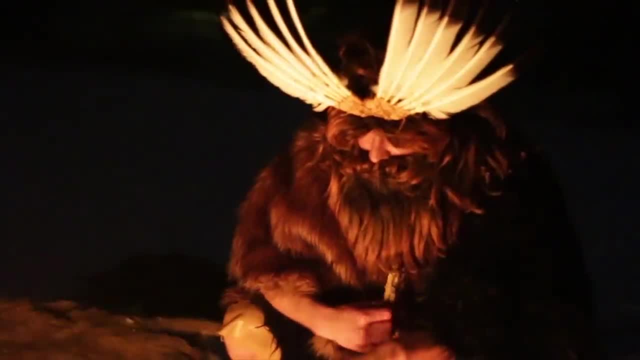 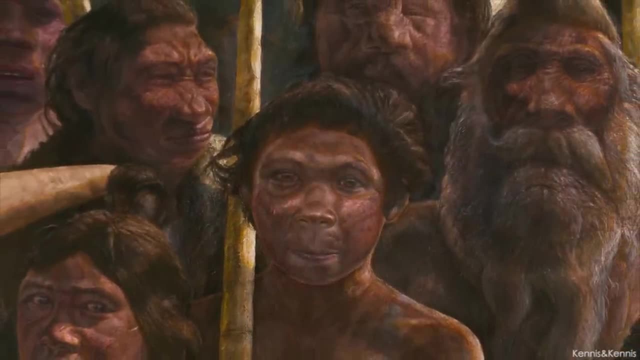 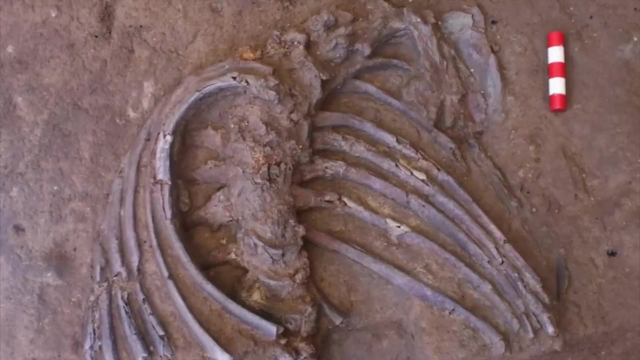 on these people, though at a human level we can relate to their feeling of loss. These people loved each other and even after death they had residual feelings that compelled them to bury their dead and sometimes leave them with valuable goods. When considering all of our evidence of Neanderthal burial, it does not appear to have been exceptionally. 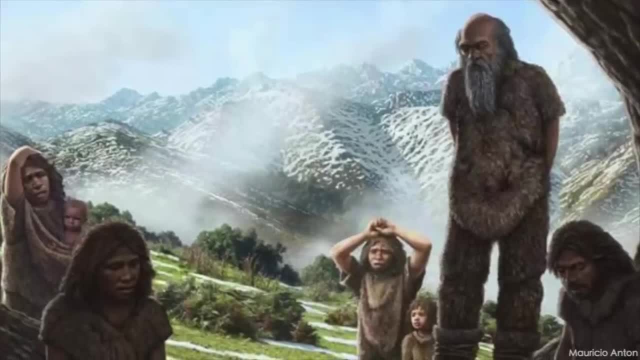 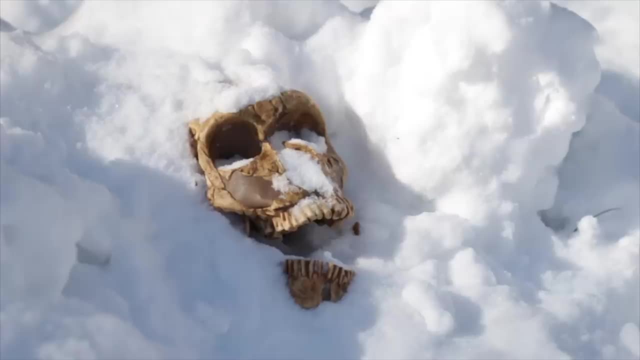 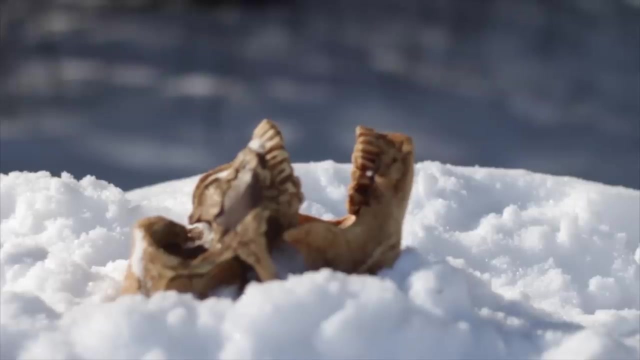 common. The oldest burials occurred 70,000 years ago and became more common as the years went by. This suggests that burials were a cultural tradition. Burials were a cultural invention that happened relatively recently in Neanderthal existence. This behavior may have increased in frequency and became more elaborate if more time was. 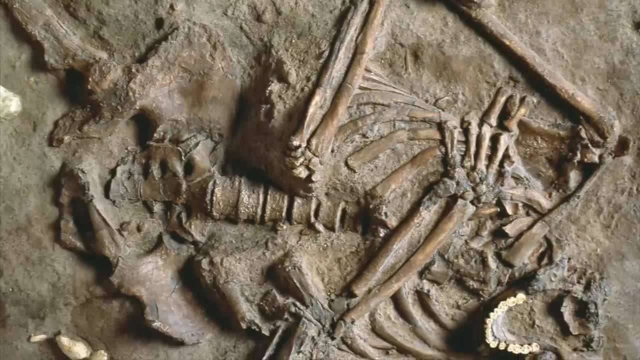 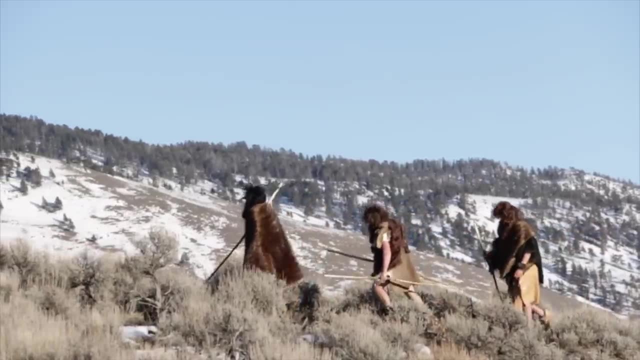 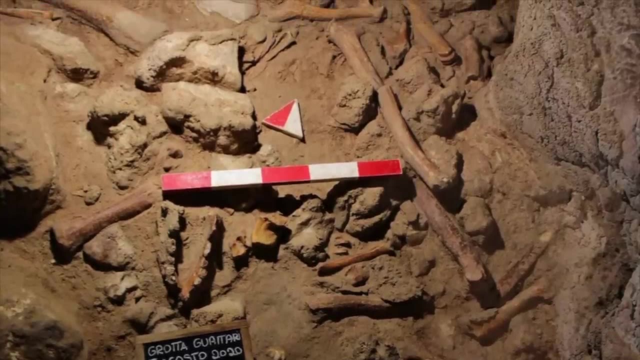 allowed. There have been over 400 individual Neanderthals discovered. This number may sound low because of the thousands of Neanderthals alive at any given time, but it is actually a lot. Fossilization is an extremely rare process and humans also have to find these fossils. One of the reasons that we have so many fossilized animals is because they are so rare. One of the reasons that we have so many fossilized animals is because they are so rare. One of the reasons that we have so many fossilized animals is because they are so rare. 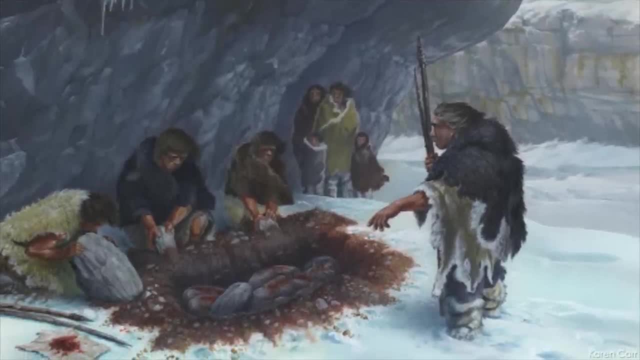 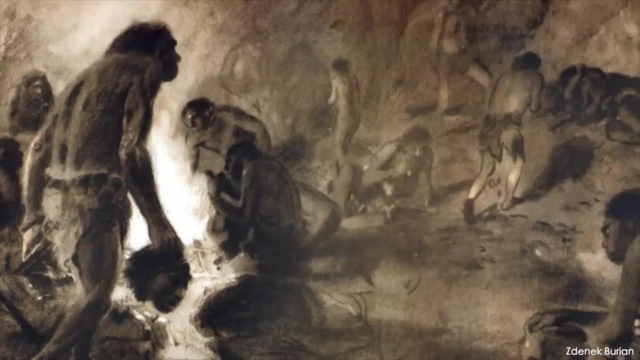 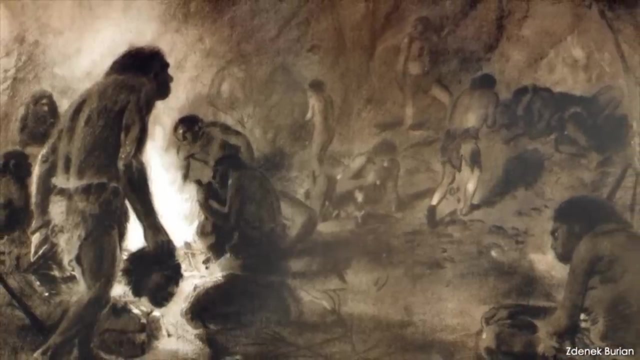 The fact that the fossils of Neanderthals is undoubtedly due to burial. Another kind of funeral we must take into account is ritual cannibalism. Though cannibalism is usually thought of as a predatory affair with an unwilling victim, this is only one kind of cannibalism. 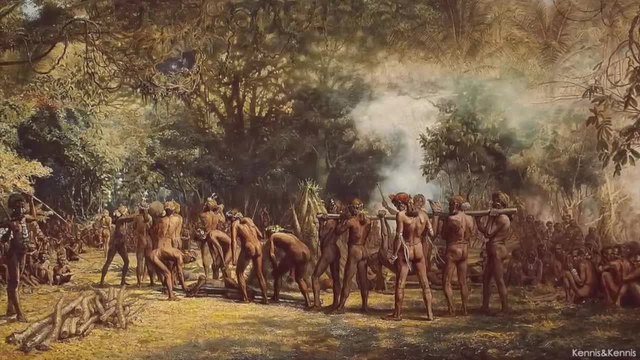 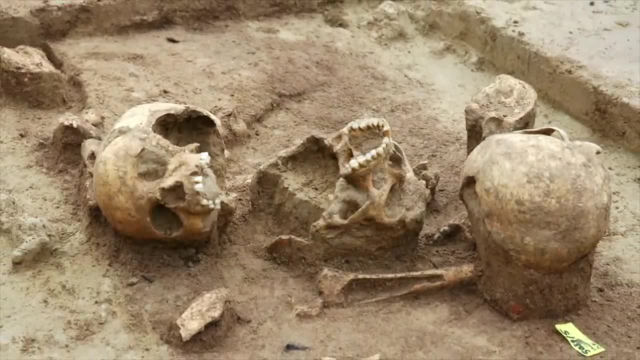 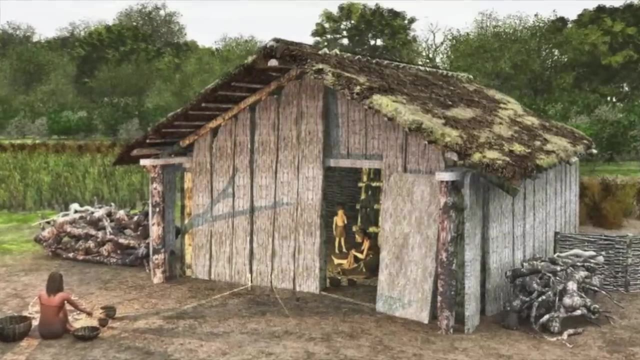 Mortuary. cannibalism was actually quite common throughout history and prehistory. At the aforementioned Neolithic site of Herxime, individuals were brought from far distances before being butchered. The ones doing the butchery were likely loved ones who brought the dead to the site as a 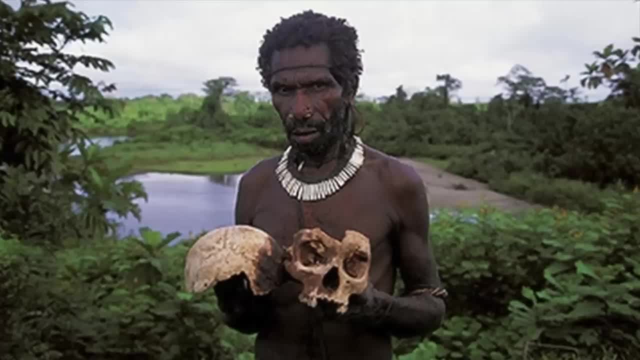 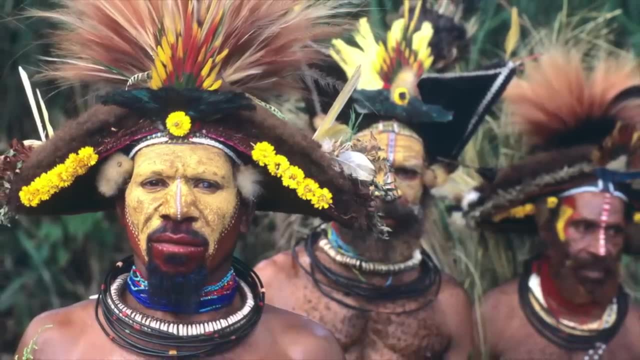 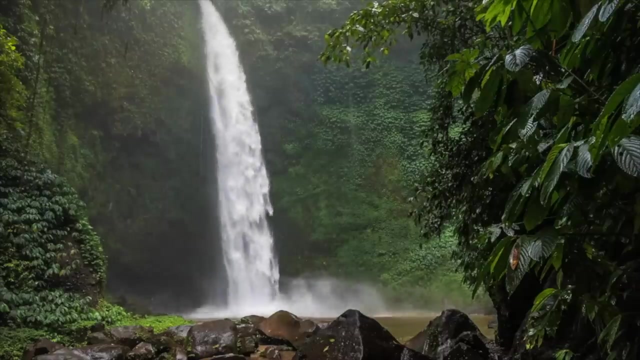 form of a funeral. Similar rituals have been seen in Papua New Guinea and Brazil. Communities of Papuans would commonly consume their deceased loved ones. The belief is that it is much better for the body to be eaten by their own people than by maggots or worms. 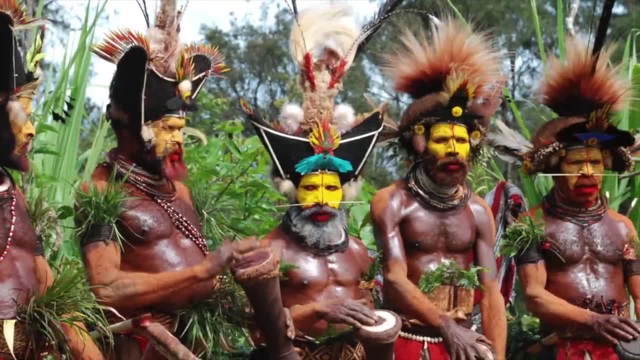 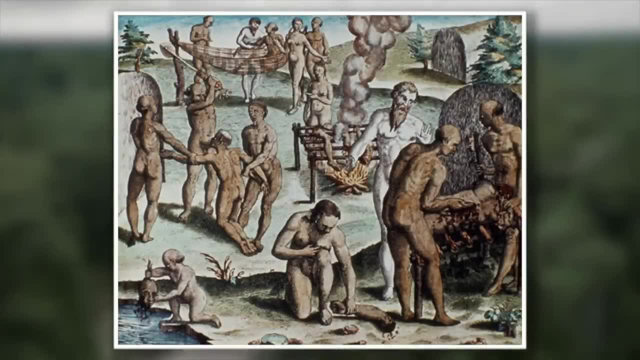 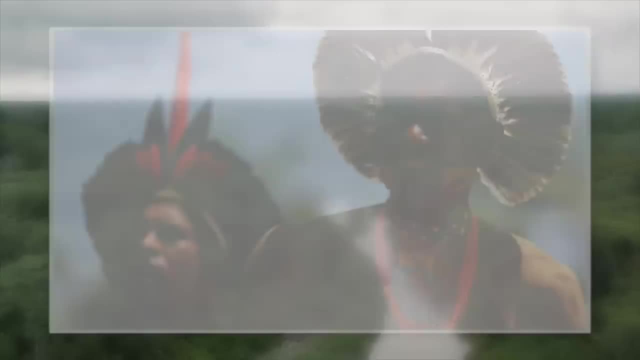 It has been reported that many Papuans would personally request this funeral before death. Another tribe in Brazil known as the Tubanamba practiced ritual cannibalism on the deceased. They believed that the soul lives on in the body of their relatives once consumed. 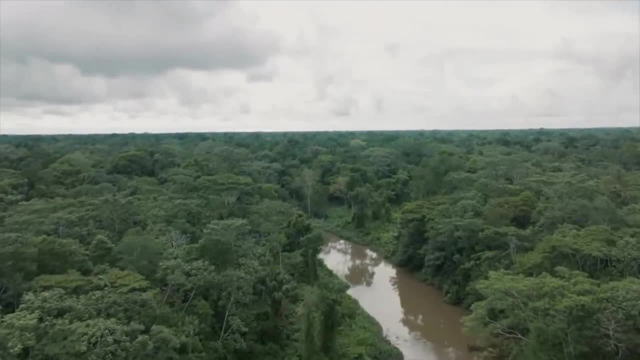 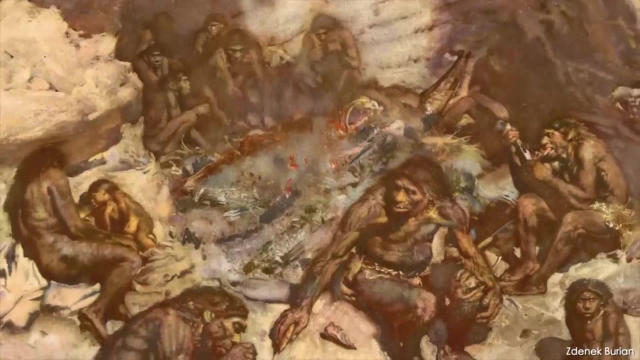 It was an essential practice to help their family relieve their grief. As you can see, cannibalism can actually be done out of great love and respect, and there is evidence that Neanderthals may have been engaging in a similar behavior At the Croatian site of Krapina, where the possible human body was found. the Neanderthals 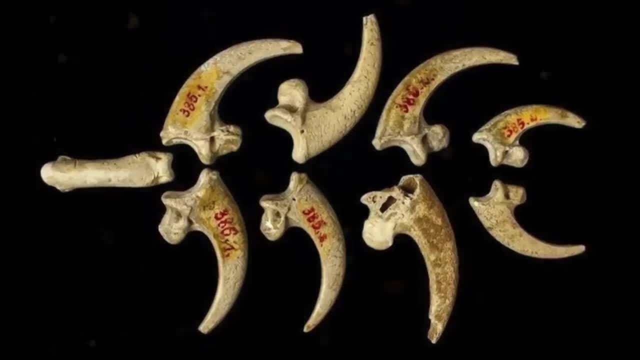 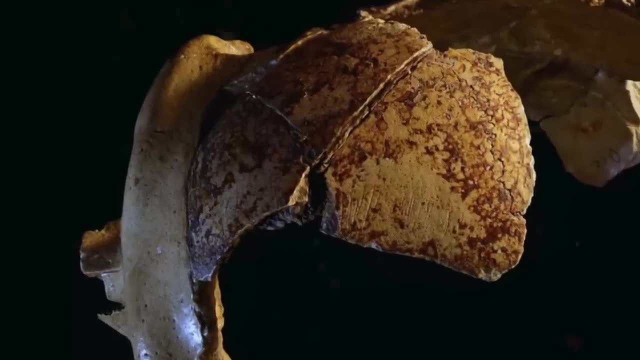 were also involved in the ritual. After the eagle talon necklace was found, another intriguing thing was discovered. A well-preserved Neanderthal's skull was found to have strange cut marks present on its forehead. At least 35 marks were made on the forehead of this individual, likely during the same. 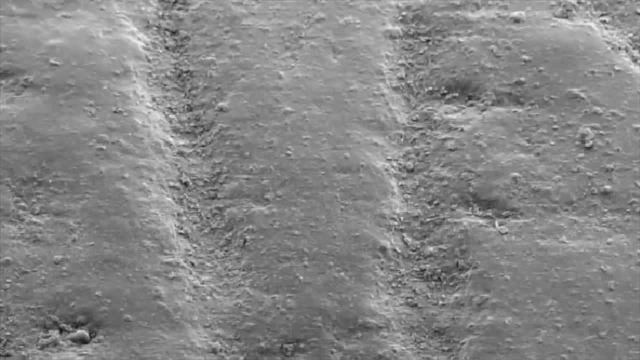 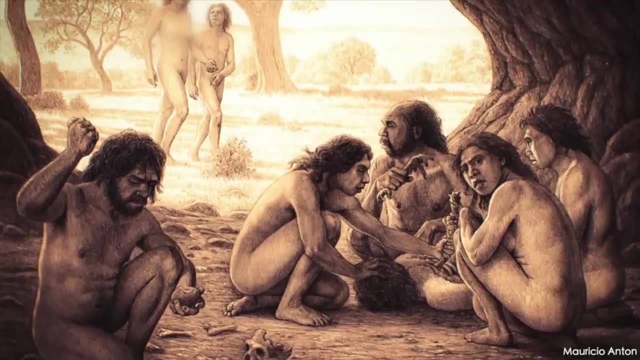 session. The cut marks are not consistent with butchery and are more likely associated with the symbolic perimortem manipulation of the dead. It is difficult to say what was actually done to this individual, though he wasn't simply scoffed down by a hunger. 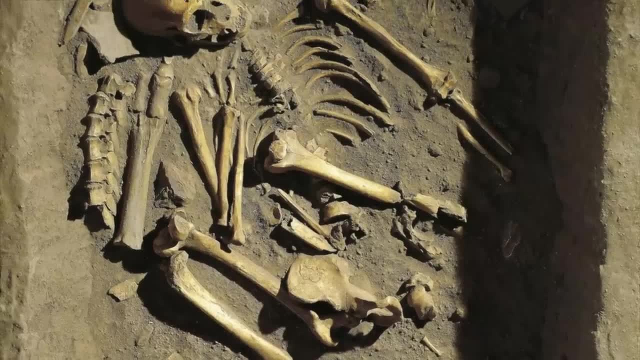 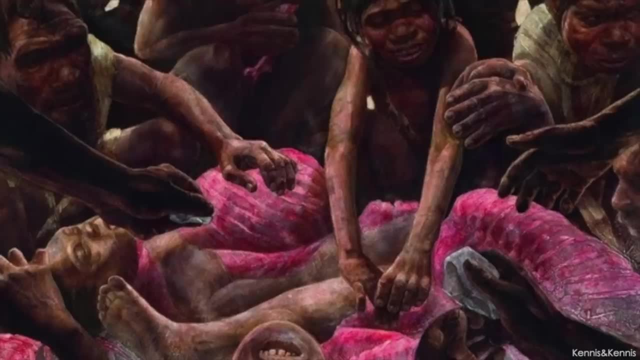 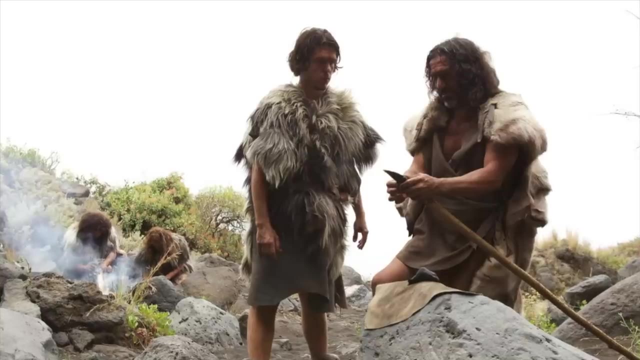 Neanderthals were treated differently in various Neanderthal populations. Some may have had many similarities with modern funerals, while others may have looked like a horror movie to us. Besides the way they treated their dead, we can also find hints of compassion in how they. 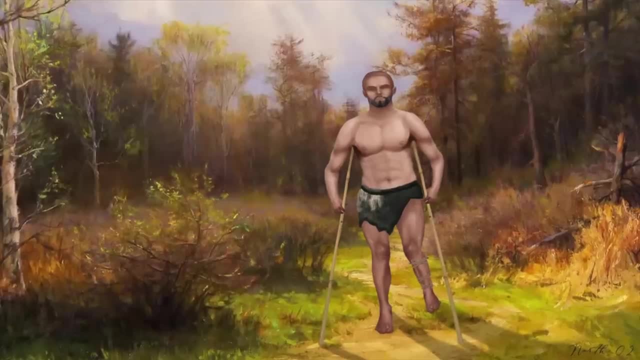 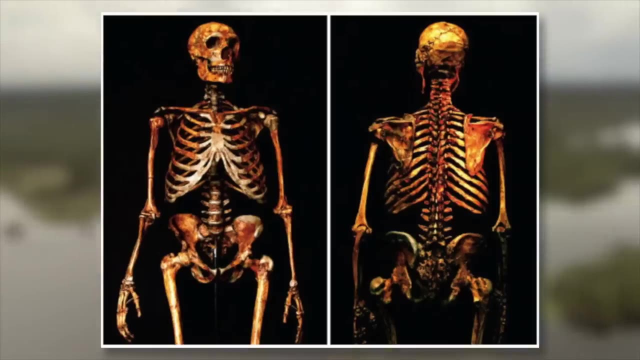 treated. the living Neanderthals lived very hard lives, and serious injuries were a common part of life. It is generally accepted that more than 80% of the skeletal remains known to be dead are remains known to archaeologists display several injuries. 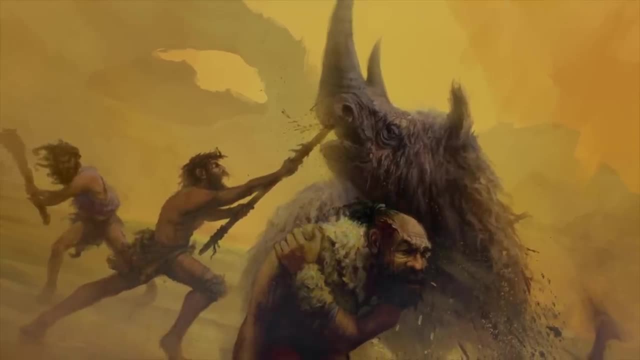 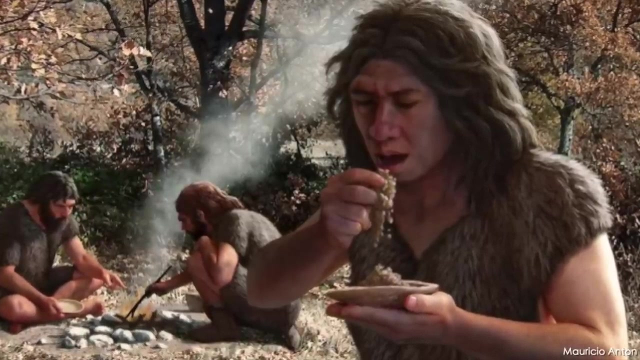 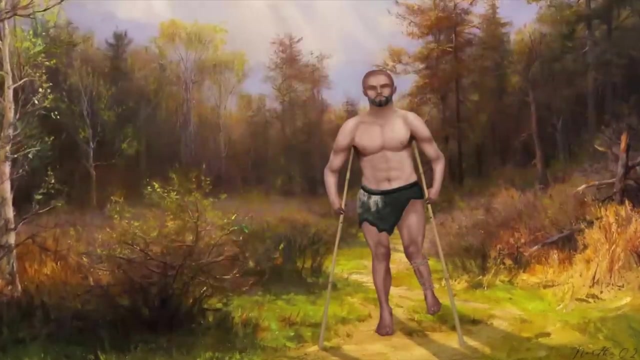 Most of these injuries were acquired during hunting or when traversing their often mountainous terrain. Despite so many injuries, many of them seem to have made impressive recoveries. Bone fractures often healed without significant deformities suggesting that they had been set with a splint of some sort. 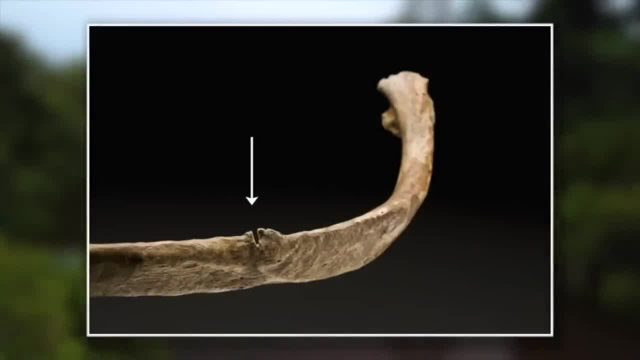 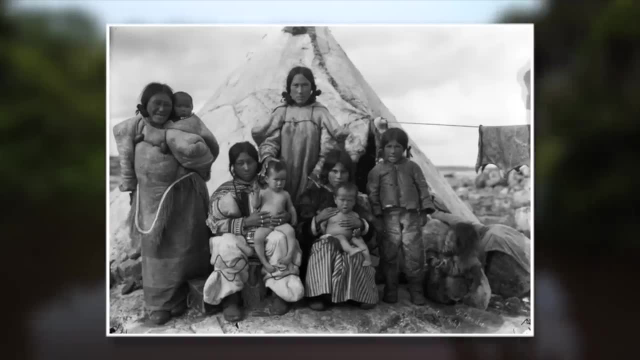 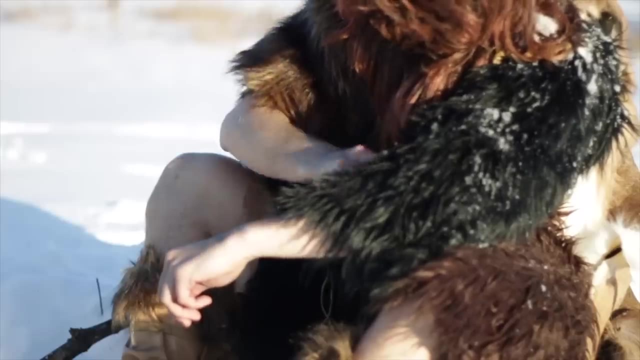 Individuals with healed head trauma and rib lesions suggest that they had methods to prevent major blood loss. Bandages made of animal skin may have been used. Some Inuit groups today use rodent skin to dress wounds. It is feasible that Neanderthals would have come across similar methods to stop the blood. 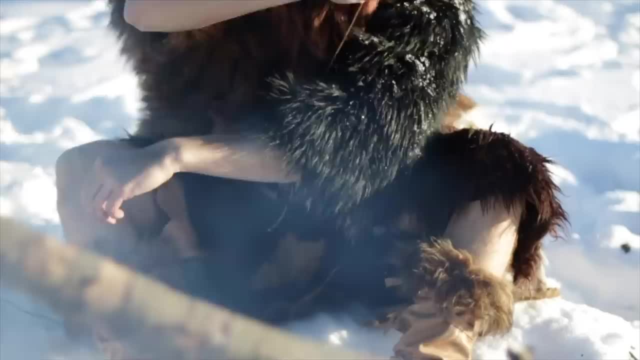 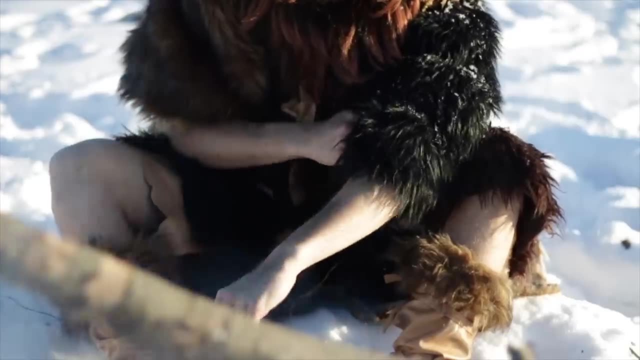 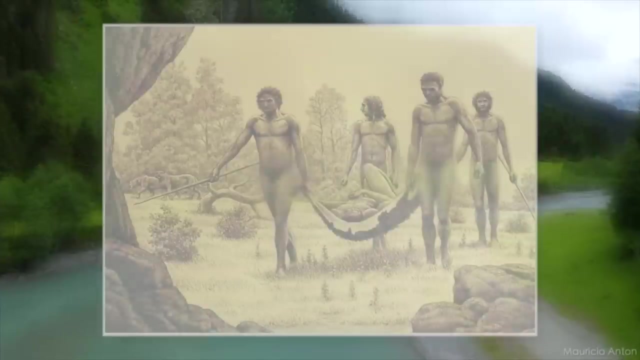 flow and to keep the wound relatively hygienic. Perhaps more impressively, they appear to have avoided severe infections, indicating good long-term treatment of their wounds. The high level of injury and recovery from serious conditions such as a broken leg suggests that others must have collaborated in their care and helped them not only ease the pain. 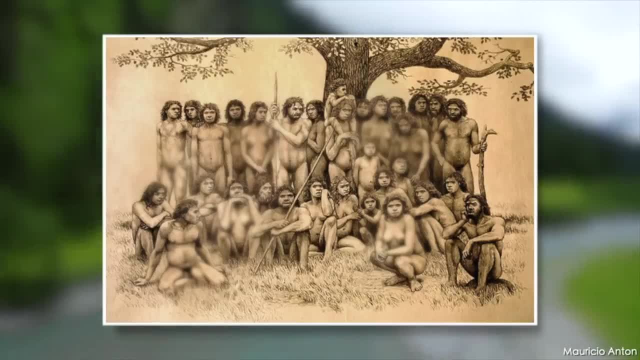 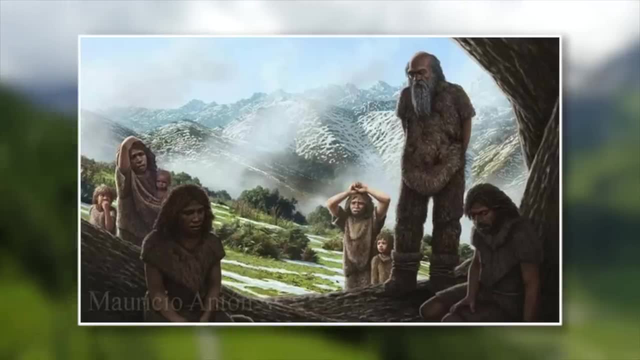 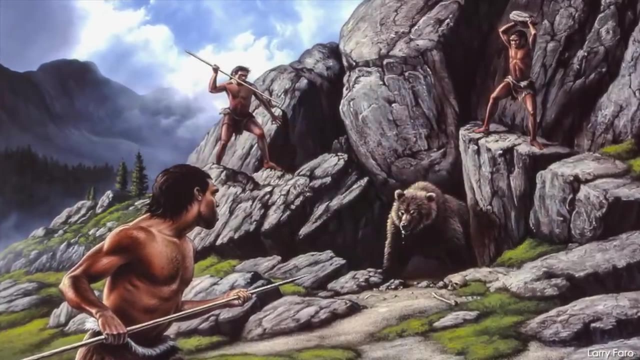 but to fight for their survival in such a way that they could regain health and actively participate in the group again. Neanderthals lived in small groups, so any loss of life could prove catastrophic for the survival of the group. Injury over disease was the most common threat, as Neanderthals didn't live in the type 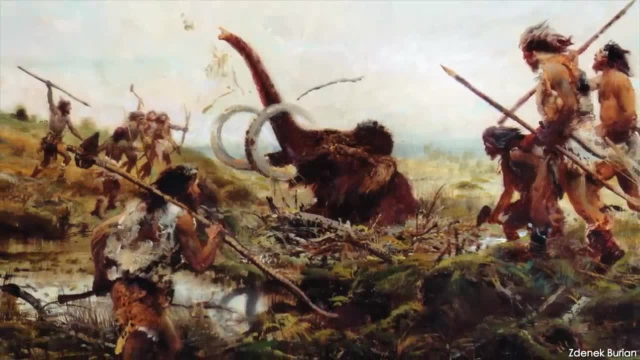 of environment or in large enough communities to be at high risk from pathogens. Neanderthals are known for their ability to heal wounds and their knowledge of medicine. medicine and medicine. Neanderthals are known for their ability to heal wounds and their knowledge of medicine. 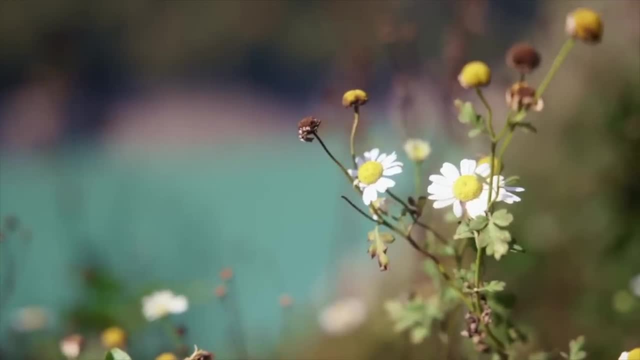 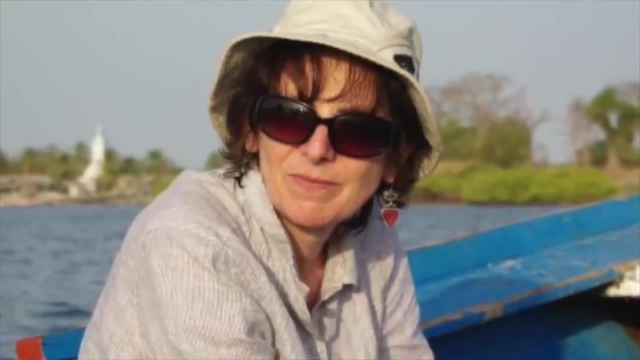 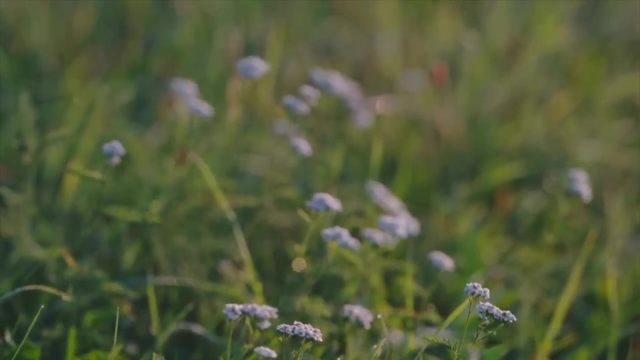 medicine, and medicine Fuels and medicinal plants appear to have been comparable to that of contemporary hunter-gatherers. Karen Hardy of the Catalan Institution for Research and Advanced Studies has spent years analyzing the calcified plaque left on Neanderthal teeth. In one individual, she found the chemical signatures of yarrow and chamomile. 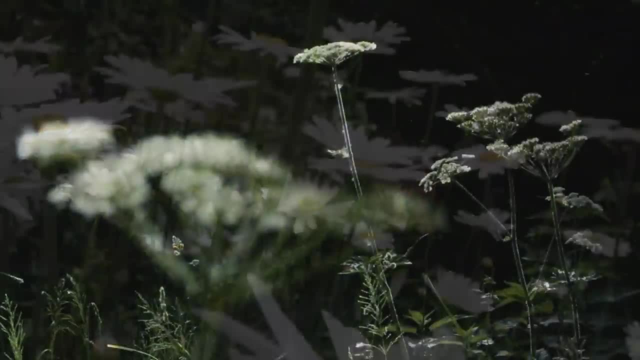 These plants may have been used as herbs, though they taste extremely bitter and have little nutritional value. She hypothesizes that they used to be plant 끝나a, our, because we always eat them. Or, in turn, maybe chestnuts. 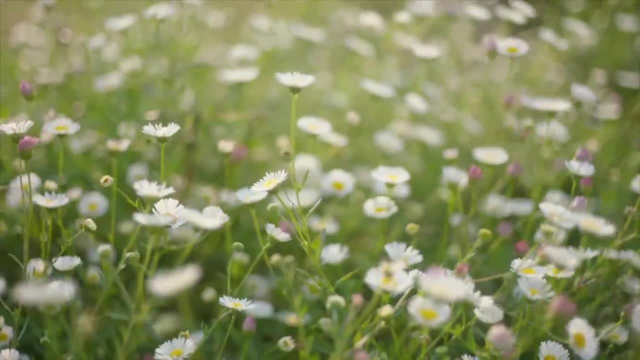 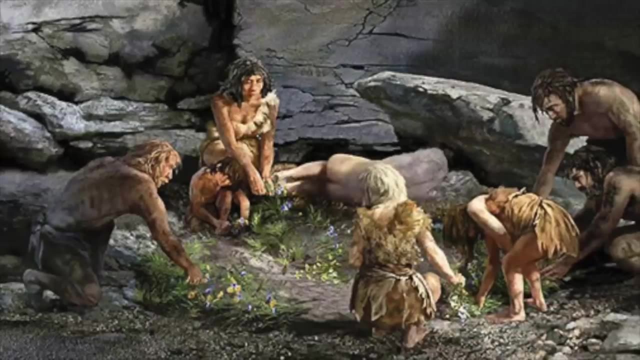 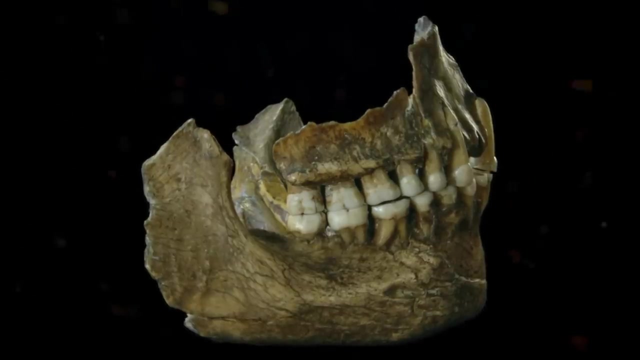 used for self-medication. Both of these plants have anti-inflammatory and fever-reducing properties. At the Shannon Dar Cave, the flower burial may have included these plants. Analysis of another Neanderthal individual revealed traces of poplar in the mold: penicillium. 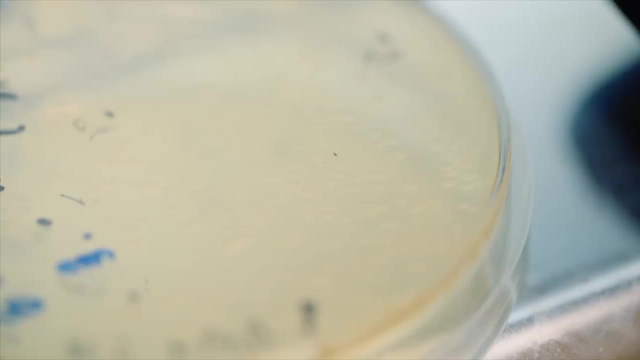 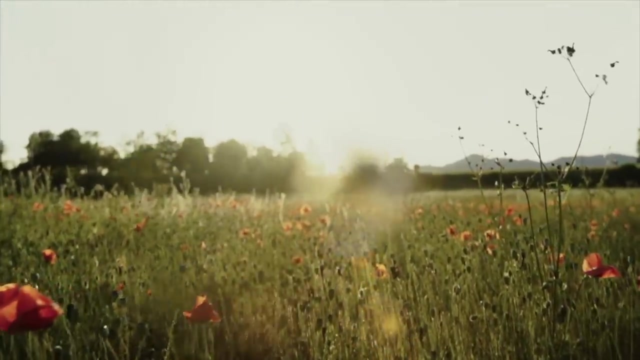 Poplar contains the natural painkiller silicic acid, while the mold penicillium is, of course, one of our most successful antibiotics. While we can't be sure that Neanderthals deliberately ingested these substances for medicinal purposes, it's telling that this individual suffered from. 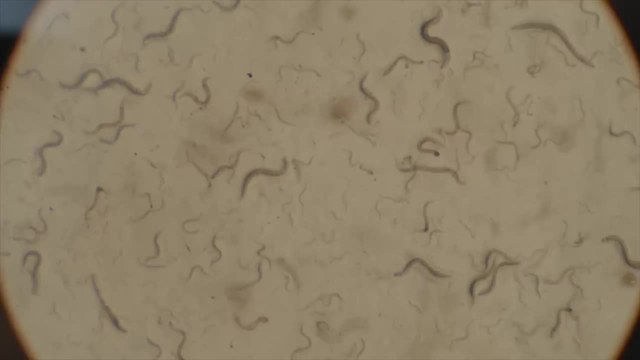 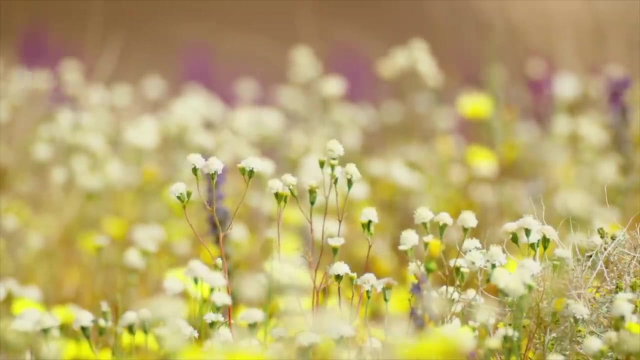 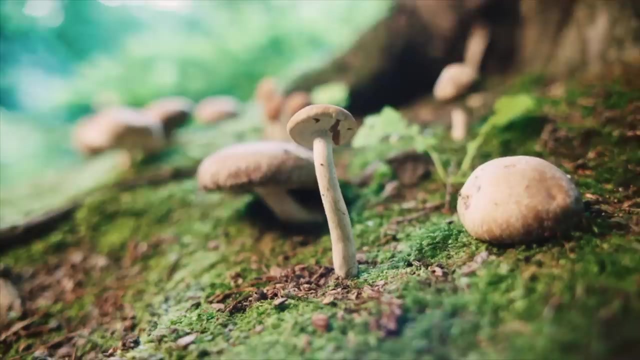 a severe tooth abscess. The individual also had painful parasites which would have caused diarrhea. These plants were likely used to cure both of these ailments. Many have speculated that early humans and other species such as Neanderthals may have used psychoactive drugs for. 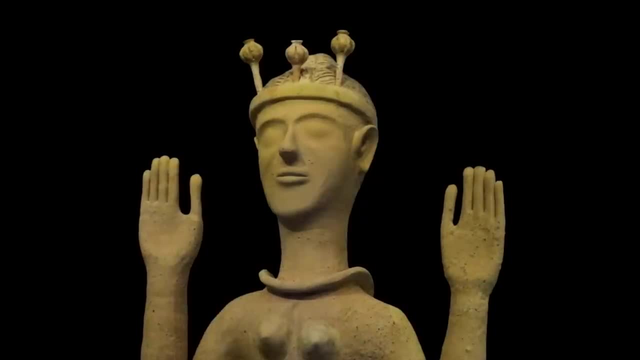 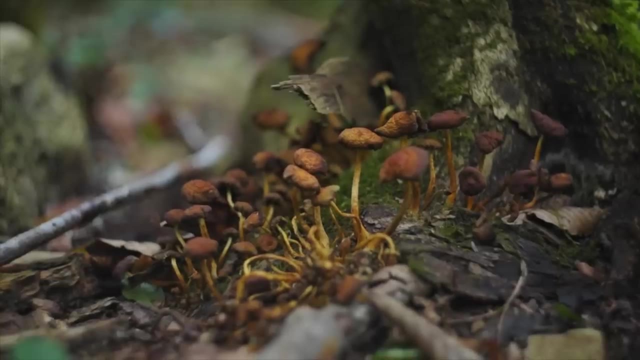 a variety of reasons. Evidence of psychoactive drug use only goes back a few thousand years. though it is likely underrepresented, Powerful hallucinogenic mushrooms did grow in the range of the Neanderthals and they would have been aware of them. 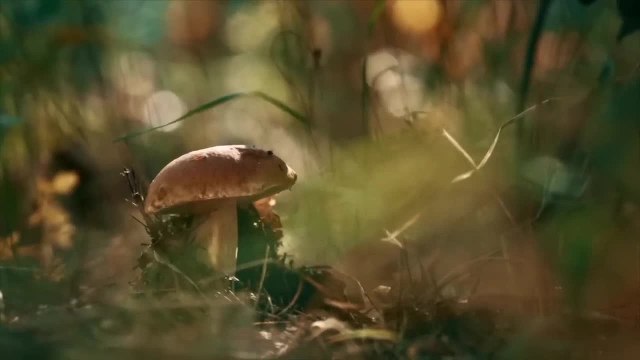 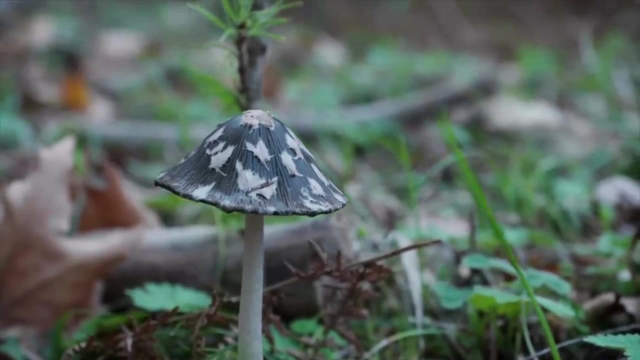 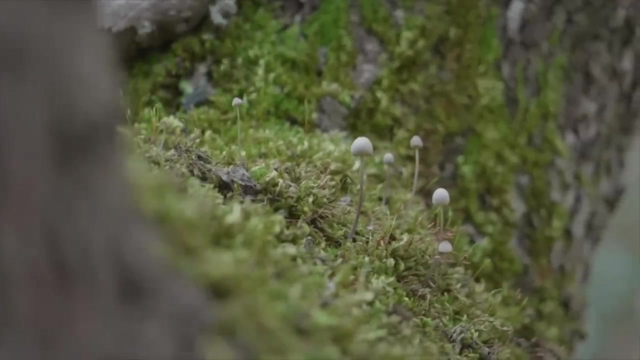 It is possible that they were consumed for their mind-altering effects, and perhaps they were even part of spiritual practices. However, no evidence of these mushrooms exists in Neanderthal dental calculus or at Neanderthal sites. It is entirely possible that these mushrooms were being consumed, though without evidence we can only speculate. 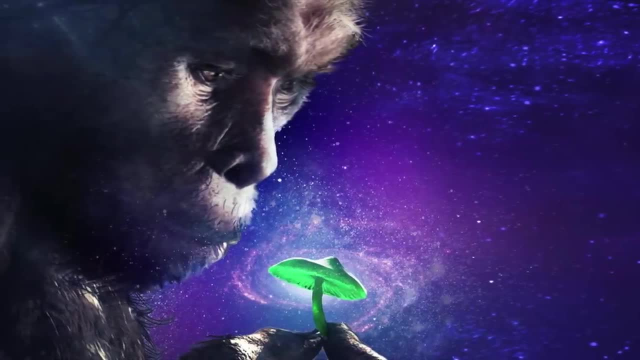 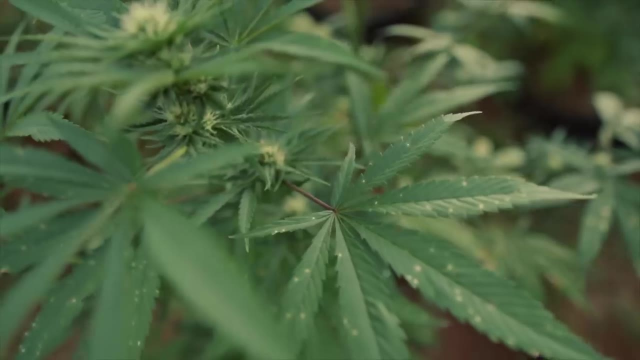 Some have proposed that psilocybin mushrooms may have had a profound effect on the evolution of our genus, though this theory has little evidence to support it. It appears that psychoactive drugs were not used very much until relatively recently in human history, Besides medicine or drugs. 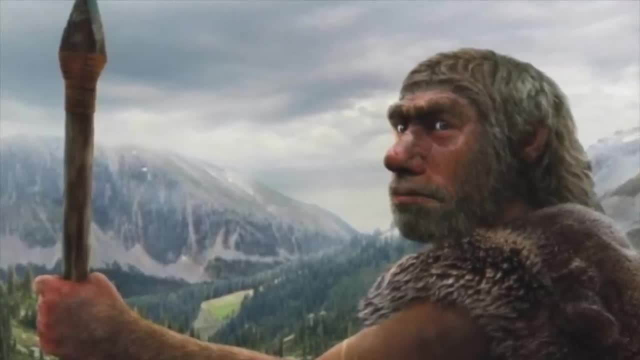 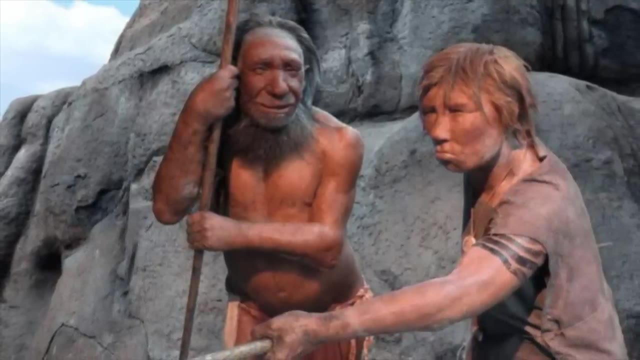 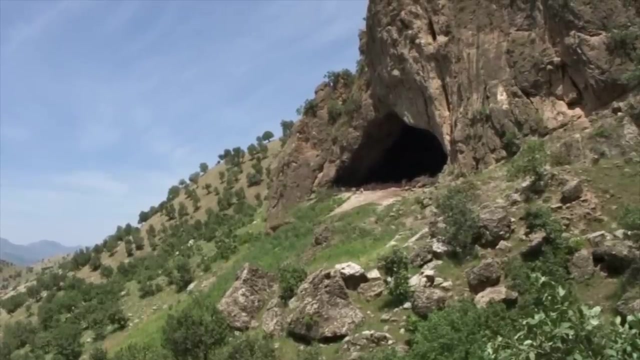 other healthcare practices would have also been very important. Sick, injured and especially sick individuals would have had to be fed and cared for. Perhaps the most fascinating display of Neanderthal healthcare and compassion comes from the remains at Shanandar Cave. Remains of a Neanderthal who survived well into his forties were named Shanandar One. 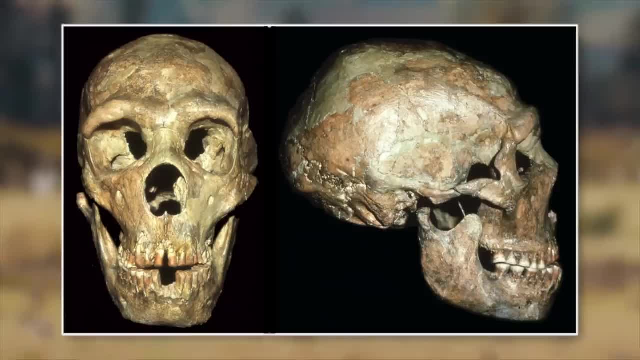 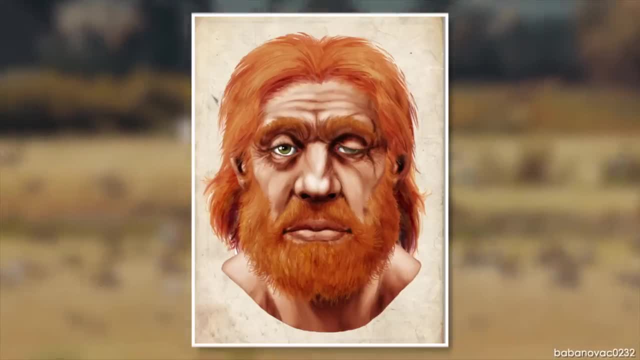 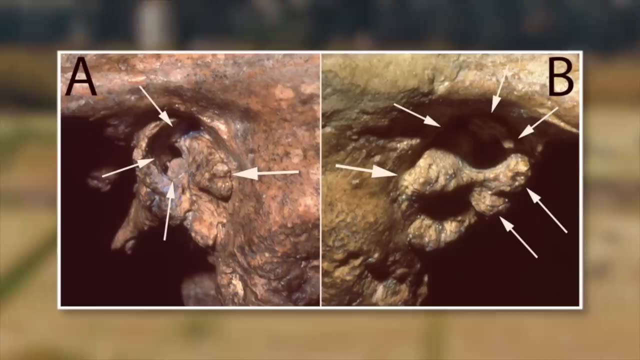 This man lived an excessively painful life. He had suffered a violent blow to the left side of his head at a young age. It fractured his orbital and left him partially or totally blind. in his left eye, These were abnormally worn, a sign of a degenerative disease He also suffered from. 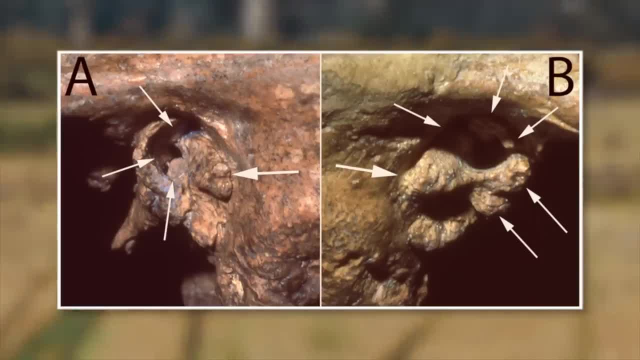 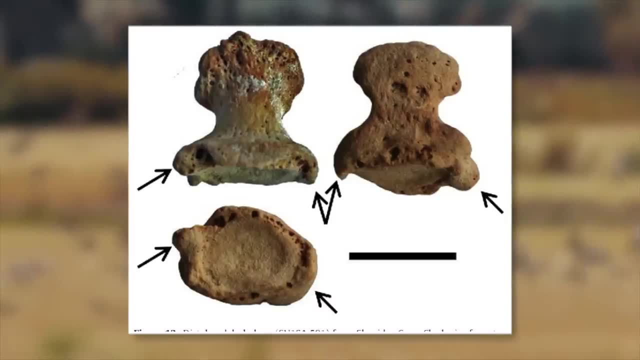 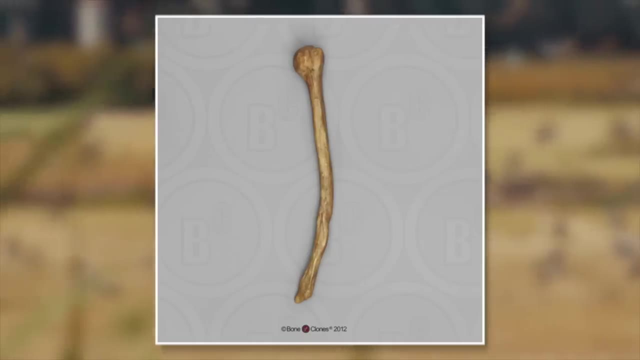 severe hearing loss which left him partially deaf in one ear and likely completely deaf in the other. Damage to his C5 vertebrae caused his right arm to lose muscle function. This arm was likely amputated later in his life. If so, it is the earliest evidence of amputation. 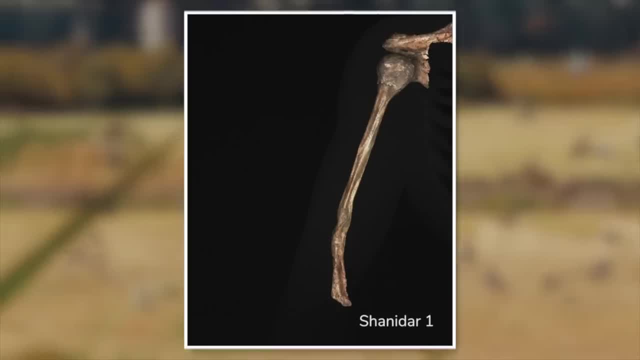 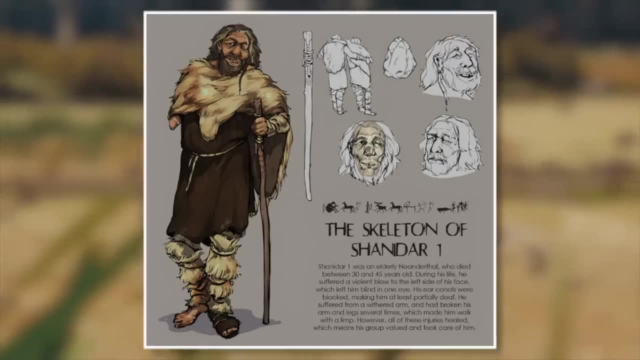 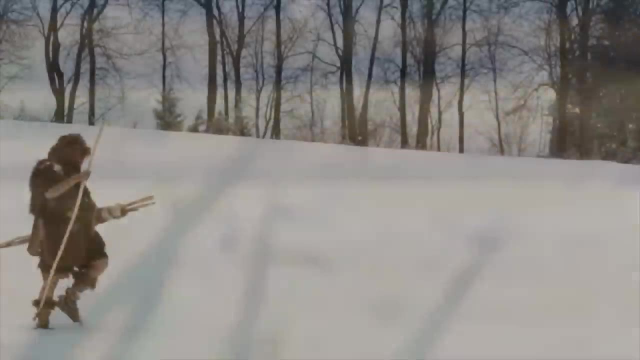 on a living individual. The damage to his arm and vertebrae caused some paralysis on the right side of his body And to add to all this, he suffered from not one, but two broken legs. They had healed, but left him with a painful limp. Even so, his legs seemed to have been walked on to a similar. 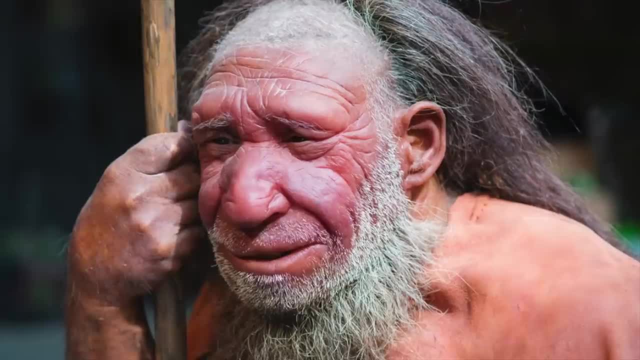 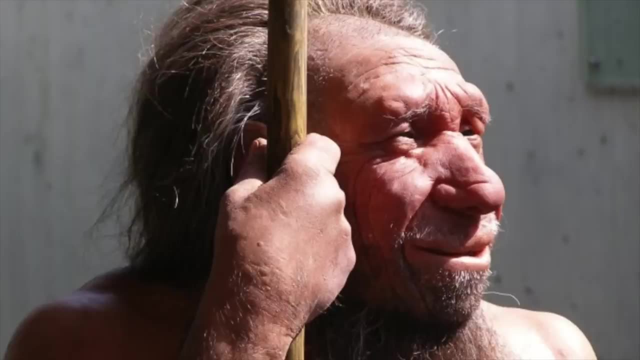 degree as other Neanderthals. With all of these debilitating injuries, he seems to have survived well into his forties, perhaps nearing his fifties, Though he was still able to walk and use one arm. he wasn't taken down, woolly rhino, by him. 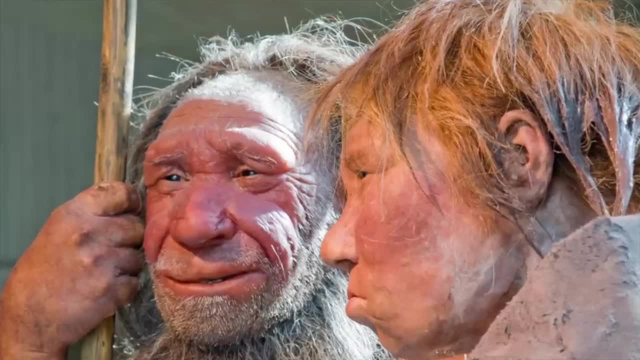 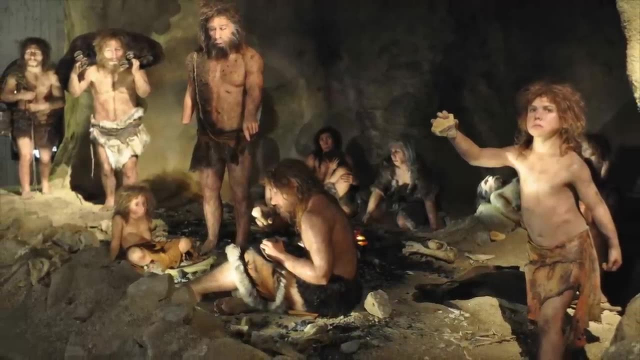 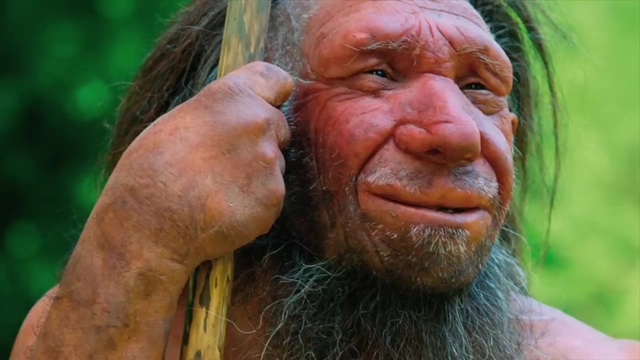 He survived with a little help from his friends. They would have had to at least partially feed him and certainly protect him from predators. After a long and loving life, he appeared to have died of natural causes. This level of altruism is hardly ever associated with Neanderthals, Even some human hunter-gatherers. 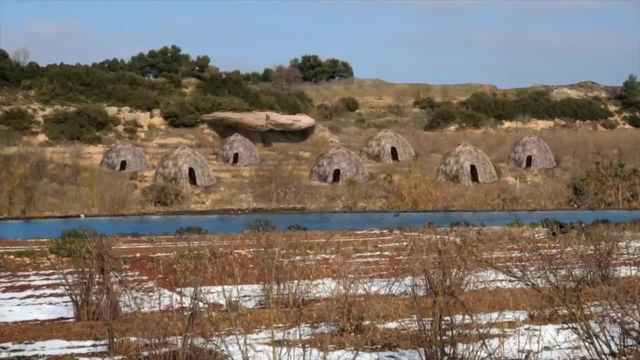 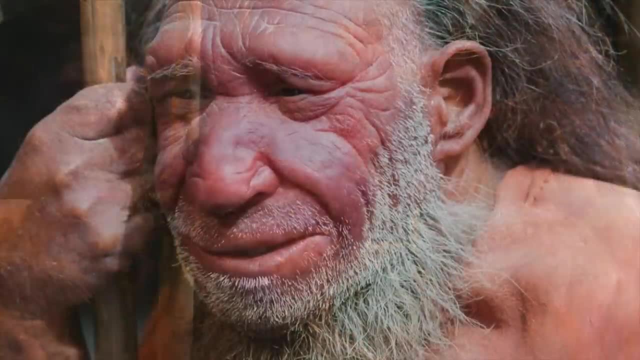 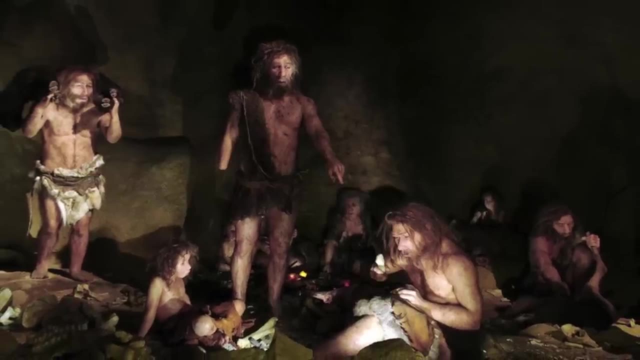 have practiced killing off the weak and elderly for the good of the tribe. But these Neanderthals, all those thousands of years ago, valued this man. He was a part of their family, a father, a brother, maybe even a grandparent. At the tribe's expense, he was kept alive. 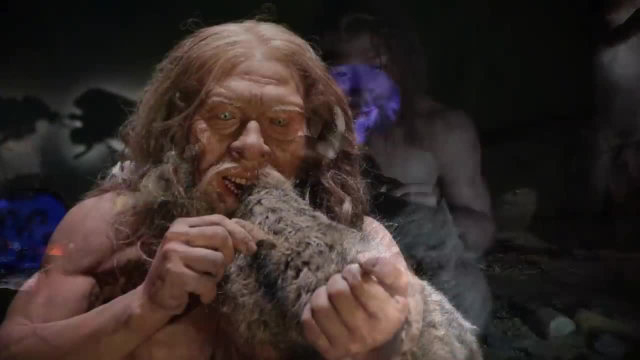 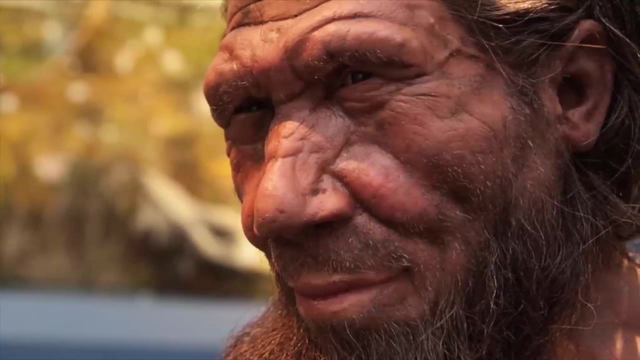 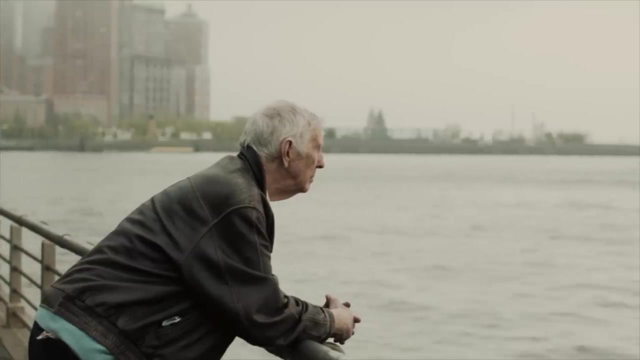 Perhaps he actually provided the tribe plenty of valuable information that actually benefited their survival. Elderly Neanderthal remains are not exceptionally common, though there are misconceptions regarding their lifespan and life expectancy. Lifespan is defined by the maximum number of years that an individual can live, while life expectancy is the average. 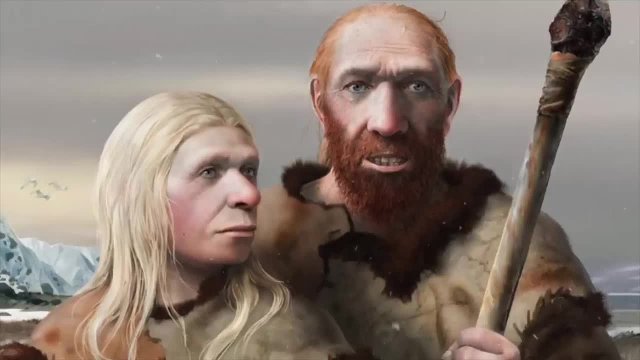 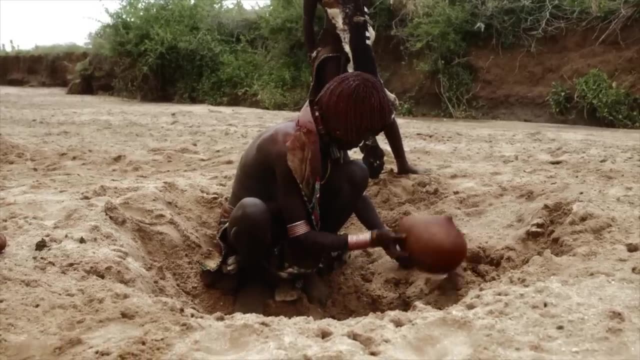 number of years that an individual lives. Neanderthals had a life expectancy of between 25 to 40 years old. This is about the same as modern human hunter-gatherers, depending on what population you are looking at, But these hunter-gatherers can have lifespans. 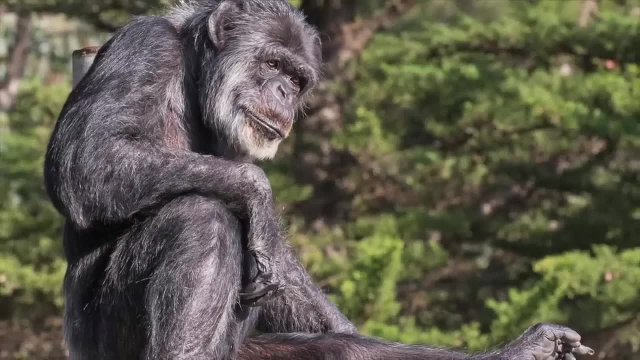 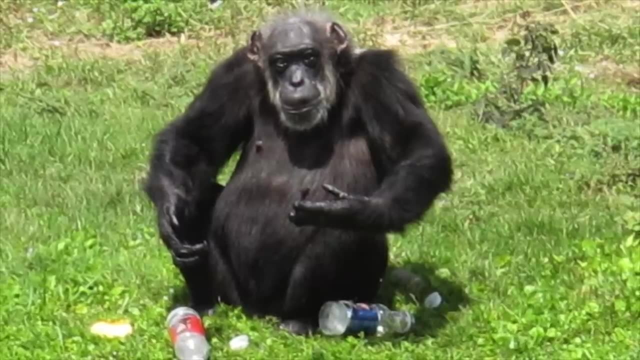 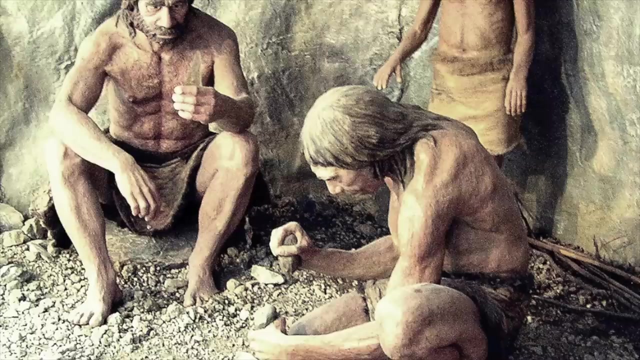 over 70 years of age. Even a wild chimpanzee reached an age of 63, while captive individuals reached their late 70s or early 80s. It is perfectly reasonable that a very small number of Neanderthals could have made it to a similar age At any given time. a Neanderthal group may 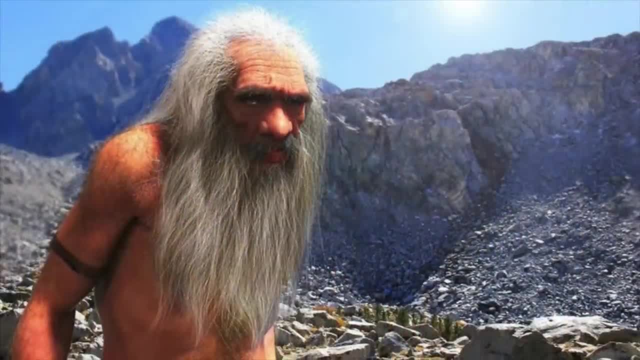 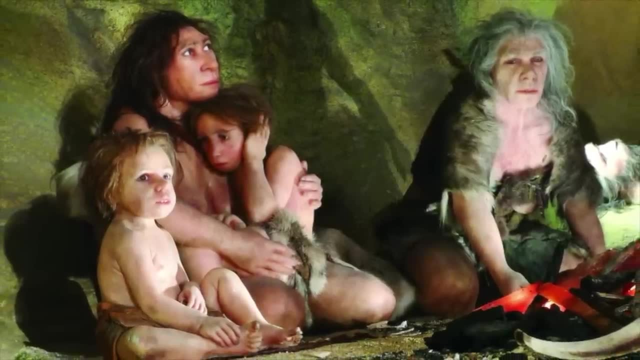 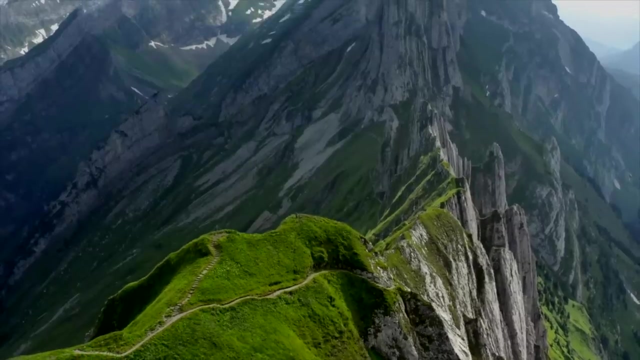 have even had individuals in their 40s or even 50s who actively participated in daily activities. Three living generations would have not been out of the ordinary for any group. Older individuals would have been highly knowledgeable about many things. They would have had a much more. 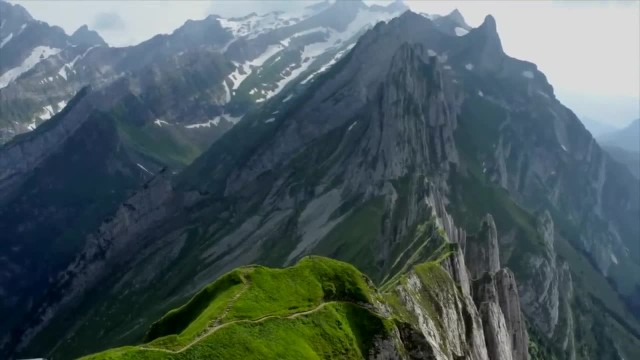 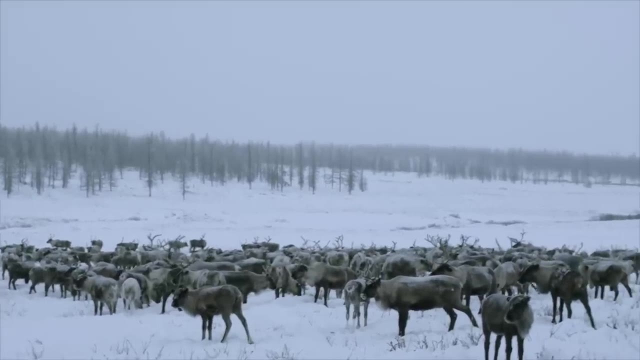 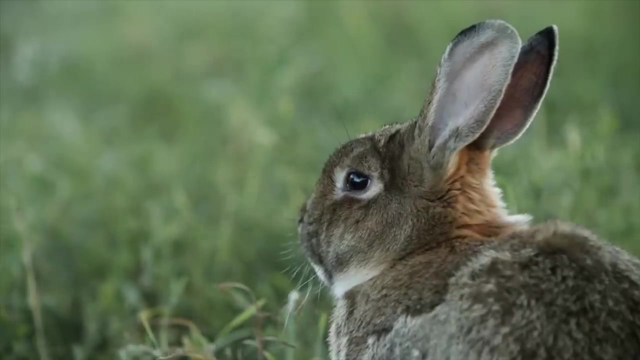 detailed mental map of the landscape than younger individuals. They could also remember seasons where there may have been much more snow or times when herds migrated in unexpected ways. Even if they were not able to directly hunt large game, they would have been competent at hunting small game, time-consuming, foraging and taking care of the little ones. Young Neanderthals. 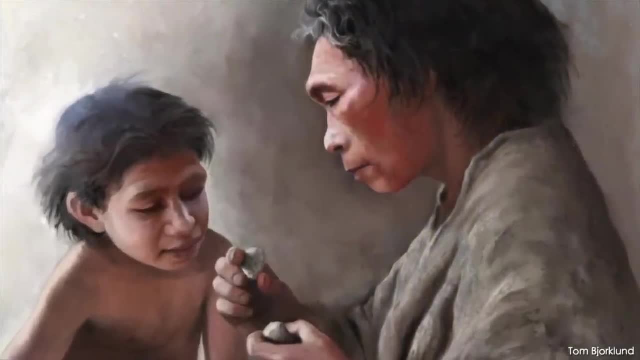 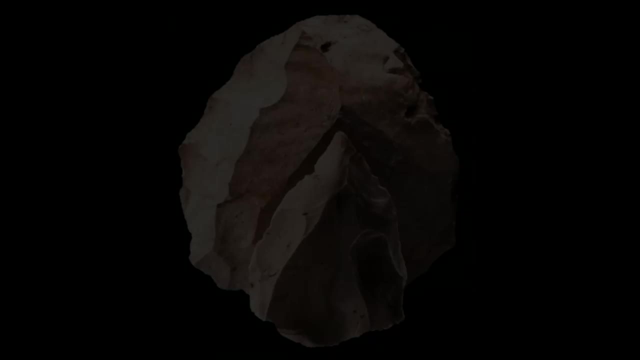 would have had to have been taught flintknapping for many hours. Though some Neanderthal tools may be simplistic, creating them can be a challenge even for modern flintknappers. We also have to think about the fact that even prime-aged adults would have been injured fairly frequently, and 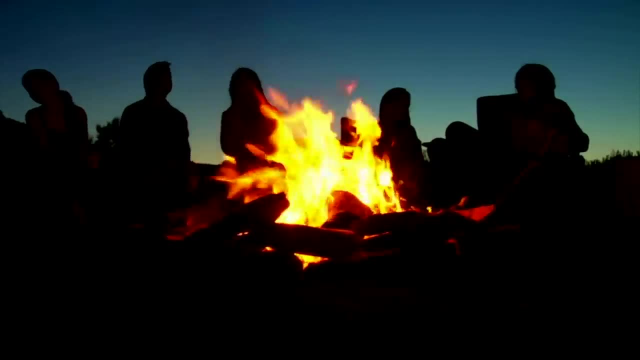 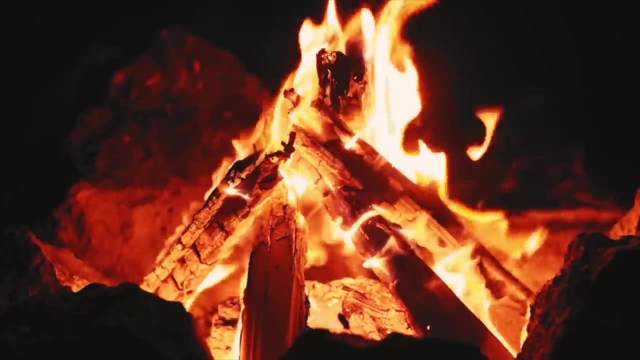 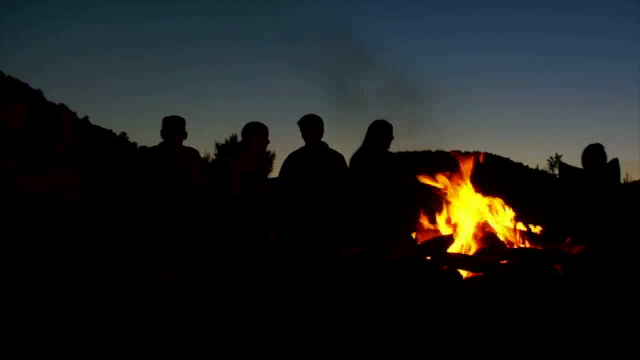 would have needed care. We also cannot underestimate the importance of elders telling stories around the fire. A simple tale about an old friend eaten by a cave bear may have served as an important educational moment for anyone listening. Stories from long ago may have been passed on for many generations. 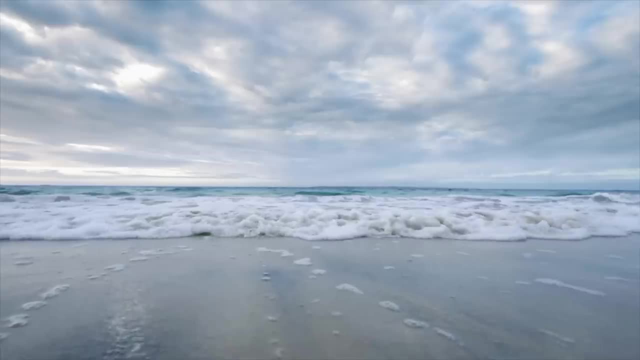 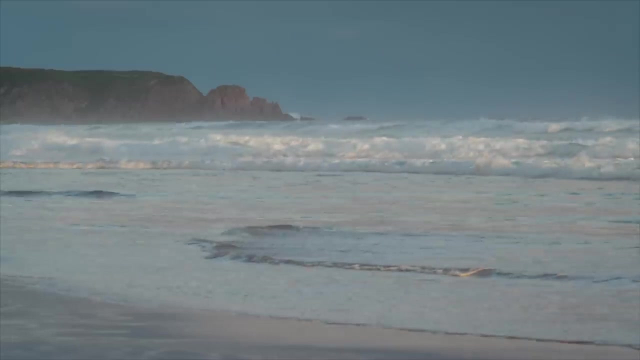 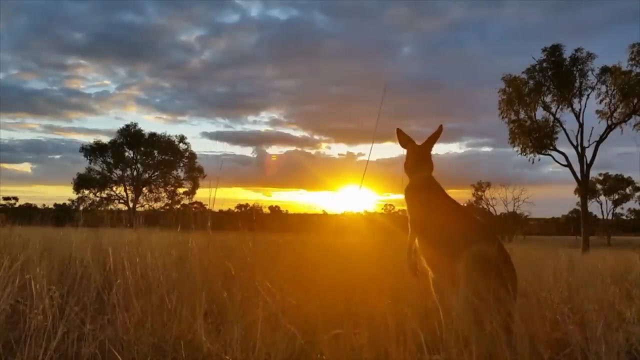 Australian aboriginals from coast to coast tells stories of when the sea rose long, long ago. Much of Australia is surrounded by extensive shallow shores, no more than 9 meters or 30 feet deep. Over 7,000 years ago they would have been grazing grounds with many. 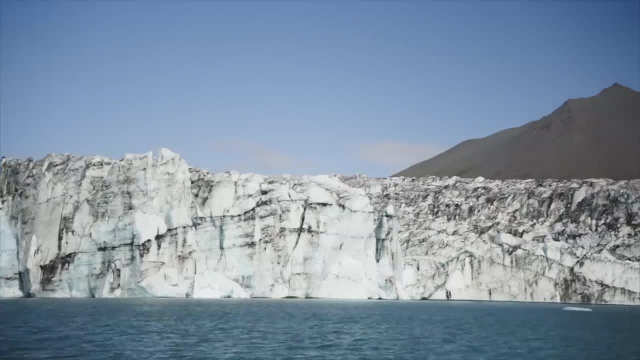 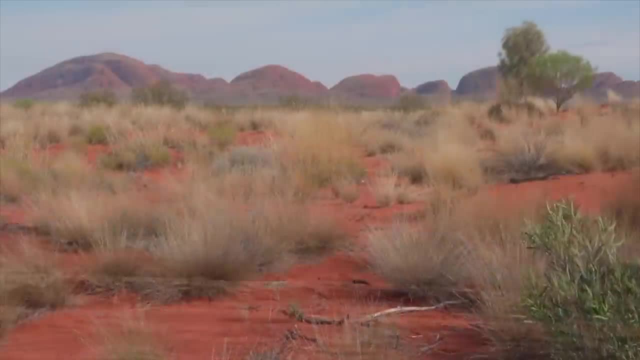 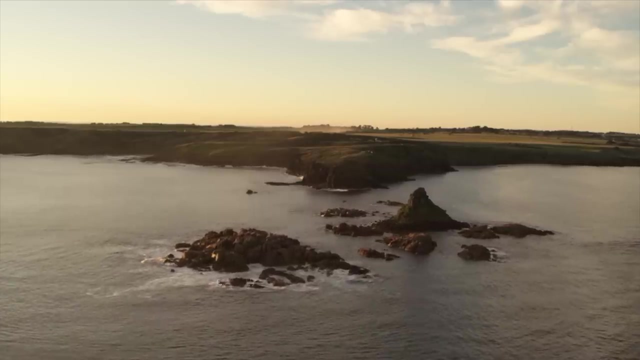 other islands sitting offshore. After the glaciers melted, the sea levels rose and an unimaginable amount of land sank beneath the shore. Over the next 400 generations, stories about the rising waters persisted. Some even recall the names of great islands that were once above the waves. 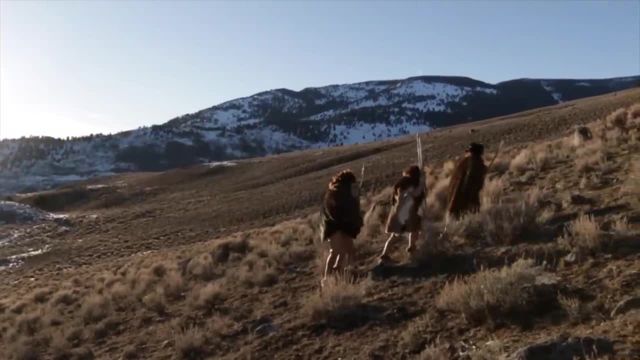 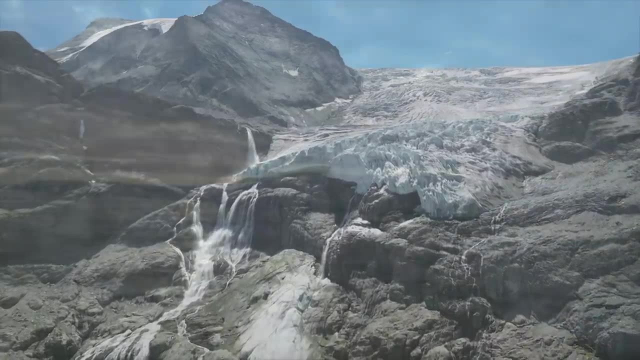 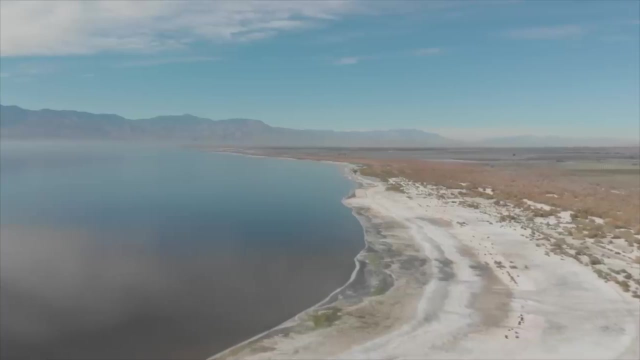 Similar stories may have actually been important for Neanderthal survival. Their climate was ever-changing and herds moved accordingly. Stories of massive glaciers or rising sea levels may have persisted for hundreds or even thousands of years. It is even possible, if not likely, that some of these stories were passed on to the newcomers. 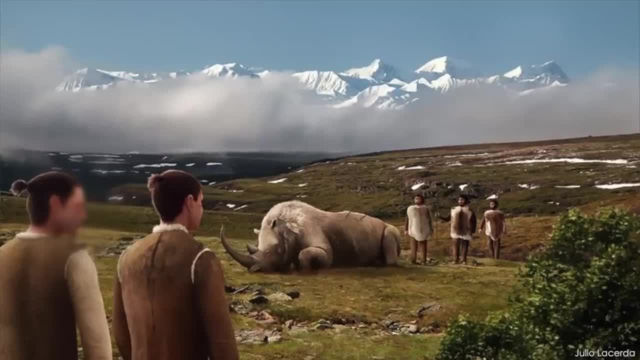 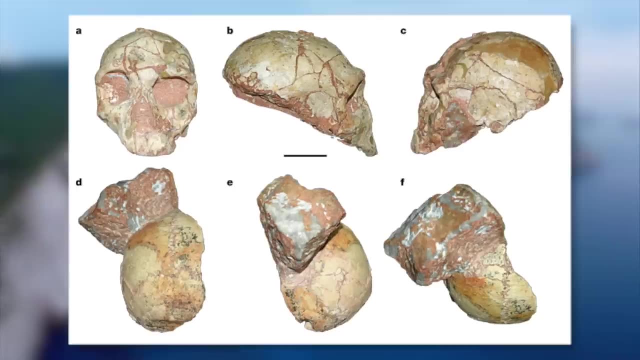 from the south. Neanderthals and Homo sapiens were not completely isolated from each other for hundreds of thousands of years. Remains from Apidema Cave dating to 210,000 years ago suggest that archaic Homo sapiens may have been present in Greece much earlier than once thought. 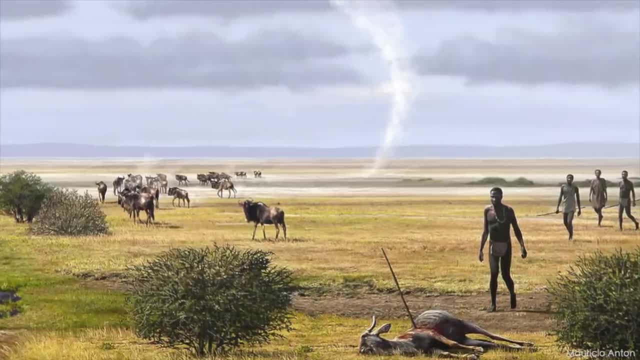 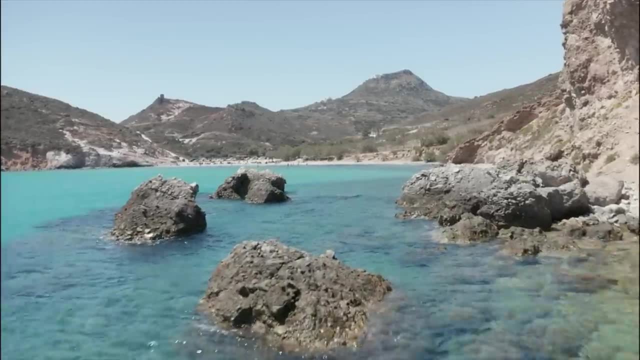 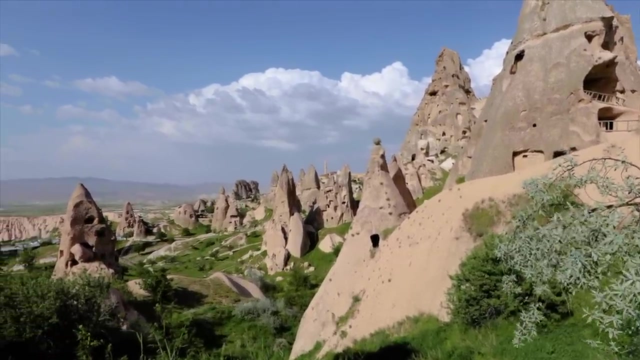 Though, if these fossils do represent sapiens, they do not appear to have stayed long. The fossils may represent an occasional unsuccessful migration deep within Europe from the Near East. The Near East was a very important place for our species and for Neanderthals. 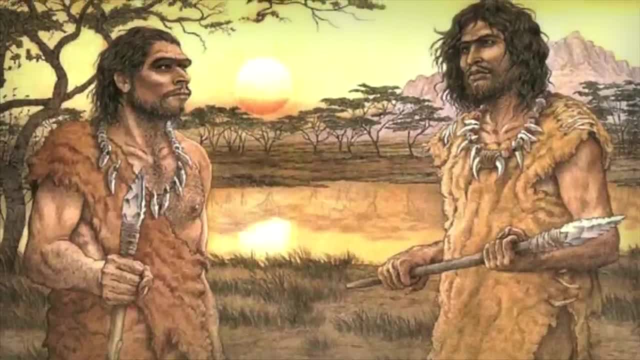 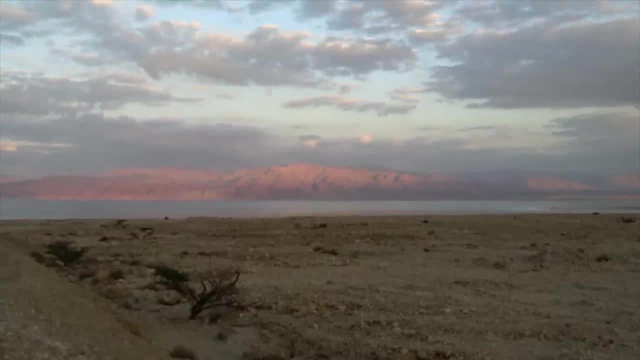 Both species ranged throughout it and genetic suggest that interbreeding occurred as early as 120,000 years ago. Homo sapiens remains from a number of sites in Israel date as far back as 200,000 years ago and nearby Neanderthal sites date to the same period. There is no doubt about it, doubt that Neanderthals and modern humans in the Near East regularly interacted and even created families together For over 100,000 years. both Neanderthals and modern humans lived in this region. Meanwhile, other populations of modern humans were spreading throughout much of Asia. 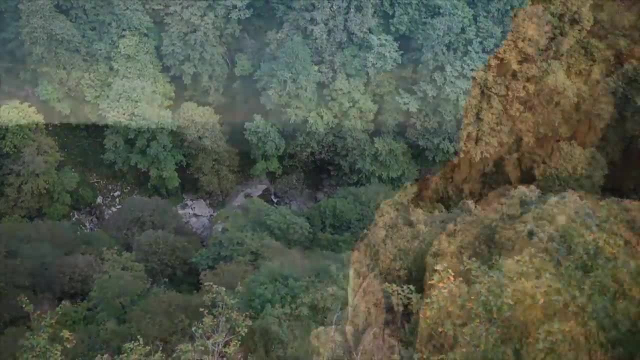 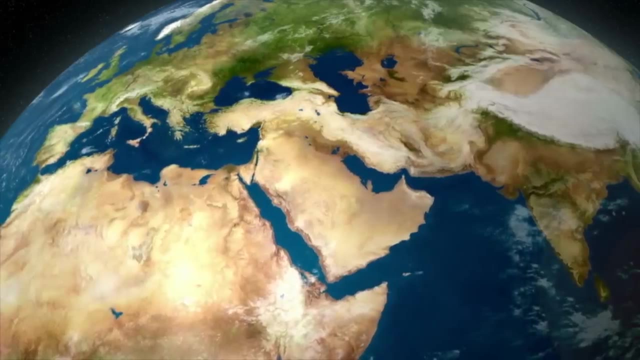 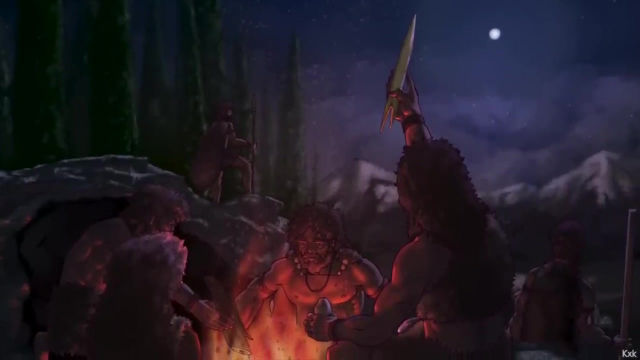 They made it to the Indian subcontinent by 80,000 years ago and even Australia by around 65,000 years ago. Meanwhile, the modern humans in the Near East do not seem to have encroached into Europe until later. The appearance of modern humans in Europe is very complicated. It was: 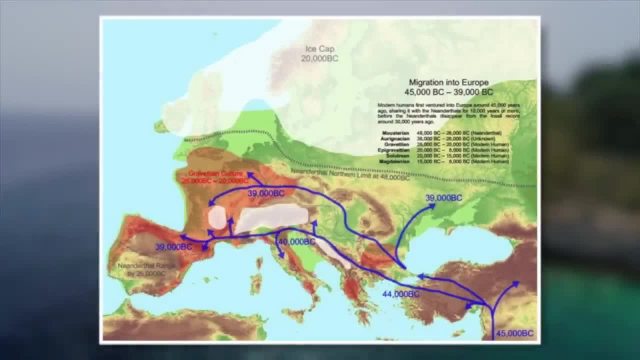 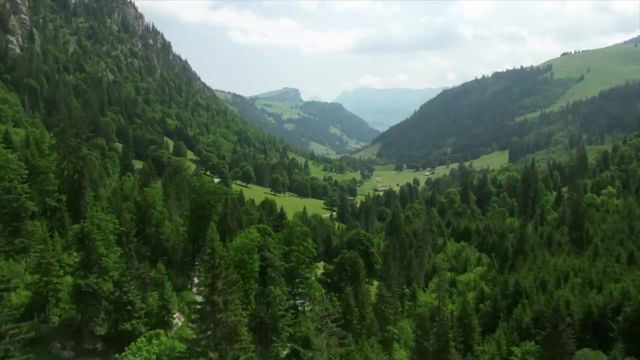 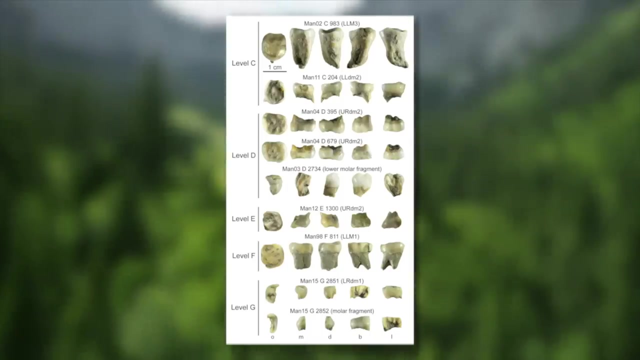 previously thought that sapiens first followed the eastern Mediterranean coast to enter southeast Europe between 43,000 and 48,000 years ago, Though a 2022 study found modern human fossils in France dating to between 51,000 and 56,000 years ago. Alongside their remains were peculiar stone tools. 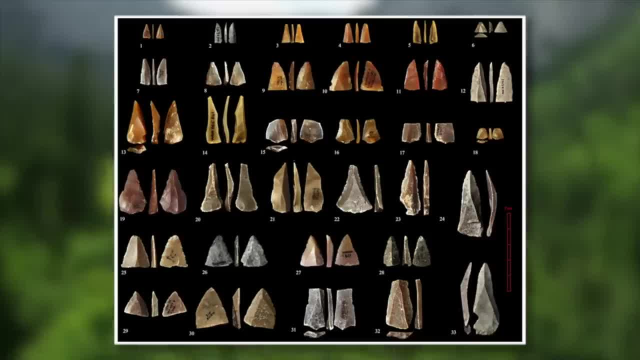 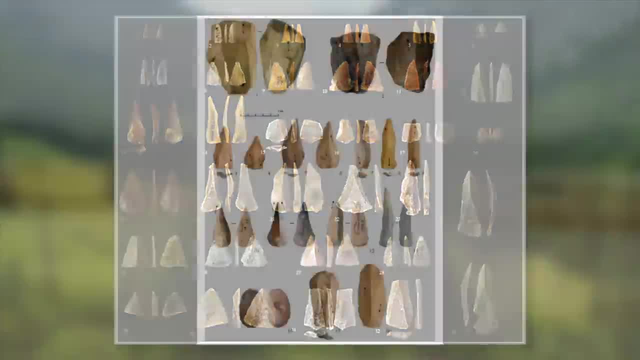 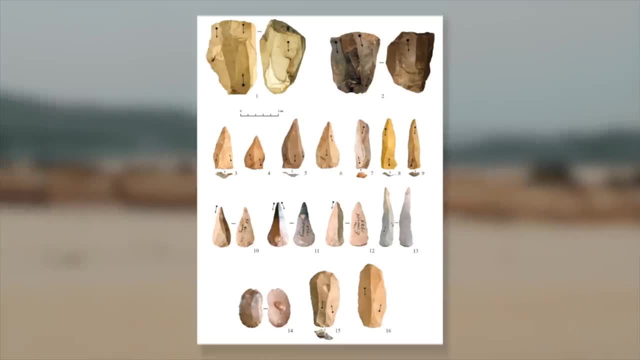 dubbed the Neronian tools. They consist of small projectile points that may have been spears, though they could have also been atlatl points or even arrowheads. This technology is similar to technology from Africa and the Middle East, which now makes sense, considering that it was likely modern humans that made it. 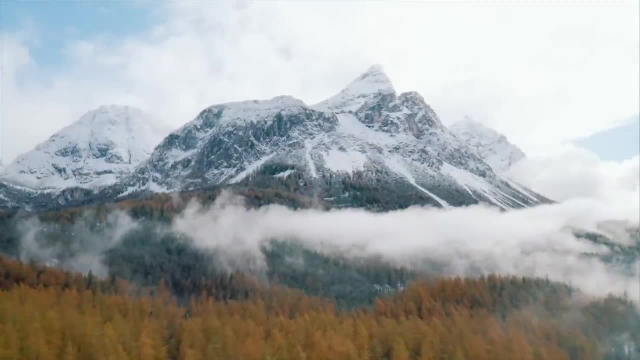 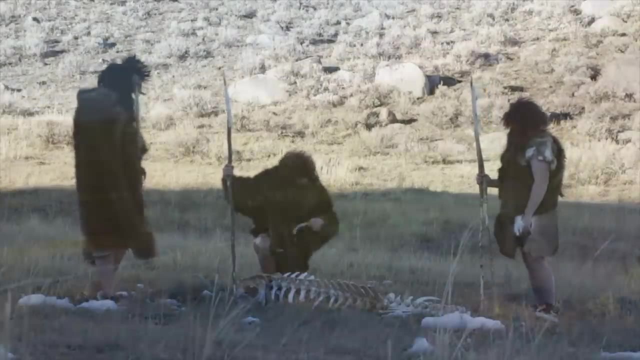 What is even more interesting is that just as soon as they came, they left. Neronian tools and human remains sit below additional layers of Neanderthal occupation. The remains at Grotte Mandarin may represent the remains of Neanderthals and Neanderthals, The remains of Neanderthals and Neanderthals may represent an unsuccessful migration by a population of modern humans, And this brings up an interesting point about this period: Europe was so sparsely populated that sapiens may have simply migrated in without even coming into conflict with Neanderthals. 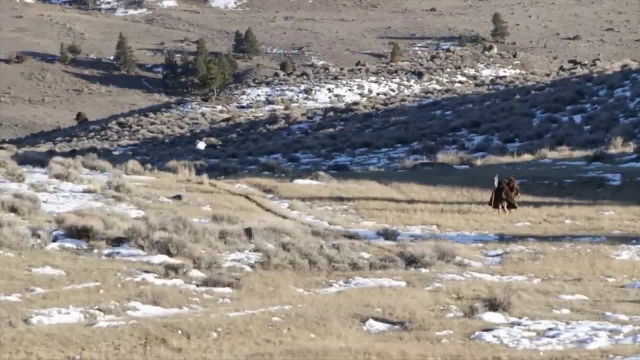 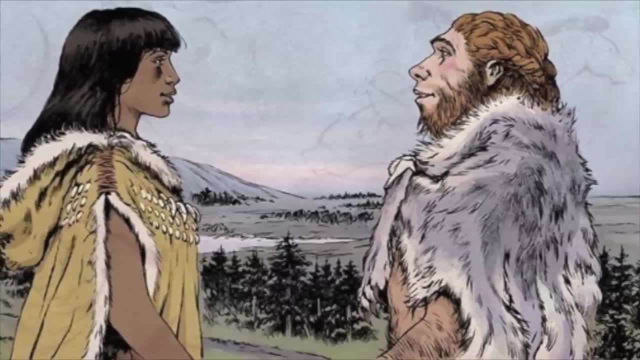 Neanderthals themselves likely would not have seen sapiens as anything but another group of humans. Modern humans may have looked slightly different, being taller, slimmer and likely darker, though from other examples we clearly see that Neanderthals and Neanderthals may not have been. 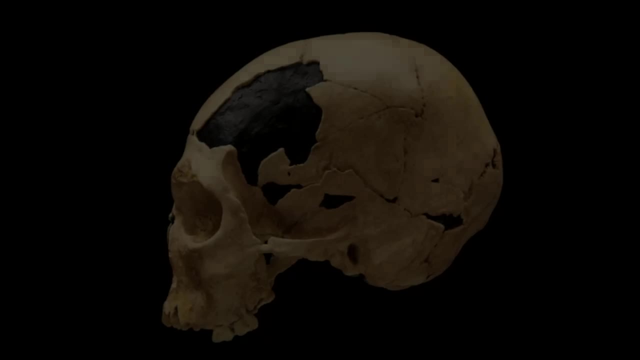 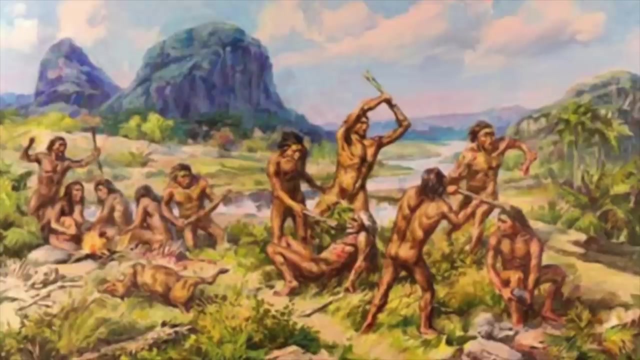 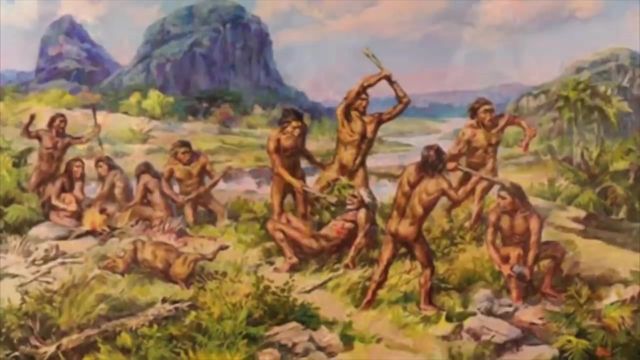 in conflict with Neanderthals. Neanderthal war parties fighting off encroaching warmongering sapiens is a scene of fiction. Once again, the Paleolithic does not appear to have been nearly as violent as some make it out to be. in regards to intergroup violence, We have not discovered 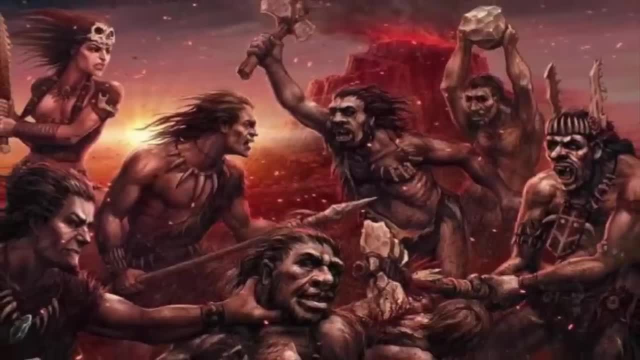 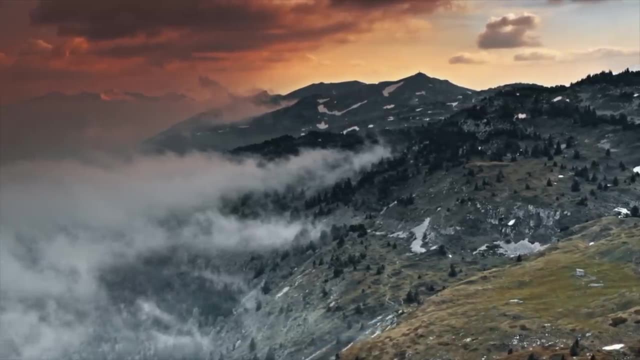 any evidence of sapiens or Neanderthals, who appear to have died in an interspecies war. The reason that sapiens had difficulty migrating into their region may simply be because Neanderthals were already living there. They were the ones adapted for the environmental conditions. 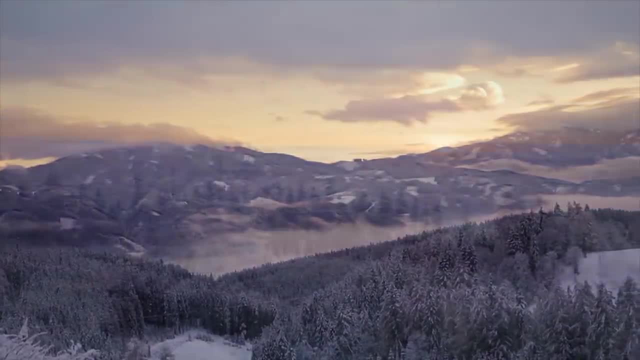 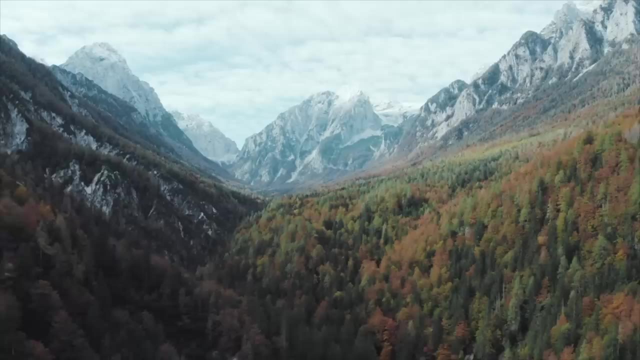 and there may not have been room for other humans. It does not appear that modern humans were able to find much success in Europe until they made technological innovations. This is why, even though humans were present for a short time in France over 50,000 years ago, 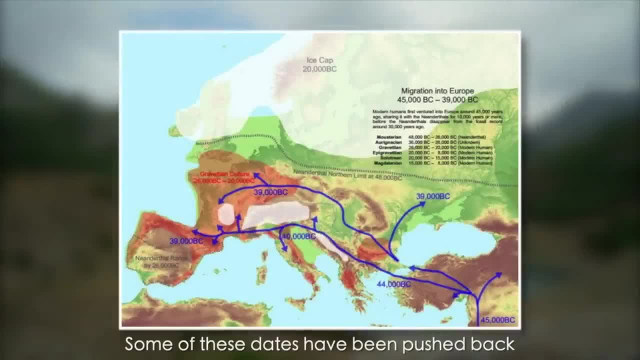 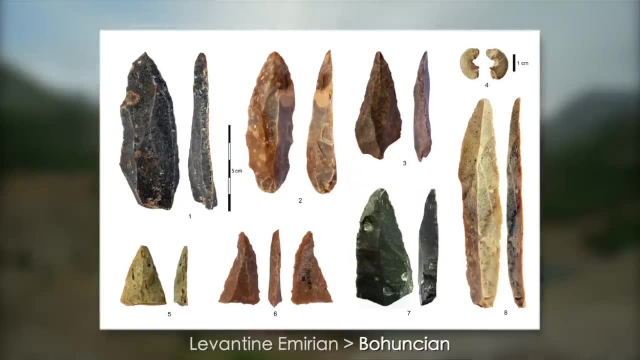 actual significant migrations did not seem to have occurred until around 48,000 years ago in the Balkans. Here, the Bohanty region is a typical example of modern humans being able to make a living in Europe. industry appears to derive from the Levantine Amerian industry. The Bohangian seems to be a 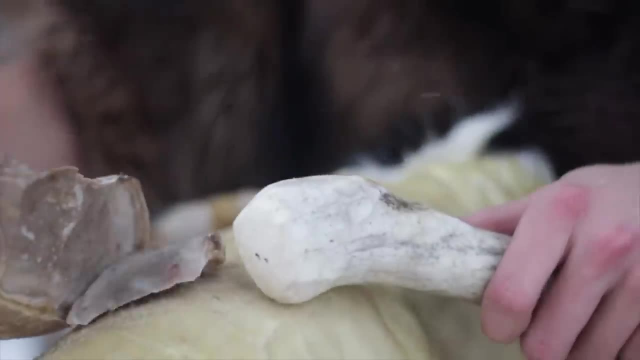 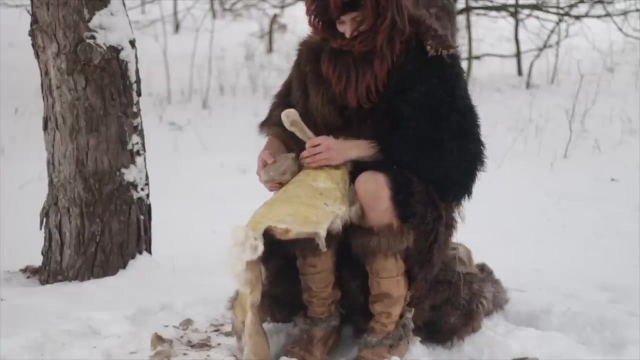 transitional industry between the Neanderthal Malstarian and the later Sapien Aurignacian. These tools may have been made by a population of both Neanderthals and modern humans, though we do not have fossil evidence. A few thousand years later, this industry would. 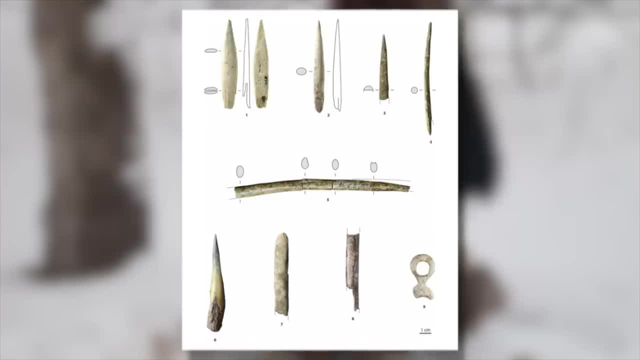 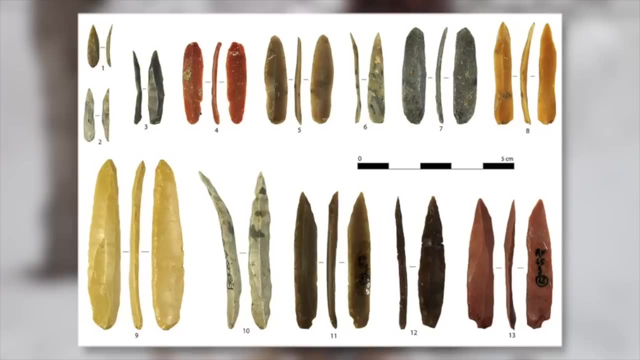 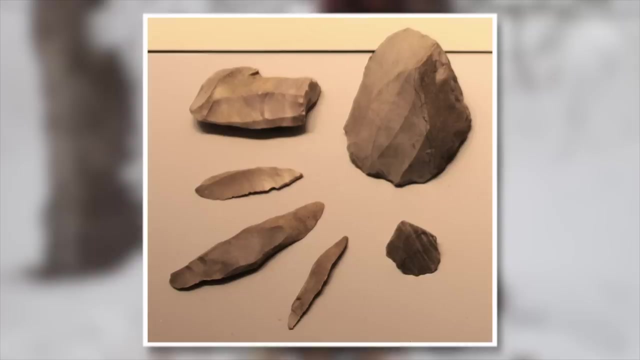 evolve into the Proto-Aurignacian. This technology consisted of bone and antler points, bone needles and awls and fine stone blades and bladelets. These blades could be attached to composite points to create very deadly weapons. Small cores that could easily be carried had the 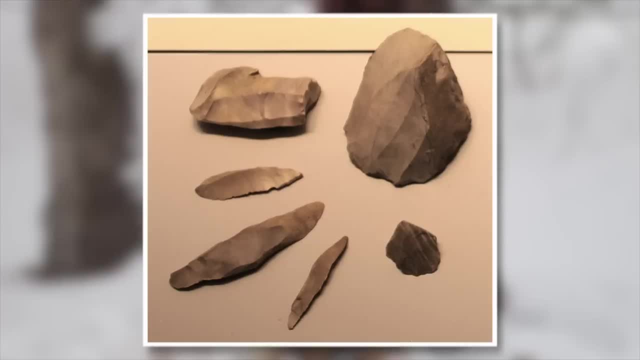 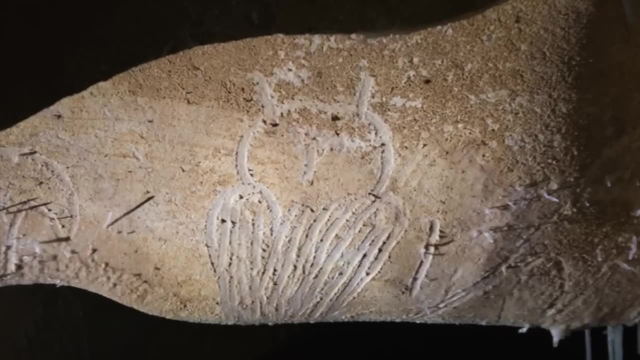 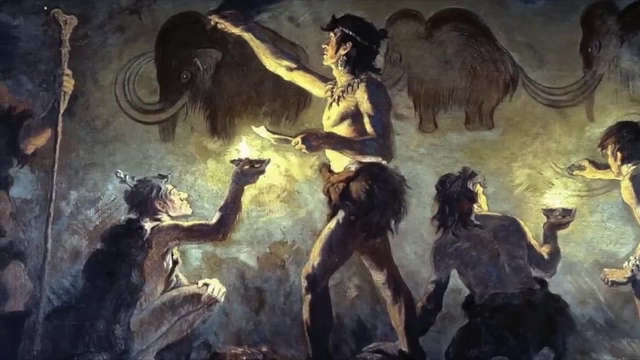 potential to create dozens of these razor-sharp microliths. Besides tools, upper Paleolithic technology is often associated with many cultural innovations, such as a variety of cave art and the formation of long-distance trade networks From about 45,000 years onwards. 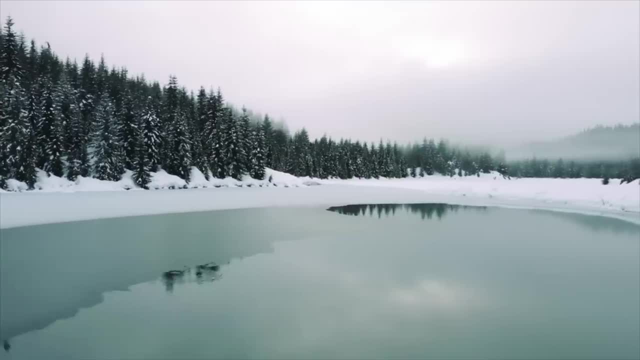 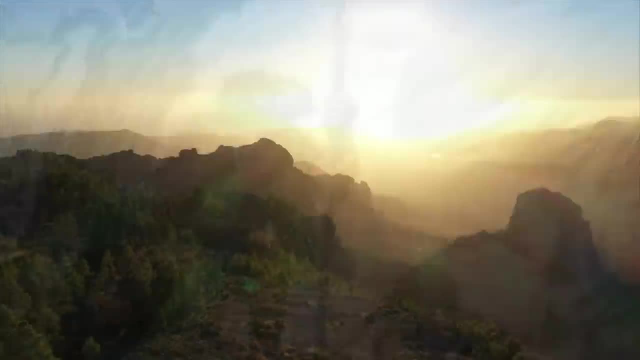 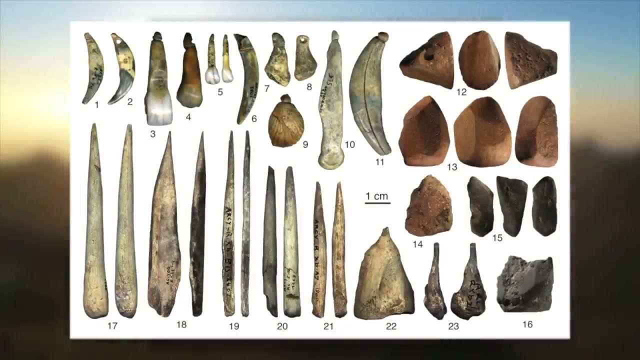 this culture and its Sapien creators would spread out throughout much of Western Europe. But the replacement of the Neanderthals was not so simple. Another stone tool industry from France and northern Spain called the Chateau Peronien existed from 45,000 to 40,000 years ago. 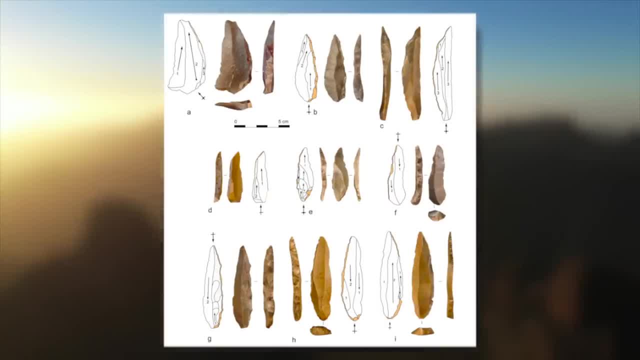 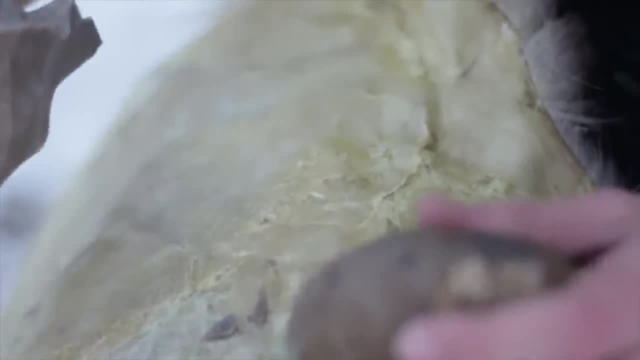 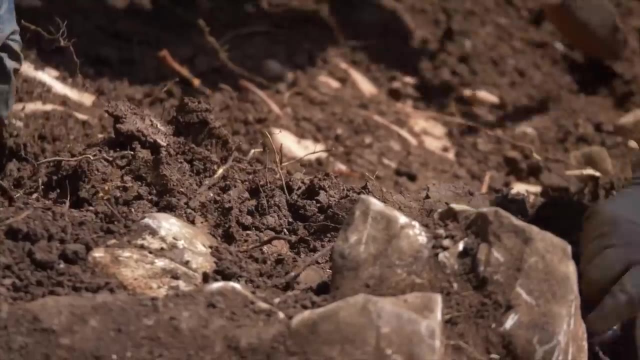 This industry was also upper Paleolithic and may have been produced by Neanderthals. Some have suggested that Neanderthals were adopting Sapien technology, while others believe these tools were made by hybrid populations or simply by Homo Sapiens. The industry may also partially be the result of disturbed archeological records from the 19th Century. 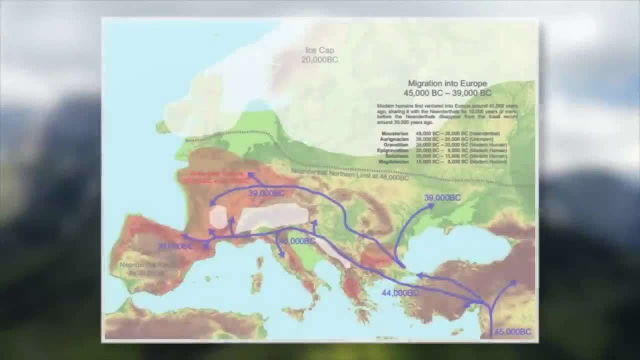 Though this may all sound confusing, the larger picture is that Sapiens migrating into Western Europe brought with them new technology that mixed with other technologies of the region. A 2022 study found that modern humans and Neanderthals co-existed in Western Europe for. 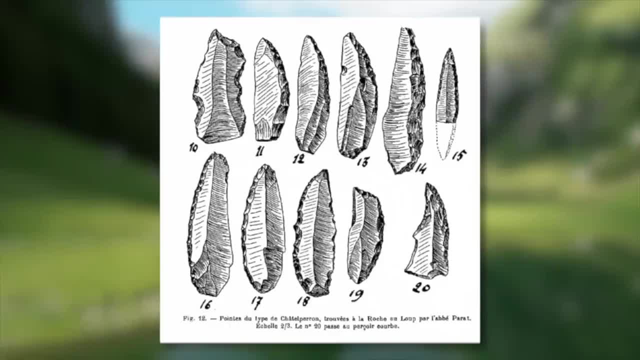 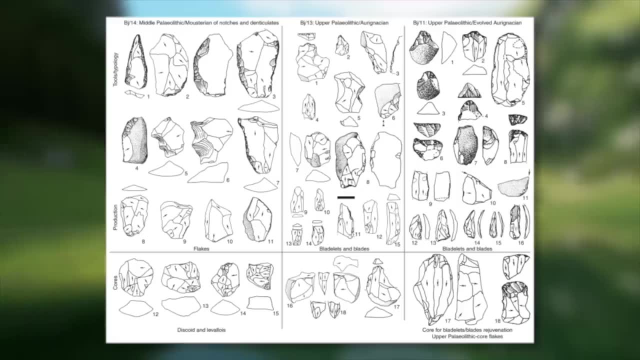 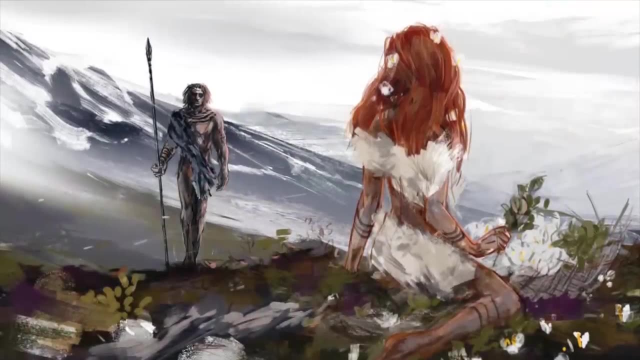 1400 years. This helps explain why the archaeological record is so confusing. Old ways of toolmaking adopted new techniques and eventually it appears that the new techniques were favored by both Neanderthals and modern humans. The coexistence of these species. 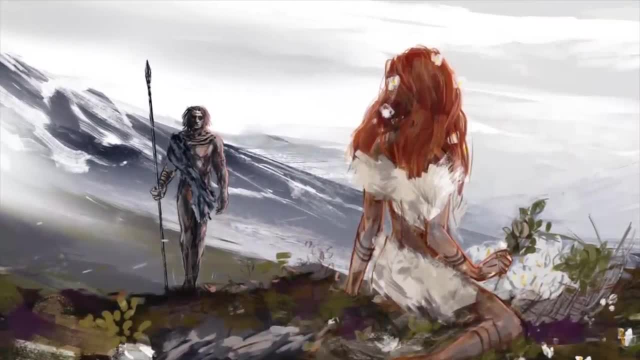 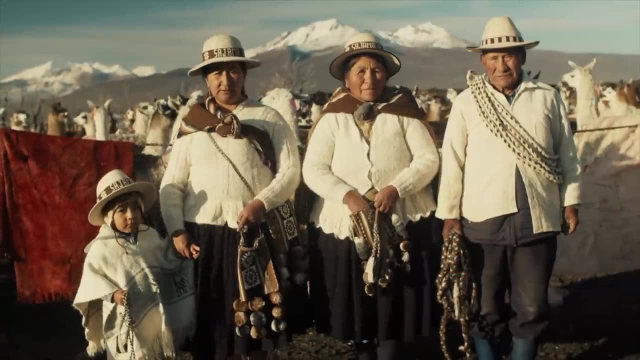 undoubtedly included centuries, if not millennia, of hybridization. We know that hybridization occurred because all modern humans have Neanderthal genetics, but we will talk about this later. Besides this fact, our remains from this period clearly show that they were hybridizing. 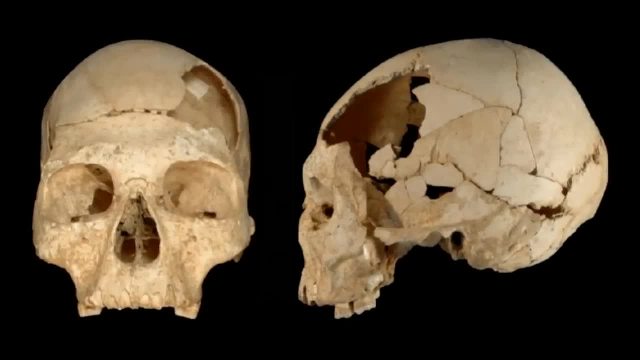 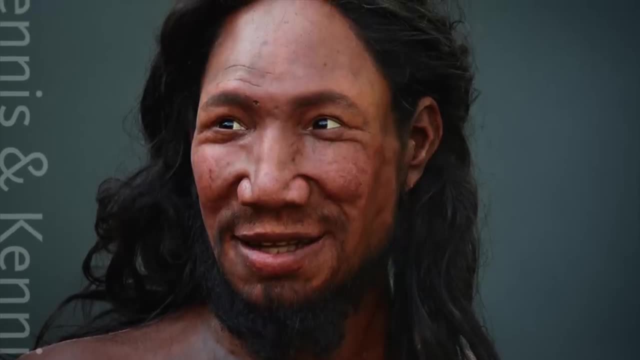 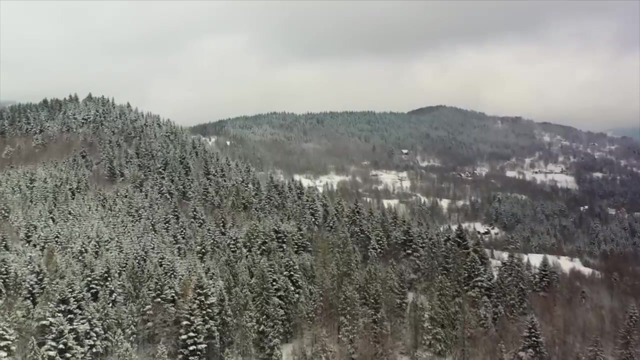 The 40,000 year old Oace 2 from Romania was found to have 6-9% Neanderthal DNA. This suggests that he had a Neanderthal ancestor only 4-6 generations earlier. With this example, you must keep in mind that by 40,000 years ago, Neanderthals were already on. 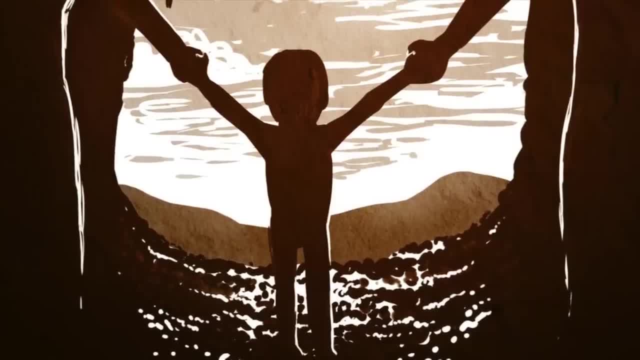 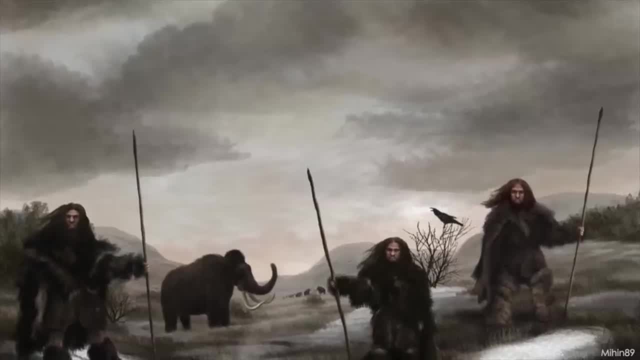 the brink of extinction. When considering the initial periods of intermixing, for example, Neanderthals were already on the brink of extinction. First-generation hybrids would have been much more common. Neanderthal populations across Western Europe seemed to decrease drastically after around 43,000 years ago. The reason for their decline is not entirely understood, but it certainly had to do with their population size. Neanderthal population size fluctuated mainly based on warmer times, though after about 100,000 years ago their populations began to decline regardless of modern humans. The reason for this? 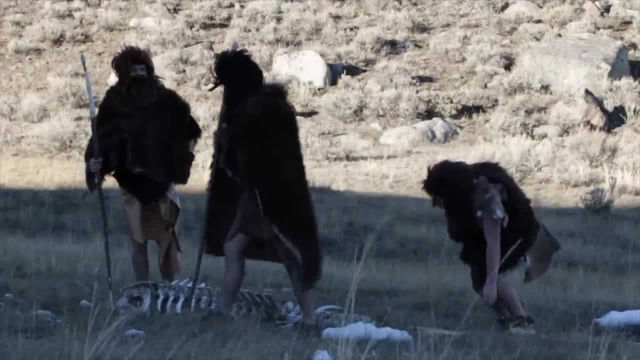 decline is that Neanderthals were not as large as they used to be. Neanderthal populations were not as large as they used to be. Neanderthal populations were not as large as they used to be. This does not seem to have to do with competition with modern humans, as it started before they even 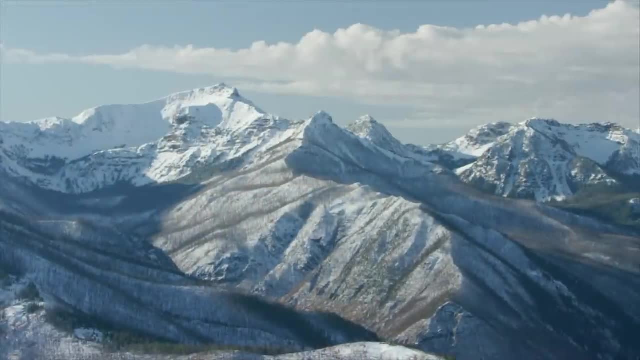 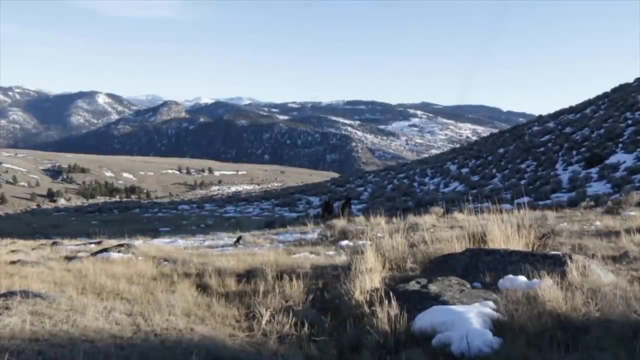 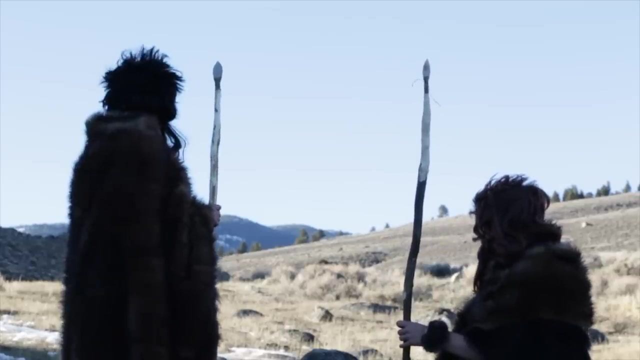 appeared on the landscape. Even when modern humans entered Europe, there were plenty of resources to go around. Both Neanderthals and early modern humans would have been rare on the landscape. Their decline instead seems to be tied to low fertility rates and assimilation. Neanderthals- 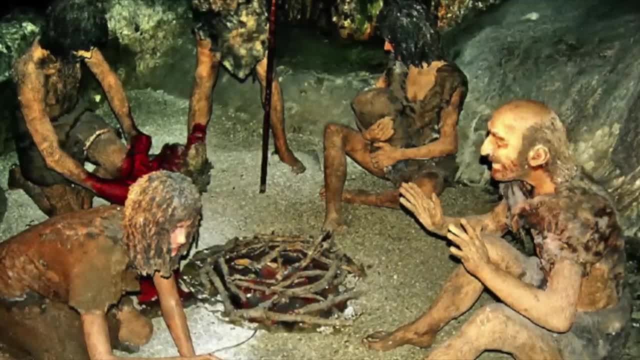 seem to have suffered many negative effects due to having low genetic diversity. The mitochondrial genes of Neanderthals and Neanderthals seem to have suffered many negative effects due to having low genetic diversity. The mitochondrial genes of Neanderthals and Neanderthals seem to have 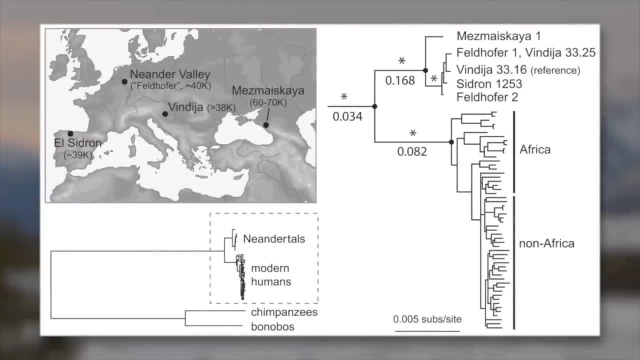 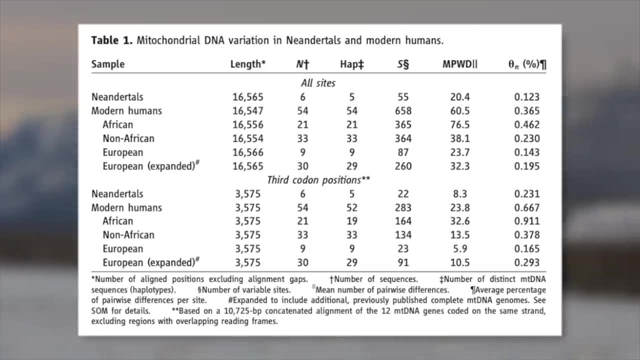 many negative effects due to having low genetic diversity. The mitochondrial genes of Neanderthals from across Europe only differ at 55 locations out of more than 16,000 locations. They had about three times less mitochondrial diversity than in modern humans. This resulted in the proliferation of harmful gene variants which may be tied to their low fertility rate. It appears that Neanderthals were already having a hard time when our new innovative species moved in. It didn't help that our population seemingly had a much higher fertility rate than Neanderthals. Our population seemed to have swelled as much as tenfold around. 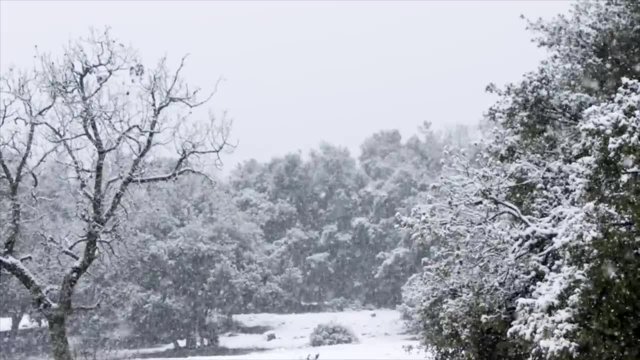 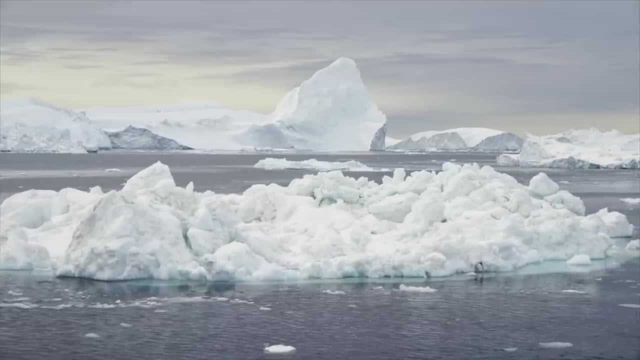 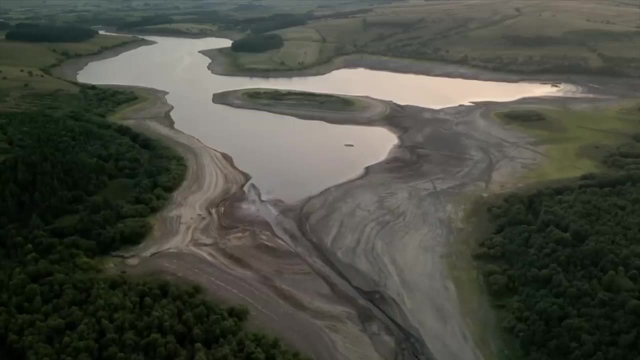 40,000 years ago. This may be tied to the onset of the Heinrich 4 event, which also occurred during this time. A Heinrich 4 event is caused by ice breaking off from glaciers in the Atlantic, which causes extreme seasonality. These conditions included drought-ridden summers and frigid. 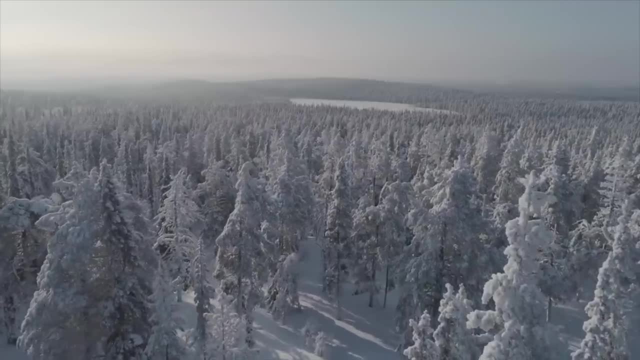 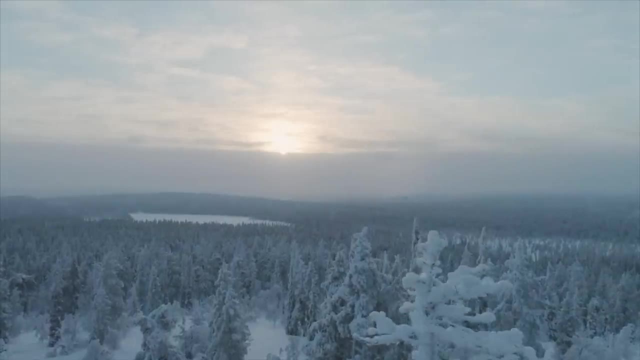 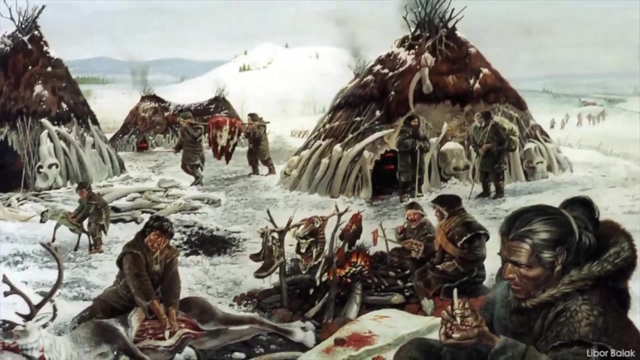 winters. The periods lasted for centuries. Neanderthals had survived a few of these events before, though their populations had decreased in prior Heinrich events. However, this time, Homo sapiens were there. Sapien populations appear to have done very well during this period, perhaps because of their technological or social organization, Though you must keep in mind that this population had significant Neanderthal genetics and even peer-bred Neanderthals. As OAC1 shows us, many modern humans were able to survive a few of these events, though their populations had decreased in prior Heinrich events. 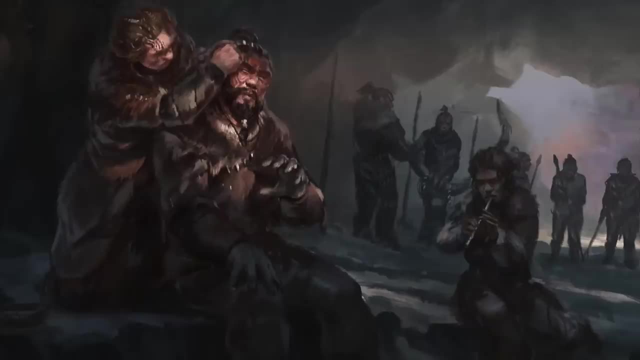 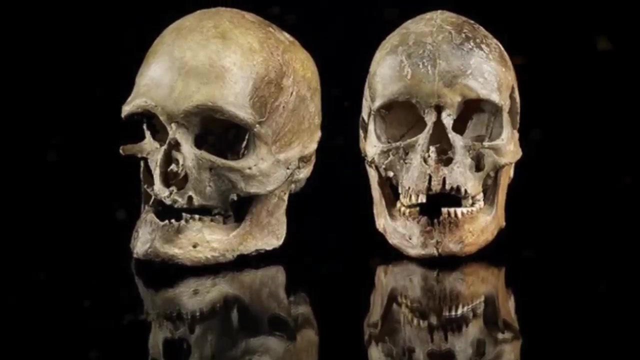 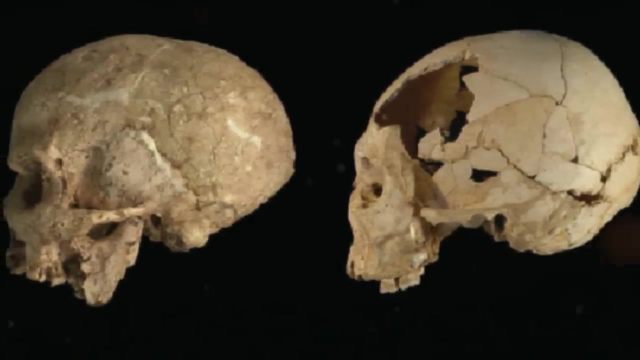 Neanderthals would have had a significant amount of Neanderthal DNA and may have even had full Neanderthals in their group. Early European modern humans at large display many features that are reminiscent of Neanderthals. Many had slightly flattened skull caps and prominent occipital buns, as well as heavily 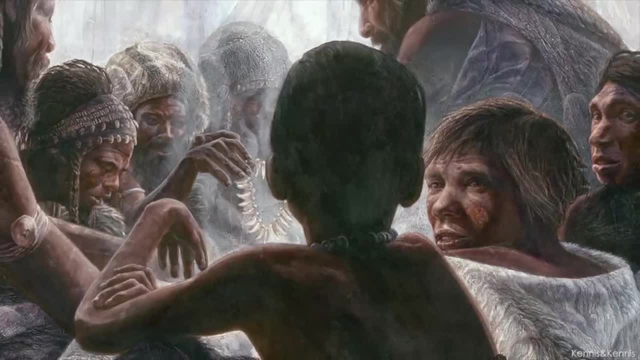 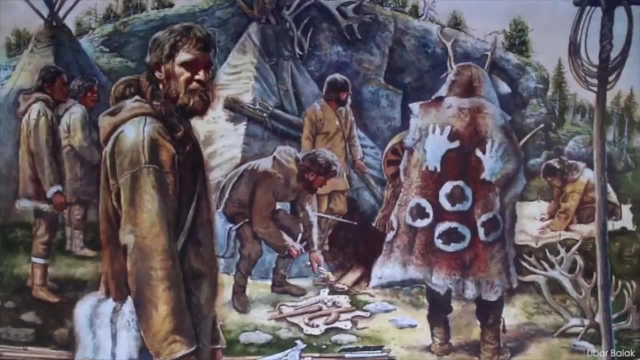 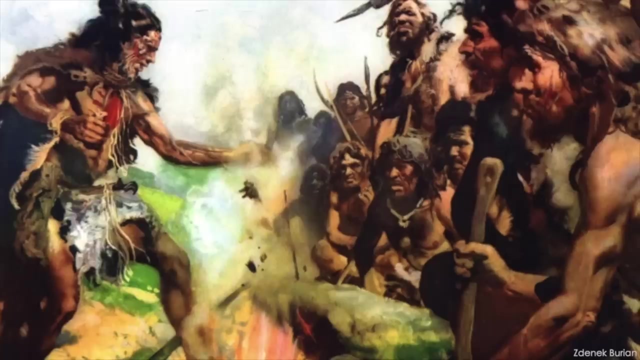 built skeletons. The frequency of these features in early populations suggests that interbreeding was much more common than once thought. These features would persist for tens of thousands of years, though they significantly diminished throughout the upper paleolithic. It appears that many Neanderthal genes were eventually naturally bred out of the population throughout. 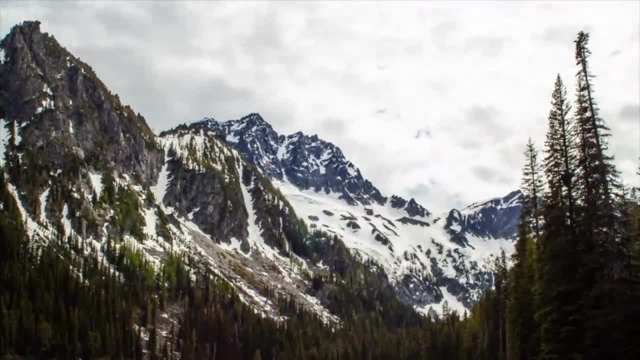 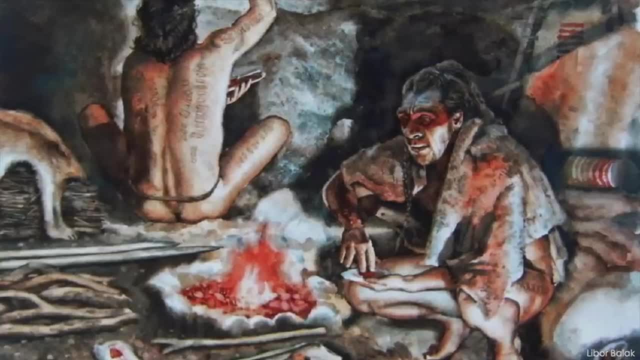 time. Some of these genes were initially quite harmful, though others may have helped these newcomers adapt to the European environment. When considering the disappearance of Neanderthals, we must understand that it was a very long process. Neanderthals appear to have been. 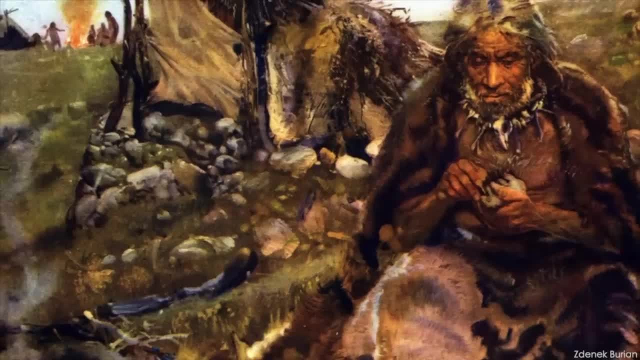 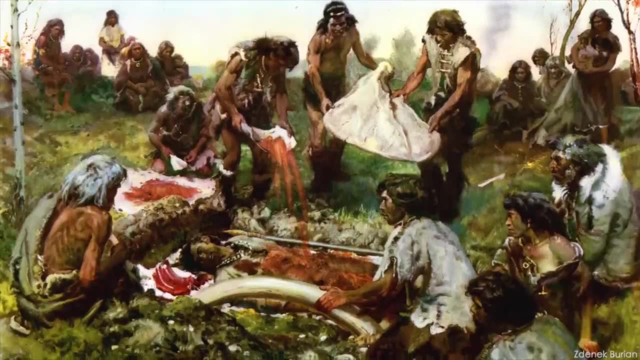 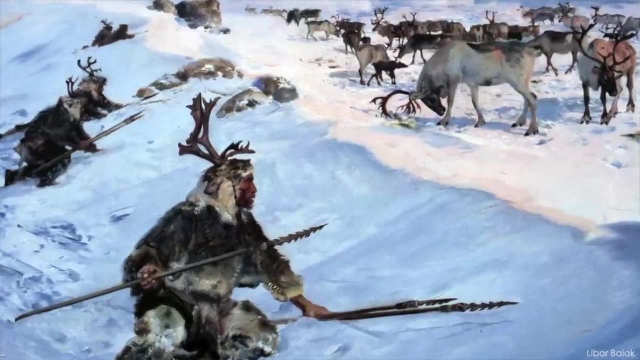 more or less bred out of existence. Many of their genes were initially bred out of the population. Many of their populations were simply assimilated into our own populations. Their genetics in subsequent hybrid populations were watered down by the more numerous Homo sapiens. Other groups of Neanderthals may have been outcompeted for food resources by 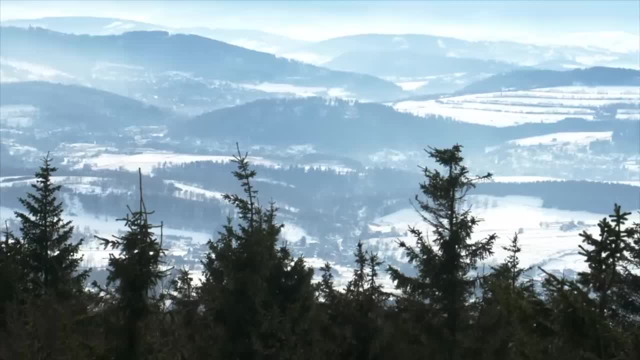 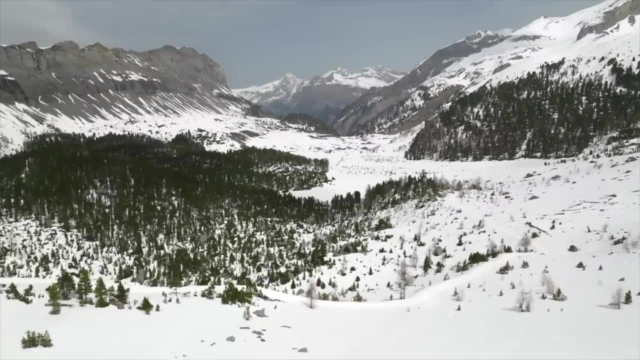 groups of sapiens or hybrid groups. However, remember that Europe is a big place and it was underpopulated during this time. There would have been plenty of room for many of these groups to coexist. Still, the Neanderthals were not the only ones who were bred out of the population. 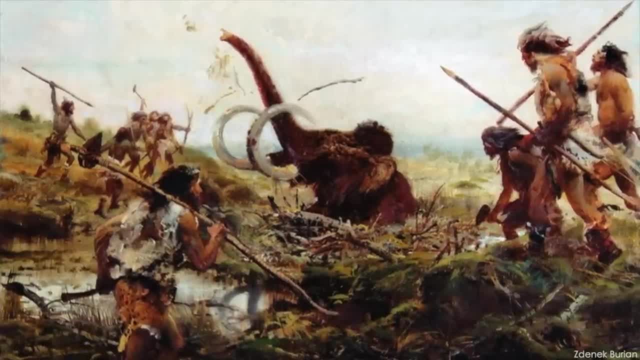 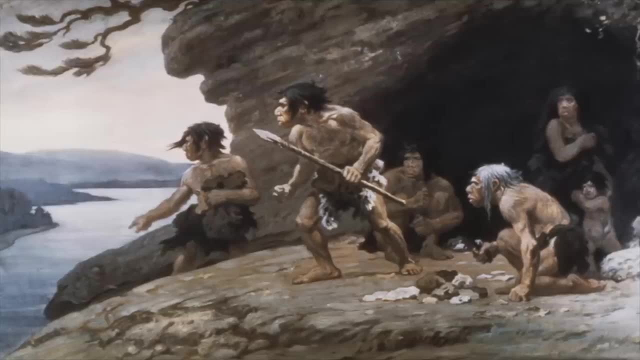 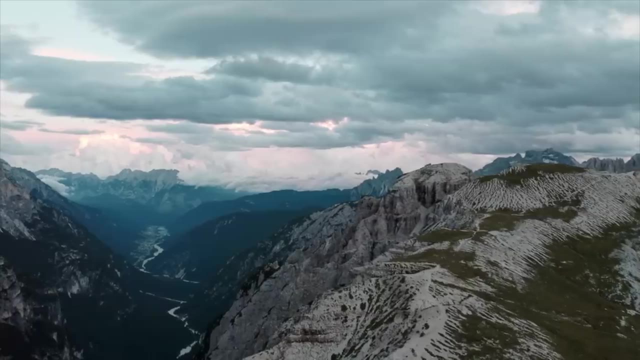 Some of the groups of Neanderthals were outcompeted or perhaps, in rare occasions, even targeted for violent attacks. Another aspect to consider about their extinction is: when did the last true Neanderthals actually go extinct? The Neanderthal range is full of isolated, hard-to-reach. 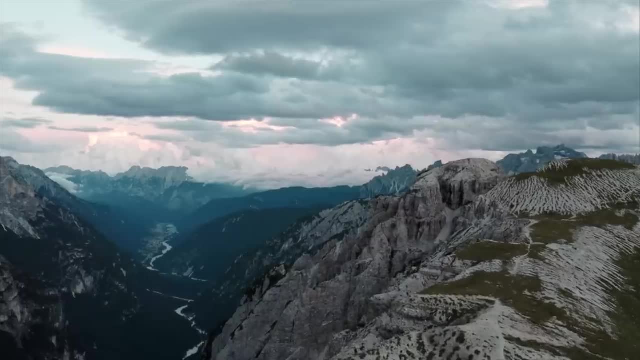 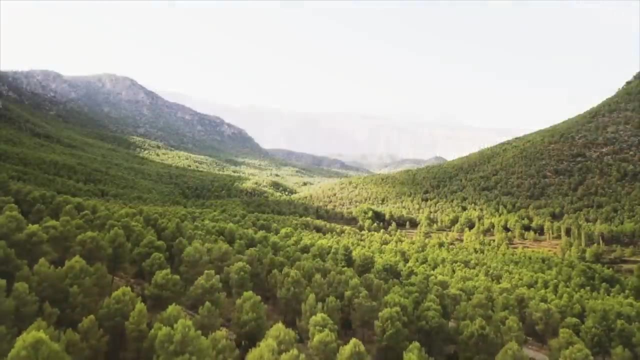 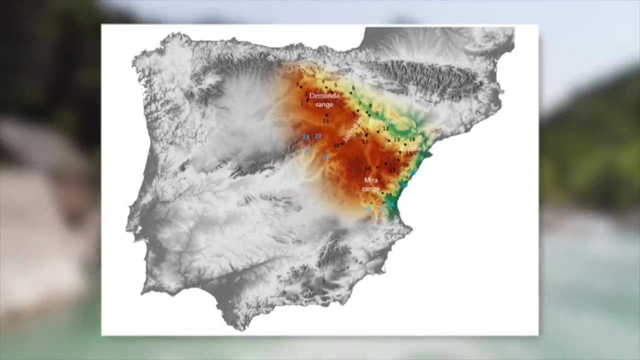 areas that could have harbored Neanderthals for much longer than mainland Europe. Even the entire Iberian Peninsula seems to have remained isolated from sapien dispersion. It has been hypothesized that the Ibro River in northern Spain may have been a formidable 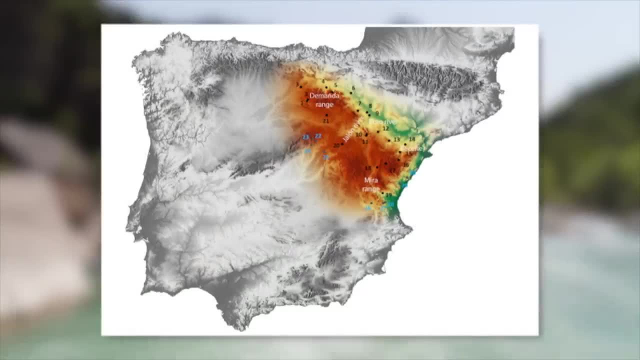 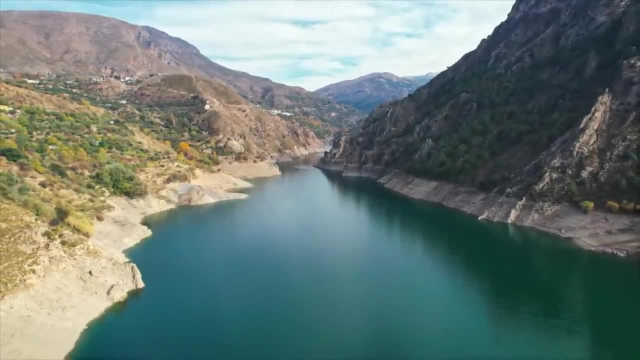 geographical barrier for sapien populations. Re-evaluations of sites suggest that sapiens may have been able to cross the river even over 42,000 years ago, though Neanderthal populations may have still remained in isolated areas throughout Iberia post-40,000 years. ago, Most purebred Neanderthals were already absent from western Europe. However, some Neanderthal populations may have been able to cross the Iberian Peninsula even after 40,000 years ago. Some Neanderthal populations may have been able to cross the Iberian Peninsula even after. 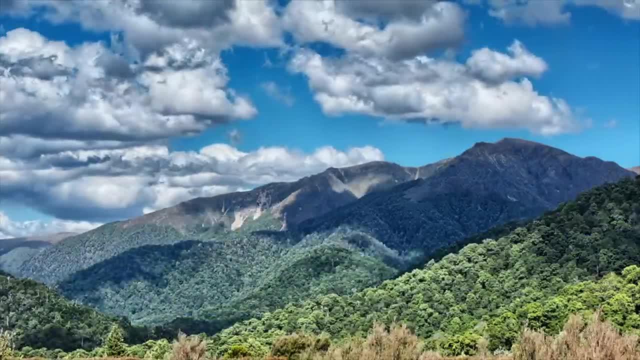 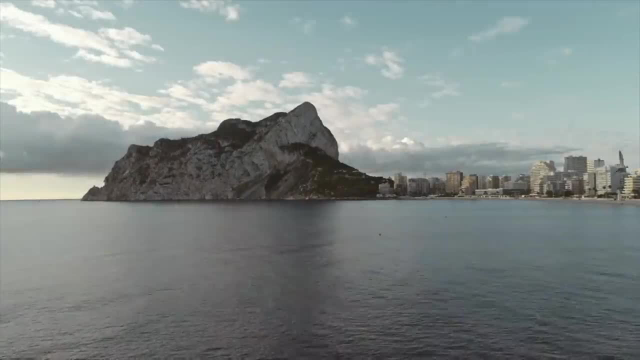 41,000 years ago. Most purebred Neanderthals were already absent from southern Europe at this time and whimpered to virtually nothing in the next thousand years, Though Neanderthals in Gibraltar may have survived much longer, possibly as late as 30,000 years. Though the 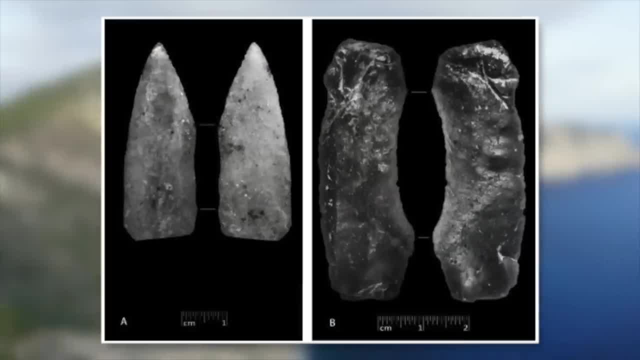 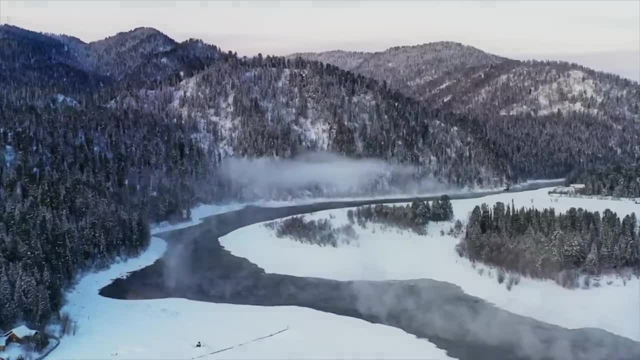 evidence for this is based upon unusual artifacts and climatic patterns rather than direct dating. Populations anywhere else may also have survived much longer. Maus, cunninganās種 Funker. animated monitored passes are predicted to now be in hand. Zimmermannnæo будуq sche 살아ittoli. 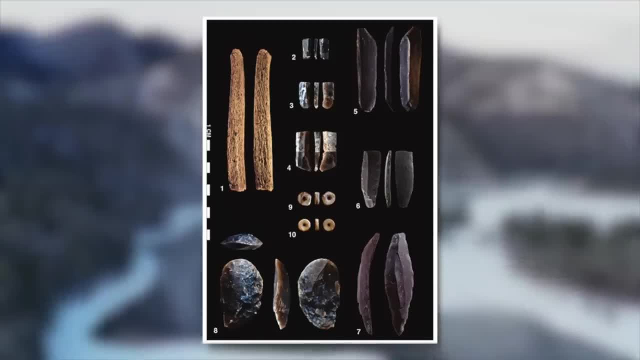 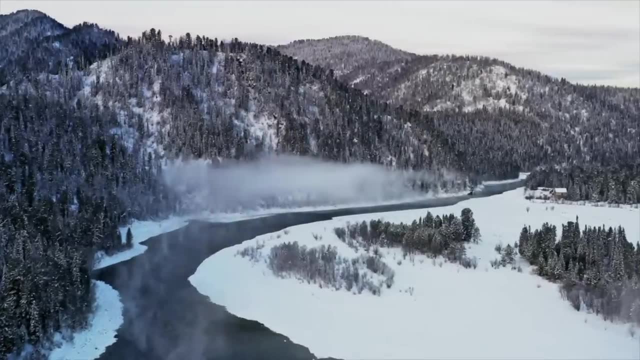 Most Mнал wiggle-tearing moose manner focused ciao-sp browser in northern Siberia may represent late-surviving Neanderthal population. Though these tools could have been made by sapiens as well. More direct evidence would need to be found. Neanderthal populations living in Central or 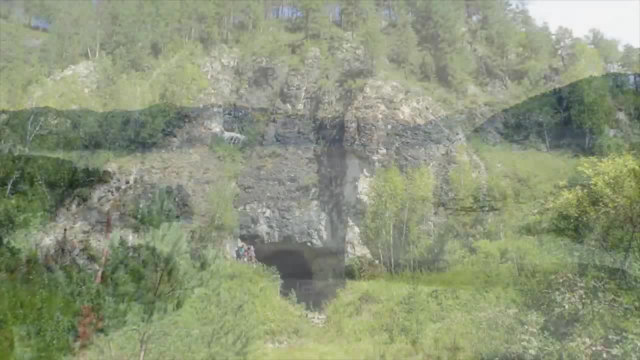 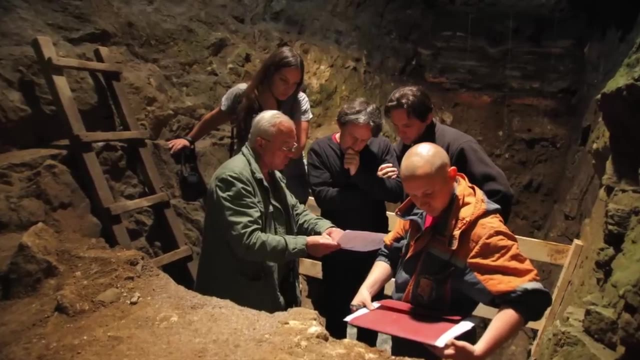 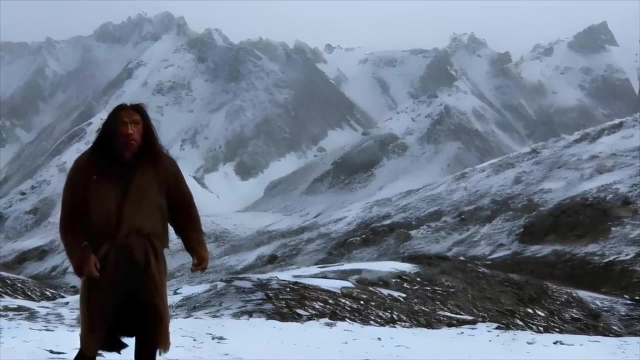 Eastern Asia may have been some of the last. Though Neanderthals have only been found as far east as Denisova Cave, they may have been more widespread in the region than the fossils suggest. Overall, it is clear that no exact date can be given for the extinction of purebred Neanderthals. By around 40,000 years ago, Neanderthal populations were nearly non-existent and any evidence after 37,000 years ago is very rare and often controversial. The last Neanderthal likely took their last breath in some remote mountain refuge, perhaps surrounded by a family. 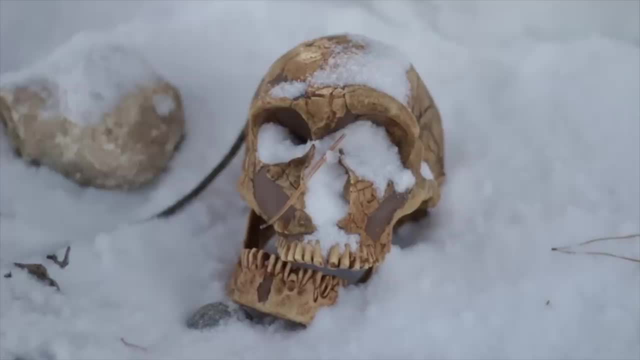 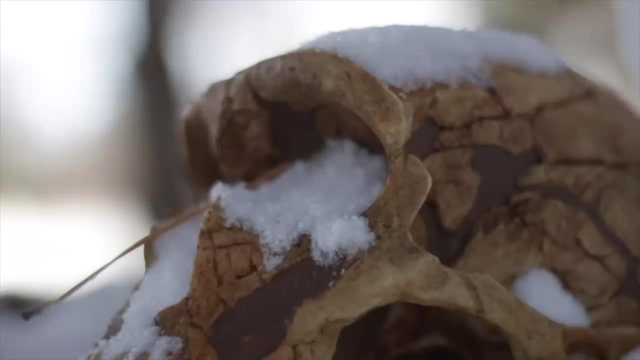 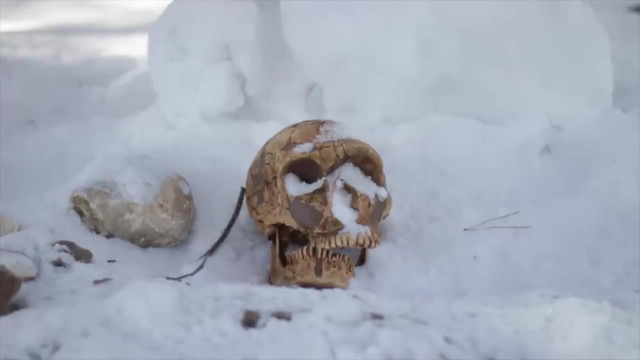 of hybrids and sapiens, Subtitles by the Amaraorg community. The picture of Neanderthal extinction I have laid before you is one of assimilation, infertility and gradual decline. This picture is supported by much more evidence than sensationalist claims that Neanderthals went extinct because they couldn't hunt this or that, or because their 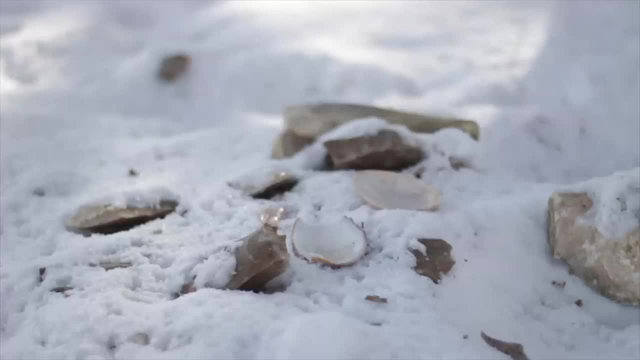 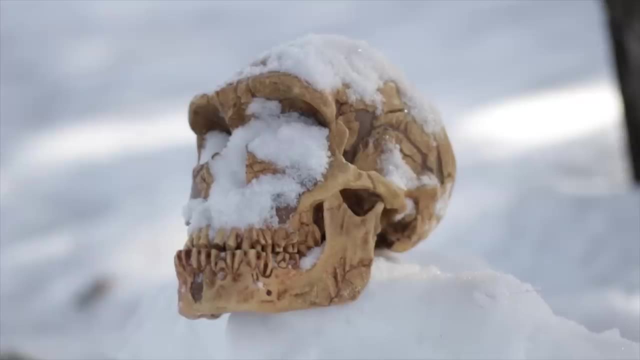 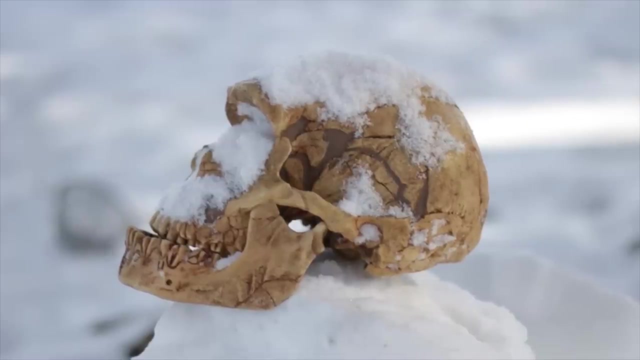 technology was not as complex as some other Paleolithic technologies. There are many reasons why Neanderthal populations may have been suffering, such as diseases or unfavorable changes in the climate, but the larger picture is that they were essentially absorbed into modern human populations. It could be said that Neanderthals as a species were less innovative. 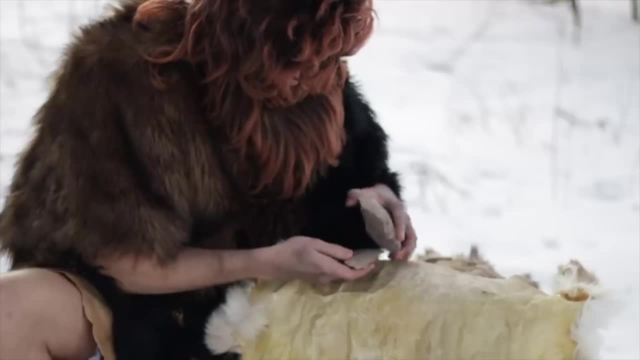 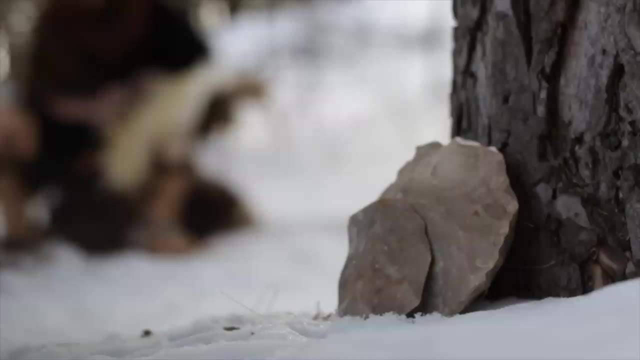 than Homo sapiens, though there are many nuances involved in this assessment. Neanderthal technology did appear to stagnate for tens of thousands of years, though we can only really assess their stone technology. We do not know exactly what kind of advancements were being made. We are aware that Neanderthal cultures adapted to different conditions, such as the reindeer hunters of the quinoa Neanderthals, but their technology did not actually advance. It was just utilizing similar techniques in a different way. Homo sapiens, on the other hand, did appear to improve their technology more. 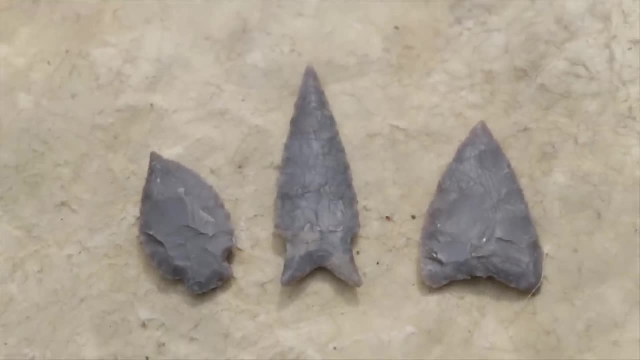 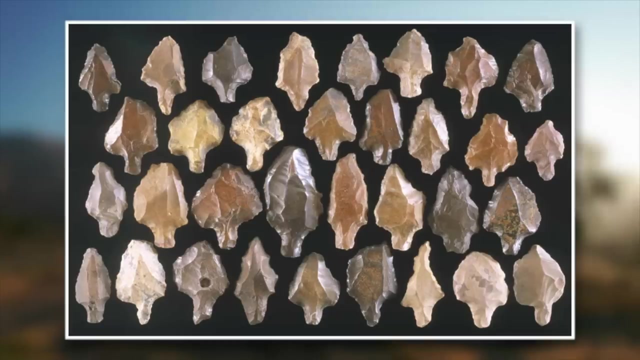 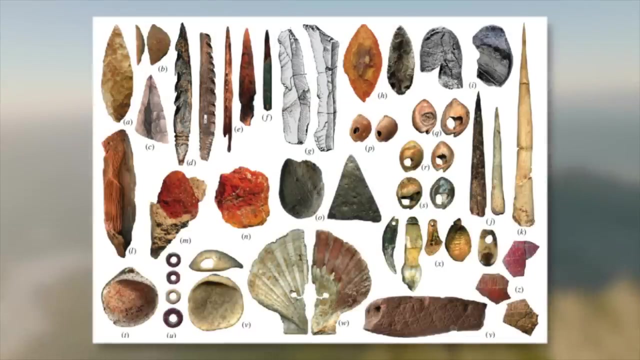 frequently during the past 100,000 years. Sapiens living in North Africa over 100,000 years ago began to produce light tanked points which may have sat at the tip of projectile weapons Around the same time, sapiens in Central and South Africa were creating complex bone and stone. 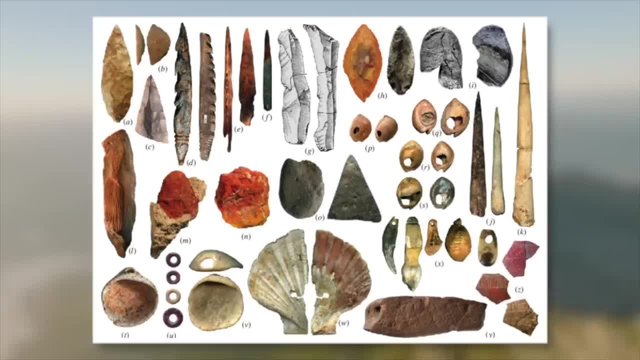 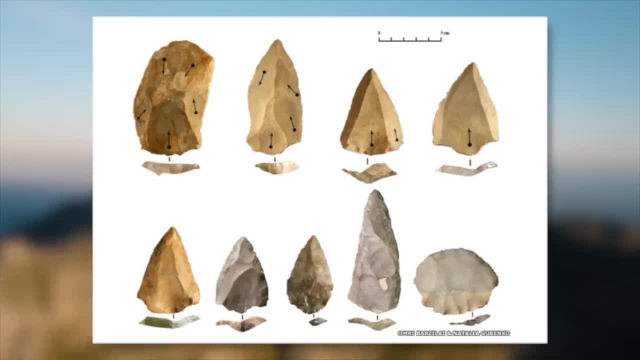 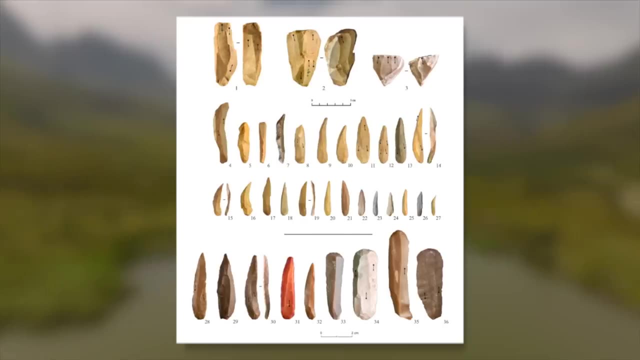 tools such as the Katanda harpoon. Further developments would happen in the Middle East, such as Levawa points being retouched to create objectively better Amerian points. Other tools from the Amerian culture display a high level of complexity and only appear to have been made by modern humans. Though, before we get ahead of ourselves, we must 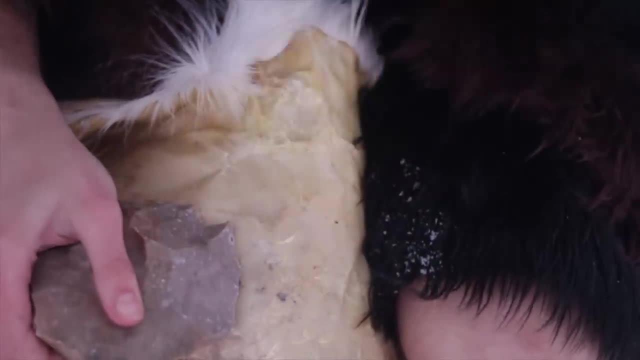 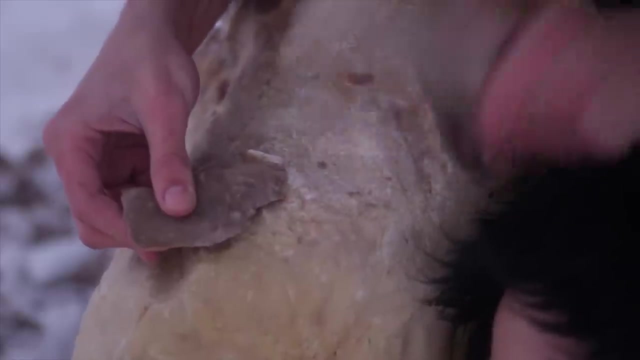 identify that Neanderthals, during this time, were also beginning to make more complex technology, Though they still utilized mousterian technology. bifacial points of considerable complexity were being made, such as the leaf shaped points found at Hull Felz and other sites. 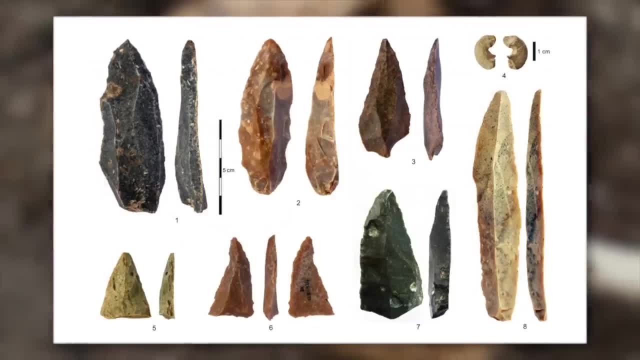 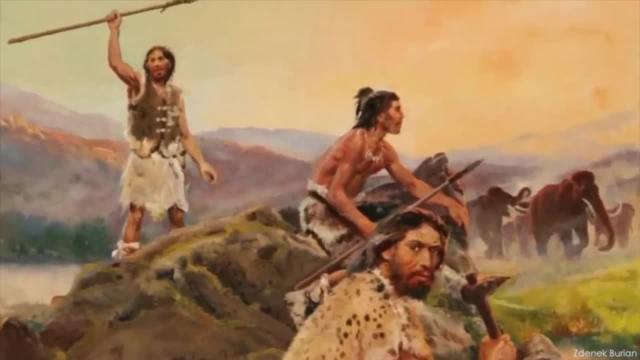 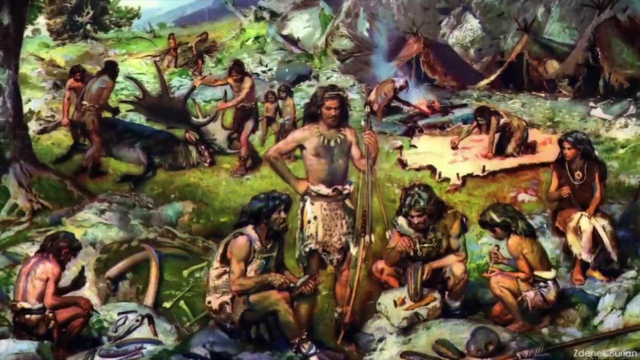 The point is: just when modern humans began to make technological breakthroughs, Neanderthals were on the verge of extinction. Technological innovation is largely based on population size. The more individuals there are, the more likely that new ideas and methods will emerge. 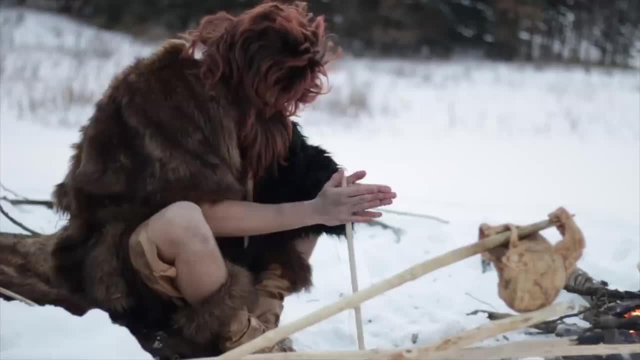 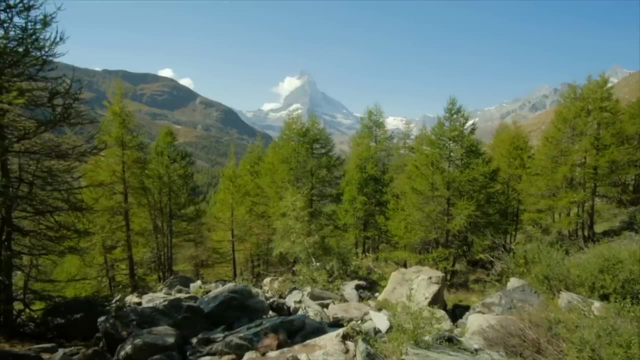 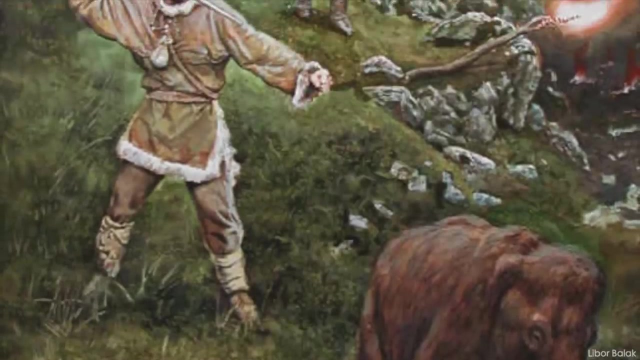 Since Neanderthal populations were always quite low, their ability to innovate also remained quite poor, Though, after Sapiens moved into Europe, interbred with Neanderthals and expanded their populations, innovation became much more common. This period is called the Upper Paleolithic. 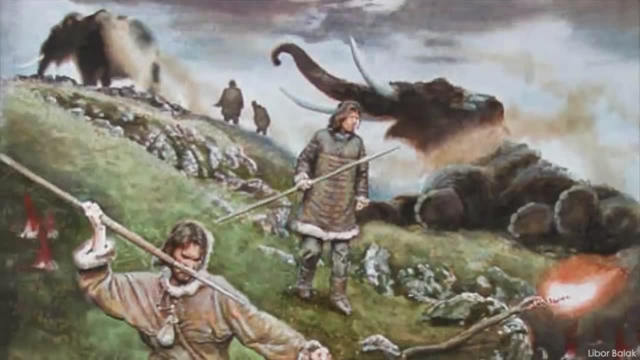 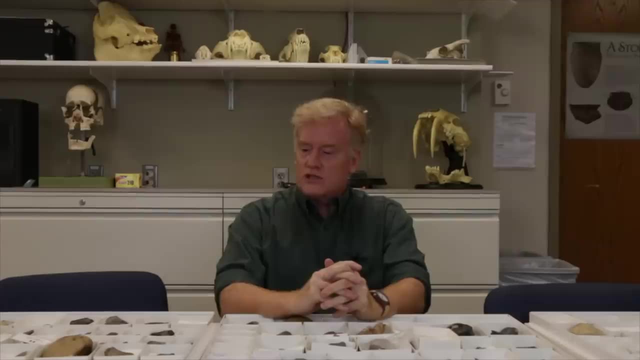 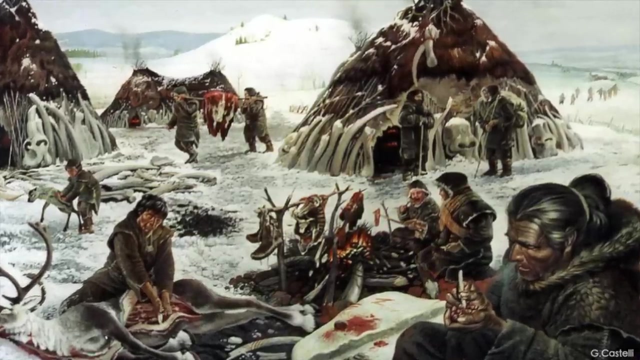 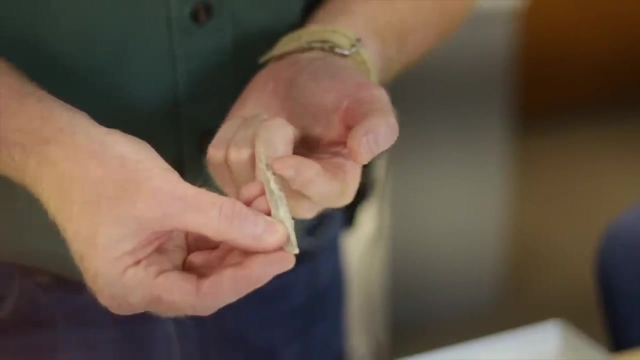 Regional stone tool industries appeared with art and complex culture. The Upper Paleolithic is something that the culture changes quickly, So we can talk about every eight to ten thousand years. we can recognize a different Upper Paleolithic cultural entity where they make different stone tools, they make different bone tools, different forms of art. 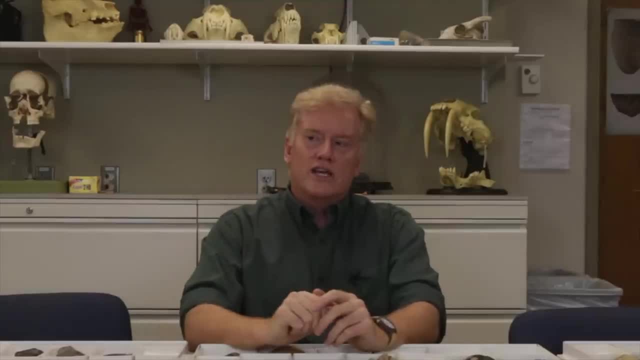 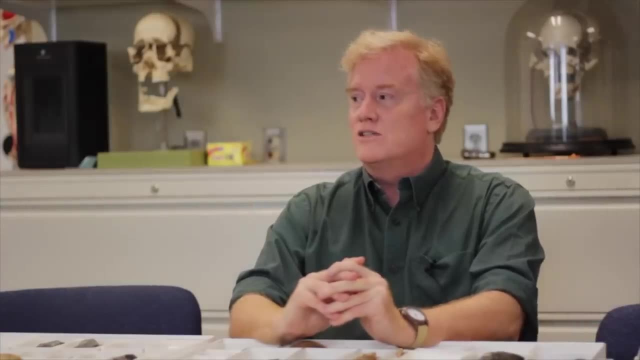 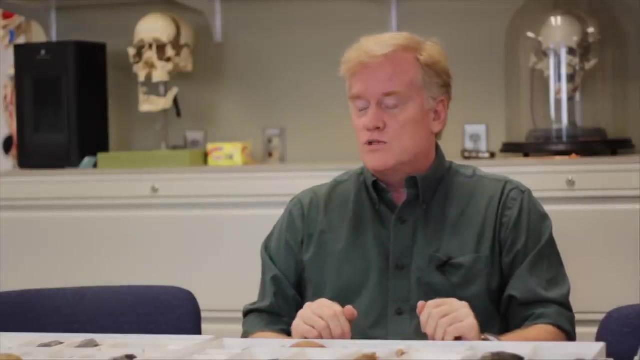 and they change every five to ten thousand years, Whereas Neanderthals have the same access to the same resources and they did not change at that rate. Things didn't go viral across, let's say, Eurasia, or at least Western Europe, to Central Europe, which we see with modern humans in the Upper. 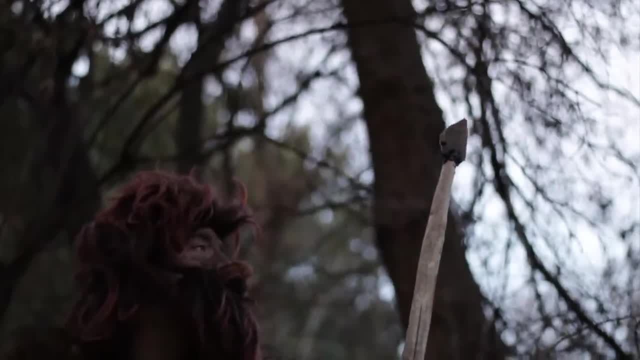 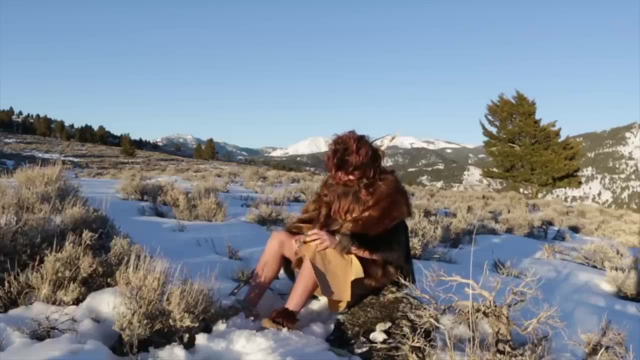 Paleolithic. It is easy to take in this information and simply think that Neanderthals were cognitively unable to advance as our species was. But you must consider that Neanderthal technology may have simply innovated over time. Neanderthal technology has been used for many, many, many, many years. 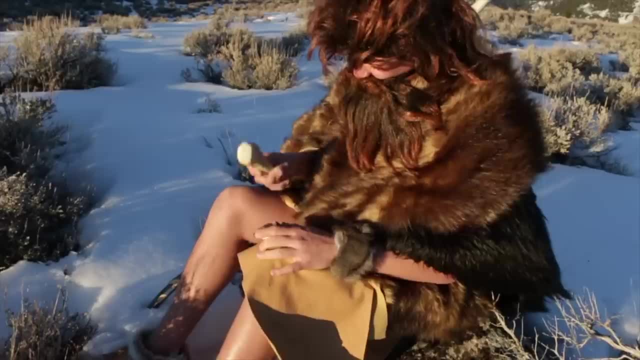 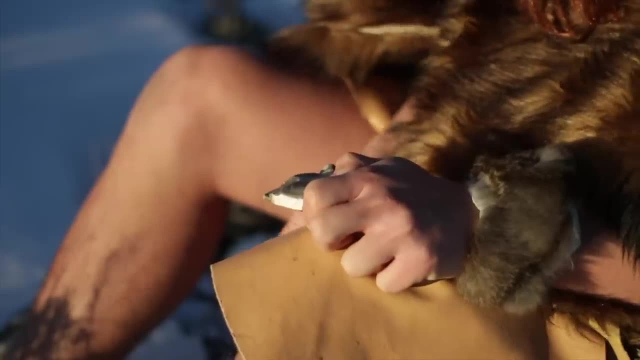 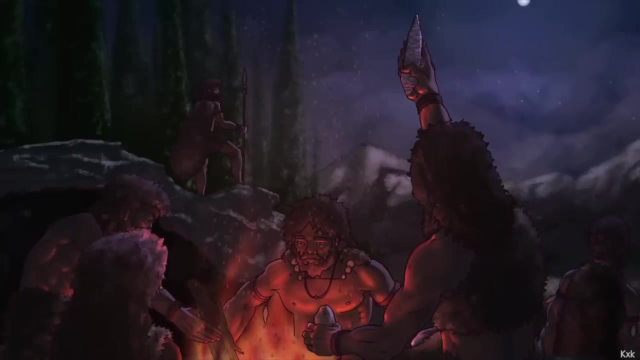 It is important to identify that our own ancestors were living with relatively similar technology to Neanderthals for hundreds of thousands of years before gradually innovating and expanding around the world. It therefore may have been our culture which propelled us forward, rather than our anatomy. 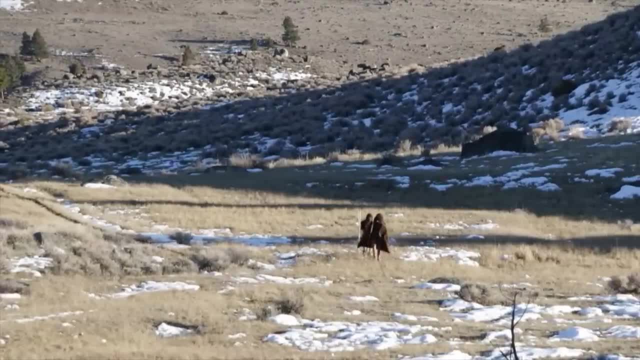 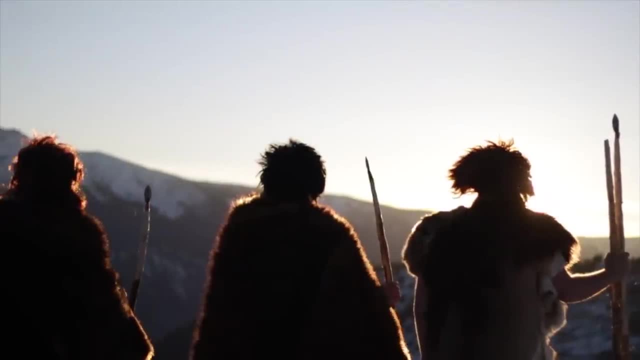 Neanderthals were certainly able to survive with their anatomy, but their culture stagnated and was assimilated and replaced. Neanderthals were able to survive with their anatomy, but their culture stagnated and was assimilated and replaced. If the dice rolled differently, it very well could have been Neanderthals that expanded around the 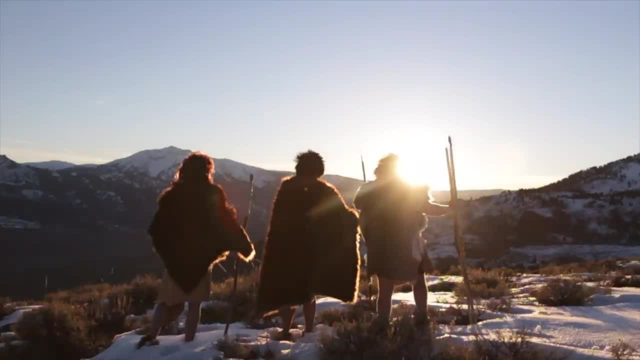 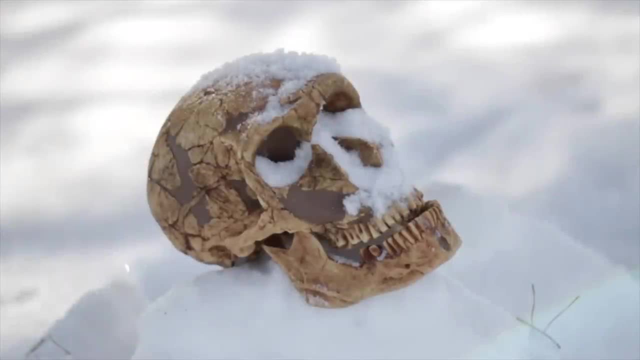 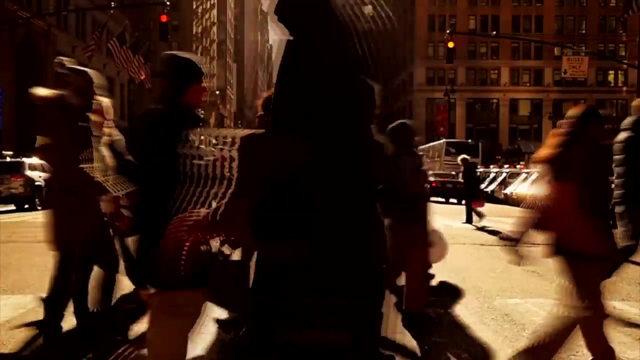 world. After all, we are both just descendants from the same common ancestors with a slightly different anatomy. Another question regarding their extinction is whether we can truly even consider them extinct at all. Neanderthal genetics exist in every modern human population alive today. Though Neanderthals primarily lived in Europe and parts of Asia, their genetics can be. 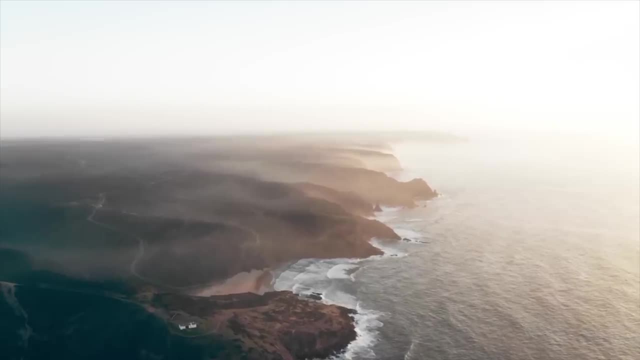 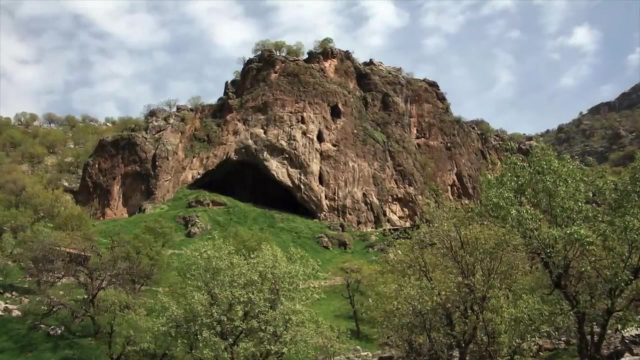 found all over the world. This is, of course, because any population of modern human outside of Africa had to pass through the Middle East and inevitably run into Neanderthal ancestry. It was once thought that populations of Sub-Saharan Africans did not possess Neanderthal genetics. 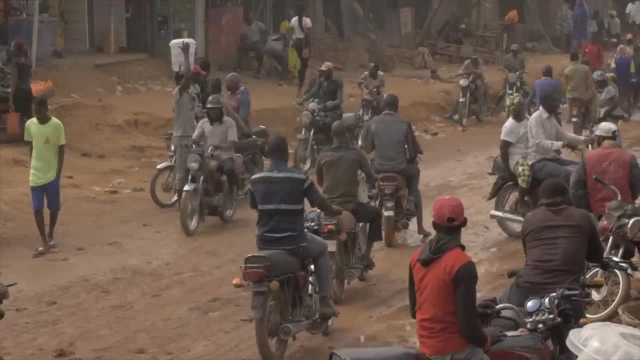 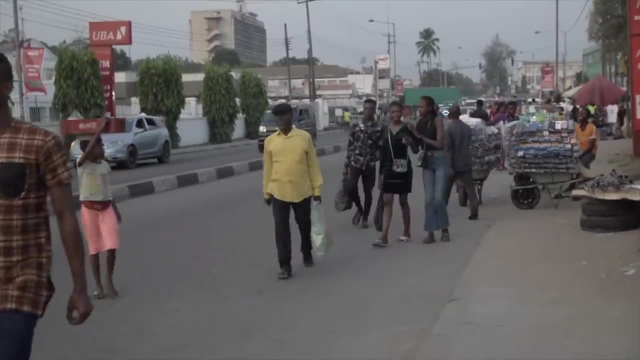 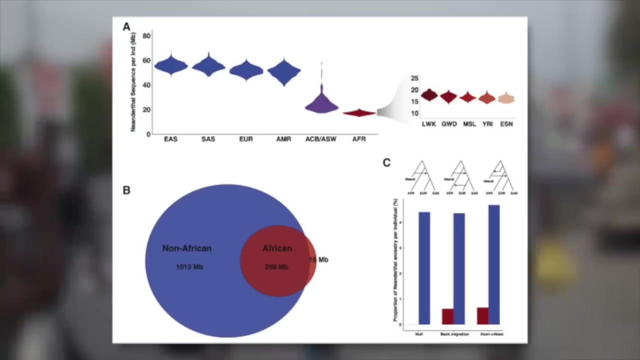 though this is found to be false. Recent studies have proven that every African population has some degree of Neanderthal DNA and, surprisingly, more than once thought. On average, African individuals have about 17 megabases of Neanderthal DNA, or 0.3% of their genome. These genes entered 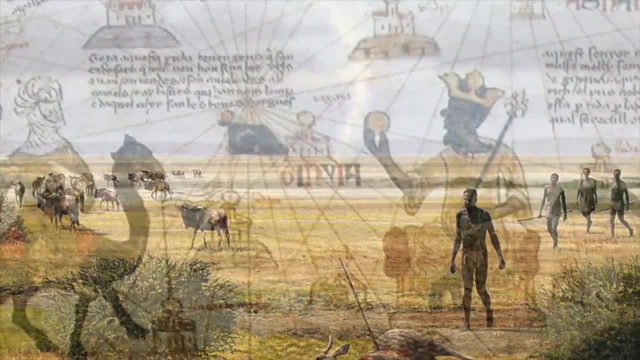 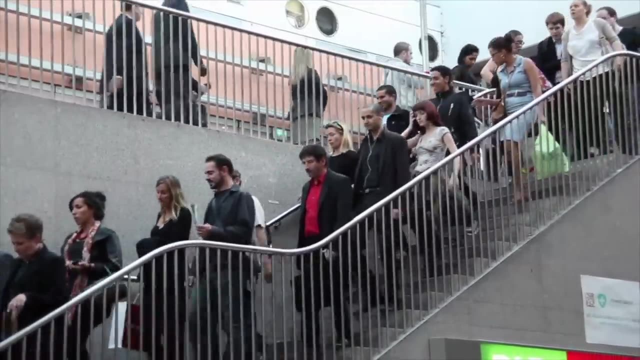 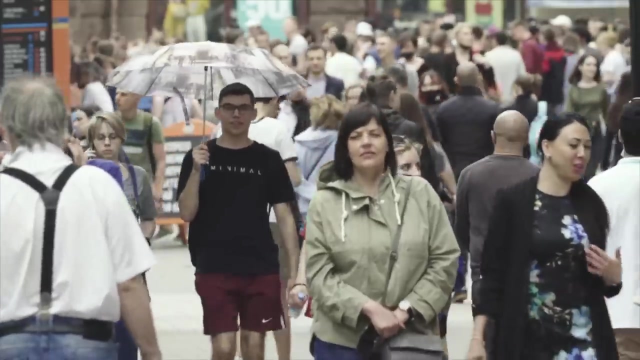 African genomes when populations migrated back into the continent, and also throughout prehistoric and historic periods. People throughout the rest of the world have comparatively more Neanderthal DNA. Despite the fact that Europe was the main home of Neanderthals, Europeans do not have the most. 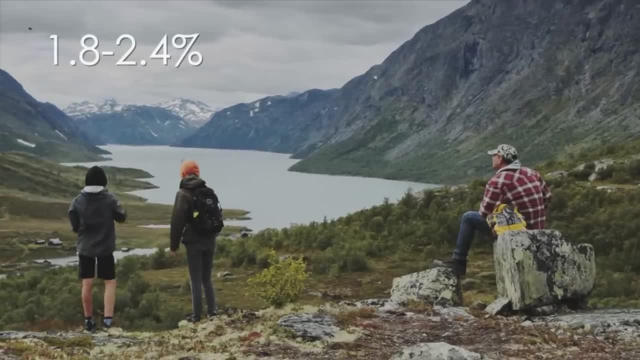 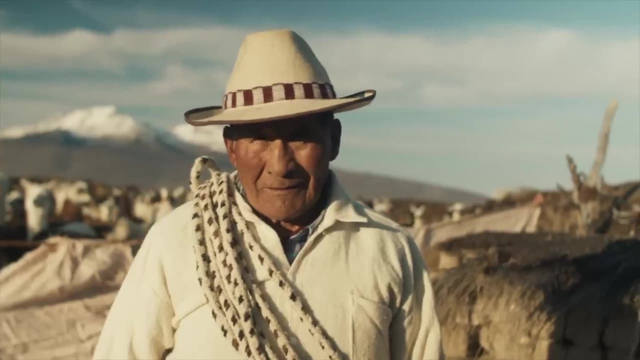 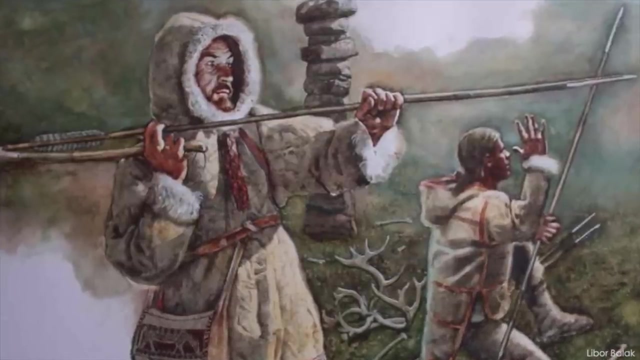 Neanderthal DNA. They have between 1.8 to 2.4% Neanderthal DNA, which is the largest Neanderthal gene in the world. While East Asian, Oceanian, Aboriginal, Australian and Indigenous Americans have between 2.3 to 2.5%, Pre-agriculture Europeans appear to have had similar levels. 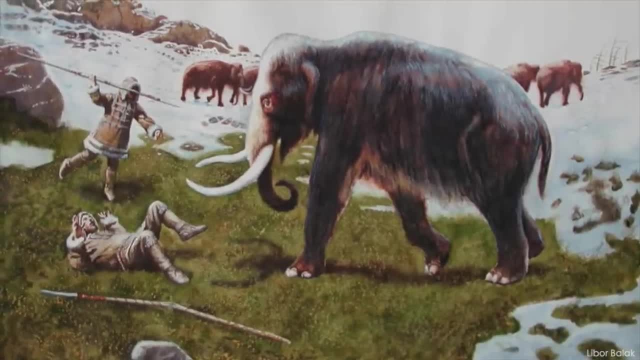 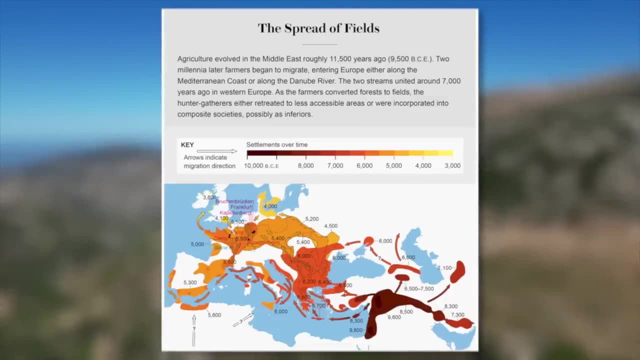 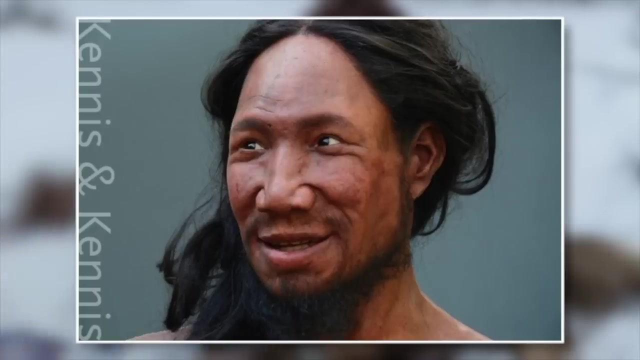 to modern Asians, but these levels have decreased with migrations. Interestingly, most modern European DNA actually comes from Western Asia and only spread to the region in the past 10,000 years. In fact, Boasi, the man with the recent Neanderthal ancestor from Romania, is more closely related to Americans and East Asians than 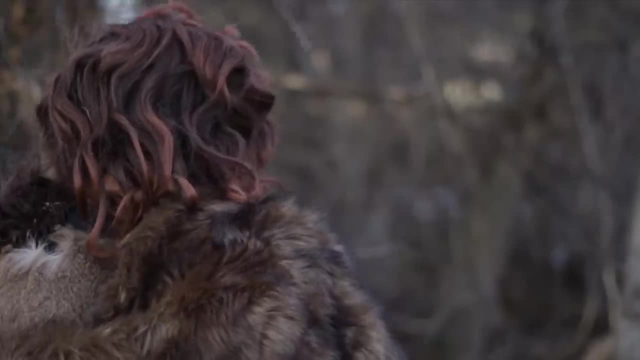 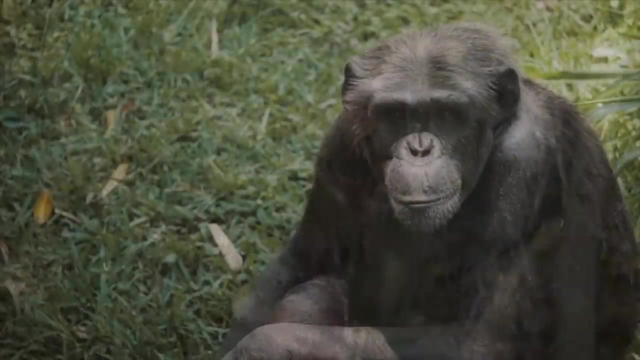 to any European, While it is clear that Neanderthal genes are present in all modern humans. but what does 2% Neanderthal DNA even mean? After all, don't we share 99% of our DNA with chimpanzees? 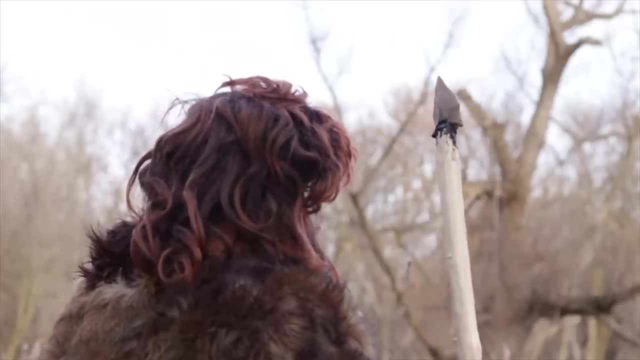 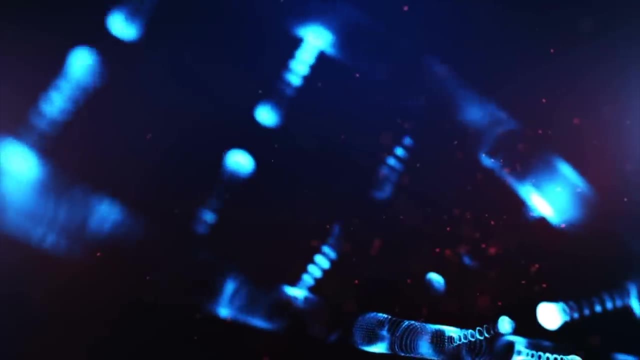 This is a question commonly asked in regards to Neanderthals and it is reasonable to ask. Between 95 to 99% of our DNA is in the same gene sequence. The other two are in the same relative position as chimpanzees. 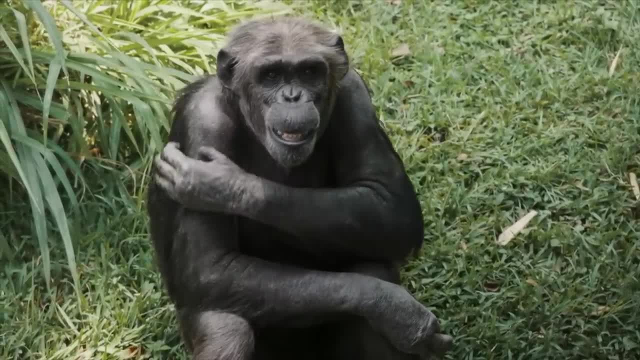 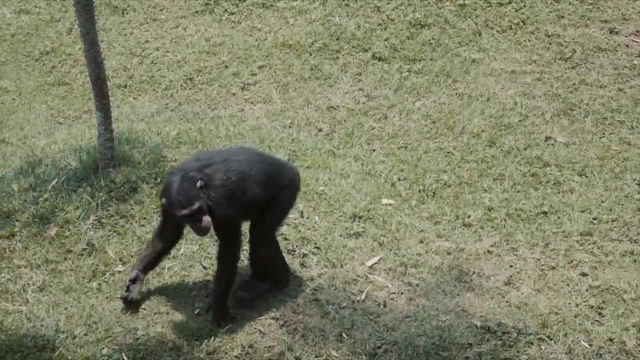 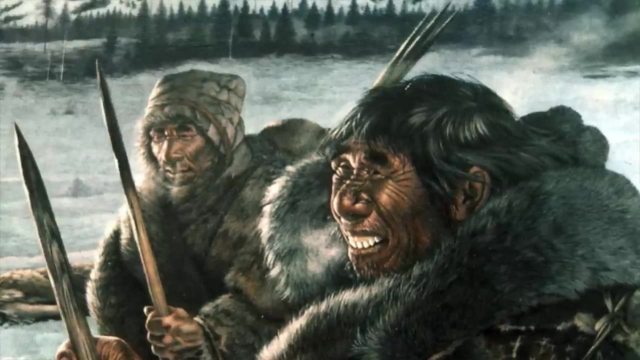 Though this calculation ignores some stretches of DNA not present in both species, Actual genetic similarity between chimps and humans can be calculated between 71 and 95%. Neanderthals, on the other hand, share about 99.7% of their DNA with us. 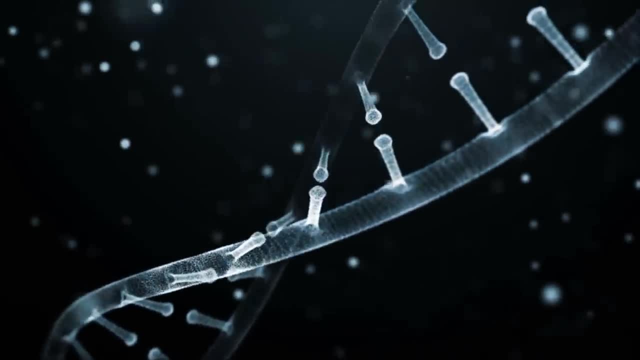 but only a few percent of our DNA is fully identical to Neanderthals as in the same genes in the same sequence. The other two are in the same relative position as chimpanzees, but only a few percent of our DNA is fully identical to Neanderthals as in the same genes in the same sequence. 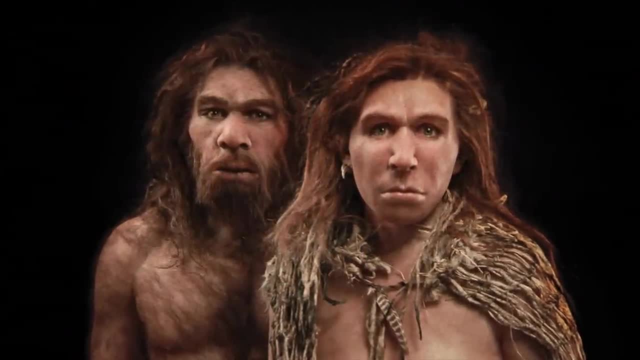 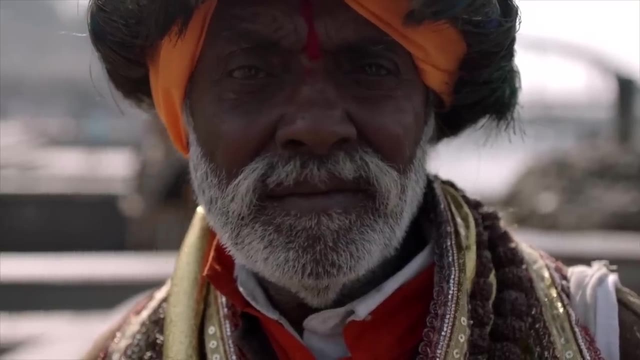 The other 97 to 99% of the human genome is still very similar to that of Neanderthals, though not identical. When considering how this affects modern populations, it is important to note that someone with 2 to 4% Neanderthal DNA only has about 0.006%. 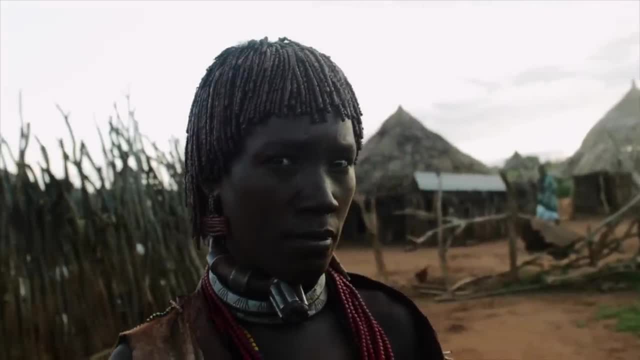 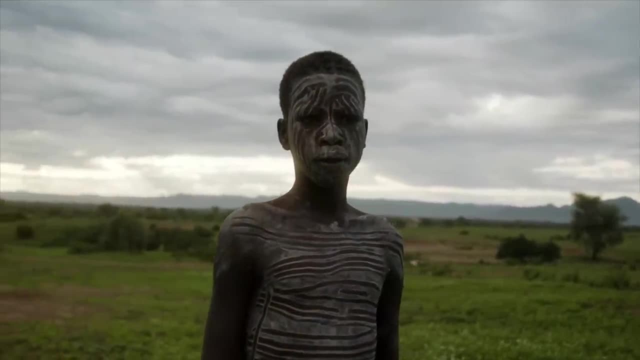 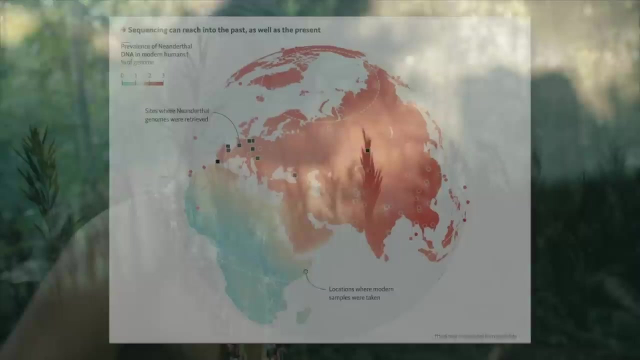 different DNA than someone with nearly no Neanderthal DNA. Eurasians and Africans do not primarily vary genetically based on Neanderthal ancestry. it is just a small part of their variation, And even their entire variation is genetically quite small. Populations across the world have similar levels of Neanderthal genetics, but they are not the same. 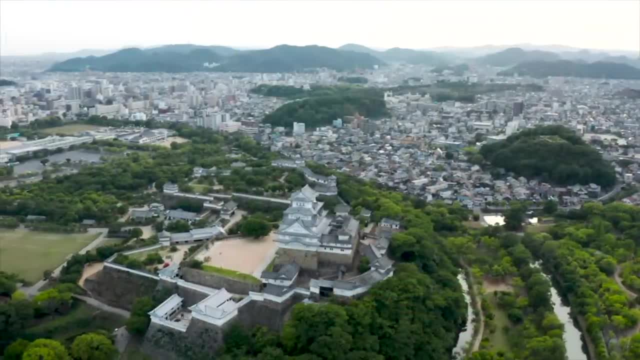 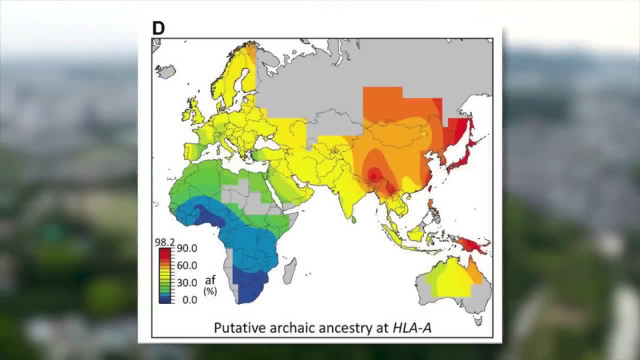 Neanderthal genetics in Europe differ from the genes found in Western and Eastern Asia. This is likely because of different Neanderthal populations, as was which genes were held onto. A gene that is useful in frigid Ice Age Germany may not be very useful in Tropical Thailand. Overall, it appears that Neanderthals have more genetic similarities than humans, And this is just one example. about 20% of the Neanderthal genome survives across modern human populations, meaning that around 20% of their genes were useful across our species and have survived into the modern day. 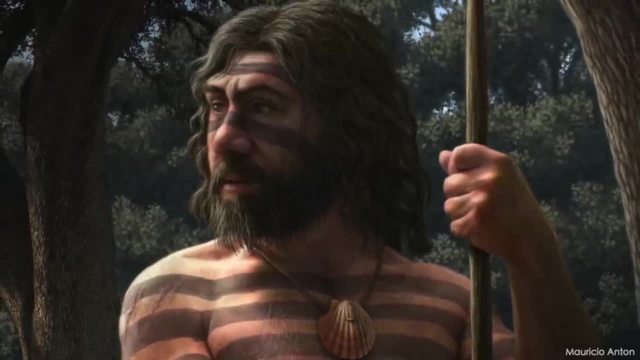 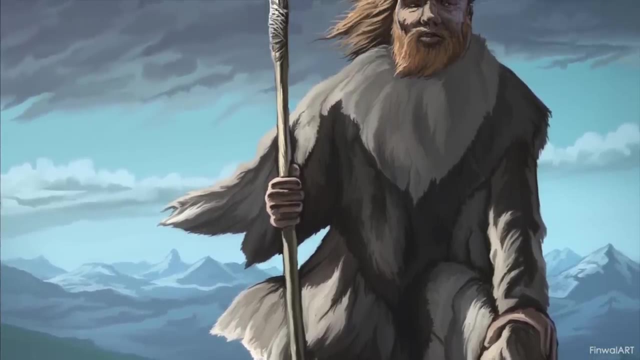 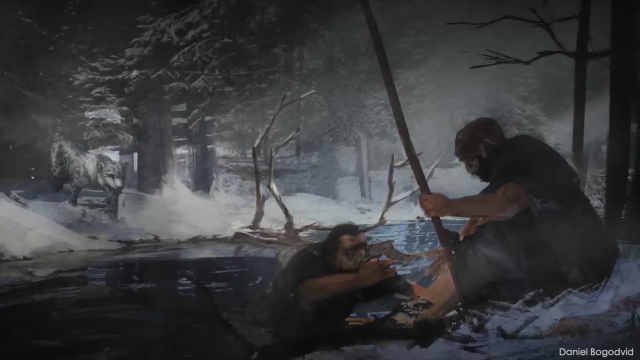 Though, when considering our initial hybridization with Neanderthals, it may have been quite harmful, Due to small populations and inbreeding Neanderthals accumulated several harmful mutations that would eventually be bred out of our populations. Initial hybrids experienced an estimated 94% reduction in 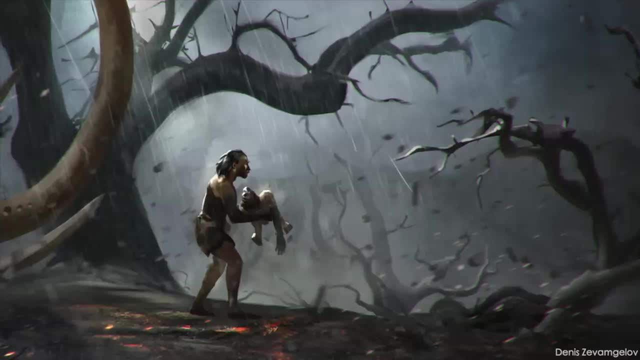 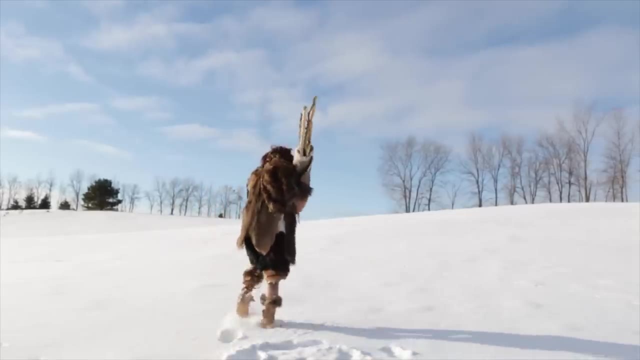 fitness compared to other populations. Many Neanderthal genes were bred out quite quickly, though others appear to have been useful for adapting to the new Eurasian environment. Our species kept Neanderthal genes associated with circadian rhythms due to the darker conditions of. 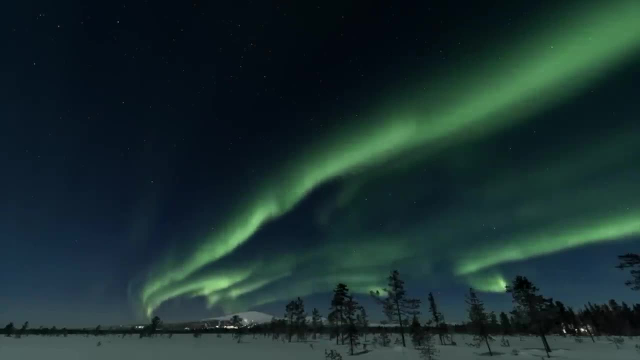 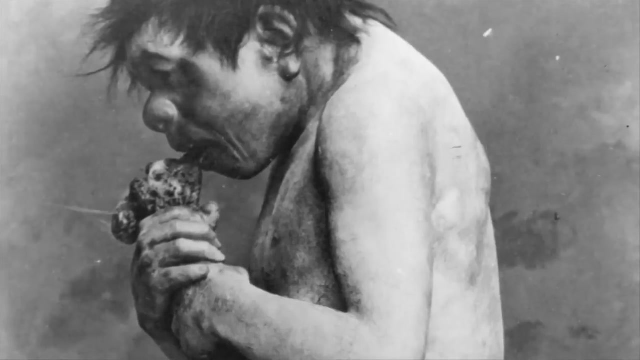 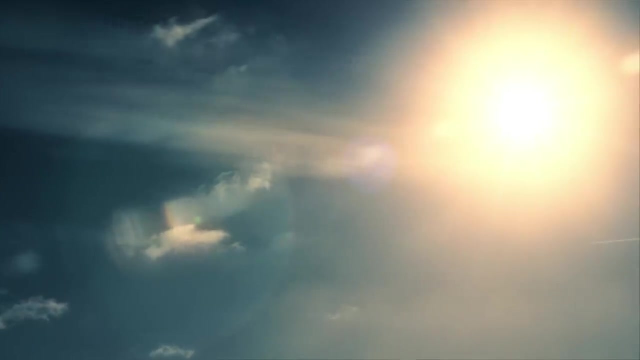 European winters Due to the cold. they also kept genes associated with thermal efficiency and metabolism, Though these genes, which helped starving Neanderthals pull through a long winter, appear to be linked with diabetes in the modern day, Other Neanderthal genes associated with UV radiation. 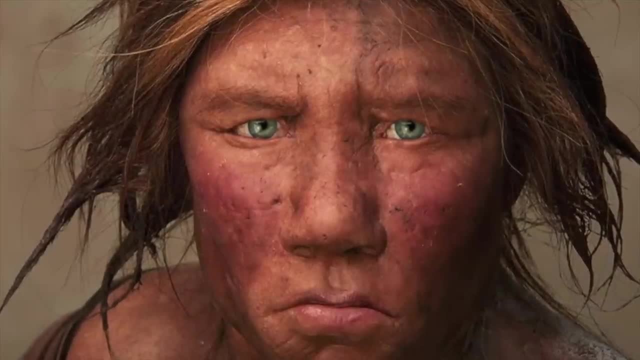 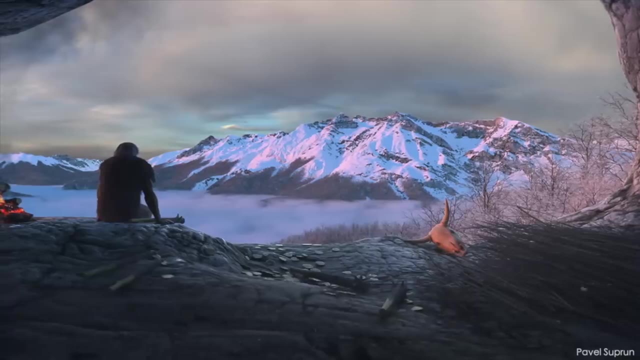 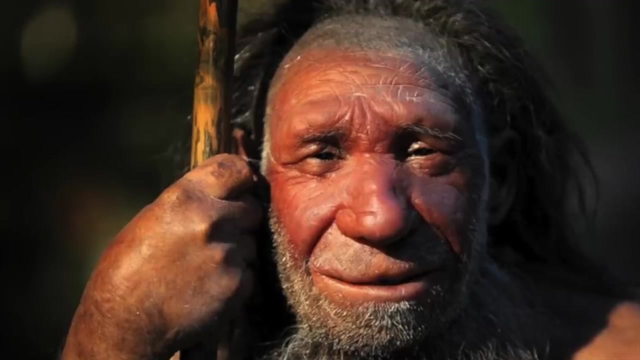 sensitivity and red hair found in some European but mainly Asian populations may have helped us adapt to the generally less intense Eurasian sun. Other Neanderthal genes are associated with depression, digestive problems, blood clotting and miscarriages. Perhaps the most significant way that. 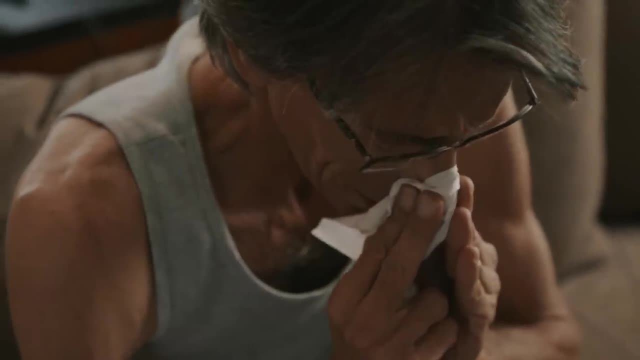 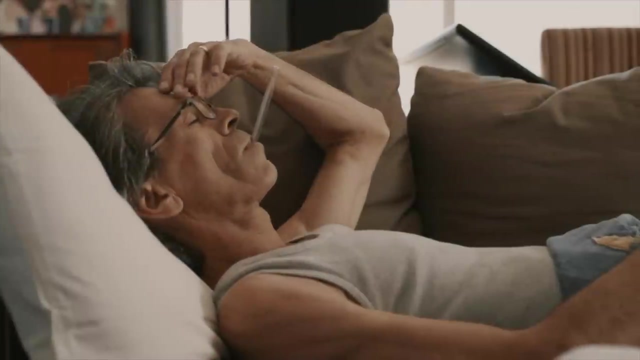 Neanderthal genetics benefits some modern populations is in regards to viral immunity. Between 20-30% of all Neanderthal genes in modern humans are related to the immune system. These genes may have initially helped us adapt to the pathogens found in Europe. 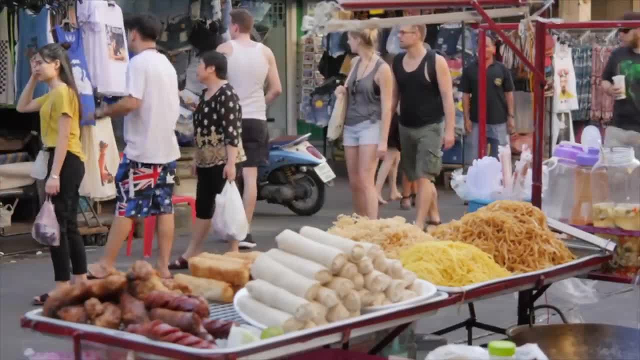 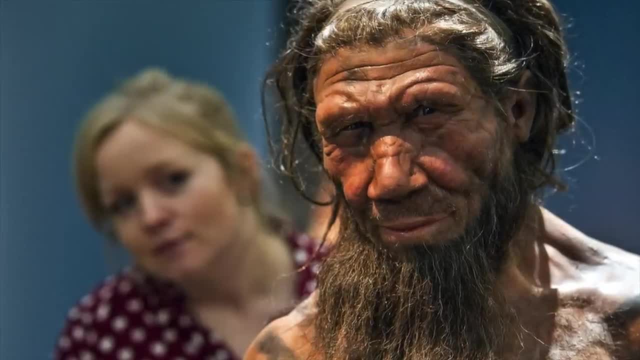 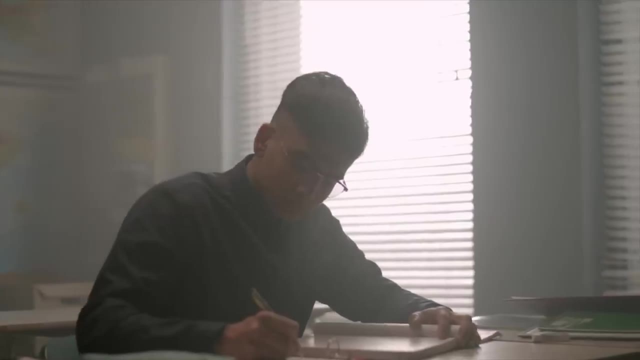 They also still affect modern populations in both good and bad ways. In 2020,, it was found that one chromosomal section from Neanderthals in modern humans may serve as protection against COVID-19, while another may significantly increase its severity. A limited number of Neanderthal genes may affect cognitive function in modern humans. 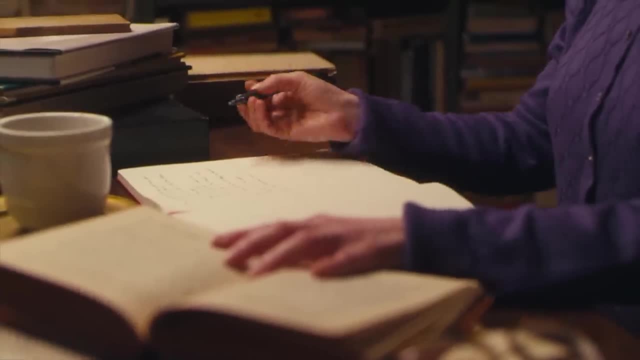 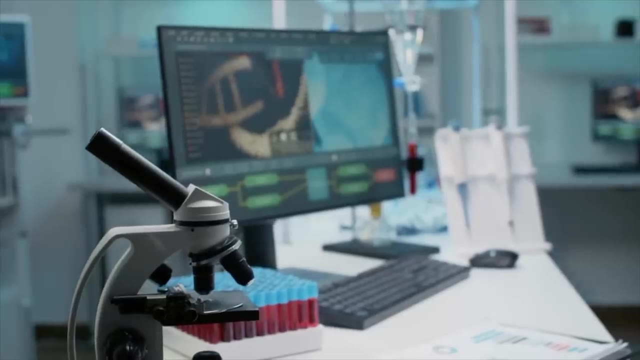 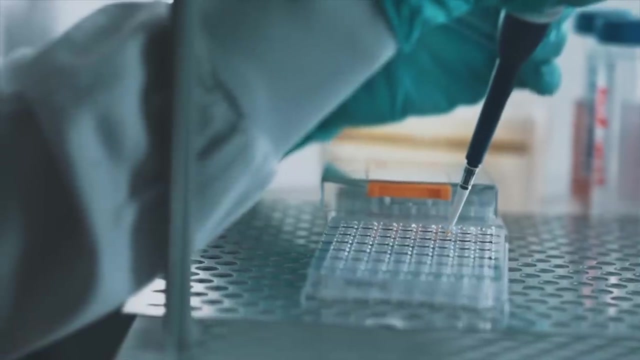 Some may benefit advanced thought process, counting and calculating. Other genes may actually have negative cognitive effects on modern populations. Much of the Neanderthal DNA within the modern human genome has little to no effect on us. It is non-coding DNA, also referred to as junk DNA. 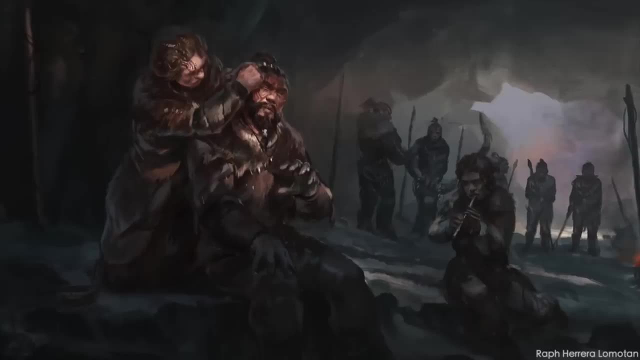 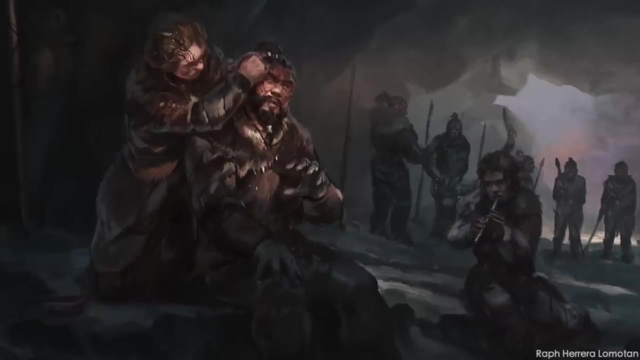 that does not do much. The absence of Neanderthal-derived mtDNA suggests that interbreeding between Neanderthals and sapiens primarily consisted of Neanderthal men and sapien women. This has caused some to assume that these Neanderthal men may have been having unconsensual. 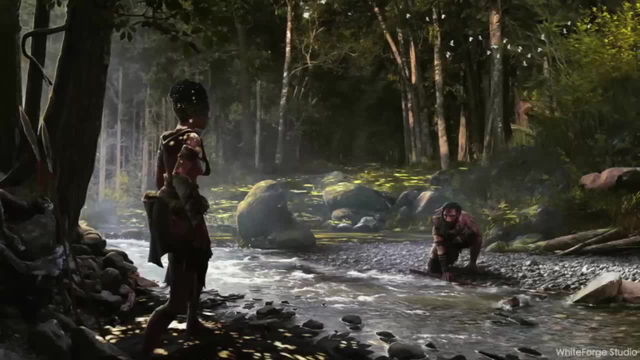 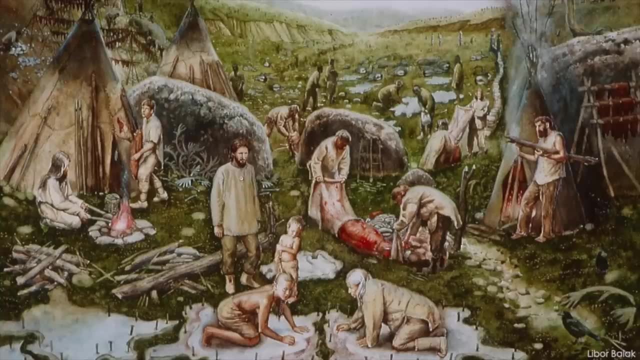 sex with these homo sapien women, and perhaps sapien men had no interest in Neanderthal women, Though other possibilities to explain this do exist. It is possible that couplings between sapien men and Neanderthal women encountered fertility issues. 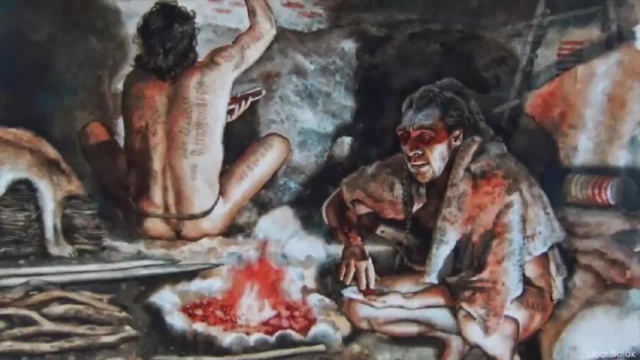 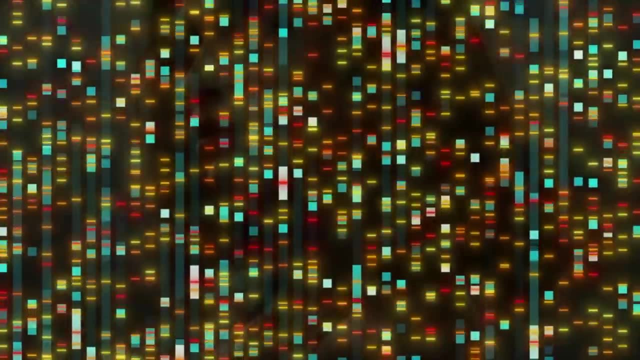 Perhaps these couplings often resulted in miscarriages or the offspring itself was infertile. Additionally, the lack of Neanderthal-derived Y chromosomes, which passed from the father to son, suggests that it was mainly hybrid females that contributed to modern sapien genes. 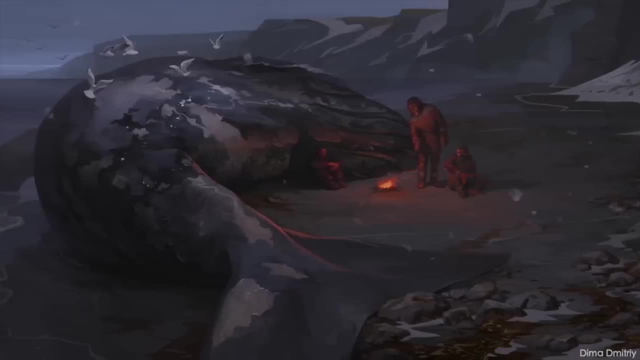 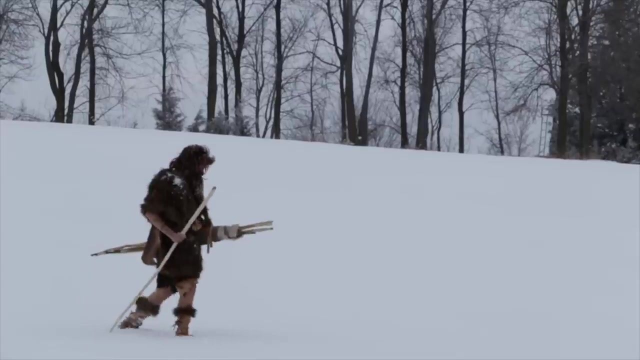 Though we do not entirely understand why these genes passed on this way, the possibility of fertility issues may be evidence that Neanderthals were indeed a distinct genus. While modern humans may have only inherited between 1-3% Neanderthal DNA, it is a significant 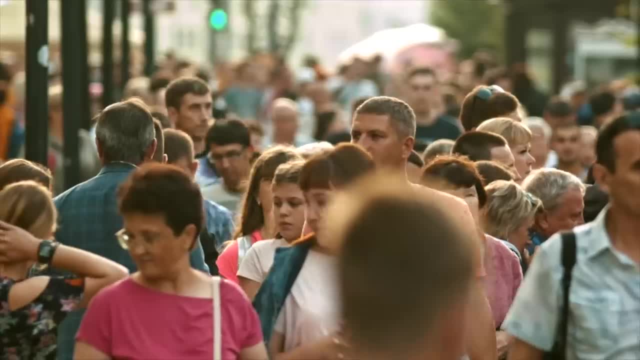 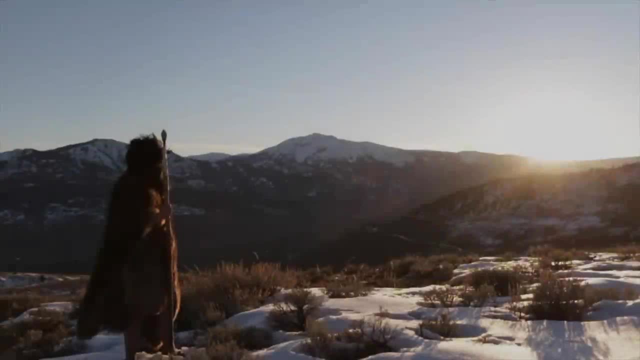 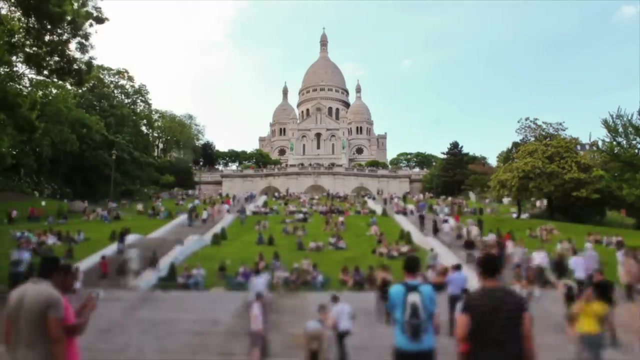 amount, with observable implications. There is no doubt that modern humans are still affected by the genes of our long lost cousins. Though the Neanderthal anatomy may be extinct, there are more Neanderthal genetics passing around modern populations than there ever was in the paleolithic. 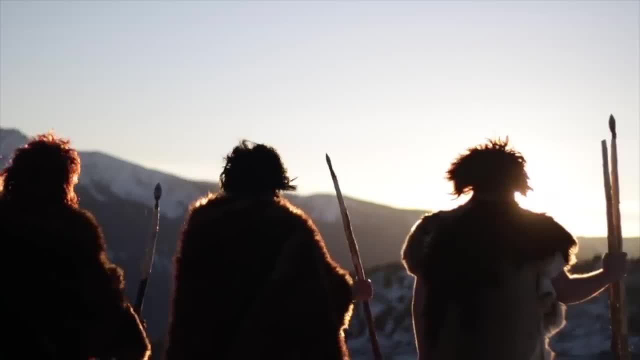 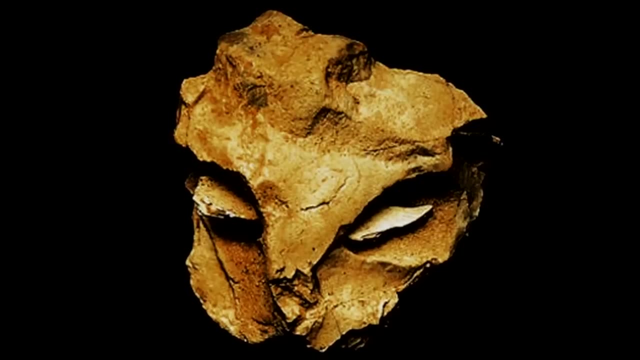 In a way, Neanderthals are more in the nuclear system then they ever were in the actual human species, successful now than ever before. Their legacy lives on with us and they will forever be a part of our story. With wise stones and fortunate fossils. we are given just a miniscule glimpse into the